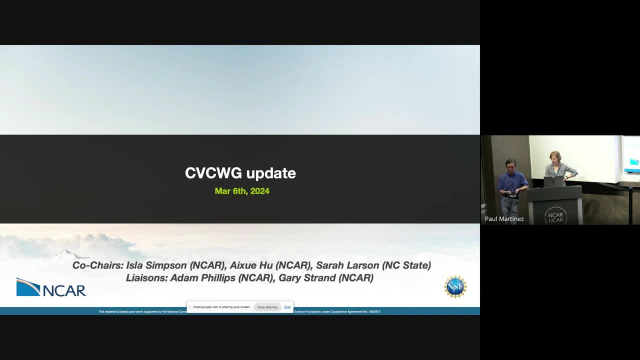 Working Group Meeting. We are the co-chairs. It's Isla, me and Sarah. Today I'm going to turn the morning session, Isla will turn the afternoon session and Sarah she will watch the online part. First of all, I want to make an announcement. 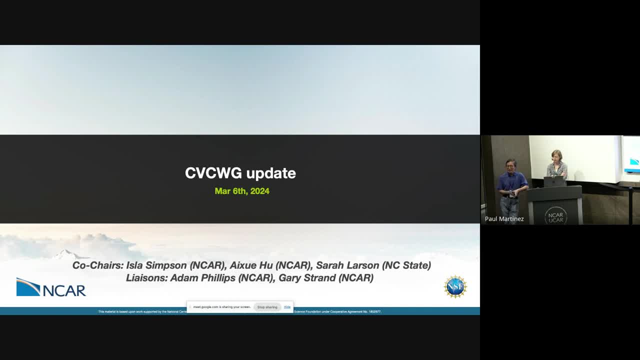 We are organizing a Deer Meal Symposium at the AMS meeting 2025, which is January 2035.. And the symposium will be on Tuesday. We plan to have a whole day symposium and also at 7 pm on Tuesday And a welcome. 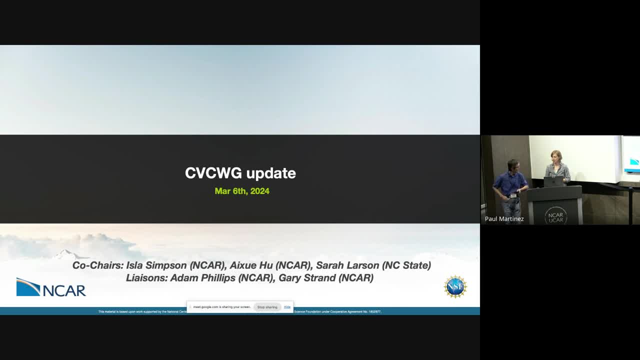 effort to submit your abstracts, And now I'd like to give the activities of the working group a copy. Thanks, So, yeah, thank you all for coming in the room and online. So we're going to kick things off. for the first half an hour We're going to just have some updates of the working group activities. 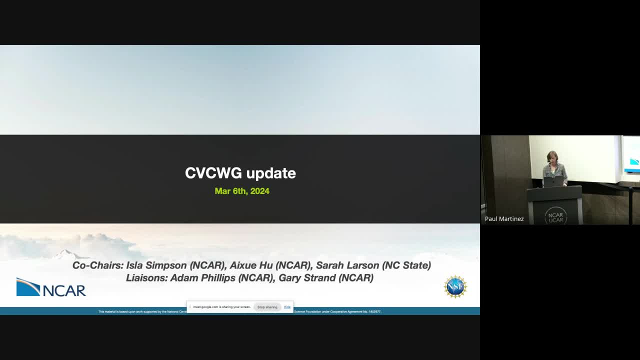 and the plans for the working group moving forward And maybe some time for discussion at the end of that. but we're going to have more time for that. So if you have thoughts and you don't voice them right now, we have plenty of time for that. 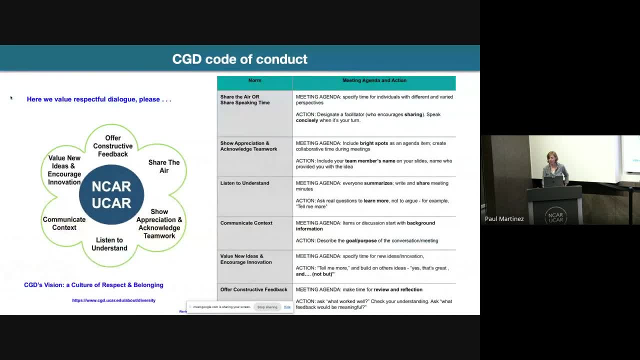 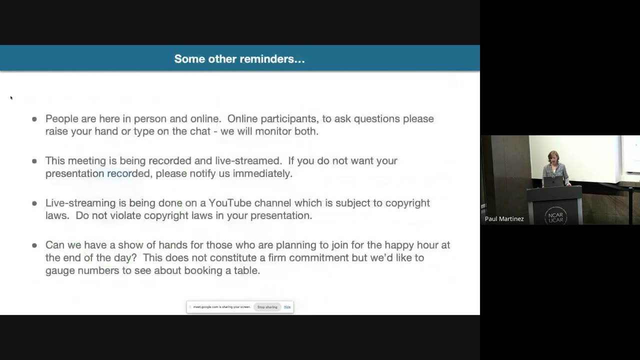 later on. So first of all, this is the CPD code of conduct. Please be respectful to everyone and allow everyone to have their chance to talk and give constructive feedback on all the presentations. So just a few logistical things. We have people online and in person. 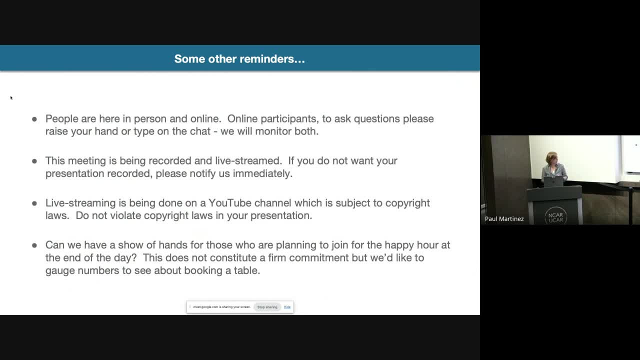 And so for the people online, hopefully you can hear us, And if you have questions, feel free to either raise your hand or post in the chat. We're going to be monitoring online in the room as well. The meeting is being recorded and live streamed on YouTube, So 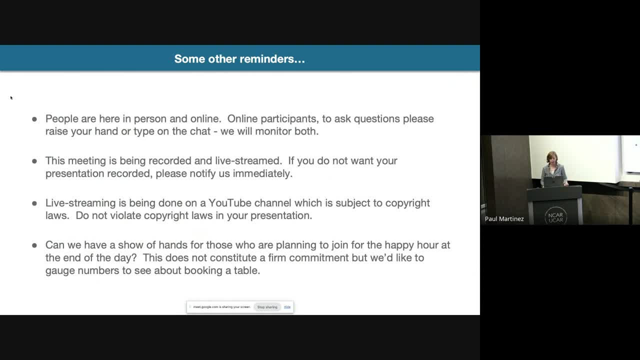 I sent a message to the speakers. if you don't want your talk recorded, please let us know immediately, because I think it's a little hard to change kind of on the fly And make sure you don't uh in any in your presentations, um, because that i think youtube doesn't like that, um, and if you 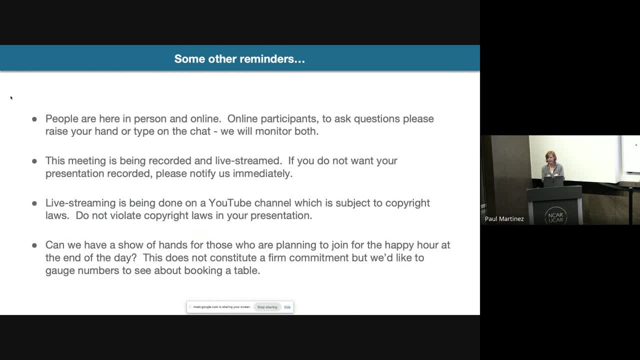 want to make any last minute changes to your presentations. we have the ones that have been uploaded so far here, so let me know if you do make any changes, kind of over the course of the day. uh, we are planning to go down to under the sun at the end of the day for a happy hour and i'm just 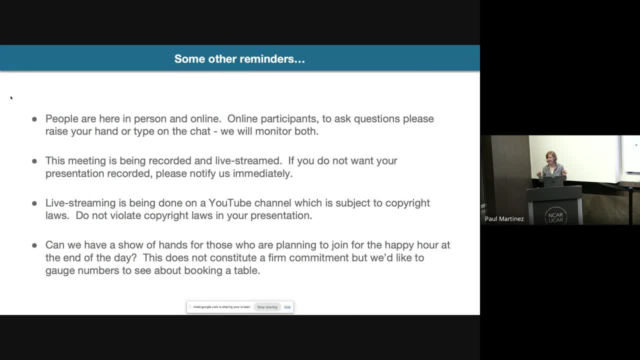 wondering who is interested in that. this is not a not a firm commitment, but just we might try and book a table. so we've got one, two, three, okay, at least enough to warrant booking the table. so i'll try and do that at lunchtime. uh, i feel like there were other things i wanted to mention that weren't 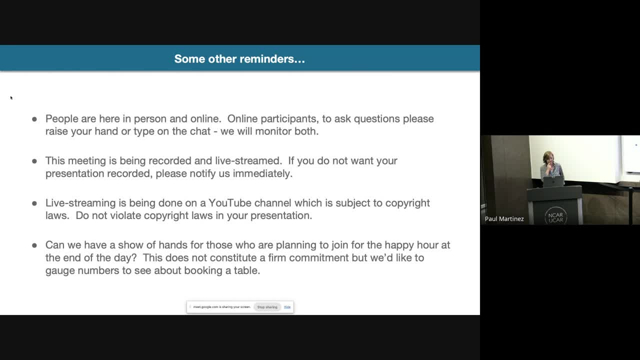 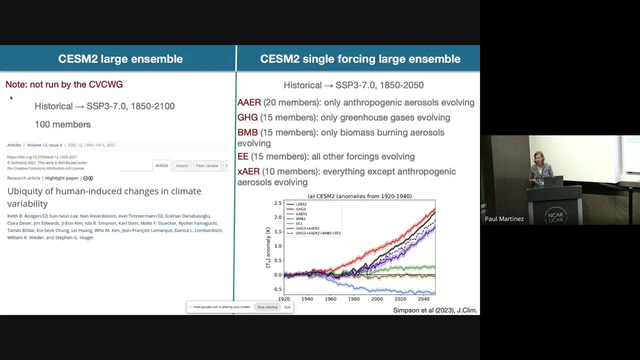 on here, but maybe i've mentioned them already or maybe they'll come back to me. i have a question, oh yeah, um, about copyright laws. yeah, can i you include figures from other papers if they're properly cited? yeah, yeah, okay, that's fine. thanks, making sure, okay. so some of you maybe are not familiar with the working group and all its activities, so i 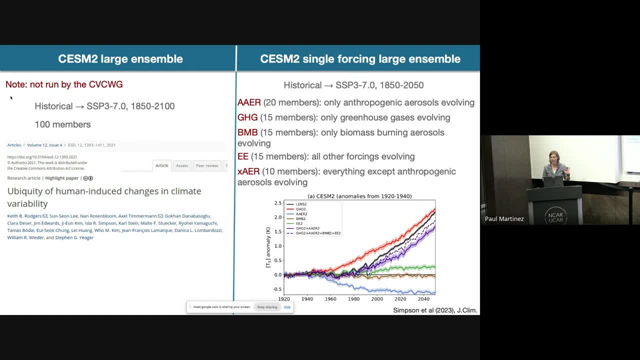 just want to, before we mention all the new things that have happened, mention a couple of big data sets. these are not new, but these are big data that are kind of available for everyone to use. so there's the csm2 um. i'll share a little bit about the working group. um, the working group is the large ensemble. this was. 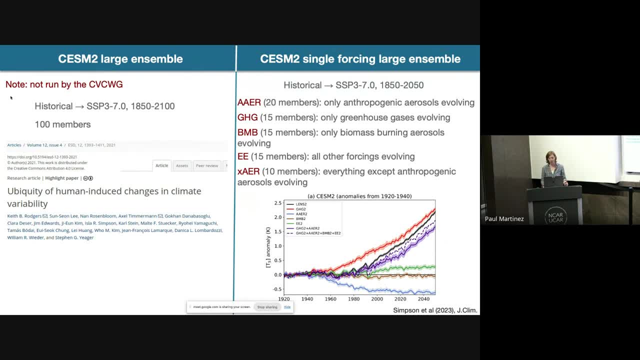 not run by the working group but it was many of the working group members participated in that and so this was run in collaboration with the group and ibs in tucson and the sides korea. and so this is a hundred member ensemble of simulations with csm2 that are run over the historical period from: 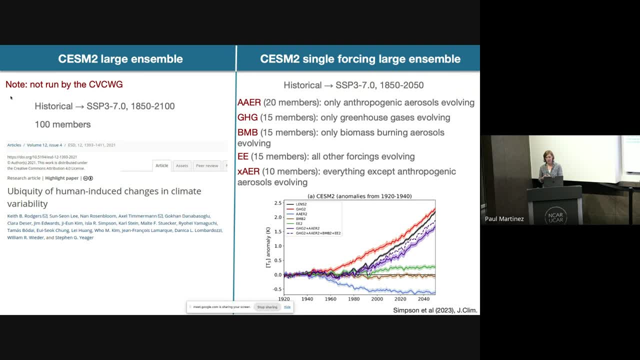 1850 to 2014 and then it into the uh ssp370 scenario period up to 2100.. so that's a resource that the. If you go on the Climate Variability and Change Working Group web page, the information is there. 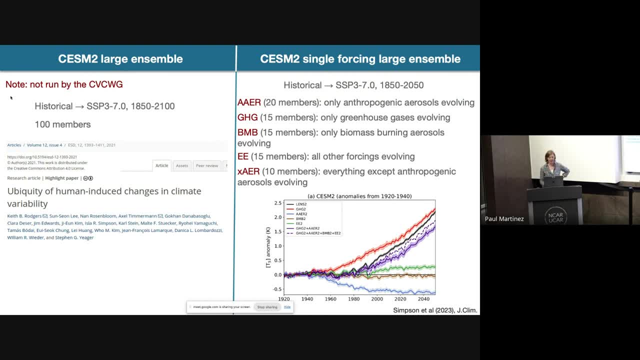 You can just Google Climate Variability and Change Working Group, CSM, and it should come up. In addition to that on the right is a data set that was produced. the paper came out last year. It's kind of complementary to the large ensemble, but it's a single forcing large ensemble. 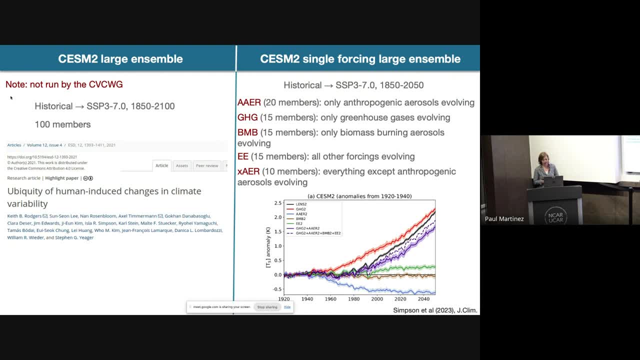 So these are smaller ensembles of 15-ish members each, where you can decompose the influence of all the forcings in the large ensemble into the contributions from anthropogenic aerosols, greenhouse gases, biomass, burning aerosols, and then everything else. 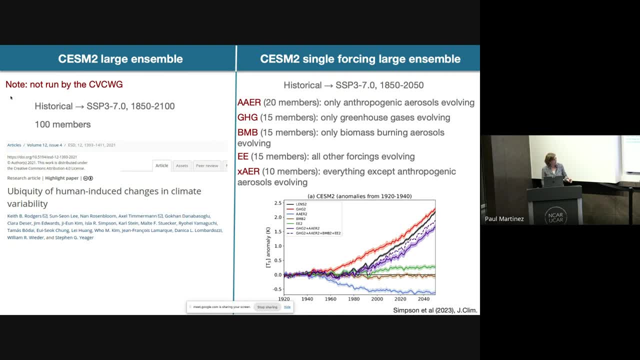 So you can kind of sum up the contributions. We also have an everything except aerosol ensemble because we find there were pretty big monolinearities in the response to aerosol forcing and it matters what met the need. So, just in case you were not aware, these two big data sets are there and available. 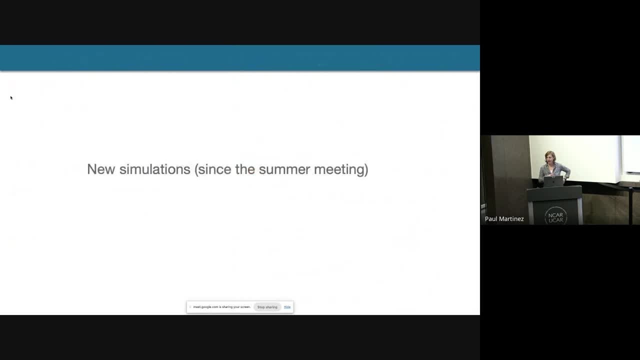 for everyone to use. So now we'll move on to kind of the newer stuff, the things that have happened since the last update, which was during the summer thing, So one thing that I'm pretty excited about, but I haven't really had a chance to look. 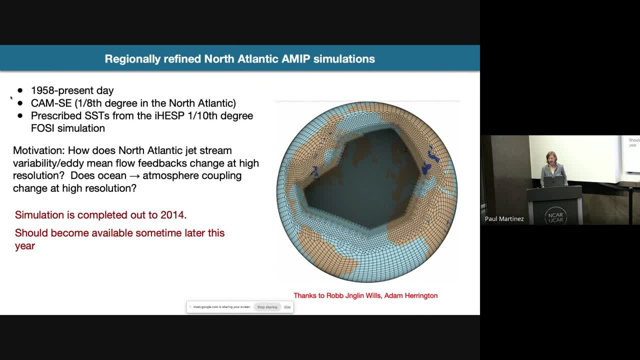 at yet is this regionally refined North Atlantic AMIP simulation. So this is using the CAM Spectral Element Dynamical Core to do regional refinement. Oh, I just remembered one of the things I wanted to say at the beginning about the laser pointer. 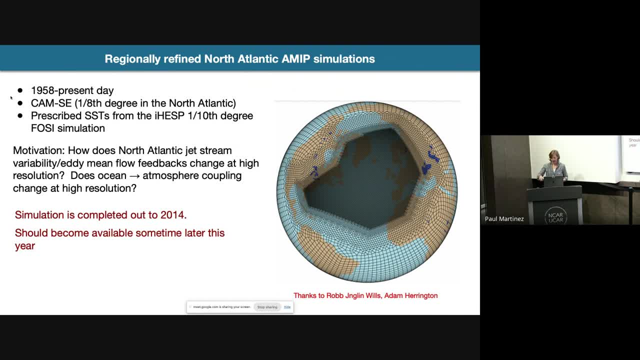 So for the speakers, there is a laser pointer here and I think, if you like, hold it down long enough. Oh, it's there. Okay, Yeah, it works. So this is going from one degree everywhere, except it's regionally refined down to one. 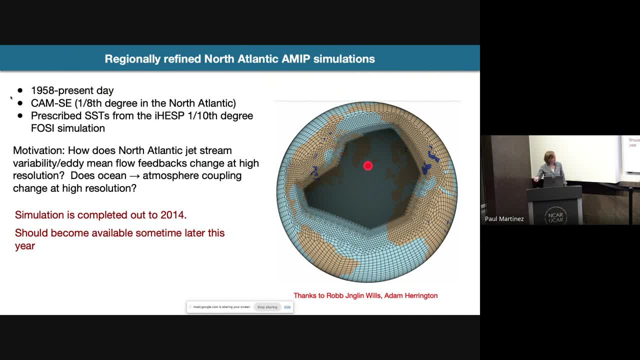 eighth degree in the North Atlantic region, And so the motivation here is that there's kind of growing body of evidence that we don't get jet stream variability in the North Atlantic right and that resolution might matter for ocean-atmosphere coupling. And so this simulation goes from the late 1950s to present day. 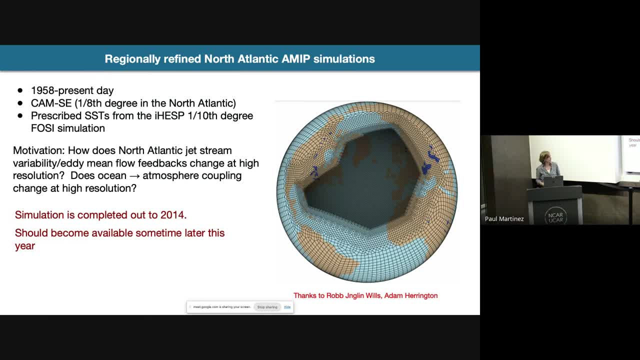 It's out to 2014 at this point, which is the end of the historical period. So this is using sea surface temperatures taken from a one tenth degree forced ocean sea ice simulation, So using the ocean and the sea ice models, offline, Of course, with observed meteorology, and what that means is that we can get high resolution. 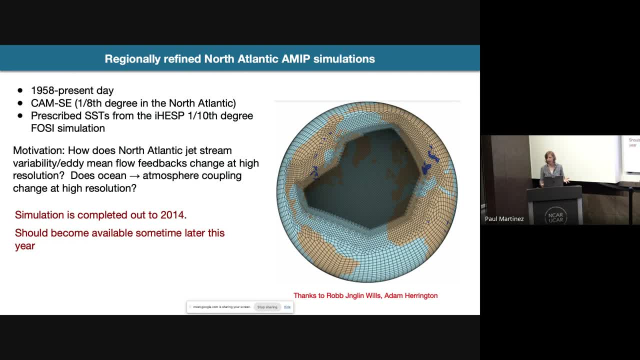 SST variability, higher resolution than we really have in the observations over this time period, But it's still kind of following the observed low frequency Atlantic multi-decadal variability. So we're going to start looking at this, hopefully soon, and come up with a description paper. 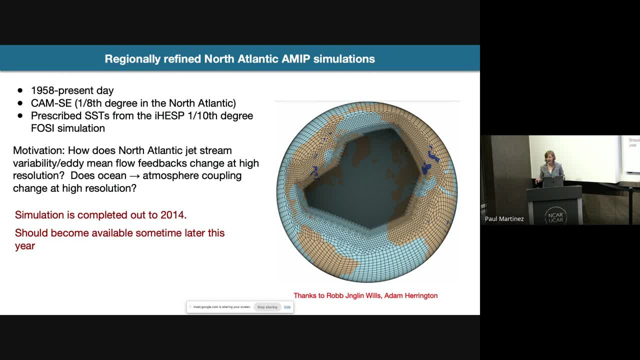 and try and make this data available. The goal is sometime by the end of this year, But it really depends on how thick it is. It really depends on how things go, But this should be a pretty useful data set for anyone who wants to look at high resolution. 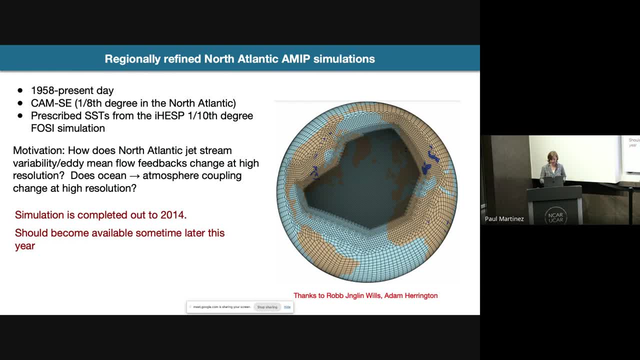 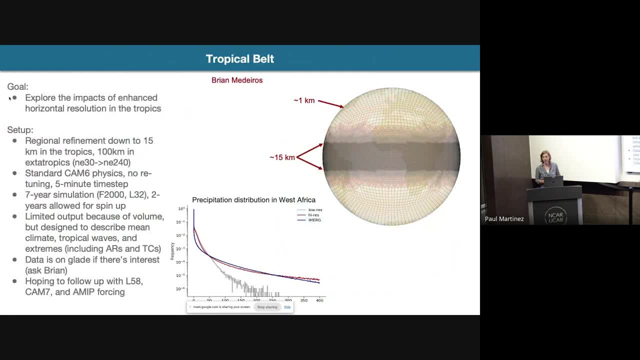 features in the North Atlantic over the full historical record. Sticking with the theme of regional refinement, Brian Medeiros has been doing this tropical belt simulation, which is a similar idea. So there's one degree resolution and then regionally refined into. about that should. 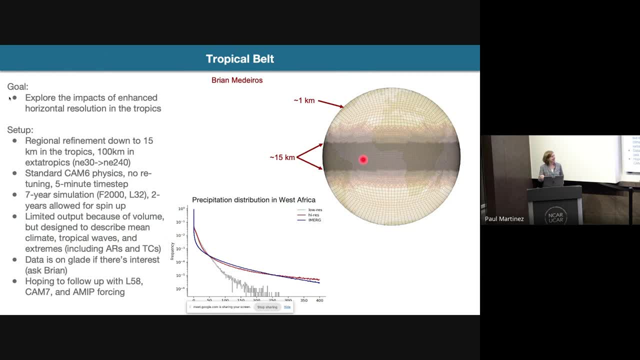 not be one kilometer. That should be 100.. It's regionally refined into 15 kilometers in the tropics. These are pretty short runs, but they're long enough. I think there's basically seven years and two years of spin-ups, but five years in which. 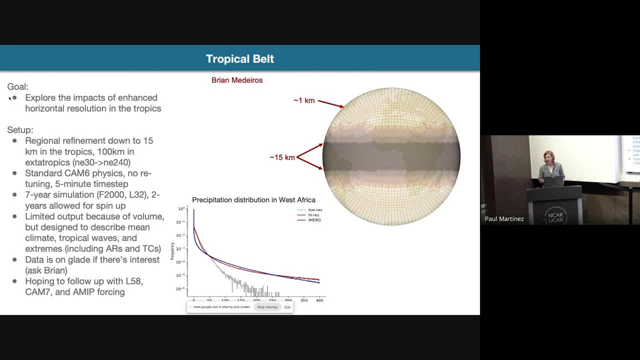 to look at things like tropical waves and see how they depend on resolution, And the figure here is showing the precipitation distribution in this run. So the gray is the low-res model, The blue is the observation And then the red is the regionally refined model. 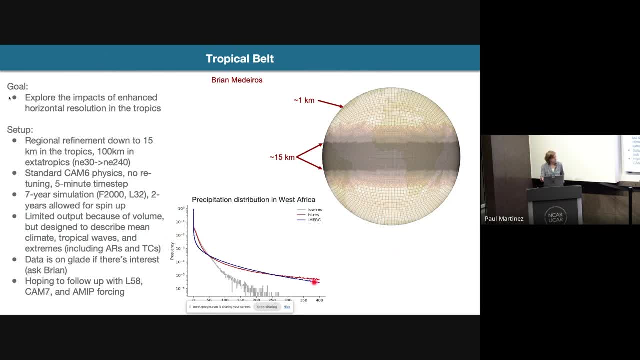 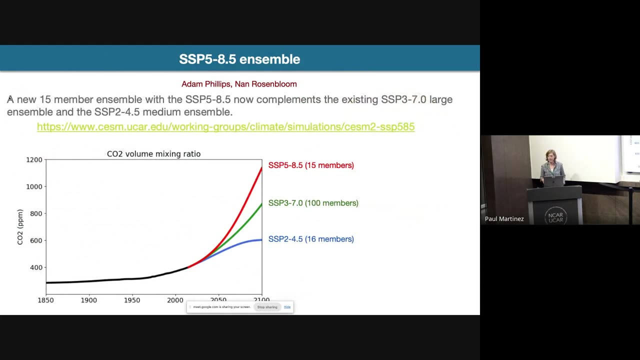 And so you can see that you're- as you might expect you're- doing a much better job at capturing the precipitation distribution over West Africa here, particularly in the high intensity precipitation rate. A new ensemble that's been available now since the last meeting is an SSP 585 ensemble. 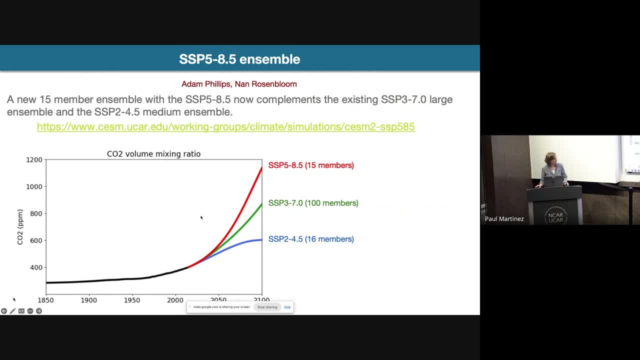 So the large ensemble was using the SSP 370 scenario. We had previously run an SSP 245 media ensemble of 16 members And now we have an SSP 585 ensemble of 15 members. So we can span this range of scenarios and you can look at how the scenario impacts future. 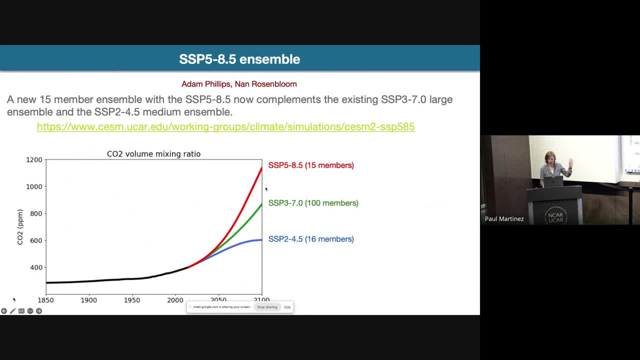 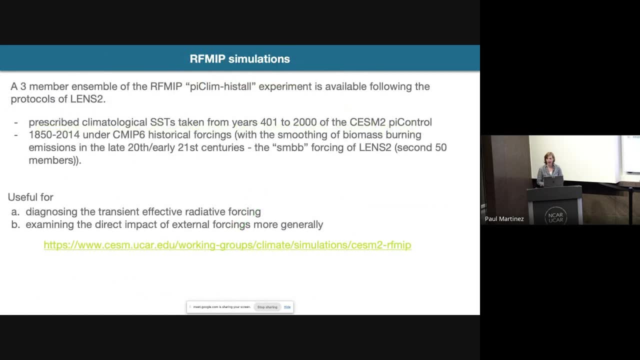 projections across these ensembles And again go to the work and group webpage to find out how to access those. We've also run an RSMIC type simulation. So this is basically following the process, Following the protocols of the EI-CLEM-HIST-ALL experiment of CMIP6. 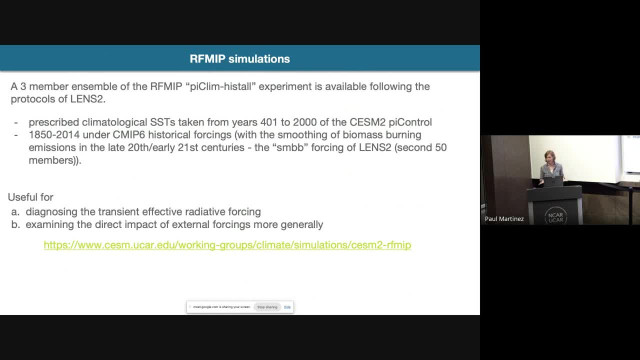 So this is where you run with prescribed climatological sea surface temperatures from the pre-industrial control And then you run with only the external forcings. So you can look at the direct impact of the external forcings absent any SST changes. So this is useful for if you want to diagnose a transient effect of radiated forcing or 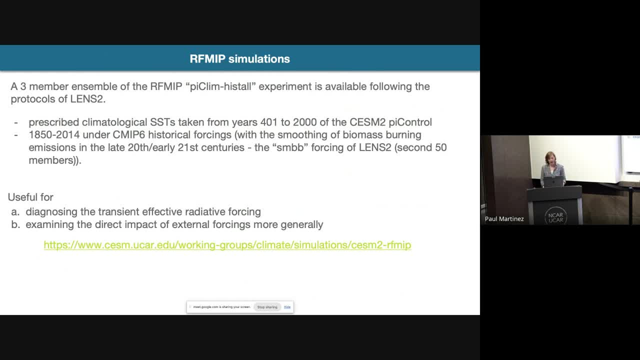 just look at what is the direct impact. So the forcings, And this is run with forcings analogous to the second 50 members of the large ensemble. So if you want to diagnose the radiated forcing in the large ensemble, this is run. there's. 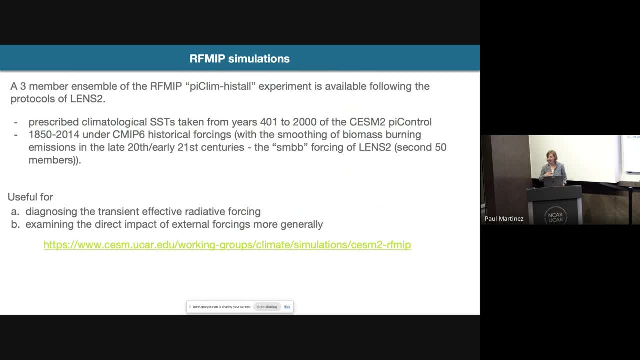 three members that run over the historical period And we may run- I know you is interested in this running single forcing versions of this or scenario versions of this, And so keep that in mind for the discussion if there are ones of those that you're particularly. 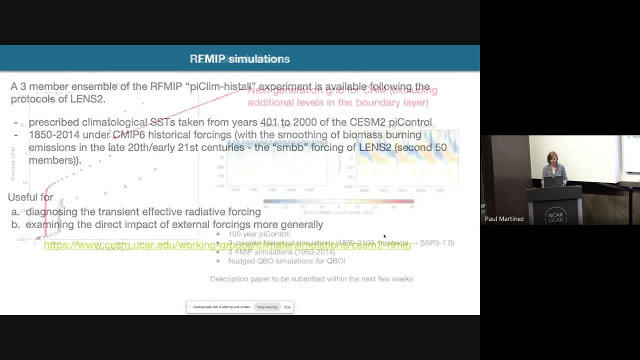 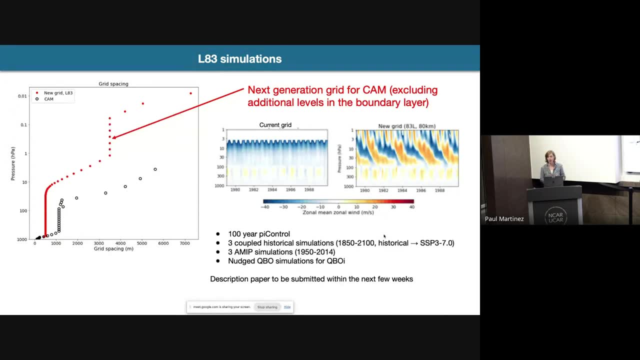 interested in. We'd like to hear about that. Another set of simulations is using this new vertical grid, So CAM is going to go to higher vertical resolution in CESM3.. So what you're seeing here is the grid spacing on the X axis and then the height of the model. 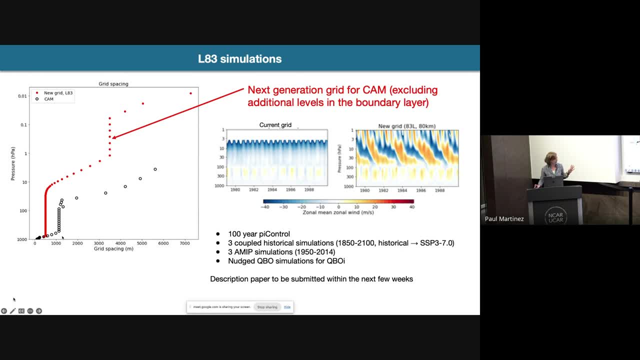 in the Y axis. So the black points here are the current CAM grid- The model top is at 40 kilometers and the resolution here in the troposphere and lower stratosphere. So that's about 1,100 meters. And the new grid is going to go to 80 kilometers and has a resolution here of 500 meters. 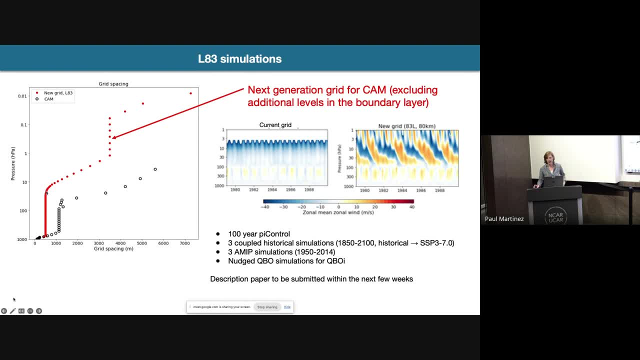 And what that means is that we can now represent the quasi-biennial oscillation of zonal mean zonal wind in the equatorial stratosphere. So this is what CAM looks like. in equatorial zonal mean zonal winds, There's no QBO. 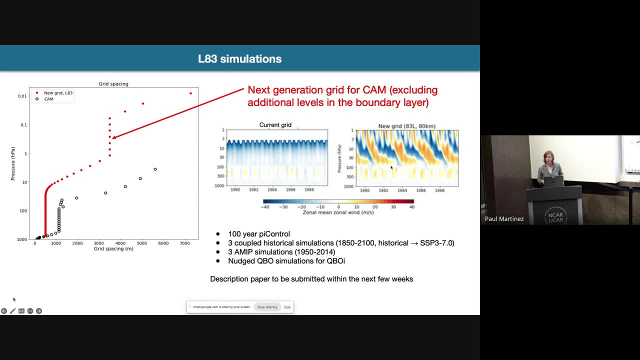 And this is what this new vertical grid looks like. So we can now explore what is the impact of that on climate variability, And this has a better representation of the polar velocities as well, which I think people have shown matter for things like ENSO teleconnections. 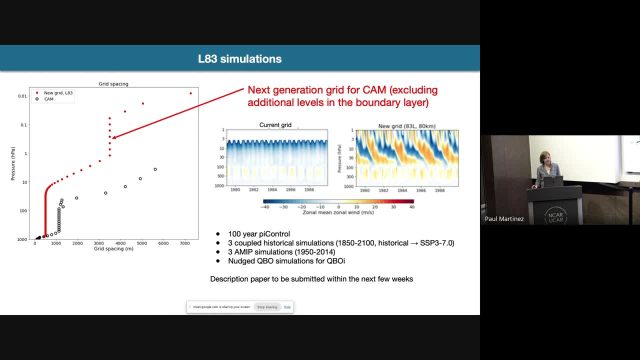 So we have a suite of simulations which are using this enhanced vertical resolution, So everything else is the same. The next version of CAM is also going to change the resolution in the boundary layer, but we haven't changed it, Because when you do that, you have to change all of this. 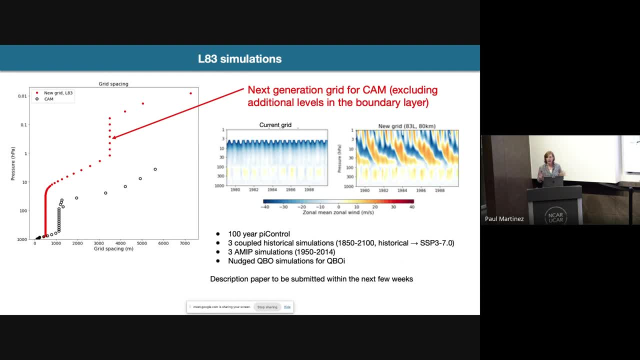 And then you have to change the tuning and the physics. So really everything else is the same except the grid here, And we have pre-industrial control, three coupled simulations over the historical period that go to the end of the 21st century under the same forcings as the large ensemble, and 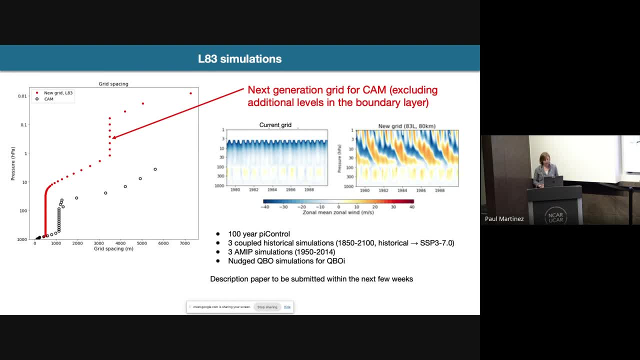 three AMEB simulations And, if you're really into the QBO, there's also some nudged QBO simulations that were run for the QBO Intercomparison Project, where the QBO is being nudged towards observations Despite the fact that we now have our own beautiful QBO in these simulations. 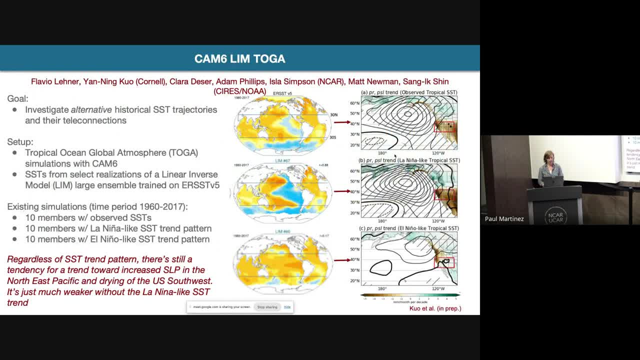 There's also been some work going on with our collaborators at Cornell, So Flavio Lehner and Yanen Kuo are leading this project And they've run a suite of TOGA-type simulations. This is where you're time-varying sea surface temperatures. in the tropics you have climatological 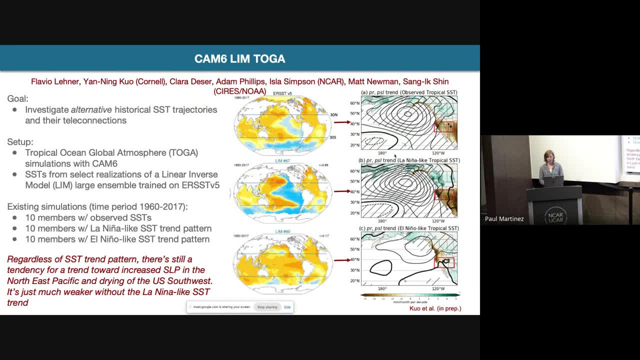 sea surface temperatures in the edges And normally we just do this with observed sea surface temperatures. But they've been investigating what could have happened in the past if we had had a different realization of internal variability. So some of the sea surface temperature evolution we've seen is forced, some of it is internal. 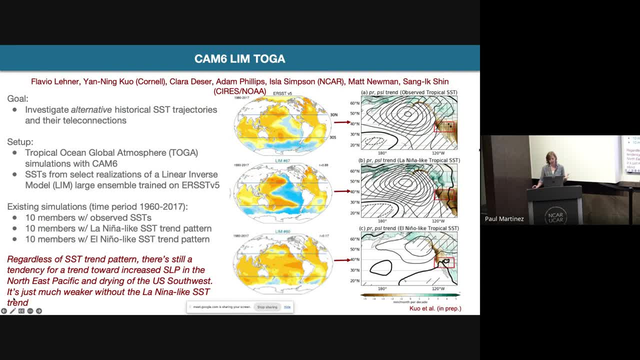 And they've been using SST variability from a linear inverse model to look at different potential histories that could have happened. So the one on the top Here is the observations. This is kind of extreme La Nina trend scenario And then this is a more of an El Nino-like scenario. 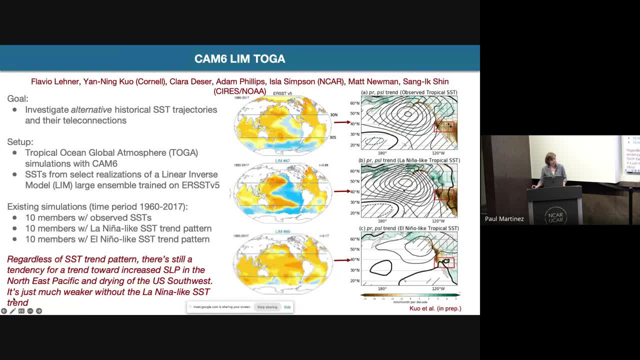 And so they're looking at the connections to the extratropics and in particular to precipitation over the Western US. And so it's been argued in the past that this kind of La Nina-like trend of the observations has been leading to this drying over the Western US. 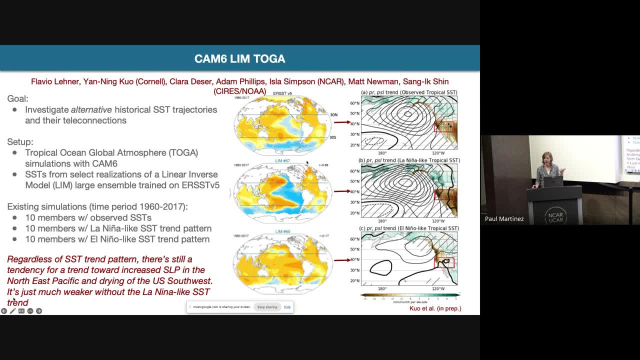 And these experiments suggest that if we had a different realization of internal variability, that could have been more severe if we had a La Nina-type trend. But interestingly, even if you have the kind of extreme El Nino trend due to internal variability, 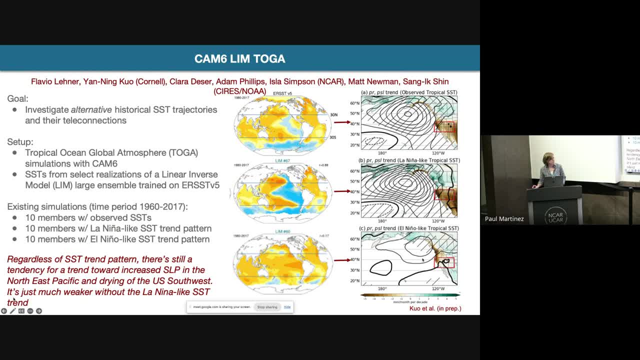 you still end up with this anomalous high pressure over the Northwest Pacific and the drying over the American West. So it's kind of like No matter what the internal variability would have done, there's kind of a sense that the sea surface temperatures wanted to force drying over the American West. 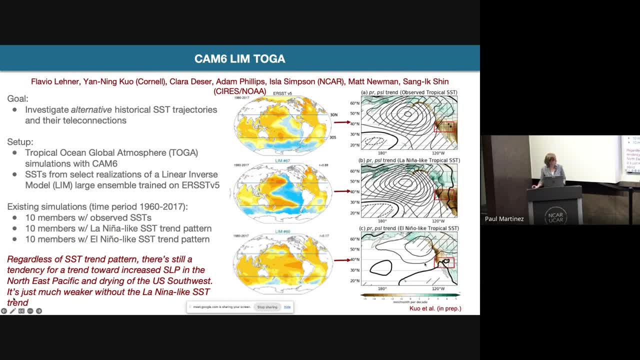 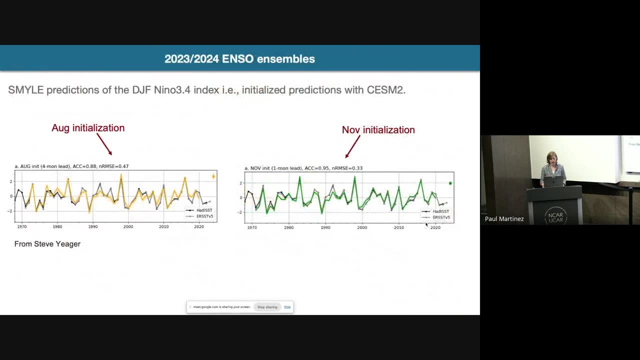 And they're trying to figure out exactly why you get that. in this bottom case. It's not totally obvious, But it also shows that if we had had different internal variability we could have had pretty different overall trends in the hydroclimate of the Western US. 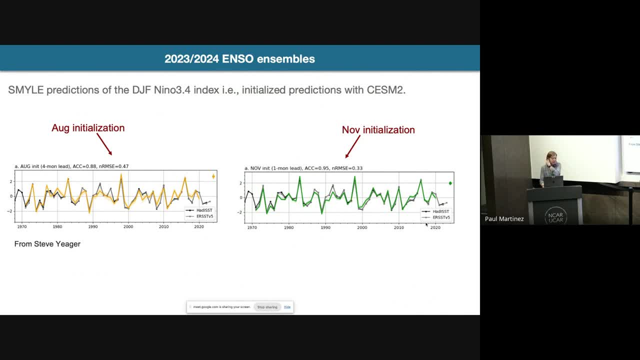 If you were at the seminar yesterday, you might have seen a lot of the data that we have. And if you were at the seminar yesterday that was part of the Earth System Prediction Working Group, you would have heard Clara talking about this. With the Working Group resources, there's been these large ensembles run of the 2023-2024. 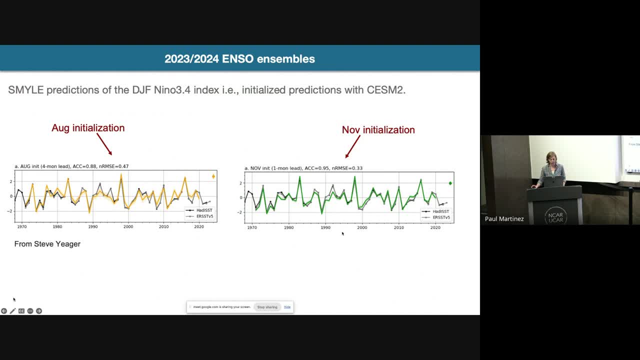 El Nino event. So these are some figures from Steve showing the predictions of this year's El Nino, with the initialized predictions with CSM, which we're calling SMILE for single to multiyear large ensemble. That's what that study is. 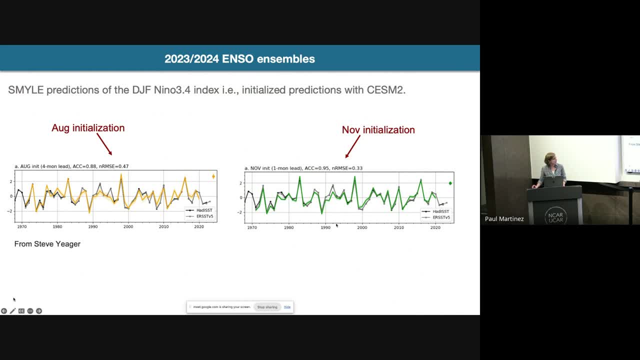 That's what it stands for. These are the August initializations and these are the November initializations, And what you see is that, over the historical period, CSM2 does a really good job of predicting the wintertime. ENSO index. 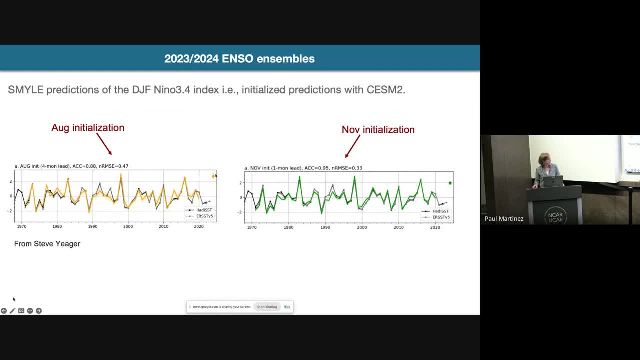 And so back in August Steve noticed that there was this prediction of a very strong El Nino, kind of as strong as the 1997-98 El Nino. By the November initialization that had gone down a bit, But it's still a pretty strong El Nino. 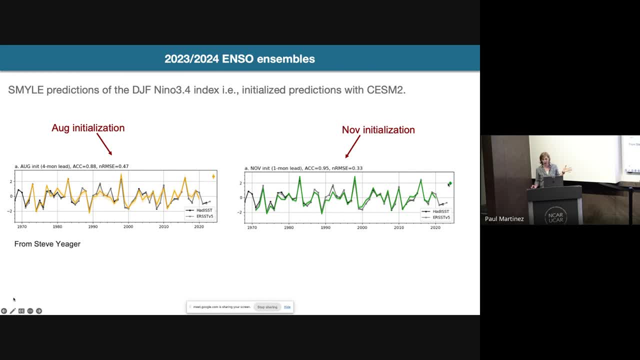 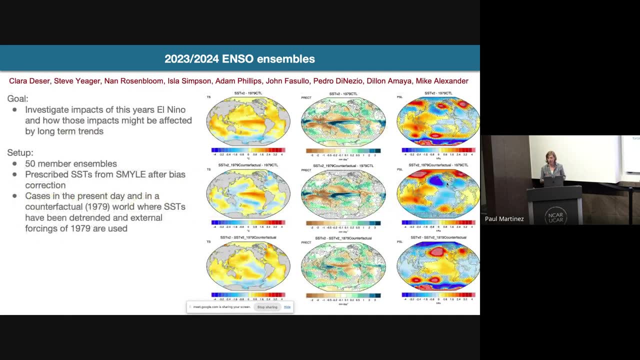 But it's still a pretty big El Nino, and this has verified pretty well against observations. And so, then, what Clara has been doing is been running ensembles with this El Nino event, with the sea surface temperatures taken from those initialized predictions after some bias. 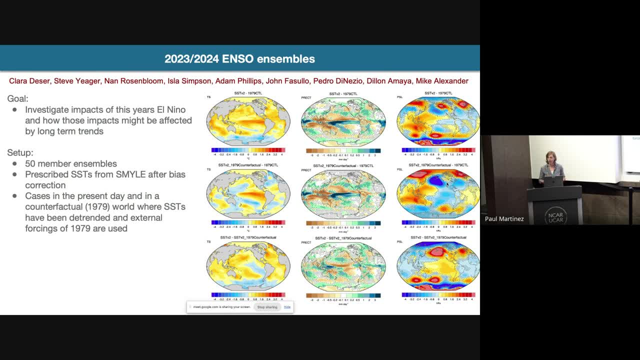 correction. So running kind of 50-member large ensembles of this one event, you can kind of get a sense of what are the uncertainties in the ENSO telecast, The ENSO teleconnections associated with the event, and she's also been running these counterfactual. 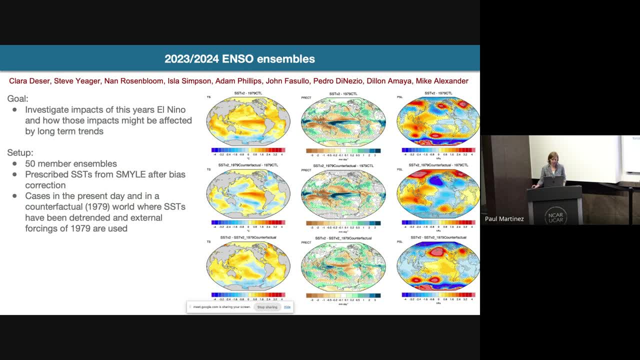 cases under different climate kind of time periods. So on the top there what you see are the sea surface temperature precipitation and sea level pressure anomalies for the 2023-2024 ensemble case And in the middle is kind of a counterfactual case which is run under 1979: radiative forcings. 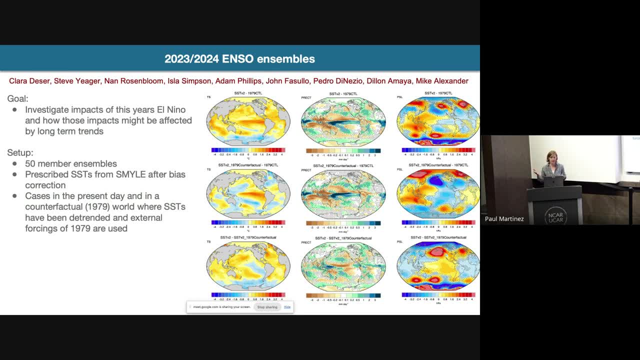 and also has the data And in the middle has the trend from 1979 to now removed. We don't know whether that trend is forced or internal. It's probably a bit of both. So not trying to make any claims about that, but trying to see how has the kind of evolution? 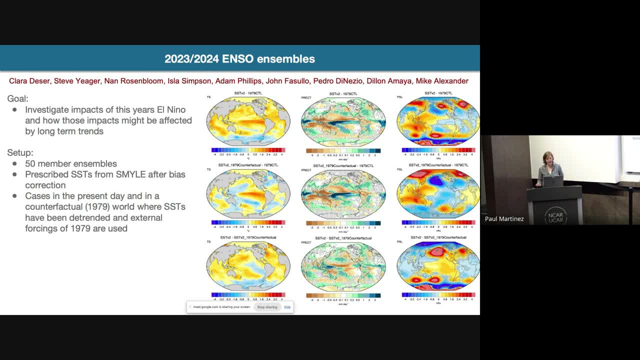 over the historical record changed how we might experience the anomalies due to an event like the one we're experiencing right now, And the difference between them is on the bottom and you can see that the differences are pretty large. Changes in the sea surface temperature, mean state and the radiative forcings have contributed. 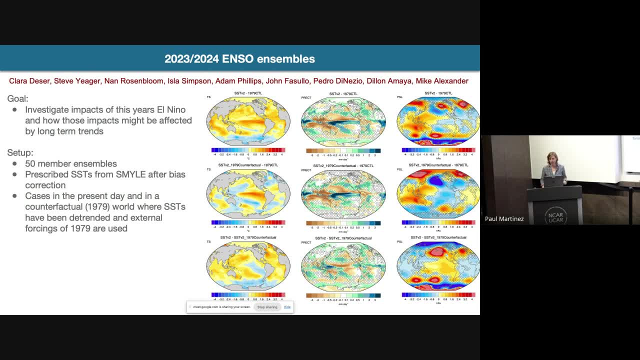 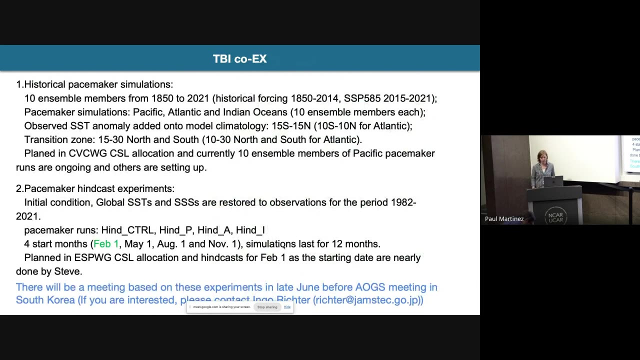 to changing how we experience an El Nino event like the one we're experiencing now, and they're working to try and understand exactly the origins of those changes, at least as similarly advised models. Okay, I'm going to hand over to Aishu to describe the next couple of slides. 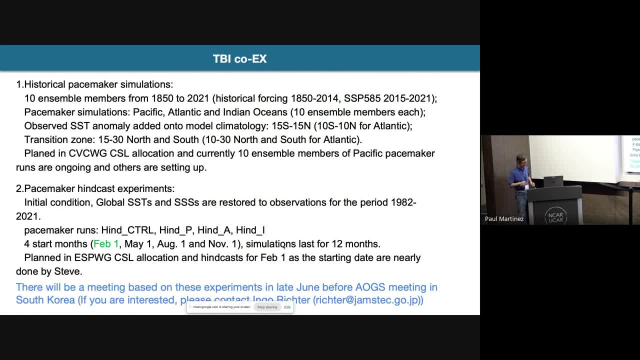 Okay, Before I started I forgot to mention that the first word announcement with that wave outlined in the theory of the model wave. that means Yilumi Yaga Gokhantha and Xiangbing Xie from TRIPS and Teo Bader from DOE Lab and Antonieta from NOLA. 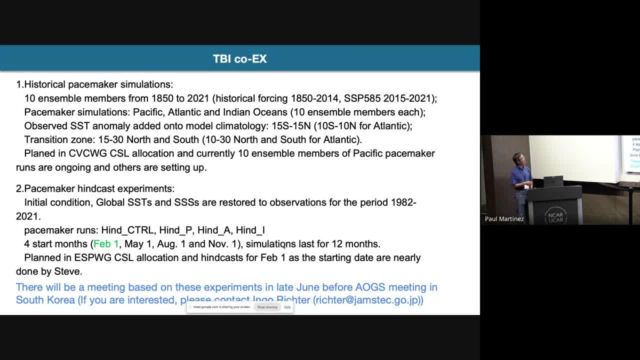 Here I talk about this topical-based interaction project. This is a very interesting project. Okay, All right. So we have a research focus and talk about the interaction between deep and tropical ocean visits And right now the experiment design is basically has been agreed on and we'll carry out this. 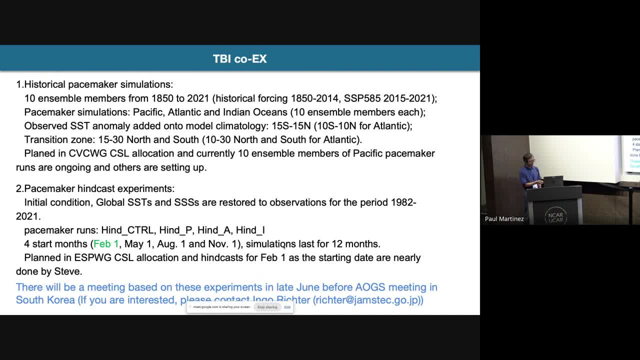 experiment For CBCWT working group. we are doing the first part, the historical. We're going to attend some members from, I think, the rest of the group And right now we run it from 1880 to 2031, because we don't have the proper research. 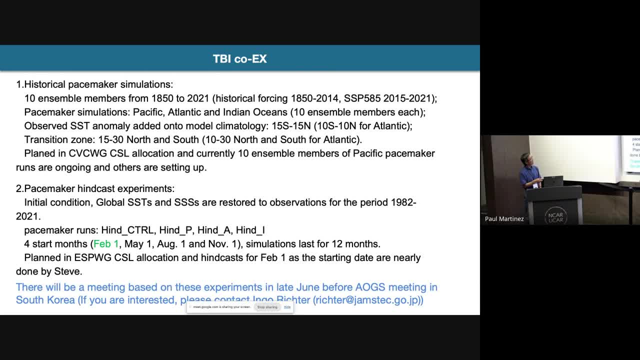 files for the earlier years And we have run 10 and several members from Pacific Peacemaker Simulation. They are ongoing and I think we are finished. I need to confirm this with them And for other peacemaker simulations. right now it is setting up. 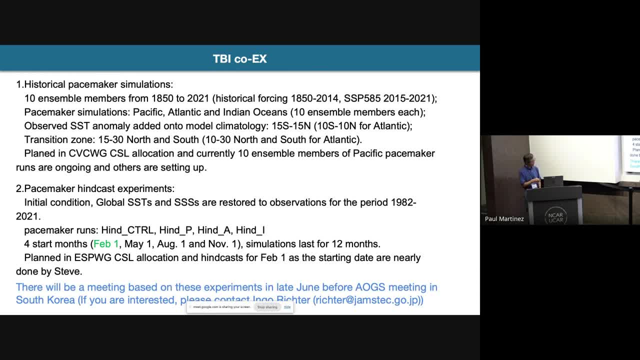 Hopefully we will get it done in next few months And for the Peacemaker Handcraft Simulation, we're going to have 10 and several members from Pacific Peacemaker Simulation. They are ongoing. We're going to have 10 and several members from Pacific Peacemaker Simulation. 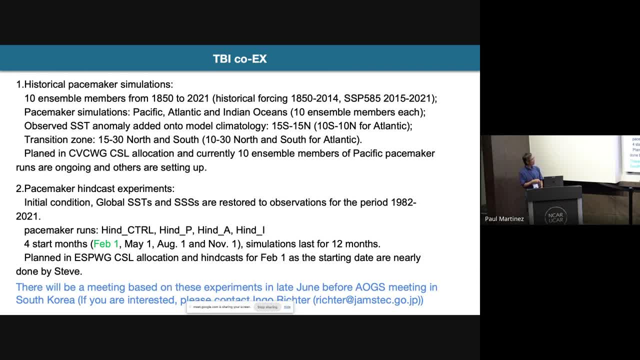 And for the PACAS experiment, which is by the Earth System Prediction Group, which is by Steve, and Those simulations they have, The February 1st one has been finished and Steve is working on to read the papers. After that the data can be released. 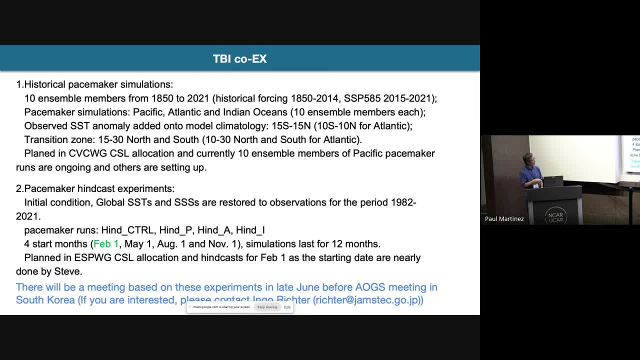 And before the AOisko meeting in late June there will be meeting about about TBI. I think it will be two or three days meeting. so if anybody is interested in the TBI experiment or interested in the travel-based interaction with them, and contact the Ingo Richter to join that meeting. 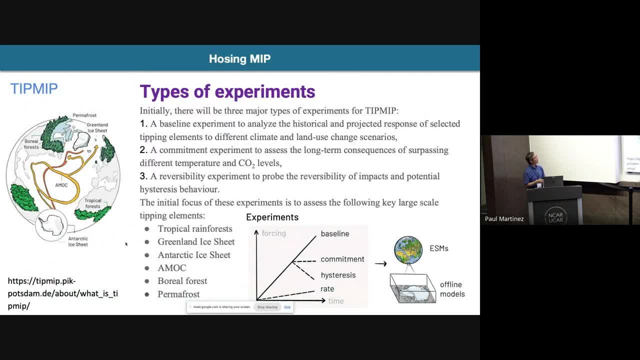 next is the hosting experiment and firstly, we are doing the North Atlantic hosting model inter comparison project. they have six models participating in this project and right now in Europe there's a new project called the TIPMAP project and there is a hosting map and right now we are 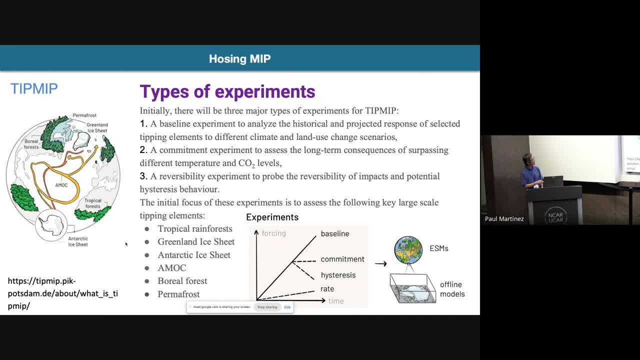 going to be part of this TIPMAP project. TIPMAP starts from this year and for the first phase there will be three years- 24,, 25,, 26- and they are planning for a second phase too and for this TIPMAP. mostly they want to do a few. 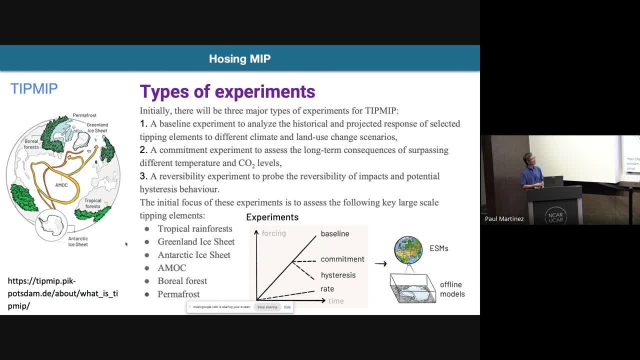 things. one is a pre-train experiment analyzing the historical and projected response or selected tipping elements to different climate and land use change scenarios. and also the second one is the community experiment to assess the long-term consequences of surpassing different temperature and the CO2 levels. and third one is the 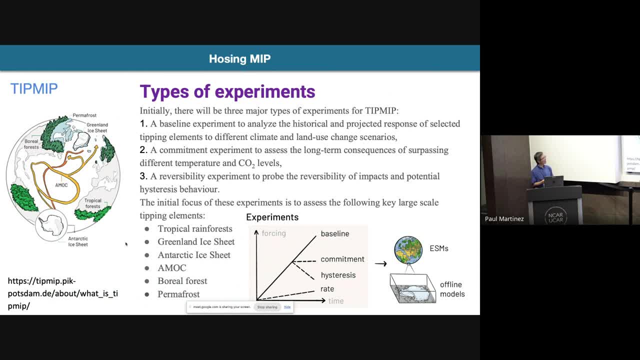 reversibility experiment to prove the reversibility of impacts and present hazard behavior. the experiment design is basically: we want to run a 1% CO2 experiment, either by drilling by concentration or drilling by emission. right now, I think that this experiment design is still in the process and we are going to be doing it in the next few days. 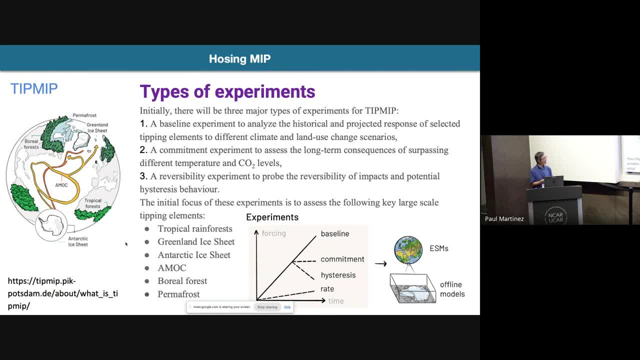 and we are going to be doing it in the next few days. and we are going to be doing it in the next few days and it's not really finalized yet, because right now there's another European project called TIP-ESM, the tipping point versus the model, and that's why they propose to run. 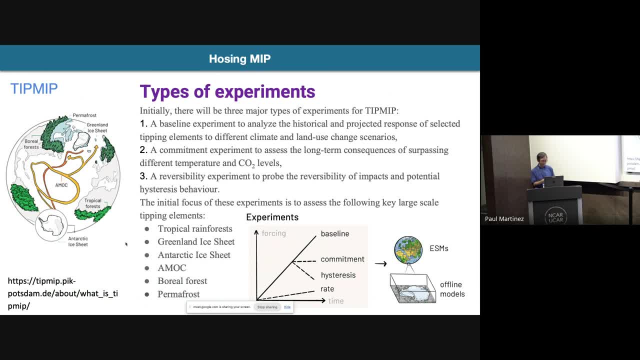 simulation using emission driven simulation. ESM may participate right initially. for the TIPMAP there's a six tipping element will be focused on the tropical rainforest run, an ice sheet and top of the ice sheet, AMOC forest in the spring frost. right now I'm getting involved in this AMOC. 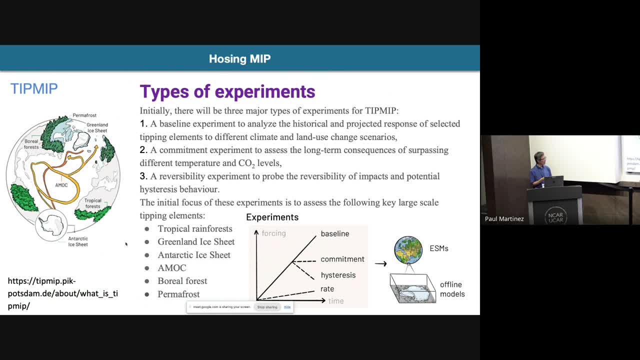 and they'll co-lead on the experiment design related to the AMOC and this will start the simulation. I think in the next few months, once we get this experiment design finalized and this TIPMAP may become part of the simulation. I just remembered the second thing I wanted to say at the beginning. I forgot. 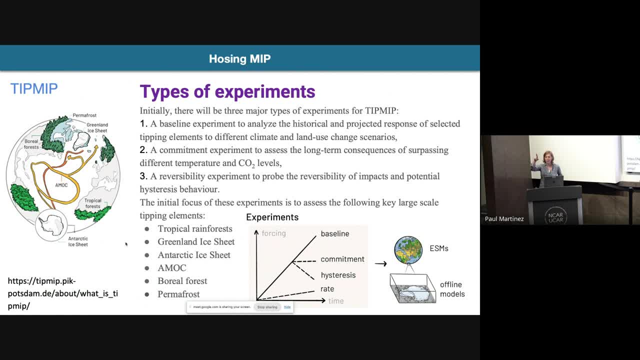 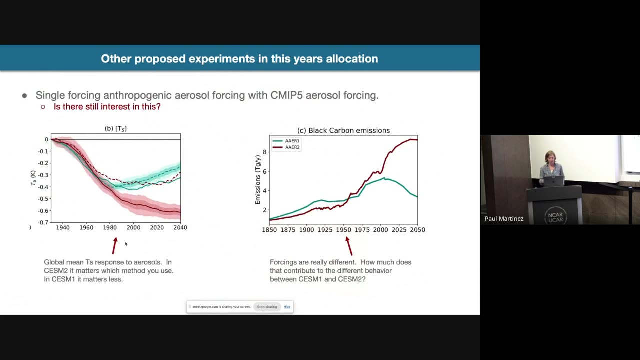 we're using those ceiling mics and when they're green people online can hear everything you say, so just be aware of that and you people will hear when you ask questions and things using those. okay, so now I just want to spend a couple of minutes talking about the plans for the next few months, so our 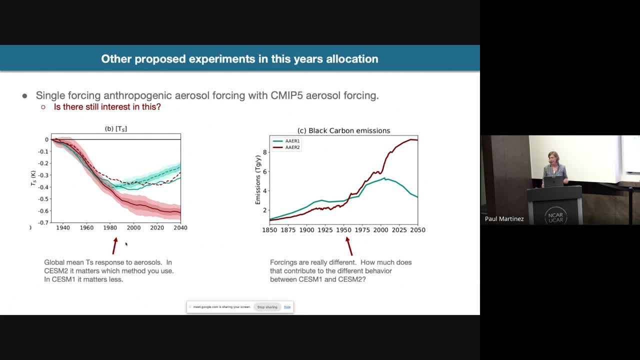 next couple of minutes talking about the plans for the next few months. so our next couple of minutes talking about the plans for the next few months. so our we have this computing allocation that lasts for two years and we make a. we have this computing allocation that lasts for two years and we make a. 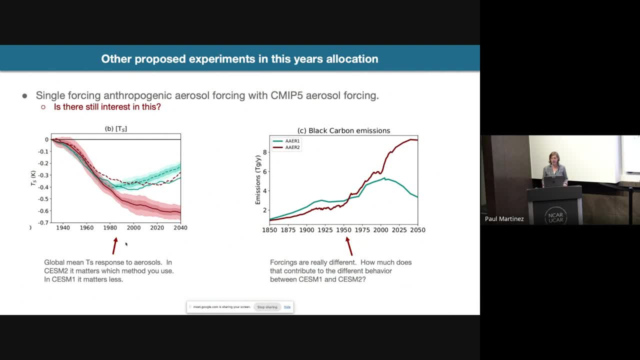 proposal for all the things we want to do over the course of that two years and that that goes until, I think, the end of our until September of this year. so I'm gonna just kind of run through the things that we have proposed that are kind of still on the agenda. but of course the priorities can change, we can. 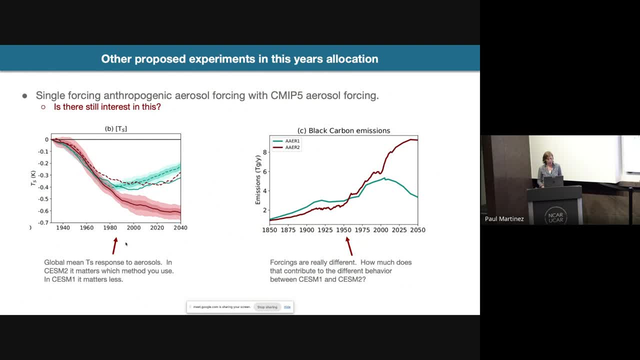 make adjustments and so glad to hear any thoughts on what people think about this. make adjustments and so glad to hear any thoughts on what people think about this. proposed ensembles we plan to do was to run another single forcing aerosol ensemble, but with the CMIC5 aerosol for things that were used because we had 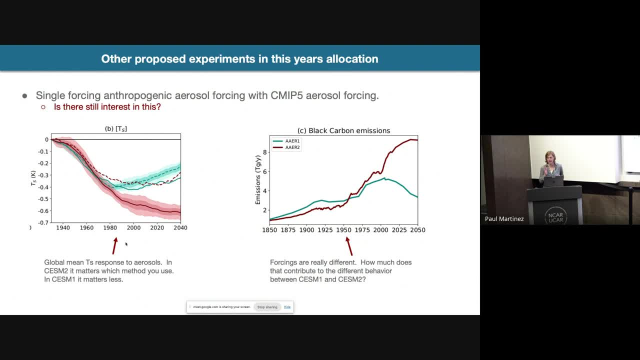 found pretty different responses to aerosols between CSM1 and CSM2 and you can see that here in the global mean temperature on the left. so there's no legend here, sorry. so the the solid lines are only aerosols and the dash lines are everything but aerosols. 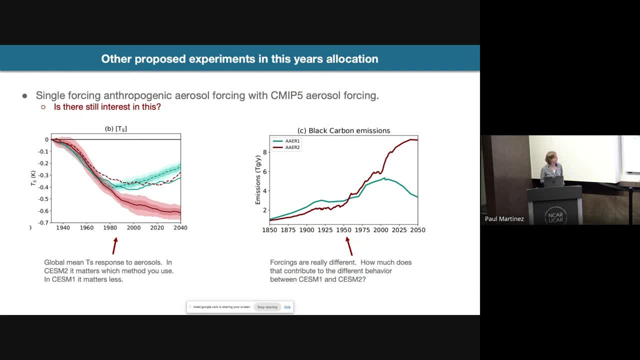 the green or teal is CSM1 and the maroon is CSM2, and so what you see is that in in CSM2 we have a big dependence of the method of the response on the method that is used, whereas in CSM1, the difference between the teal lines we have less of a. 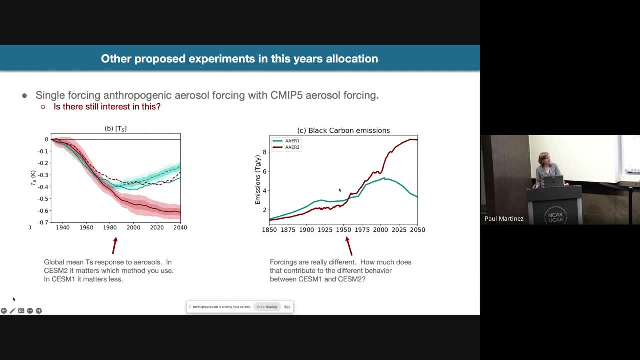 dependence on the method that was used. on the right. here is an example of the difference in the aerosol emissions between the CSM1 and CSM2 simulations, and part of that is a different scenario. we use a high aerosol emission scenario in CSM2, which is the 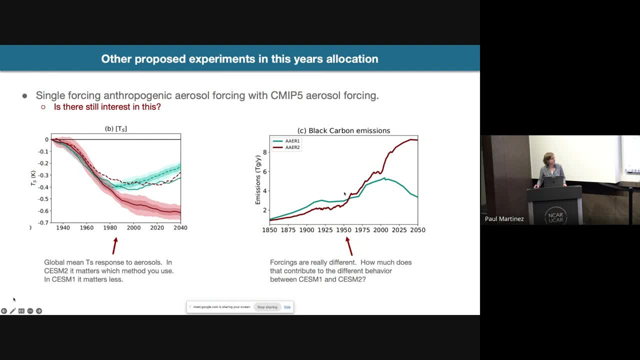 moving one and a low in CSM1, but there are also big differences over the historical period in the aerosol emissions, and so there was a project led by Marika Holland and Cecile Hane to run CSM2 with CMIC5 forcings, and so the plan here was to build on that and run an ensemble of only 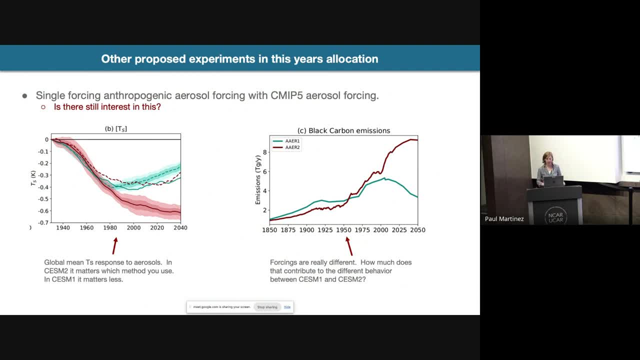 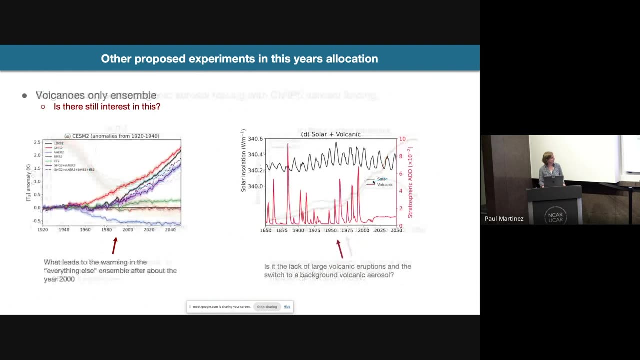 aerosol forcing so that we could look at what is the impact of the different emissions between CSM1 and CSM2. so that's still kind of on the agenda, unless anyone objects, or it would also be good to hear if anyone is particularly interested in this type of experiment. another plan was to run 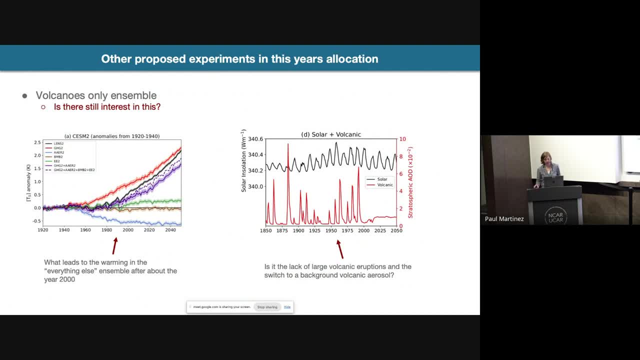 an ensemble of only volcanoes, and this is another thing that was motivated by the single forcing large ensemble. so if you look at the green line and the one on the left, that's the everything else run which contains solar volcanoes and land use, land cover change, and you see that there's a warming anomaly in that everything. 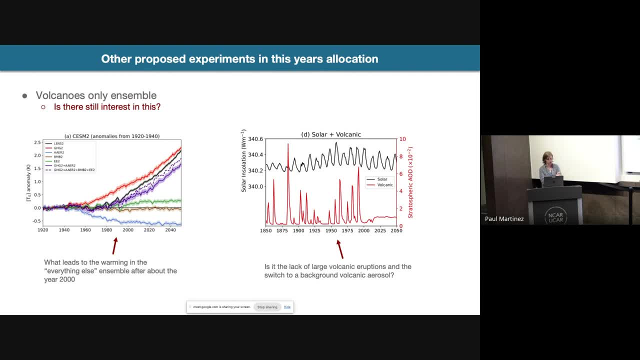 else run in the early 21st century and it seemed like a likely candidate for producing that might be the volcanoes which we see on the right in the red, there that we kind of transition from having these this period punctuated by large volcanic eruptions to having this steady volcanic background. 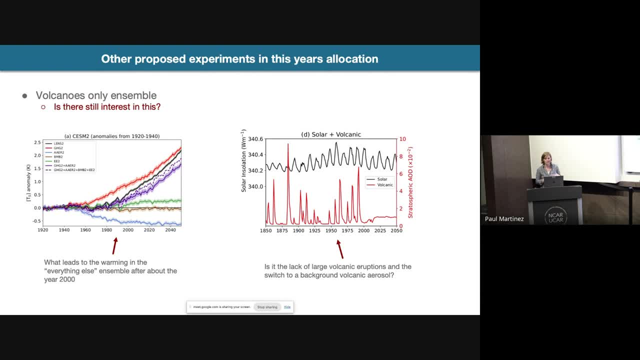 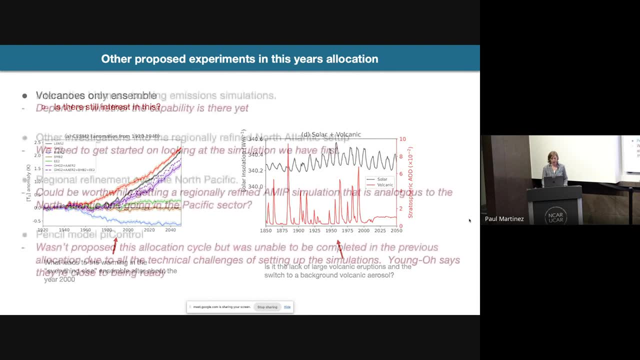 and so we were kind of interested in running our volcanoes, only to see whether that really was the cause of that warming in the. in the green line on the left here are a few of the other things that were planned. one was to run some simulations with 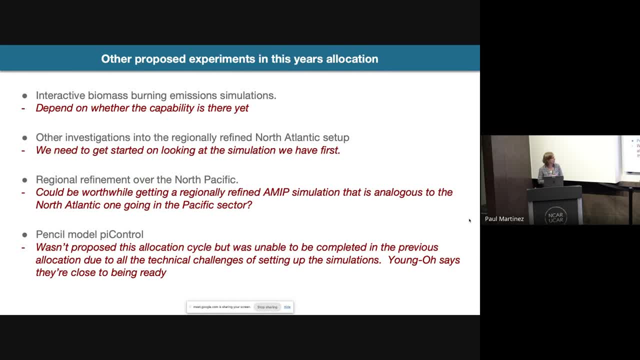 new interactive biomass burning emissions, which is a capability that's under development. I don't know if Dave can speak to whether there's that's likely to be ready or not. I did email some people but didn't hear back yet. we were going to do some more investigation with the regionally refined. 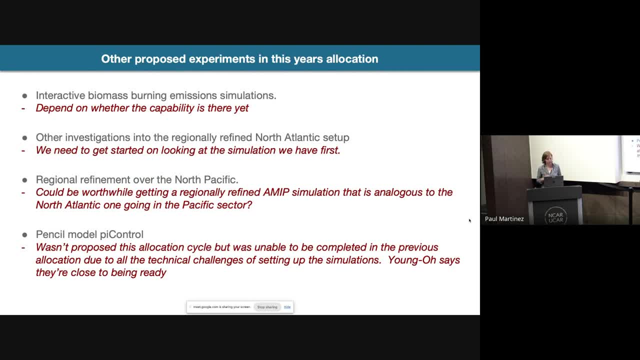 and I really need to just spend some time looking at the time that we have before we think that I want to do with that. next, there were some regionally refined North Pacific plans. I don't know if you still have plans in that area. we can talk about that later. and then there's this pencil model. 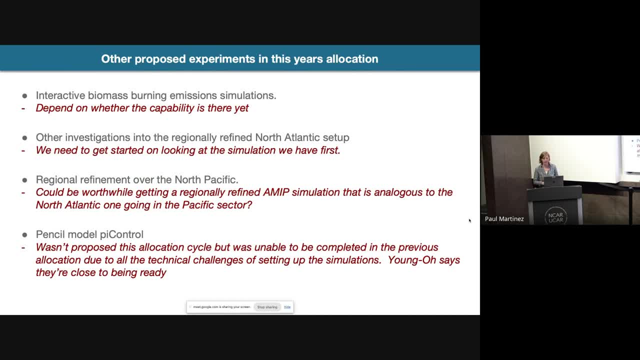 which is kind of in between a slab ocean and a cup fold model. this is being developed by Yango, Quan and Gokhan, so this is basically a single column ocean model at every grid point which allows you to have prognostications, mixed layer debts, which is not something you have in a slab ocean. so it's kind of a nice. 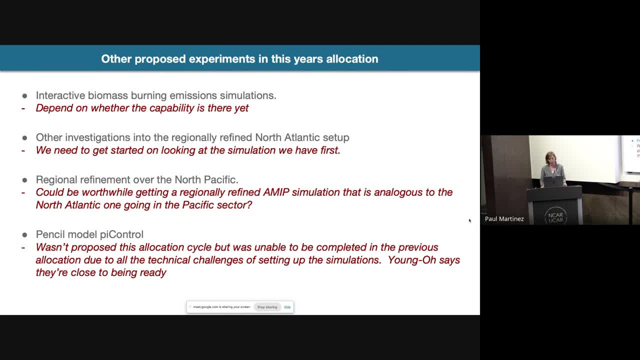 intermediary between the slab ocean and the fully coupled model and that was in our previous allocation but there were many technical difficulties in setting it up and you know things that are almost there and might be ready to run a pre-industrial control with that configuration in the next few months. so that's kind of what we have on the agenda, but definitely 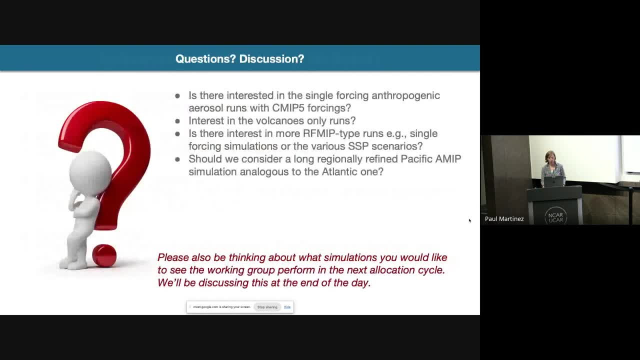 happy to hear any thoughts, um, and so we're. we only have a couple of minutes at this point for discussion, but we can we have time at the end of the day for more discussion. so, um, those are some of the questions that i had for for any of you, um, based on what we're going to do over the next few. 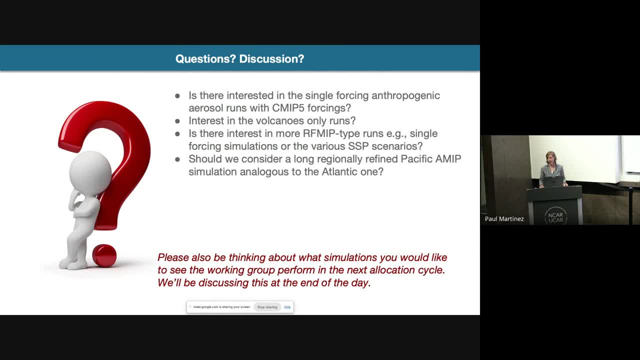 months. but also it'd be great if, over the course of the day, you could think about experiments that you would like to see the work and group run um in the next allocation, because we'll be planning that in the summertime. so we have this meeting and then the summer meeting is the chance to kind. 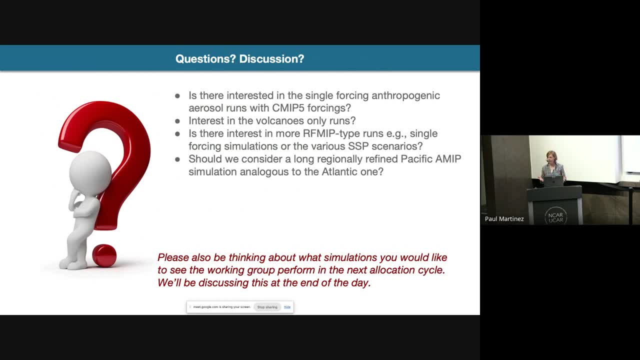 of discuss that more. so i'll end there. we have a few minutes. if anyone has any things they'd like to bring up at this point, uh, actually feel free or be thinking about what we'd like to bring up in the discussion session, i can bring it up later. we're still planning to do those simulations, we're. 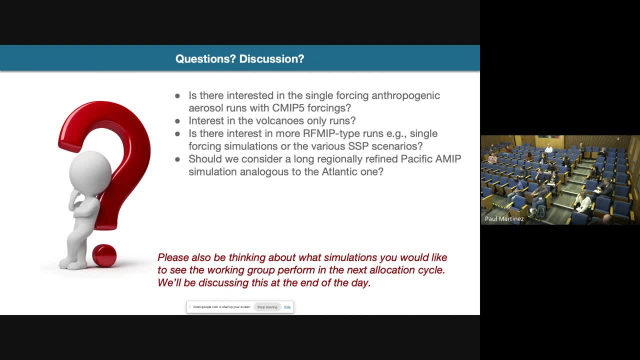 still struggling with some design choices, okay, but- and the other thing i'm thinking of doing and i've talked to people doing ocean sciences- is- and i'm sure everyone knows that- the high resolution, csm, has all these unique responses, regional responses that i think this community, i'm sure, is excited to look into and perhaps there's 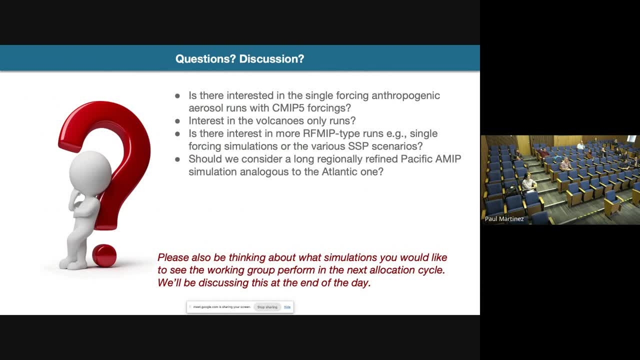 some and and all that is doing by people here at anchor and ping chang at texas a and m. but i think there's perhaps room for this group to think of maybe pacemaker run. i mean, those are going to be like extremely expensive but perhaps not every single pacemaker. 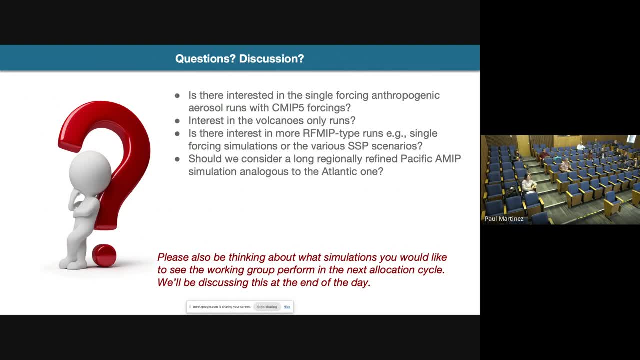 run with with the irs but and the computer allocations are going to be massive, so perhaps there's other mechanisms and tac has these big allocations that were used to run the fully coupled simulations. perhaps we can also meet a computer time proposal or anyone that is interested. i'm 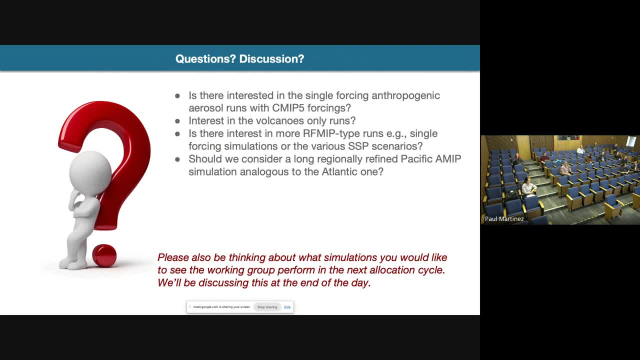 happy to coordinate and leave it. it's something i've discussed with uh kate monigal in ocean sciences and we're thinking of proposing- okay, defining- a subset of all these experiments that we normally do, perhaps single forcing. there's none of that with that version. 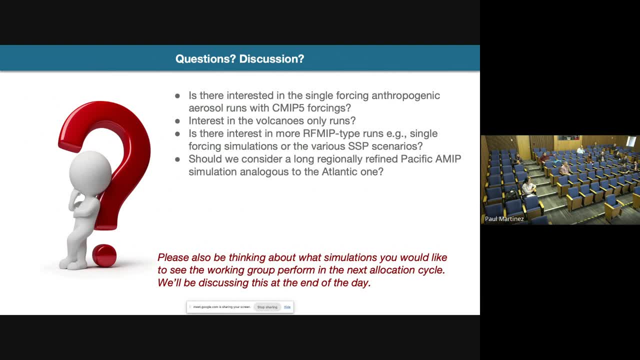 of the model. yeah, so we need to be strategic because there's it's so expensive to run, yeah, but it's definitely. we should definitely pull apart all of the, the origins of those different. yeah, even the mixed resolution like these are full, increased resolution in both the ocean and the. 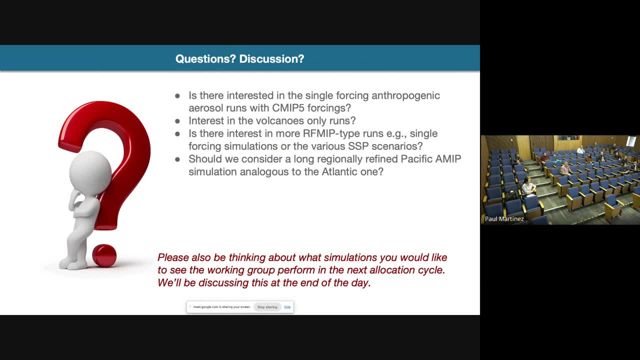 atmosphere, horizontal, and- and some of the responses come from the ocean, others from the atmosphere, and i think even learning. that would be useful. yeah, definitely, i mean there are. i know there are a number of proposals and steve has one and i think you have. oh, i have one, yeah, but they're more. 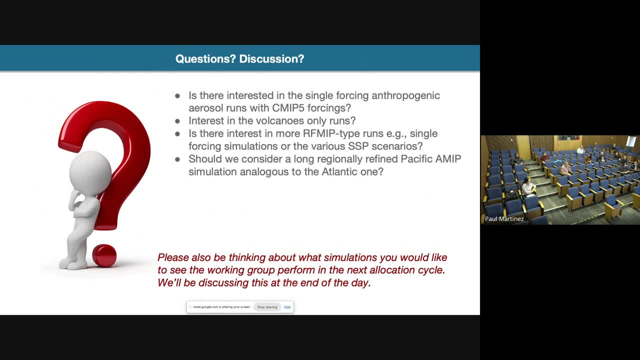 specific, i'm thinking of more community resources. yeah, beyond what we probably will do in, we should probably at some time get all of the interested people together and think about what would be the right experience. that's what i was thinking. yeah, we were thinking of. we came, we were thinking of. 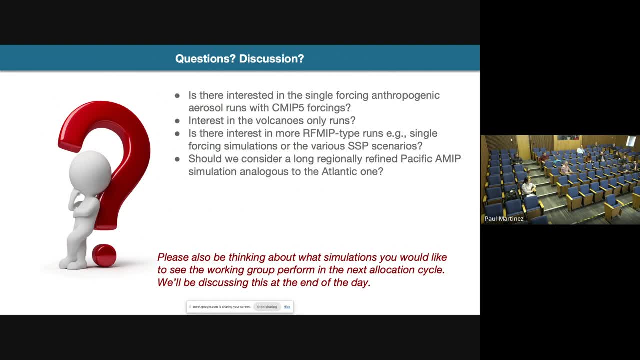 proposing a mechanically decoupled like ensemble, but everything you do is super expensive. it's like climate modeling 20 years ago- yeah, yeah, i was not here again. just briefly about biomass burning emissions. we have that. peter lawrence is actually running that now. so outside of the common variability change and he's testing an historical um for this. 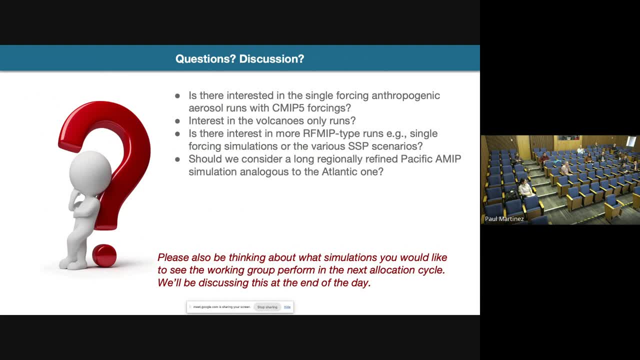 msf growing convergence project on climate interventions. okay, so you could maybe take it off the list of things you need to do, but it hopefully will be some simulations that will be available, okay, yeah, so yeah, i mean, we definitely have allegations set aside, so if there was interest, 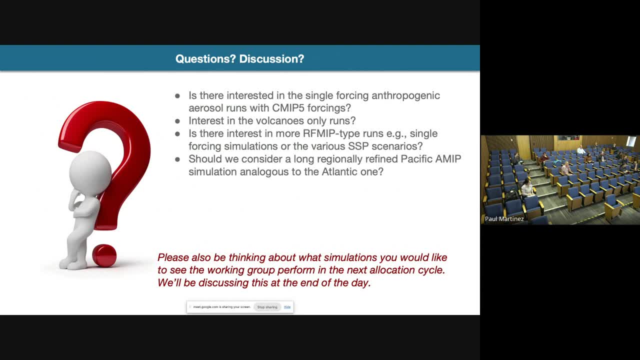 in running more members, or you know we can. okay, yeah, i'll let peter know that if we, if it's allocation, starts carrying an issue, that will come back to you maybe. uh, i don't know if i'll be here this afternoon for the discussion. you in general, just this is an obvious point. but 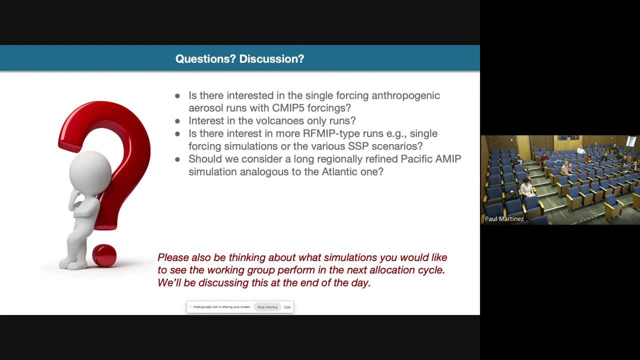 there's a lot of simulations that are available right um, and so how are you tracking those? and one idea is that we can advertise somebody through the newsletter, but but having a web page, maybe it already exists. that i don't know. yeah, we have the climate variability. 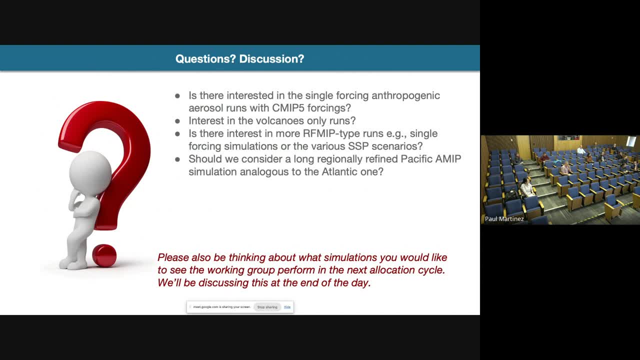 and change working group web page that has links. adam maintains it has has all those simulations and if you go in there there's step-by-step instructions of how to get at them. some of them are not on the earth system. oh, there's a climate data gateway, so some of them you just 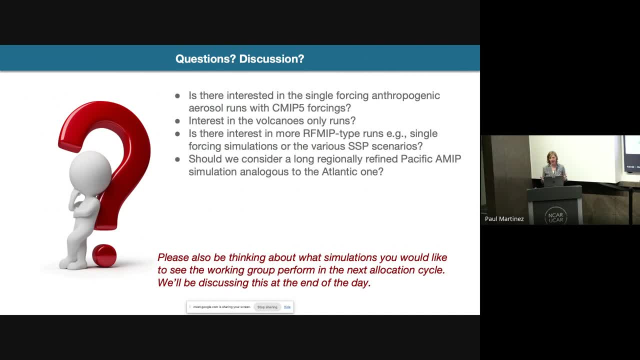 need to email adam to get them. um, so i think that's a good point. i think that's a good point, adam, but i guess if there's many people emailing, then maybe we would change that and put them on there. yeah, let's just take advantage of a newsletter to, to you know, give it a brief overview. 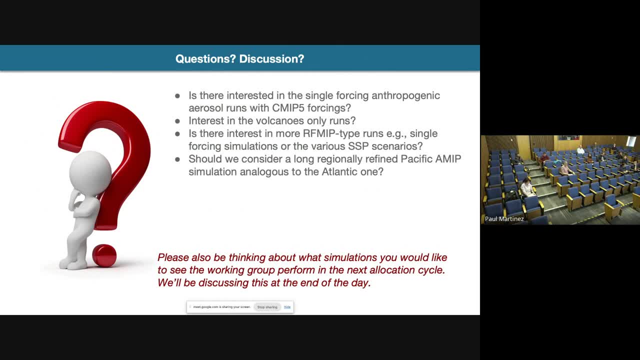 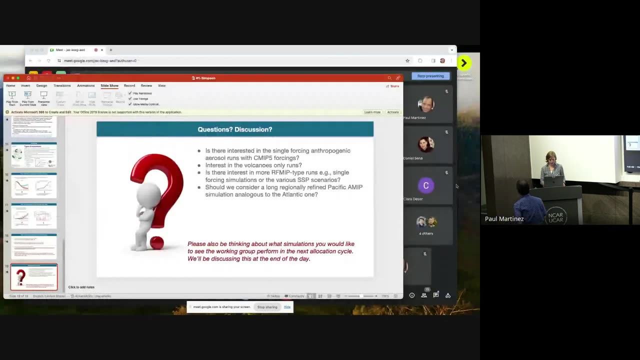 of that and point people. it's just because some people don't know about it. yeah, sounds good. well, we're already two minutes behind, so let's um move on to the talks and please keep all your thoughts for the discussion at the end of the day. so i'll hand it over to aisha, to the chair. 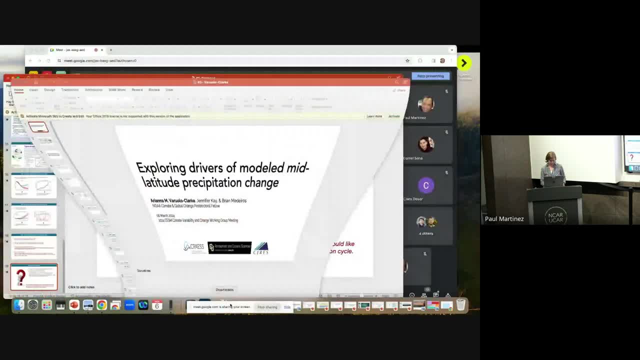 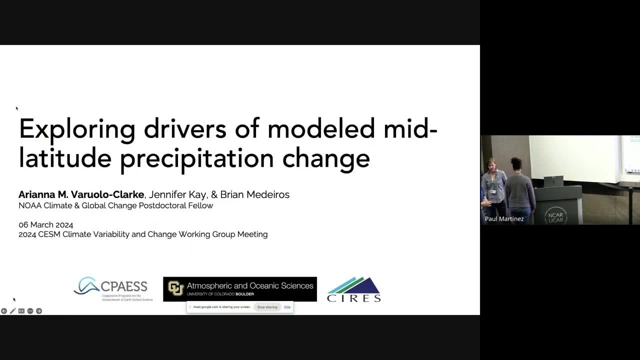 for a little bit isn't by a random. we'll just give you a 12-minute warning. i'm just gonna time to wrap up. perfect, thank you. um. good morning everyone. um, i'm really excited to be here. i'm a relatively new postdoc here working with jen kay at sweden folder and then brian materials. 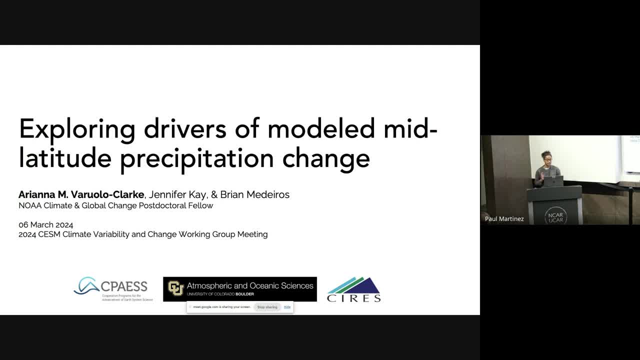 up here as a noaa climate and global change postdoc um, so i'm excited to share with you some very um work in progress: ongoing work in exploring mid-latitude precipitation change. i'm interested in this because during my phd i was focused on trying to understand. let's jump. 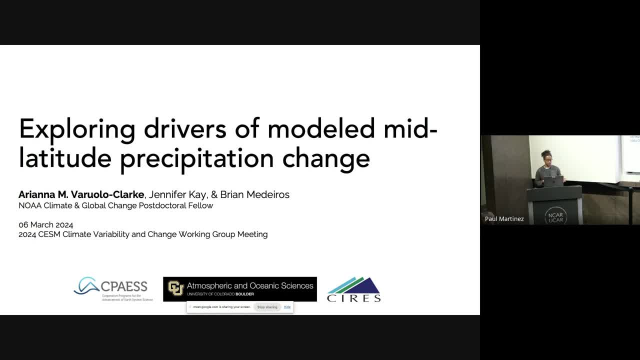 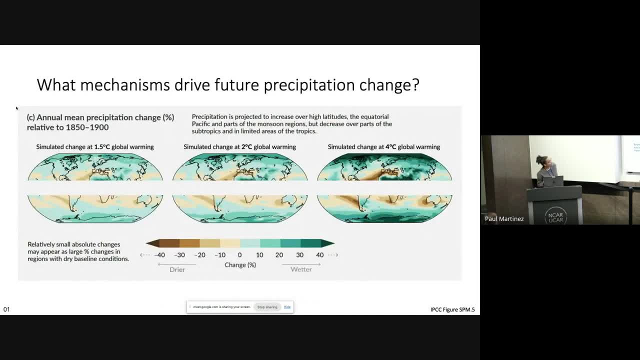 the slug increase and summertime rainfall in south korea, south america. i'm somewhat motivated by these broad hydroclinic trends and changes questions. i wanted to start by looking at this art piecing scene figure to orient everyone. i'm sure how many of you have seen this, but this just 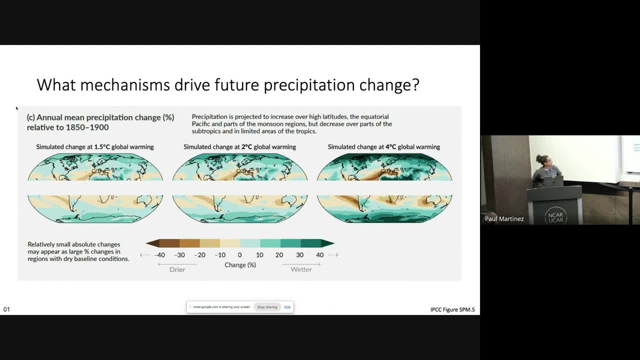 animal. mean precipitation. change in percent relative to the 1850s and 1900s. mean different levels of global warming. i apologize to everyone really excited about the tropical pacific and what's going on there, but i blocked out that region just to compare better with. 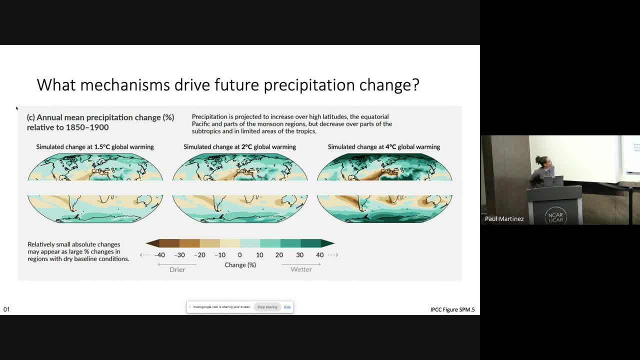 my later work that is just focused on the mid-latitudes, but so we can see these broad strokes, increases in rainfall or precipitation over the mid to high latitudes, and here's warning where we're trying over the subtropical. it is really hard, wow. once you get it pointing to there, you can then move it over to the screen. 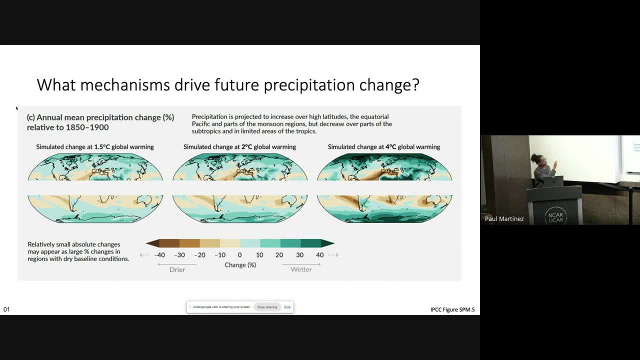 and so yeah, so we have more or wedding kind of in the mid to high latitude drying kind of over the subtropical regions, um, and these kind of patterns increase or um become stronger as you increase their higher levels of global warming. so i'm really interested in what mechanisms drive future, future precipitation change and then, more specifically, 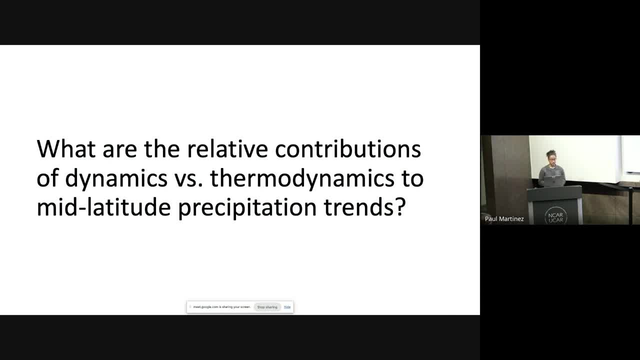 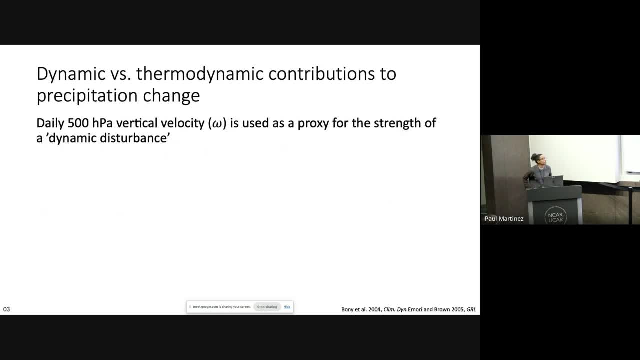 i want to think about what are the relative contributions of dynamics versus thermodynamics to mid-latitude precipitation change specifically? and so, in order to do that, there's lots of different ways to think about this, right? um, i just want to tease apart the dynamic versus thermodynamics. 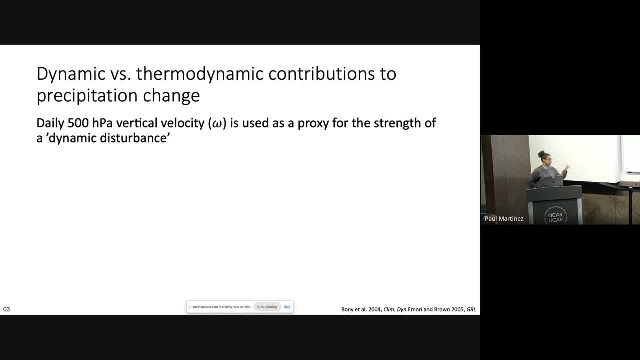 to precipitation change, and i want to use the this methodology that was set in place by Boney et al some 20 years ago now, where they were looking at the dynamics versus thermodynamic contribution to cloud change, and then, just a year later, Anne Marie and Brown used the same methodology, but to specifically look at precipitation change. 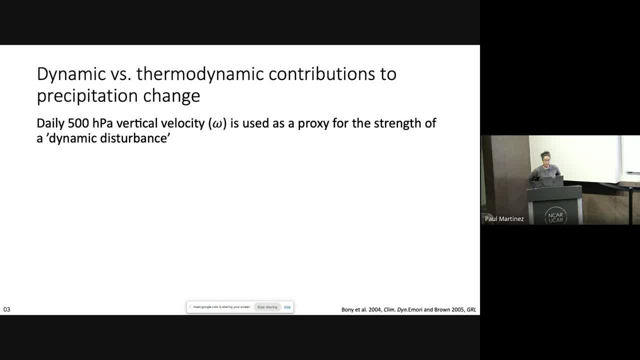 So, in order to do this, we consider daily 500 hectopascal vertical velocity, or omega, as a proxy for the strength of dynamic disturbance. This is just one metric that we can use right, and so I'm curious of people's feedback on a different method that we can use. one thing might be like: 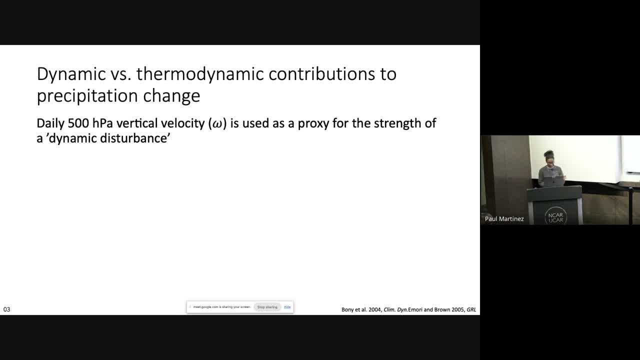 eddy, kinetic energy, for instance. but anyway, starting here, what we do is we obtain the probability distribution, or pdf, of omega for historical period- here we're considering 1981 to 2000 compared to a future period 2081 to 2100- and so we get this pdf, so we have the 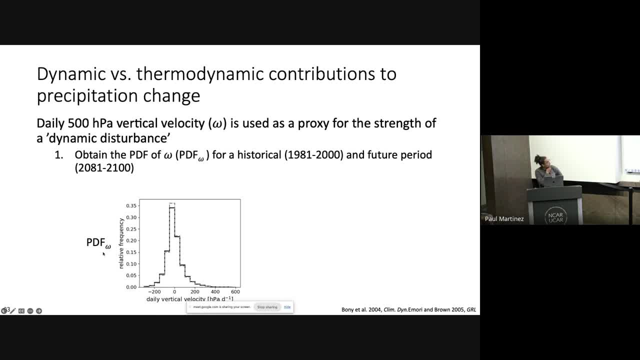 daily vertical velocity on the x-axis and then the relative frequency on the y-axis. black is the historical period and the gray bars is the future period, and then we composite the daily precipitation for each omega bin for both periods. so now we're looking at the vertical velocity again on the x-axis, but now the y-axis is the. 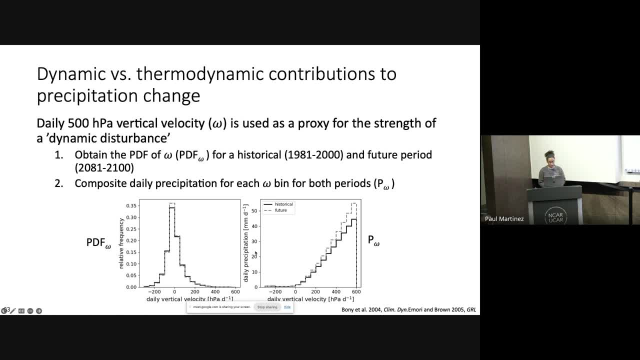 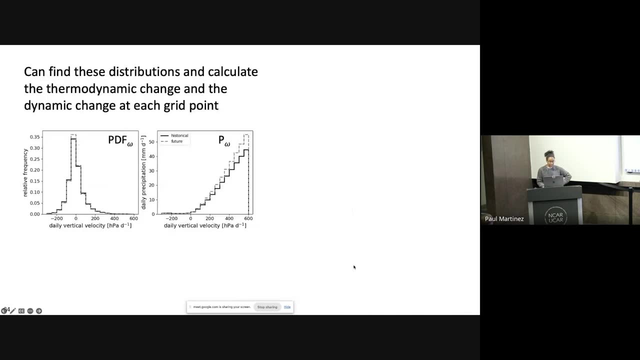 daily precipitation bin for each of these omega. so you can see the historical period in black and then the gray dash is the future period. so we're getting more precipitation occurring at the uh vertical velocity values, and so what we do is we- this is just an example- averaged over 20 to 70. 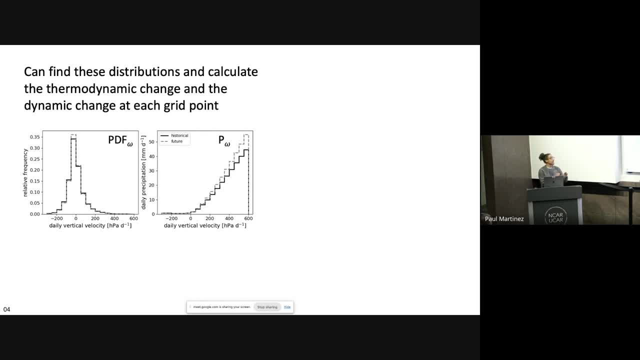 degrees south, but we can find these distributions at each grid point. and then we can consider the dynamic term to be where we take the historical precipitation distribution and multiply it by the difference in the vertical velocity distribution, and then the thermodynamic term is where the circulation doesn't change, but then we're considering these two of our precipitation. 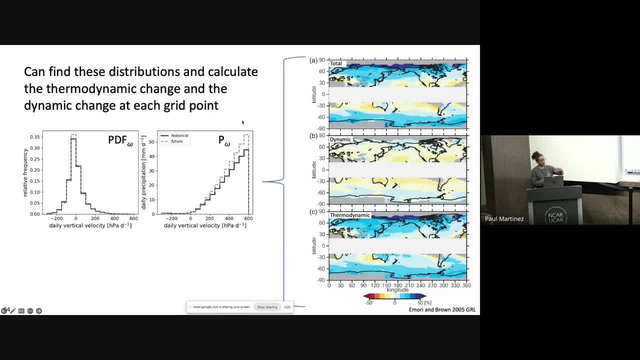 distributions. We do that at point and we get. we can get these nice maps like from Emery and Brown that show you that you can get the total precipitation, which is the combination of the dynamic term and the thermodynamic term and the residual or co-variability they did not show. 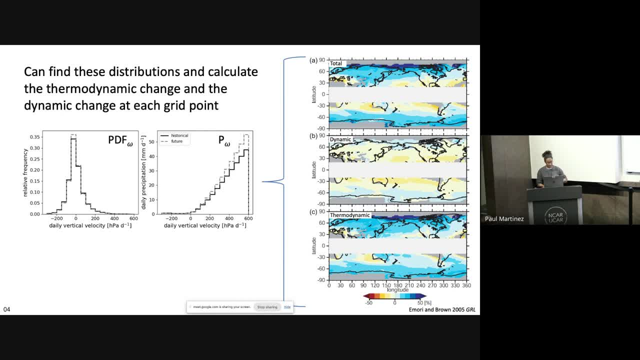 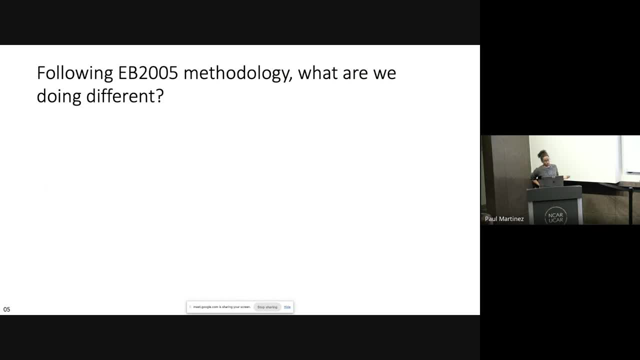 And so I'll talk a little bit more about these results that they presented later on, but this is the methodology that we're following for now, And so, following this methodology, what are we doing different from this Emery and Brown pp 2005 paper? So, first of all, they're just considering 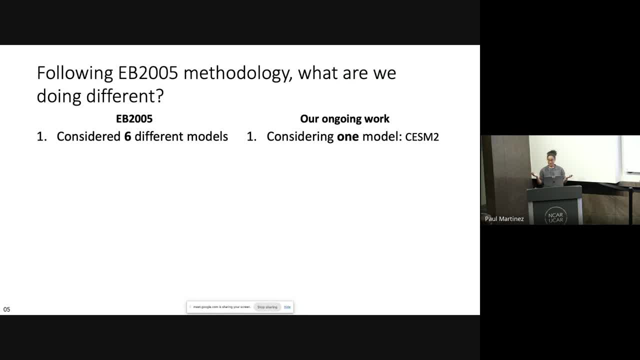 six different models. we're focusing on one model for now, cbs on two, of course, and they in Emery and Brown just looked at one run for each model. so only six different, six runs total, and so we're considering 50 for now. what I'll show today, just to sum up, six things. 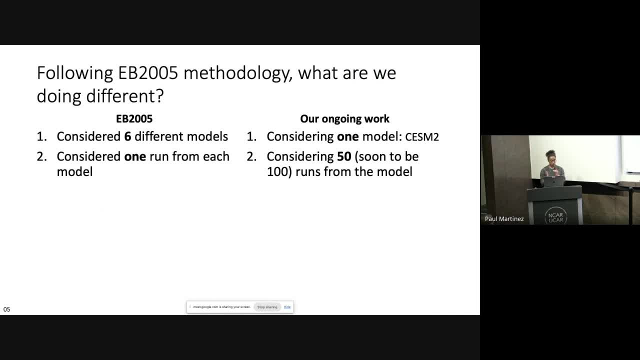 of the CESM2 large ensemble, but soon I'll include all 100 runs. And then they, in the 2005 paper, just considered annual precipitation and I'll be focusing on all seasons, specifically winter and summer, since that gives us kind of the most extreme. 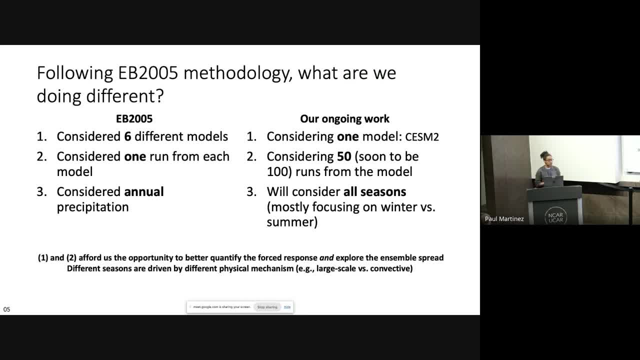 of these different mechanisms that drive precipitation And so, by the differences in one and two, kind of afford us the opportunity to better quantify the course response right and explore the ensemble spread, which is something I'm really excited about. And then different seasons are driven by different physical mechanisms, of course right. 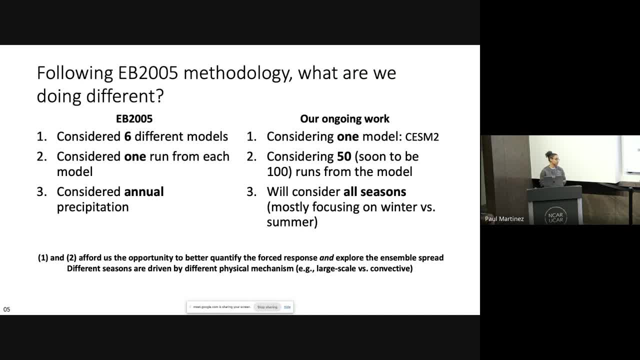 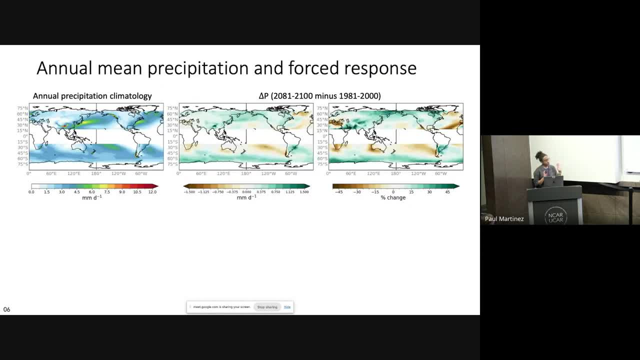 So in winter we have more large-scale precipitation versus more convective precipitation during the summer. Okay, so I'm going to start with the annual mean precipitation and course response and then compare that to Emory and Brown before I dive into the different seasons. 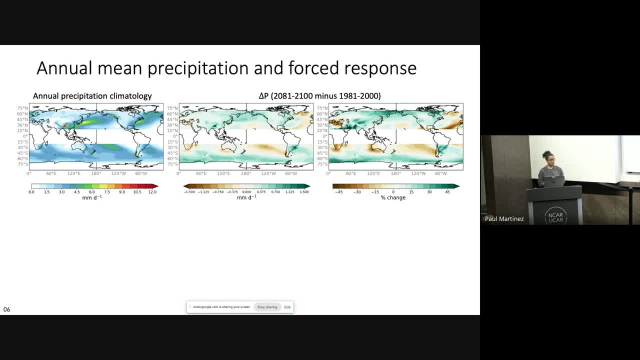 So, starting with the annual climatology For 1981 to 2000,. we can see we get the nice storm tracks over the oceans, we get the Asian monsoon popping out really well, and then we're just showing the differences. So 2081 to 2100, minus the 1981 to 2000 period, and I'm showing in millimeters per day as 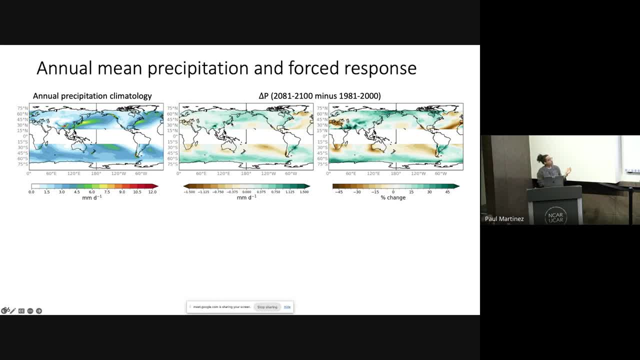 well as the percent change and you can see similar to what we saw in the IPCC figure. we get this increase in rainfall across the mid-to-high latitudes, some drying in the region, especially in the Southern Hemisphere oceans, and then we can look at the contributions. 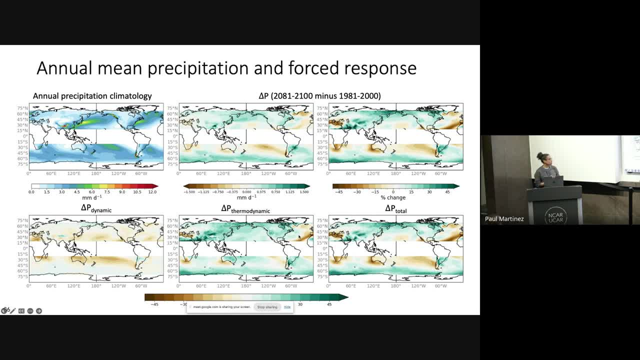 from the dynamics versus the thermodynamics and what we see is that the dynamic term is really contributing to some drying in this region, whereas the thermodynamic term is contributing to a wetting signal, which makes sense when we think about cosmic hop around and the theory behind all of this. 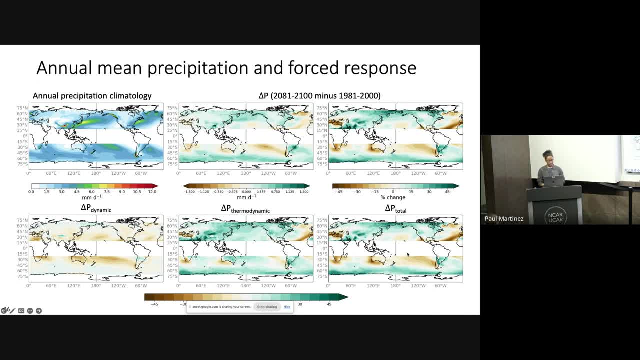 And then this change in precipitation. total is the linear combination of the dynamics and the thermodynamics and the covariance. Okay, So we can see the variability, which I'm not showing but should be quite comparable to this top panel here, which was the actual calculated difference. 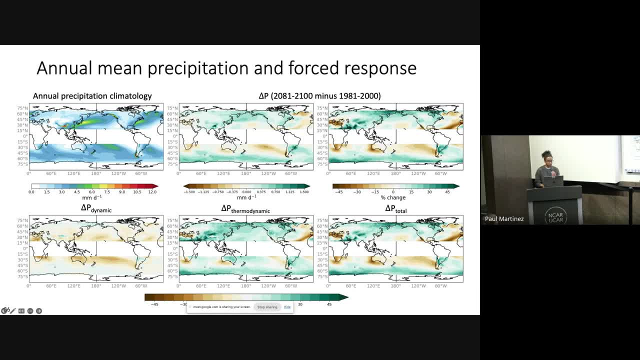 And so what you can see in this is that the total really reflects more of the thermodynamics, especially throughout the continents and in the Northern Hemisphere we have some stronger dynamic signal being reflected in the total terms over like Australia, for instance, And again, this is like these: 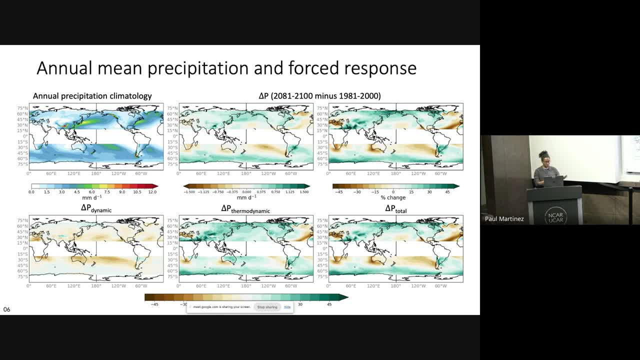 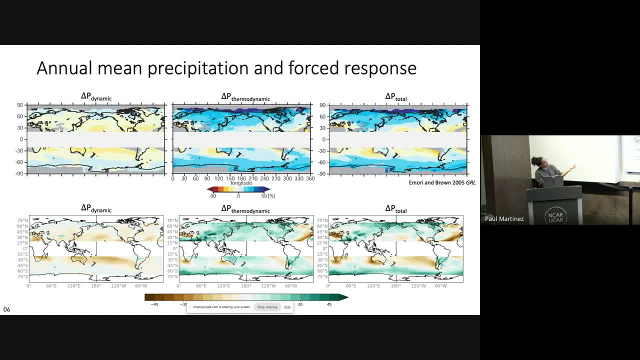 Some of these results are caught off the press so I don't want to interpret them too much, but just to kind of highlight the methodology And then just to compare. so now these are the results from Emory and Brown, So we can see that CESM, the results from CESM2, look quite comparable to earlier models. 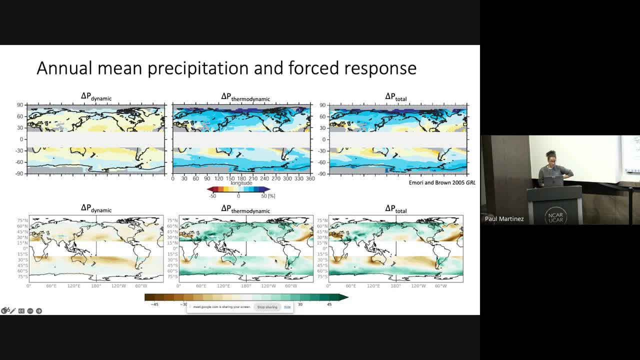 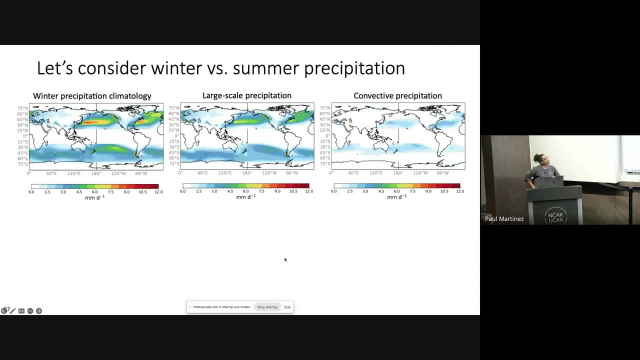 where the dynamic term is really contributing to some drying. thermodynamics is contributing to more of the wetting signal and then the result is, especially in the Northern Hemisphere, over land, definitely driven a lot by the thermodynamic term. Okay, So now we want to break it down into seasons so we can start just thinking about the winter. 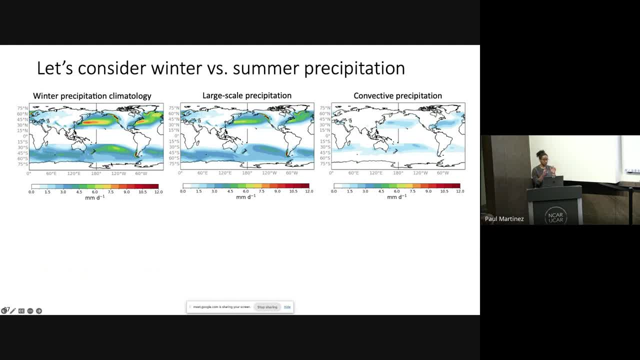 precipitation, climatology and, as I do, the season: the Northern Hemisphere- this is DJF and the Southern Hemisphere is JJA, so we can see the really clear storm track features popping out in the climatology, and then I've just broken it down into the large-scale precipitation. 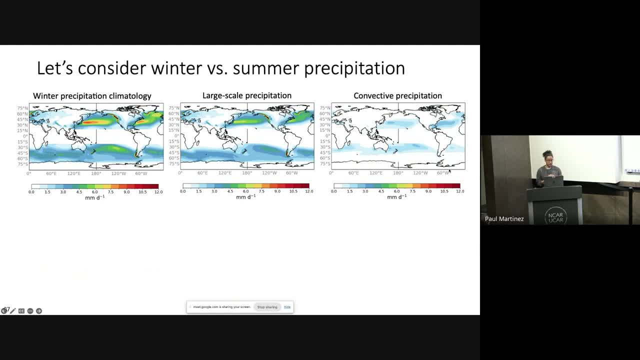 versus the convective. Okay, Just to kind of highlight that when we're thinking about the convective, precipitation in the models, of course that's going to be something that's parametrized so hard to kind of nail down at this resolution. 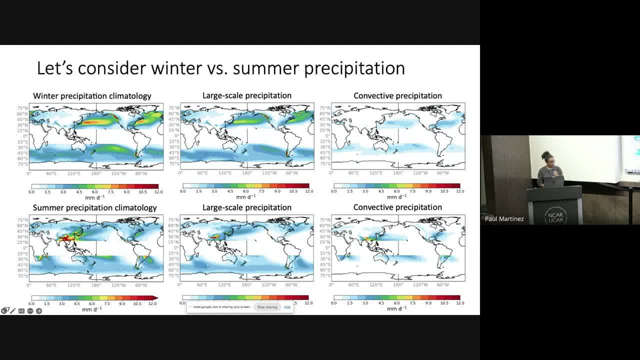 And then the summer precipitation. climatology of course looks quite different from the winter precip. We're getting more of the monsoon signal over Asia, a little bit of the North American monsoon, which I did some of my master's research on. 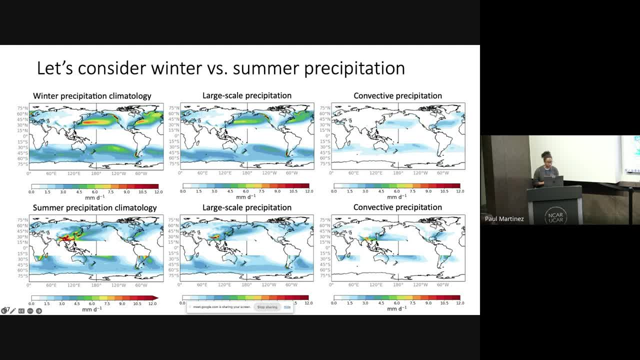 So, again, I think there's this kind of pullward effects of the South American monsoon. We see this as well in the large-scale, but then, of course, we have more convective precipitation over the continents during the summer. So, considering these differences, let's dive in to what's driving the winter versus summer. 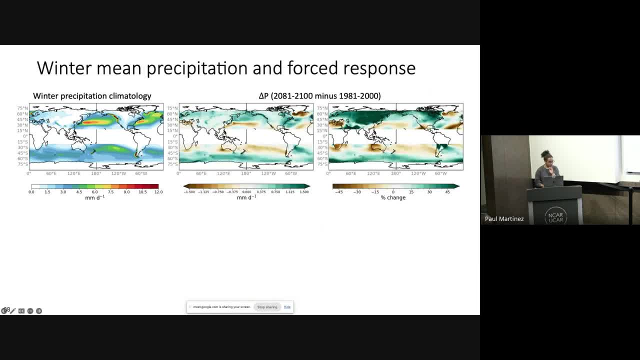 precipitation changes for the end of the century, So this panel will stay the same: winter precipitation to the summer And then the change in precipitation, again in millimeters per day versus the percent, so we can see real increases throughout the northern hemisphere mid-latitudes. 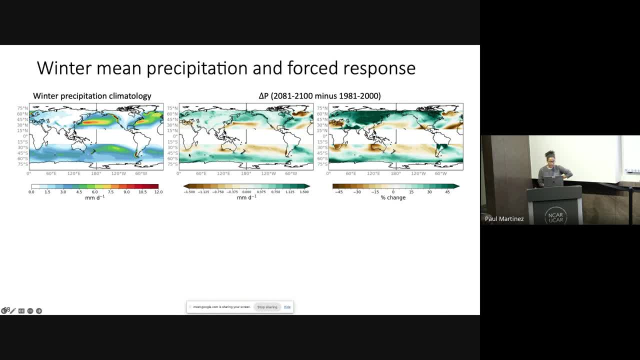 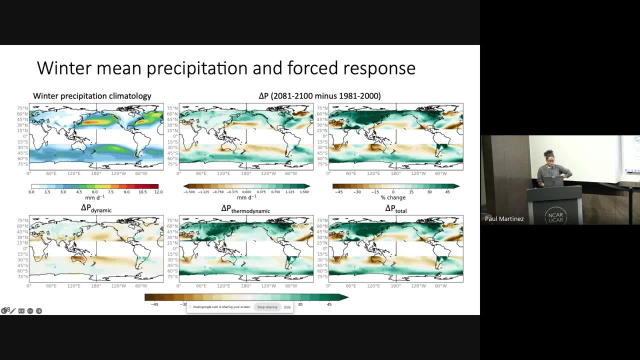 real drying over australia and south america, based on the percentages. but then when we look at the raw values, these are kind of dry places that are just getting a little bit wetter. and then we break it down by the dynamics. you can see kind of again the dynamic signal overall. 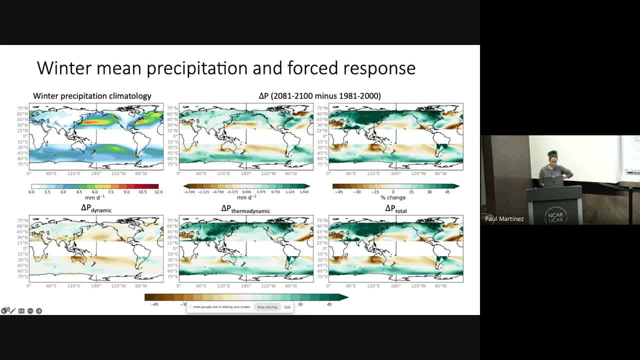 as a drying trend or pattern. thermodynamics is very lots of wetting and then combined we're seeing some dry, some of this drying signal through the storm track region, kind of coming from the dynamics. again, it's really me. australia definitely is being driven by the dynamic signal. 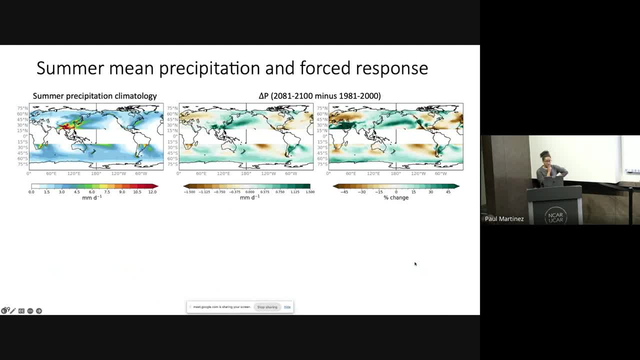 versus thermodynamic signal, and then we can go to the summer. so we saw this panel already and now looking at the changes, these changes are way kind of less homogeneous compared to what we saw in the winter, kind of overall increases in this region, but we have some drying over north america, europe and eurasia. 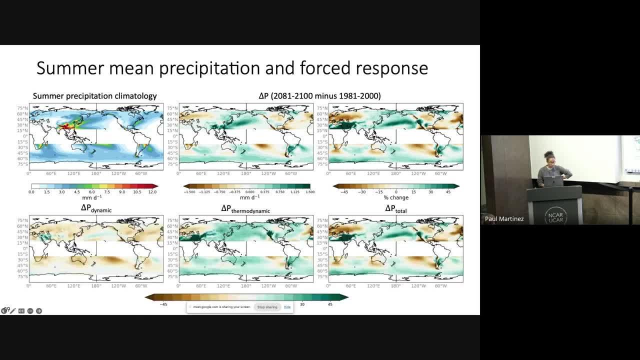 there's some clear wetting throughout the storm track region and then, when we look at the differences, there's definitely a strong thermodynamic signal but lots of kind of drying from the dynamics that are definitely reflected over the northern hemisphere continents. and again you have these, this kind of drying signal over australia, also maybe over south africa. 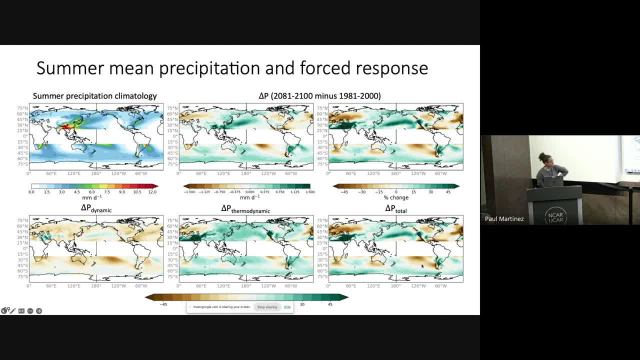 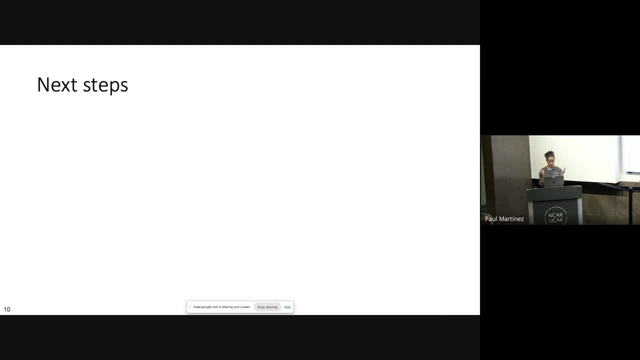 coming out through in the total precipitation chain. so that's kind of just a fast pass, an introduction to the work for what i've been working towards. and so now i'm interested in why, why these patterns look the way they do. so i want to investigate the different thermodynamic and 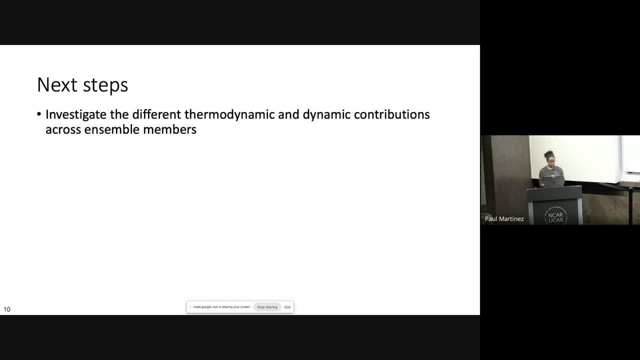 dynamic contributions, specifically across ensemble members. specifically, i mentioned australia a lot. so the dynamic precipitation change there seems to outweigh the thermodynamic precipitation change. why is that and how does that look across different models or members? how do the thermodynamic versus dynamic contributions evolve through time? so all of what i showed now was just looking at this 1981. 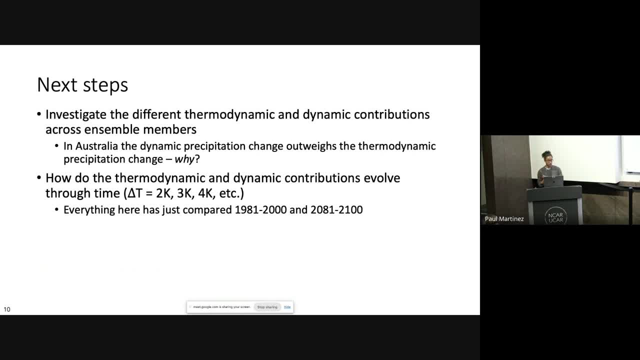 to 2000 period compared to the 2081 to 2100 period. but uh, what's kind of the response through time or thinking about these specific global warming levels, like in the ipcc figure that i started with? um, i've just used this single level, 500 pascal vertical velocity. 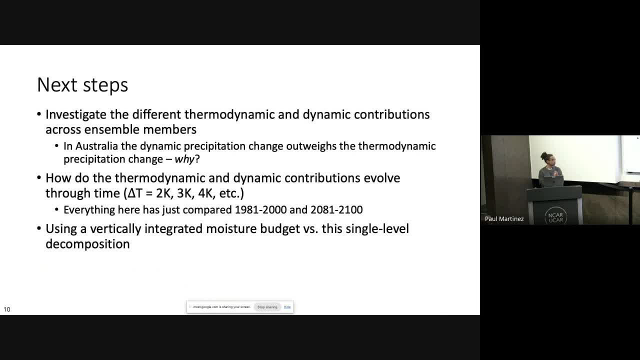 index for now, but i'm interested in using a vertically integrated moisture budget. or maybe didn't do that yet. any kinetic energy has a different metric, so different ways to kind of tease apart dynamics and thermodynamics and also think what that means when we're doing that. 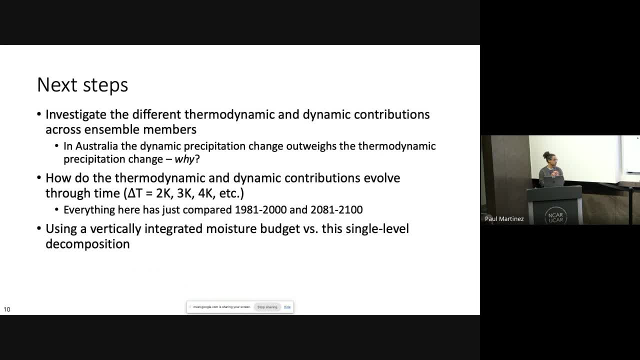 decomposition, like how perfect is it? what dynamics might we be missing? and then maybe we're gonna get kind of that, some idealized simulations. one that we've talked about and that i was excited about now would be some kind of wind nudging experiments that can really then set the dynamics. then we can. 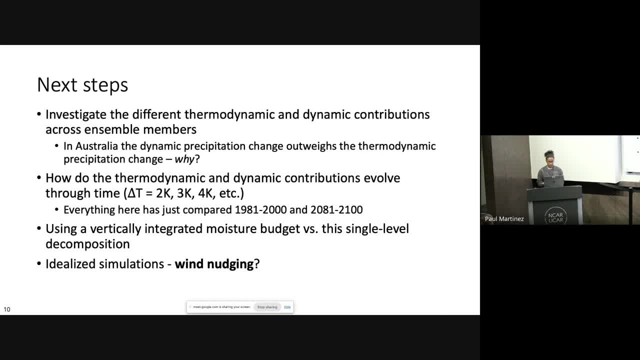 see what the thermodynamics kind of look without that. so with that, thanks for your time. i don't think any questions. any questions? all right, that was really cool. i was wondering, like, kind of the areas that are and you're kind of wanting to look at just the thermodynamic portion. is that because you're not? 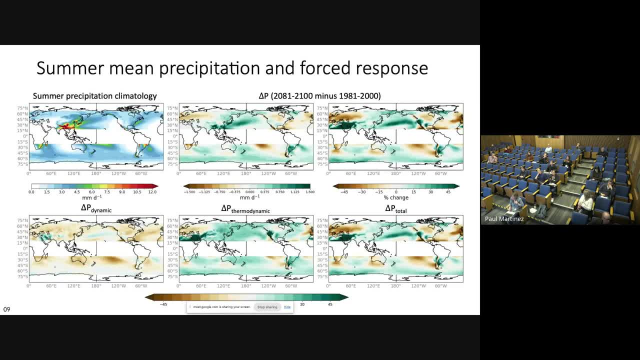 including like um, like the- i don't know what to call it- horizontal dynamics in the dynamic portion, and that's kind of where it's coming from. that's a good question. yeah, i guess, when like australia, maybe we would just think about that happening because of an increase in substance, but that's. 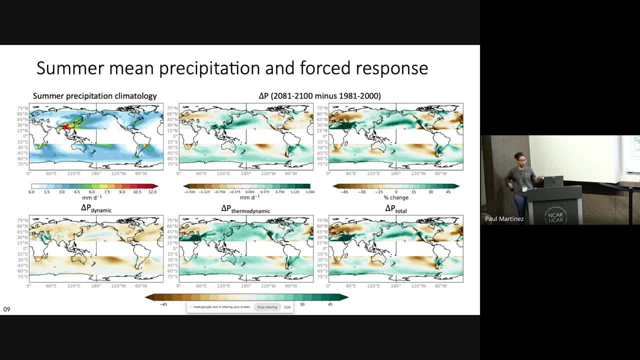 a good point of thinking about, um, like, what are the other terms and what do they? what kind of role? that would be right if you would think about those in a kind of more dynamic framework than the thermodynamic right. exactly, yeah, so this and part of the part of doing this- it's helpful for. 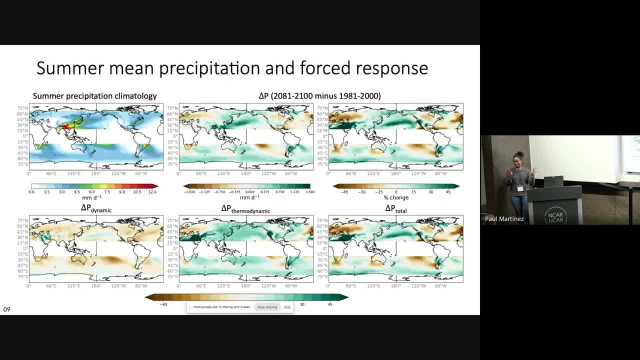 me to like, get a bigger picture sense of like what, like where the dynamics are most important, with the idea that the greenhouse or like the thermodynamic term is really about forcing term. um, so it's probably going to be consistent across the models, but can we find or elucidate? 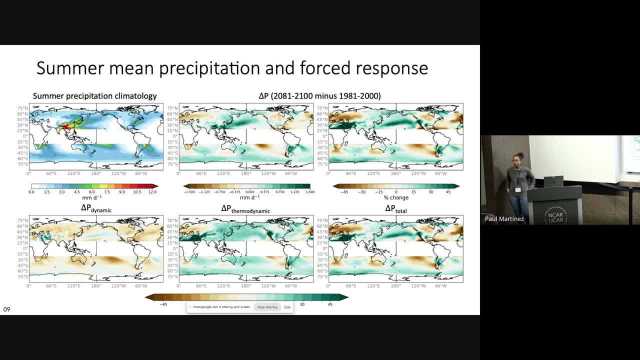 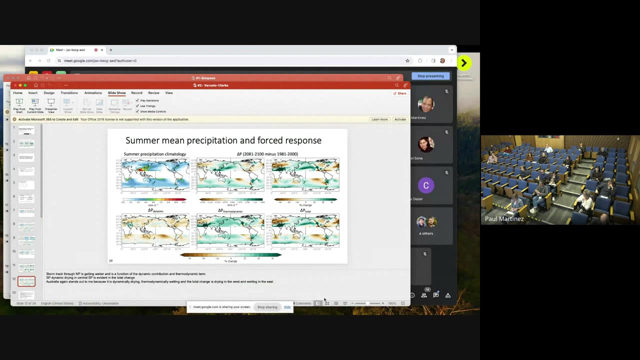 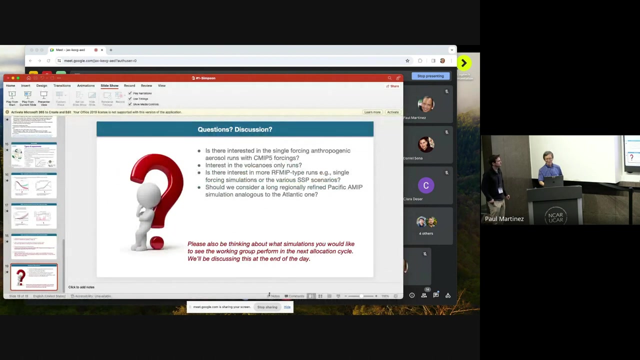 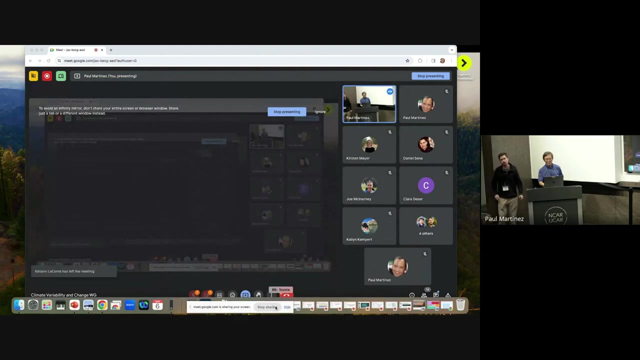 biases within those by following, just kind of getting that into gauge. okay, thank you. thank you. While he's setting this up, I'm just going to introduce myself. My name is Tim. I'm a fourth year PhD student at the University of Colorado, Boulder Department of Atmospheric and Oceanic Sciences. 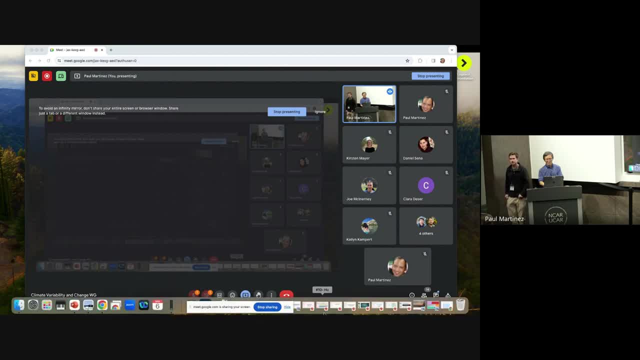 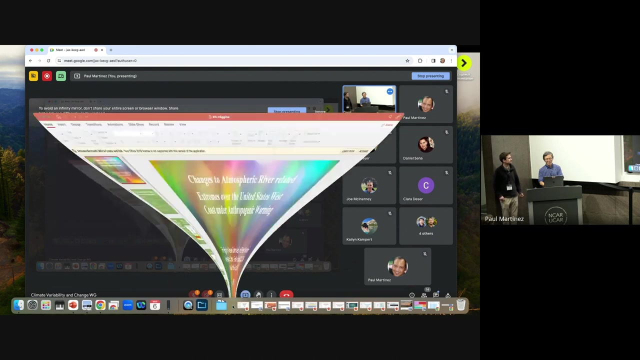 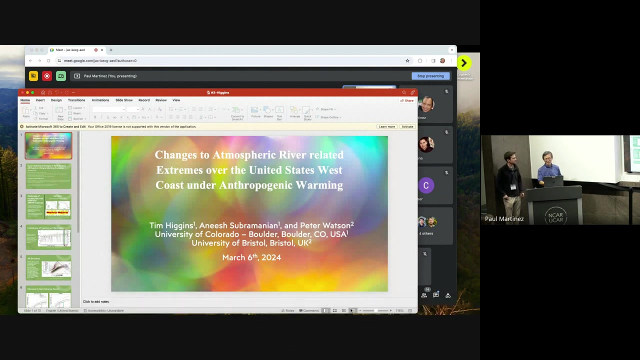 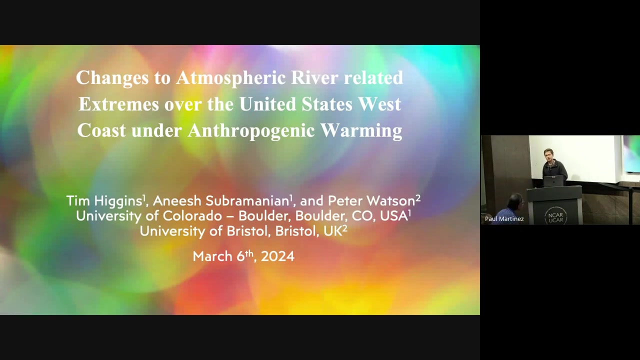 And, as of Friday of last week, I am an ASP graduate student visitor here at NCAR, So some of you are going to see more of me in the next six months. Just click on hide. Great, thank you. So for this project I focus on trying to understand some of the changes to rare, extreme atmospheric rivers. 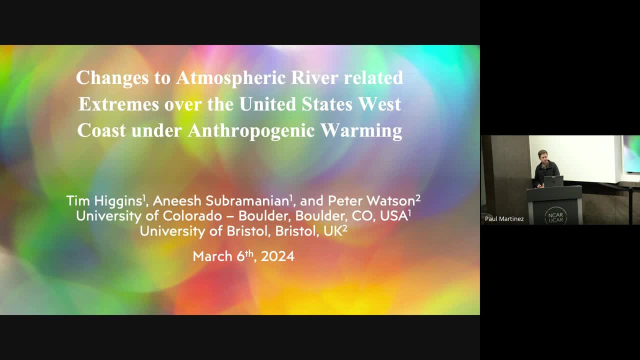 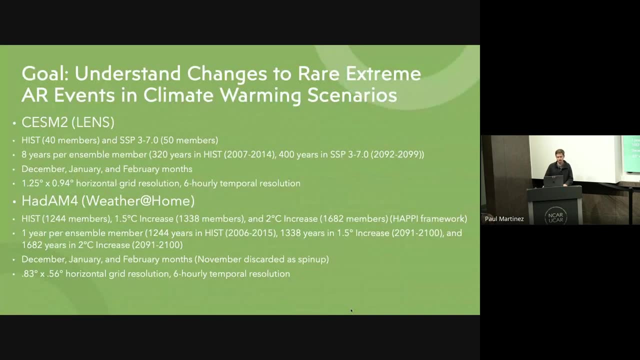 So for this project, I focus on trying to understand some of the changes to rare extreme atmospheric rivers. So for this project, I focus on trying to understand some of the changes to rare extreme atmospheric rivers, And I'd also like to give a special thanks to both of my co authors and nation Peter. 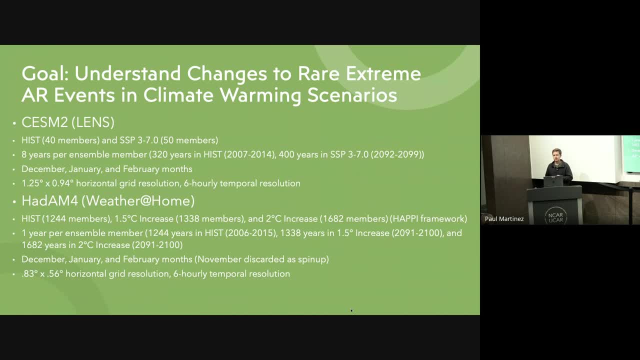 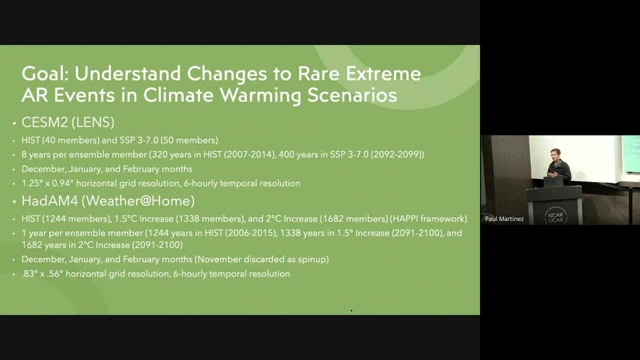 scenario. So I had eight years per ensemble member that I used for this, So 320 total seasons for the historical scenario and 400 seasons for the SSP370 warming scenario. And I used only December, January and February months because those are the months that are. 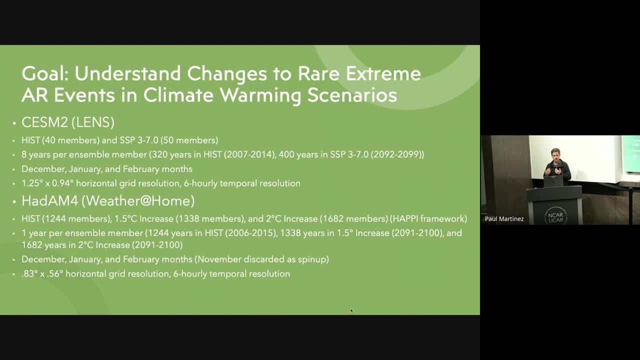 active for extreme ARs And it had a 1.25 by 0.94 horizontal grid resolution. The other model that I used came from the Weather at Home project, which used computing power from volunteers' computers to run large ensemble simulations of the climate. This particular 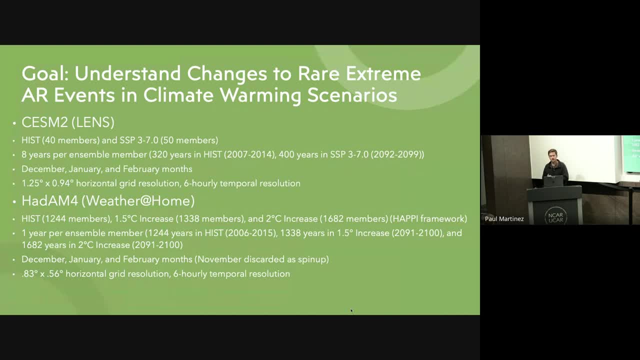 experiment used the HAD-AM4 uncoupled atmospheric model. I had three different warming scenarios. So I had historical scenario with early 21st century forcing a one and a half degree increase scenario from pre-industrial levels and a two degree increase by using the HAPI. 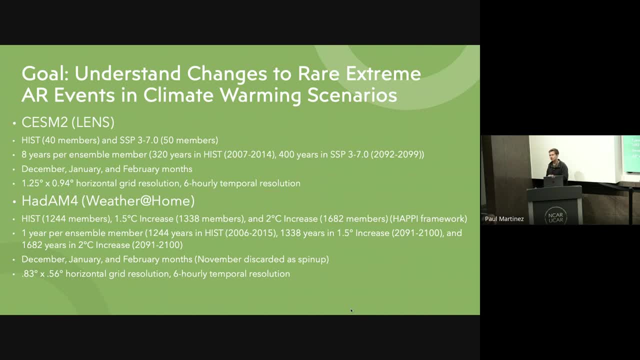 warming scenario And I used the HAPI warming scenario to run large ensemble simulations of the climate framework. I had one season per ensemble member, So November, December, January and February months. I discarded November as spin-up, so I only used BJF And 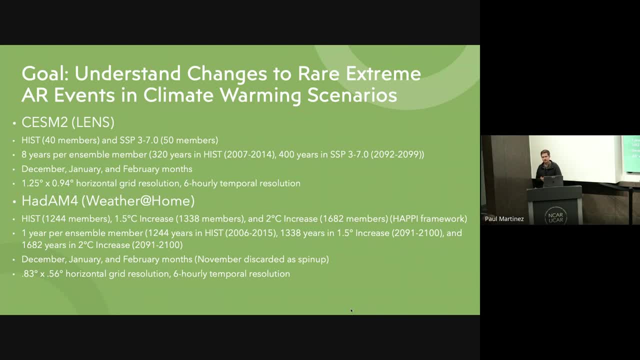 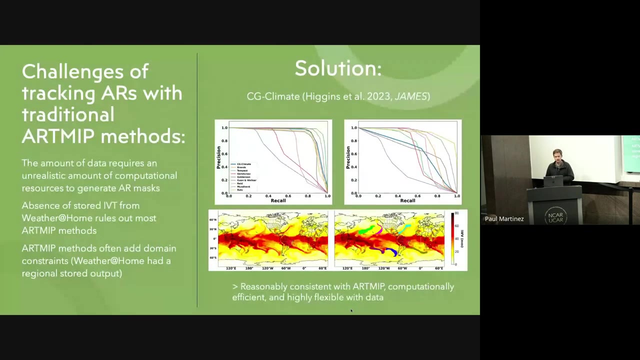 I had over 1,000 seasons for each of these warming scenarios And there was a little bit of a higher resolution with this model output. It had 0.83 by 0.56 horizontal grid resolutions. So I wanted to track ARs in this- both of these models- And I immediately ran into some. 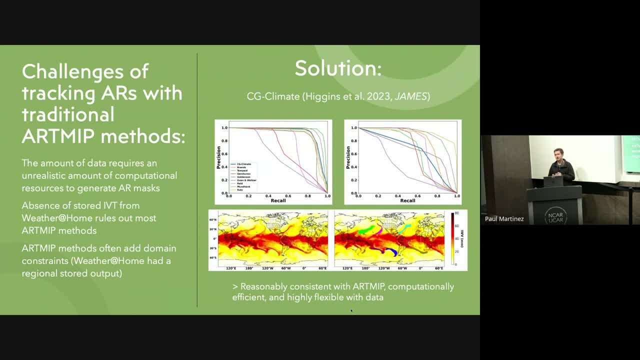 issues. So there is an atmospheric river tracking methods in our comparison project that sort of organized a lot of commonly used AR tracking methods. But I needed a lot of computational power to do this task because I had so much data And there were also some other issues. 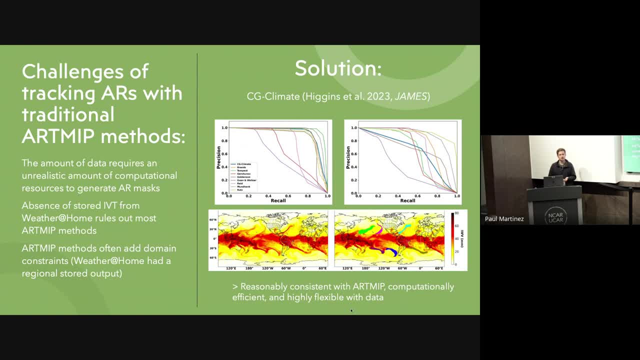 I didn't have the variables that I needed to calculate. I had integrated vapor transport, which is necessary to run the majority of AR tracking methods, And I also only had data that was stored in a regional domain for this weather at home output. So I applied a convolutional neural network. I named it CGClimate- It's. 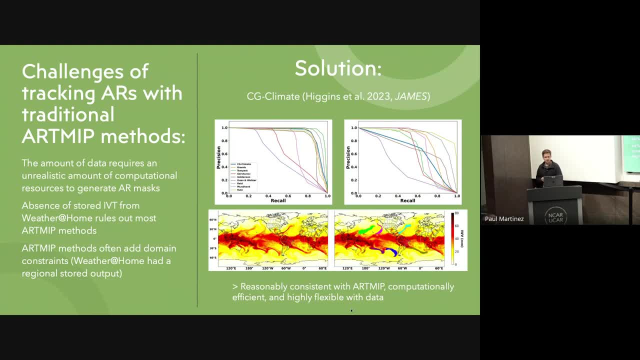 trained on human hand labels from the ClimateNet data set And I found that it's reasonably consistent with ARTMEP, It's computationally efficient and it is highly flexible with data. So that's what I decided to use. I did find that, while it is very consistent in tracking the same ARs as other methods, 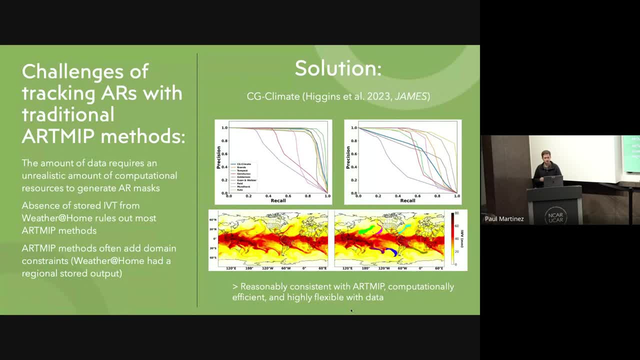 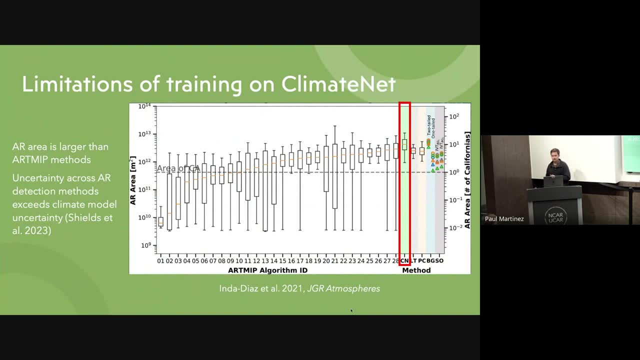 it often has a decent amount of disagreement with the exact grid points that it tracks And the reasoning for that is shown in this figure here in INDA-DS 2021.. That compares AR area across various different tracking methods And ClimateNet, which is the hand. 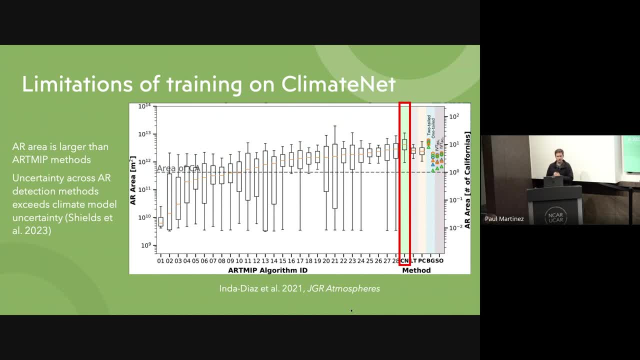 labels that I used to train. this model had the highest AR area And that doesn't mean it's wrong, but it's just different than other common methods, And it's also important to note a finding from Shield et al 2023 that uncertainty across AR detection methods exceeds. 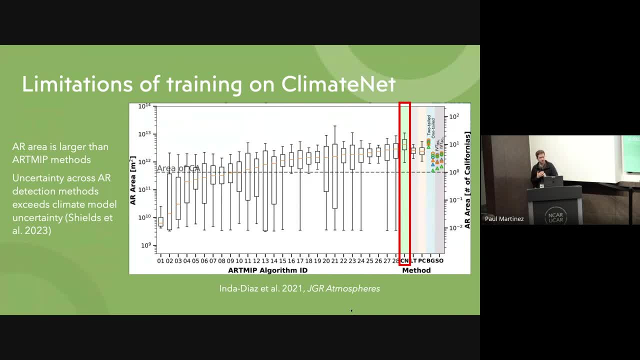 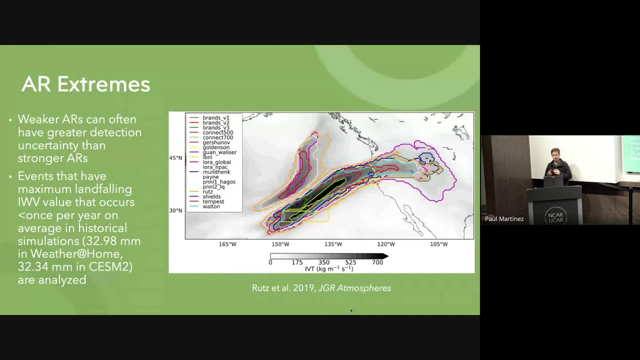 model uncertainty itself. So I had to be very sensitive to the fact that I'm using this one AR tracking method, And I want to also point out that AR area is shown on a log scale on the y-axis. So since I was only using AR extremes, I had a little bit more confidence in using this. 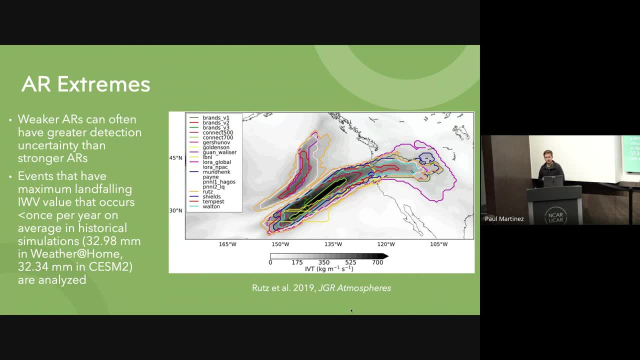 method. An example of this is shown in this figure from Rutz-Eggholt 2019.. This is the AR area. There are arguably two ARs on this screen, one towards the south and one towards the north, And you can see the more restrictive methods are more commonly going to agree that 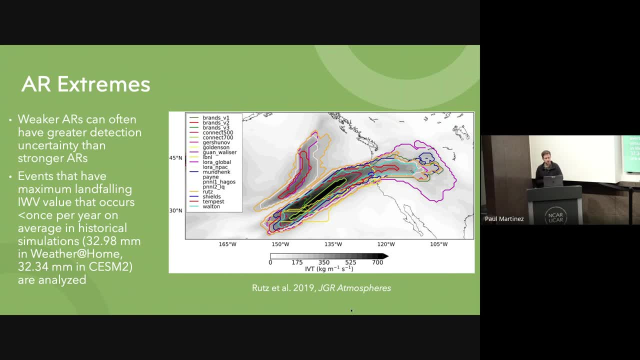 the more extreme ARs are actually ARs. You can see that almost probably maybe all the methods in the AR to the south detect an AR for that AR And then for the ARs in the north, maybe about half of the methods detected in AR. 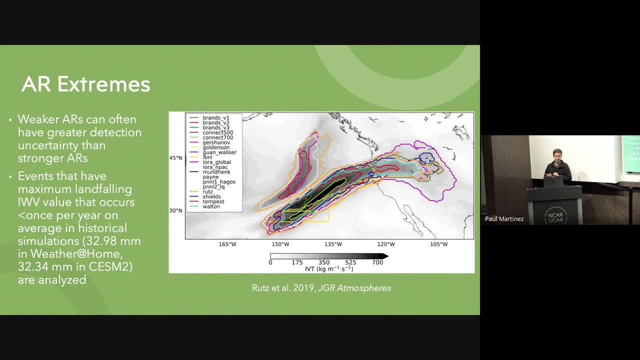 And then for my severity metric I only used the maximum landfalling AR IWB. That occurs less than once per year on average in the historical simulations And there was a similar value for that between the weather at home simulations and CSM between 32 and 33 millimeters. 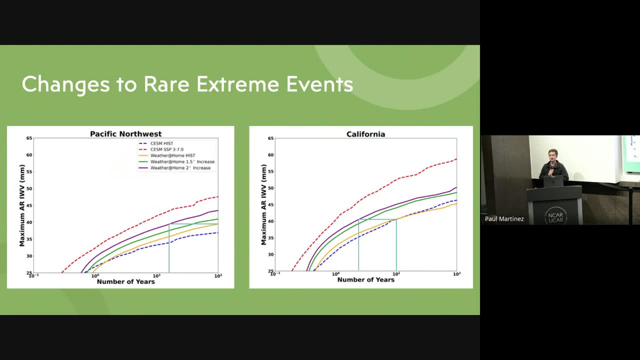 So I calculated the changes to the period, which is on the x-axis, for different severities of ARs here, And so in the dotted lines you see CSM2 results, And in the solid lines you see the weather at home simulations. So there's first of all a decent amount. 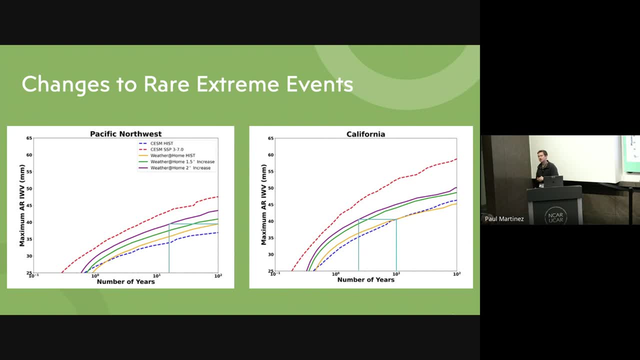 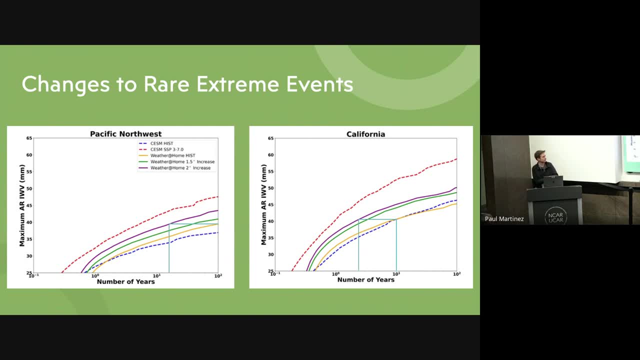 you see CSM2 results. And in the solid lines: you see CSM2 results. And in the solid lines: is it the top button? yeah, you have to, i think, hold it for some time at the screen and then maybe try and transfer it over. that's not working. oh, you're good. yeah, so i'm referring to this. uh, dotted blue. 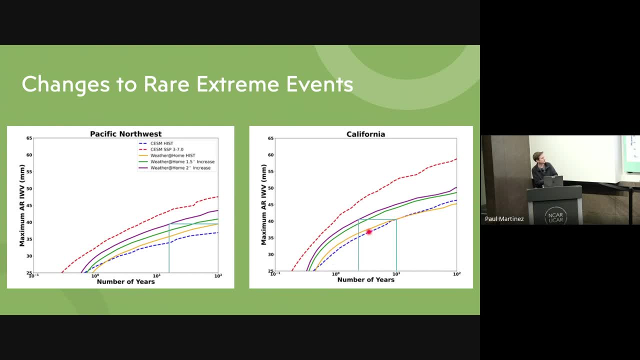 line and a solid yellow line are both the historical simulations for extremes in california and we see a decent amount of agreement between them, even despite having a little bit of a different resolution. so this same result did not really come up when i looked at precipitation extremes due to these resolution differences. and then we see for these three ssp370 scenario: 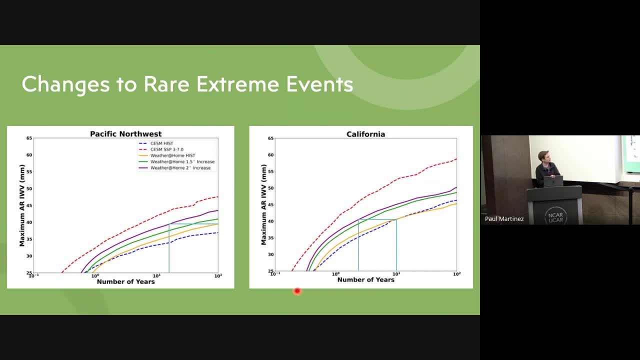 certainly many events happening once every 10 years or so that are completely unprecedented we've never seen before. and then, looking at just these weather at home simulations, we see almost an order of magnitude increase in frequency or an ar at any given severity. so once every 10 year event here happens, about every one once every uh. 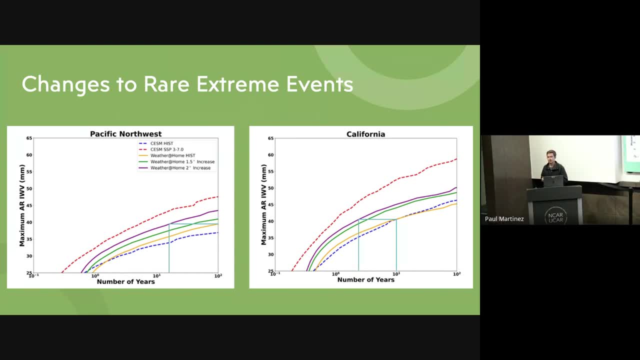 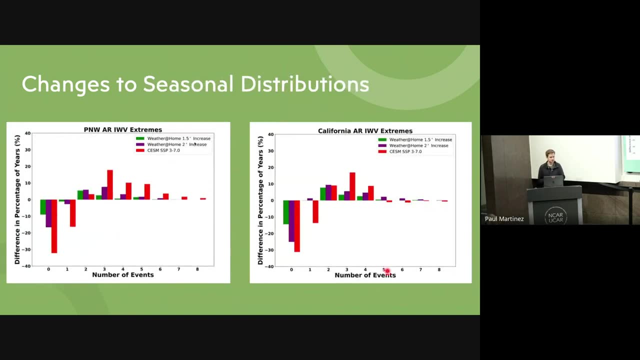 two to three years and it's just this two degree increase from pre-industrial levels. then i also wanted to look at changes to seasonal extremes. so here i'm not showing the percent difference but the difference in percentage of years in which we see x amount of events in the 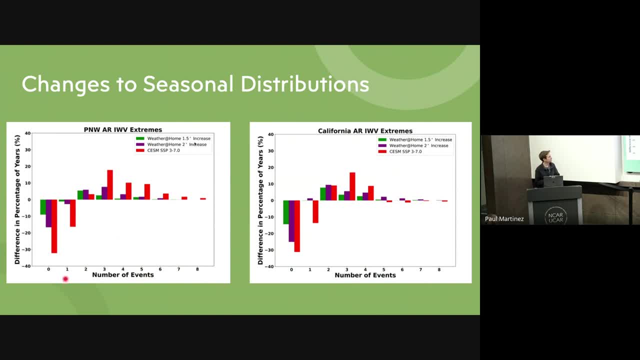 same season, x amount of extreme events. so the overall takeaway here is that when we use the warming scenarios, whether it's the ssp370 or the more mild one and a half degree or two degree increase scenarios, we see far less seasons in both the pacific northwest and california, where there are 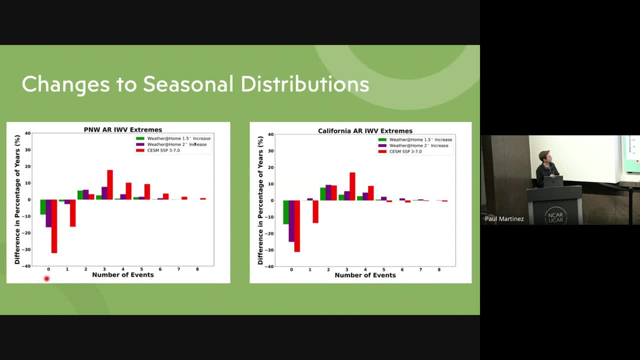 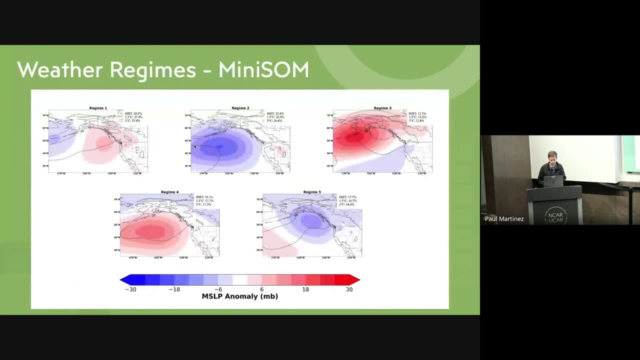 zero extreme events in one season and far more seasons where there are two plus extreme events in any given season. so a couple things that we also included. uh, first is鄺 for大概, but then i was curious to see how these wonderful 아 nadir 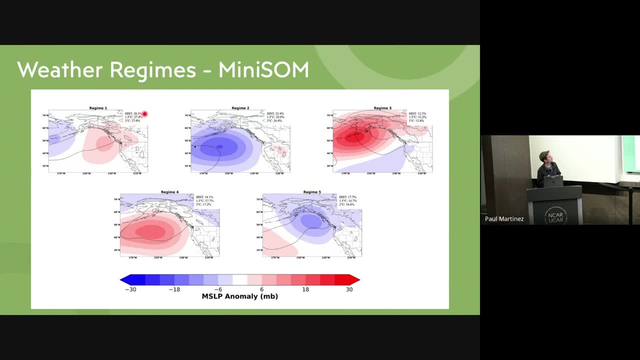 extreme help for � eighteen x new so the latest z also sleep in the percent of the time in the historical scenario and the unshaded contours represent the change in mean sea level pressure for each regime so there really wasn't a lot of change one maybe two mil bars and some in some regimes and then 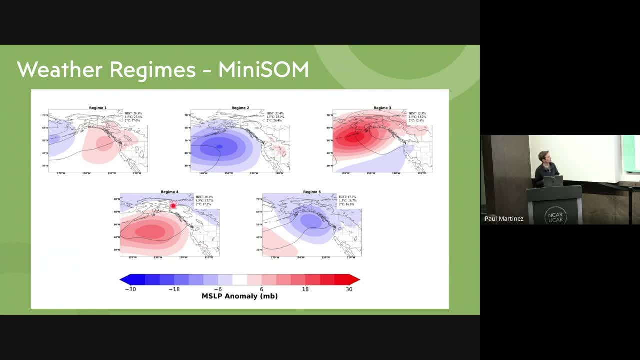 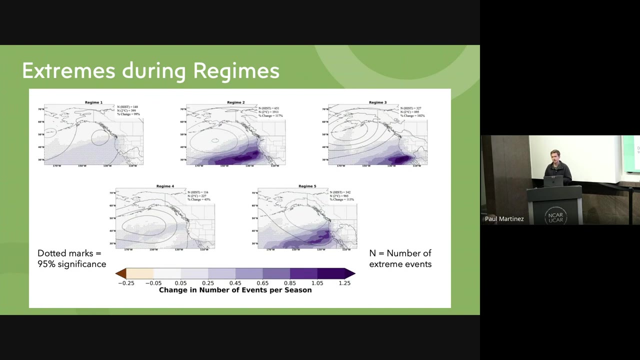 the change in percentage of regimes also did not fluctuate too much. what I will note is regime number two went from twenty three point four percent of the data to twenty six point four percent of the data, and that is also a very active regime for extreme AR activity. so looking at these extremes during regimes, 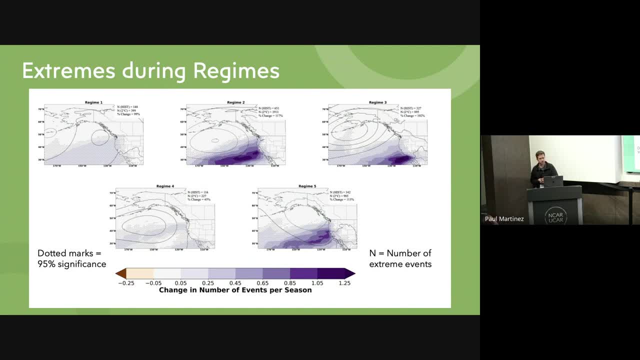 I thought it changed in number of events per season and I used dotted marks to indicate 95% significance, using a student t-test, and then these numbers at the top are the number of extreme events that occurred and then the percent change is the percent change in the number of events per season. so, overall, what we see. 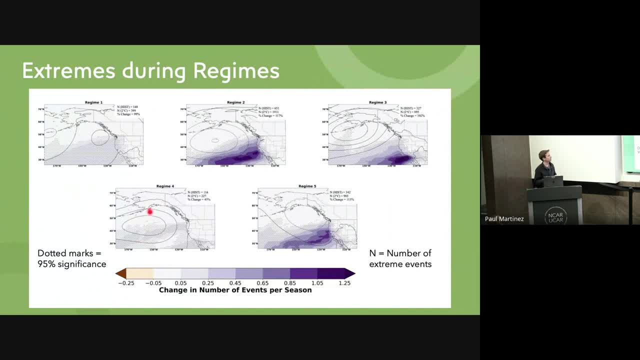 here is that regime four, for example, which was not a very active regime for AR activity, had the lowest percentage change in extreme ARs, whereas a regime two, which was the most active regime for AR activity, had the largest percentage change in ars, with 117 percent change in the number of ars. 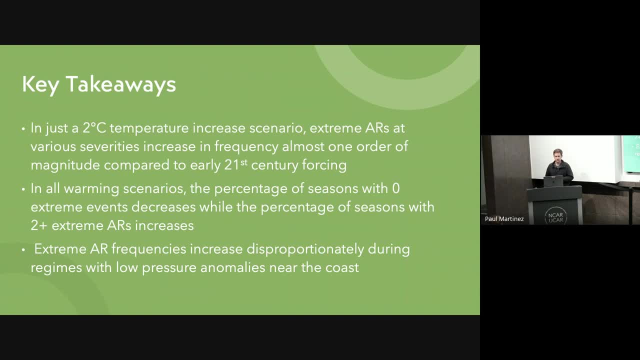 so to summarize here in just a two degree temperature increase scenario, extreme ars at various severities increased in frequency almost one quarter of magnitude compared to early 21st century coursing. i found that in all warming scenarios the percentage of seasons with zero extreme ar that decreases, while the percentage of 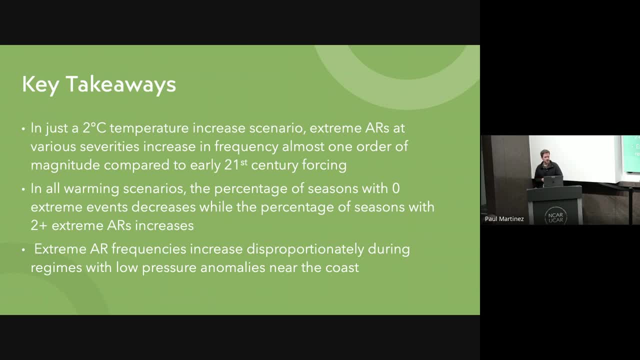 seasons of two plus of extreme ars increases and i found that the extreme ar frequencies increased disproportionately during regimes of low pressure anomalies near the coast. and that's all i have. thank you for listening and i'm happy to take any questions. i just wanted to make sure the sense of 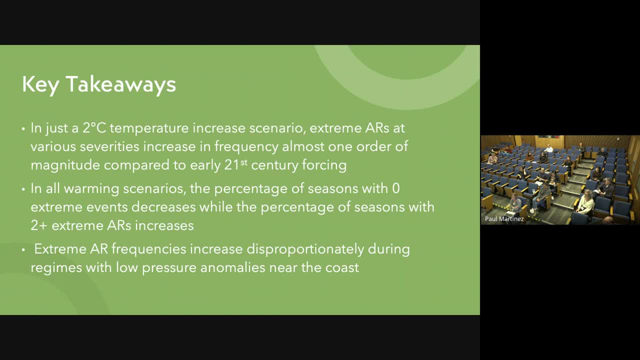 like ensemble spread and whether there's any chance of detecting changes already in that one observational record. um, it was kind of difficult to look at ensemble spread with these rare extreme events because they happen so increasingly so it's hard to really get a robust metric on that. okay, so you think it would be kind of impossible to 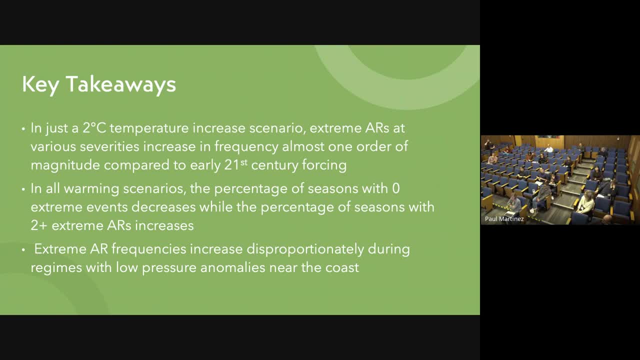 see in the future. i guess you would need a longer on like more ensembles and longer ensembles, um, with like kind of the same consistent forcing uh over here. yeah, i guess i'm curious how many ensembles you need, because- and then also curious about resolution, so 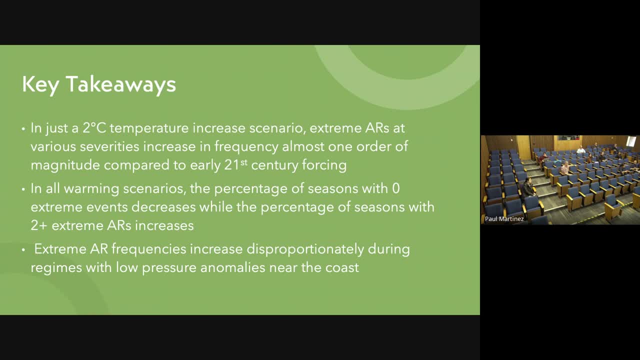 i'm wondering what would happen if you looked at this in the in this quarter degree atmosphere, 10-3 ocean ensemble over csm-1 that we're putting together and we're going to get up to 10 ensemble numbers there, so very computationally expensive experiments that pedro was talking about. 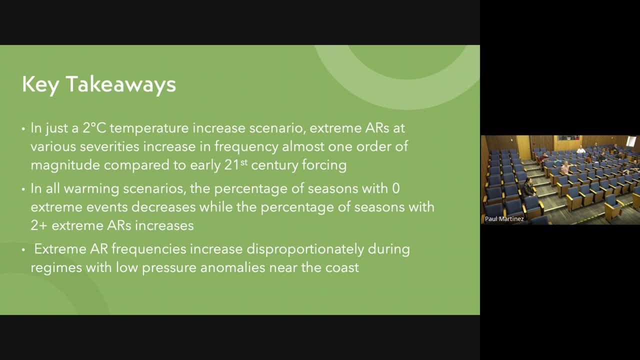 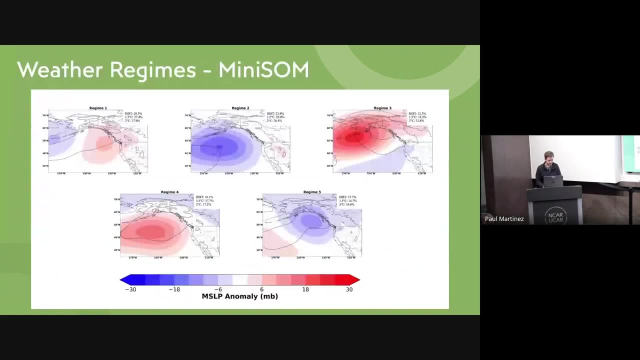 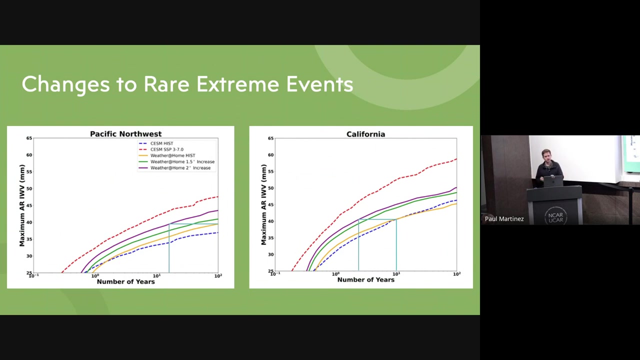 um will that be sufficient, and whether or not you expect that different signal. and so the um. so the spatial resolution, um, i think, if we're just looking at iwv extremes, integrated water vapor extremes, um, we i wouldn't necessarily expect to see a completely different result. 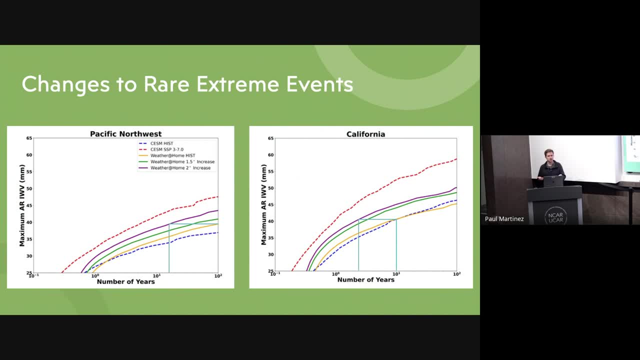 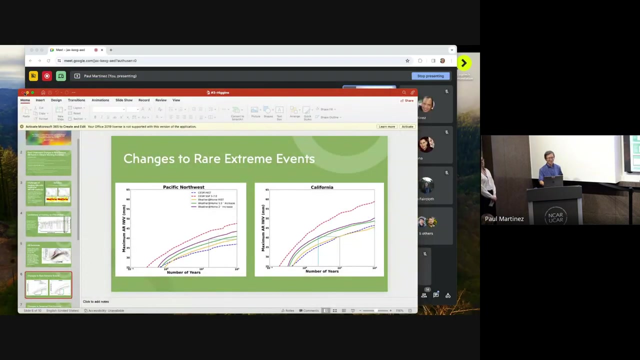 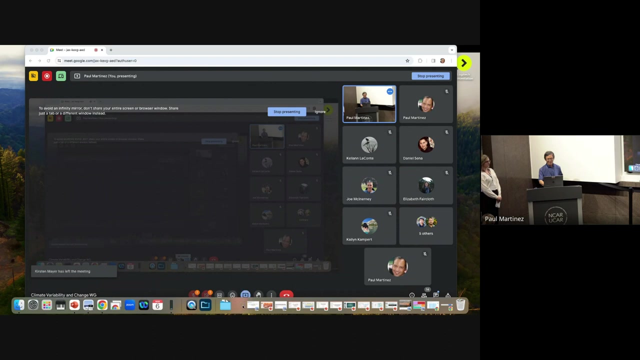 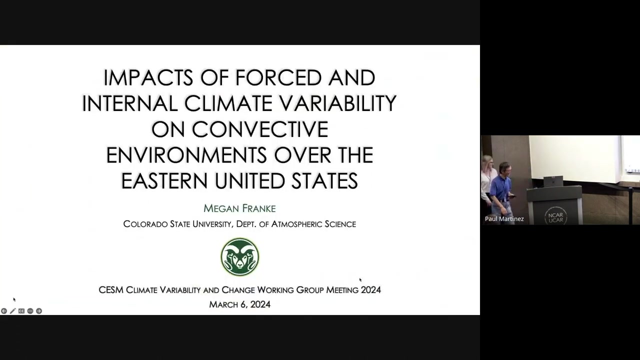 increasing the resolution. but if you wanted to look at precipitation rate extremes, a quarter degree would certainly give you a much more realistic idea of how those extremes could change. does that answer your question? three months, no questions, great, thank you. uh, next time we begin by making this one. 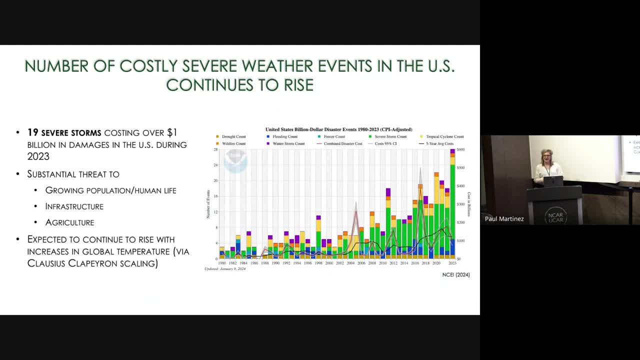 hello everyone, good morning. um, i'm going again. my name is megan franke and i am a phd student at colorado state university, working in jim harrell's group. so i just want to take a moment to thank the climate variability and change working group for putting this session on. 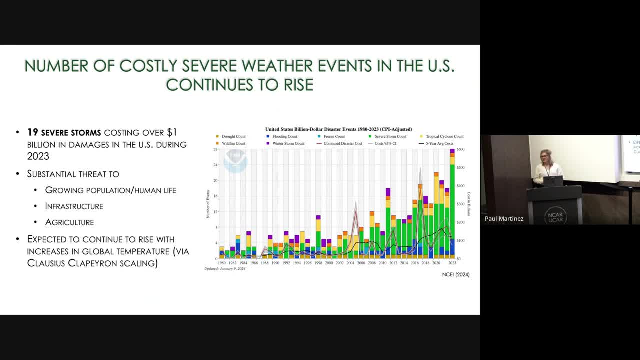 for us today giving me the opportunity to present, so with that, i'll go ahead and, uh, dive right on in. i guess i didn't realize that it moved on without me. um, so, yeah, hopping on in. as we can see, over the last um several years, the number of severe weather events has been increasing quite 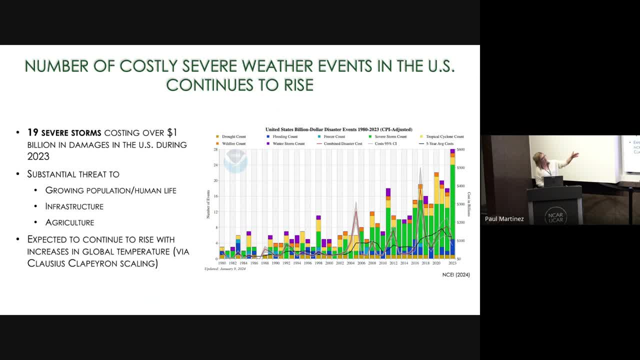 substantially over the united states. we can see here in these green columns um, or the green in the columns, are specifically severe weather events and then the other colors represent different types of disastrous weather. so um here this figure shows the number of billion dollars severe weather events um per year, so for the year 2023 alone. just last year there was 19 severe 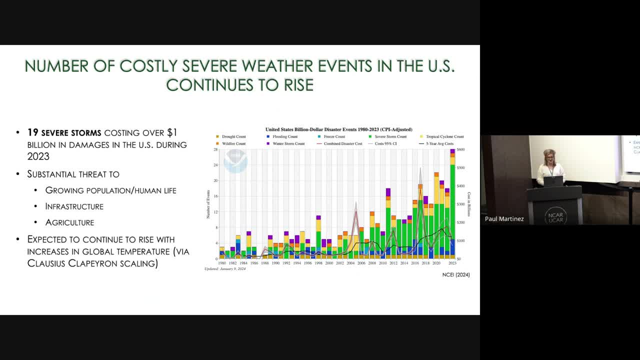 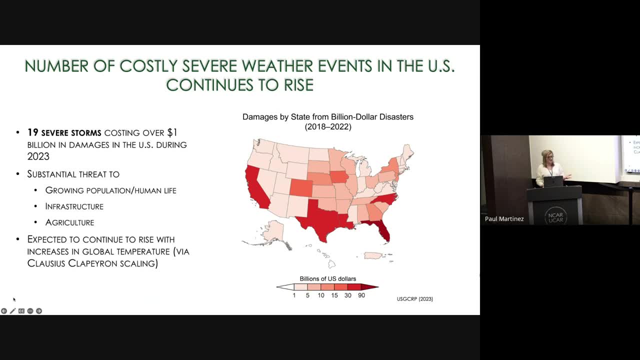 weather events costing more than one billion dollars in damage over the united states. so, um, interestingly enough, uh well, i guess. consequently, these events tend to occur in areas over the midwest, the united states and the eastern united states which cause a substantial threat to the population, human life in those areas and um the infrastructure, as well as the. 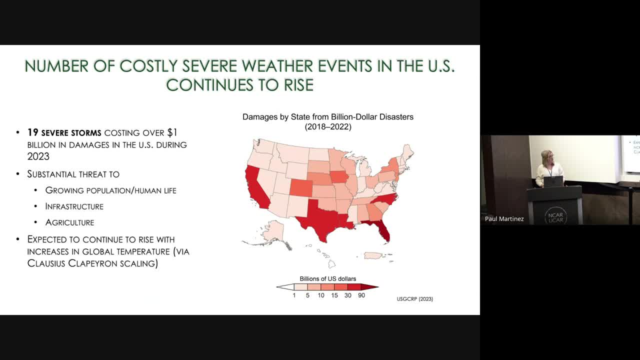 agricultural rich, rich land. so these uh costly events are expected to continue to rise as global temperatures continue to increase due to the clausius capitol scaling. so because of that, it is paramount that we take the time to understand how thunderstorms and these convective environments are likely to evolve in future warmer. 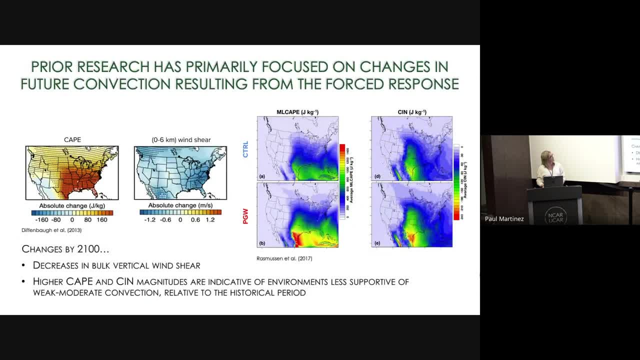 climates. okay, so there has been some prior research that has looked at this, but most of this research has focused mainly on the forced response. um particularly different at all. 2013 used the cmf5 ensemble mean to look at changes in conductive available potential energy by the end of the 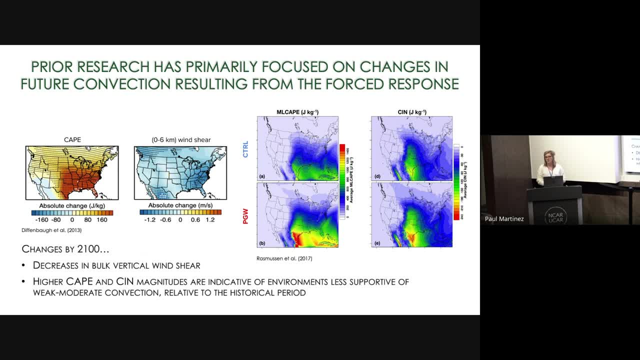 century, as well as zero to six kilometer wind shear, both of which are going to be seen here, both of which are critical for convection to occur, and that can be seen here in these two figures on the left. additionally, another study done by rasma 2017. 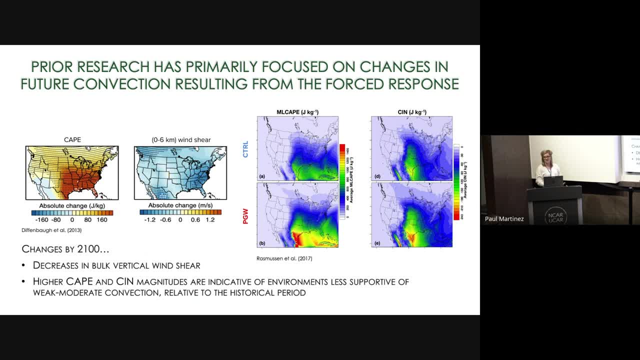 um investigated changes in connected population as well as thermodynamic environments by the end of the century, but they used um convection permitting regional climate models instead. um, although one thing we can see is, even though both of these methodologies were quite different, changes in cape which can. 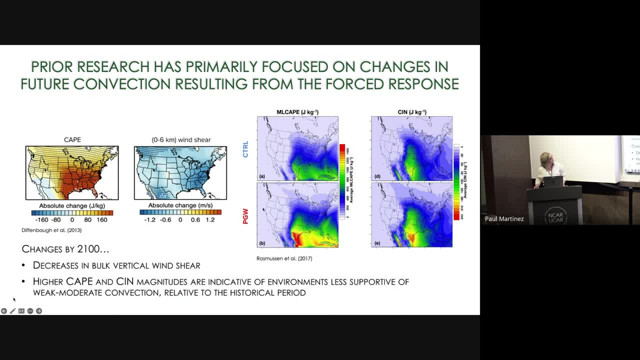 be seen here on the left, well right here in this column, as well as here on the left. changes in cape by the end of the century are quite comparable between these two studies, with higher cape and indicating more explosive energy for these thunderstorms to develop. so, as i mentioned, most prior research has focused on changes in the forced. 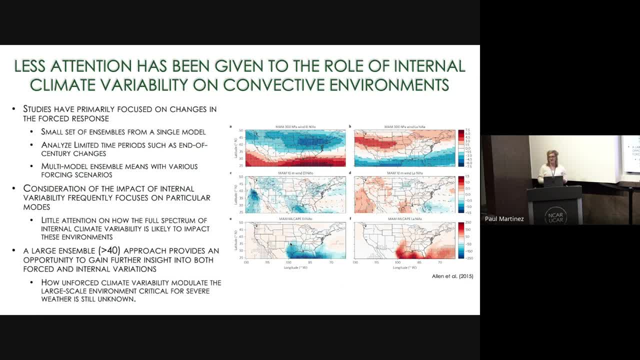 response. using either a small set of ensemble members analyzing a limited time period, or using a multi-model ensemble mean to measure a specific time period that has various forcing in future scenarios mixed in. quite less attention has been given to the impact of internal variability and the attention that it does receive. 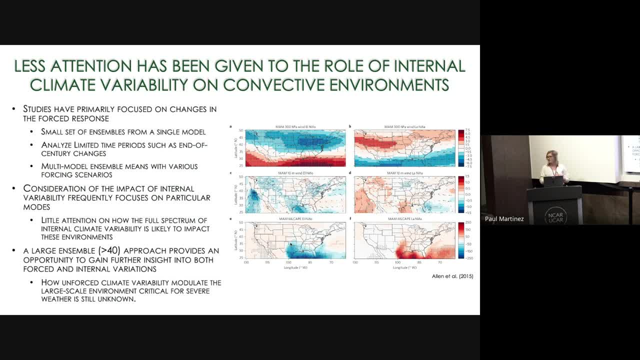 frequently focuses on specific modes of variability. so, for instance, this study by allen et al in 2015 investigated how the el nino southern oscillation impacts different convective variables over the united states in this boreal spring season. so you can see that during el nino events on the left column here. 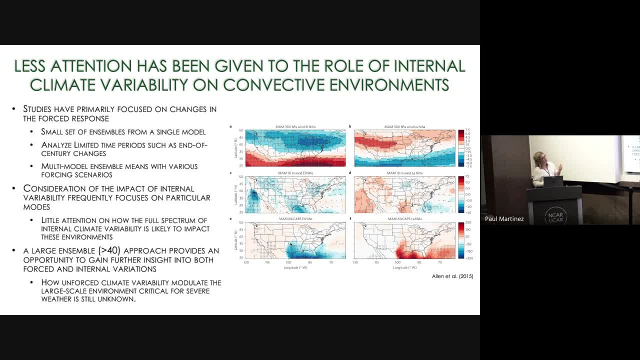 Winds aloft at 300 hectopascals typically tend to be a lot slower than normal Winds at the surface a little bit slower, but not much of a change. And then the values of CAPE during springtime in El Nino events are anonymously lower as well. And then of course, the opposite is true during. 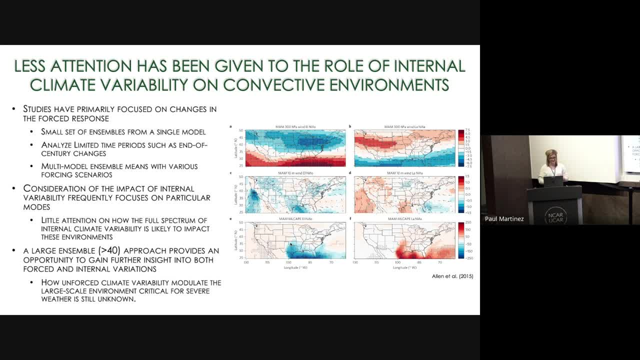 La Nina events which we can see in the right column. So, as I mentioned, very little attention to that internal variability aspect with looking at these studies, And particularly there has been really no attention given to how the full spectrum of internal variability is going to impact these convective environments, Which fortunately that gives me a great opportunity. 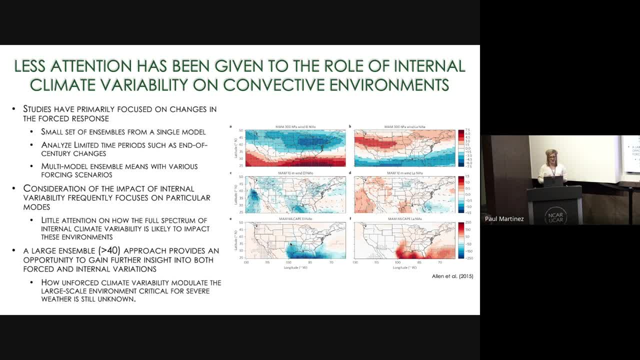 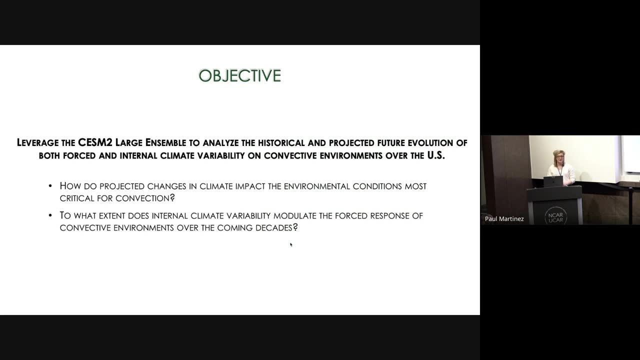 to utilize the large ensemble approach to really investigate how both of these components of our climate system work together to modulate the convective environment over the United States. With that, I'll go ahead and dive on into the objectives of this study. We wanted to leverage. 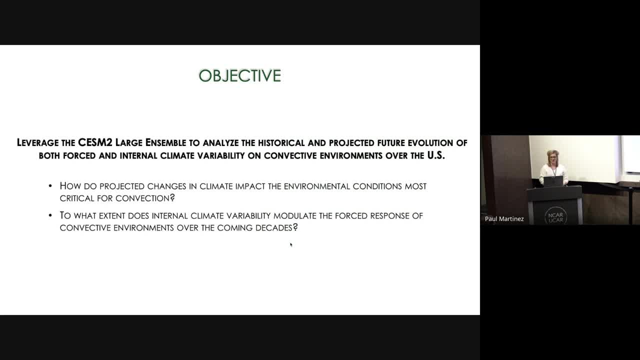 the CEF 72 large ensemble to analyze the historical and projected future evolution of both force and internal climate variability on convective environments over the United States And particularly, we wanted to answer these few questions: How do projected changes in climate impact the environmental conditions most critical for? 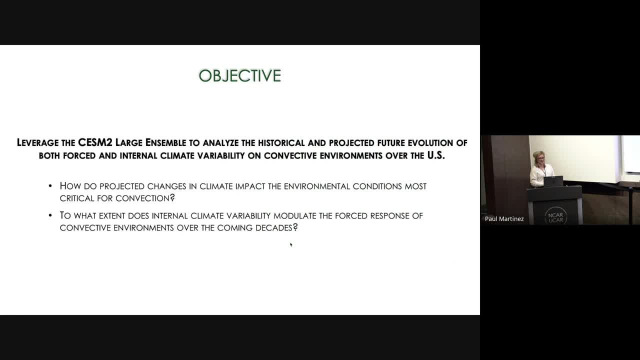 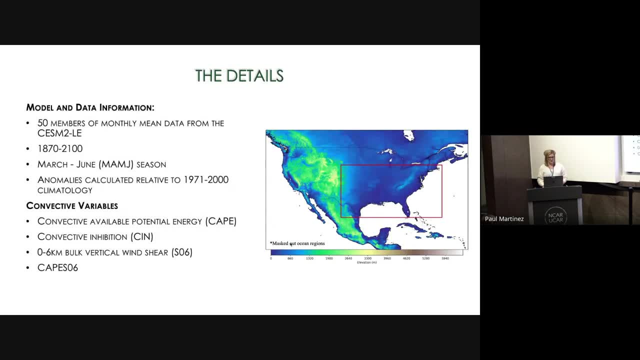 convection And, furthermore, to what extent does internal climate variability modulate the force response of convective environments over the coming decades? So just getting into some of the details of this project, here, As I mentioned, we use the CEF 72 large ensemble, specifically the first 50 members of this ensemble, the monthly data. 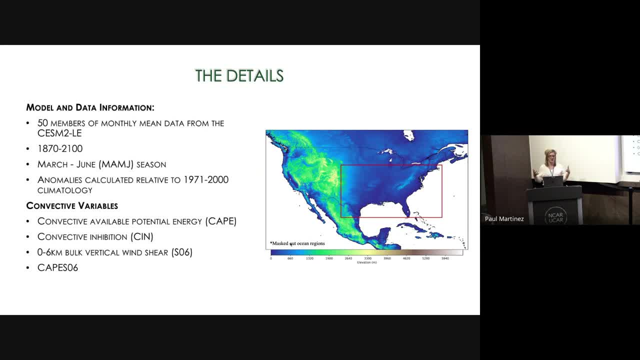 We use the period 1870 to 2100, pretty much that full time period that the data set was available at the time And specifically we were interested in the months of March, April, May, June, as this season is the most convectively active season in our region of interest, which is highlighted here. 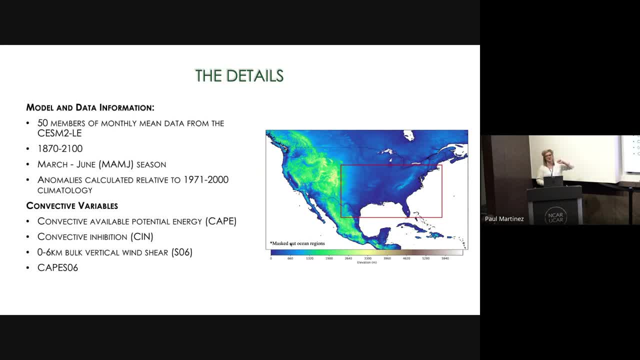 in this red box in the figure. I do want to note that the ocean regions were masked out for this whole analysis. So, in particular to analyze our convective environments, we looked at these four different variables. I'm sure a lot of you are familiar with them, but I'll just give a quick overview in case. 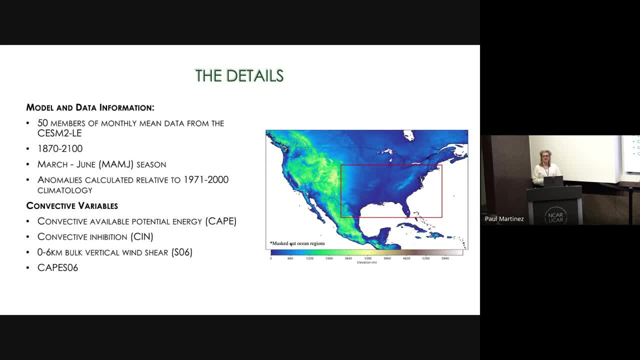 I know this is more of like a climate focused talk. So there's conductive available potential energy, or CAPE, which is the integrated measure of buoyancy in the atmosphere. The conductive inhibition, or the SIN, which is just the energy a parcel needs to overcome to be able to freely. 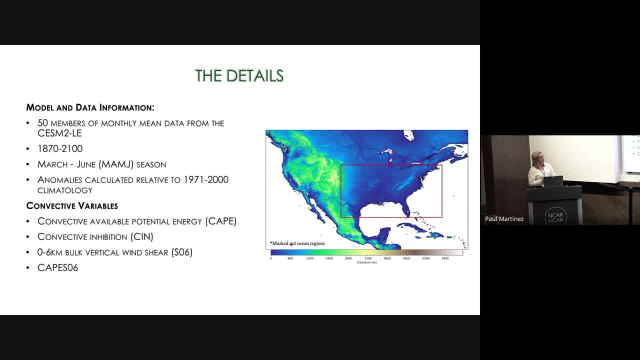 conduct The zero to six kilometer wind shear, both vertical wind shear, so just the difference of the wind speed at the surface in six kilometers. And then finally the product of CAPE and SO6, which is commonly used to distinguish and diagnose between different storm severities. I do want to make a quick note on the conductive 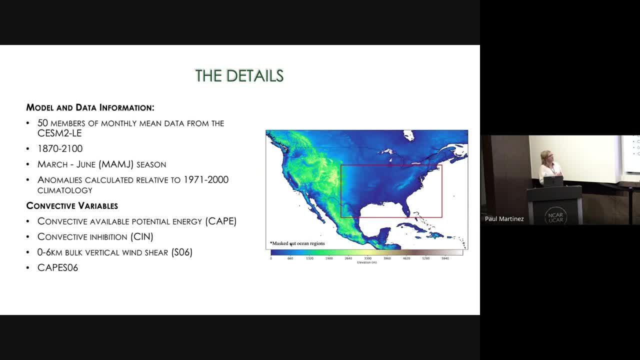 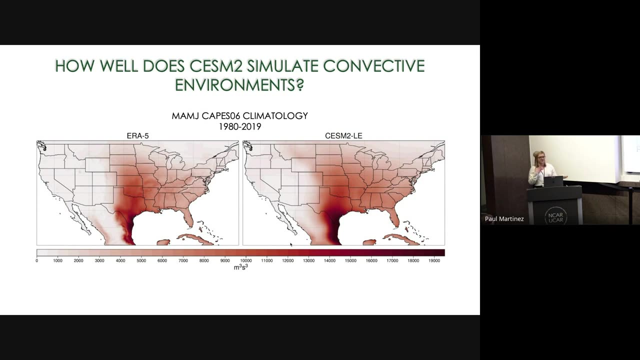 inhibition, As this parameter is typically defined as a negative value. any time we see a decrease in this means that we are actually obtaining more SIN in the atmosphere and therefore a more stable atmosphere. So before we dive quickly into the results, just wanted to evaluate exactly how well 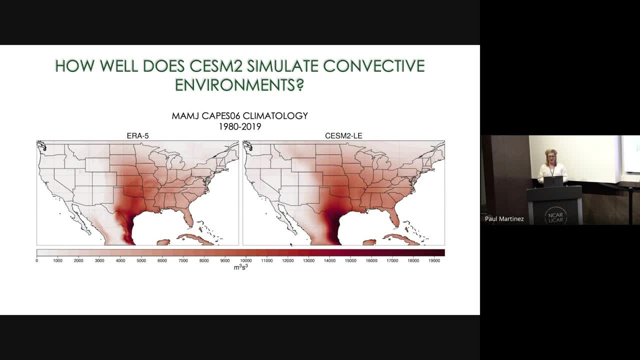 does the CESM2 do at capturing these variables we're interested in? So here we have just the March, April, May, June CAPE SO6 climatology for the full reanalysis record 1980 to 2019.. And, as you can see, there is a pretty spatially coherent similarities between these two models. 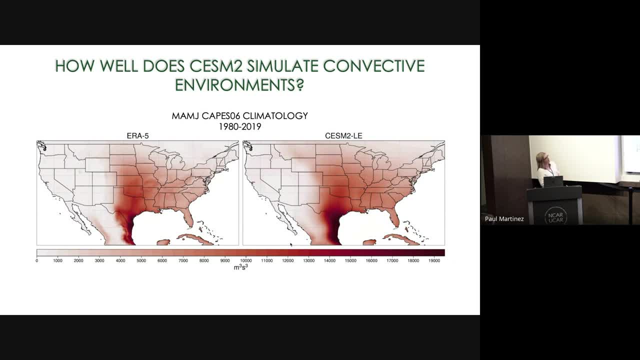 ERR5 and CESM2 large ensemble, as well as a similarity between their magnitudes. I do want to note that, although CESM2 large ensemble looks like it has a lot more SIN, the CESM2 large ensemble looks like it has a lot more of a robust signal, particularly over 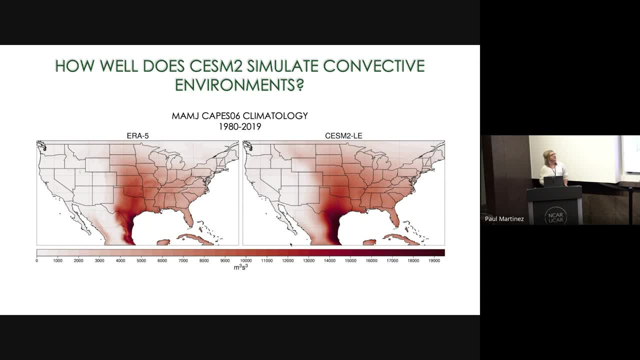 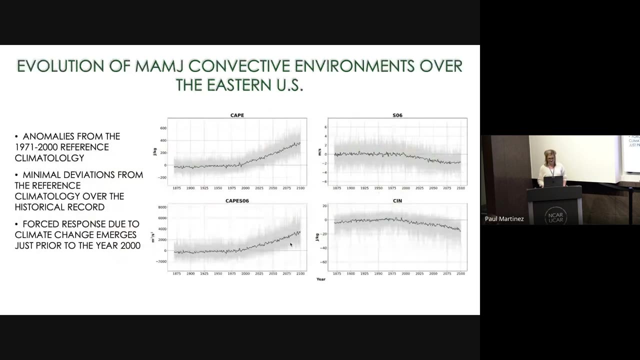 eastern Texas and the central Great Plains. This was created using the 50-member ensemble, mean so there's 50 members comprised in this calculation, whereas ERR5 is obviously just one single representation of reality. So here we have, our time series of different anomalies for our 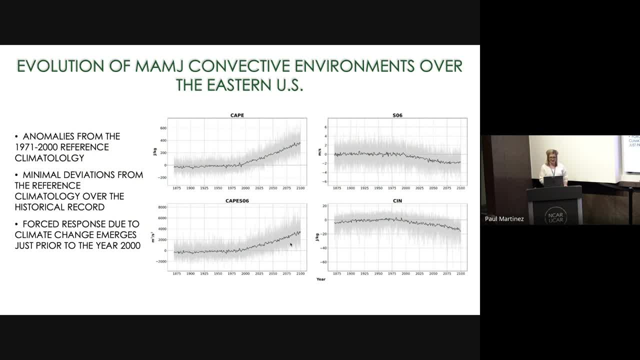 conductive parameters, all relative to the 1971 to 2000 climatology. We can see in the light gray in the background that there is a pretty substantial deviation between inter-annual and decadal variability in our light gray lines and those all represent the 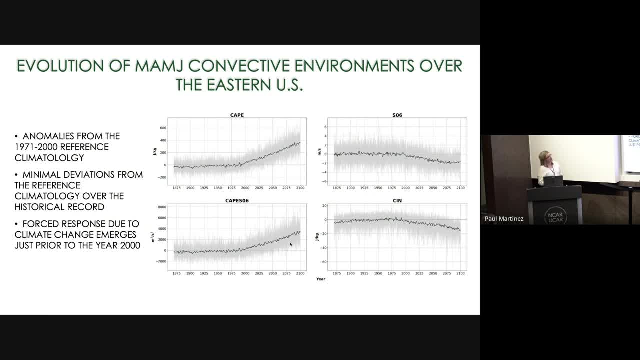 single 50 members. If we turn our attention instead to the solid black line that represents our ensemble, mean We can see there is very little deviation of our ensemble. mean signal throughout the historical record up until just prior to the year 2000,. 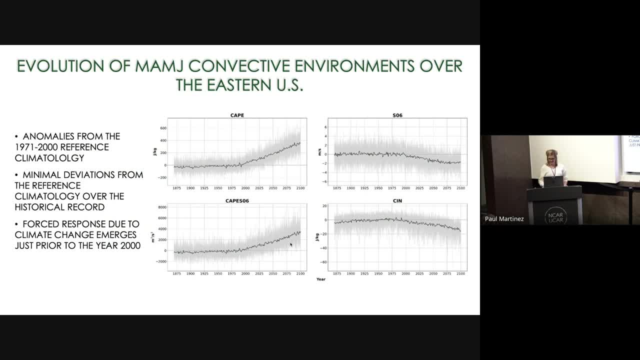 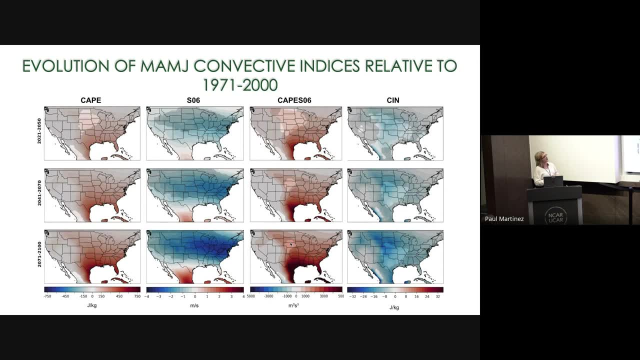 where that signal begins to emerge, And then just kind of taking another look at that same thing. this is just the anomalies of our conductive parameters over time, plotted spatially. So up in that first row we can see there are coherent increases in both CAPE and CAPE-SO6. 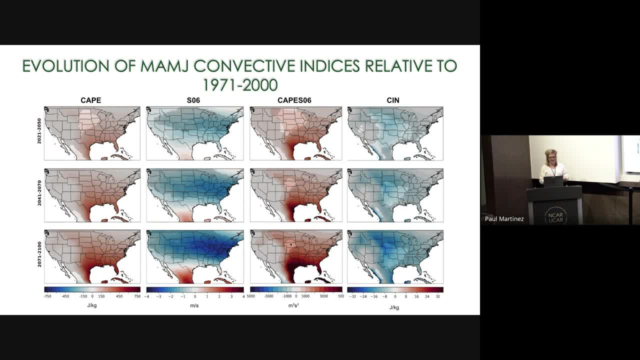 in the near term, with decreases in SO6 and SIN, And we can also see that these changes in CAPE-SO6 look to be particularly driven by the changes in CAPE rather than SO6, which I think is something to keep in mind. And then we can also see that these changes in CAPE-SO6 look to be particularly 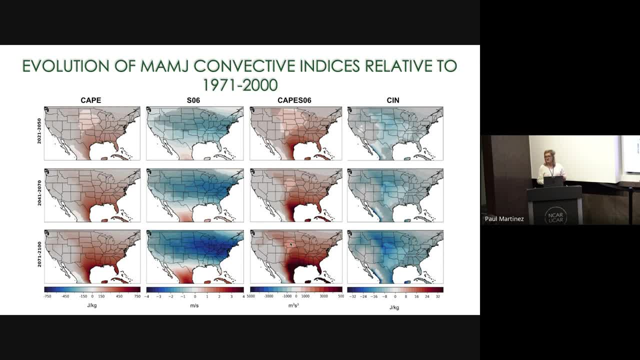 driven by the changes in CAPE rather than SO6, which I think is something to keep in mind. As we move forward times to the middle of the century, which is seen here in our middle row, we can see that these changes just continue to strengthen for all four of our indices And 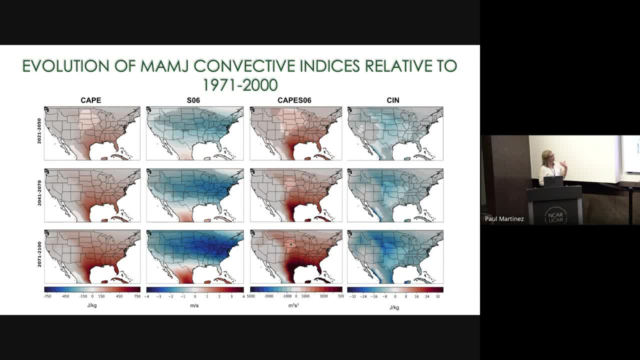 then, finally, by the end of the century 2021,, we can really see these strong increases in CAPE and CAPE-SO6 along our Gulf Coast and the southern plains, And then large decreasing swath of SO6 to the northeastern United States, over the whole country really, And then a main target of 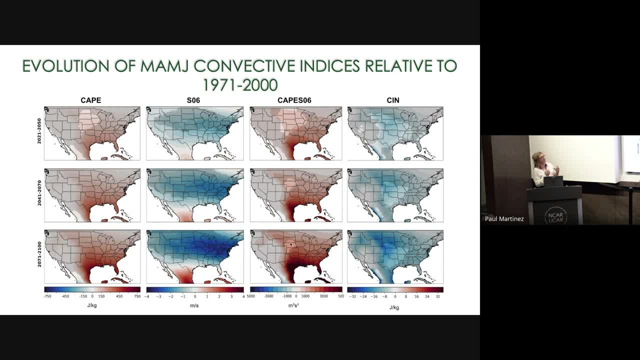 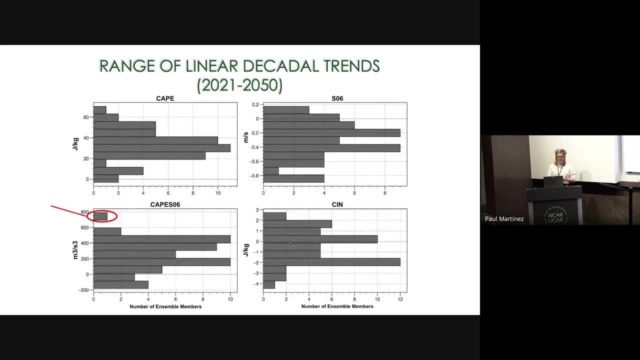 decreasing or higher magnitudes of SIN, And then a main target of decreasing or higher magnitudes of SIN over the central and northern Great Plains. So, taking this a little step further, I calculated the linear decadal trends for each of these conductive indices for all 50 of the ensemble. 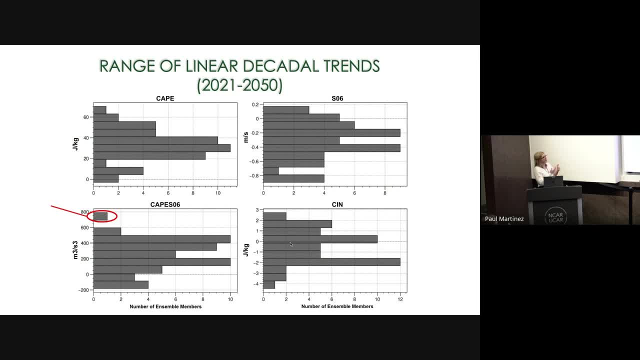 members. So here in these histograms it just kind of gives us an idea of exactly how many ensemble members project the different types of trends. So for instance, all 50 members are projecting a positive trend in the next 30 years. And then the next 30 years, all 50 members are projecting a. 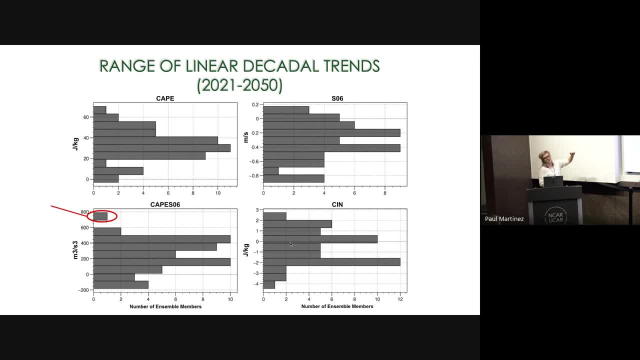 negative trend, Whereas for SO6, only about a third of the ensemble members project positive trends. We move down to SIN. we can see that it's pretty much a 50-50 split between positive and negative trends over the next 30 years. And then finally with CAPE-SO6,- sorry about that. 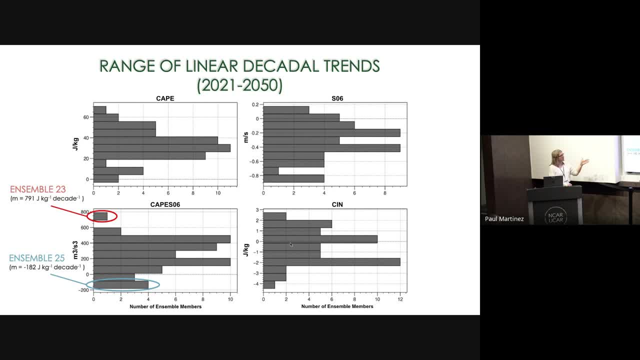 nearly 17 of our ensemble members, or nearly seven of the ensemble members, produce a negative trend, whereas the other 43 members are all projecting positive trends over the next 30 years. So, as I mentioned, a goal of this research was to really investigate the role of internal climate. 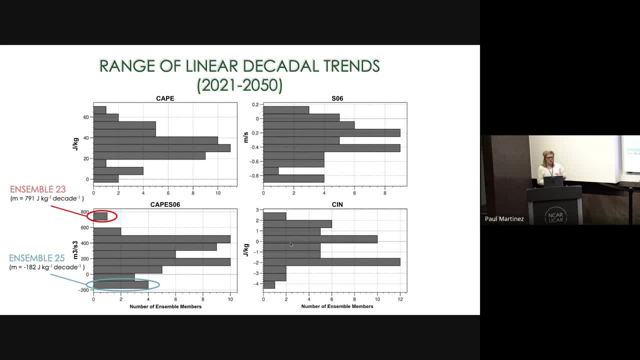 variability in modulating the forced response. So to do this we selected the two most extreme ensemble members of the 50. So we can see here ensemble member 23,, which represents the strongest trend over the next 30 years of CAPE-SO6, and ensemble member 25,, with the smallest. 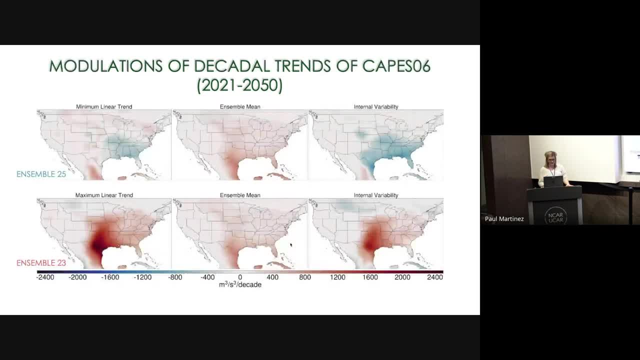 trend of CAPE-SO6 over the next 30 years. So here, as I mentioned, we have ensemble member 25, that low trend and number 23 on the left-hand side, If we simply subtract our forced response or the 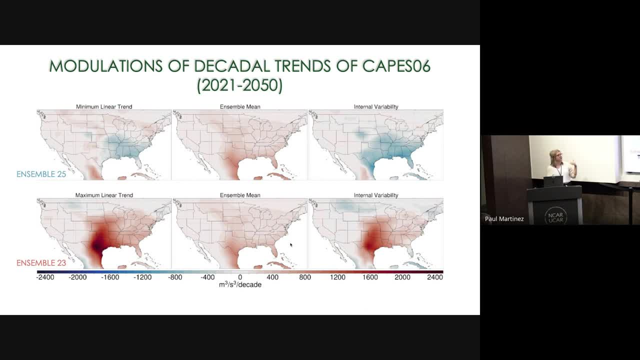 ensemble mean from each of these members. then we're left purely with the changes due to internal variability which we can see on the right-hand side in our column, Specifically kind of diving into this and looking at how internal variability impacts this. on the top row we can see over the 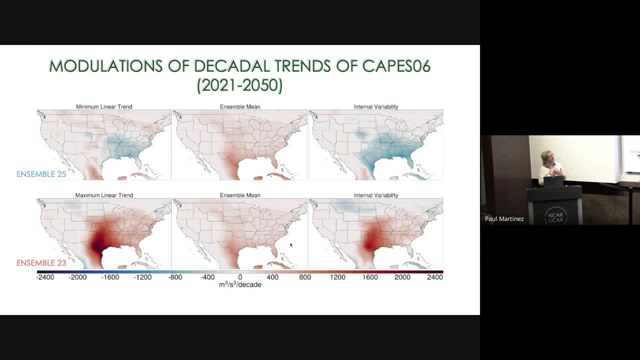 southeastern United States. that negative trend from internal variability tends to counteract the trend due to the ensemble mean, leaving us with overall and negative trends of CAPE-SO6 and ensemble member 25 in this simulation. Similarly, if we move down to our maximum linear trend, 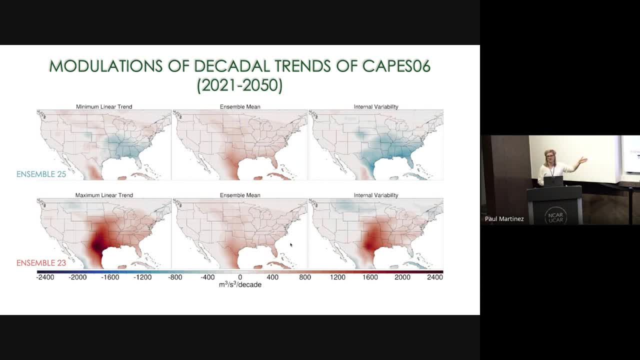 we can see that the internal variability actually acts to augment the forced response, leaving us with an even higher trend for CAPE-SO6 over the next 30 years, particularly over Texas and the southern plains. So with that, I'll go ahead and leave you with a 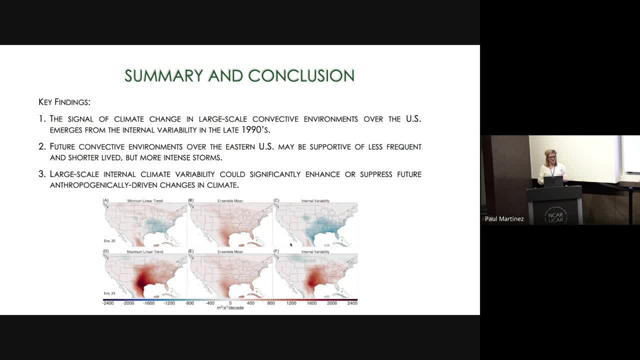 few of our conclusions and findings for this study. First of all, the signal of climate change in large-scale conductive environments over the United States emerges from internal variability in the late 1990s, just prior to the year 2000.. Number two: future conductive environments over the eastern United States may be more supportive of less frequent and shorter-lived, but more intense storms. And I come to this conclusion because, as I mentioned, we have really strong increases in CAPE, which I said is important for the buoyant energy of the storm, Of course. 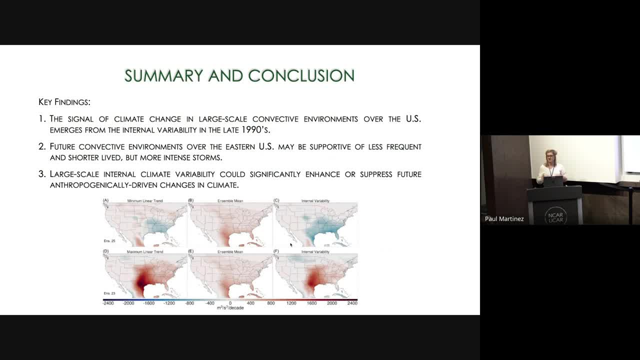 we also have strong increases or decreases in the magnitude of SIN. So in the future, as we have a more stable atmosphere but more accumulation of conductive available potential energy, once that energy is finally able to break through the CAPE, the storms can be potentially a lot more. 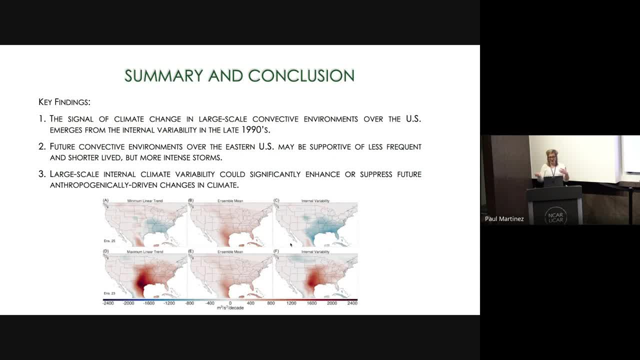 explosive and more intense. And then, finally, our third point was that large-scale internal climate variability could significantly enhance or suppress the future anthropogenic-driven changes in climate. And then, finally, our third point was that large-scale internal climate variability could significantly enhance or suppress the future anthropogenic-driven changes in climate. And then, 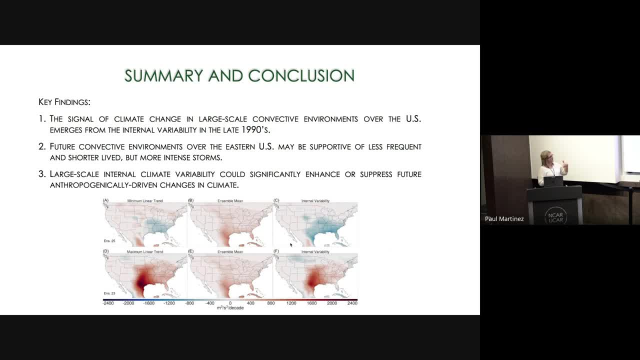 I think that was really really well demonstrated by the figure that I talked about in the last slide, which I just kind of posted up right here to keep in your minds as we go through the questions. So with that I'll just thank you all again for joining us today and thank you again to 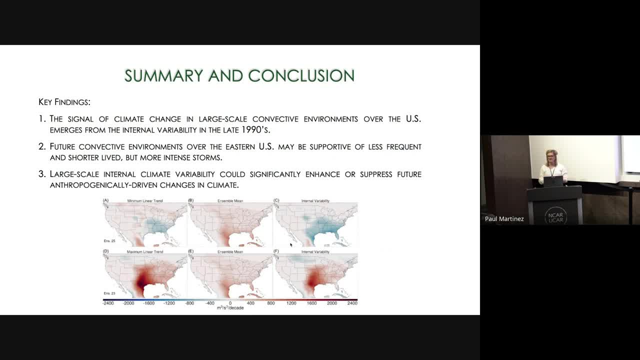 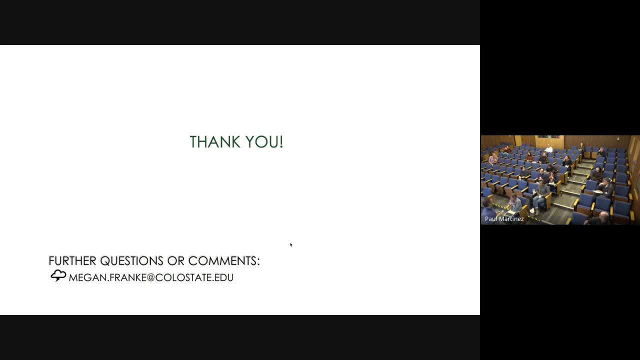 the Climate Variability and Change Working Group and I'll go ahead and take questions. I'm wondering what the time series of the internal variability part looks like. Is it like a steady linear trend going in that 30 period, or is it almost like a spike during the first or the 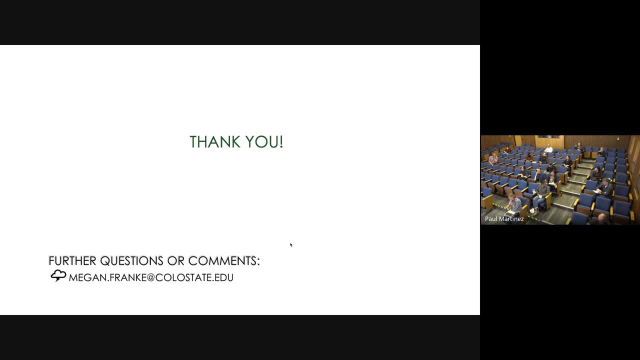 second bit of that time series that's mean to what looks like a trend but maybe doesn't have a strong R squared Right, So I actually didn't look at that, but that seems like something really interesting that I might dig into. The only time series that I really took the time to look at was 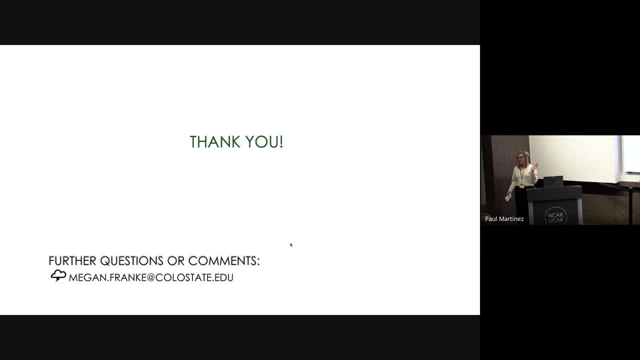 that one that I showed you initially. that showed all 50 of the ensemble members, the spread of that as well, as then the ensemble mean. But I do, I think that is a really interesting idea. I might dive into that, see what I can find. Thank you. 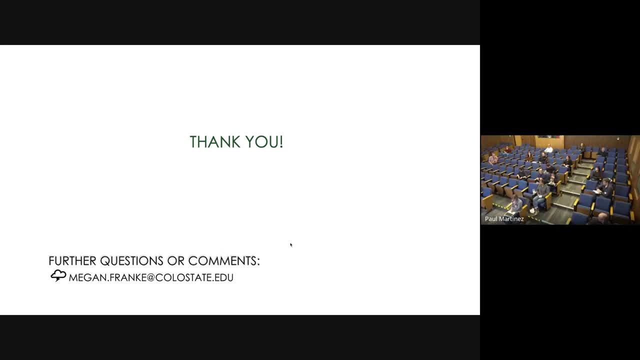 I'm wondering: you looked at the mean values. If you were to look at the extremes and like CAPEs in that kind of product index, how do you think it would change, given that I guess the extreme events are more on like the tails of the distribution of this variable? 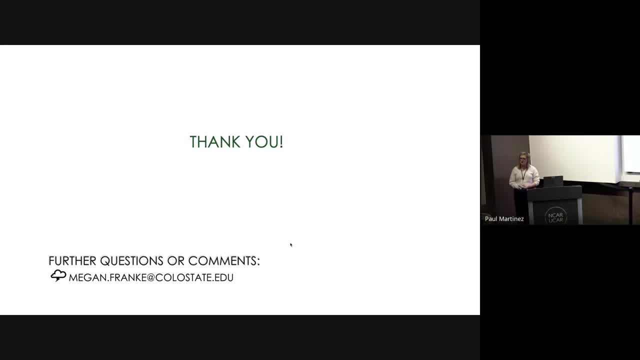 Like, how do I think it would change in what sense? Like, if you're looking at CAPE but the 90 percent of CAPE, do you think that the results would be consistent? Would there be, like greater increases in CAPE in the forced? 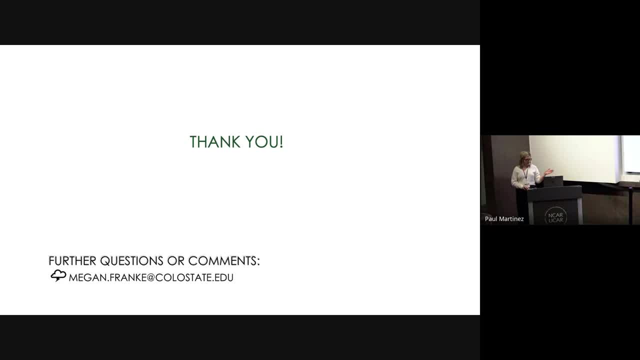 response. I see. So I actually on one of the figures I should have mentioned there was: I did use a statistical significance test on it And it does appear that by the end of the century that those changes are really becoming more significant as time goes on. I don't know if 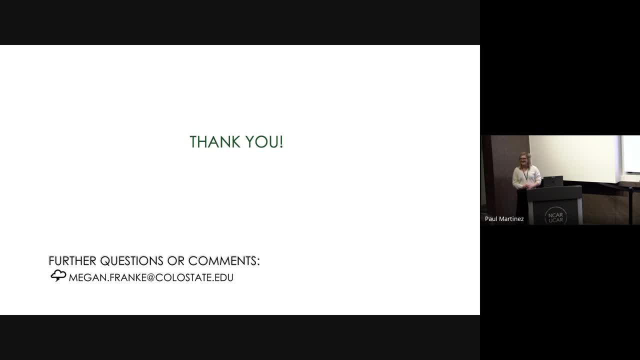 that necessarily answers your question and what you're asking. Yeah, I'll find a way to phrase it Totally. Yeah, we can talk later on or during happy hour. I was wondering why you think you didn't see any changes going up to your baseline, So you're using like 1980 to something. 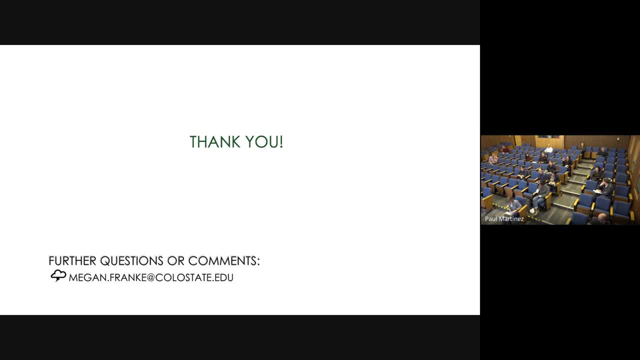 Yeah, to about 2000.. 2000.. And so I was wondering if you've thought about why there you maybe didn't see any changes in. it seemed like you didn't see any changes in your variables leading up to that. Is there maybe like an aerosol signal in there, Or 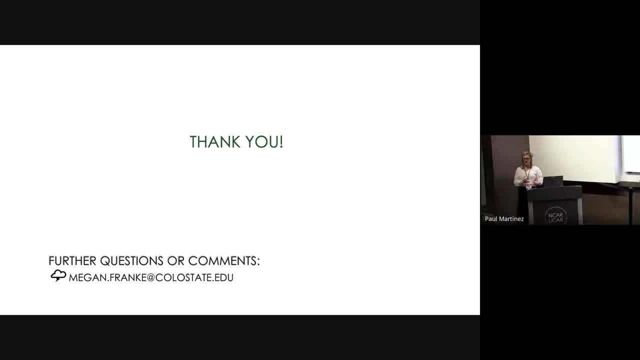 something like that. Yeah, I think that we are kind of under the impression that at that point in time, that's when the external forcing from greenhouse gases really begins to take over and emerge from the background noise, And so that is kind of our hypothesis at the moment of why it. 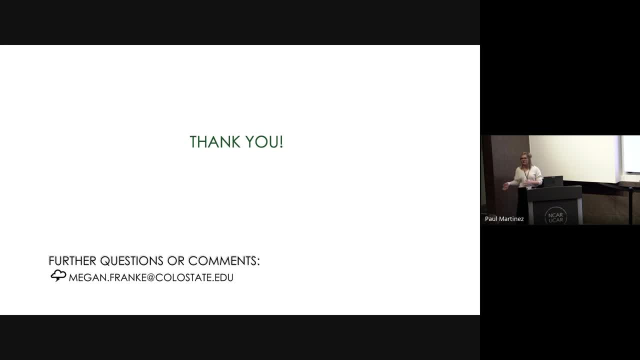 didn't really change anytime in the historic period up until that point. Thank you, I think it's the same kind of question that others are asking, which is I'm trying to understand. you know you've really got a trend. What's driving that? What are the like, the mean state? 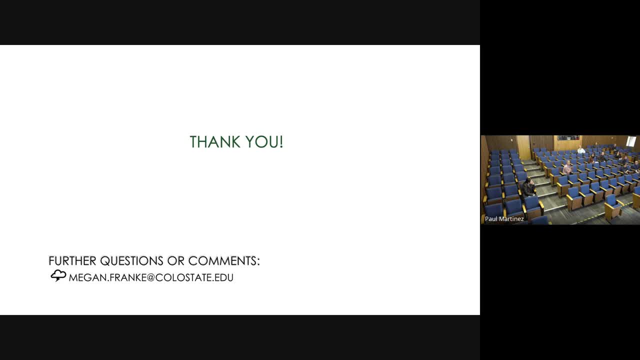 or the mean state trends are sort of driving that and asking the question whether or not that's what's controlling whether or not you're getting the increase in severe storms versus, you know, the extremes happening more frequently. I again also can't quite answer the question. 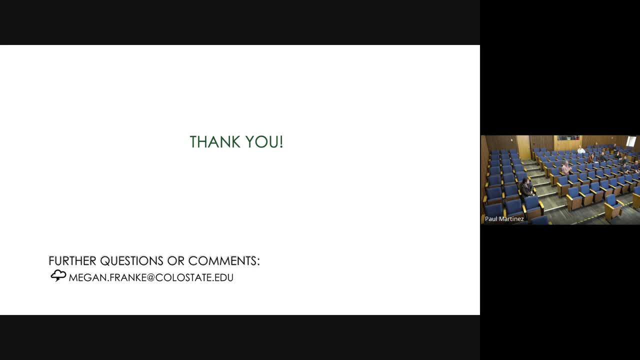 But I kind of feel like there's something in there that maybe needs to be explored a little bit further to understand. you know how that? what is it looking Like on a on a season by season basis? you could imagine one season having a lot of severe events. 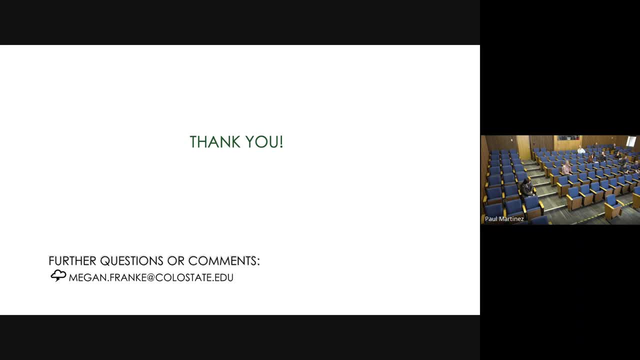 the next one not having it and it's showing up as a trend but not really being a trend. And yeah, I'm sorry I might ask also, quite asking or like if the distribution changing. Yeah, Maybe It's something like that. Yeah, it is kind of they're in your 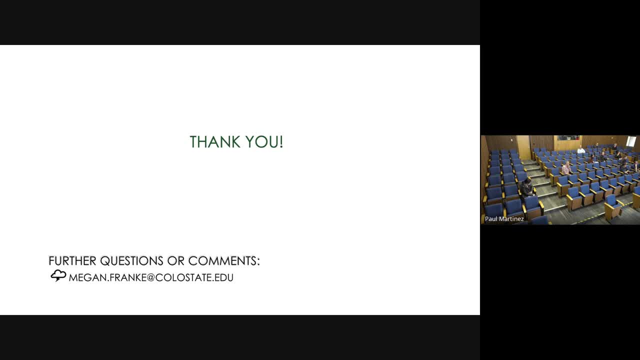 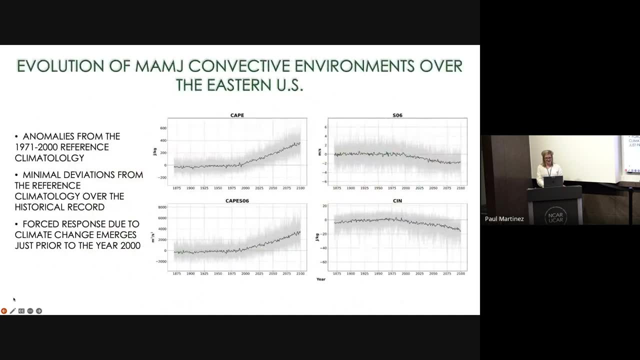 great library area. It's what are you? Yeah, And I guess I can pull out, go over that, But it doesn't appear that over time that distribution is really changing. at least the range from internal variability. It appears to stay pretty constant as we go through the. 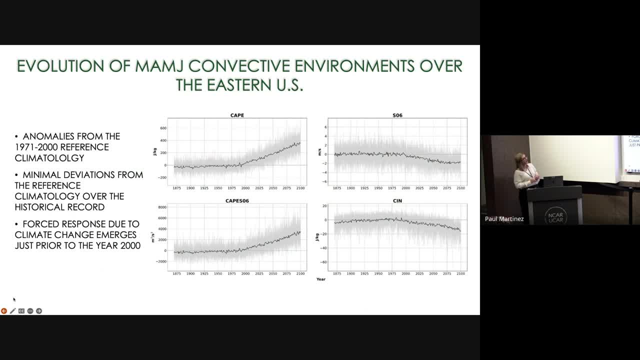 last century and this future one here. Yeah, for CAPE, I think it does a little bit and then, but like SO6 and SYN, we don't quite as much. Yeah, I didn't really look into that a lot for this, but I definitely think that can be. 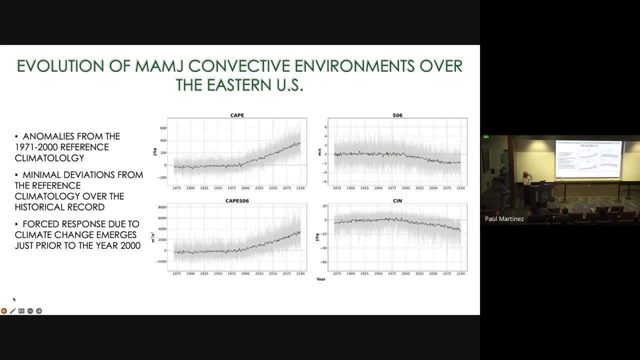 expected with this And I think like a lot this framework that we've approached this with, of course, using this model, is much too low a resolution to be really to say anything specific about specific storms and those losses that can occur with them, But overall I think that this kind of shows that those losses are expected to. 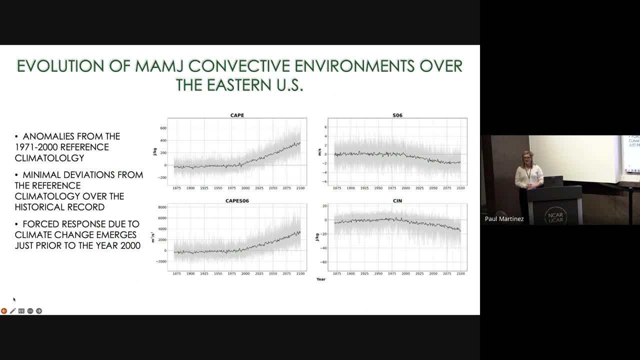 continue to increase Any other questions? Okay, now we'll have our break and we'll recalibrate at 10.45.. Can we do it again? Yeah, we'll recalibrate at 10.45.. Can we do it again? Yeah, we'll recalibrate at 10.45.. 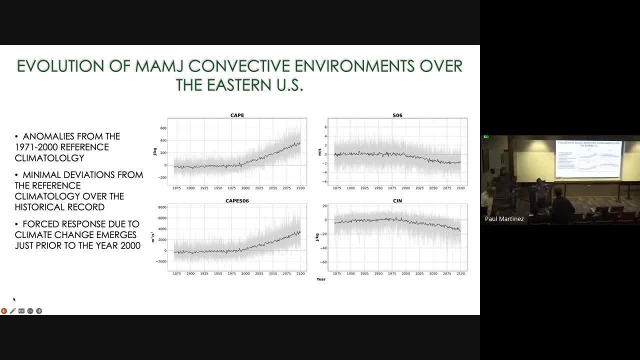 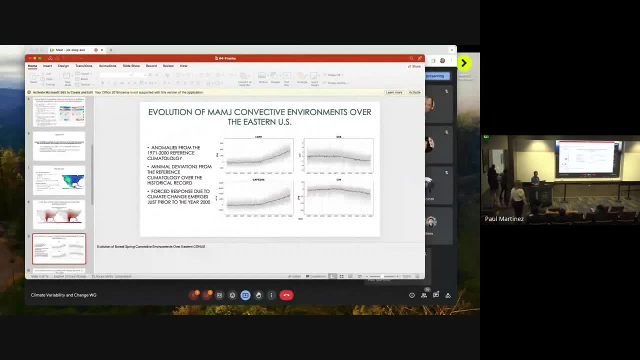 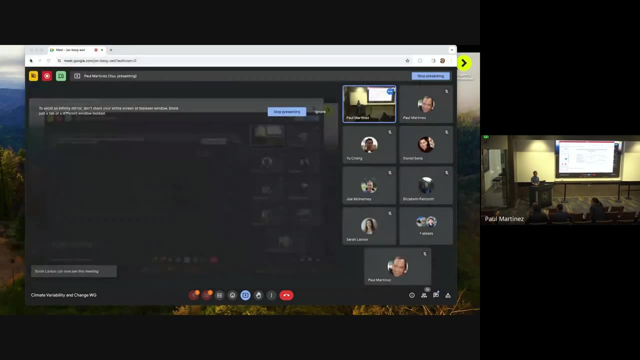 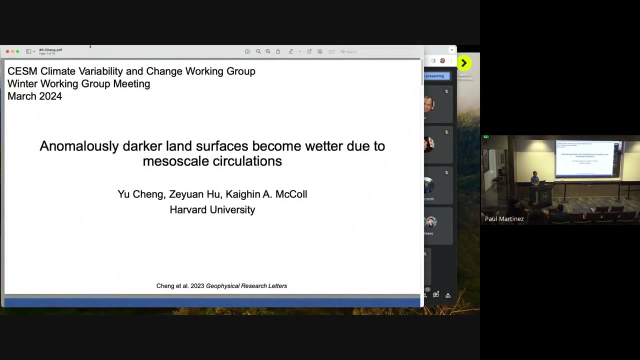 We don't have coffee and cakes, we just have to get some out of bizi. We don't have coffee and cakes, we just have to get some out of thus. Yeah, How was your birthday? Did I make you a pumpkin? 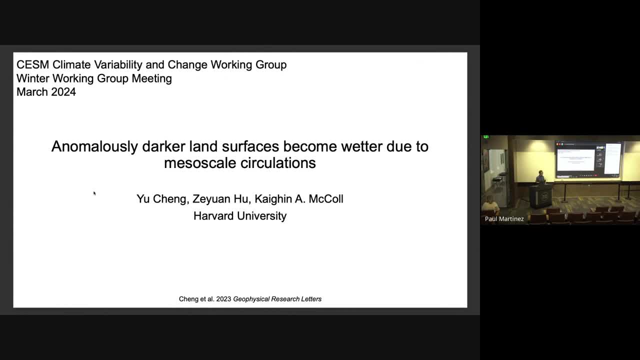 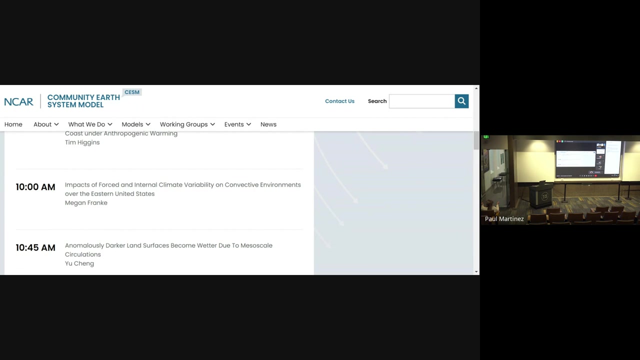 Not sure. I think so. You are you online. You always think you have it. You are you online, Not sure? You are you online. You are you online, Not sure? You are you online, Not sure, Not sure. 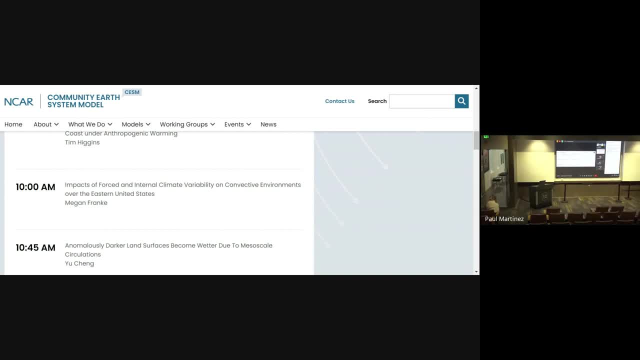 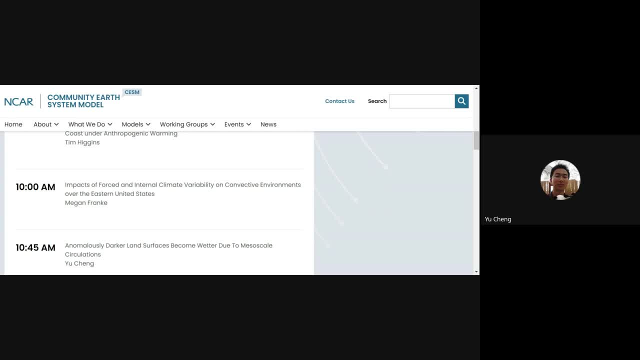 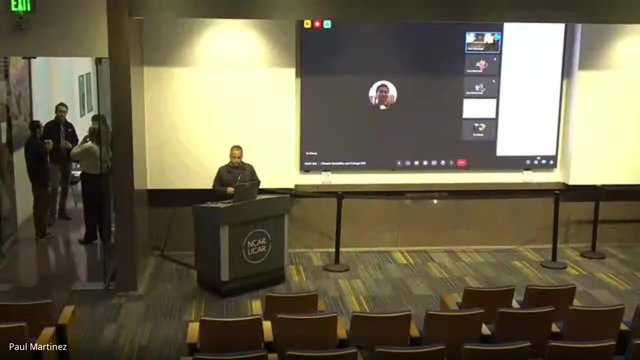 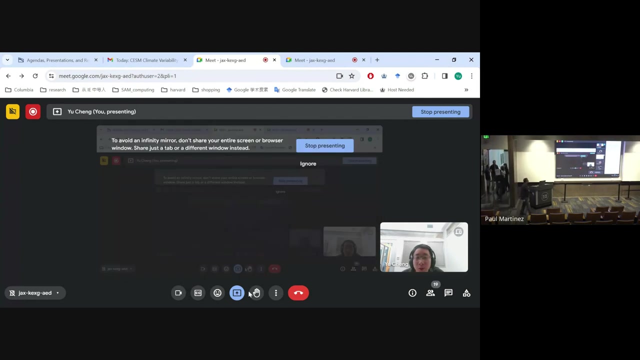 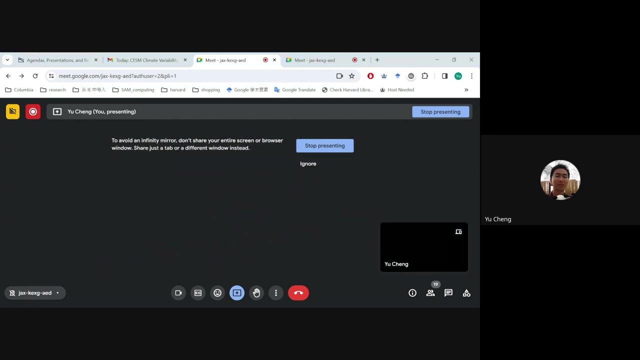 actually sharing it, but I'm not sure if you can see that. oh okay, let me see you. I have your talk. if you're having a hard time sharing that, I can share it on my end and you can just advance to the next slide. um, can you see my presentation now? I can see you, but I can't see your. 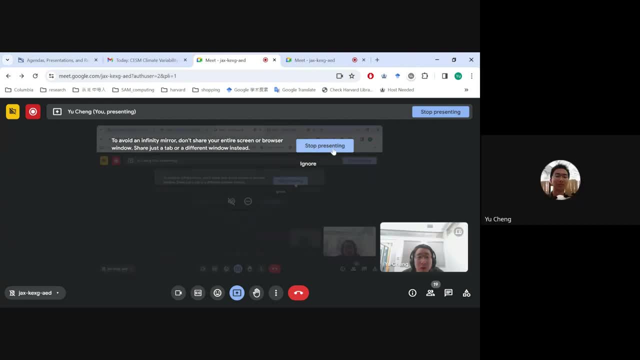 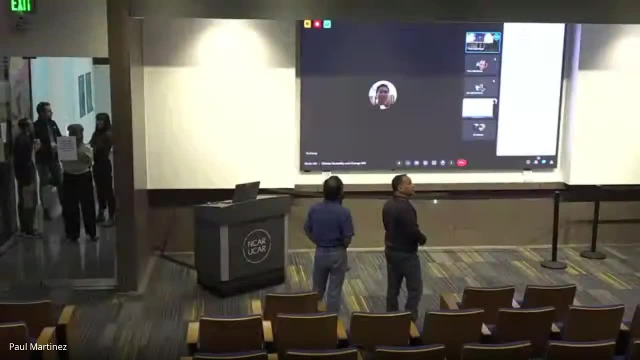 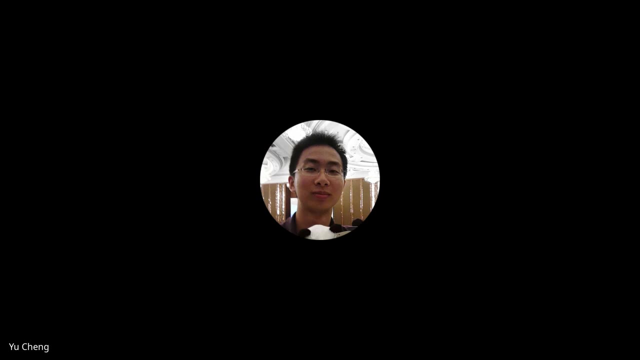 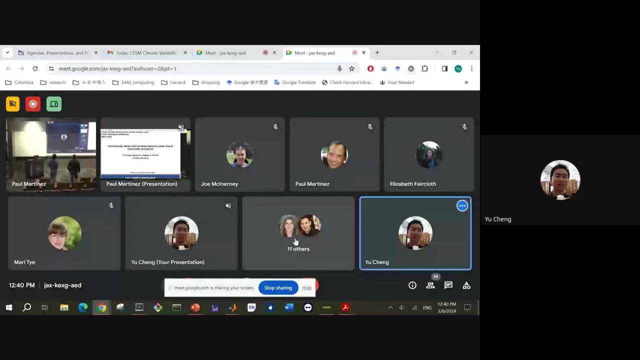 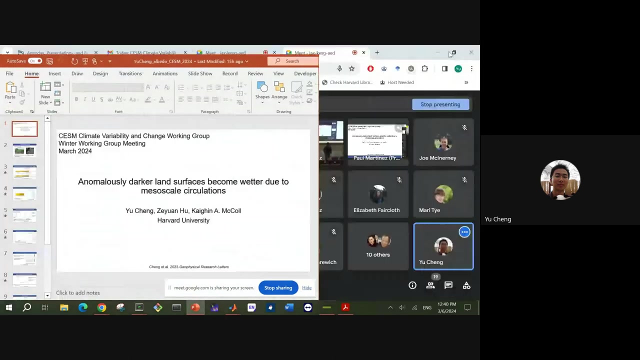 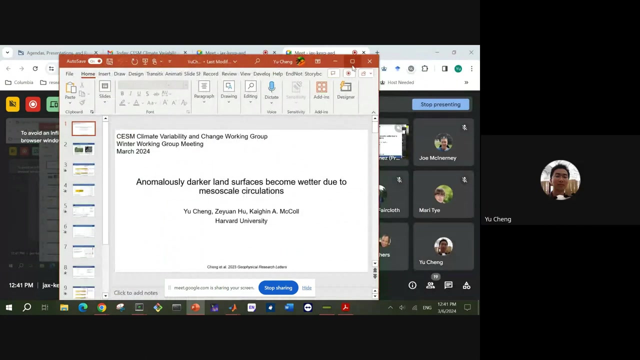 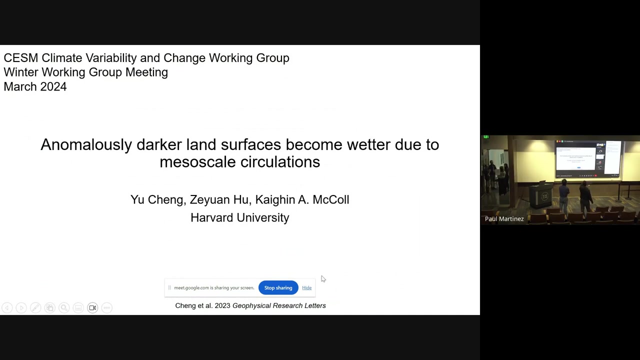 presentation yet. okay, uh, let me just try once again. so, um, you might want to share the entire screen and then bring up your presentation, okay, um, there we go, okay, okay, good, thank you, sorry about that, it's okay. can you go full screen for us? okay, perfect, and then, uh, on the bottom, if you could just click on hide. okay, there you go, we're ready. 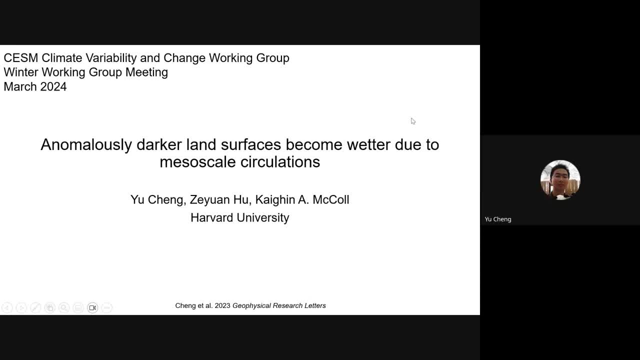 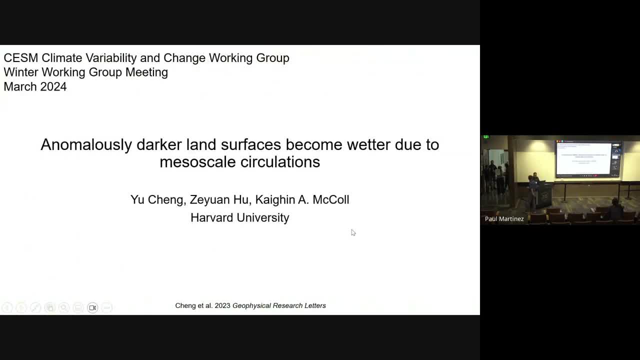 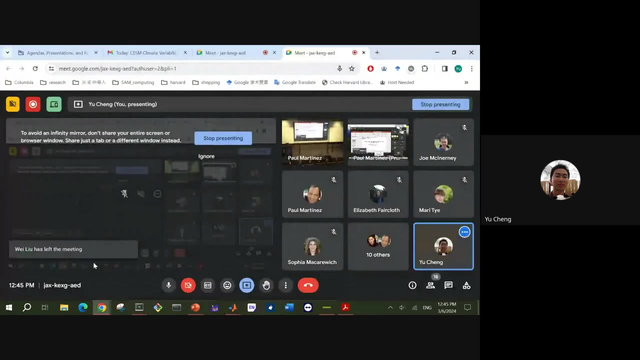 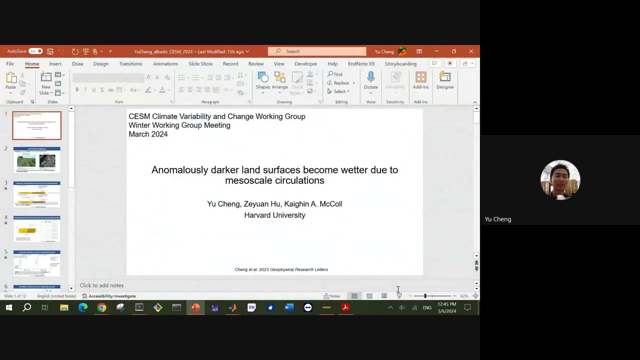 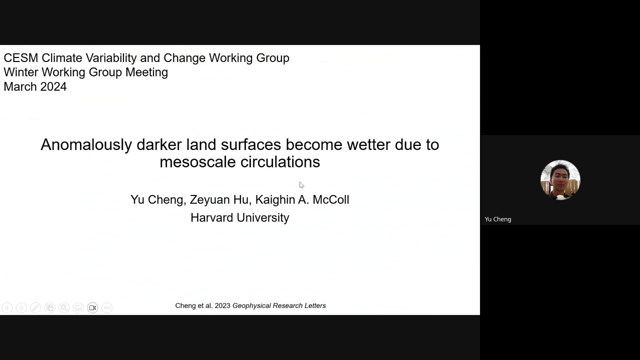 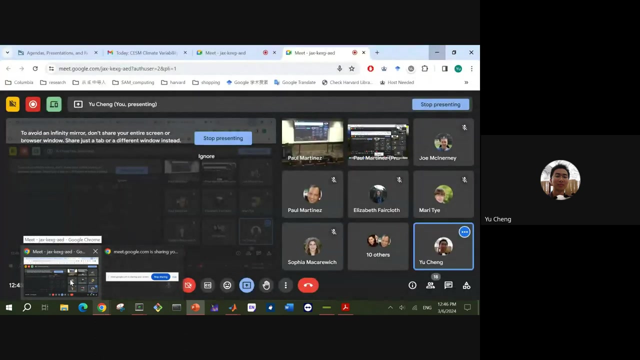 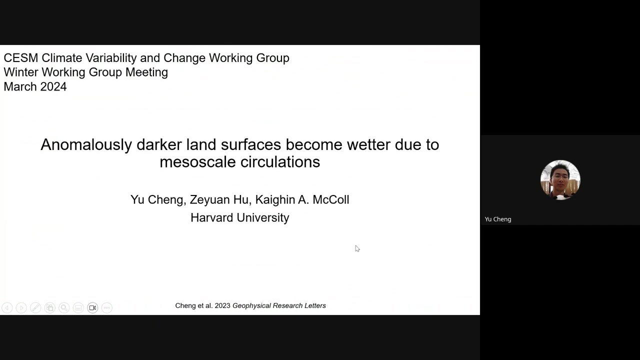 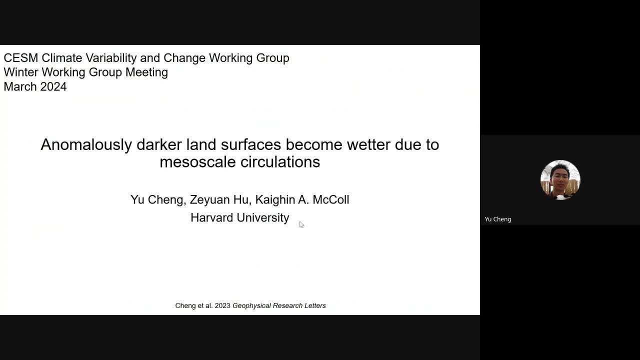 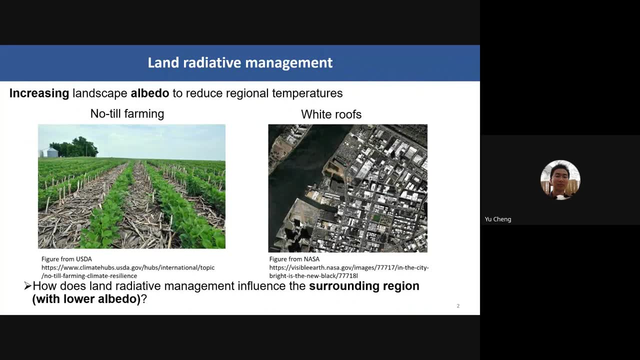 Metascale Circulation. First I would like to thank my co-authors Zhe Yuan and Kagan. Land Radiation Management has been used to reduce regional warming. Land Radiation Management typically increases the land surface temperature, Thus typically increases the land surface. 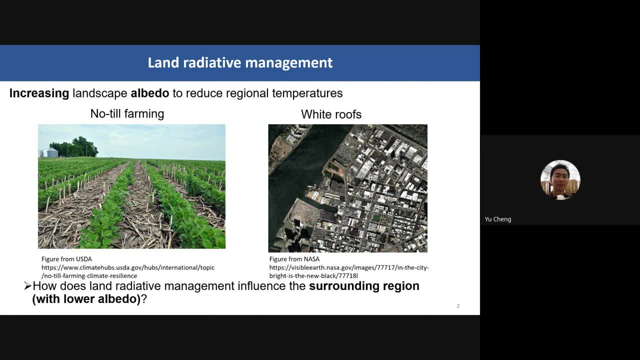 orbital, thus decreasing the absorption of net radiation reaching the surface and thus decreasing the land surface temperature. So no-tier farming and white roofs are two examples of land radiative management. No-tier farming is practiced on approximately about 12% of the global cropNAERA, and 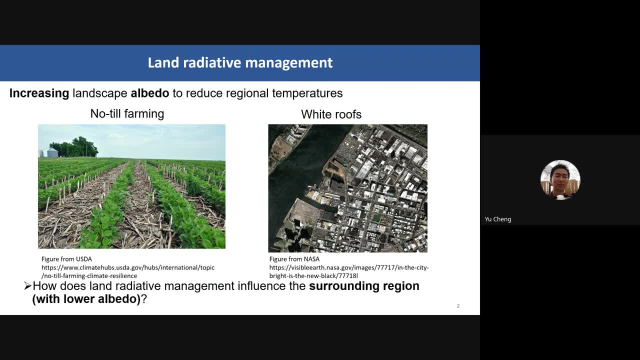 white roofs have been adopted in cities like Chicago and New York. White roofs have been shown to reduce land surface temperature from satellite images. The role of land radiative management on the local regions with high orbital is widely recognized. However, the impact of land radiative management. 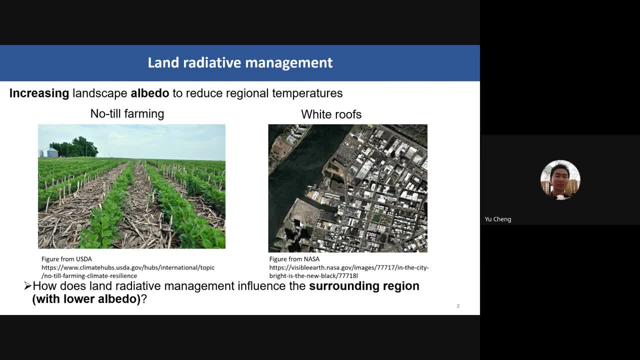 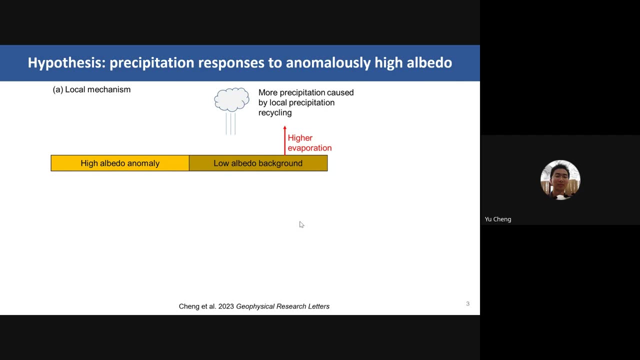 on cable roads or on wet roads with a relatively low orbital remains unknown, and here we would like to understand how land radiative management influences the surrounding region with relatively lower albedo. So we proposed a hypothesis on the precipitation responses to a high albedo anomaly. 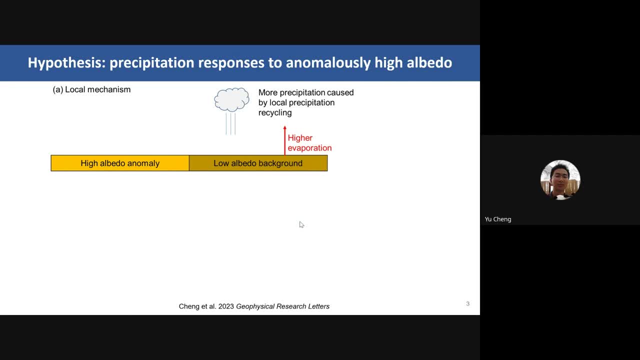 So over an idealized land surface with heterogeneous albedo, net radiation is higher over the low albedo patch, And the higher net radiation can lead to higher latent heat flux and higher evaporation. over the low albedo patch, The higher evaporation could further. 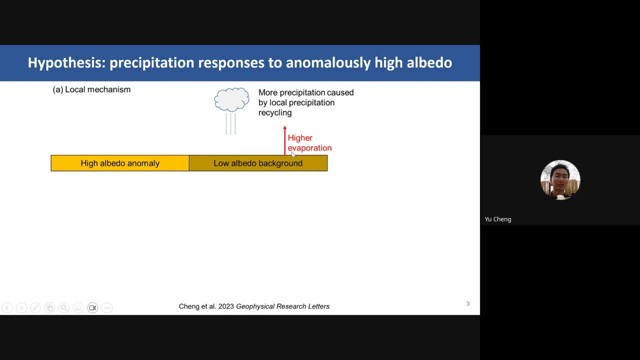 lead to more precipitation due to stronger precipitation recycling, And we call this mechanism the local mechanism. In addition, the higher left radiation over the low albedo patch can also lead to higher sensible heat fluxes. The higher sensible heat fluxes can further lead to metascale circulations. 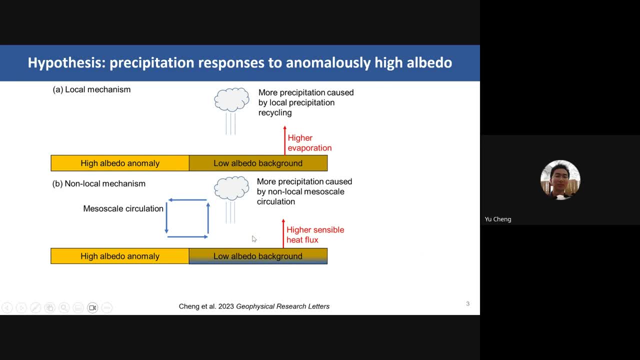 And metascale circulations can promote precipitation over the low albedo patch, And we call this mechanism the non-local mechanism. So, then, an important distinction between the local mechanism and the non-local mechanism is that there are no changes in soil moisture for the local mechanism, 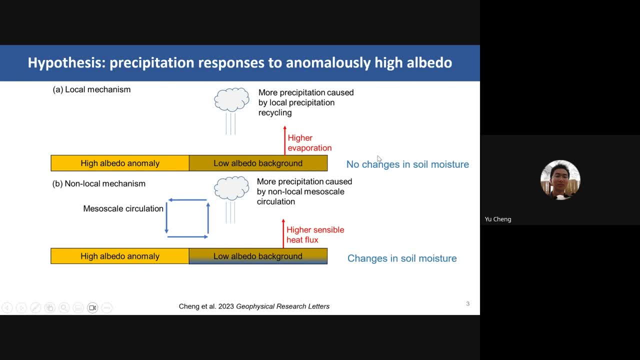 since there are no net horizontal moisture transport. Here we would like to understand the equilibrium precipitation response to a metascale albedo anomaly in isolation. So this question has largely been neglected in previous studies. First, the integration timescales. in previous studies 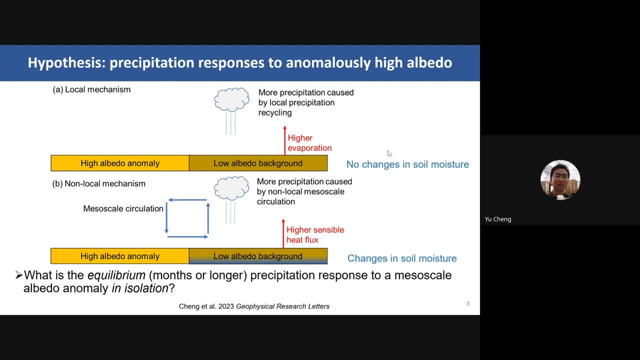 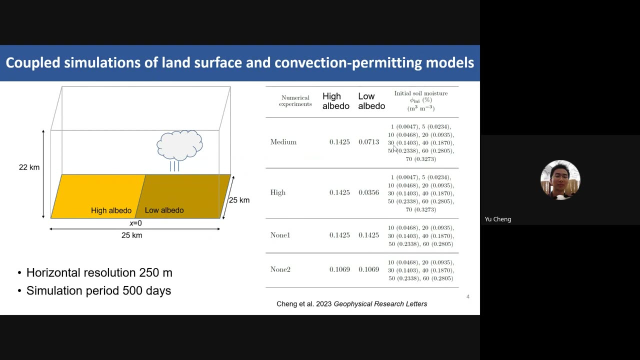 are typically on the order of the date, thus not reaching equilibrium state. Second, previous studies typically investigate multiple land surface heterogeneities like albedo and roughness simultaneously. Then we conducted an idealized conversion from permitting models over a heterogeneous land surface with different albedo. 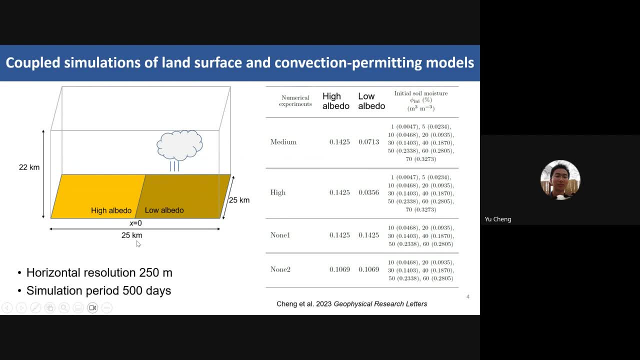 And the size of the computational domain is 25 kilometer times 25 kilometer and times 22 kilometer, And then the horizontal resolution is 250 meter and the simulation period is 500 days. We conducted numerous experiments prescribed with different albedo gradients and different initial soil. 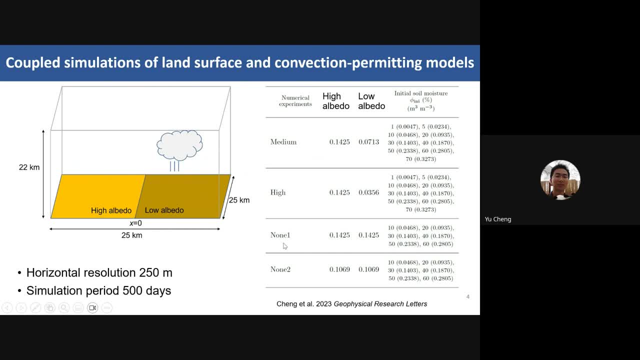 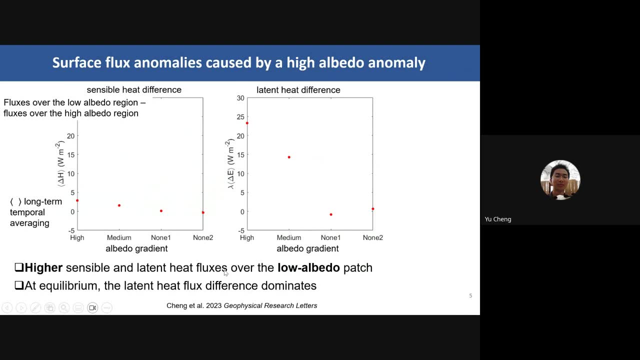 moisture conditions. In addition, we conducted control experiments where there are no prescribed albedo gradients. As expected, both sensible and latent heat flux is larger over the low albedo patch And we can also find that as the prescribed albedo gradient increases both the sensible heat difference. 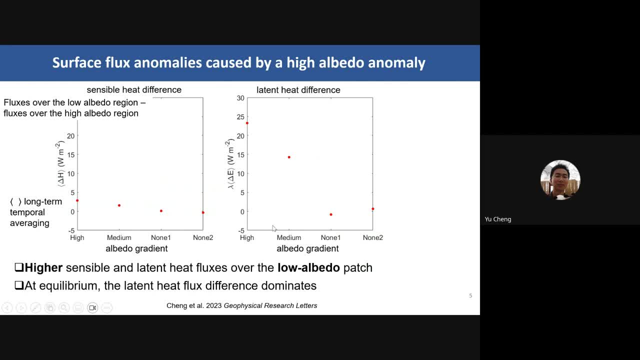 and latent heat flux difference between the two patches increase, And we also find that the latent heat difference is much larger than the sensible heat flux difference when they are averaged in the long term. Thus at equilibrium, the latent heat flux dominates. Then this is consistent with the local mechanism. 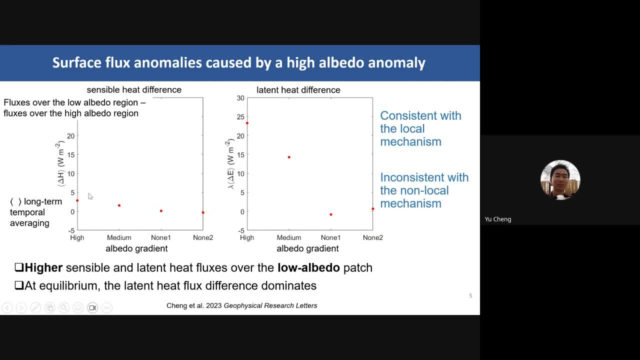 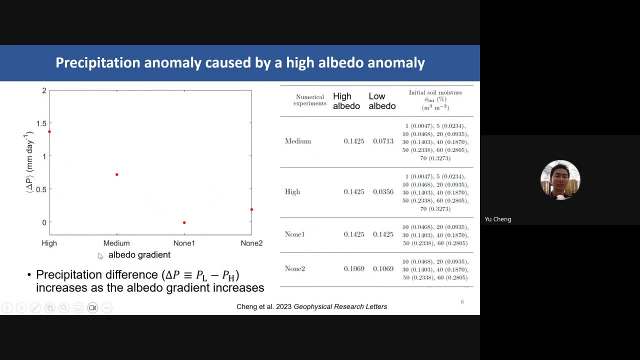 since the latent heat flux difference is much larger than the sensible heat flux difference, And the positive differences in both sensible and latent heat flux can further lead to positive precipitation difference. That is to say, precipitation is larger over the low albedo patch And as the prescribed albedo gradient increases. 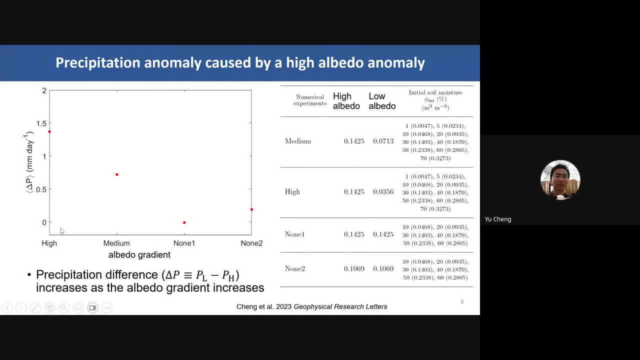 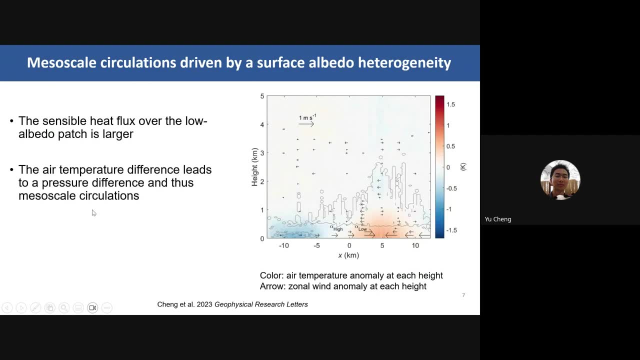 the precipitation difference between the two patches increases And as the prescribed albedo gradient increases, the precipitation difference between the two patches also increases. Although the long-term average sensible heat flux difference is much less than the long-term average latent heat flux difference, it can still lead to metascale circulations. 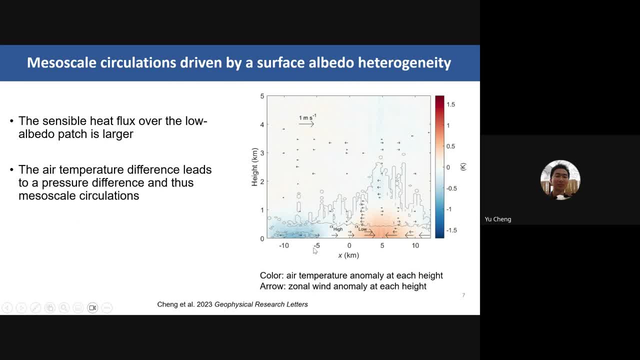 over relatively short time periods And on the morning of a typical day. in our numerical simulations we can find that the sensible heat flux is larger over the low albedo patch, And the higher sensible heat flux over the low albedo patch can further lead to higher near-surface. 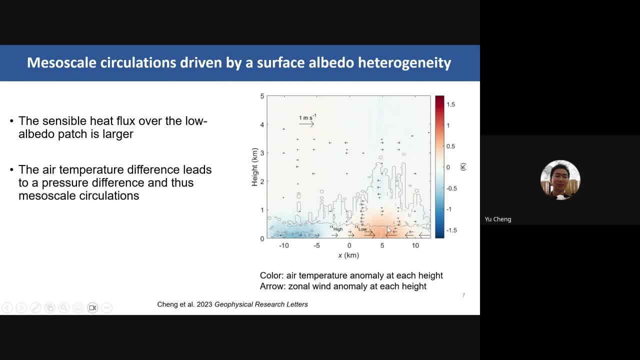 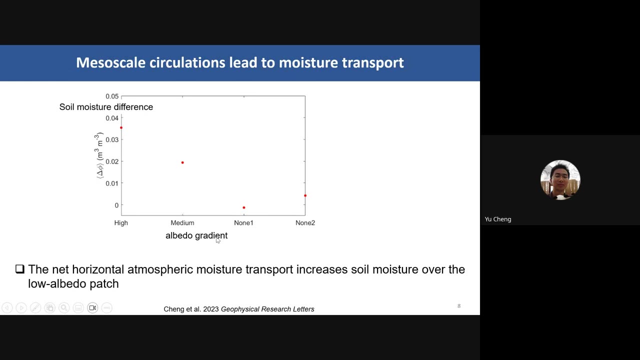 air temperature And the near-surface air temperature difference can further lead to a pressure difference and thus trigger metascale circulations. And here we can also find that as the prescribed albedo gradient increases, the soil moisture difference also increases, That is to say the soil moisture over the low albedo. 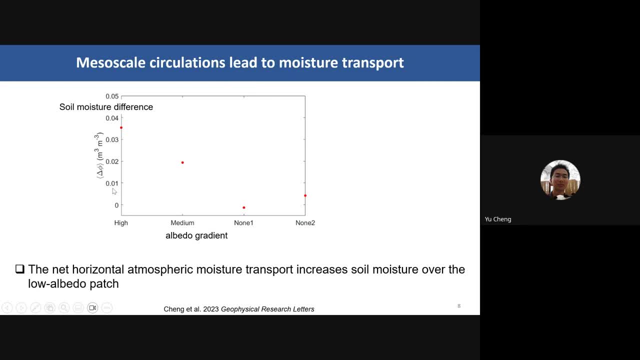 patch is larger compared to that over the high albedo patch, And we can find that this is due to the fact that the soil moisture difference is lower due to the fact that the metascale circulations can transport atmospheric moisture into the low albedo patch. 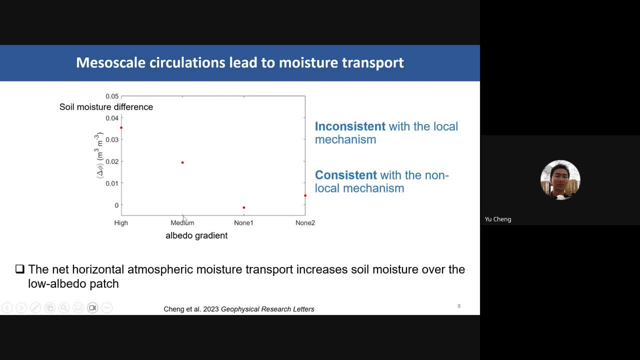 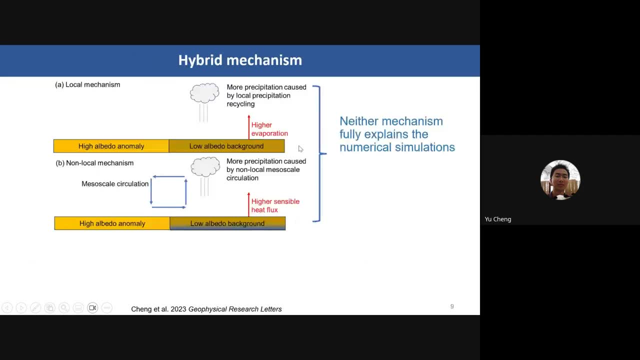 and then increase soil moisture there, Then this is inconsistent with the local mechanism, because we would not expect a soil moisture difference just due to the local mechanism. And then, to summarize here, we can find that neither the local mechanism nor the non-local mechanism can fully explain our numerical simulations. 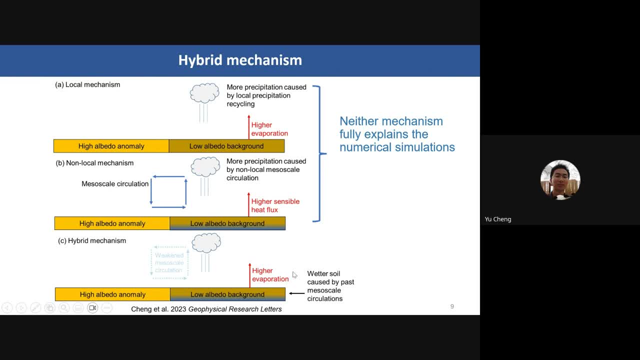 So then, instead we proceed to the next slide. Instead we propose a hybrid mechanism. And first, the higher net radiation over the low orbital patch can lead to higher latent heat flux and a higher operation. And the higher operation can further lead. 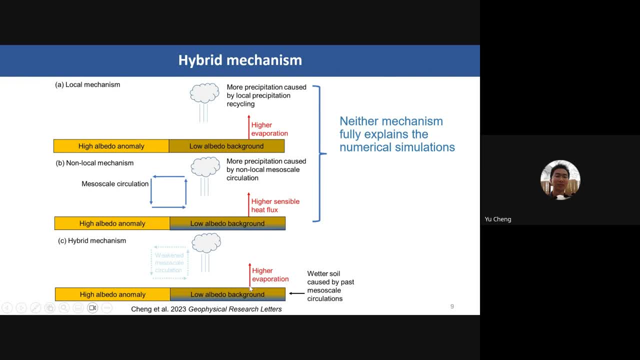 to higher precipitation. Second, the higher net radiation over the low orbital patch can further lead to a higher sensible heat flux, And the higher sensible heat flux can also further lead to mesoscale circulation And the mesoscale circulation can transport atmospheric moisture into the low orbital patch. 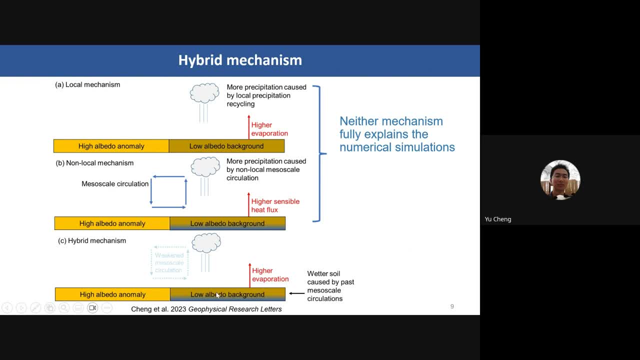 and increase soil moisture. there The soil moisture accumulates over the low orbital patch. At equilibrium, the soil moisture difference between the high orbital patch and low orbital patch becomes sufficiently large to significantly weaken the differential heating and mesoscale circulation driven by the prescribed orbital gradients. 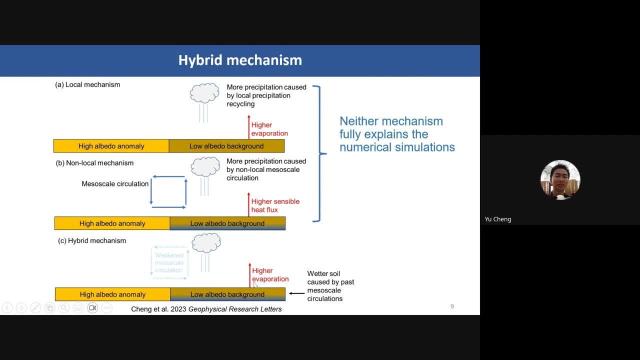 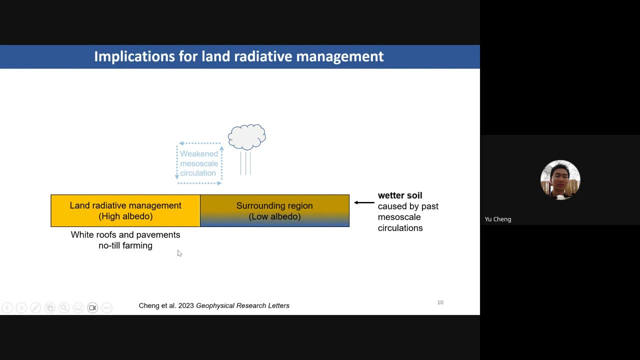 Therefore, at equilibrium, the latent heat flux difference and the evaporation difference dominate. However, there are water soils caused by past mesoscale circulations. Our results have some implications for land radiative management. So land radiative management increases the land surface. 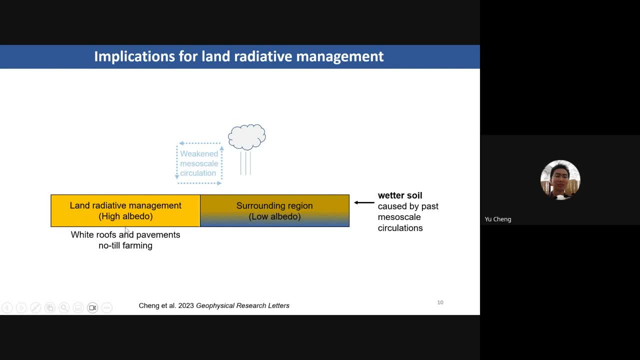 orbital over the local region, And here we showed that land radiative management can also increase soil moisture over the surrounding region, since there are water soils caused by past mesoscale circulations. Therefore, the land radiative management can potentially cool the surrounding region. 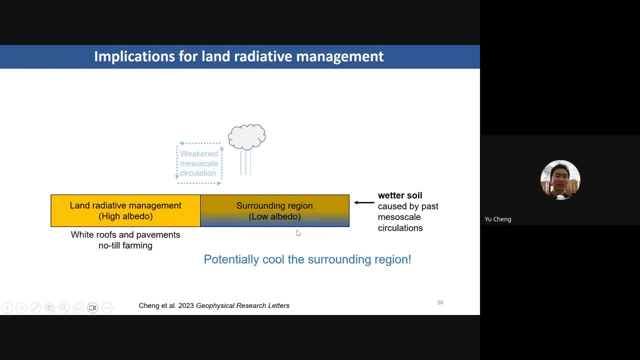 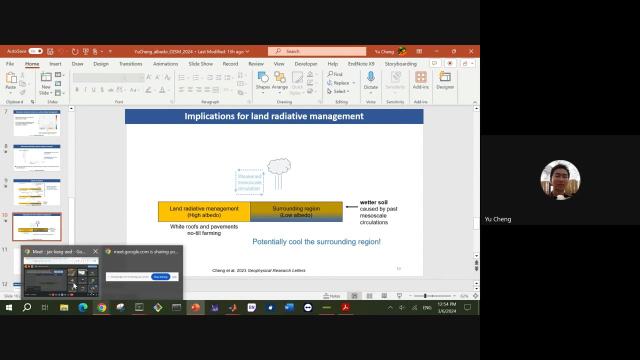 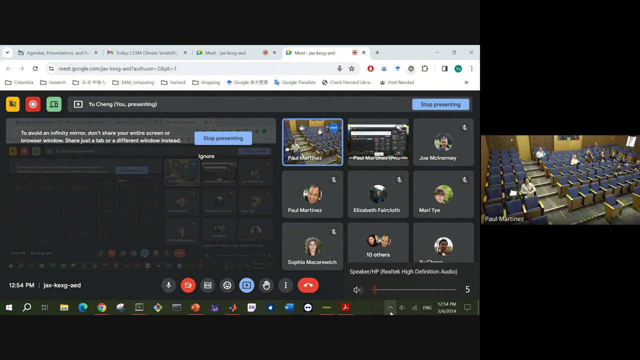 since more net radiation can be partitioned into latent heat flux rather than sensible heat flux. Thank you for your attention. Thank you very much. I'm curious about how much you tried with the horizontal horizontal resolution or the spacing between bright and dark. 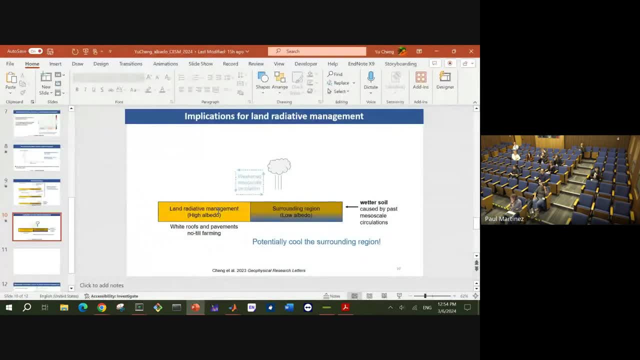 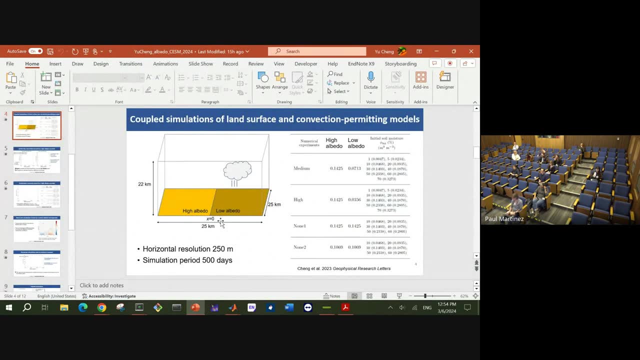 surface. So what was the? I guess the typical length scale here was 10 to 20 kilometers, But did you try other? Yes, we actually tried different. So, for example, the size of a domain: we tried the size of a domain to be like 50 kilometer times. 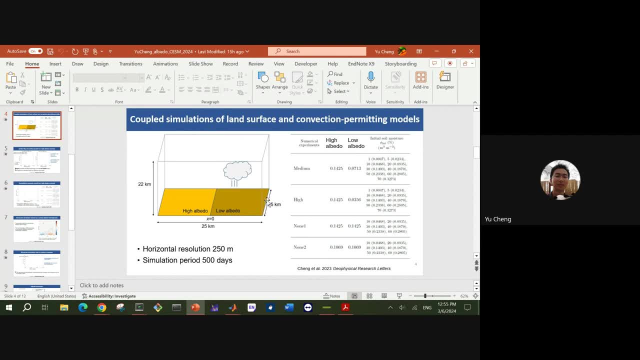 50 kilometer, And by then it doesn't seem to influence the major finding here, especially for the precipitation response due to the prescribed orbital gradient. And then an important note is that the prescribed orbital heterogeneity should be sufficiently large, So typically it should be like several times. 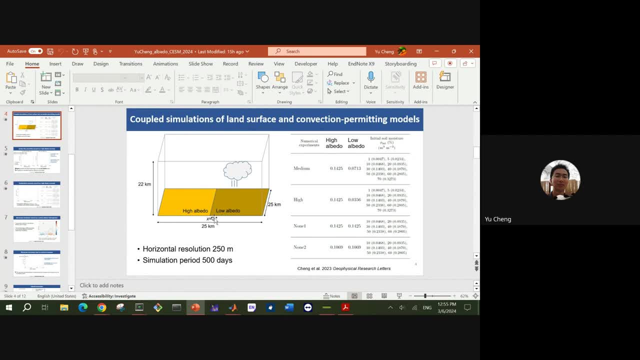 of the atmospheric boundary layer height for such kind of mesoscale circulation to be triggered? Sorry, Thank you. So this is all happening on scales smaller than our CSM grid boxes. Do you have any thoughts about what the net effect of not having these subgrid scale? 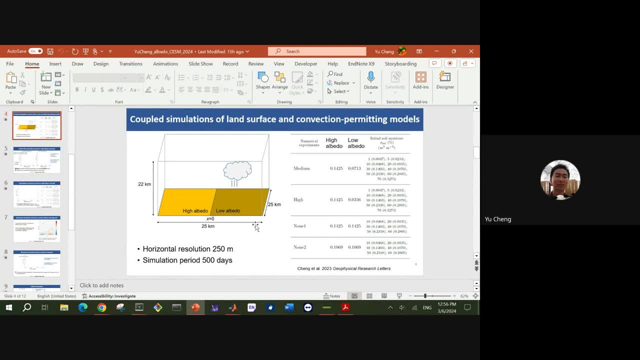 mesoscale circulations and heterogeneity would be. Yeah, thanks, That's a great question, And so I think those kind of processes- I think are very- are not resolved by cost resolution. CSM, It seems that there are already some land gradient management. 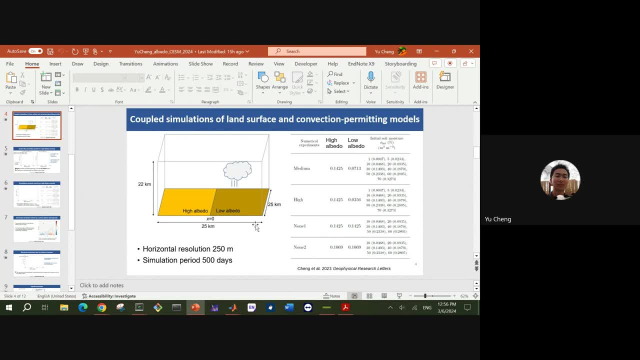 like wet roof. So it seems that those kind of increasing soil moisture and precipitation over the surrounding region of the land gradient management seem to might have been neglected in counter-numeric simulations. So it might have some current CSM might have underestimated the precipitation and soil moisture. 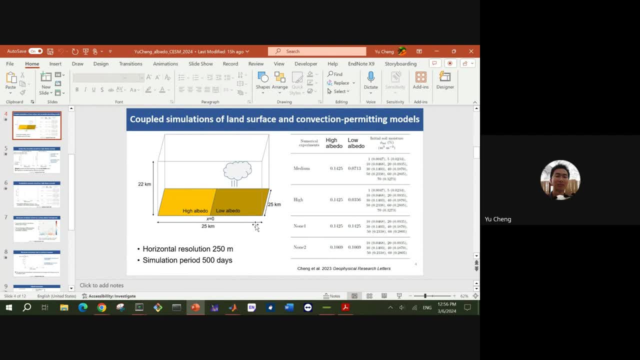 over the surrounding region of such kind of land gradient management? Yeah, I know they're trying to parameterize this. Are experiments like yours informing that You mean for the of such kind of subgrid scale primarily? Yeah, exactly, Yeah, that's a great question. 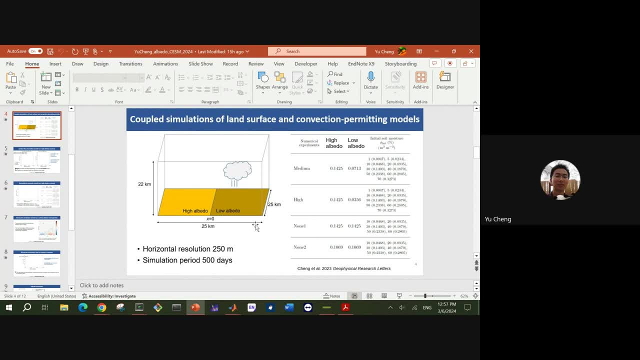 So we have not done such kind of subgrid scale permutations considering the net effect of heterogeneity. but we know that some other groups have done such kind of studies. As of now we haven't really identified if they really could observe what we are finding here. 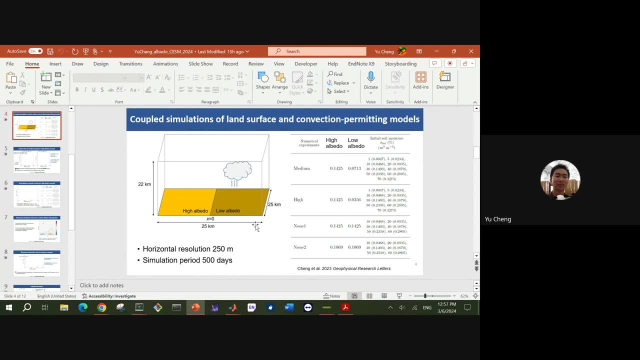 because there still have been some ongoing processes in the permutations of subgrid scale land surface processes. So because so typically when they permutate such kind of subgrid scale land surface heterogeneity, they compute the surface flux using different types of land cover and then they would use some kind 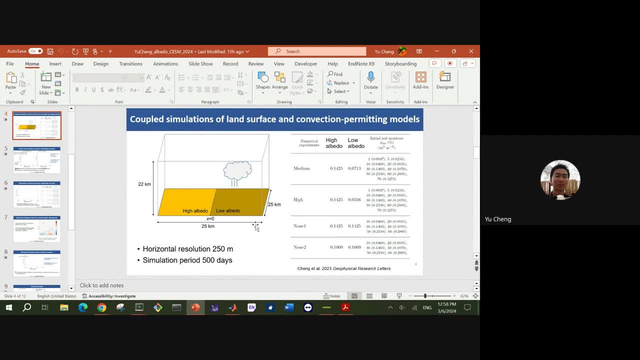 of average method to compute the real fluxes, But I'm not sure if that really could be correctly captured here. But it's a great question to look into later on. I have a question Right now. from your commanding it seems like we only have two patches in this model domain. 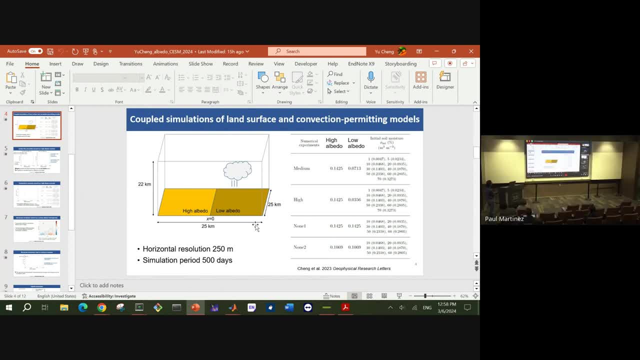 Or do you have multiple patches? Is the result going to change or not? Yeah, that's also a great question, And here this is a highly idealized numeric setup, And then it's periodic in the horizontal direction. So then, if you are allowing those kinds of heterogeneities, 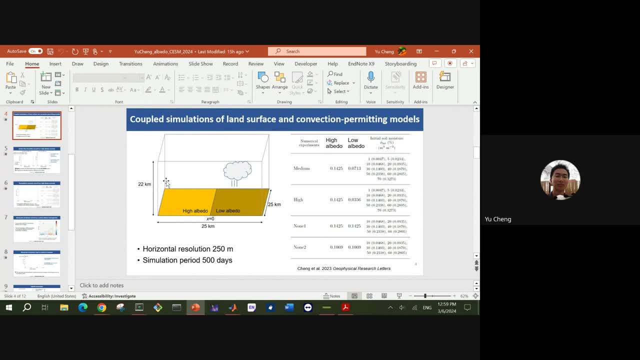 to occur infinitely in the horizontal direction. so it seems that this kind of soil motion and precipitation might still occur. But if you prescribe some other kind of land surface condition, so then we are not sure. So it would really depend on the exact condition. 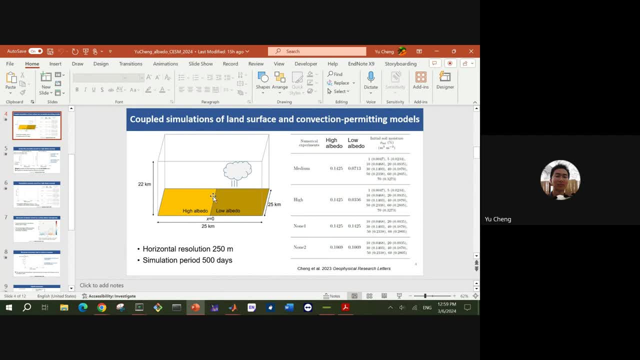 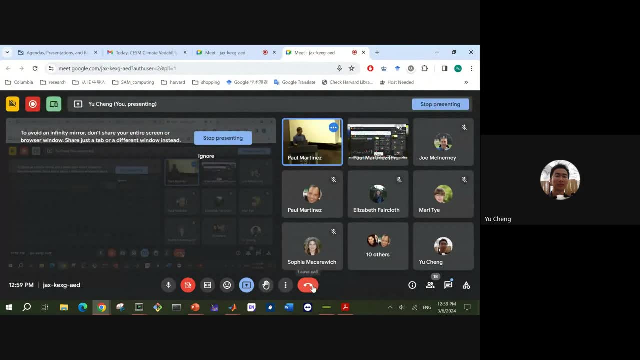 of the land surface condition. Thank you, Thank you, OK, let's move on to the next one. OK, Next up will also be outline as presented by Danila and Nicole. She's here. Oh, she's here, Yeah. 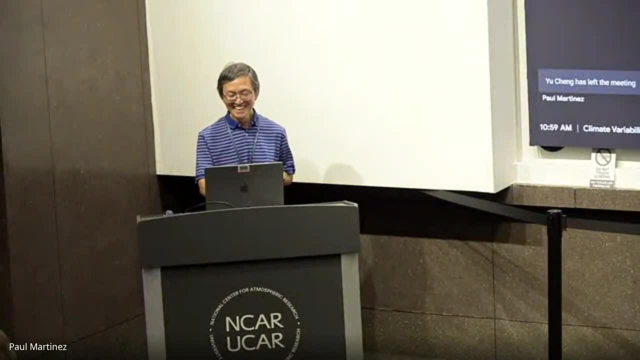 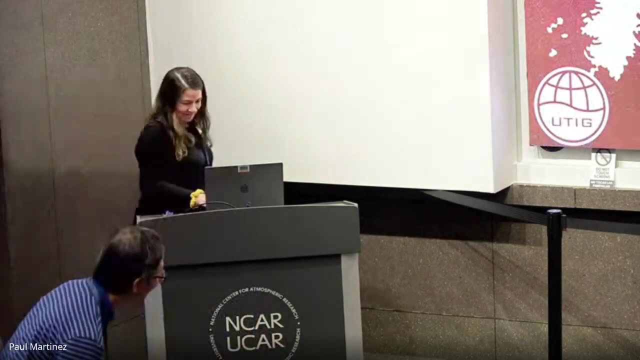 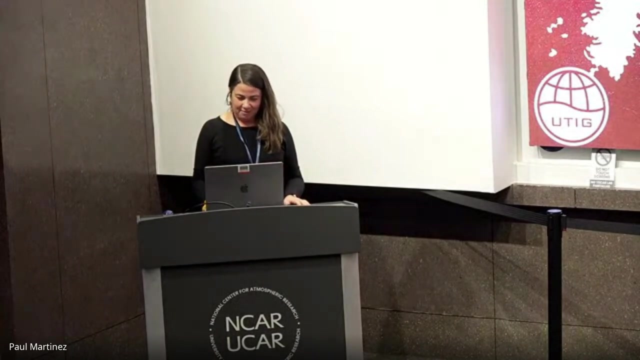 Oh OK, Hi up here. Hi up here. OK, All right, thanks for having me. Good to be here in person Today. I'll be talking about work I've been doing in the past year and a half or so. 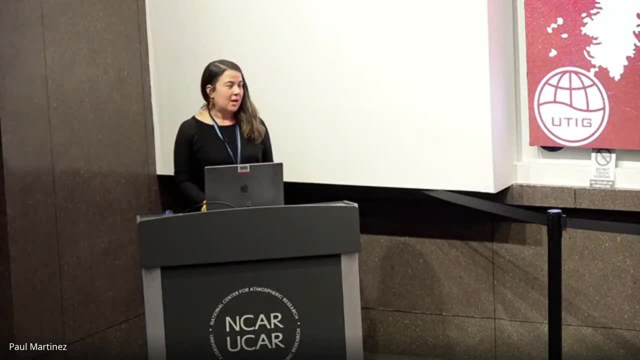 I started as a postdoc here with Clara Odesser and now continuing on at UT Austin, So I've been really interested in extreme fire weather events in the past. I've been looking at them for the past four or five years now And there's still some remaining questions. 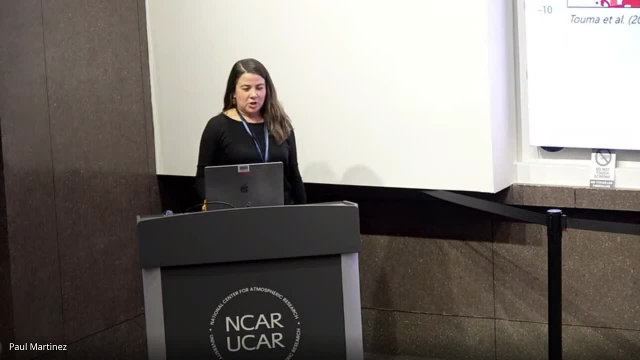 that I'm trying to answer. So we know that extreme fire, weather events, so conditions that are warm, dry and windy- that can lead to- I'm not sure they're seeing online. OK, I don't know if we'll be starting them up. 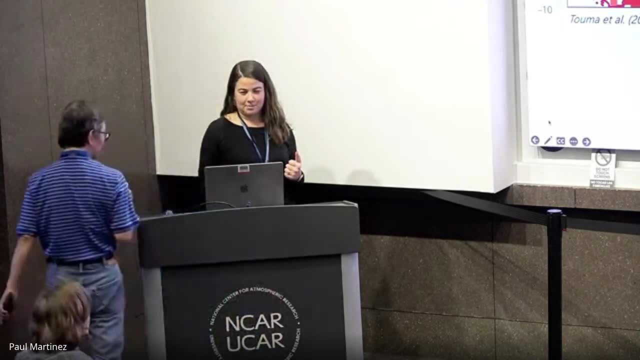 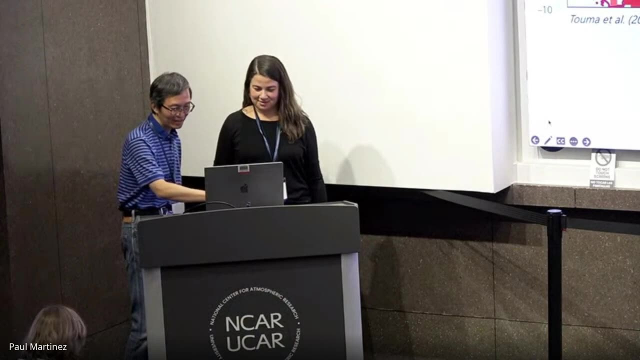 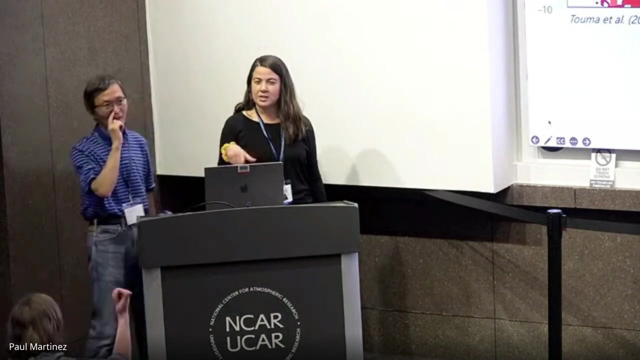 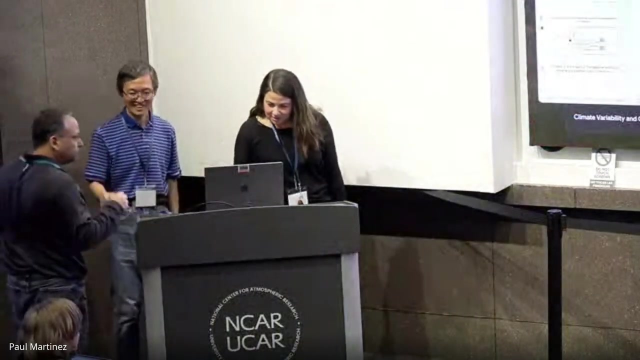 Cool, We're not starting them up. Pause: No one online. Could you stop sharing? OK, Yeah, But we're going to start sharing the virtual- Yeah, OK. Do you want to do it? Yeah, OK. So that's the first one. 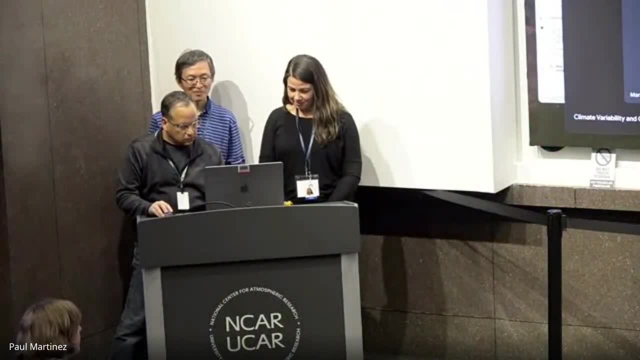 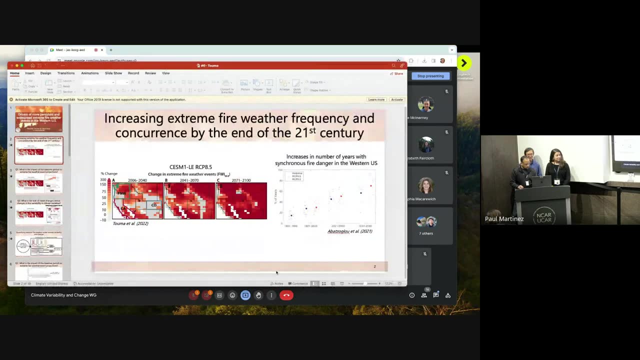 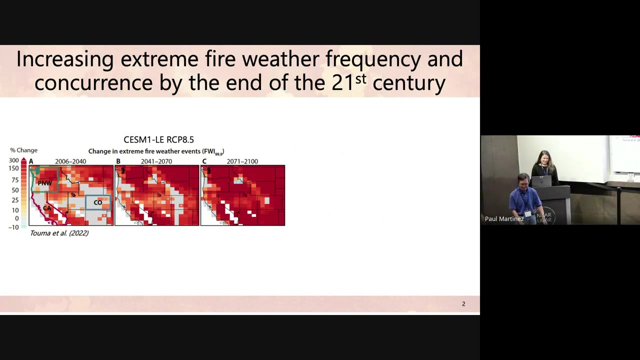 Thank you. So this is a little more of a technical question. So you didn't miss any cool graphics yet, so I'll just hook you in. So we know that extreme fire weather events- so warm, dry, windy conditions- are expected. 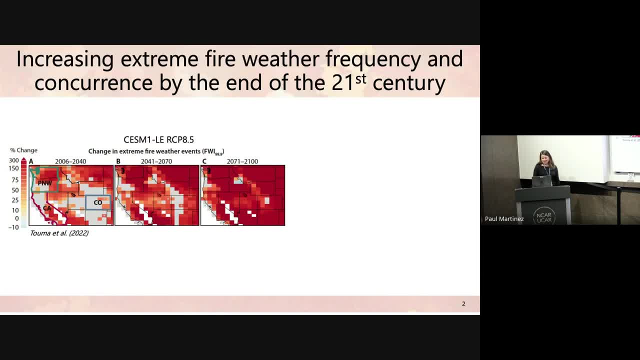 to increase by the end of the 21st century. So this is a little bit more of a more specific question of the 21st century in our future climate simulations. So this is an example of these projections, using the CESM-1 large ensemble under the RZP 8.5 scenario, and you can see that. increases in extreme fire weather events are expected almost everywhere in the western US, almost everywhere in the western US going into the future up to 2100.. And we also other studies have also shown that the number of years with synchronous fire danger in the western US- so multiple regions having fire danger at the same time- 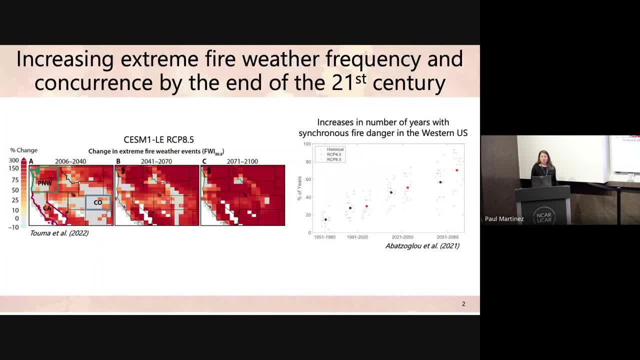 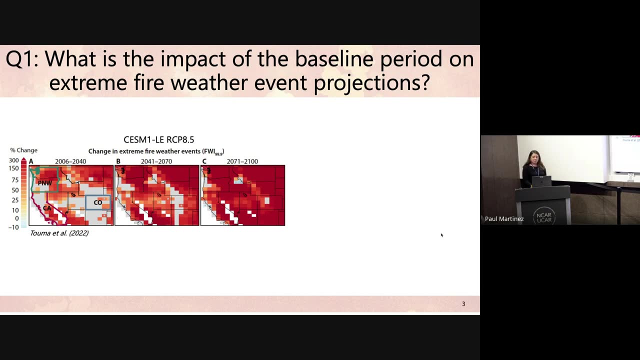 is also expected to increase in the future. So not just the frequency but kind of the concurrence or a spatial extent of these events are expected to change or increase. And so one question I had is how does the baseline period that we choose in terms of defining extremes impact? extreme fire, weather, event projections? 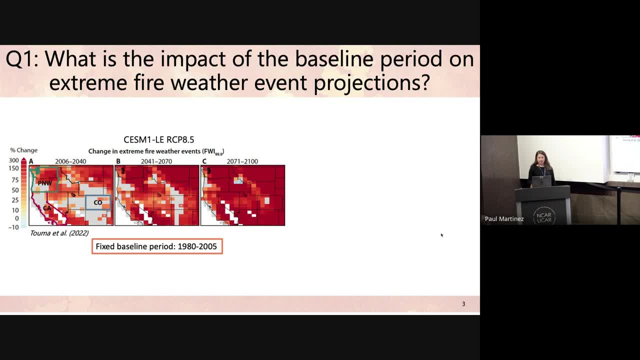 So in this study, for example, we use 1980 to 2005 as the baseline period and that's why, probably, we see so many increases going to the future. But recent. there's been a recent discussion among people who study extreme fire, extreme climate events in general. 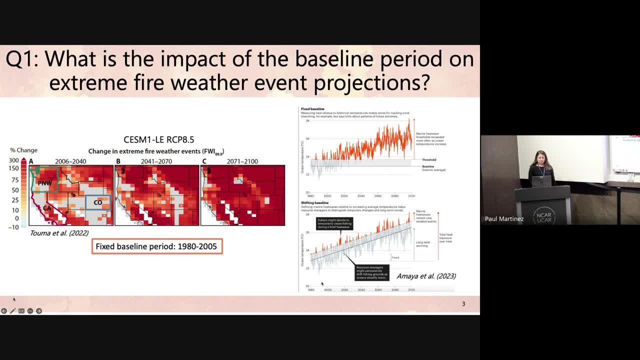 to understand what the kind of impact of different baseline periods are. So you can either use a fixed baseline- so kind of looking at two sides of the spectrum- you can either use a fixed baseline, shown in this example here, where you kind of understand changes in your 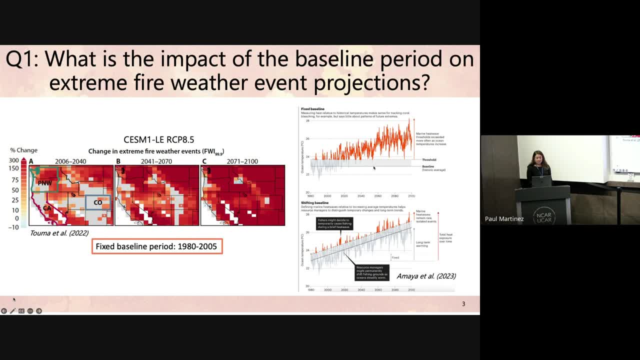 in your extreme events compared to this period, this historic period, or you can use a continuously shifting baseline which kind of allows you to understand extreme climate events if we were to adapt to them. So you can either use a fixed baseline or you can either use a fixed baseline. 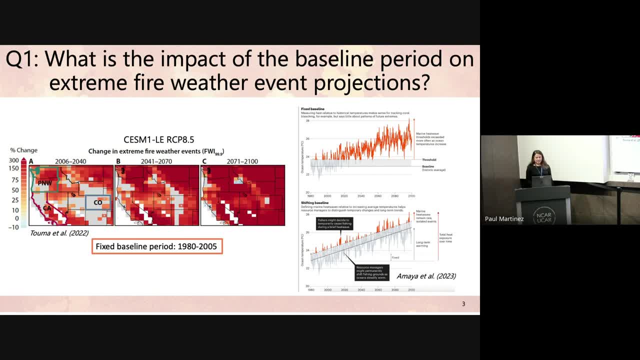 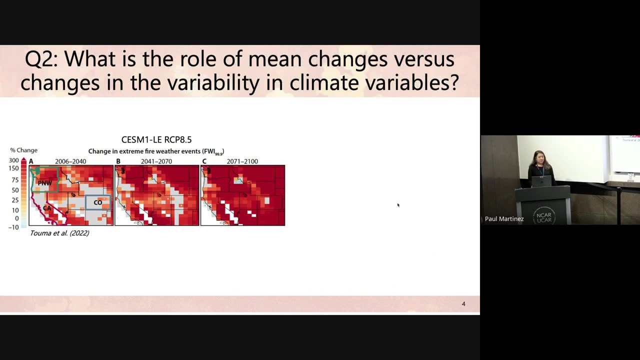 As we go along into the future, and this kind of also helps us understand why extreme events might be changing due to changes in the mean versus changes in the variability away from that mean. The second question I wanted to answer is: what is the role of mean changes in the variables that? 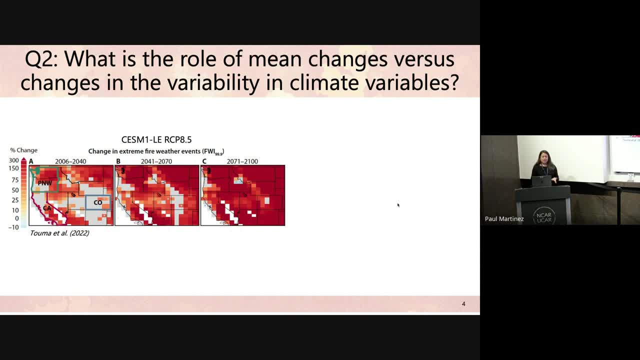 contribute to extreme fire weather events versus their changes in their variability across time. So previous studies, including mine, have kind of isolated the impacts of different variables on extreme fire weather event increases, And so we found that for the western US that temperature increases in temperature and decreases in routes of humidity. 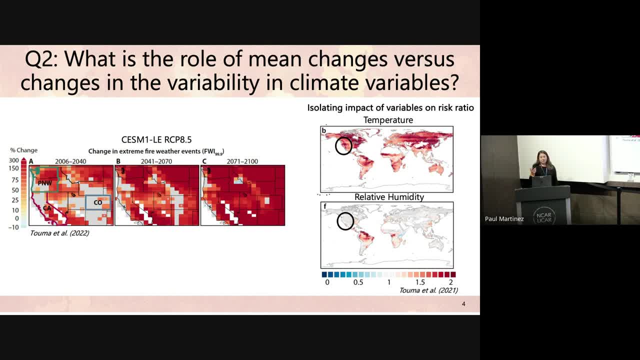 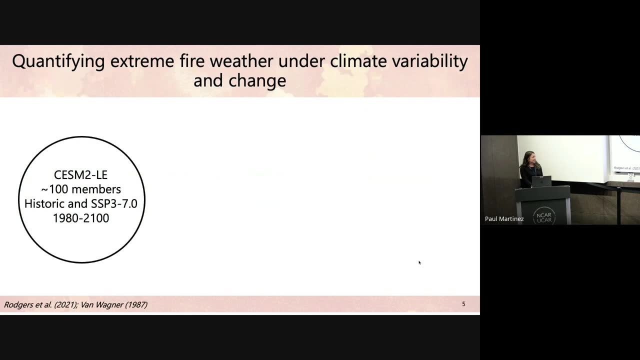 are driving much of these changes in increases in extreme fire weather events. But I wanted to understand whether it was the mean changes in those variables or the changes in the variability in those variables, or both. So we have a really nice data set that we can use to understand these. 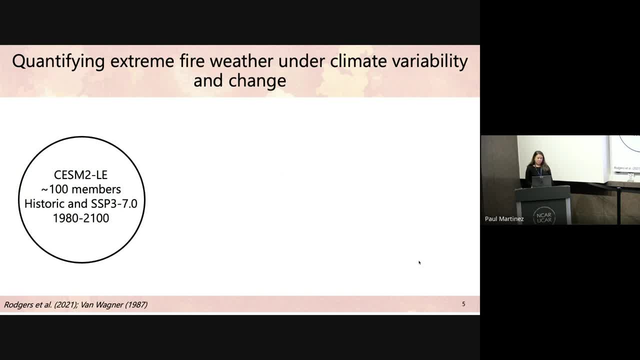 questions. I'm using the CESM-2 large ensemble. This is a 100 member ensemble and I use a run in the historic and SSP-37 scenarios and I'm using the data from 1980 to 2100.. And for each one of 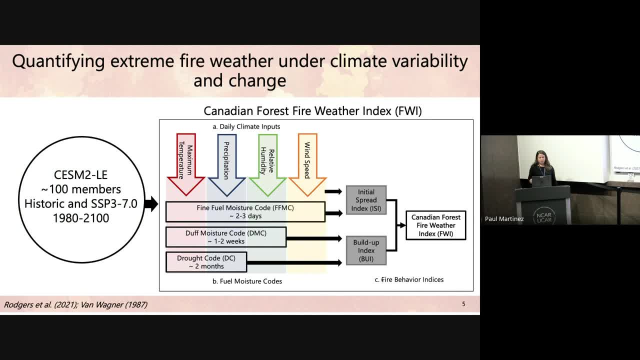 these members and each grid point across the western US. I calculate the Canadian forest fire weather index, which takes into account- I don't know where my mouse is- takes into account maximum temperature, precipitation, relative humidity and wind speed on daily scales, And using this index, we can. 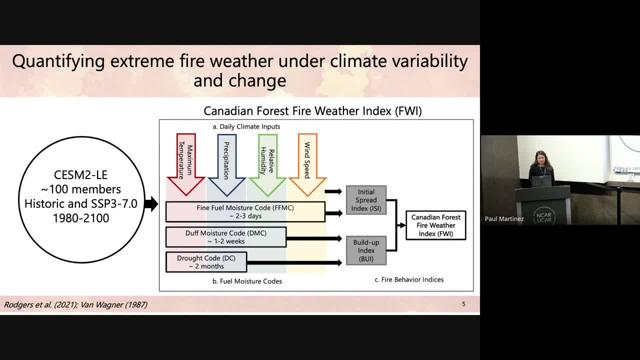 kind of quantify what the weather conditions are in a given day and how that relates to fire weather, So weather that is conducive to wildfires to occur or to spread, And so I now have a fire weather index time series for each member and each grid point in the western US. 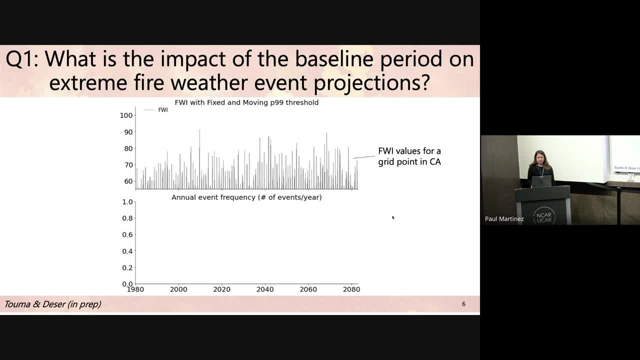 So, going diving into the first question, what is the impact of the baseline period on extreme fire weather event projections? So here I'm showing an example time series of the fire weather index for one simulation for one grid point over California. I don't remember where in California, but I can. 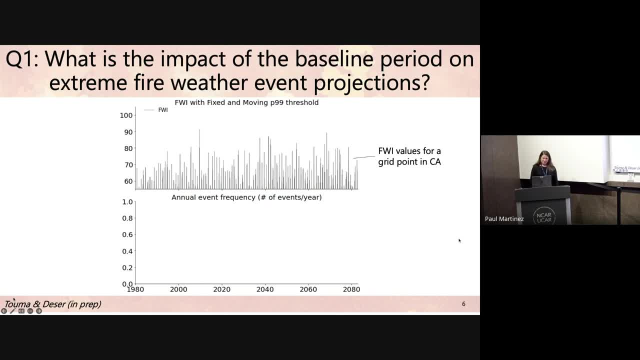 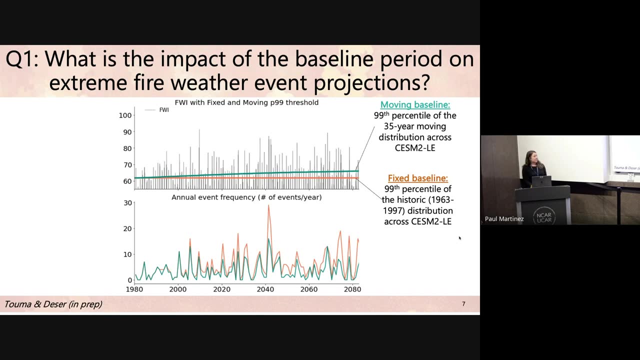 look it up if you guys are really curious. But- and here I've zoomed in to kind of like the top part of the y-axis to be able to look at just kind of extreme values of the fire weather index, And so I've defined two different baselines. One is the fixed baseline. 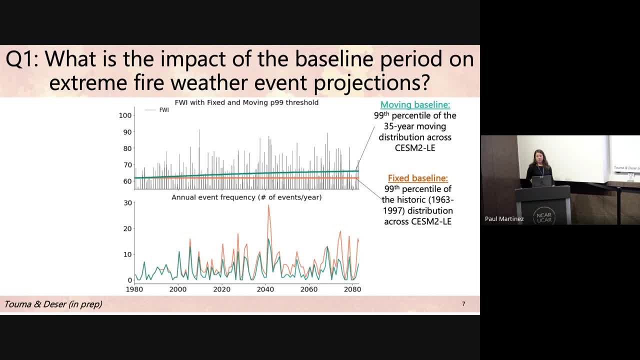 which is this orange line, which is the 99th percentile of the historic distribution over 35 years centered on 1980.. And this gives us this orange line which is basically the same going across through time, And I've also defined the moving baseline. 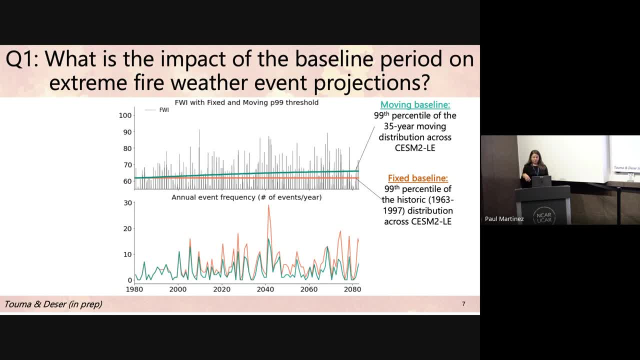 which takes the 99th percentile of the 35-year moving distribution across the full ensemble. So it moves every year through time and gives us a different 99th percentile that we use to define our extreme events. So this time series at the bottom kind of shows you the outcome of using 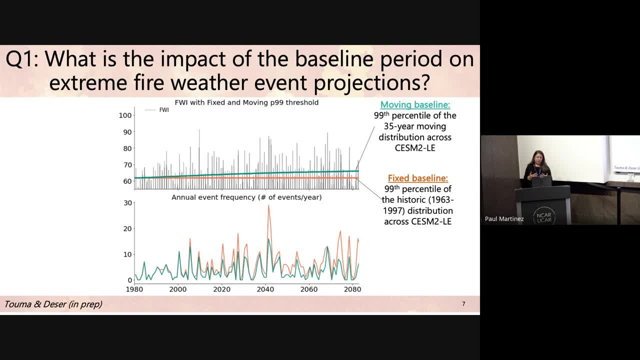 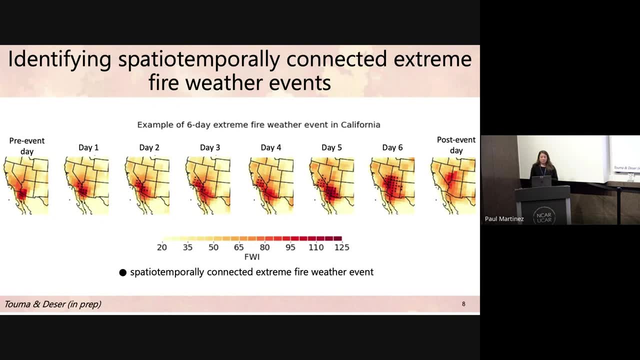 these two different baselines And you can see that using a fixed baseline generally gives you more events, especially going into the future. And we also wanted to identify spatio-temporally connected extreme fire weather events to also try to understand how change, how extreme fire weather events are also expected. 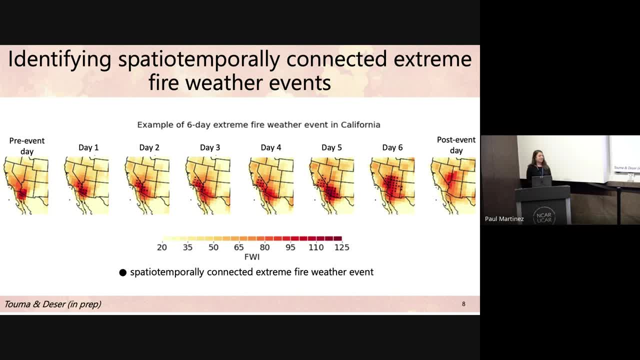 how the area and duration of these events are also expected to change. So this is an example of how I've defined events in these simulations. So here I'm showing an event that's centered over California, So I'm only looking at this event when it's over California. 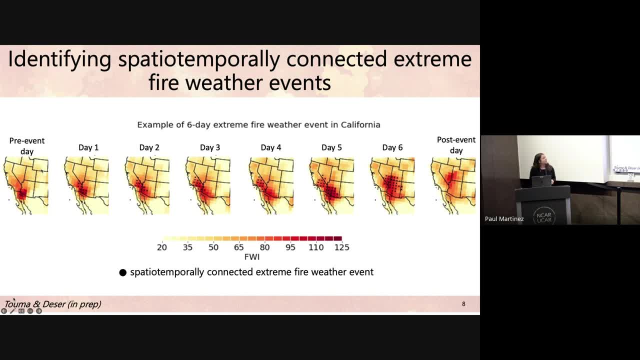 And you can see the shading is the fire weather index value on a given day. And the dots here- I don't know if you can see them, but the dots here show one event, so an event that's connected to recent time, And you can see how it starts off like a little baby event at the beginning and then 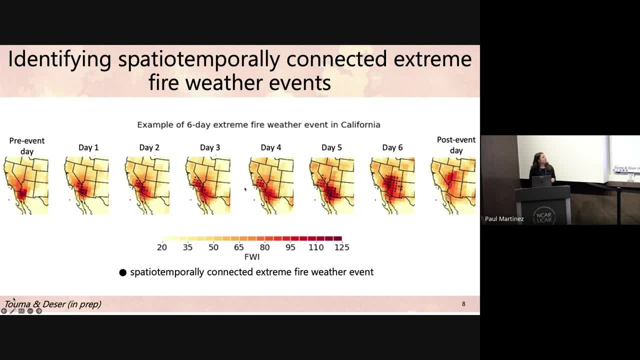 moves, going into the next days. It grows, expands, it moves around And by the end of the sixth day when i stopped counting it. so that's one example of one event. so i've identified all these events. i've identified over um, i would say like 10 000 events, i think um using the tsm, large csm, one, two. 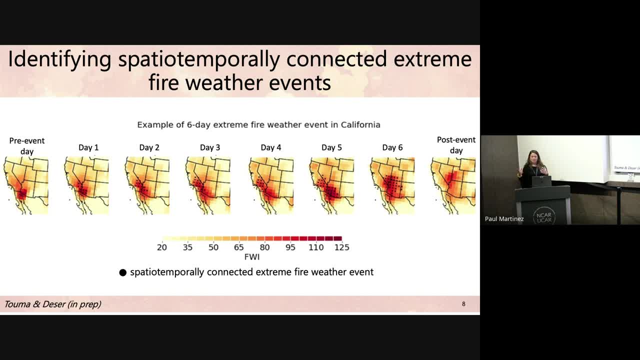 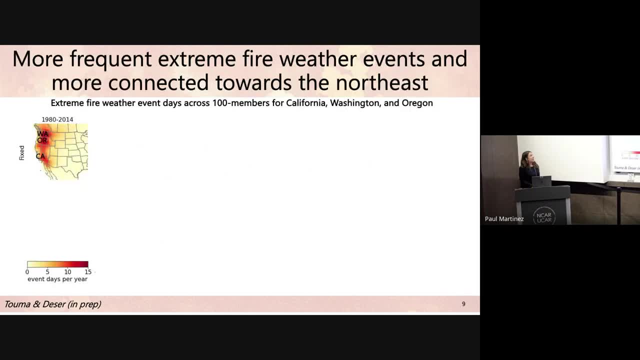 life ensemble and they all have an area, duration and multiple other characteristics you can dive into as well. so, um, sorry, so, uh, here i'm showing the frequency of the frequency of events, um, for the historic period 1980 to 2014, and these are events that are centered over washington, oregon. 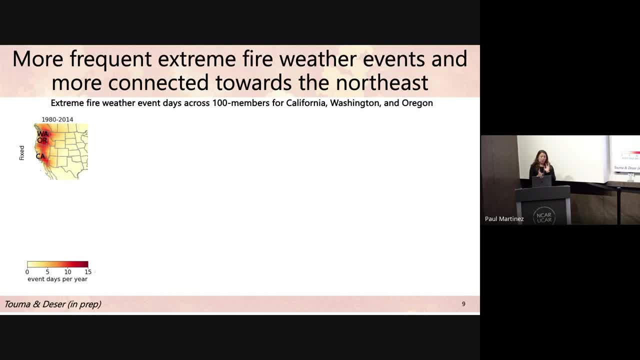 or california. so they have to have at least one grid point in one of these states at a given time and you can see that most of them are centered over those states, but they're also centered kind of inland, which is why they're centered over the state of california, which is why they're centered. 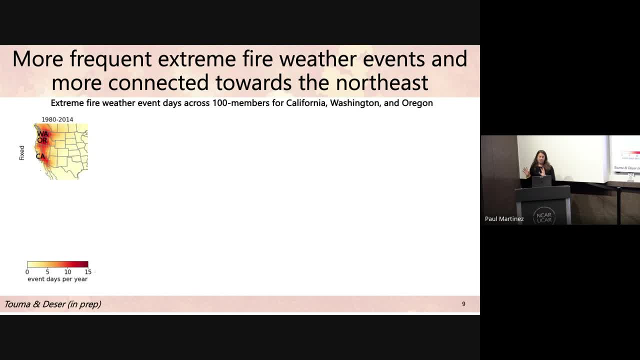 over the state of california, which was interesting to me, and they also tend to spread a little bit eastwards as well, going into the future. we see that one the frequency of these events increase, kind of what we've seen, seen in previous studies already. so just kind of confirming that. so we see. 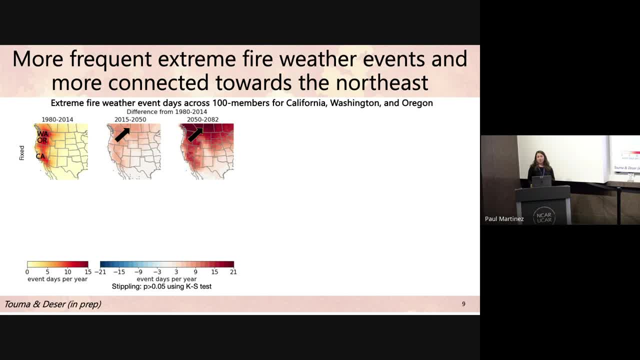 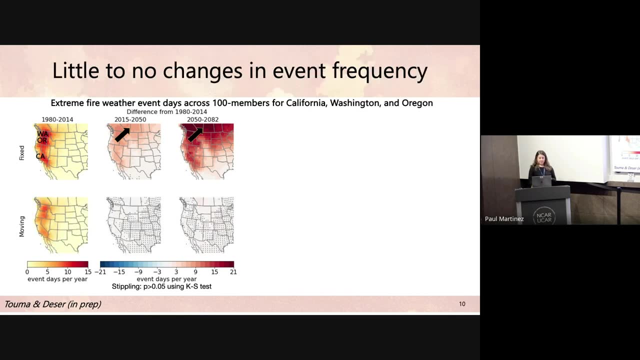 a greater number of events, but we also see that these events are starting to become more connected to locations in the northeast of this region, especially- um, not so much in the southeast, but mostly in the northeast, so i thought that was really interesting. when we use our moving 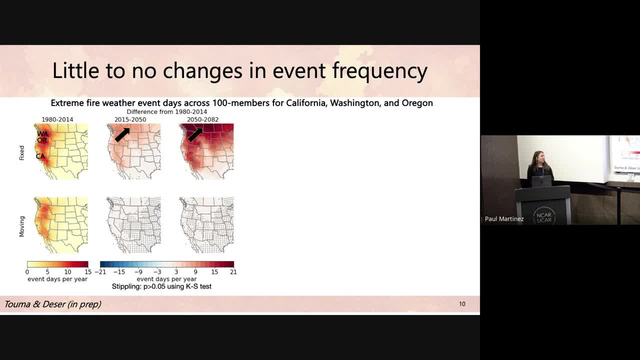 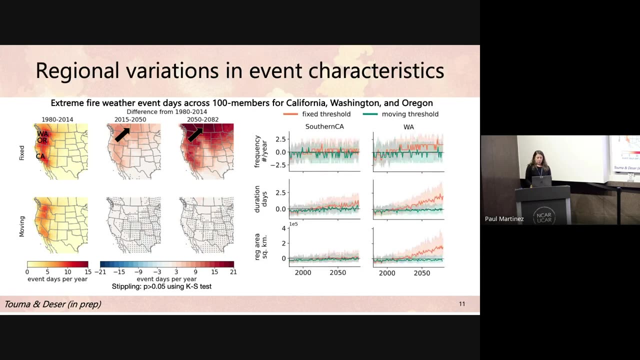 threshold. we don't see much changes in the frequency, but we do see hints of maybe some more widespread events, and more events may be connected to these northeast regions, like we did in the fixed baseline. we also see some regional differences in the characteristics of these events, so we see that. 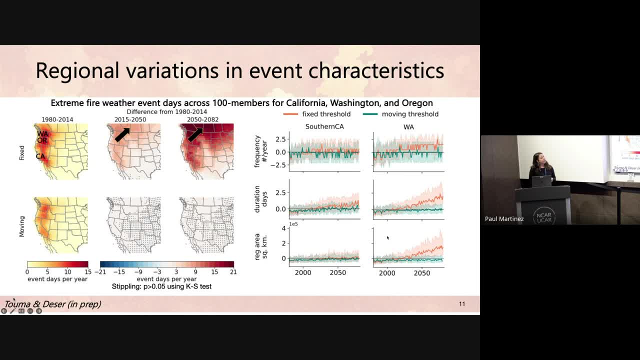 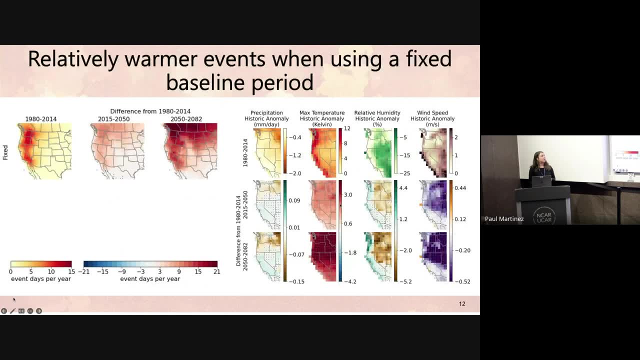 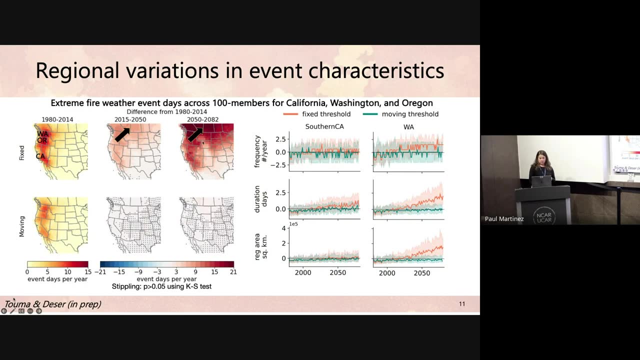 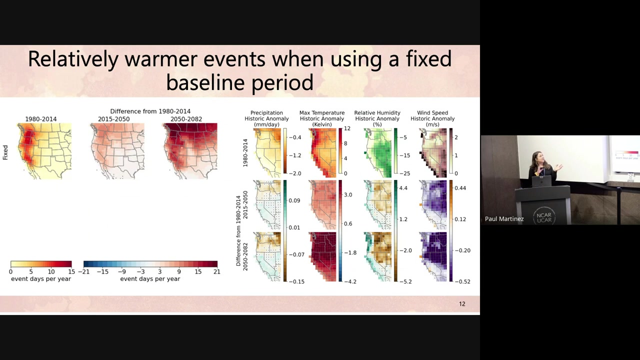 for example, washington has much larger differences in the duration area and frequency of events compared to southern california, which has much smaller increases through times, and that's kind of what we can see from the maps as well. so what is underlying these events? so now the maps on the right are: 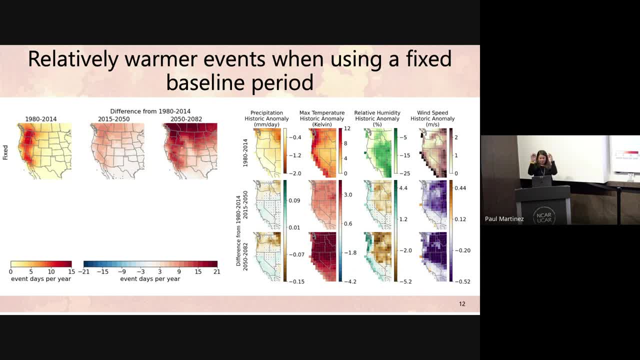 oriented in a different way, where you're going through time from the top to the bottom and each column represents a different variable that goes into the fire weather index, and what we see is that, going into the future, events are much warmer than they used to be using this fixed baseline. so it's really this increases in temperature that are driving these. 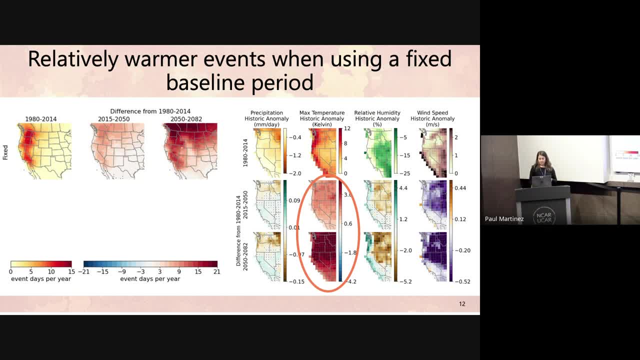 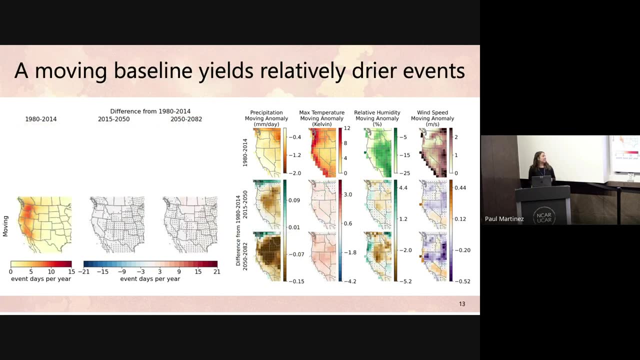 increases in extreme fire weather events over time and there is some drying, some drier events as well, especially in the pacific northwest, and that's probably what's driving these increase, larger increases up there as well. what's interesting is that, with the moving baseline, even though we don't see much changes, 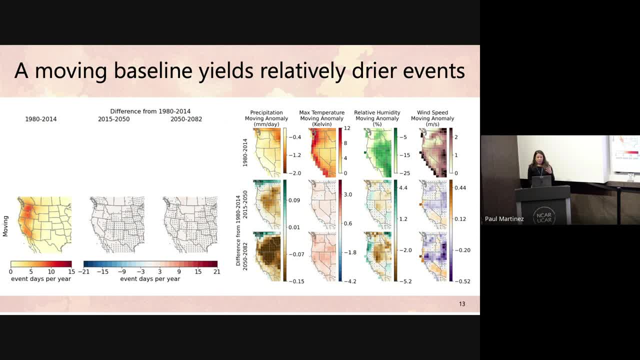 in the actual events. um, like the duration area or frequency of these events, we actually see that they're actually much drier relative to a moving baseline as well. so so this might be what's driving, what's leading to these events in the future years, compared to the fixed baseline. 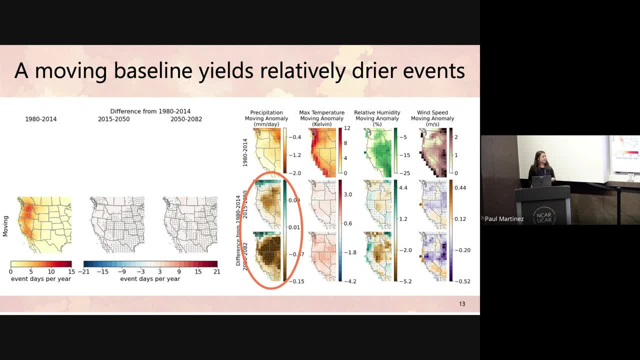 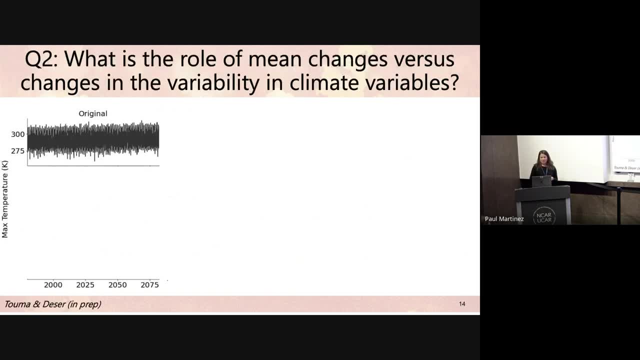 which kind of relied just on the changes in temperature. so we wanted to keep going on with this question and so we are trying to understand better um how the changes of the mean of these variables um lead to these changes in fire weather events, and how the changes in the variability of these variables might change to extreme fire weather. 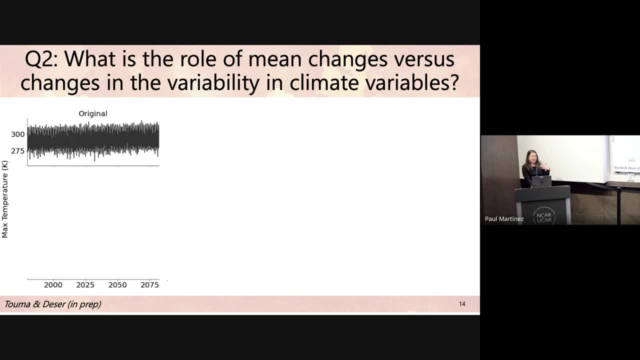 events. so to do that, we recalculated the fire weather, recalculated the fire weather index for our ensemble members, using two new time series. so i'll just quickly go through how we created these new time series. this is um an example of an original what we find in cdsm2, large ensemble. 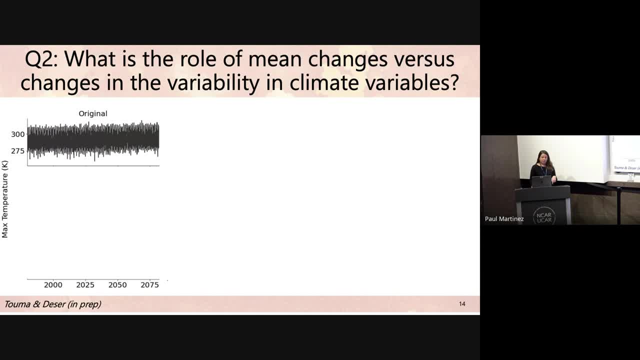 for one ensemble, fine, for maximum temperature. we then create a new time series with the changes in our wayward moved. so these are. you can see. you can't really see, but you do see that the time series, time series that's kind of flattened, and on the right I'm showing what that change in the mean. 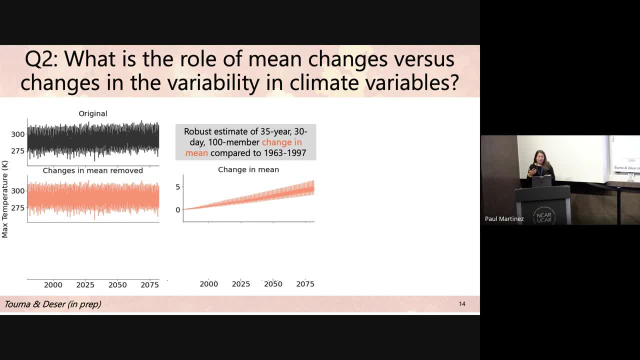 that I removed actually is, and this is basically an estimate of the 35-year 30-day 100-member change in the mean compared to the historic period. so just kind of what the mean looks like compared to the historic period. and then I created a second time series using quantile mapping to kind of 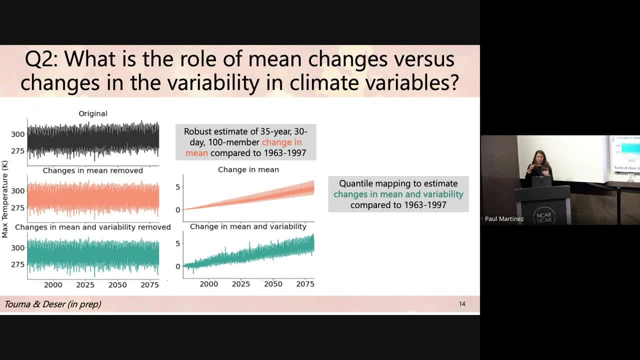 constrain that, the variability and meaning of full time series to just the historic variability and mean. so this quantile mapping is borrowed from bias correction and but we can use it to kind of constrain our time series to just the historic period in both mean and distribution. so you can see what that, what the difference looks like here. so you can see that it includes. 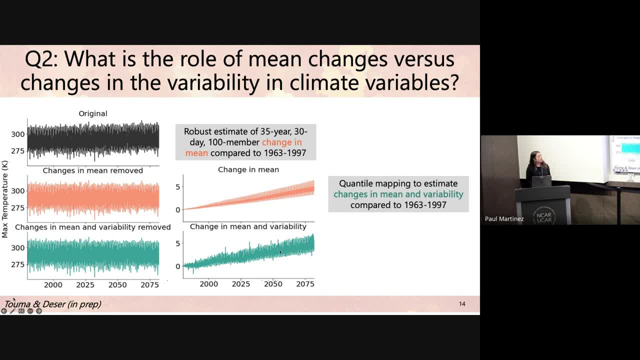 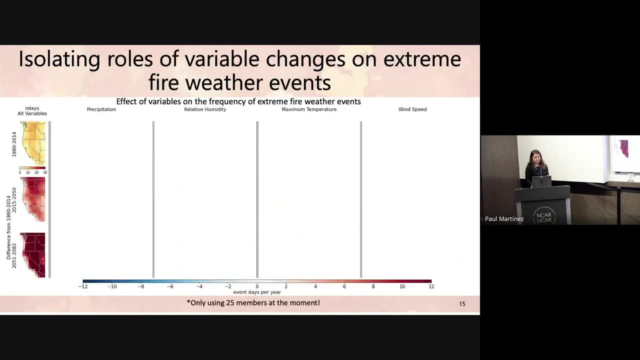 the change in the mean but also includes change in the variability over time. and then we can kind of estimate by subtracting the this teal line from the middle column, from the orange line, to get the change in variability of these time series. so what did we learn from this giant exercise? is that if we look at the changes in the full, 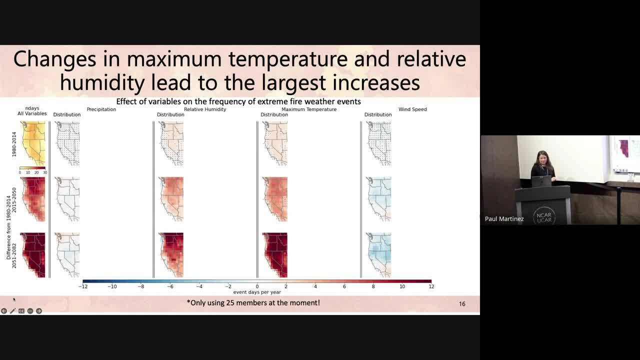 distribution, we find that relative humidity and maximum temperature are leading to the largest increases in the frequency of extreme fire weather events. so the column on the left is what I've already shown you in terms of the projected changes and the columns all to the right is kind of showing 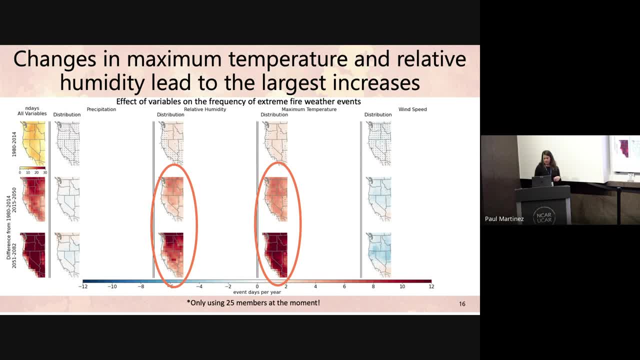 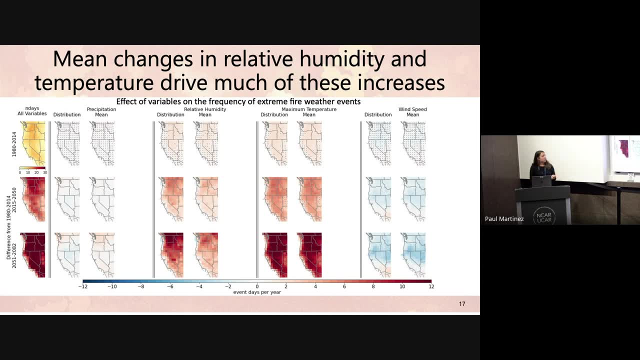 each, the effects of each variable isolated, and then we look at what this, look at the impact of the changes in that mean and we find that it is not only the changes in the mean and the relative and relative humidity are leading to most of these increases in extreme fire weather events. 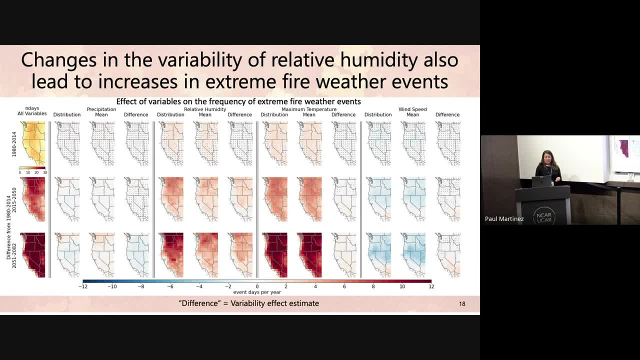 but what's interesting to me is that if you look at just the impact of the changes in the variability, we find that the changes in the variability of relative humidity is actually causing is also causing much of these increases. so it's not just a change in the mean of relative 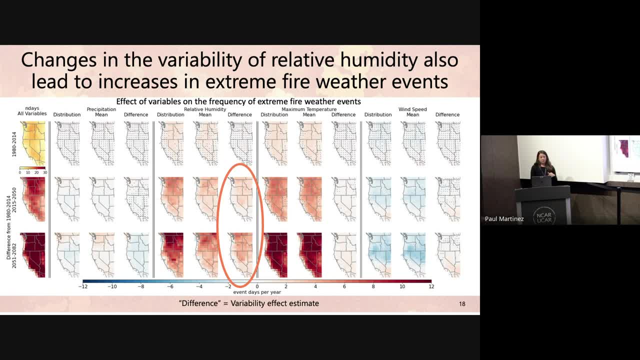 humidity, but also kind of the day-to-day variability of relative humidity that is leading to much of these increases in extreme fire weather events. on the other hand, the changes in variability of other variables seem to have a much smaller impact compared to their changes in the mean. 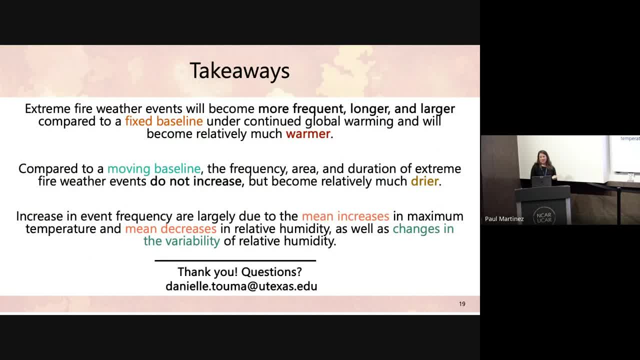 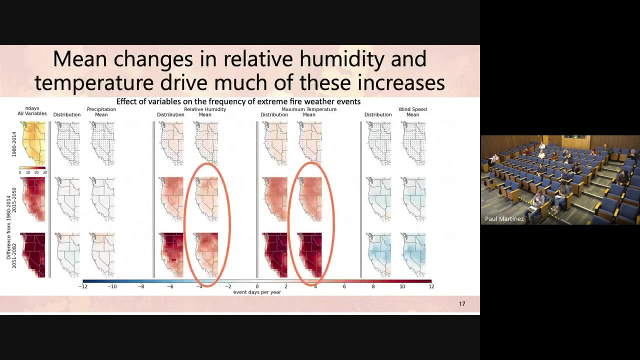 so i'll stop there um and take any questions. thank you, hold on a question. thank you very much. i'm curious about um the definition of the fire weather index um. colleagues of mine in zurich have invested yankee kai and fulton but finish have recently investigated how different. 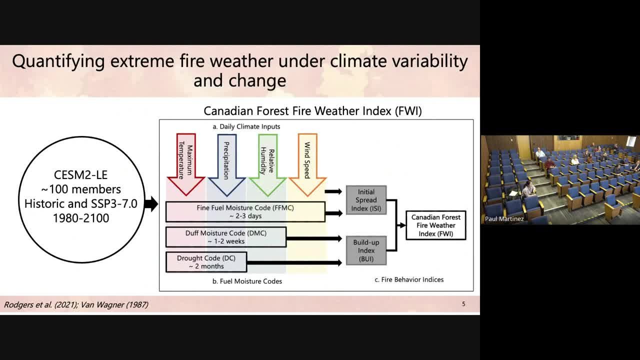 daily values influence your fire weather index. so taking noon values versus daily maximum values and stuff like that, did you uh spend thoughts on that or did you just go for and focus on variability? uh, i just went for this study. we just focused on variability. i have done. 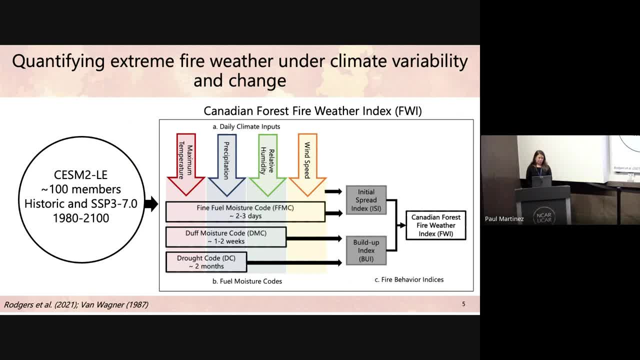 some work with um, other, uh, another um data set, csm2 data set um, and tried to. they didn't have a maximum temperature shape, they only had temperature save. so i actually calculated it with just temperature and we did see some differences where we're getting a much. 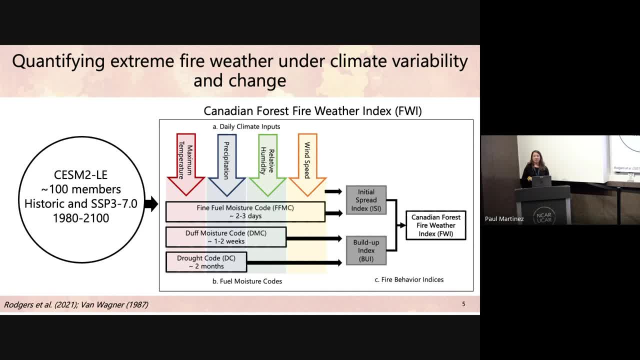 much lower fire weather index values if we only use temperature versus, like average temperature versus maximum temperature. um, it would be. yeah, i think using noon time temperature would be great for all of these, but or like using the actual definitions of. so this is a slightly modified version of the fire. 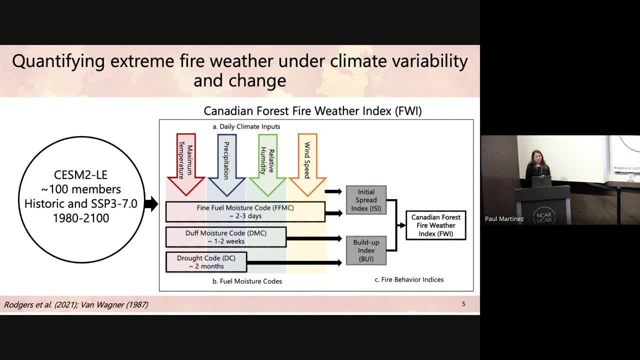 weather index. um, but i i don't want to kind of find new time temperatures in the csm2 larger sample, but if you have a time series that i could easily use, i'm happy to use it instead. um, yeah, but yeah, there's a lot of um different ways. you can kind of modify this to suit your data set. but 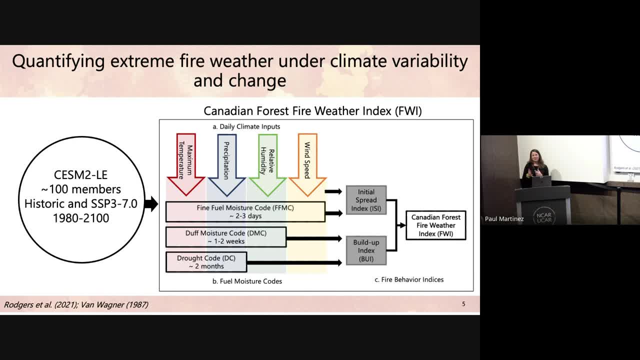 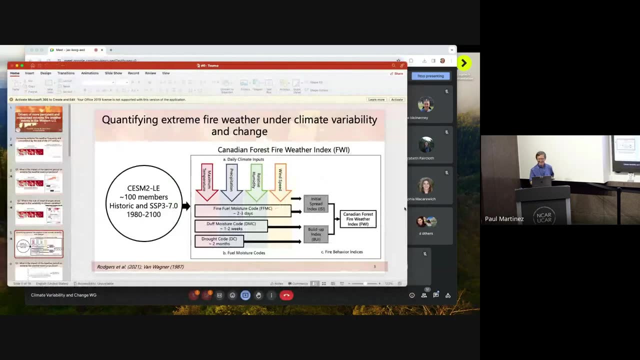 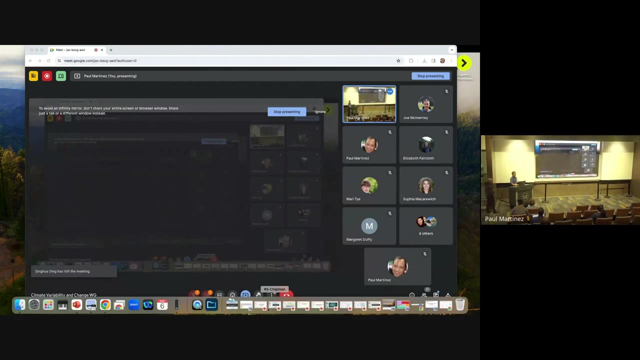 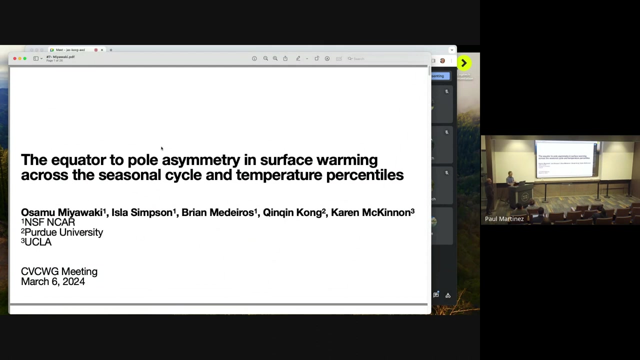 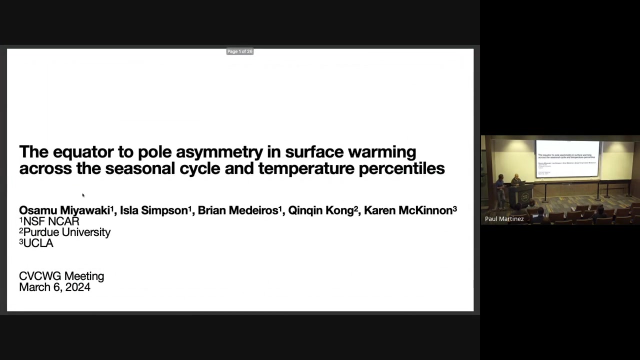 that definitely yields a lot of can yield some differences for different regions. yeah, okay, thank you. thank you, and our next presentation will be filmed by um. the cover page. oh yeah, that's like a. yeah, i found online copyright. thanks. this is in collaboration with aila brian here at ankar, and ching kong and perdu and karen. 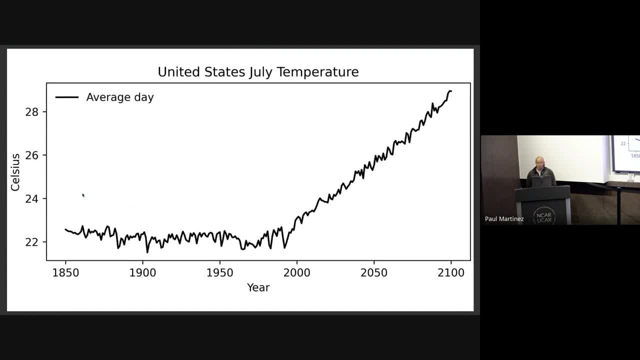 um. so a lot of climate science? um has focused historically on changes in the mean. uh, what we see here: the us temperature in july? um averaged over all july day. so average temperature. we have a lot of mechanistic understanding of how me changes occur. people like feedback analyses. we. 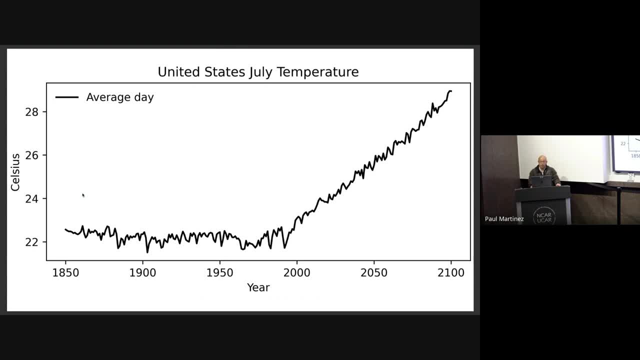 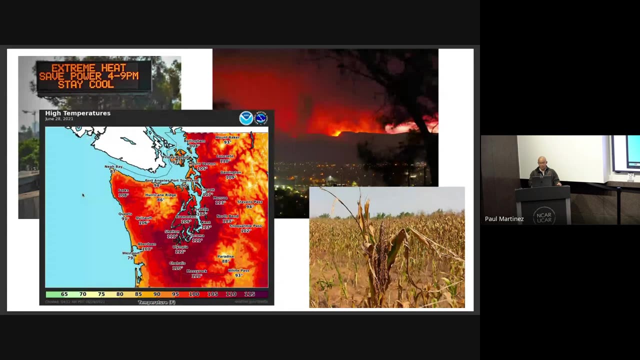 know how. implication or land, ocean, contrasting, warming, all these behaviors about mean changes in climate, i would say is premature. but uh, from a societal point of view we, in a lot of cases we care more about the extremes and the mean. so for things like heat waves and its impact on 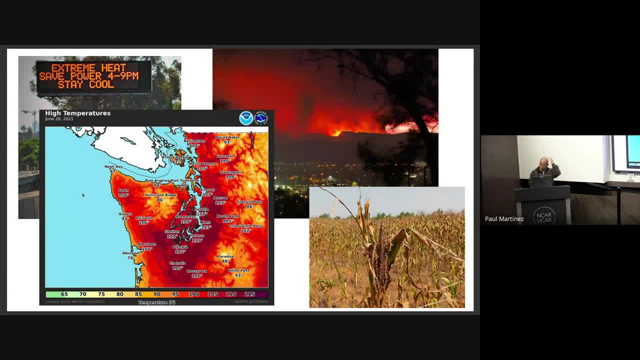 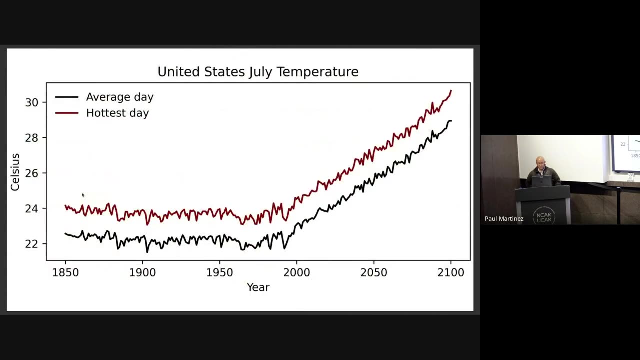 human health, wildfires, as we just uh heard about, and crop failure- all of these tend to be more disproportionately influenced by changes in extremes. so that motivates us to think about how extremes will also change in the future. and then we make uh on this plot show the hottest. 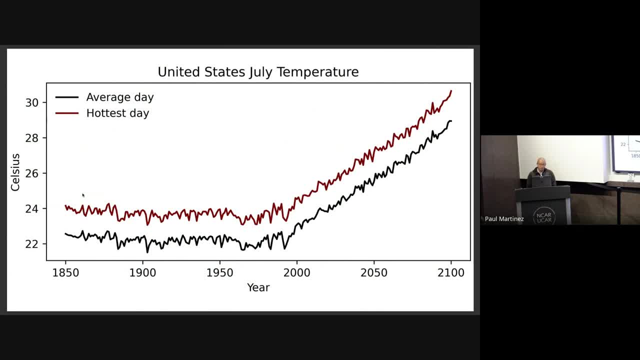 day change so on in july. just looking at the hottest five percent of the eight, at first glance we see something that looks very similar. it's just offset from the mean warming. but um, maybe this is sort of a good lesson and maybe we shouldn't just trust our eyes and seeing. 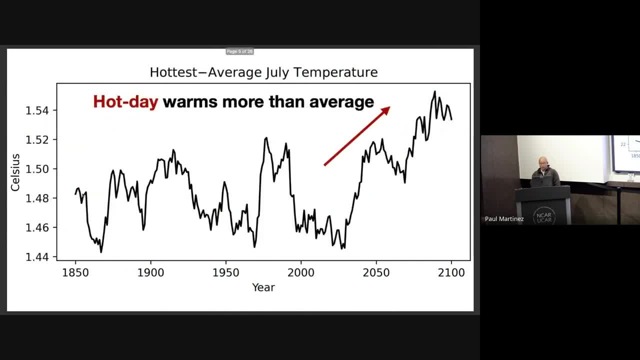 if there's any difference or not, because if you take the difference here um up until about 2030, this is all model world. up until 2030, generally the hottest days are changing pretty much in lock set with the average days, but beyond 2030 we see this pretty systematic rise in how much the hot. 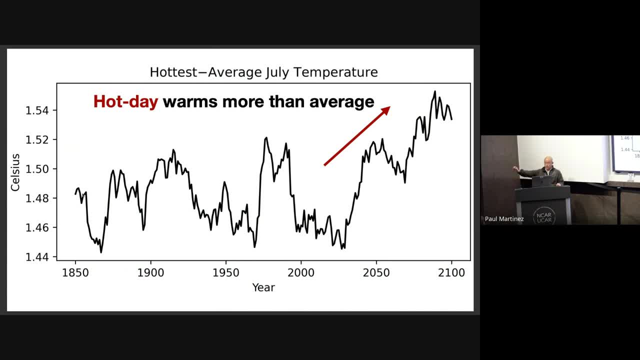 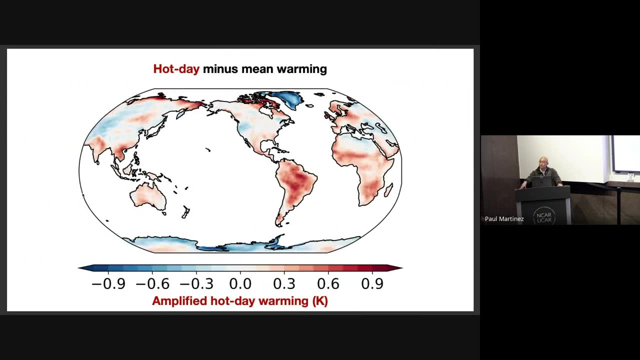 days warm compared to the mean and by 2100 we're seeing uh unprecedented levels of temperature increases in hot days compared to the mean. this is all just average. drove the continent for the entire united states. but if we look at the spatial pattern of what this relative warming of hot versus mean days looks like, it's very messy. 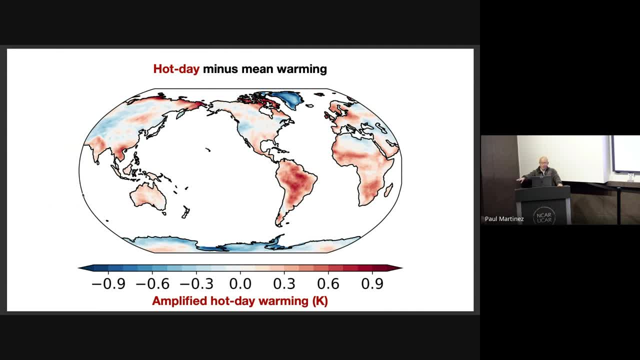 especially in the mid-latitudes. so in the us there's a lot of cancellation going on, where some regions, like the northwest you actually see hot days, warm less than the mean, whereas in the south east you see a very pronounced, systematic increased amplification of warming and quantities. 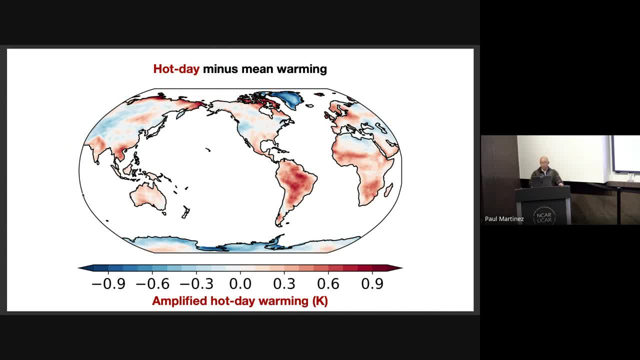 compared to the mean. um so the mid-latitudes is really messy, but if we look in the tropics you might kind of see that there's a systematic warming of hot days that's greater than the mean, and so why is this? one way you can think about it is from the perspective of surface energy balance. 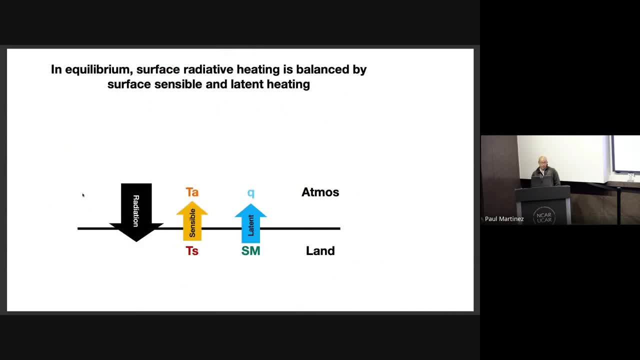 and the idea goes that well, first with surface energy balance, radiative heating balanced by a sensible and latent cooling of the surface or heating of the atmosphere, and in a future warmer world, we have more water vapor. one of the things that we expect from the simple conceptual understanding is that precipitation comes in larger, more extreme. 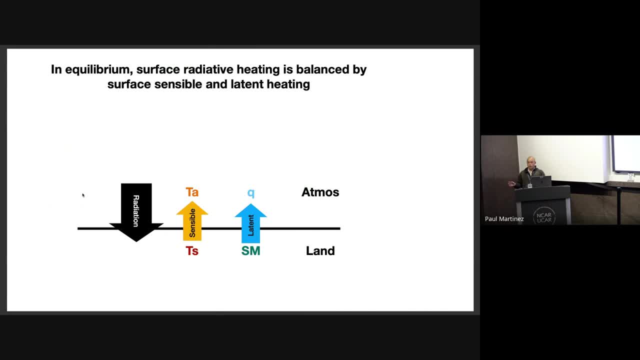 bursts interspersed by longer periods of dry and drought, so that leads to more runoff and a decrease in soil moisture. and since slating heating um to first order, you can think of it just as feeding off of the gradient in moisture between land and atmosphere. the soil 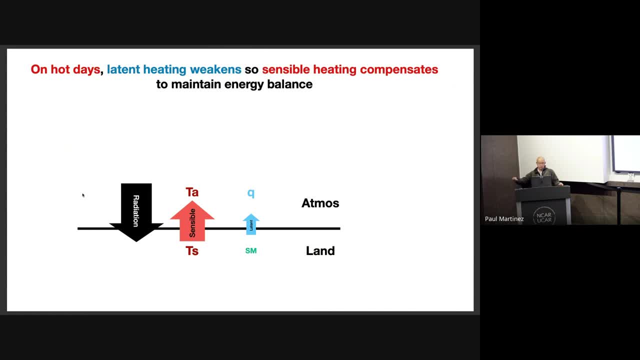 raises and so on, and if you think the sedimentation is more severe and less, and if the soil dries, then latent heat flux will also decrease, and so if there's there still has to be a surface energy balance, the radiative heating doesn't contribute to change that much. 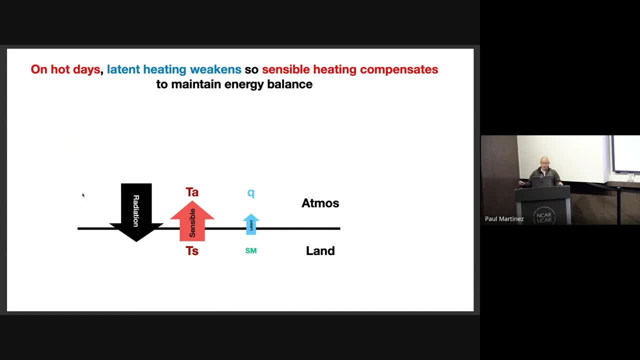 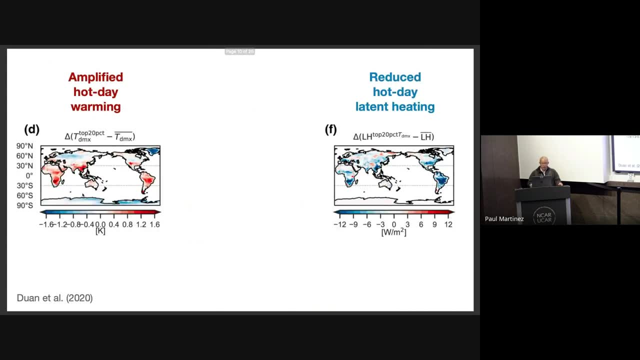 with climate change. so the idea here is that sensible heat flux increases to compensate for this decreasing soil moisture and latent heat flux. and this idea of the repartitioning of surface turbulent fluxes has been shown to explain the spatial pattern of this amplified hot day warming very well, and 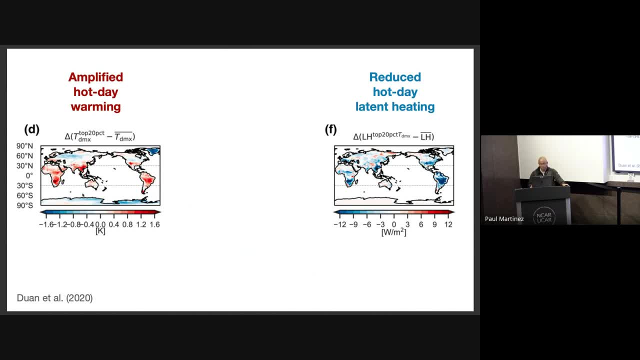 This is work done with CMIP5 data by Si-Chin Kwan. We're seeing the same kind of map of hot day warming relative to mean warming on the left, with the systematic amplification of hot day warming in the tropics, And those same regions also show up as where, on hot days, you get a reduction in lane heating that's greater than in mean days. 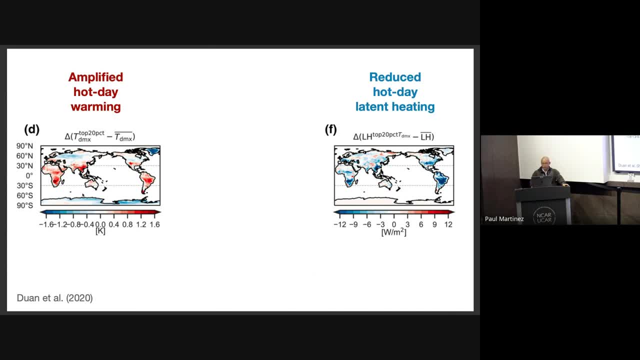 It's all the blue regions on the right panel- And that this decrease in lane heat flux on hot days is balanced by an enhanced sensible heating on those days. This is the center panel now, So this is sort of the understanding that we have for the spatial pattern during summertime. 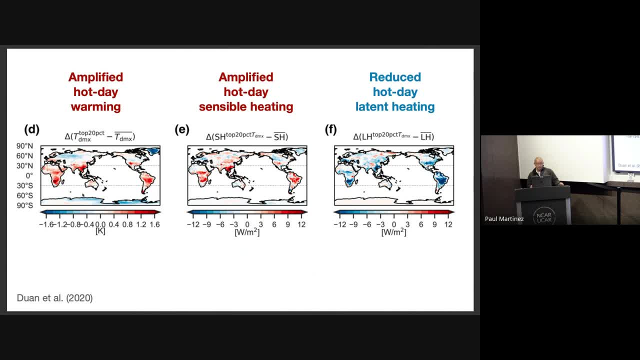 But one thing that hasn't been explored is the seasonal cycle of what this warming looks like, And I think it's important to generalize or think about what the summer amplified warming is in the context of what happens through the rest of the year. So if you look at the 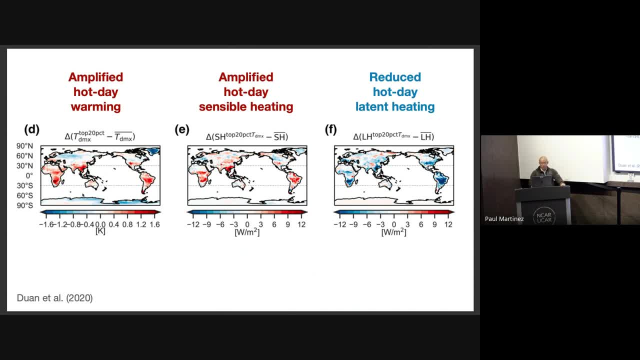 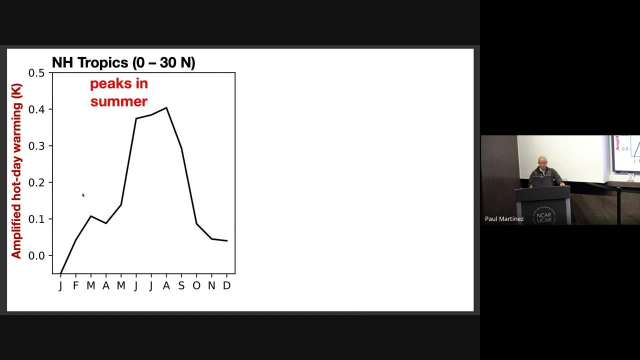 So the seasonal cycle of this behavior of amplified hot day warming in the tropics. So this is averaged from equatorial order of 30 degrees. first, looking at the northern hemisphere, The y-axis shows the amplified hot day warming metric that we've been looking at. 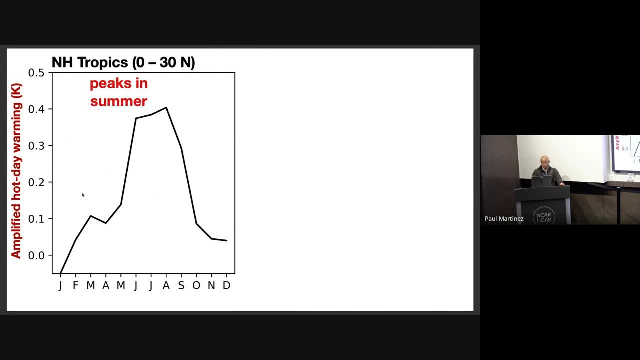 We see that there's a very clear peak in summertime during JJA. If we now look at the southern hemisphere, we see the same kind of behavior during summer in the southern hemisphere. So there's a robust seasonal cycle. We see that there's a very clear peak in summer in the northern hemisphere. 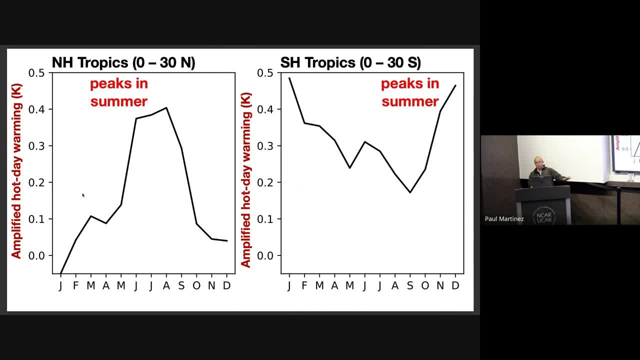 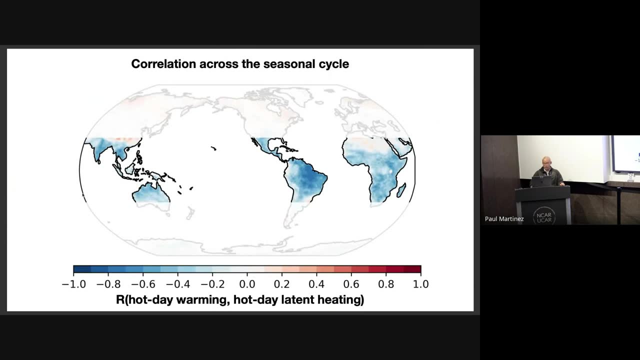 And the first order, you might just think, is the same concept of decrease in latent heat flux being balanced by increase in sensible heat flux. Is that operating also for the seasonal cycle of amplified hot day warming? And this plot shows that it, Yes. the answer to that question is yes. 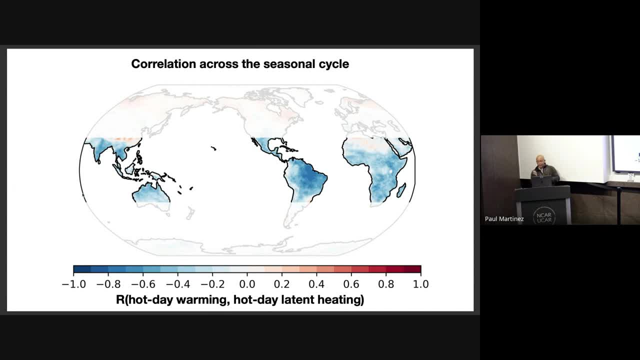 If you take the correlation of the seasonal variations in amplified hot day warming against the change in hot day latent heat flux, we see a very strong negative correlation across the seasonal cycle. So the same mechanism is able to explain the seasonal cycle in amplified hot day warming. 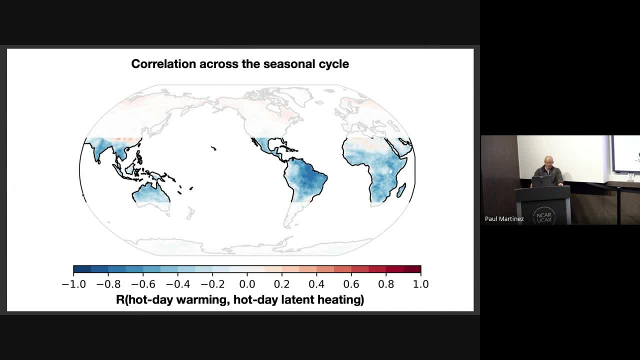 So the question becomes: why is there an amplified decrease in latent heat fluxes in hot days, just during summertime, or more so than during the rest of the year? And so one way, We mentioned that soil moisture is a key variable in controlling latent heat flux. 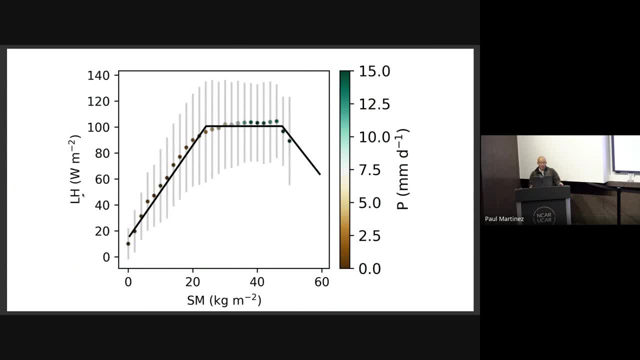 And if you actually do it more quantitatively, if you do a more quantitative analysis of what the relationship between latent heat flux and soil moisture is, it's a very non-linear function. So I said that latent heat flux scales with the gradient in moisture between land and atmosphere. 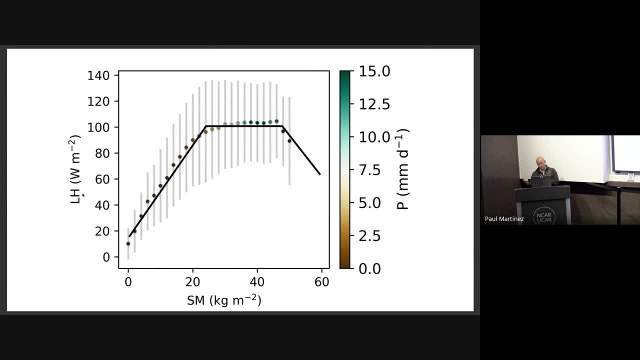 So all else equal. if you increase the soil moisture as you go to the right of this plot, you would expect a larger latent heat flux, because you're increasing the gradient between the moisture in land and atmosphere, And that works. This positive slope to the 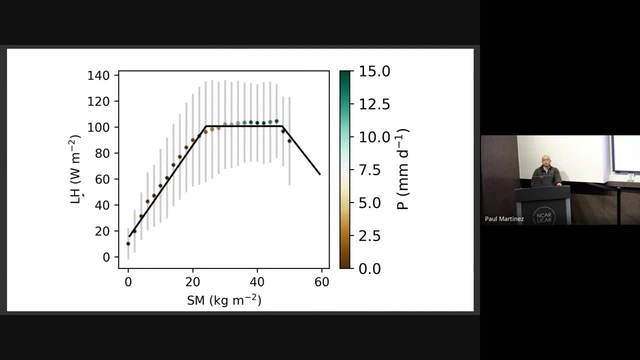 to the very left of this plot. it works until a certain point, because after a certain point your soil moisture is plentiful, but you actually don't have enough energy with the latent heat, radiative heating, which is the other component that's important. 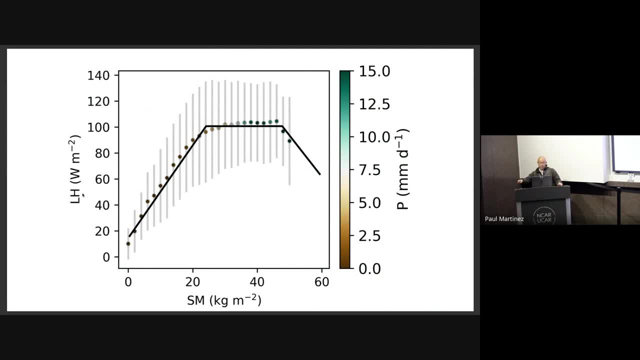 So at some point you plateau and you actually get a negative relationship in really moist days, because in those days the atmosphere becomes saturated. So that's the relationship we have, And the key thing to get at here is that, wherever you're, to the left of this plot, 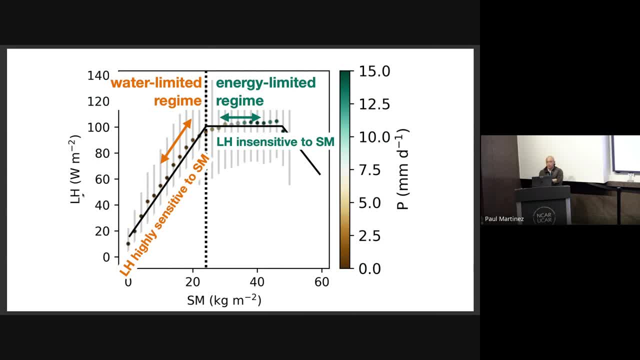 this dashed line, you're going to have a large sensitivity of latent heat flux changes, soil moisture changes. wherever you're to the right, you're not going to have a large change. So we can envision larger changes in latent heat flux happening for hot days. 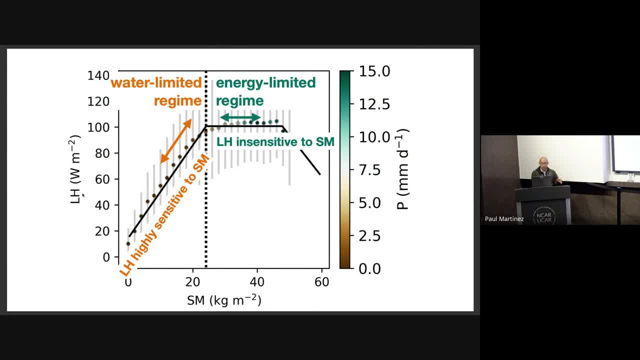 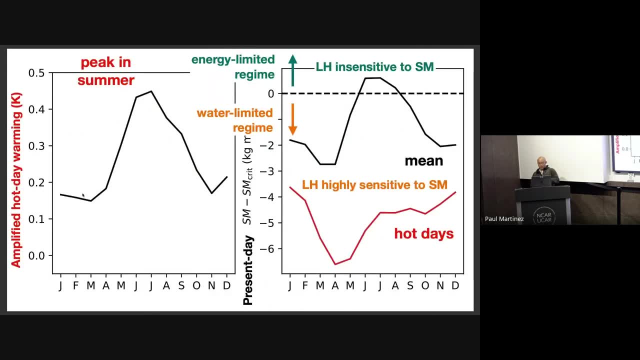 if those days are left of this critical soil moisture, this vertical line, but if the mean day is to the right. So if you plot the seasonal cycle of what part of that curve is the day in for the seasonal cycle? this, On the right panel of this plot I'm showing the deviation of the soil moisture on those days from the critical soil moisture. 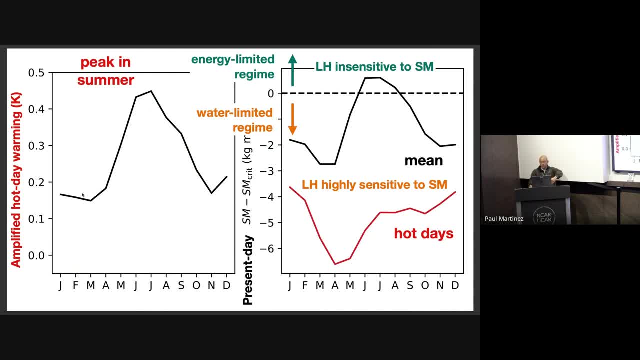 Wherever you're below this dashed line, you're in the water limited regime, and whenever you're in the energy limited regime For hot days, it's always in the water limited regime throughout the year, But for the mean days in the summertime. 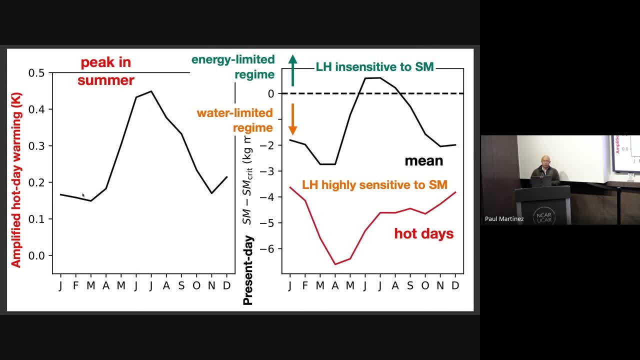 this is when you have the shift of the ITCZ towards the hemisphere where the installation happens. That's the rainy season, That's the monsoon season in many parts of the tropics, So that moisture gives this push of the mean days up to the energy limited regime. And so you get this amplification in summertime because that's the unique time of the year when, on the typical day, is moist And so it's insensitive to changes in soil moisture. But hot days are sensitive to soil moisture changes, So that explains the seasonal cycle in the tropics. 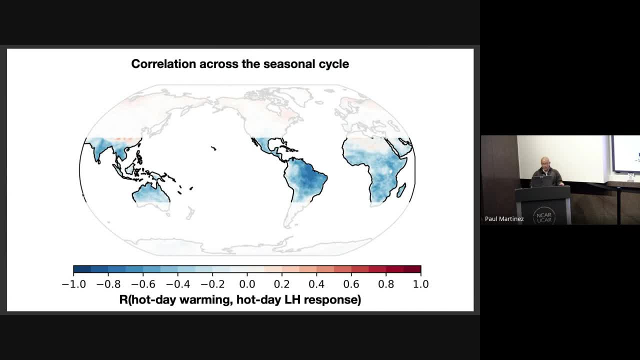 This whole latent heat flux picture, But in the high latitudes it's not that simple And it's this whole hypothesis doesn't work at all anymore, in fact, because they're positively correlated. It's not a repartitioning at all. 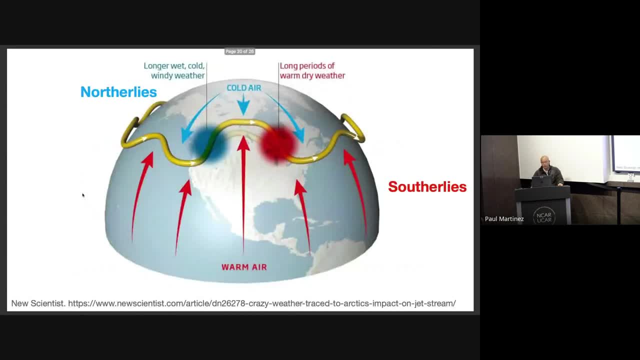 So what's going on in the high latitudes? Well, in the literature, the way we think about temperature variations, cold or warm anomalies in the mid and high latitudes where we live, are these where the, where the anomaly they're coming from. So if you think about cold, cold days, that's usually associated with troughs in the jet stream, where you have cold Arctic air coming in from the north. Warm days are the exact opposite: ridges in the jet stream, where you have warm tropical air coming in from the south. 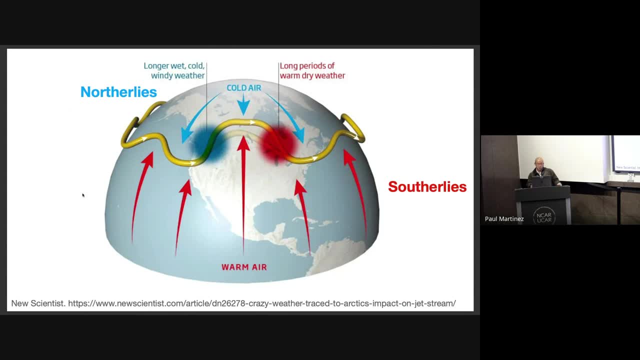 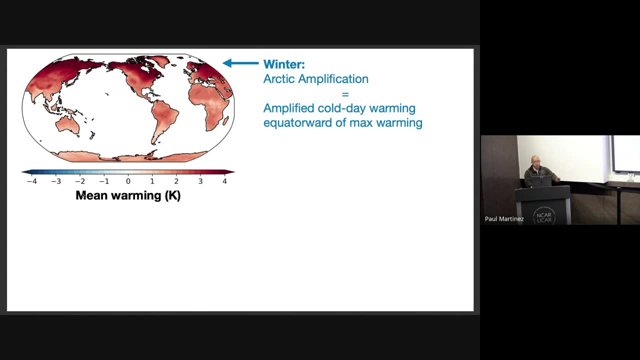 So then you can sort of get a very simple conceptual understanding of what might happen, based on just the structural, the spatial structure of mean warming. So in the wintertime the maximum warming happens in higher latitudes. This is known as Arctic amplification. 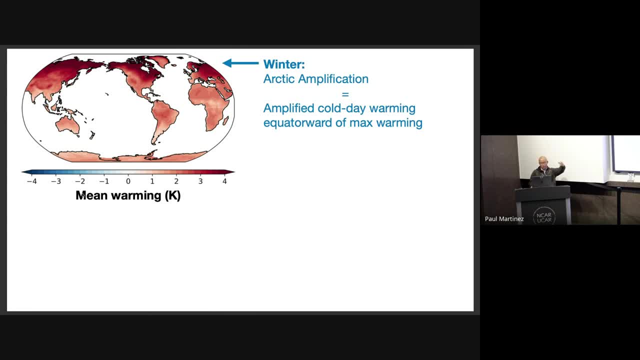 So what that means is that wherever you're equatorward of the point of the maximum warming, you're going to feel a larger warming on cold days with sources that cold air is coming from, compared to any other day, And so in winter, we expect cold days to warm just from this very simple picture of what is a cold day in the extra tropics. 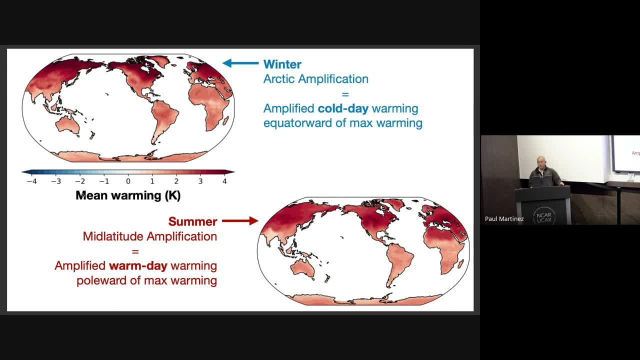 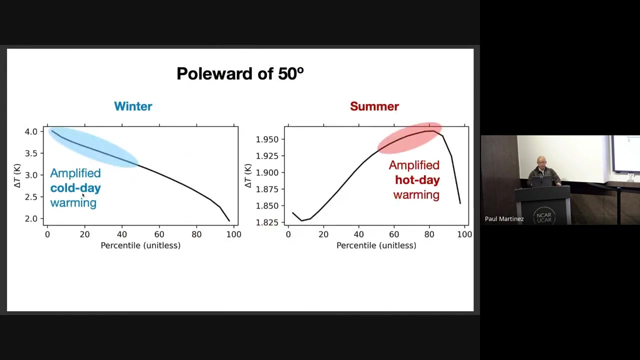 And in the summertime you actually get largest warming in the mid latitudes, And I guess you could call this mid latitudes. So what theробes considercu 밖에 will find in central partic Apache National Park are in land cold or 50 degrees, and look at the warming as a function of the percentile of the day as a 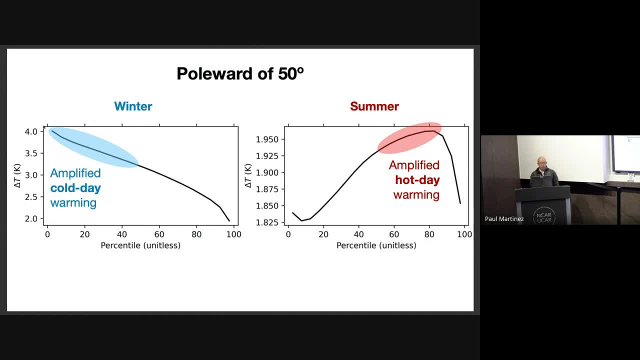 function of temperature percentile. you indeed see that during winter you get the largest warming in cold days, so below the 50th percentile, and during summertime it's the exact opposite: you get the largest warming during the hot and the warm days. there's a lot of open and i'll end with a few open. 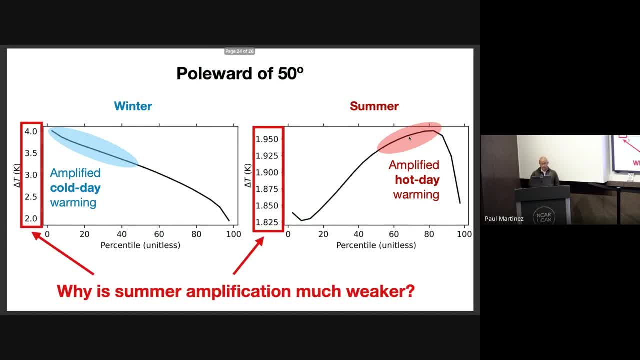 questions. this is still ongoing work, so i'm interested in hearing some ideas, if you have any. there's a. if you look at the y-axis, there's a huge difference in the amount of warming. the amplification on on the cold days is much stronger in winter than the amplification of 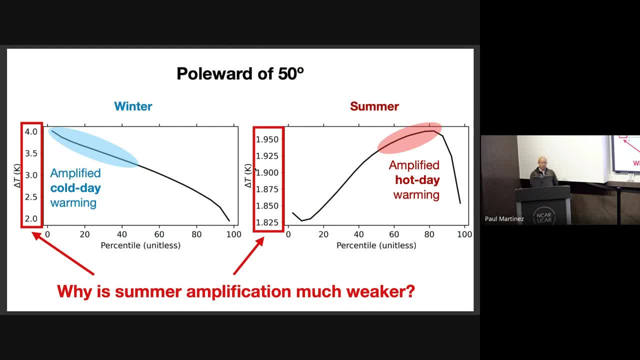 warming on hot days in summer, and this i i don't think this has been explained in the literature and it's actually not. i don't think it's that simple because if you look at the actual temperature affection, it looks seasonally symmetric, so that temperature of action. 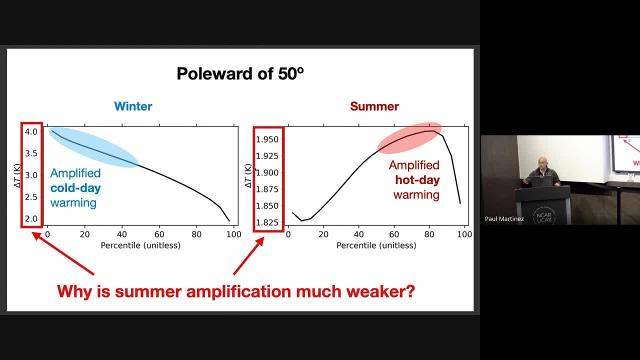 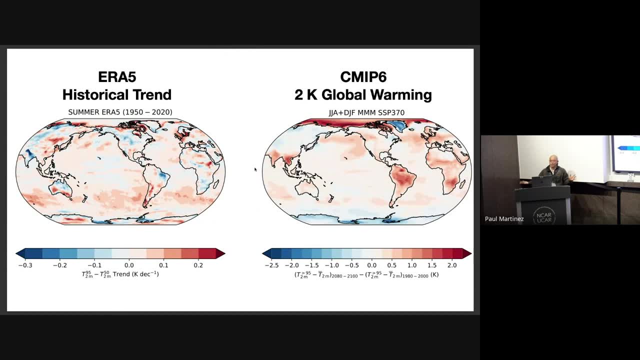 seasonal cycle doesn't really. it's not consistent with what we see in terms of surface warming- i think an open question there- and all of this has focused on the model world, so we obviously want to connect it back to observations and, if you look at this, amplified hot day warming and historical 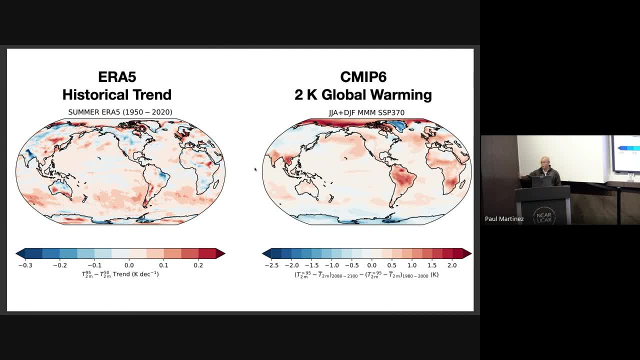 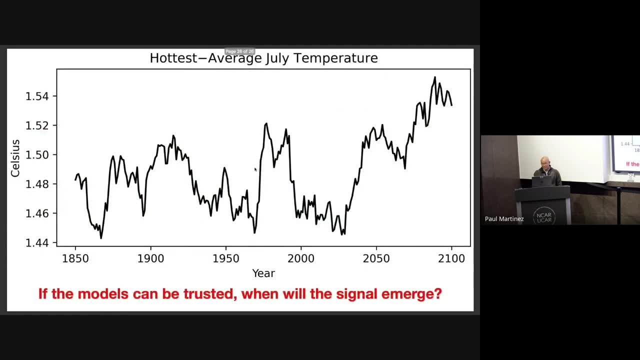 trends. it really doesn't look anything like we project the people climate models project into the future. of course it doesn't mean that we can't trust the models. we did say that there's a lot of you know noise going into this time series if we just go back to the us, so maybe it's just that. 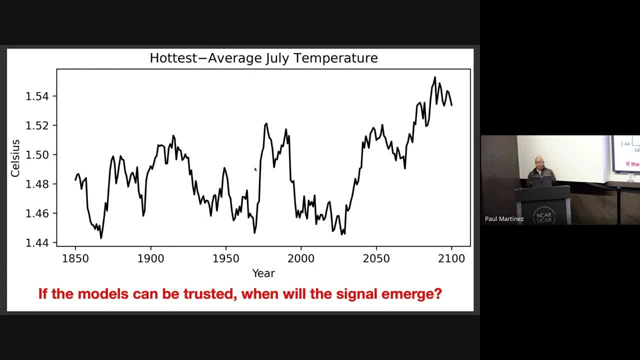 the signal has a lot of impact on the climate models. so i think it's an open question there and all of this has focused on the model world, so we obviously want to connect it back to. observations hasn't emerged yet, so there's good we could, uh, explore these questions. if you look at like 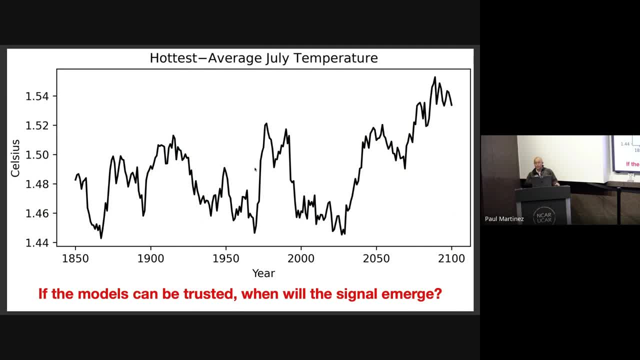 large ensembles and look at the historical trends. are any of those ensembles consistent with observations and maybe that gives us some confidence that the models can be trusted? and if the models can't be trusted, when do we expect the signal to emerge? these are all open questions that 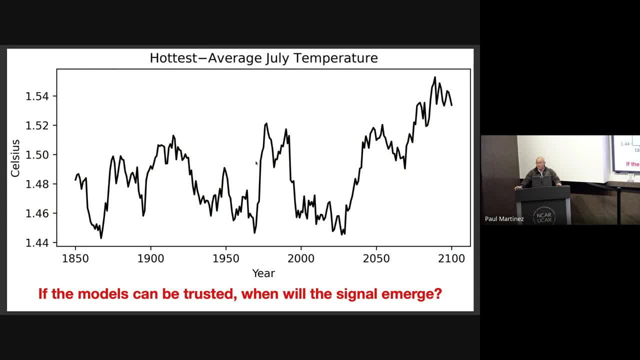 i'm thinking about and i'm happy to take any suggestions or questions. now i have one question. so isla recently showed some work, that the surface moisture is not following the models, and so i'm wondering, given that you're living in model world and we know that this? 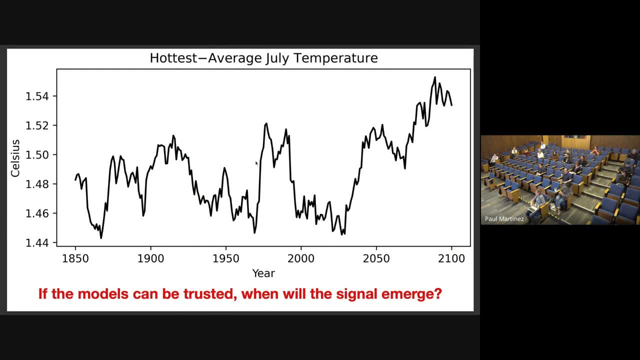 bias exists, do you expect the hot day amplification to be even more, given that kind of inability of the models to capture um like surface moisture decreases right, so it's hard to sit. so i kind of looked at the tropics and the highest latitudes and those. 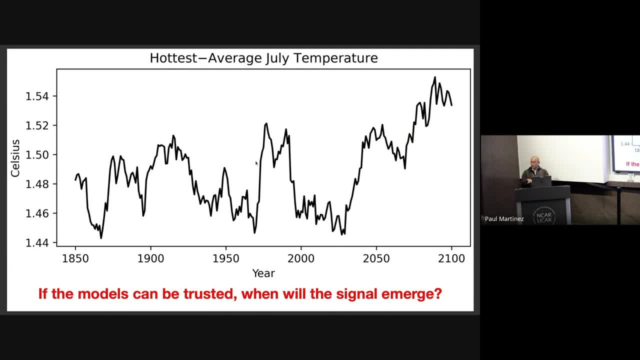 air and dry regions, except for, like many of the sahara or generally, is we parked the latitudes i didn't focus on? so if we, there's a work by mike byrne where, if you look at the tropics only, you expect more warming if the days get, or those days are, drier in terms of humidity, which is what 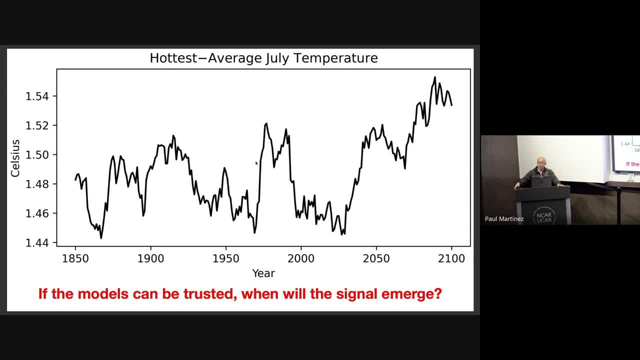 i look for so that. so if you just blindly apply mike's theory, then i agree with you that models are probably maybe even underestimating what the amplification might be for hot days. but i don't know if we can extend that to the arid and semi-arid region and maybe i- i can't remember i love was that bias. 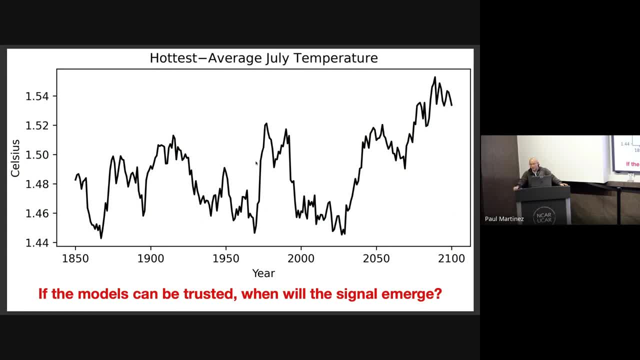 also like beyond arid and semi-arid regions? is that by hysteria it was there in the most arid times of the year in other locations? so i definitely think that's a good question. i'm going to have a look at the other questions in the questions section because it's kind of up to you. 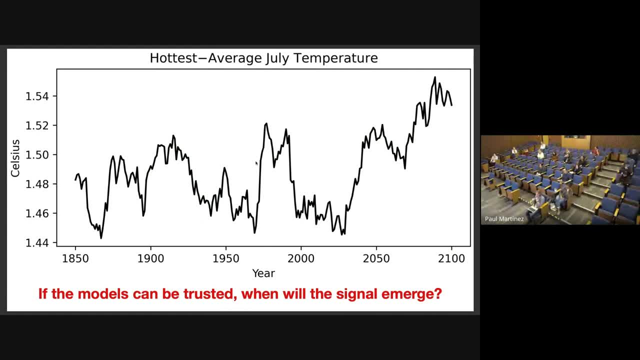 um, actually i have a question which is, yeah, in the tropics, and in the tropics maybe, i don't know- is that the models are constantly needs to be dry. so the assumption is that the models just keep, are keeping on evaporating and reality doesn't seem to do that. so it seems like it could impact that, but 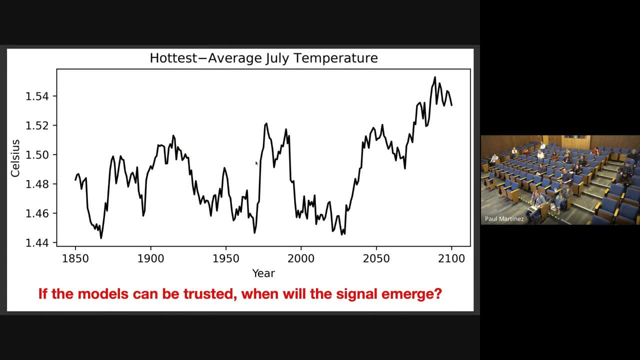 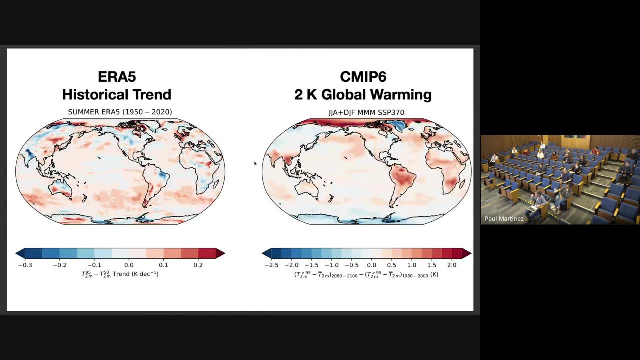 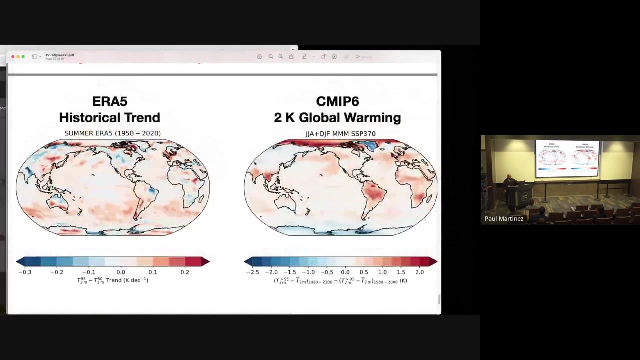 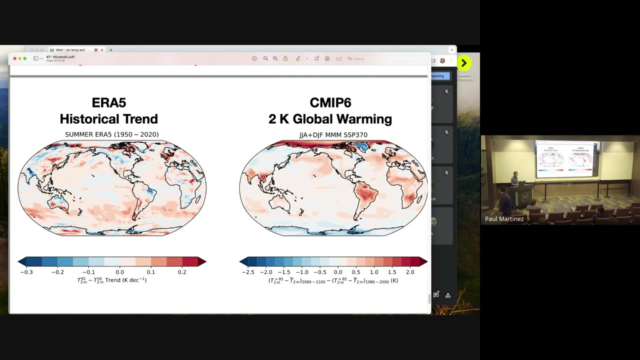 that we haven't looked at temperature, but yeah, i think there are some regions in the tropics, like where it was an issue, like somalia, yeah, but yeah, morocco is in your area, but you're right, that mostly is in the subtropics. thank you, thank you. next time we'll keep going. don't end shop. 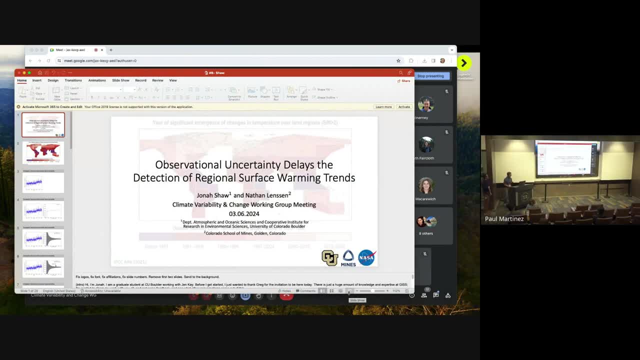 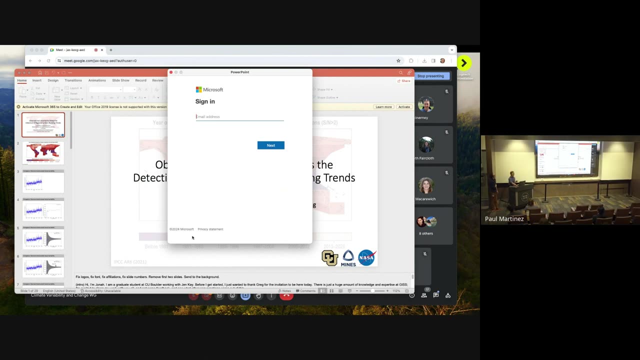 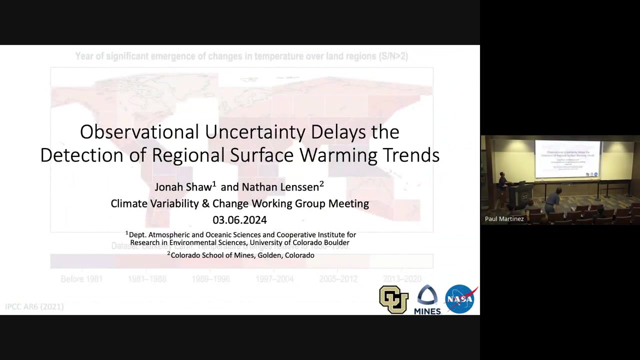 you. let's see if I can this. hi, Jonah, I'm a student at CU. I'll be talking today about something that I guess someone was mentioning a little bit, which is emergence and actually detecting changes, and specifically, I'll be looking at surface temperature trends from a regional perspective and being able to 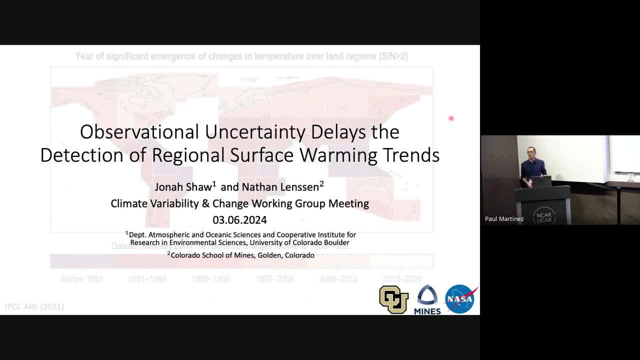 incorporate some of the changes that we've been talking about in terms of how we can incorporate estimates of observational uncertainty into this, our ability to kind of detect and attribute these trends, and this is work that I've done with professor Nathan Watson at School of Mines, so, sitting behind this, 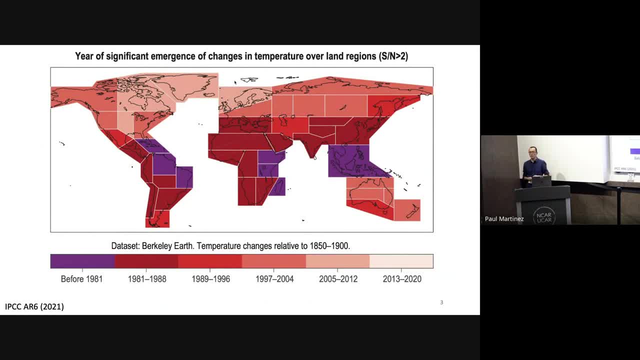 figure or this title is this figure from the executive summary of the most recent IPCC report? so what we're looking at here is that in IPCC regions and years in which we're able to kind of detect a surface temperature change- and what I'd like to point out here is that we tend to see this kind of spatial 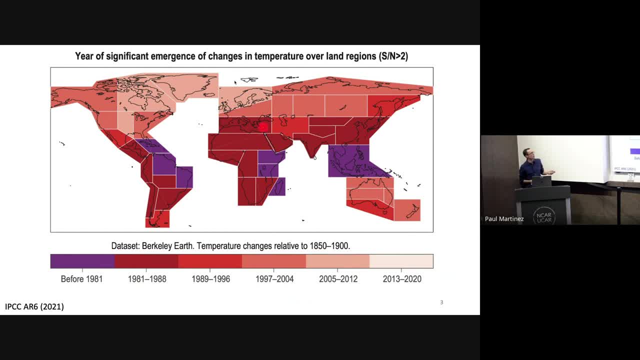 structure of earlier changes emerging in the tropics and that in the northern hemisphere and high-rise. we see a kind of lengthening amount of time for us to do detection, and what this is saying here is here of significant emergence is that our ability to detect and attribute changes is fundamentally a comparison of 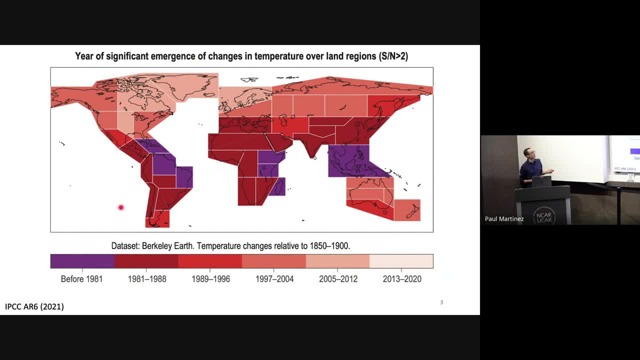 change and variability. so we know that we see rapid change in the polar regions, but that there's also high variability. so this is kind of can be simply thought about as a signal to noise question, but it's really important is that we can detect changes at the global scale, and we've been able to do. 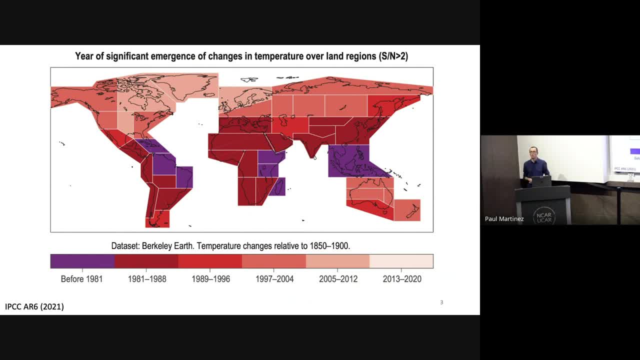 this for a while, but of course, we live on a small scale, a scale that's even much smaller than these IPCC regions, and so in our ability to kind of have granularity and detecting change- I think is important for communicating science- and also thinking about the processes that we're dealing with and the 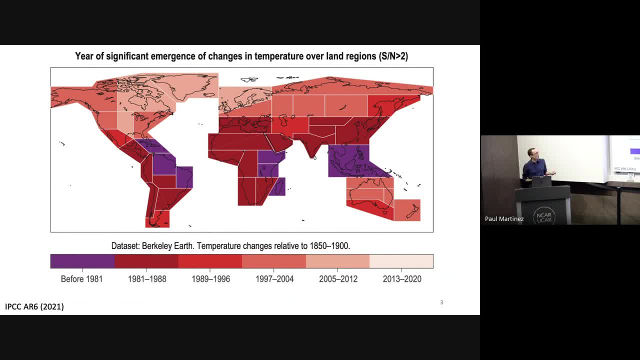 processes that are driving the changes themselves. and the last point that I'll make is that this figure from the IPCC report does not account for any observational uncertainty, so we assume that the record here- and this is the Berkeley Earth data set- has no uncertainty associated with it, and so you know our 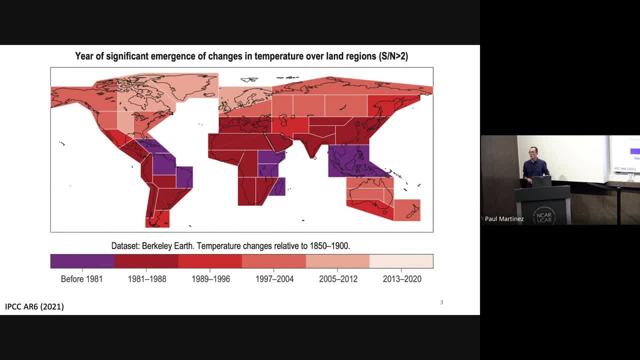 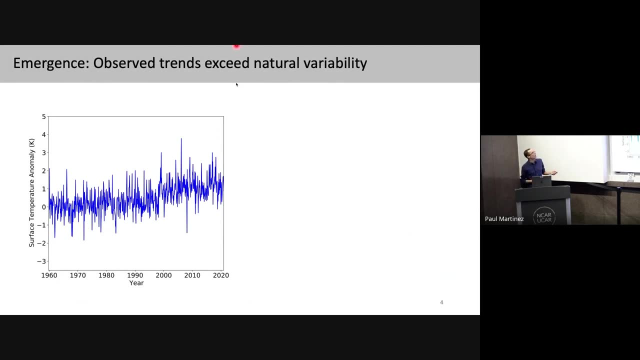 uncertainty is going to be spatially and temporally heterogeneous, and so we're going to incorporate that uncertainty into these estimates and see what happens. um, to briefly talk about this kind of signal to noise question of climate change, detection or emergence, the simple quest or kind of sentence I'll give you is that emergent. 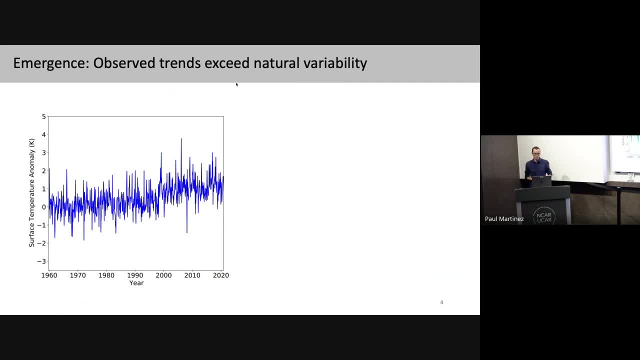 is when an observed trend exceeds natural variability. and so if we start with a time series- of circuit temperature, this is just in one of those IPCC regions and we convert it to an observed trend by starting at three years, kind of regressing out the linear fit, taking that trend, going to a fourth year, recalculating our trends. 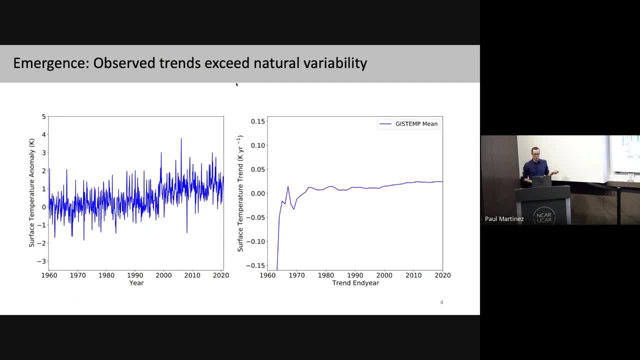 and then kind of iterating that forward in time. so now we've moved in the right panel to a trend space, and so what we can see here is that, um, there's kind of a lot of noise and initially there's a negative surface temperature trend in this time series. but as the length of our record 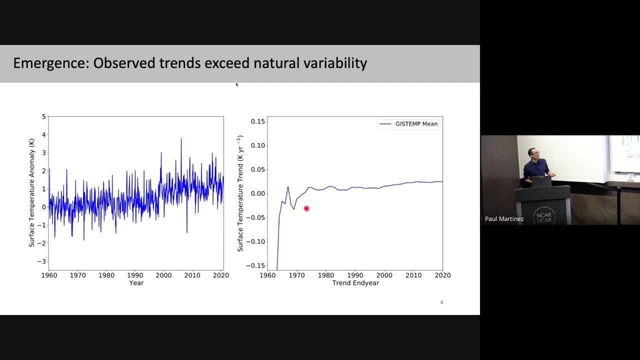 increases. we see a pretty clear um positive trend that actually kind of increases in the last two decades of the record. but to actually kind of complete the sentence is that we need to take this observed trend and compare it to natural variability. and how we get that here is by using a pre-industrial control run of a climate model. 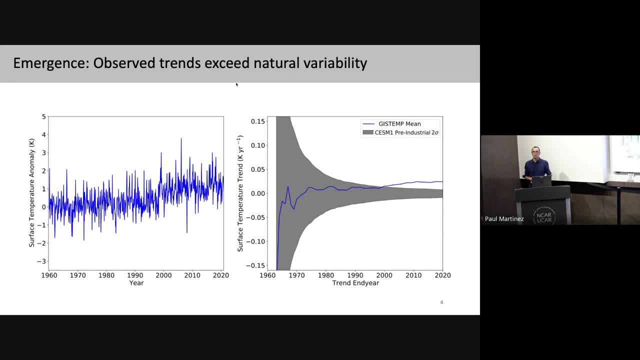 simulation. so this is the CSM1 pre-industrial control simulation and we've kind of created this now cone of internal variability that we're comparing our trend against, and we do this effectively by resampling traps in the pre-industrial control and then explicitly determining confidence intervals. so, for example, we have a 10-year trend from our time series, from 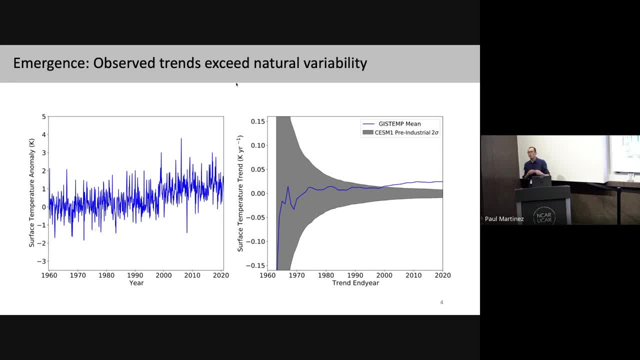 1960 to 1970. but we can resample all 10-year Trends from 1800 years of the pre-industrial control simulation and then just construct for 95 confidence interval from all of those Trends. so now we can look and say when does our trend exceed natural variability? and it turns out that it's right. here we can kind. 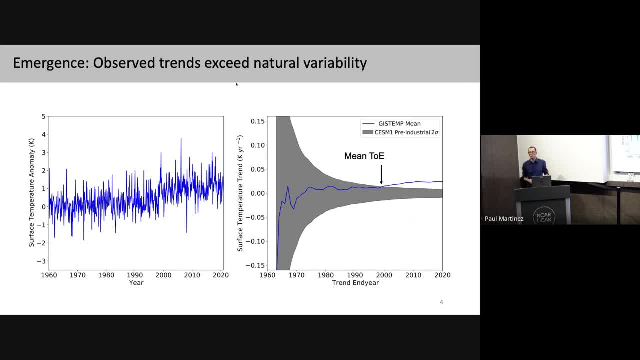 of visually identify it, and so this toe is our time convergence. but now what we're kind of adding to this kind of standard format for looking at detection is that our surface temperature trends like that, they look like this, they're uncertain, and so a more robust and strict method of detecting. 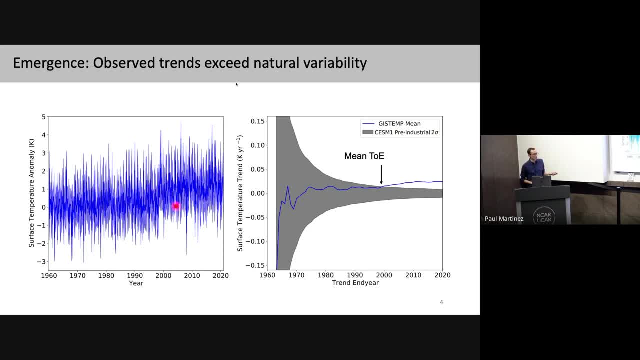 climate change means that we need to construct a confidence interval on our Trends as well, and now we can wait until all of those Trends are detectable, and this is like actually kind of accounting for what our surface temperature records actually look like and how we do this. 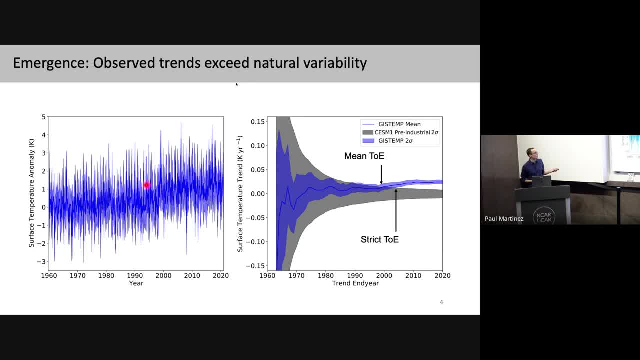 just to kind of explicitly describe it is that this data is from the GISTAM uncertainty ensemble, which gives us very equally likely surface temperature members, and so we calculate the Trends for each of those 200 members and we calculate the time of emergence for all those members and our strict time of 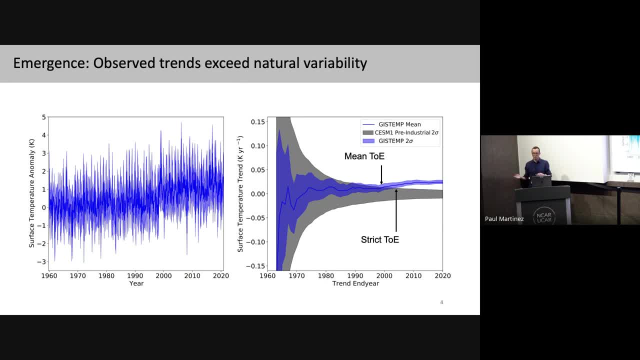 emergence is when 95 of them are distinct from the pre-industrial, and so we can see here to kind of answer the question or motivate: the title of the presentation is that there's a delay between our mean and our strict. in this case it's about four years, and so you can kind of have your own. 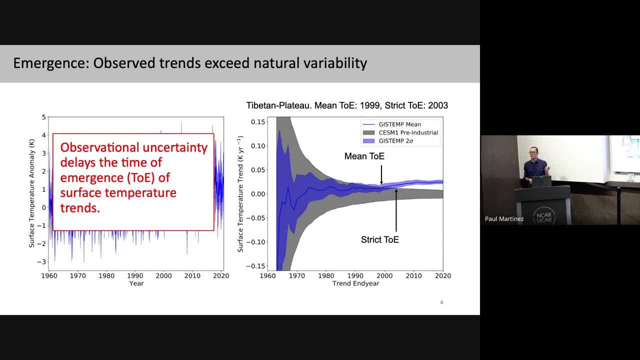 opinion about how much that matters, but I'd say it's not something we should ignore. and so we are getting delays and our ability to detect the surface temperature Trends just from the observational certainty. so now we can take this analysis. we've done it here. this was just kind of picking the Tibetan Plateau region for. 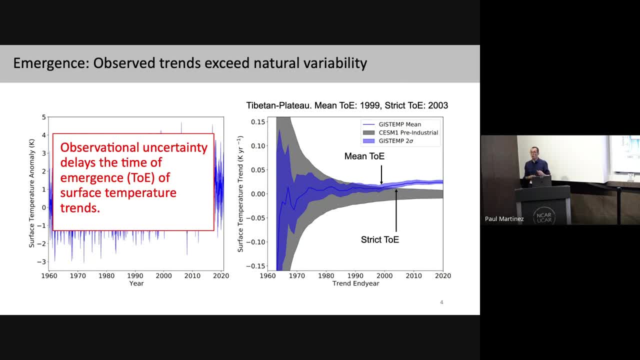 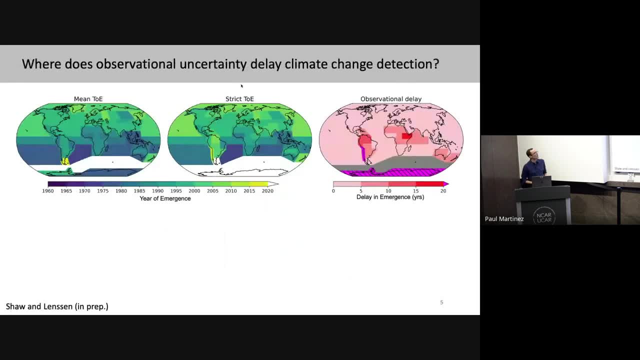 no specific reason, and we can repeat this analysis for all those ibcc regions and see what kind of spatial free features we get in our time of emergence, in our delay, and so that's exactly what we're looking at here. we have this mean kind of standard. previous definition. 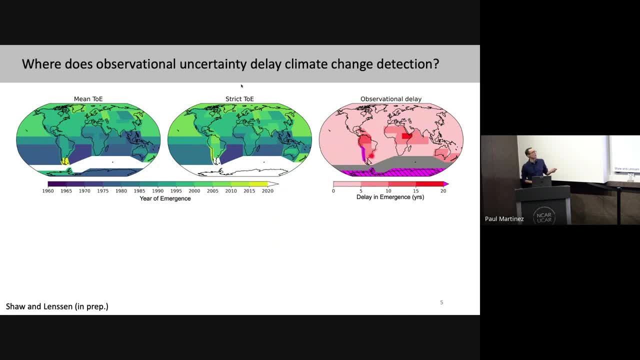 of time of emergence, our strict time of emergence, and then the difference between the two is our delay. and so I think we'll point out here is that for much of the globe our delay is in kind of that one to five year region that we saw with that example region. but if we look, there is regions. 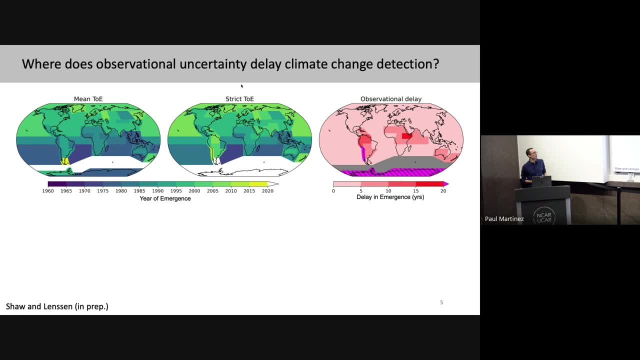 that are kind of specifically in the tropics and also in Antarctica, where we're seeing delays that are five upwards of 20 years. so the inclusion of this observational uncertainty is really important in specific regions and additionally in that ipcc plot we saw that these regions are actually tend to emerge. 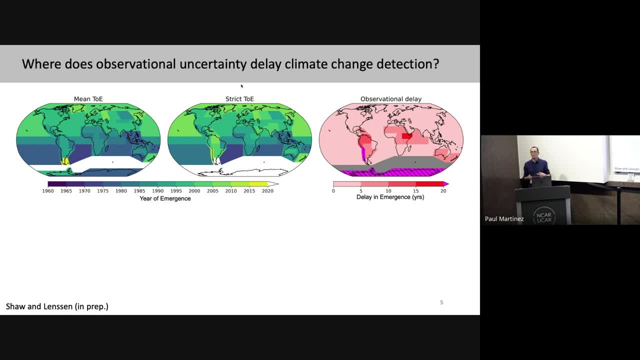 earlier, when we ignore observational uncertainty, and so the effect for accounting observational uncertainty is flattening a bit of that spatial structure that we were seeing in our time of emergence, but kind of going back to the point that granularity is actually really important for understanding climate processes during communication. is that these ipcc regions are? 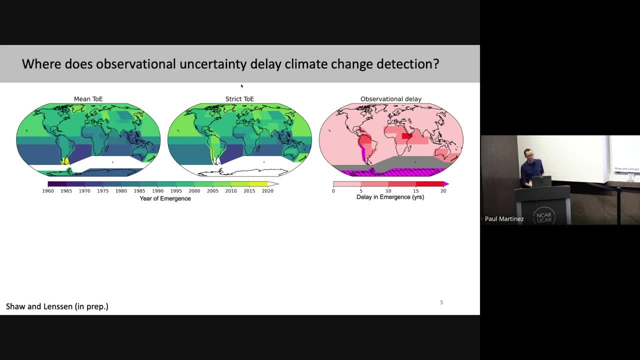 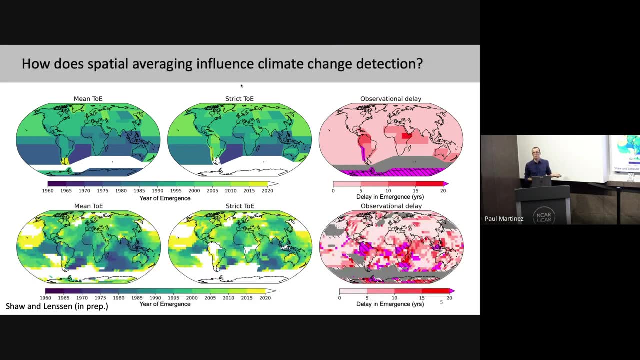 really big and they're maybe not that relevant to us, and so we can repeat this analysis on the native resolution of our uncertainty product, which is five by five degrees, and we can look at the results there. and so this is the same data just repeated at a smaller scale, um, and so we can see there's a lot more kind of features going on, and 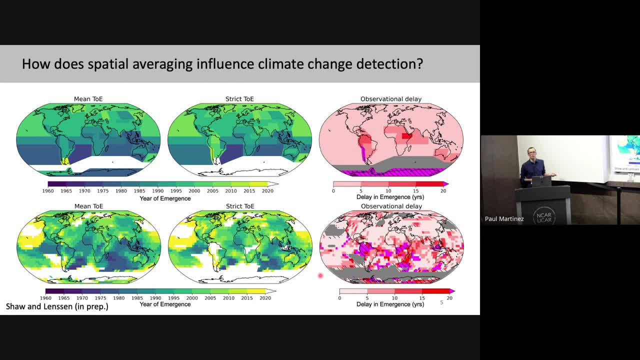 there's also a lot more, um, kind of white, which means that we haven't detected a change here. so that kind of first conclusion there is that the smaller scale we go to, um, it becomes harder to detect changes, and this makes sense, of course, because there's going to be some kind of 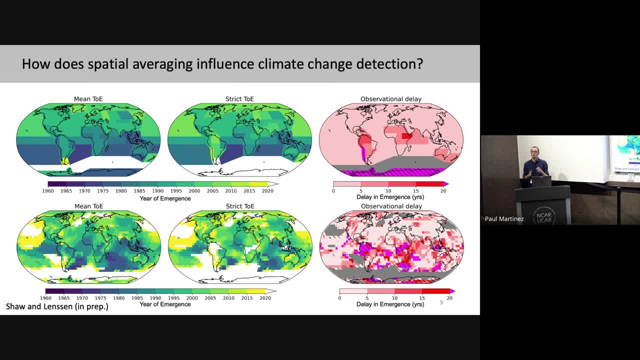 temporal, spatial time scale of our variability, and the larger our region is, the more noise we're averaging out um. we can also see that the delays are greater in this finer resolution. so we're seeing kind of more red in pinks, um, but they're also still concentrated um towards kind of the. 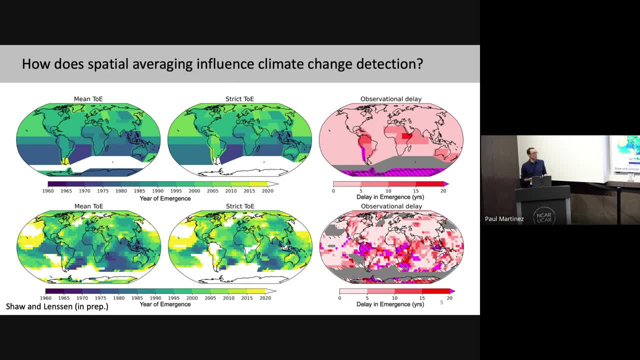 tropics, and so our effect of accounting for this um or changing our spatial scale is both to kind of delay things by um, reducing our ability to average out noise, and also we get an enhanced delay from the observational uncertainty itself, which has its own kind of um scales that we're averaging over um and what we're going to do now. 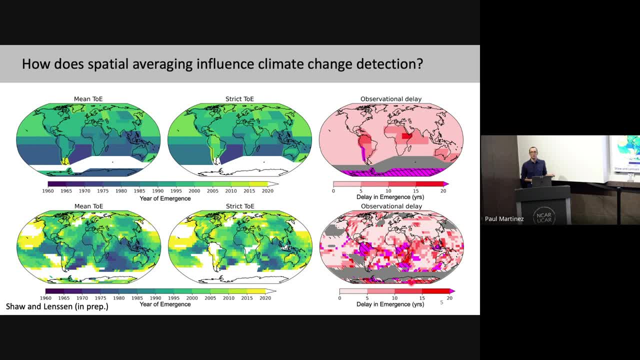 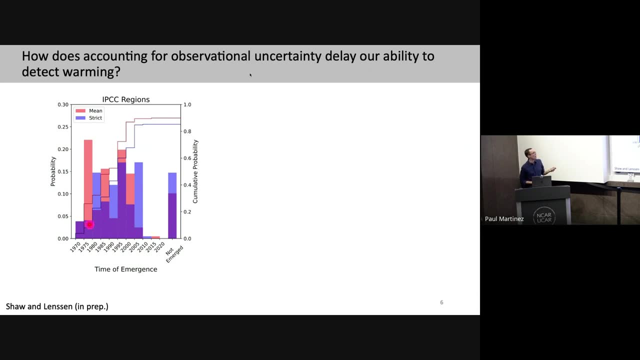 is basically take this data and aggregate it. um, using histograms to think about rough fraction of the earth's surface is kind of being delayed. where does our, when is our detection occurring? so we're looking at: here is this histogram. these are those ibcc regions and these boxes are all. 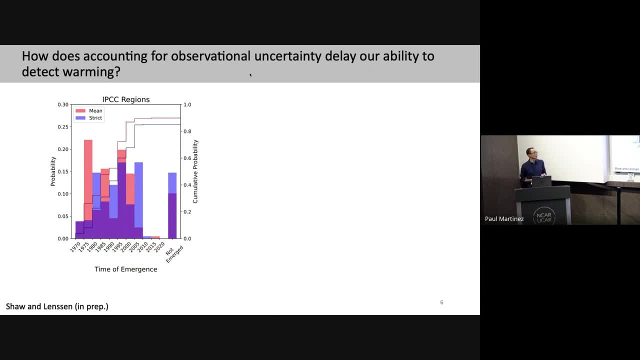 five-year periods where a portion of the earth could emerge, and on the y-axis this probability is effectively kind of the fraction of the earth's surface. so we're taking those ipcc regions and putting them in histogram, but grading by the size of those regions as well, and so effectively. 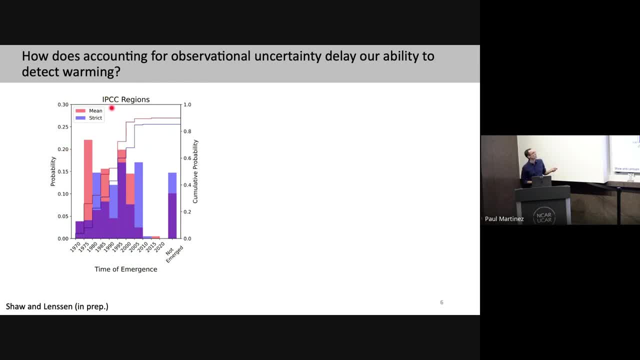 we see here is that our mean sense, that kind of ignoring observational uncertainty sense, and our our offset. so our blue histogram is offset to the right, indicating our delay in our time of emergence. we can also see that these cumulative histograms, um, in the lines um is that we're? 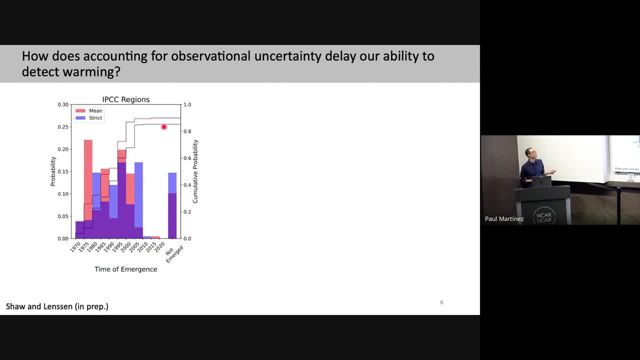 reduced, kind of at the end of our observational period in 2020. we detect about 90 percent of the earth's surface emerging when we ignore observational uncertainty, and it's reduced by five percent when we account for the observational uncertainty. so just an indicator that, um, this really does affect our observational uncertainty. Heartland-Arlington, North Carolinaores. 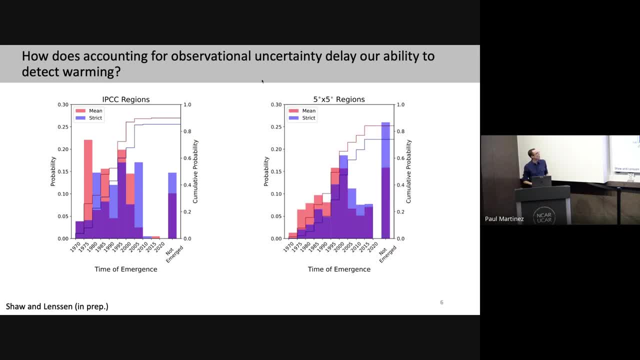 Waukesha, Ohio, Chicago, Ohio, Alabama, USA, Alaska, Minnesota, Oklahoma, Arizona, Alaska, Oklahoma. ability to attribute these surface temperature changes When we look at our 5 by 5 degree regions. first of all, we see the histogram looks a little nicer. 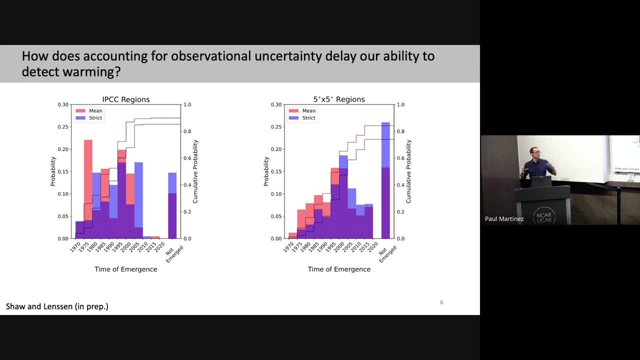 just because those regions are nice little boxes and not these big kind of clunky regions. But we also see that the histograms are offset to the right because our spatial scale makes it harder to detect the changes, And also that in the cumulative histograms there's a larger difference between 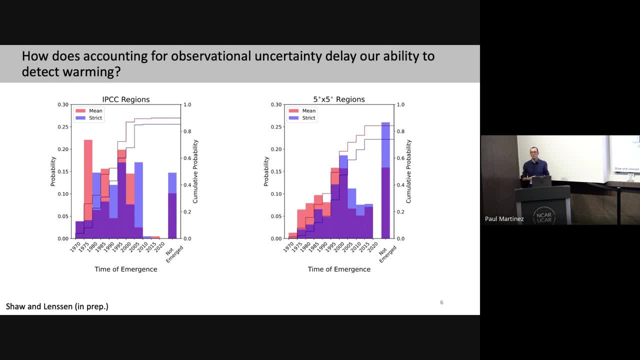 carpe and in our strict, And so going to a smaller scale and then accounting for observational uncertainty makes it harder for us to detect these changes. But we want to make sure that these results are robust to our choice of data, And so here we used to get an uncertainty ensemble and the CSN1. 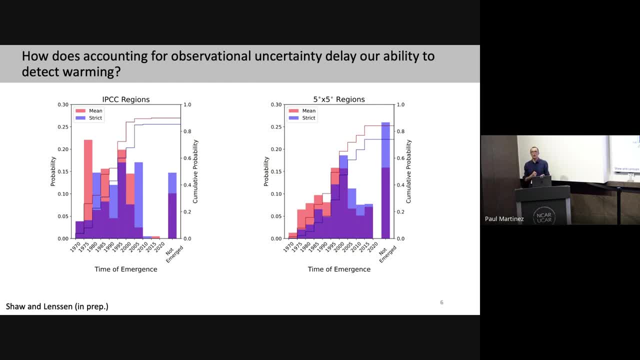 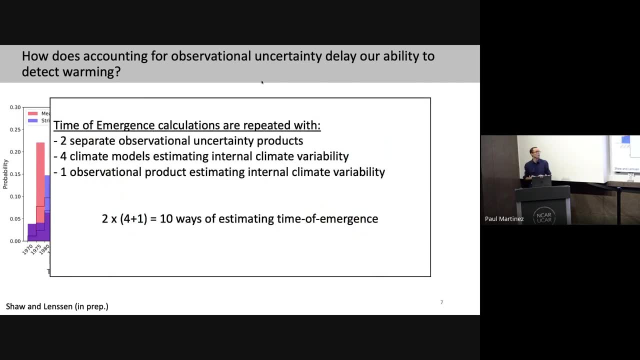 pre-inductive control simulation. But of course there's all kinds of datasets for this information out there, and so we want to repeat our analysis and see how robust it is to the data set, And so there is actually only one other uncertainty product that we're familiar with, which is the Had-Q-T. 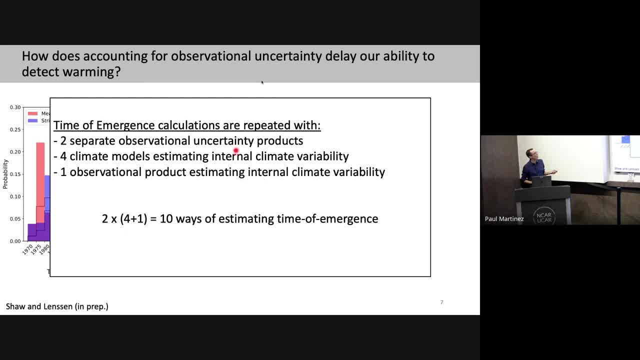 uncertainty. But we also use four different estimates of internal variability from different climate models and one estimate of internal variability from observations, which is the McKinnon Observational Ensemble, where we've removed the force trend and just resampled the internal variability. So, given that we can kind of mix and match our observations and internal variability, 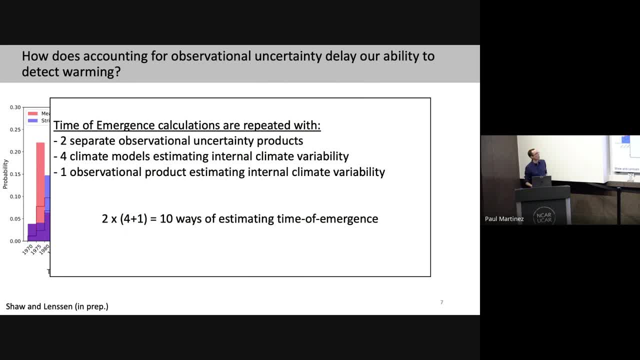 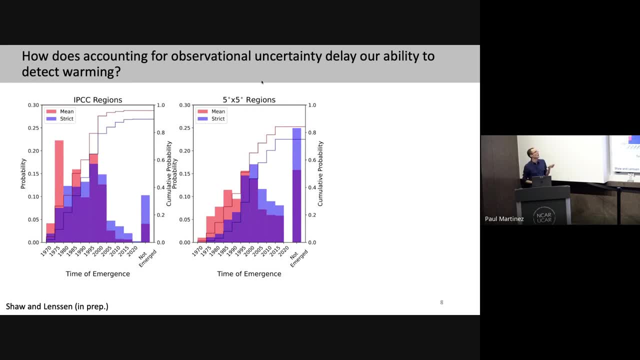 now 10 ways. we're kind of enhancing our data and looking at the robustness of our results. So the conclusion here is that these look very similar, So the results are robust to our choice of internal variability and observational product. Finally, what we'll do is we'll take our histograms and we'll extend them to the delays itself. 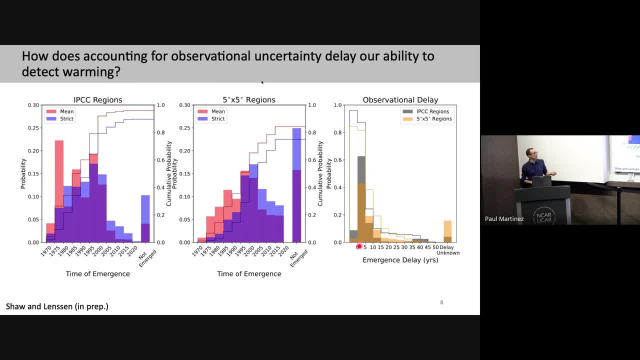 And so now we're looking at where do we experience delays of zero years, of one to five years, of 10 to 15 years, And instead of looking at a cumulative histogram, we're looking at one minus our cumulative histogram. So we can understand. 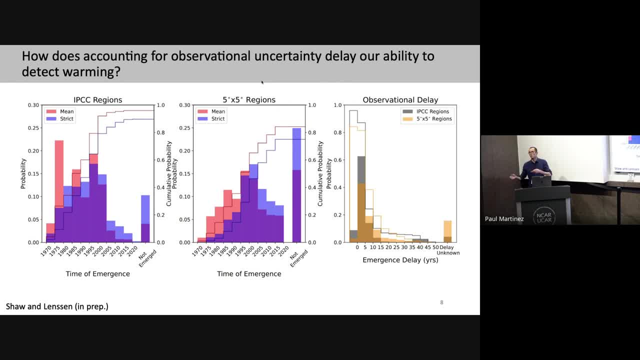 What fraction of the Earth's surface is delayed by more than X many years? So effectively? what this histogram is telling us is that the most common delay is between zero and five years, but there's a pretty long tail here, So there's lots of regions that are delayed in excess of five years. 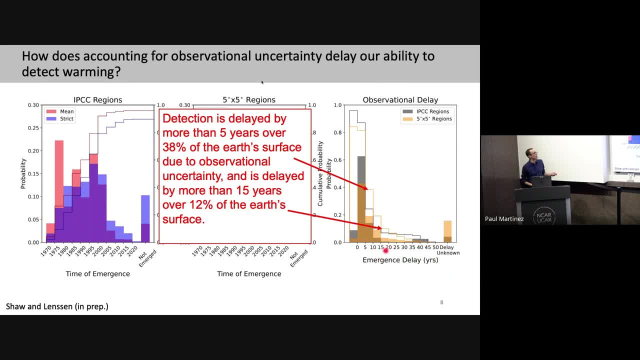 And by looking at these kind of one, minus our cumulative histogram, we can see that in excess of five years, almost 40% of the Earth's surface in this kind of five by five degree resolution is delayed. And we can see that, And over 15 years, more than 10% of the Earth's surface is delayed. 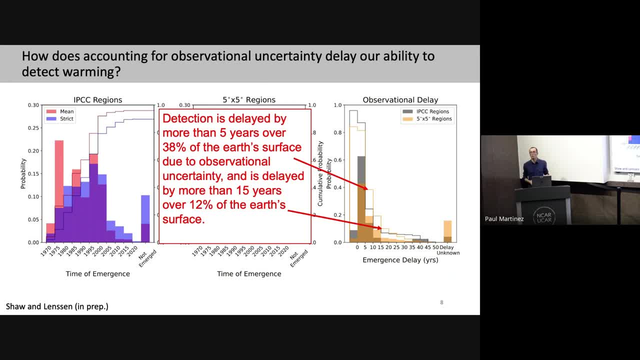 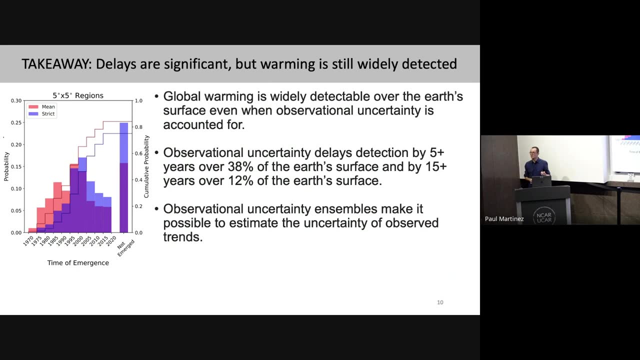 And so accounting for the observational uncertainty is affecting if not a small fraction of the Earth's surface, It's basically everywhere in. the significant portion of the Earth is pretty large. to just kind of wrap things up, We are still detecting surface warming. I don't want to provide fodder for climate change deniers, but observational uncertainty. 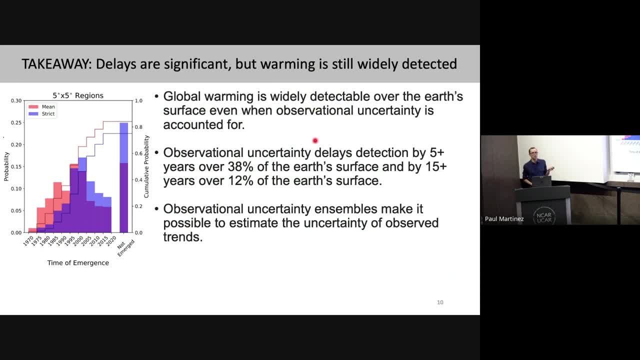 is really important because it delays our ability to detect these changes, And those delays have a spatial structure That I could talk about more later. There's a reason that the delays are more in the tropics and less in the extra tropics and polar regions. 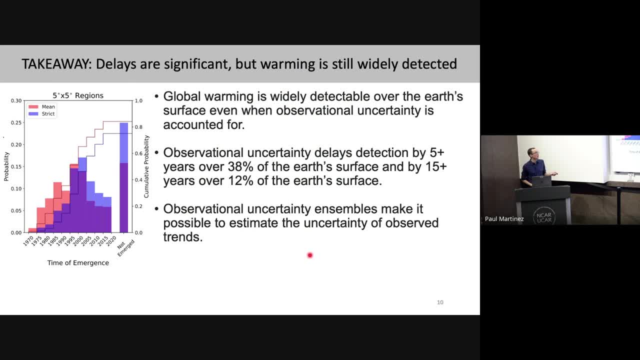 And specifically I kind of gave these numbers for delays, and that this work is really made possible by these uncertainty ensembles And so having uncertainty ensembles, maybe for extremes or for precipitation, enables this kind of work. Thanks so much for your time, Thank you. 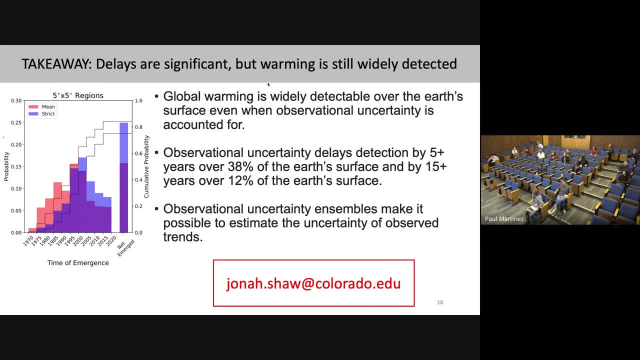 Really nice talk, Thank you. I'm curious to know- I'm sort of extrapolating your results out with going from the large regions to the five by five- If you were to continue increasing that resolution down to like some of these new client models. 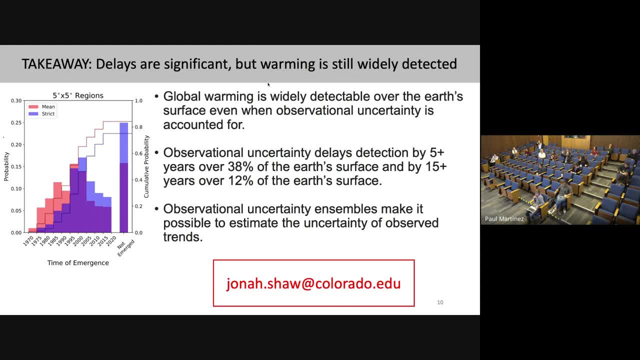 are running at like one kilometer right. Would you expect your distribution to continue to shift to the right or would it asymptote out at some point? That's a really good question. Yeah, We haven't been able to do that. I don't think it would indefinitely increase, but I would say that on a resolution we don't. 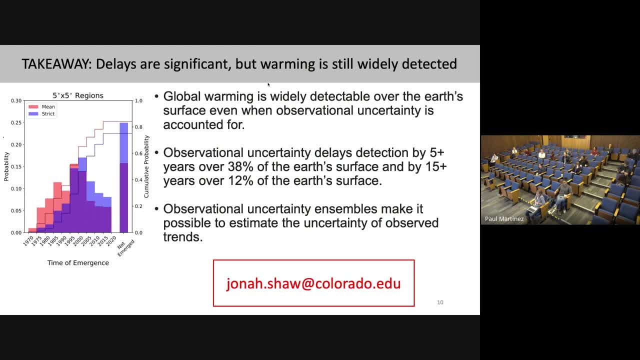 have observational records at that kind of resolution. So there's a reason that these uncertainty products are at five by five degrees and it's because in some regions there's like the uncertainty product. it just gives you like a man or something because it doesn't know the surface temperature. 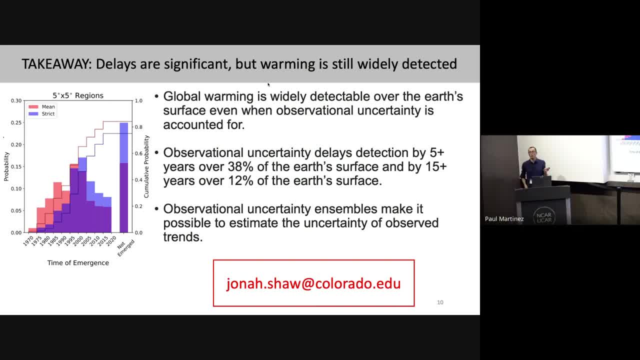 So I'd say it could depend a lot. It depends a lot on where observations are for that kind of specific granule that you're interested in. Thank you. You mentioned you have two products with the spread, but I'm wondering: how does that spread? 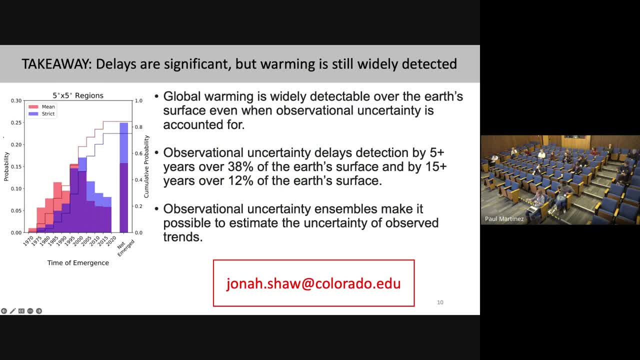 compare to the difference between just individual products, Is it similar? Yes, So you're saying like within the Hadcrutee Ensemble there's a spread, within the GISS Ensemble There's a spread. But how does that compare to the? 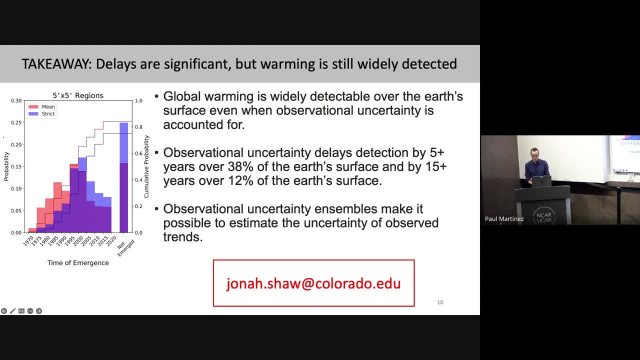 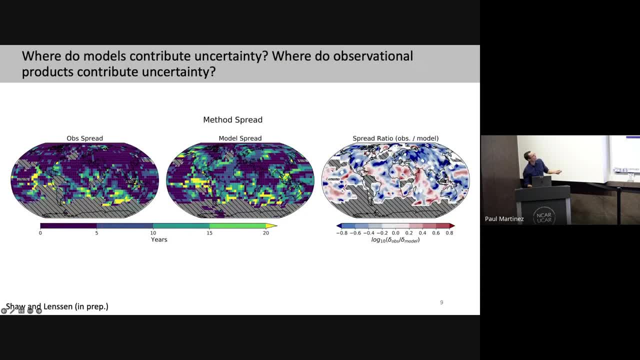 Yeah, And then other products that might not have a spread, like BEST or Yeah. We haven't looked at that question specifically. What we have looked at is the spread between observational ensembles and the spread, or between the observational products and the spread and the models that are used for the 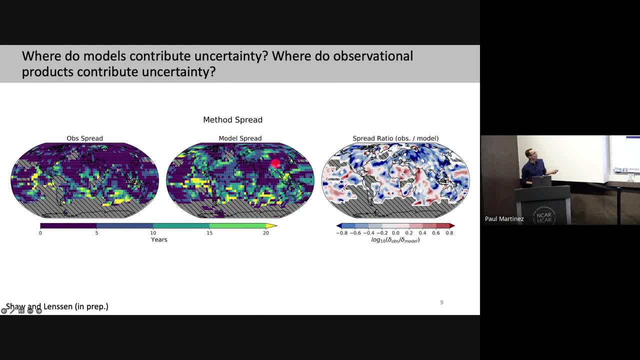 internal variability. So this doesn't explicitly answer your question, but maybe it gets at it a little bit, which is that the uncertainty from the ensemble methods Is like also concentrated, or like it has a clear spatial structure, whereas the models tend to be a little more like they're actually at spread in the polar regions for the observations. 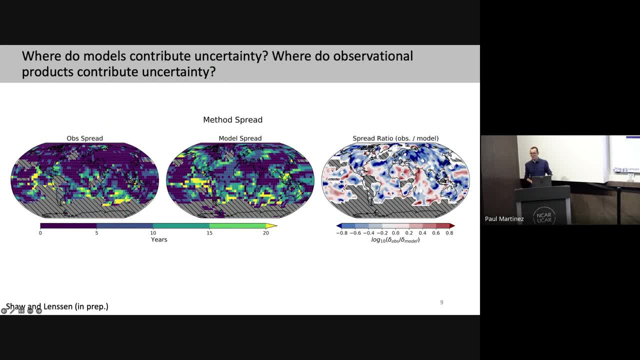 though, But that's not really I don't know. I'm not really answering your question. So the one in the middle is like internal variability included in the spread, and the spread is kind of your structural uncertainty. So this is like uncertainty resulting from which choice of model you use. 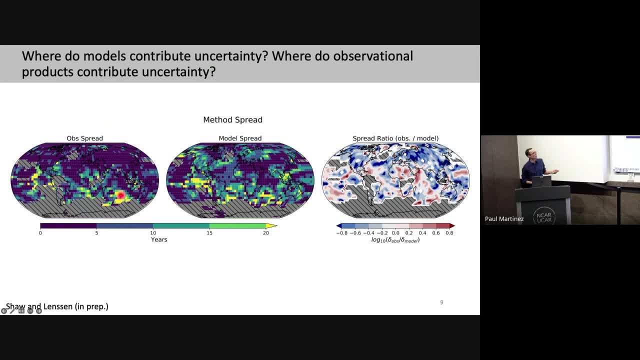 To estimate your internal variability, and this is spread from which observational product you choose. Okay, So yeah, it's not really answering Right. Yeah, It seems like that would be. If the spread among observational products is big, that could also be a big contributor. 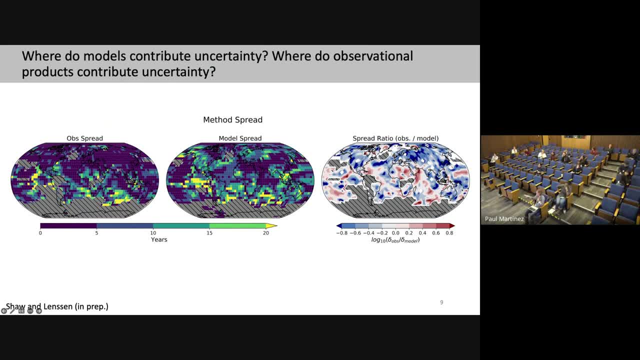 to the time, Like different separate products, not the spread within one product. That could be a big contributor too. And just looking, I don't have like individual maps for the products, but we've made them and looked at them And they are pretty. 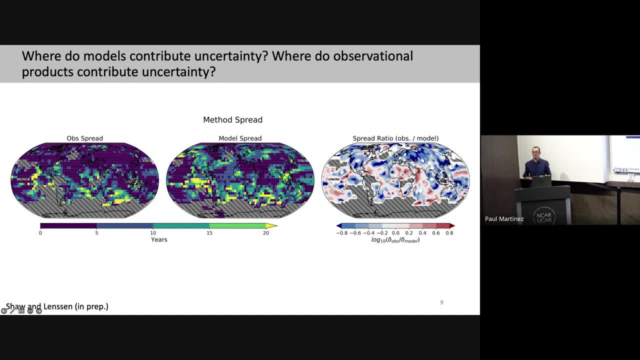 They just have like kind of some interesting features that we haven't fully explained yet, Because these products, the way that they go about creating 200 different realizations, is really different. Some of them assume kind of a constant way like scale over the entire surface of the. 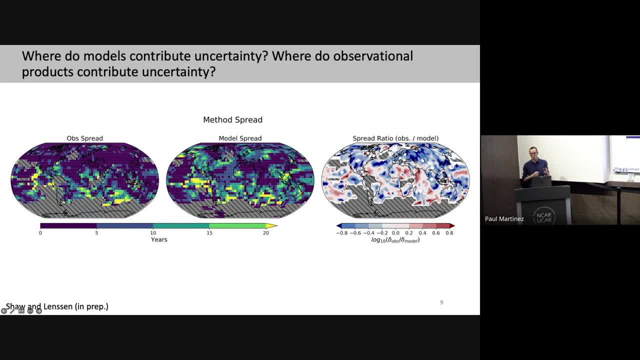 planet. Some have more complex handlings of it, And so this means that the way that things average down look really different as well. Thank you, Now we need to move on to our last talk. Okay, Thank you. We will begin by Bill Chestman. 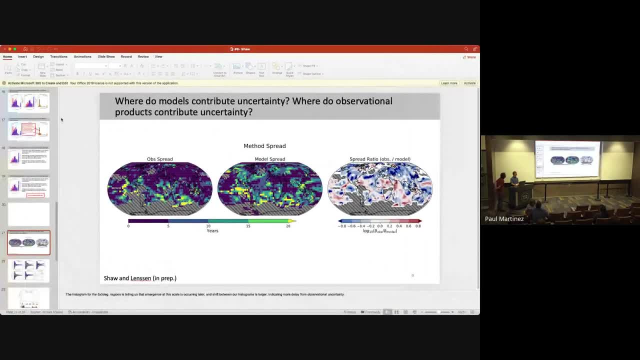 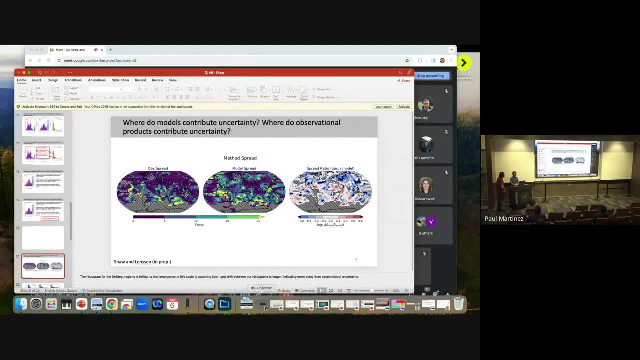 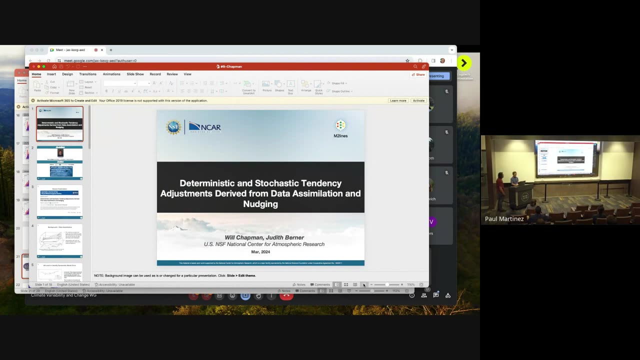 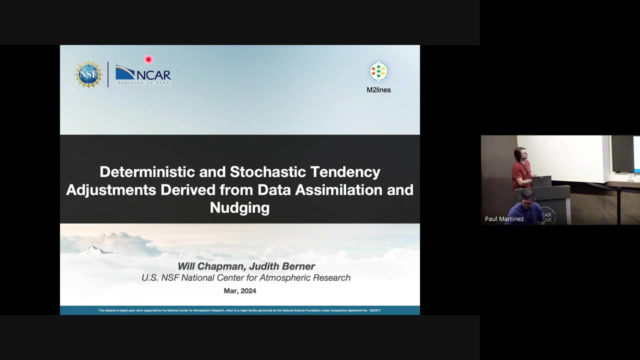 Yeah, Okay, Thank you, Okay. Well, this is going to be tough, OK, Great. So thanks y'all. One more talk between you and lunch. I'll try to get through it quick. So today we're going to be talking about a little bit. 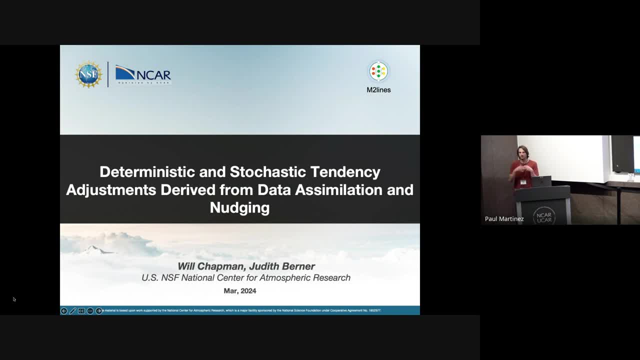 of a shift and talk about some model representation and trying to improve some of the representation of some fields with other models. I figured we were going to be looking at two. we call them data simulation techniques. One of them is actually a very strict data simulation. 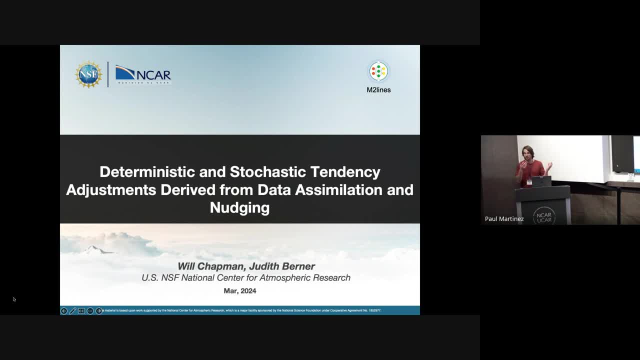 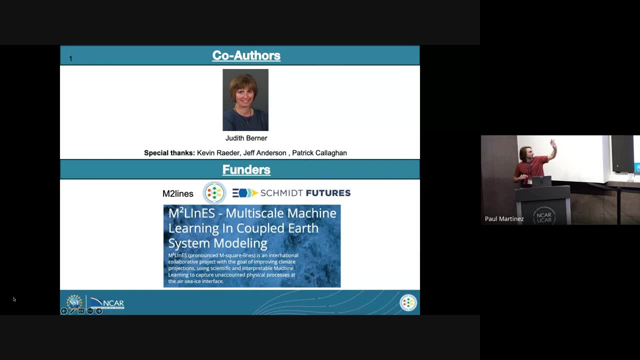 technique and one is just a linear relaxation back to observations known as nudging, And we'll kind of go through these. so we're all on the same page. The first thing I want to do is just acknowledge my co-author on this manuscript, Judith Berner. 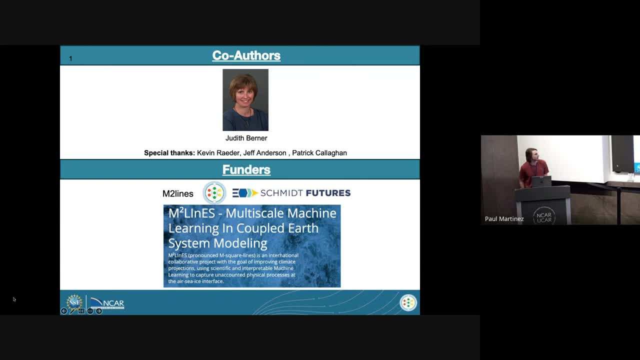 A special thanks to some of the folks here, particularly in the DA sections and also in CGD, that helped me out a lot figuring out what these increments mean or these data simulation systems mean. And this whole project is funded under the M squared line project, which stands for Multiscale Machine Learning. 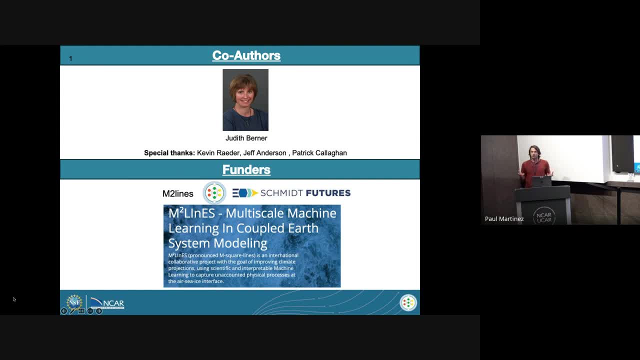 in Coupled Earth System Models in which we're trying to use machine learning to improve the representation of different fields within our coupled model appointments For today we're only going to be focused on the atmospheric component of the model, so it's not coupled yet, but we're moving in that direction. 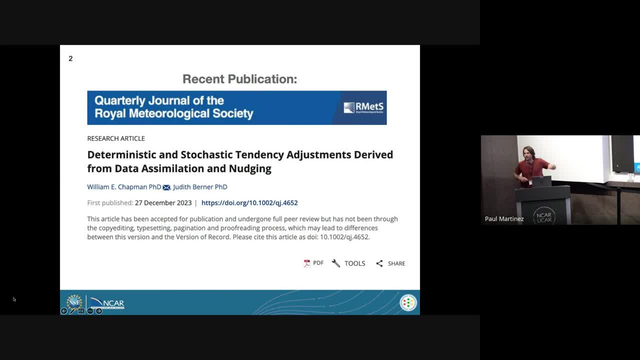 And if you want to know more about what you're going to see today. the first part of this talk, before we move into what we're doing now, is all summarized in this paper that just came out in QJLMS, So I encourage you to look at it if you are confused. 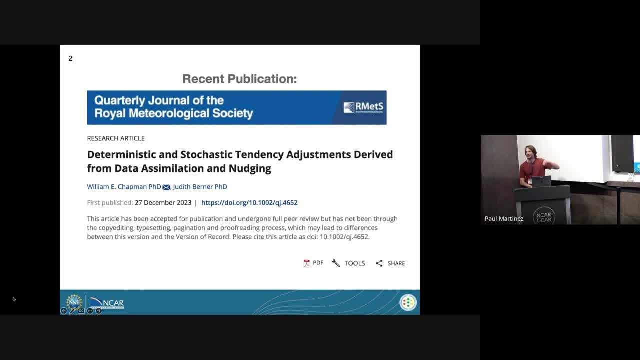 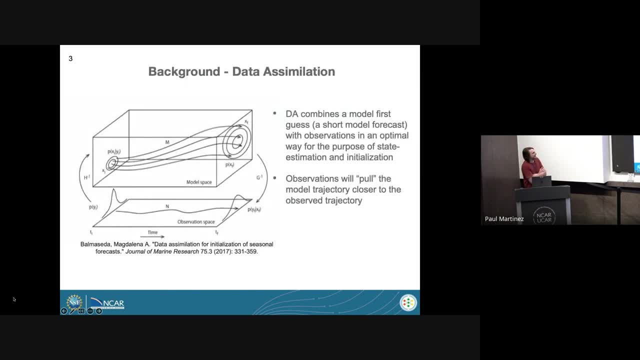 And it may confuse you more. so I encourage you to email me if you're further confused. So just a little bit of background. What is data simulation? So, really, data simulation is the process in which we confront our weather prediction models with observations. 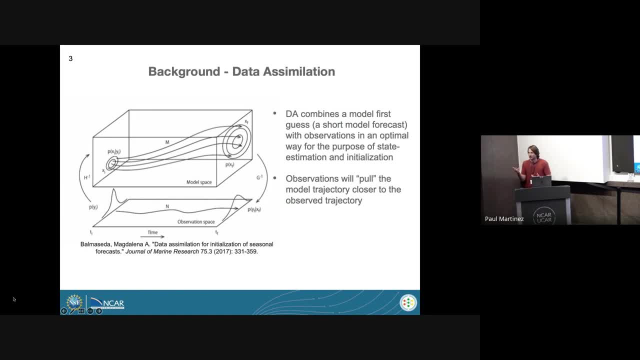 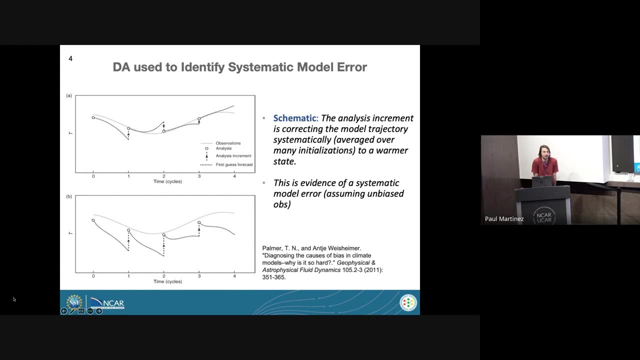 And we make some sort of optimal mapping between the observation space and the model space, Such that we can pull the model towards the observations in some optimal way. And what's been shown is that you can use these data simulation systems in order to assess the health of a model. 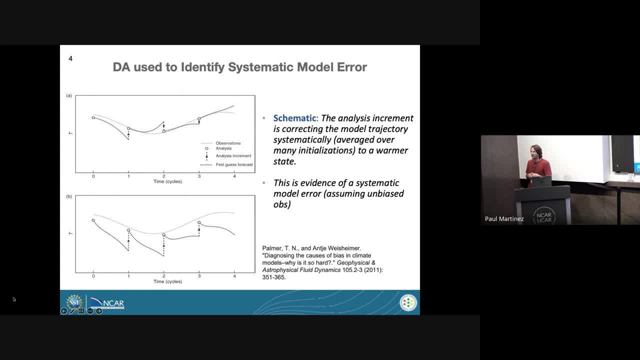 So, on the figure on the top there, this is a healthy model, or an example of a healthy model, in which you have the gray line, which is our observations, And the data simulation system is taking the forecasts which are shown in the little dash lines. 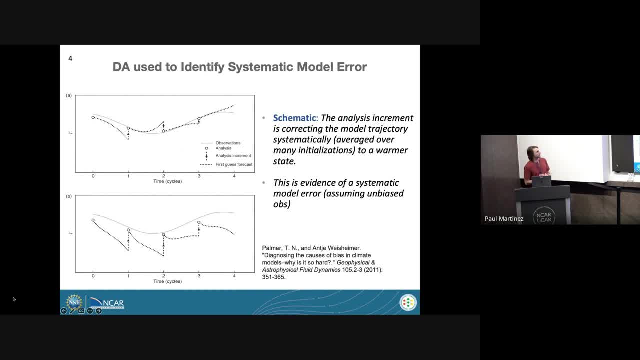 and pushing it randomly In different directions. right, So it's always going either up or down or towards a different observation space. On the bottom we show an unhealthy model And the way you can tell is the data simulation is always trying to pull it in one direction. 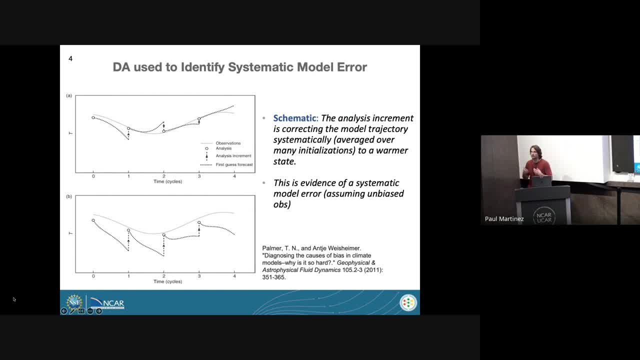 So you can imagine this were sea surface temperatures in the tropics that were too cold And the DA is like: come on, let's warm these things up always. So this is evident of some systematic model error And the big idea behind this. 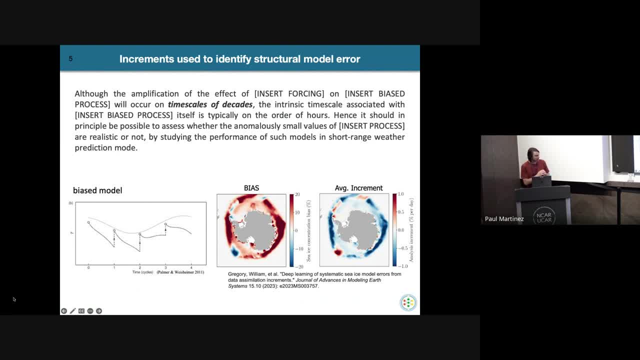 And how this leads to downstream bias is kind of summarized here. It says: although the amplification of some forcing on some bias process will occur on the timescale of decades, meaning you need to look at a 30-year run in order to assess model bias or longer the intrinsic time. 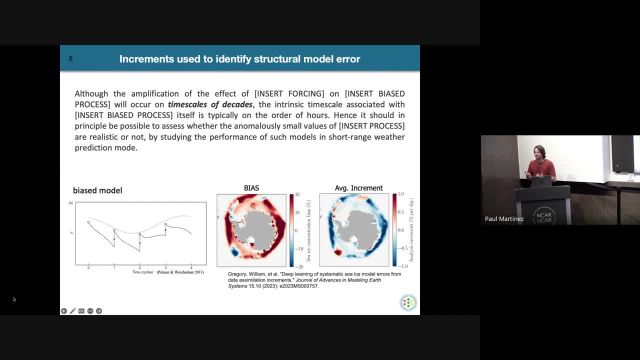 scale of those bias processes are likely happening in the fast physics, or at least some portion of it. So it's time, step to time step, And it's an accumulation of these errors that lead to some bias state that then leads to a bias model. 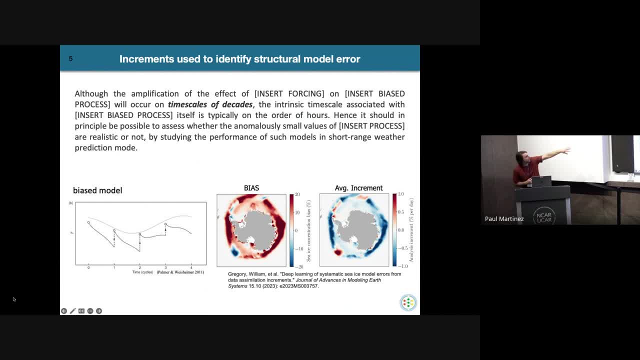 And I really like to show this figure. This is by Gregory, in which he is looking at the average increment in our in a sea ice model. So this is SISII and looking at the bias on the left And that's the sea ice concentration bias. 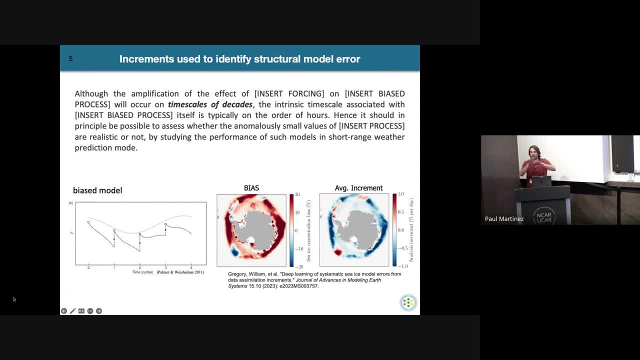 And it's the increment of the data simulation. on the right You can see it's sort of a perfect one to one matching there. So if he was able to improve the increment representation you would of the bias would be fixed there and he's shown in a nice paper that you can actually. 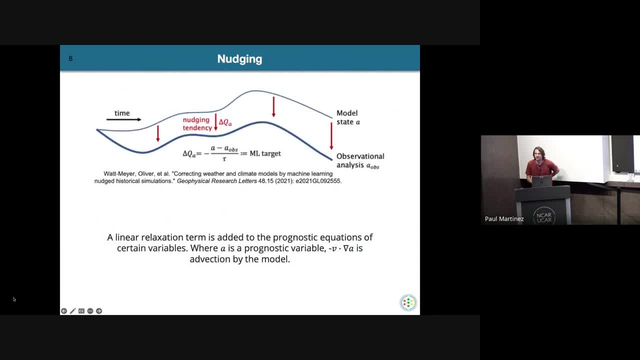 do this in the cda system. so the second system we're going to be using is just it's called nudging um. so this is just a linear relaxation back to some observed state. in this case we're using um, the era interim product, and we are taking our model run and we're just constantly. 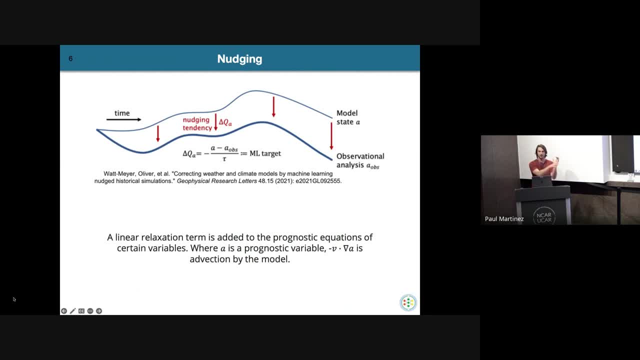 applying this relaxation term to try to have it hold the observational, observational trajectory there. um, so you just add this to the prognostic equations in the model and it then follows the observed trajectory there and you collect those tendencies and you can say these are the increments that we're using on that side. so essentially in this paper we have two learning. 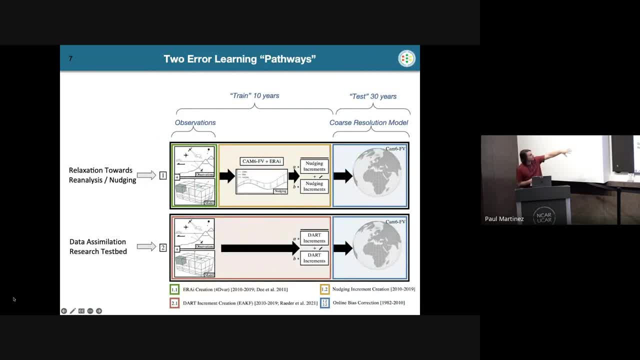 pathways that we're doing. so we're taking some observational state, we're applying some sort of da product, either nudging or data simulation, and what we're doing is we're saying: give us now the mean uh or the climatology of those nudging increments. um and uh, we are collecting a stochastic component. 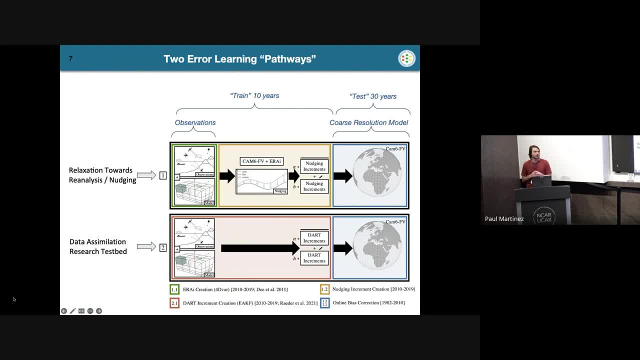 also, which is just represented by individual uh increments on each day, and we want to say, by taking the climatology of these increments and pushing them back into a model run, can we improve the model state? so, essentially, we take 10 years of the simulated data. we then move to a different 30. 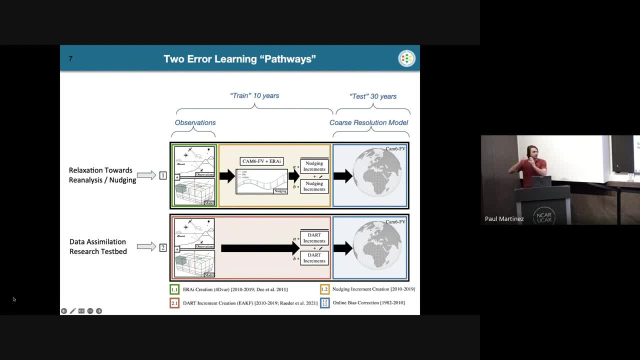 years and we say, by applying those increments in in those 30 years, can we improve the bias in those systems? right? so the first thing we wanted to do is say so. does a nudging system and a data simulation system? do they look like each other do? 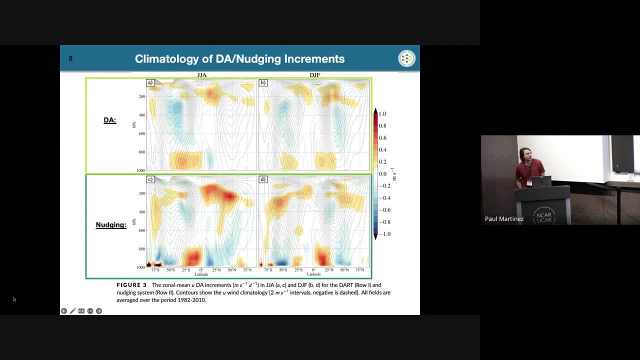 the increments. do the increments sort of result in the same representation across the field? and i would say largely no. in some regions yes, though, so particularly in the tropics, particularly the lower latitudes. here you can see across the da and the uh nudging systems, but they do. 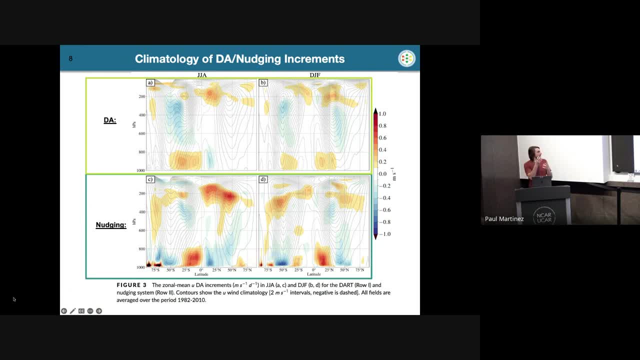 look very similar uh, also in the representation of some of the jet regions of near 200 millibars. there's also areas that project on each other well, but there are also significant differences between the space. uh, however we are, we went and we applied both of these systems. and what? 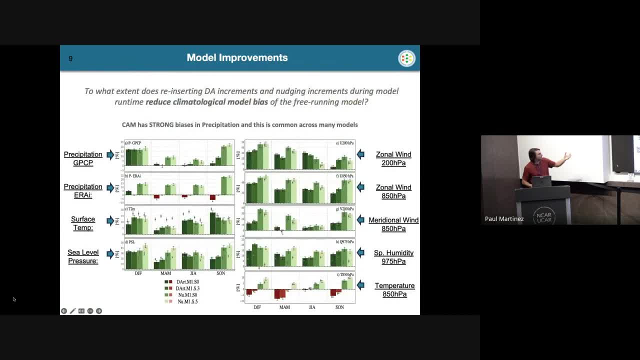 resulted, uh, in our third year. climate runs is shown here and these are represented by the improvements or deficiencies that reinserting these increments led to in 30-year climate runs in cam. and this is a lot to look in, but look at, but essentially what you want. 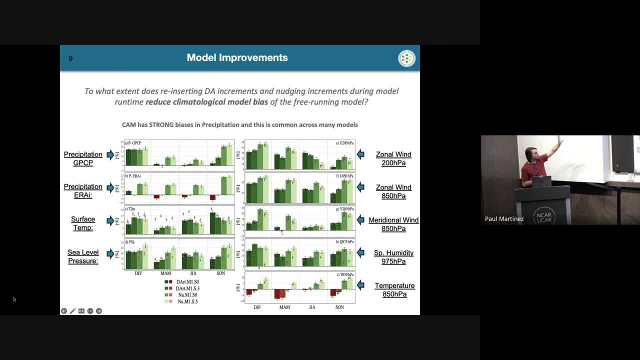 to see is green. if it's green, we are improving the model in some way. if it's red, we are leading to some deficiency here and essentially, what we are able to show is that across all of the systems- at least all of the nudging systems- we are able to. 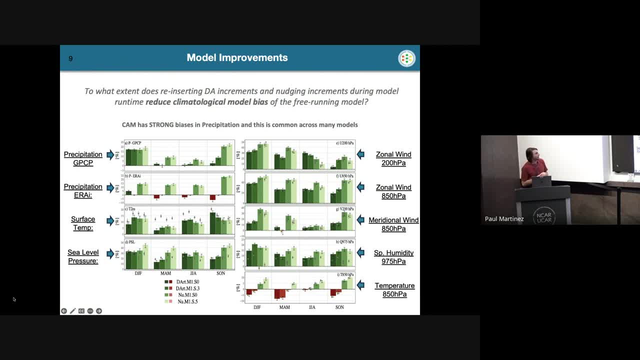 improve the model in many areas the da system did also. where we saw some deficiencies was in the upper level temperature fields, particularly when we're reintroducing the dark increments or the da increments rather than the matching increments. but largely we're leading to drastically improved models or address improved model representation, at least. 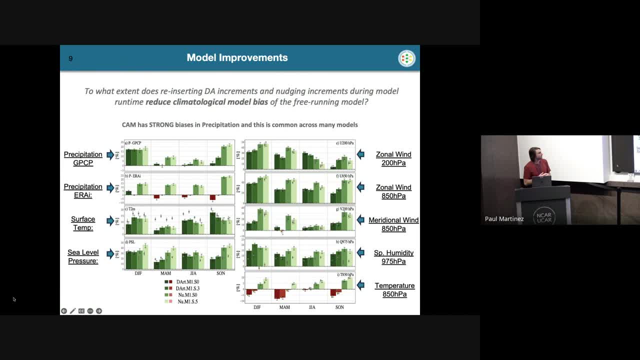 across all seasons and obviously annually too. when you reintroduce these, these tendencies, we're really happy about this. um, however, we noticed that we were just doing this deterministically and we didn't have any sort of stochastic physics in there. we were significantly altering the large scale modes of variability within the atmosphere, so we were damaging particularly the pna, the nao. 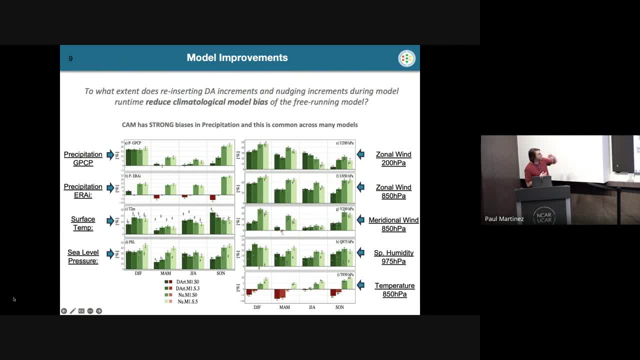 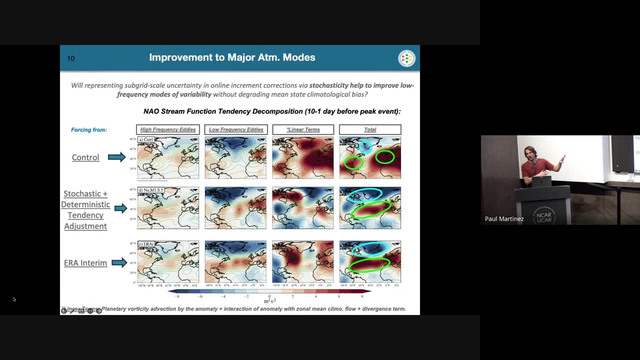 some of these really important metrics here. however, when we introduced stochasticity, we were able to really balance everything out and showed actually great improvement in the variability over just single or control models. so i want to show you a representation of that here on the nao um. so 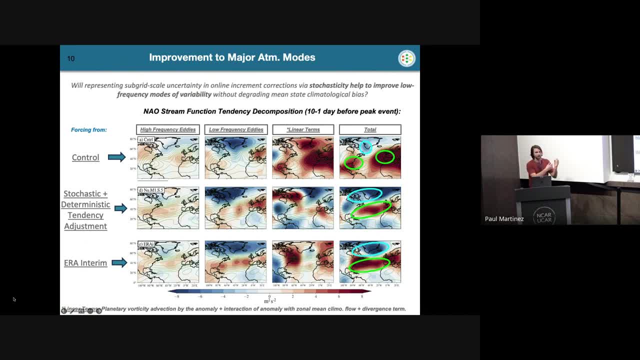 oscillation, a very important pattern for downstream weather, particularly in europe, um, and what we've done is a what's called a stream function, tendency decomposition, since we're trying to look at all the components that lead to the growth or decay of the nao. um, and i want you to focus on the bottom. we have the observations, so this is what we want: the model. 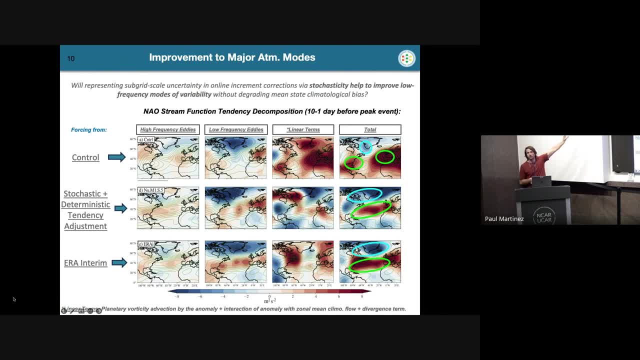 to sort of look like, and the top is a control run, so it doesn't have the adjustments that we made to the model. in the middle is a stochastic and deterministic run. so we applied the stochastic component of the of the increments, we applied the stochastic component or the deterministic component. 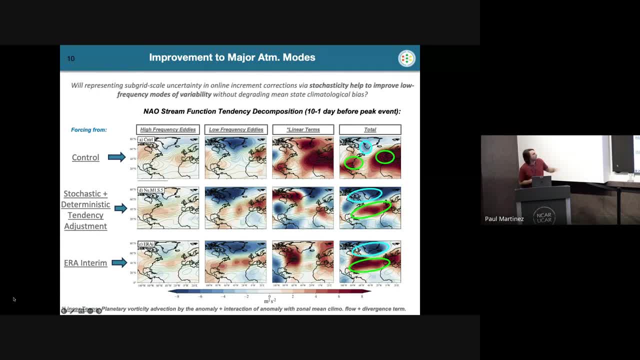 and i've highlighted just some contours there. on the right, essentially what you can see in the controls, you have this real tri-pole pattern that you shouldn't be seeing for the nao and what we showed was that was really a result of this amplification of some of these. 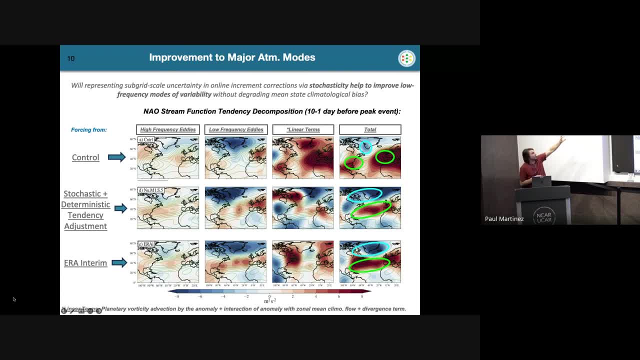 linear terms within the stream function decomposition where it should be. the nao really should be built from these high frequency and low frequency eddy interactions and what we showed is by reinserting these increments and improving the background state um is, we could really amplify the effect of the high frequency eddies and the low frequency eddies and diminish 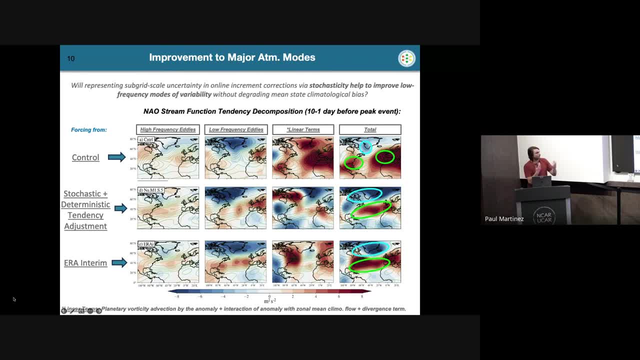 some of these linear terms which led to much better growth and eventual representation of the north Atlantic oscillation. so we know we were inserting these tendencies, improving the model and improving the nao, doing it for a physically consistent way, which we were really excited about. so the big takeaways: 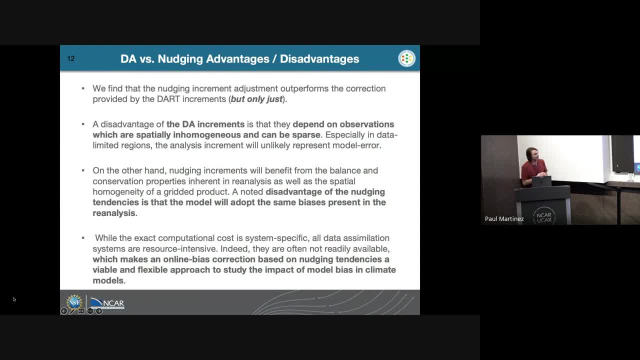 from this is there are advantages and disadvantages from using the da and nudging systems. da is physically more, it's more intuitive. we should, we should be able to be mapping directly from observations to the model, to a system, but there the observations are sparse, so you what ends up happening? is you see, real? 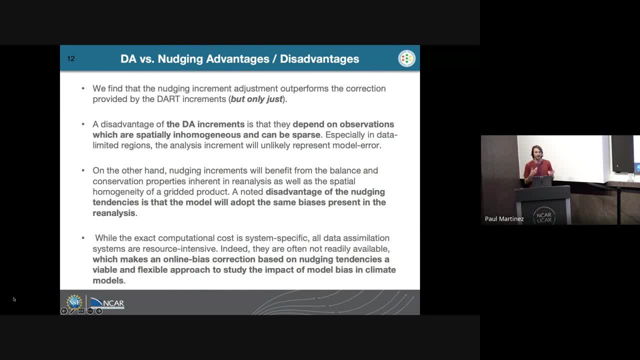 representations of our observational systems within the increments. that led to some problems. however, using the nudging, it's sort of filtered through another product and then you're able to immediately have increments that are represented across the globe. however, one of the disadvantages of the nudging system is that the tendencies will adopt any biases that are in the reanalysis. 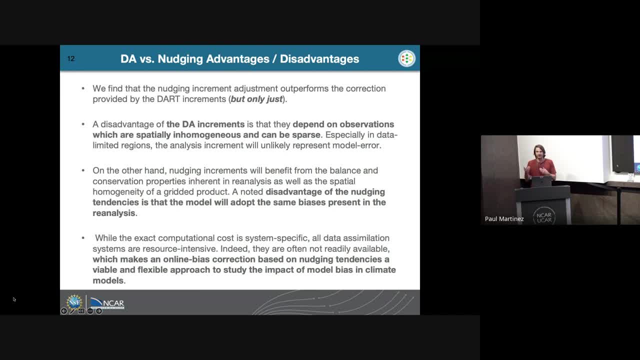 product and unless we approve the reanalysis product we're never going to improve those biases. introducing the banker model: i think the big advantage there between nudging and da is nudging is order 100 less expensive. so anytime we improve the model, we change the model, we can run the nudging system and we know that these increments that we reinsert. 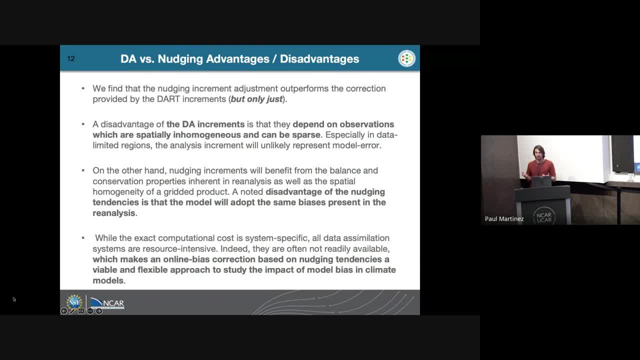 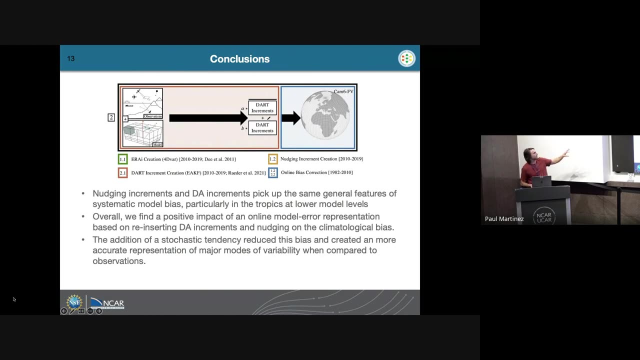 will be potentially just as beneficial as running the full da in order to develop this sort of bias correction. at least, that is what this study indicates. in our current configuration, this may not be true across every system. um so, some conclusions here. is that the nudging at least? 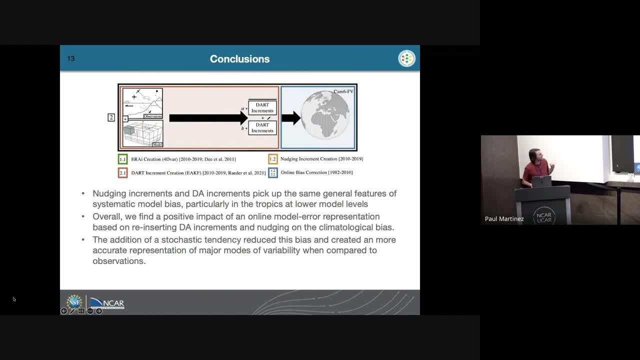 the conclusions for the first part, and then i'll just talk quickly about what we're doing. next is the nudging increments, and the da increments pick up on some of the same general feature features, particularly in the lower level prospects. overall, we find a positive impact of this online error representation using both the da and the nudging and the addition. 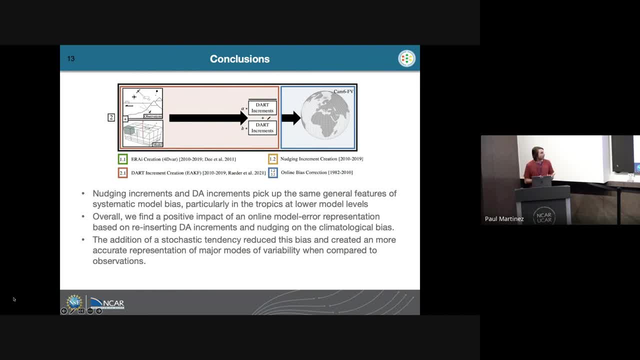 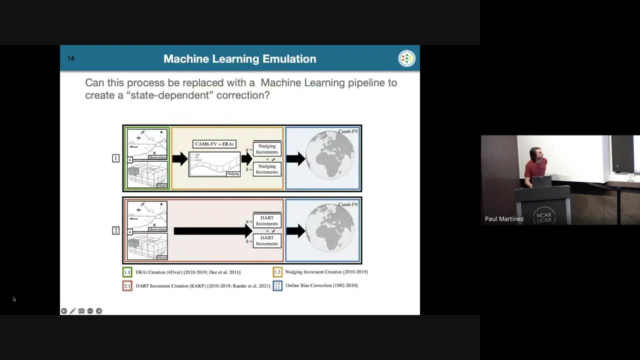 of stochastic tendencies, reduce the bias while creating more accurate representations of media modes of variability across the model. um, so where we're moving now is we want to, rather than have a sort of dumb representation of these tendencies and the adjustments they make, we want a a state dependent version of this. we want to say here's the what the model currently looks. 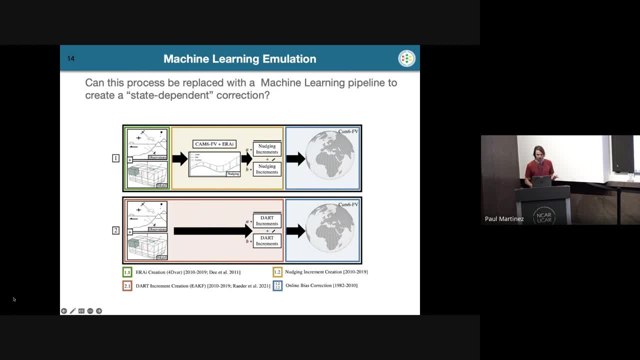 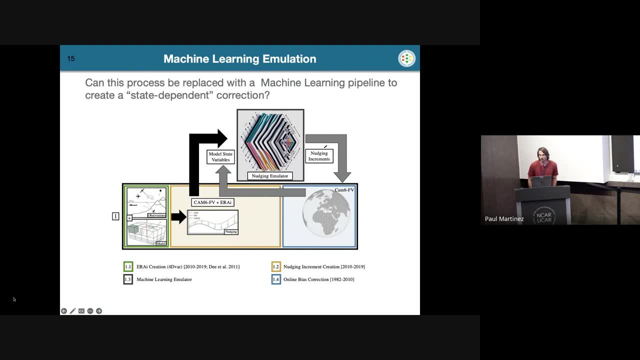 like right now? is there a smarter way that we can insert being credits, um, and an easy way to do that? part of it's easy. one way to do that is to use a machine learning model that then learns the tendencies and it picks the input state and adjusts the model uh, actively, um, so we have this. 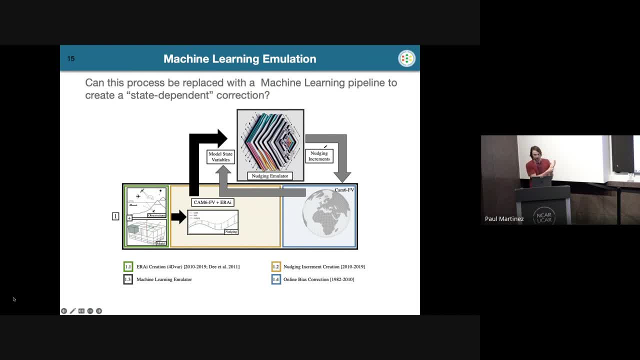 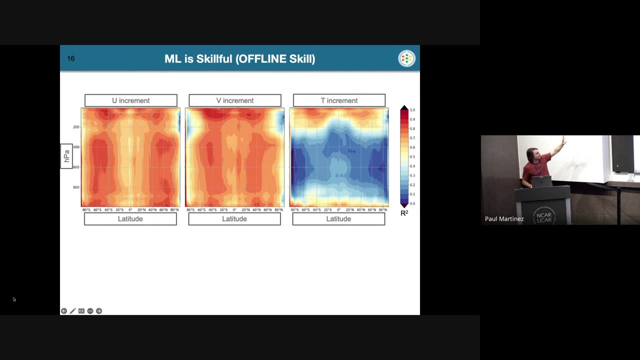 system running now within cam uh and uh. the results are too early to show within this talk. i think we're still assessing how good it's doing um, but i can show you that we are representing the increments fairly well. um, at least the zonal and meridional uh wind increments. this is an r squared. 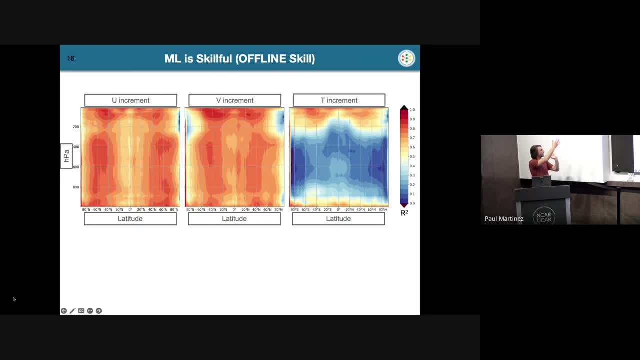 frequency, uh, this kind of uh um, historical mode, uh, and i'm showing the full atmosphere- uh, vertically along the y-axis and then part of this uh, uh mean state, uh across south to north, uh in on the x-axis, and this is the r? squared of those tendencies. so we're saying we are able to. 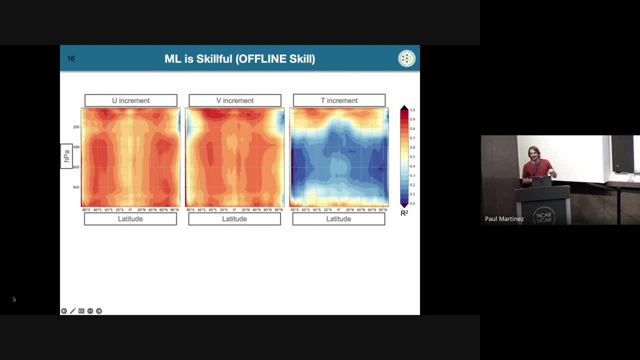 represent the u and u winds and emulate that system really well. the temperature field we're not so good at, uh, but the good news is even without adjusting the temperature increment we were able to show significant model improvements before. so if we just focus on the frequency winds, 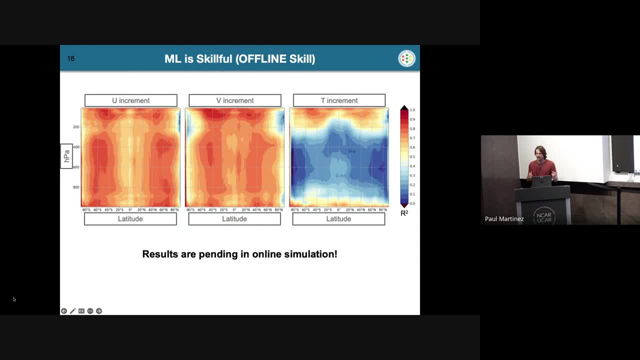 be fine within the system. so, like i said, the results are pending. we have this running online in our model now. uh, so we have what's known as a convolutional neural network interacting with the model space and those runs are analyzing those runs. now, so crossing my fingers that it's going. 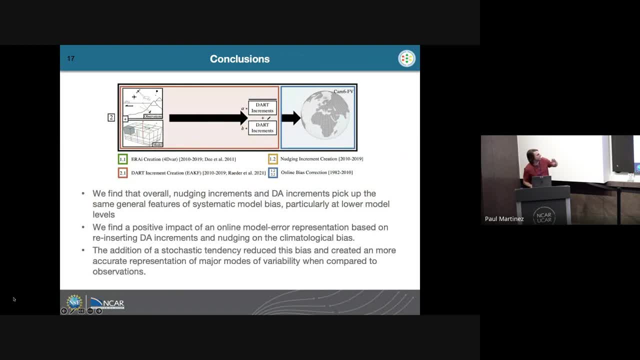 to be doing well, uh, so, in conclusion, um, this is the conclusions from before, so i won't question- mentioned that nudging was very competent, computationally inexpensive. how expensive is adding the cnn to the model? oh, um, it's a great question. currently, without gpus, uh, it represents like a four times speed. uh, slowdown of the model. um. 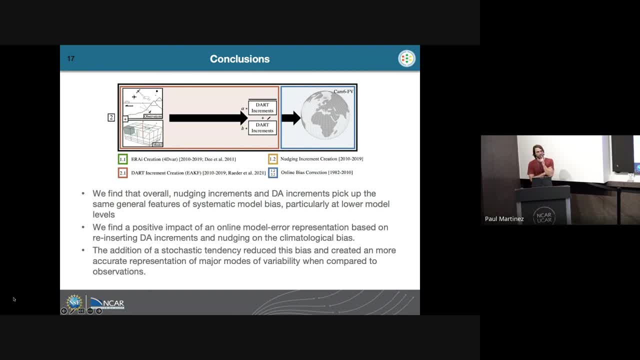 we just wrote them a gpu definition, uh, our machine definition. so we're on the gps now, and now it's like 1.5 times slower, so it is expensive. but this is someone who is not a software engineer implementing this into the model, so i imagine we can speed this process up. 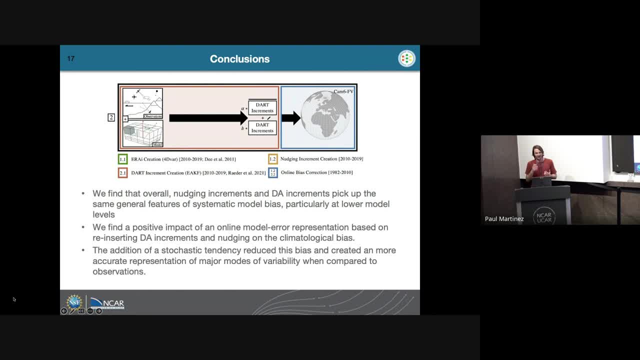 i'll just need to consult with a bunch of people in order to do that. so it undoubtedly it will be more expensive. um, but how do you split that? i think we can. we can lower those costs. you mentioned that when you just imposed the bias correction tendency without the stochastic 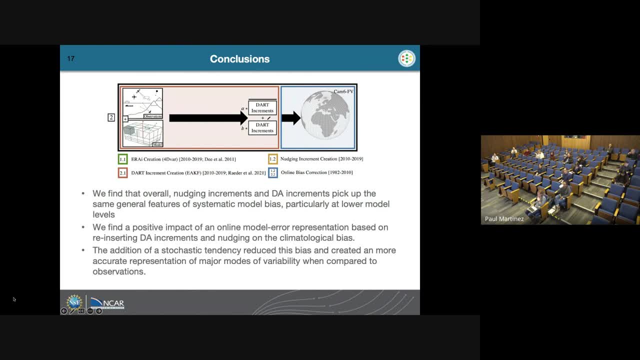 addition, the modes of variability degraded, because i haven't seen that happen when i've done that in the past. and what would you? why would that be? or are you doing? it's a smoothly varying seasonal cycle of tendencies you're just imposing it is a, it's a smoothie, so it has a, a diurnal. 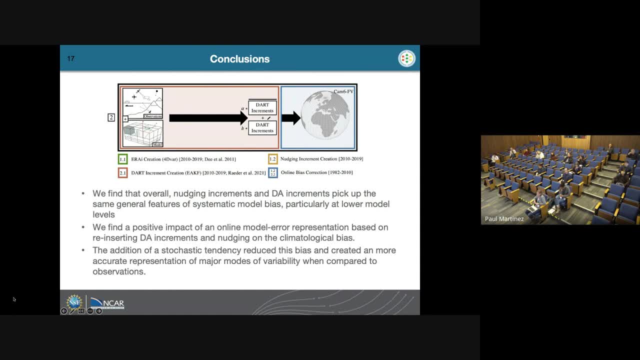 cycle and a seasonal cycle and what i saw, particularly so, the nao was bad, but it wasn't that bad, it's almost equal. it was really in the pna what we saw, um, and when i did the tendency decomposition, it was really this aerotropic anything, this barotropic feedback and it's. 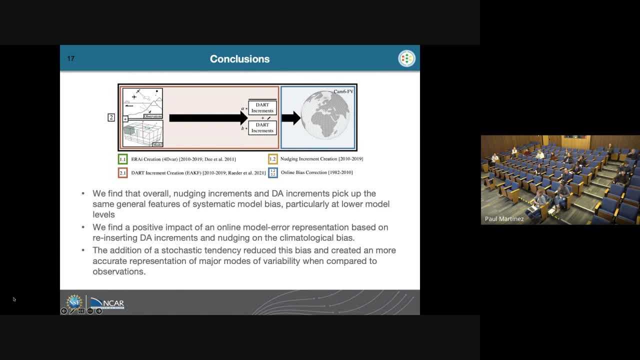 essentially we saw like these: this strong enhancement of the gradient of the jet. so we're like a big, like positive uh minus uh. we were introducing a stronger gradient there which would feed back into the growth of that, that illusion, low pattern. so we saw like this, massive: 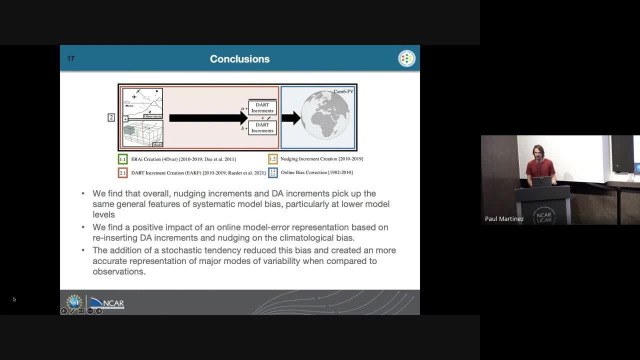 deepening of the illusion low. but that stronger gradient was an improvement in the beat state, it was an improvement in the mean state, but it degraded the, the. it essentially made the, the amplitude of the dna, like way too deep. um, this was just one member, or this was i mean. 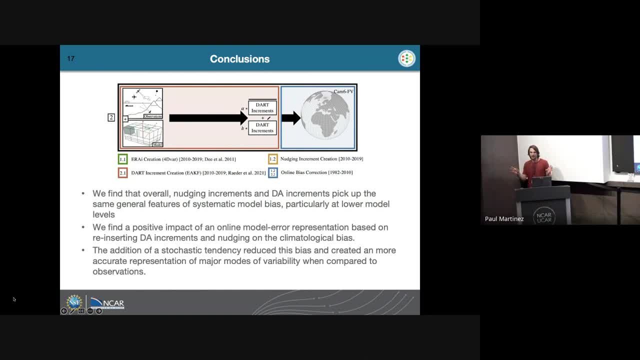 i did it. you saw it in every, in every member, so i ran it four or five times. it was technically the same thing over again, but you know. so, like four or five historical runs, yeah, yeah, and then we were also doing this: um, we were making sure that these were actually. 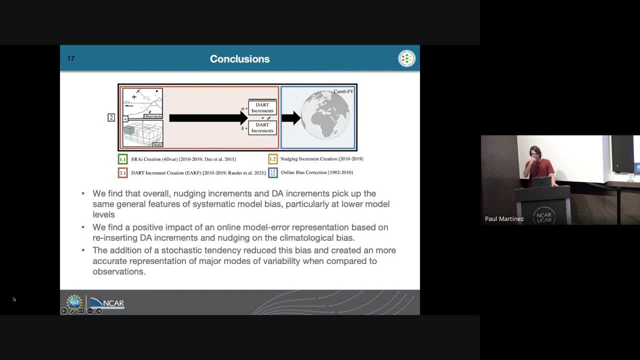 educated worth as much as you can in the 30-year run by taking the lens and seeing if, by taking 30-year chunks, we saw what was outside that range. i think it's actually your suggestion, yeah, yeah, so uh, yeah, we saw that it was a significant difference, at least using that framework, yeah. 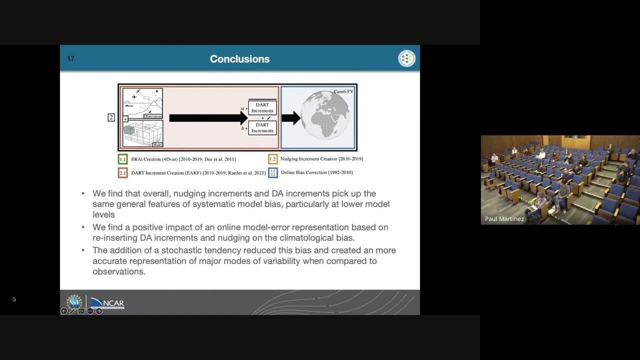 i have multiple questions, but i guess i'll ask one um. i was wondering um how do you make sure you're kind of so? this is all new to me, but i'm wondering how you figure out if you're overfitting. i guess is like the only word i could think of. like if data assimilation is kind of preventing. 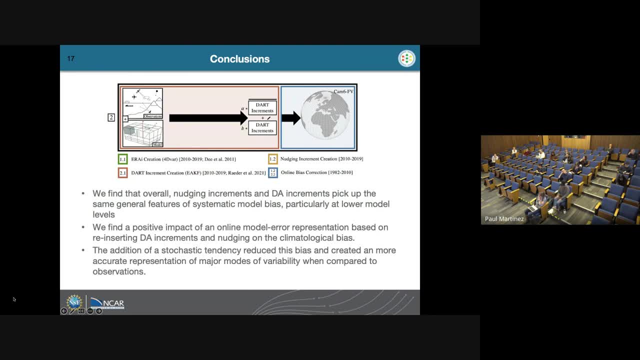 maybe, if these methods would maybe be an issue when looking at future climate change, um, and how you think about that. yeah, big, open question about the future: if we're going to go out of distribution um, and then also very hard to answer whether we'll know if we're going to another distribution. the hope is that you can use these tendencies, tendencies. 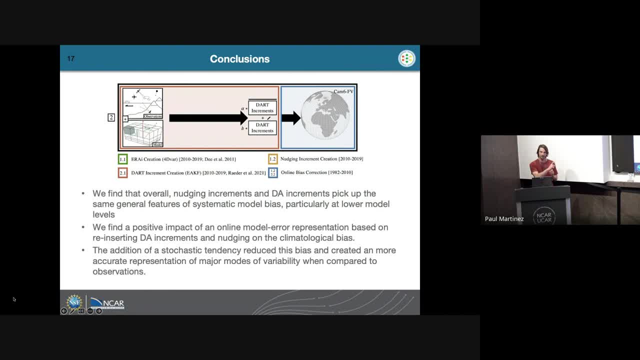 to point to actual physics schemes and say: you know, this is what we think is actually inherent in the planet. we can do that with some. There's sort of a summation of a lot of errors, so it's hard to pull out those pieces. but 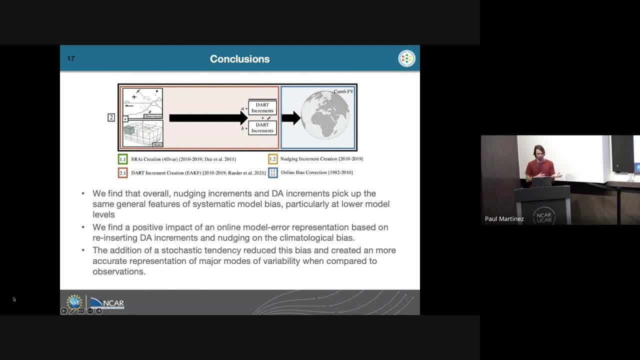 we have been able to identify a couple of things that we think are leading to problems. So if I can fix the actual parameterization fix then I feel good about it, Blindly putting it into the feature. we're going to have to figure out exactly what makes. 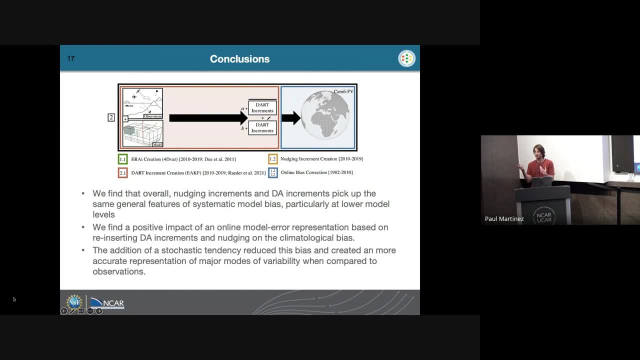 us feel comfortable And I think you can do that with perfect model runs right. So start to use one member that we know isn't there and try to correct to a different member that is in the future And we can say if we represent this climate state well, even though we're going out of. 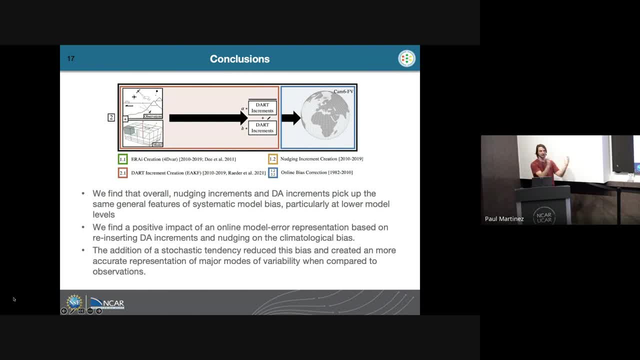 distribution, then maybe we can take our current climate and still apply these methods. yeah, So Any questions? I could ask a question You can ask. Yeah, I'm curious about the state-dependent bias correction. I'm wondering if the NN is picking up like- really like- modes of variability patterns. 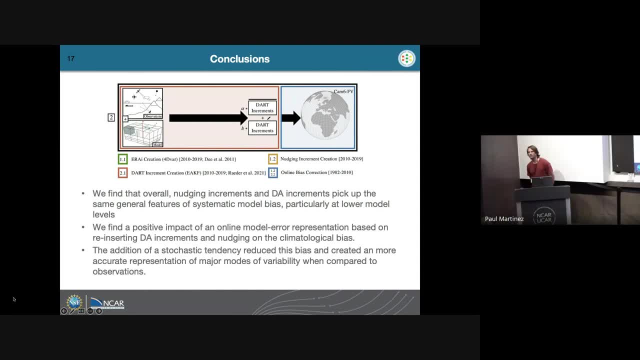 or what does that mean? So it's hard for it to pick up modes of variability dominantly, because it's looking at just like a 30-minute increment. So it's going to be like it'll see an extended jet and then give a geopotential, but that 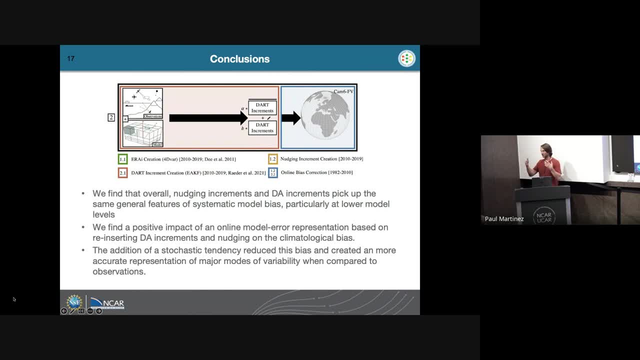 geopotential isn't going to look like, you know, P and A, or it'll be some representation of it. It'll have a level right or a high across the North Pacific, But what it's going to do is it's going to look like, you know, P and A or it'll be. 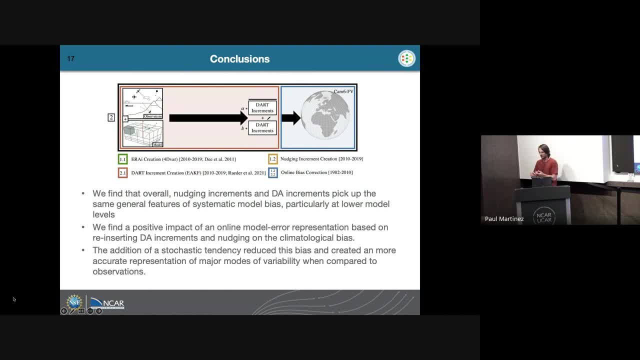 some representation of it. It'll have a level right or a high, But what it's going to feed it is representations of the prognostic variables. so u, b, t, q, surface pressure, temperature, surface wind stress, bottom temperature- a bunch of variables. 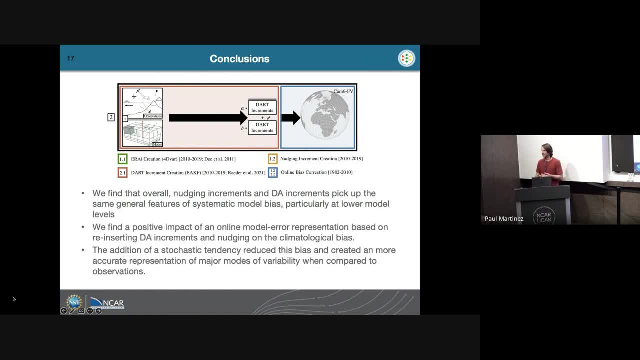 So it will have some representation of the current state, whether it can kind of like extrapolate and say, like I'm in this regime. We hope it will, but I haven't done any like direct testing. So the plan is to really say: you know, we're now in a super active MJO. 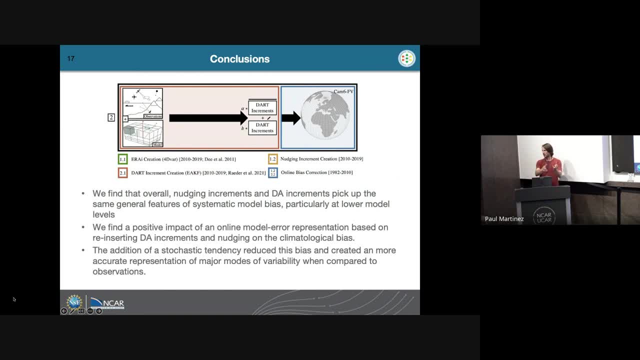 What do the increments out of the CNET look like? Or we're in a super active MJO, We're in a super active P and A. What are the increments out of the P and A? And then we'll be able to answer those questions. 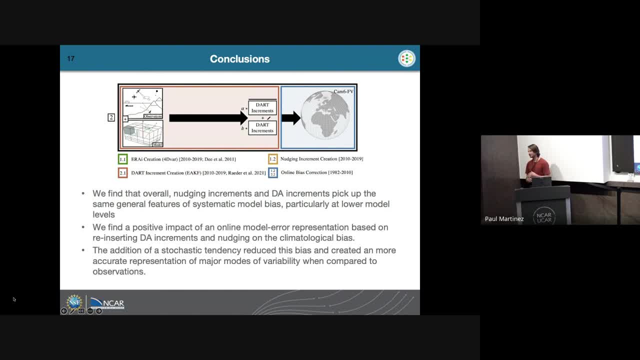 We haven't done that work yet. Okay, Ian, I don't know if I fully understood. I'll talk to you after- But it seemed like you're nudging to ERA interim, with the stochastic tendency, is yielding positive results. Is there potential then to? 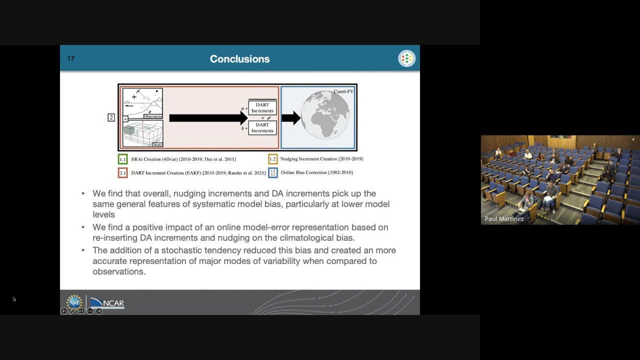 To generate a CAM reanalysis based on ERA interim. that just you know. basically, they've done the hard DA work. Now we can, you know, use what they've done to generate potentially an ensemble of atmospheric realizations on our CAM, in our CAM model. 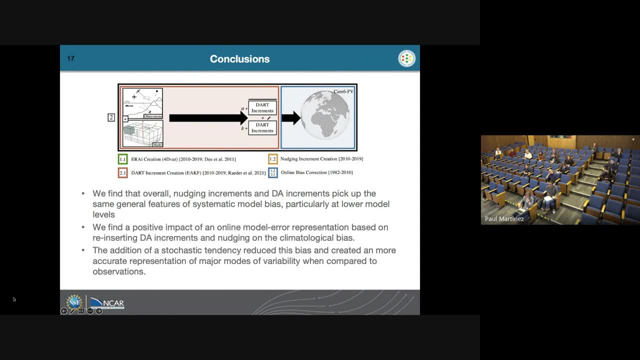 Yeah, I think there's potential there and folks are looking at this kind of cheaper data assimilation with- with you know, With- emulated neural networks. I don't want to speak out of place, though I wouldn't say I'm the expert in that realm. 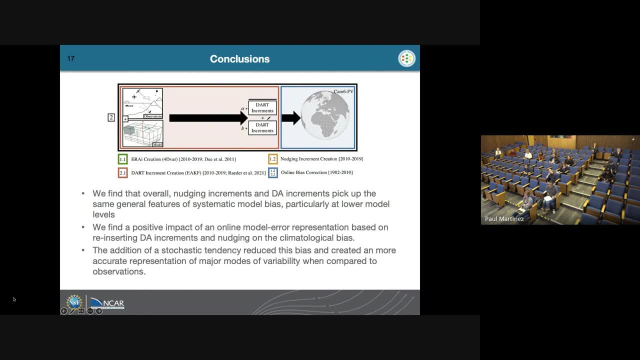 So I think it's a really good idea and I know that people are approaching it. But technically feasible, yes, but will it be better than our other products? Who knows? All right, Thank you, And let's thank all the speakers one more time. 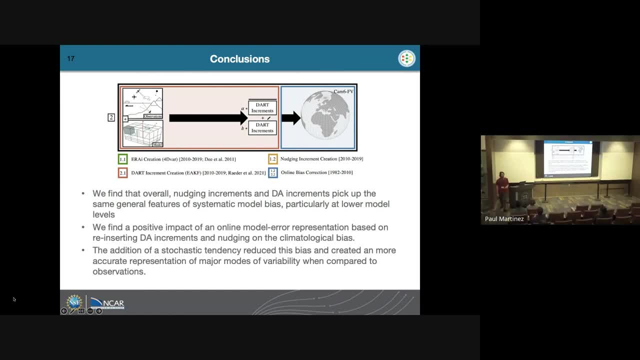 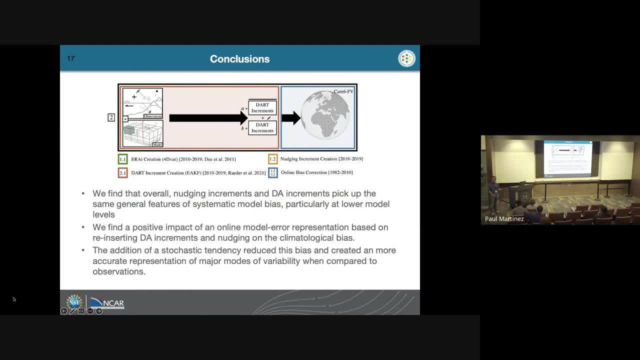 No, we should start and see if 50 minutes is long enough. We're going in at one o'clock. Yeah, Thank you, Birkhofen. that's a good thank you. Thank you, Birkhofen, All right. 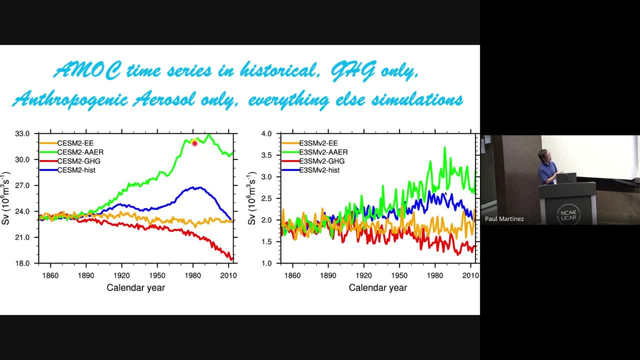 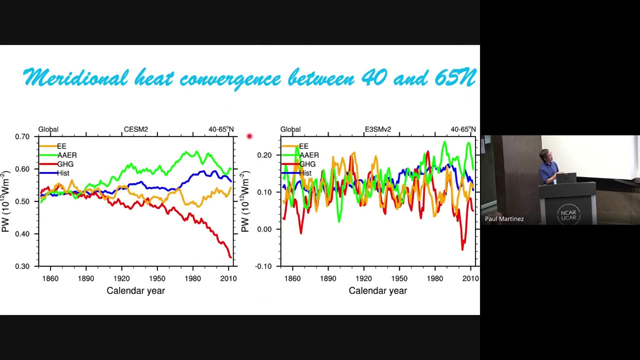 different scenarios. they're different than single photos are. supposing low policy is everything else and ground gas they are. the trend or time algorithm is similar but because the a mark change is so small, correspondingly it will affect the brady on h transfer. here i show is the meridian head convergence between 40 and 65 degrees north in a sample. 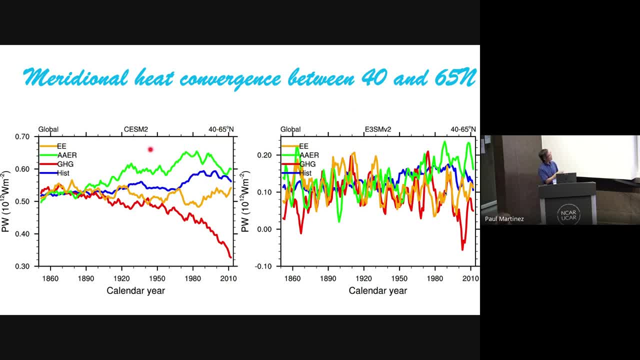 north Atlantic. we can see that for the csm, with the aerosol focusing, we can help significantly strengthen the meridian h trans conversion field convergence. that means it will cause him a warming in the south north Atlantic. at the same time it will affect other regions. therefore it will reduce. 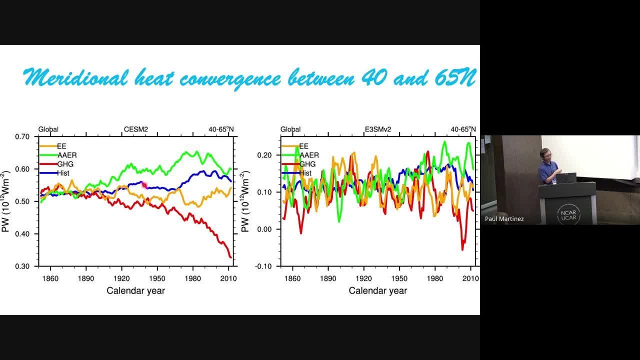 the response of the climate system to the aerosol faulting. That means that the cooling effect will be smaller in CESM than ECSM. Correspondingly, you can see, for ECSM, although the aerosol faulting also increases meridian head convergence. but this change. 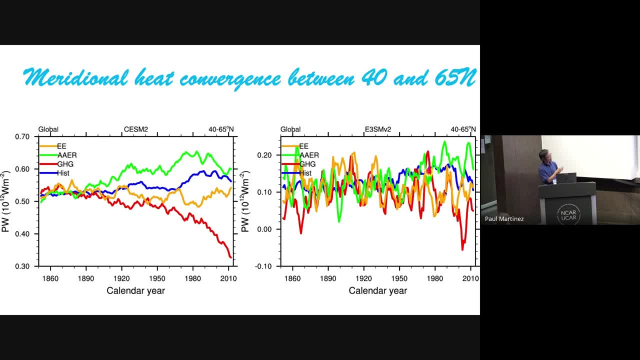 it cannot be the same. compared with the Boolean, It's statistically different. That means that although there's change, but this change may not be big enough to reduce the response of the climate system to the aerosol faulting due to an enhanced meridian co-retaining simulation. 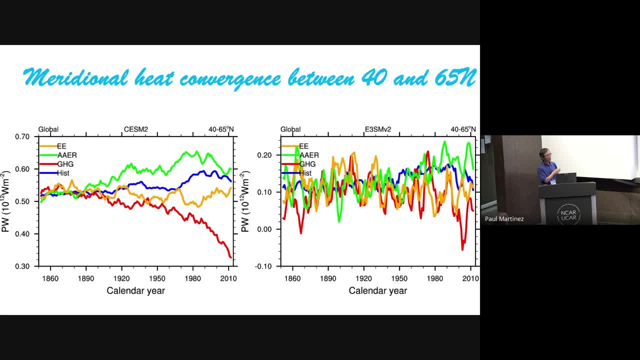 Therefore we propose that for ECSM the stronger response to the aerosol faulting may be because the AMOG in this model is too weak. So for the demonstration, we are currently running simulations by artificially sprinting the AMOG in ECSM. 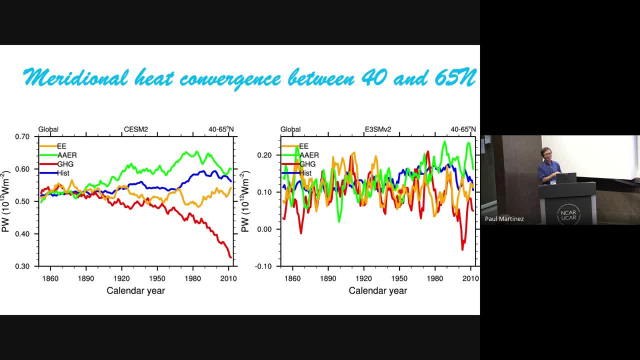 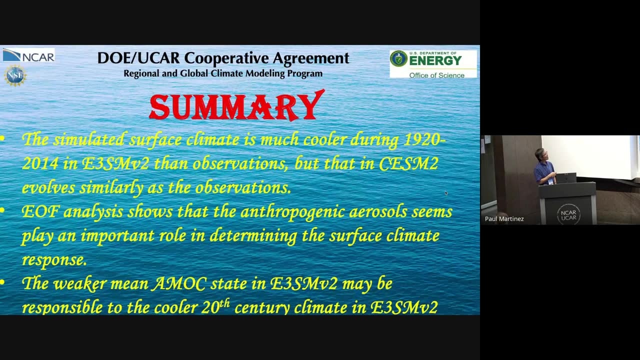 and see whether the AMOG in ECSM can reproduce better of the 20-second simulation and to see a better response of the AMOG to the change of the aerosol faulting. Here is our summary: The simulated surface climate is much cooler during the 1920 to 2014 in ECSM. 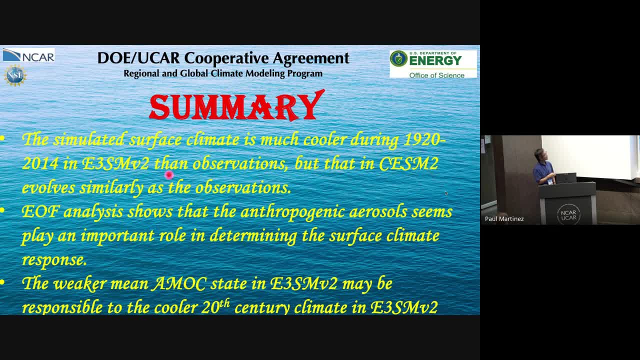 3-2 observation, but in that in CESM-2, the time revolution is similar as the observation. The new analysis Show that underfunding aerosol seems to play an important role in determining a survey climate response And the way for me AMOG state in ECSM. 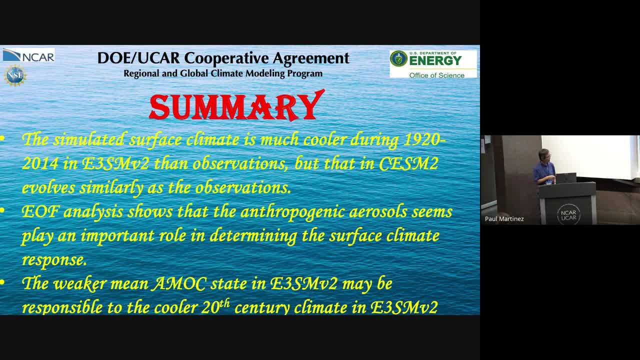 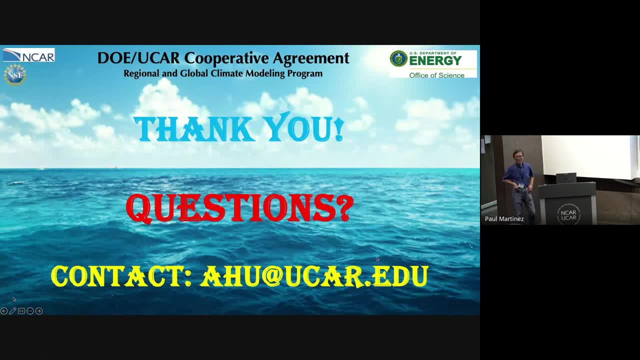 may be responsible to the cooler 20th century climate in ECSM. Thank you All right. apologies, online Didn't catch the minute at the beginning of the talk. If there are any questions, if you're online, please raise your hands or post in the chat. 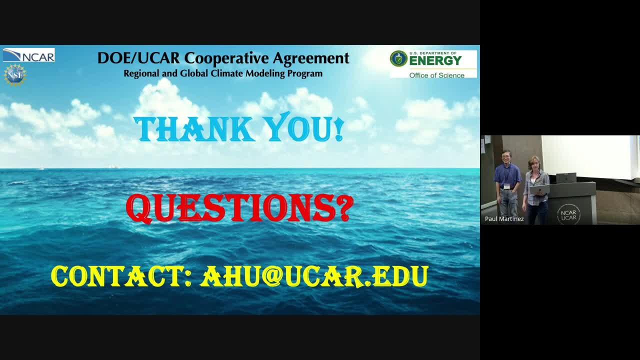 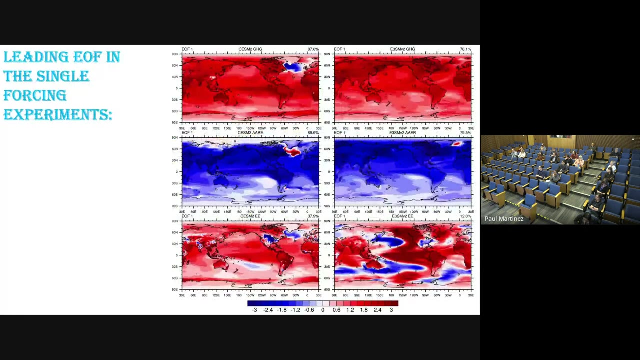 I'm looking at that. Anyone in the room? Oh yeah, Oh, nice talk. I wonder where you show the UF pattern of the greenhouse gas and aerosol, comparing between the CESM-2 and the ECSM-3.. So I wonder, like for the Pacific tropical region. 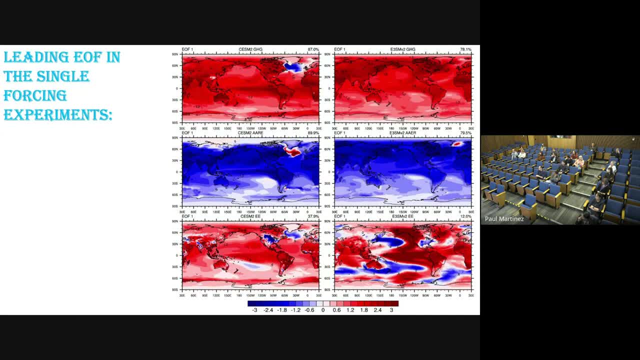 in the eastern part, where the ECSM-2 shows a larger temperature response both in the greenhouse gas and aerosol single forcing simulation relative to the ECSM-3.. Well, much of the change or the other response to other forces, the ECSM-3 is much larger than the ECSM-2. 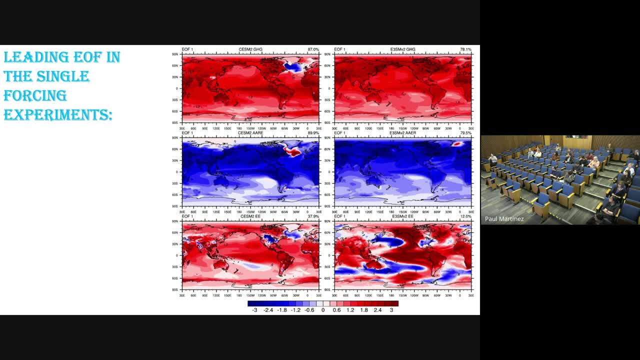 And they think that it's because of the ECSM-3, have a weaker response with anthropogenic forcing. I wonder: is it possible it's the other way around- that ECSM-2 tend to have a higher sensitivity? I wonder: if yeah, what's your thoughts on that? 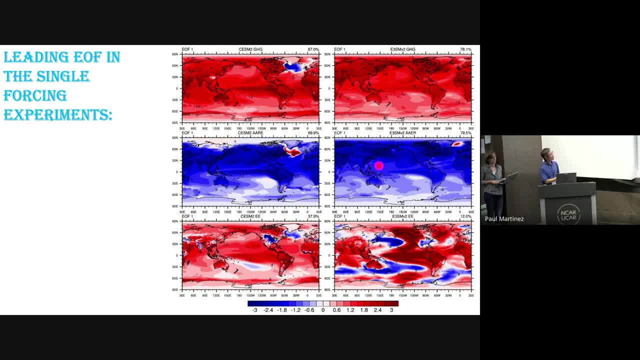 That's a good question. So for ECSM, actually for ECSM-V1, it has a similar equilibrium calamity than ECSM-3 and ECSM-2. And both of them have 5.2 degrees C. But for the ECSM-V2, the equilibrium calamity 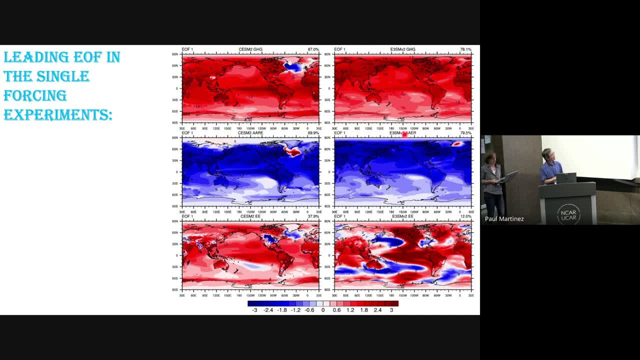 is reduced a little bit, And my explanation for the difference here is that with the wafer AMOC that surface calamity response, the transient calamity response, is much larger, although the equilibrium calamity is smaller. The reason for that is that because the AMOC is weaker, 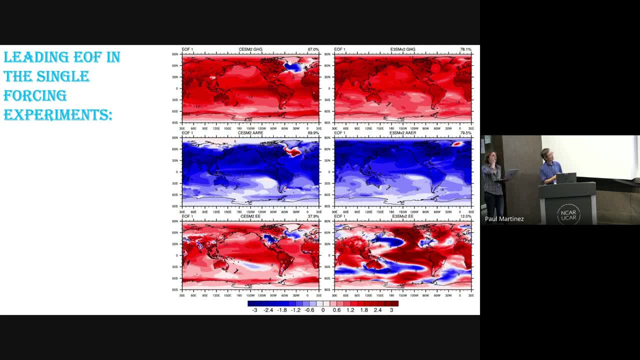 so the surface fabrication in the south pole and also elsewhere is much stronger. With stronger fabrication the surface roaming may be faster than you have when you have a deeper or weaker work force fabrication. Oh, thank you. Thanks. I'm curious how you're going to fix the AMOC problem. 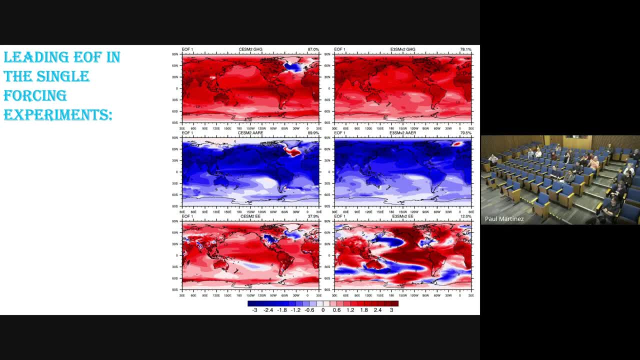 in E3SM and if you really intend to rerun all of the ensembles Right now we are planning to run one or two and 27 simulations with negative very water flow into the south pole and north pole. In this way you can artificially strengthen the AMOC. 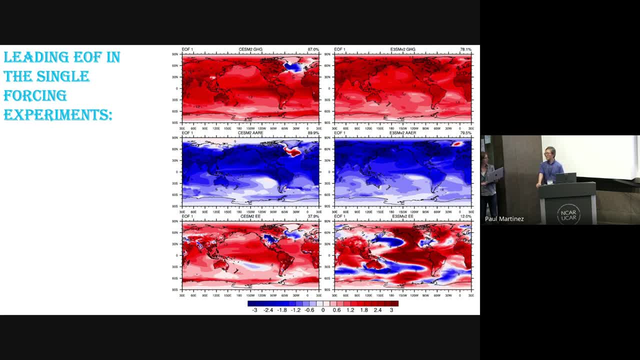 without changing the heat balance much, And right now NAN is running the simulation and I haven't gotten the results yet. Hopefully it's not fixed and I did part of the problem. All right, thank you. So our next speaker is the Shorin. 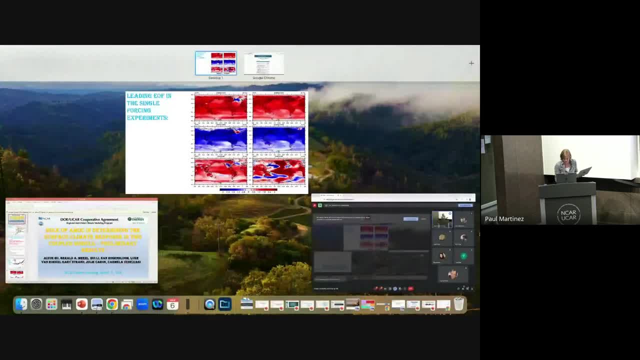 helping by the direction, indirect effects of aerosol forcing. And this is Shorin, who is the lead developer for the E3SM and the team, and he's going to talk about some of the things that we see in the E3SM platform. 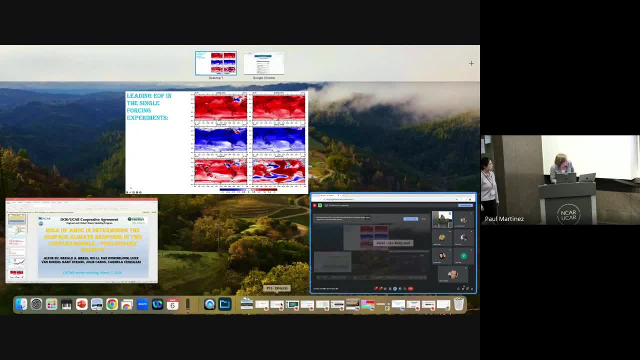 So, Shorin, do you have anything to add to that? I don't, Shorin, you can start. So, Shorin, we're going to start in the Q&A. Shorin, go ahead, Okay. 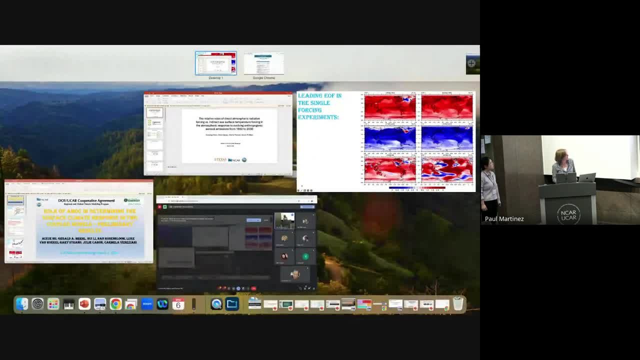 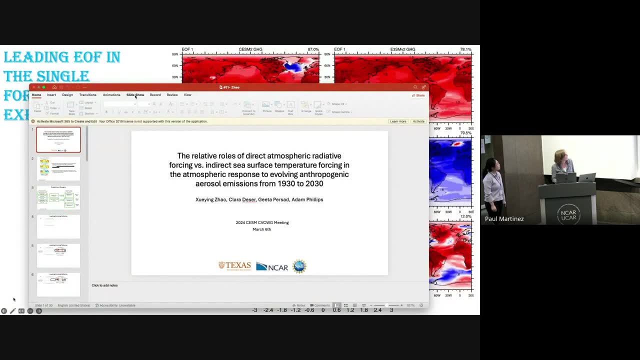 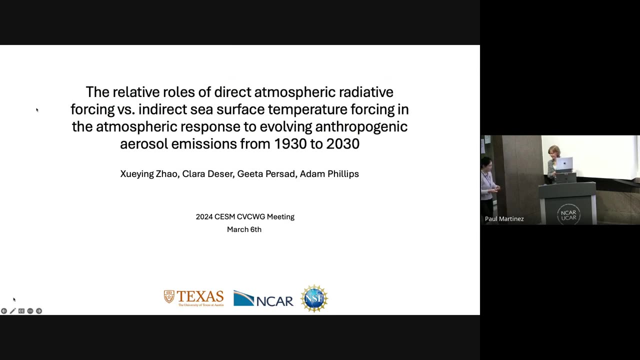 Shorin, you can start. Shorin, you can start. I'm just going to stop. I'm going to pause the Q&A and then we'll have some questions. Hello everyone, Good afternoon. My name is Shereen and I'm a postdoc from the University. 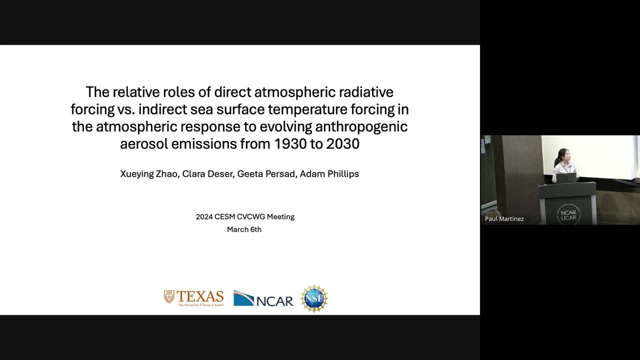 of Texas, at Austin, and I'm a graduate holder And I'd like to thank my advisors, Clara, Gita and Adam. So today I'm going to present the work about the atmospheric response to the astrophysicistic aerosol emission from 2013 through the 2030s. So we shifted the 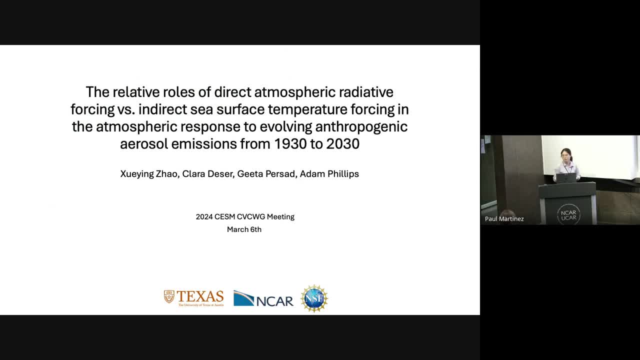 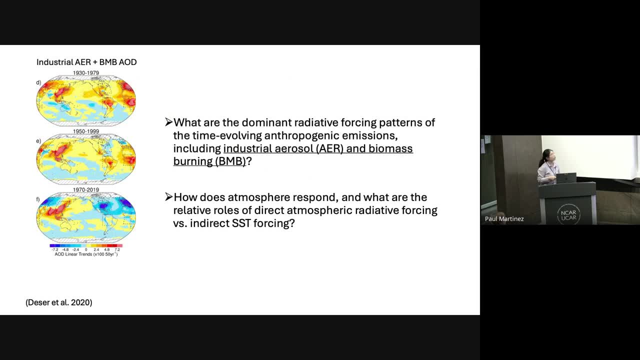 topic a little bit focused on the pathogen and image of the postdoc. So the map on the left are the trends of the AOD. You can come back with the CSM, O4K, large and thermal, minus the all but one forcing the XAR and XBMB. You can see that the AOD trend has distinct. 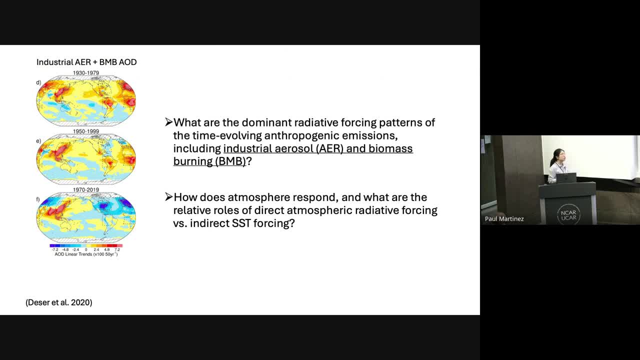 spatial pattern over the different periods in the 20th century. So we are interested in how does the time evolving after regenerative emissions would impact the spatial pattern of the climate response? So we try to address those questions. We focus on the two questions. 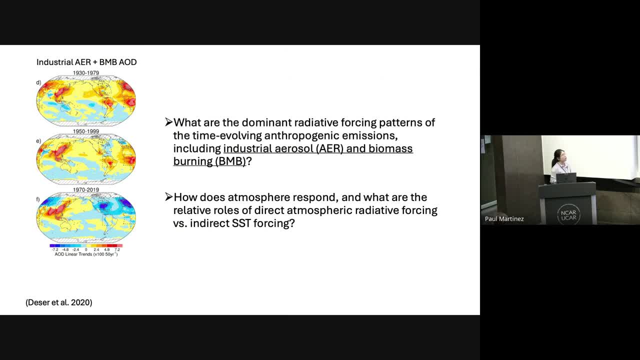 So, first, what are the dominant radio forcing patterns of the time? And we consider both the inertial aerosols and the biomass burning, while most of the previous study focused on inertial aerosol only. And secondly, this work focused on the 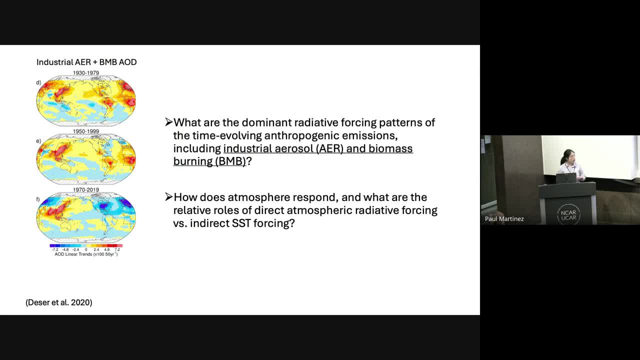 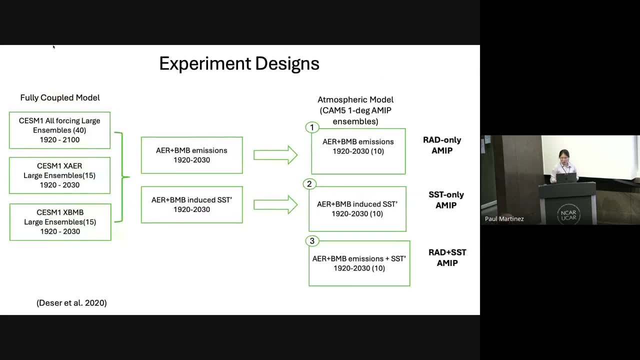 atmosphere response And we also try to assess what are the relative contributions of the radio forcing versus the indirect SST forces And we use three sets of can find one degree AMIP assembles And the first group is driven by the time-evolving CM5, the inertial aerosol and biomass burning. 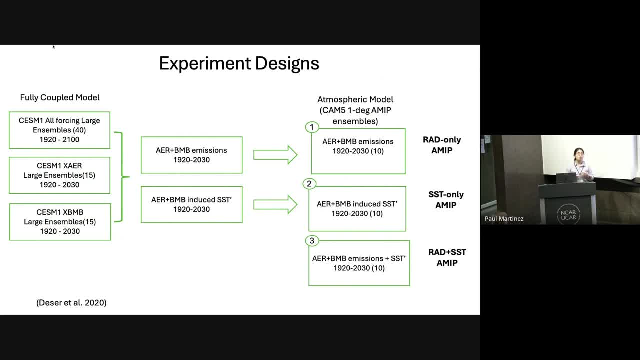 emissions, So with the SST fixed at climatology and which is called the rat-only AMIP, And the second group is driven by the SST response to the same CM5 emissions, with the emission fix, So which is taken from the ensemble mean of the CSM, O4K large and thermal, minus the 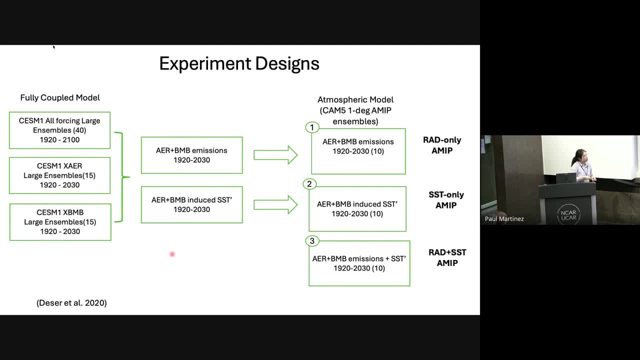 sum of XAR And the third assembles is driven by the combined forcing. So both the same CM5 emissions as well as the SST response. So we think that the response taken from the third group adds the total response to the same CM5 emission. 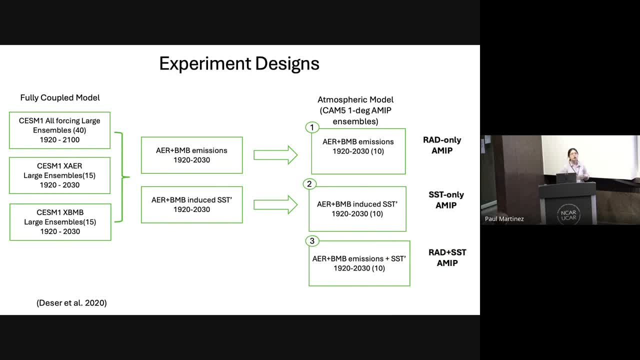 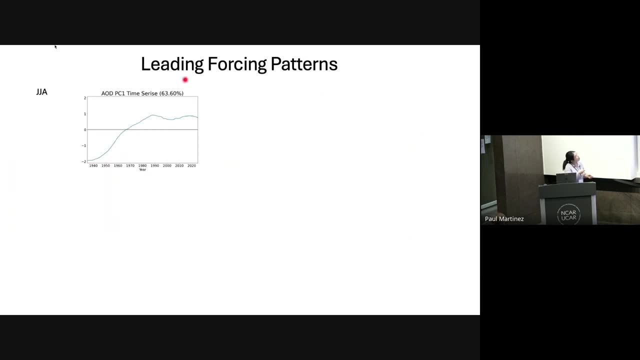 And we use the EOF analysis to estimate the dominant forcing patterns of the time involving anthropogenic emissions. In this talk I will focus on the JJA seasons And we use the 10-year rounding mean data And the time. the PC1 time series of the anthropogenic optical depths shows a monotonic increase. 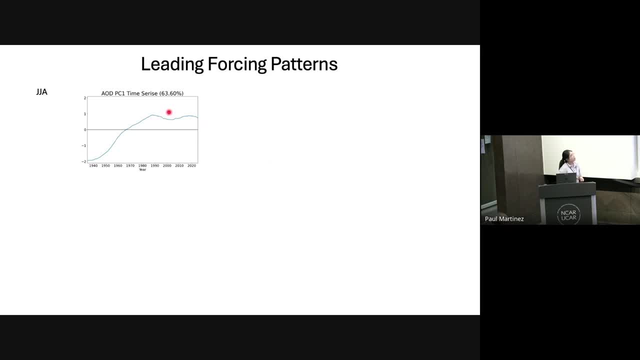 of AOD over the time and explain about 63% of the variance And the corresponding AOD regression patterns, shows the robust AOD increase mainly over the low latitude regions And where the PC1 stays nearly constant since the 1990s, and this is associated with the 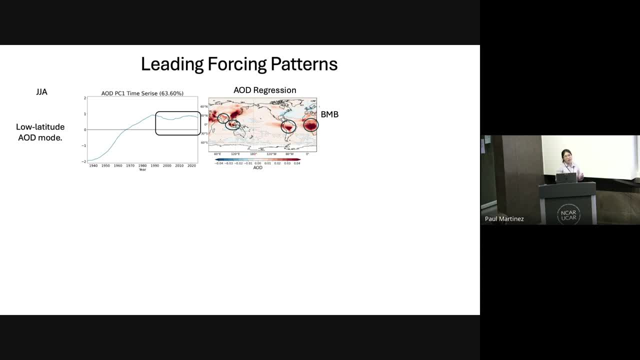 biomass burning in the tropical regions, which shows minimal change during that period of the time, And this indicates the biomass burning contribution in our low latitude mode And where the second PC time series peaks in the late 1970s and followed by a reduction. 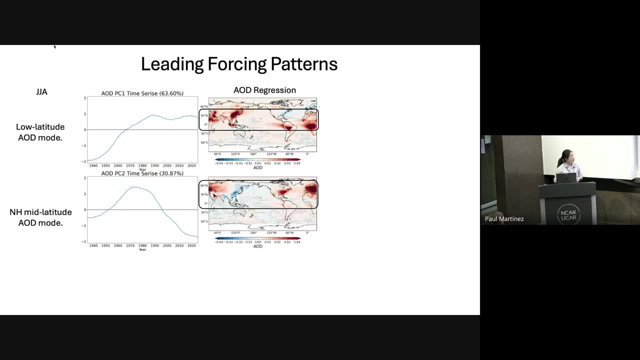 and explain about 30% of the variance. But the corresponding HLD map shows the robust AOD change mainly in the Northern Hemisphere and mid-latitudes and then accompanied by weak AOD reduction in the Eastern and South Asian regions. So the second mode describes the pattern of the industry aerosol emissions in the Eastern. 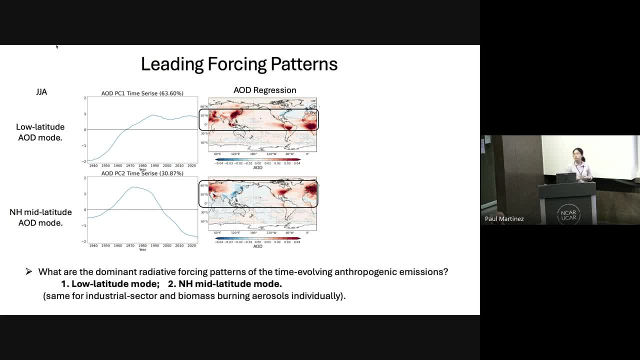 US and in Europe. So we found the two dominant modes of the radiative forcing in the time involving anthropogenic emissions, And the two modes explain about 95% of the variance, percentage of the variance And additionally we do find similar dominant radiofluid forcing. 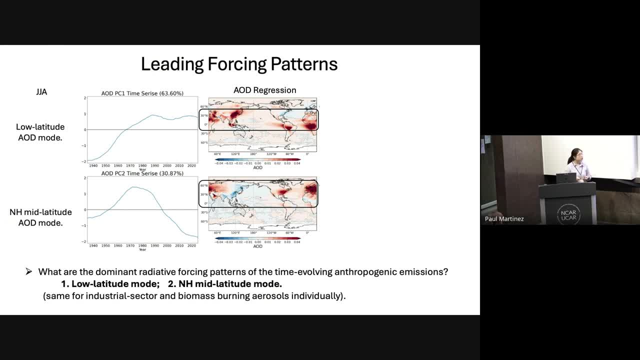 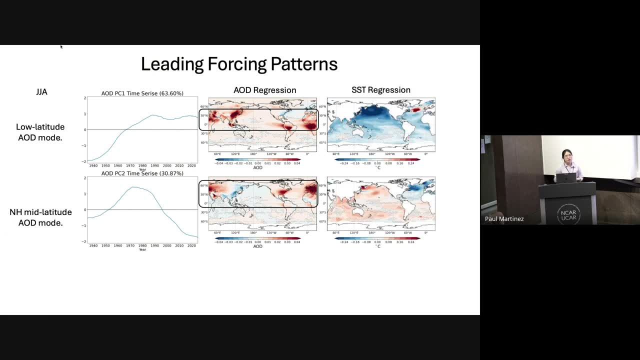 pattern from the single-forging large samples driven by the industrial aerosol and biomass burning individually And where the map on the left- oh, sorry, on the right- shows the regression of the SST response, Where in the low latitude mode the AOD change drives the 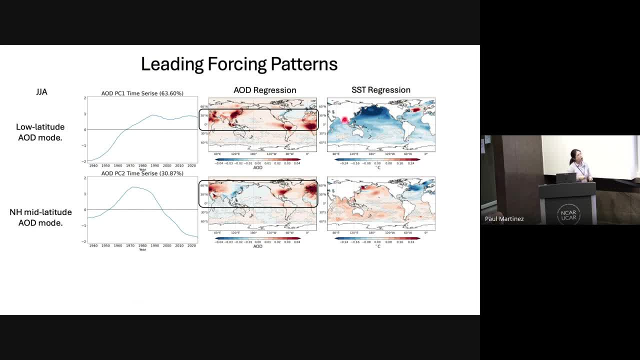 cooling in the ocean surface water. whereas the North Pacific cools the most Well, the Southern Ocean surface water shows weak changes And in the low latitude in the Northern Hemisphere mid-latitude mode, the AOD change drives the cooling in the North Atlantic and the warming. 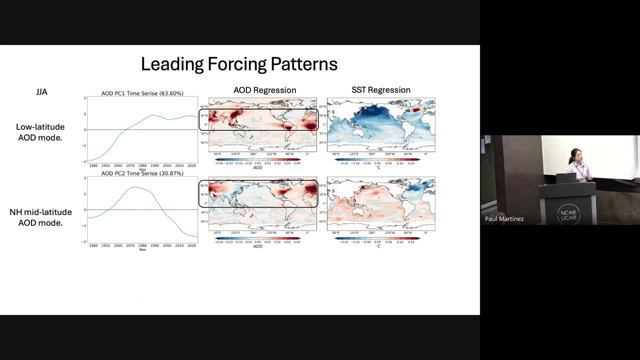 in the North Pacific. The warming in the North Pacific is associated with the weak AOD reduction in the South and East Asia, while the Southern Ocean surface water warms more, And so the pattern of the AOD regression and the SST response regression represents the dominant. 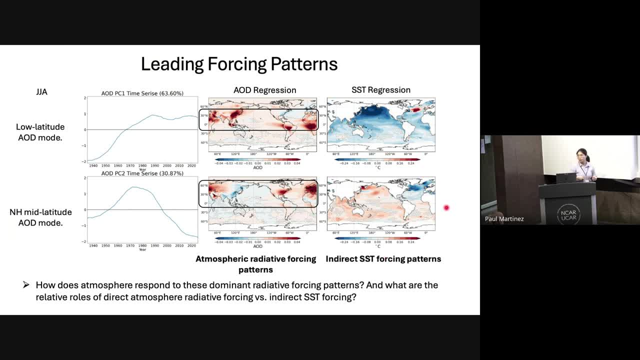 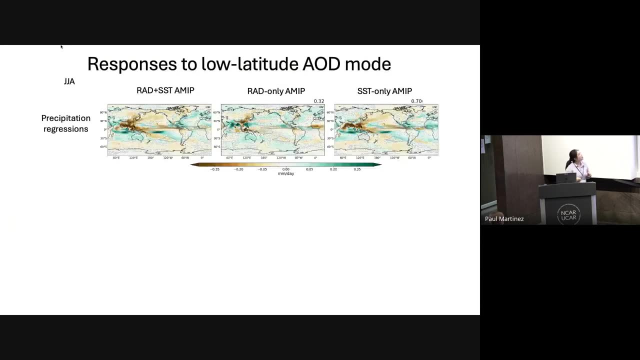 pattern of the radiant forcing and the indirect SST forcing irrespectively. And then I will focus on how the atmosphere responds to those dominant forcing patterns. And I will first talk about the low AOD mode. Sorry, low latitude AOD mode. So this shows the precipitation regressions, So the 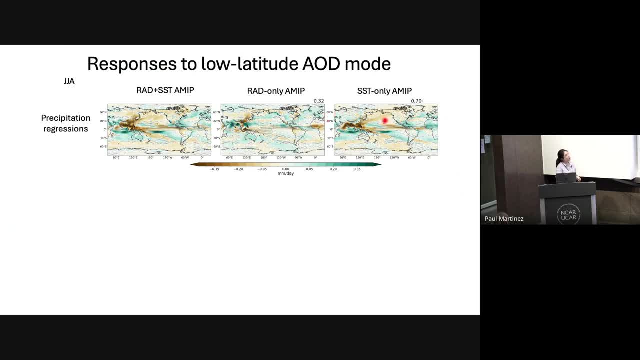 radiative force response is given in the middle and the indirect SST driven response is given on the right. So all the responses will follow the same order in the remaining tag, So well. the pattern of the total precipitation response is mainly dominated by the indirect SST. 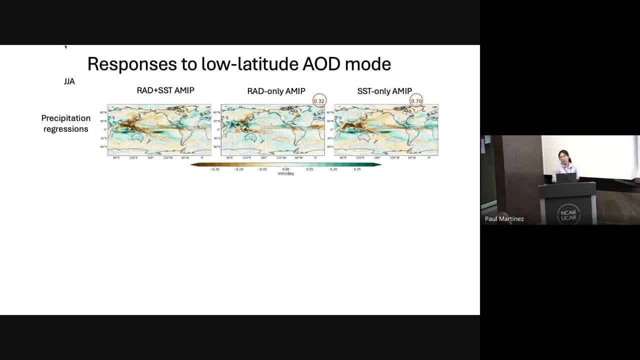 given their spatial pattern correlation of 0.3.. In contrast, the radiative forcing driven response, the spatial pattern move between the radiative force response and the full response is about 0.3. And in the full precipitation change a southward shift of the ITCZ is shown. This is: 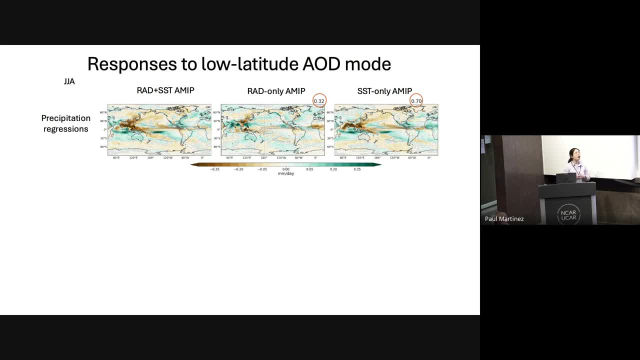 associated with the enhanced meridional temperature, a hemispheric meridional temperature. And now, if we focus on the low latitude region, now the indirect SST driven response is offset, Largely offset, by the radiative forcing driven response. The radiative forcing induces a large 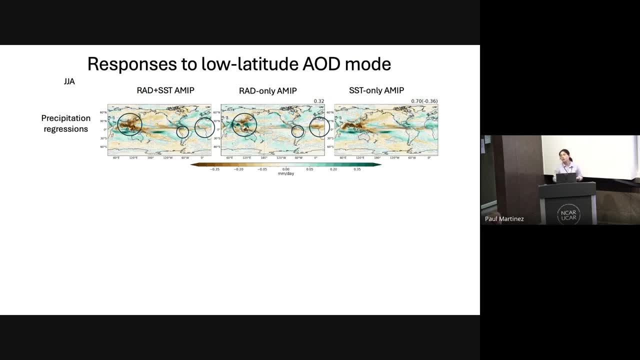 precipitation reduction in the low latitude land regions. But now if we move on to the east US and Europe region, So the total precipitation response in these regions is weaker due to the weaker change in AOD as well as in the sea surface temperature. 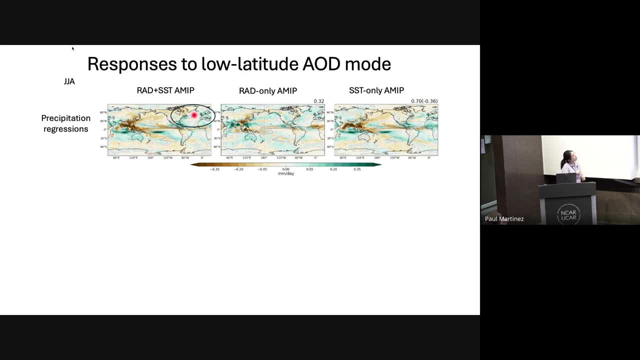 But I find interesting. is that so, where much of the precipitation change in the northern part of the North Atlantic is actually attributed to the radiative force- though the radiative force only induces a weak change in the eastern US and the Europe, And where we have the bottom panel shows the sea level pressure regressions? 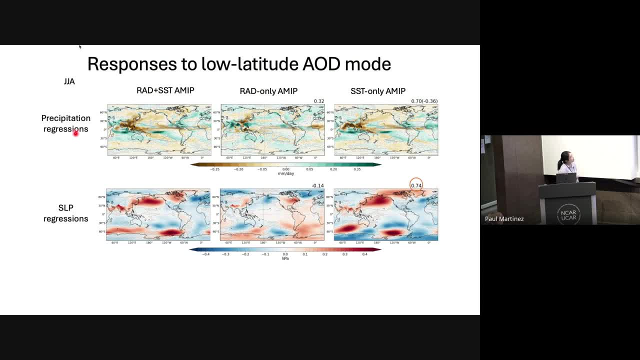 So much of the pattern of the total sea level pressure response is again dominated by the indirect SST forcing, given their spatial pattern correlation of 0.3.. 0.74, while the radiative forcing counteracts the indirect SST driven forcings. 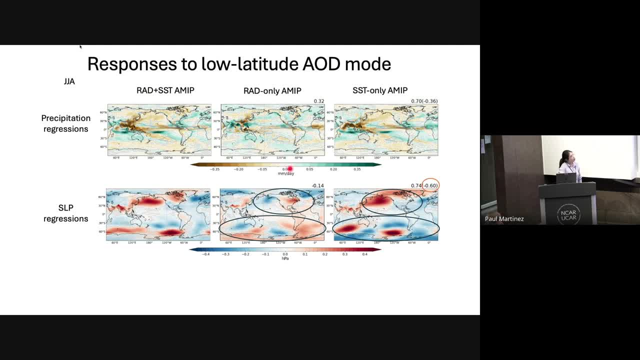 And the pattern of the atmospheric radiative forcing driven response and the indirect SST driven response is similar, given their spatial pattern correlation of 0.6.. Now, if we focus on the low latitude region in the North Pacific, the radiative forcings only induce a weak SLP response over the east and south. 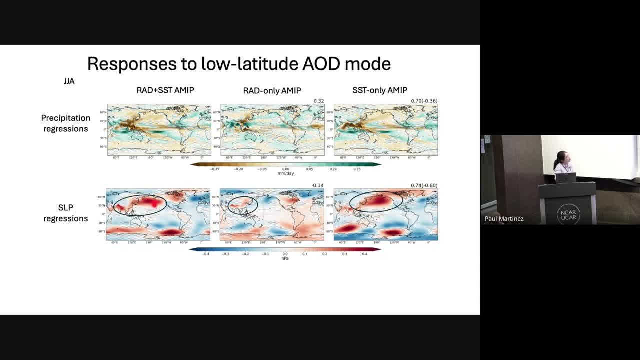 Asian emission regions, while much of the change in the North Pacific- so the weakening of the low- is dominated by the indirect SST forces. So this might suggest that the precipitation change in the east and south Asian land regions, the radiative forcing, is perturbed through more. 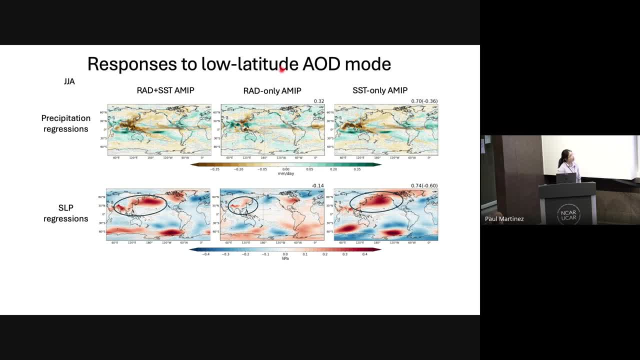 thermodynamic related process, while the indirect SST forcing perturbed the precipitation in the adjacent region through a dynamic related process. but further investigation is needed. So in short summaries, so where the pattern of the full response is dominated by the indirect SST and the radiative forcing modulates the indirect SST forcing driven response, especially over this. 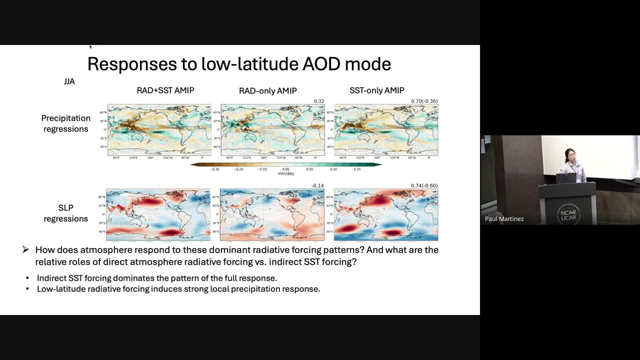 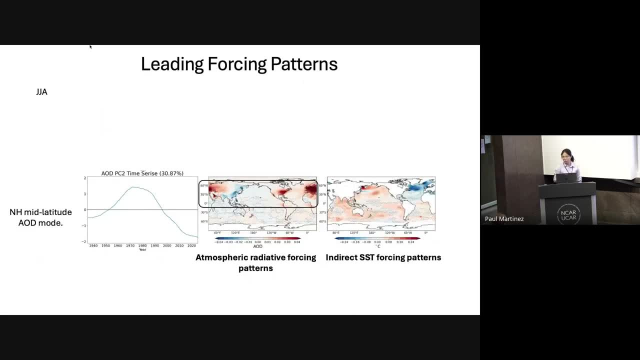 low latitude emission region which can cause a weak SLP response over the east and south Asian region. So this is the pattern of the full response which can induce a strong local precipitation response. And now we move on to our northern hemisphere mean latitude mode. 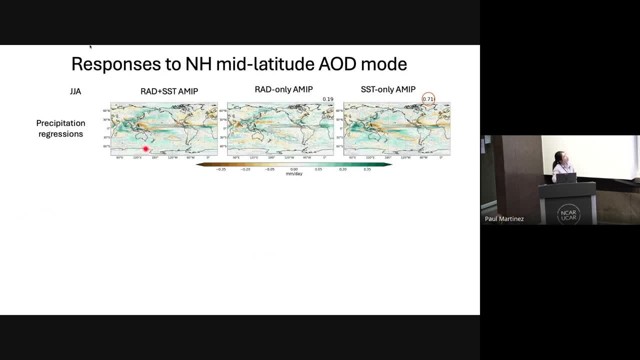 And we also find that. so the pattern of the total precipitation response is getting dominated by the indirect SST forcing, giving their spatial pattern correlation of 0.7.. And if you look back to the full precipitation response and the software shift, that ITC is also. 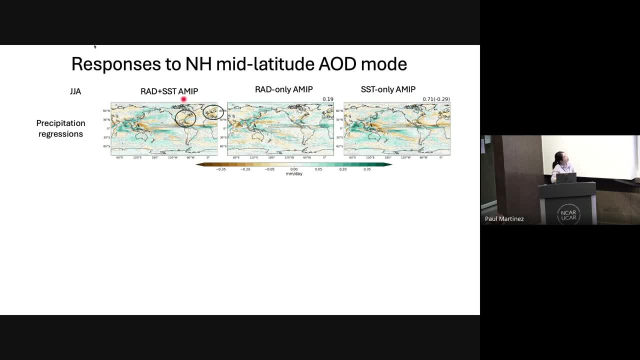 observed now if we focus on the east US and the Europe region, so much of the precipitation change here is actually driven by the indirect SST. So even though the AOD change in these two regions is robust, so the radiative forcing only drive insignificant and weak precipitation. 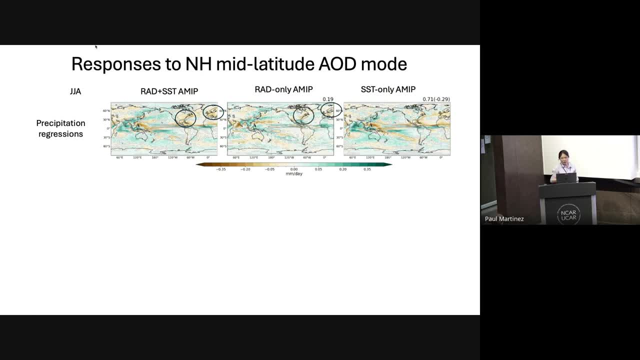 response in these regions. And now, if we move on to the low latitude region, the radiative forcing now plays a more important role. that much of the precipitation increase in the low latitude land region is dominated by the radiative forces. So if you look at the total, 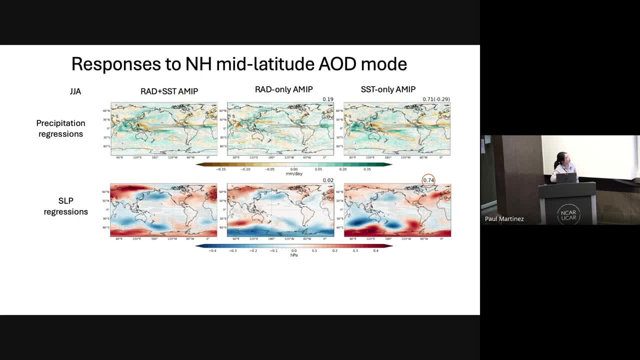 sea level pressure response. again, the pattern is mainly due to the indirect SST forces And while the radiative forcing driven response compensates the indirect SST reinforcing in the northern hemisphere and the counter axis in the southern hemisphere. And now, if we look into these, 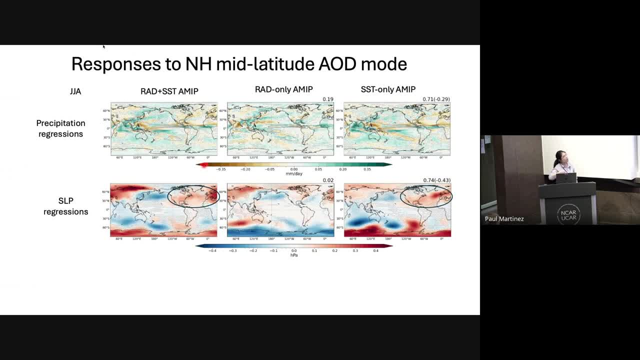 the East Asian and EU regions. so much of the sea level pressure change in these regions is due to the indirect SST forcing, And this might suggest that so the precipitation change in these regions is associated with the change in large scale, large scale circulation driven by the 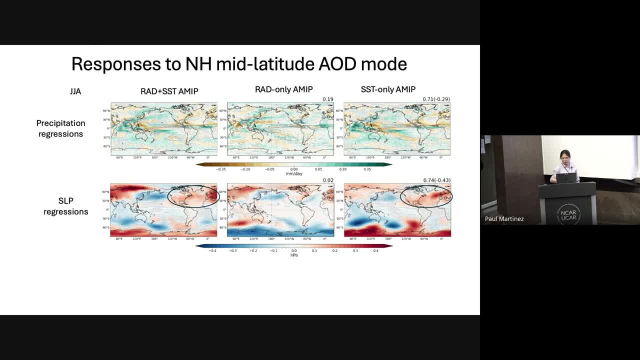 indirect SST forces. And, lastly, if we look at the Asian and the North Pacific regions, we found that the weakening- oh sorry, the strengthening- of Aluntan low is attributed to both the radiative forcing as well as the indirect forcing, even though it is dominated by 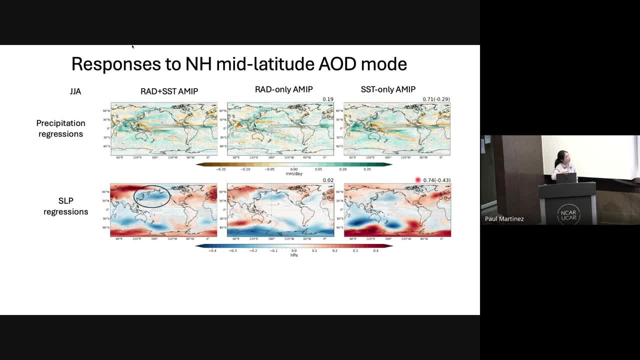 the indirect SST forcing. However, in the low latitude mode, much of the change of the sea level pressure in the North Pacific is mainly driven by the indirect SST forces, which is counteracted by the radiative force driven response. And, in short summaries, we have found the two dominant. 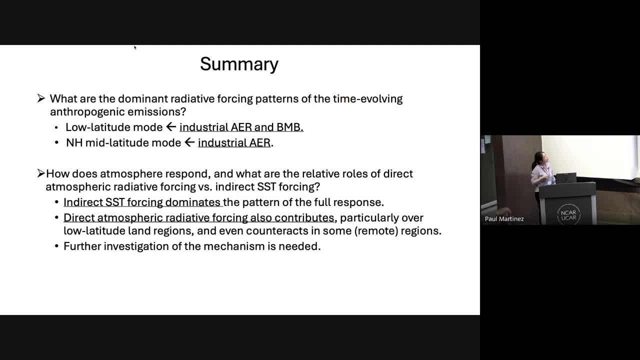 patterns of the body belonging to heterogenic emissions. And we have this first mode described the pattern of the innovative aerosol and biomass burning in the low, in the long latitude regions, while the second mode describes the pattern of the industrial aerosol emissions in the northern. 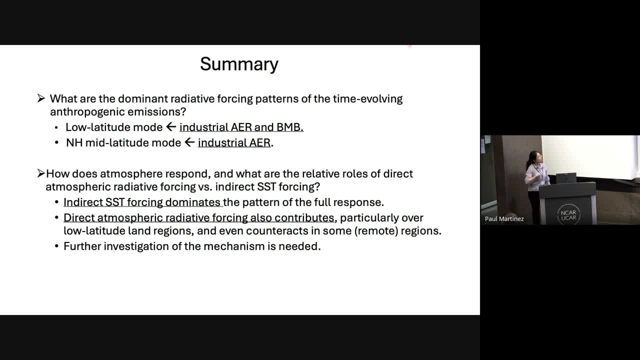 hemisphere, mid-latitudes and the pattern of the atmospheric response to these dominant forcing atoms is dominated by this indirect ssc forces, while the radiative forces modulates the, as in our ssc driven response on a regional scale, particularly over the low latitude land regions. well, the mechanism of those response is further investigations and recall what the island 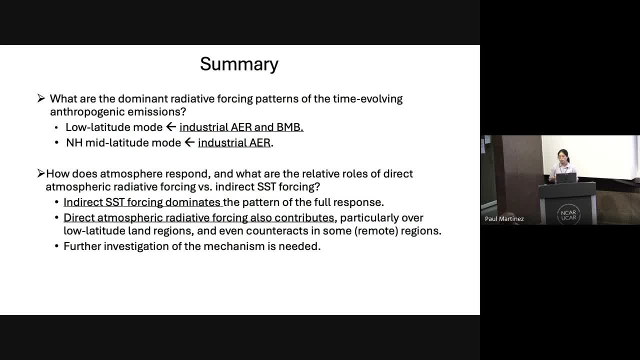 mentioned, uh, the, uh, the csm2 simulation driven by the same signifying emission. it would be interesting to compare that emission with the model that we use here and thank you. any questions? yeah, another cool result of this clarification. so, for methods, do you use your candidates leading modes by applying this uf? 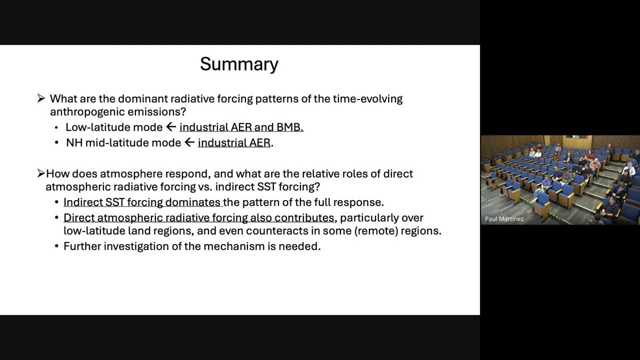 analysis onto aod. yes, of tennis as an earth or associate as more forcing or sd forcing by regressing ssc onto that leading mode of ld. yes, all right. i was wondering if you were to say: apply this uf directly to the fully coupled single force and rock generated ssts, would you? 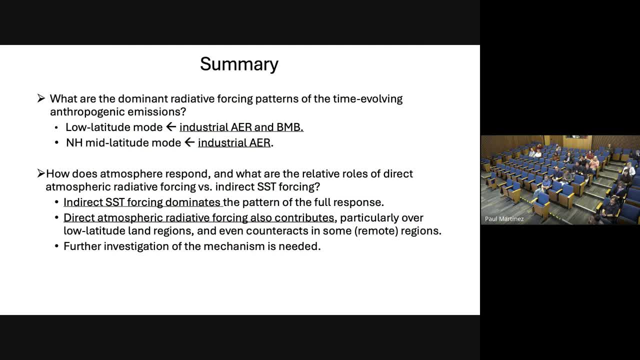 get the same patterns or modes of ssts, actually more appropriate to consider that as a direct ssc forcing to ask one of your response. um, so i did compare the uh vyrant alternative sft from the uh from fully coupled, so the ssc response okay. 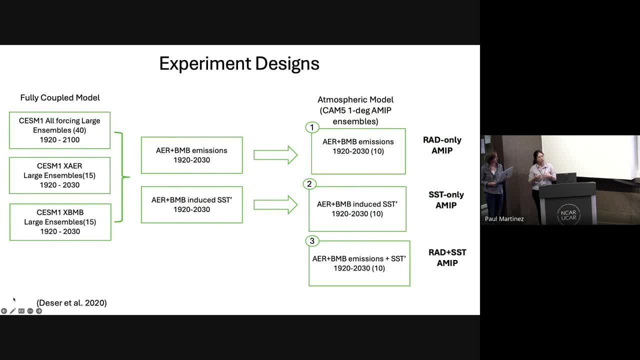 so the ssc actually used here is taken from the fully coupled information. so it would be the same as if you're reading the same data as ssc force expression. so if you are interested in that kind of thing, you can justgrow out this reference point slide if you want to do this. my other question is: 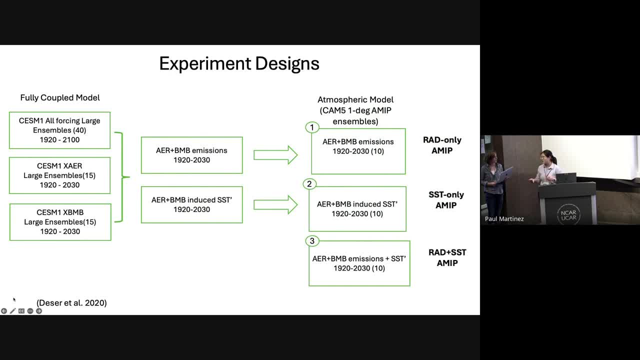 how do you explain the Emirates rc4-D 0722.5? you may use theạninical與-xs Zarate all that kind of data to regress onto the OD, the same PC timelines. I guess another thing is about the uh you're asking is about the linearity as we kind of decompose them into uh, radio forcing versus. 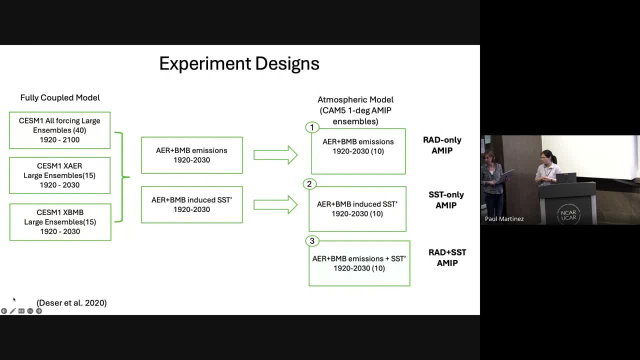 the linearity can be also interesting as it's wandering the leading pattern of sst, usually regressness. t sounds to the field in the new mode versus the leading mode. or you beating yourself because? because, even though in the fully coupled simulation this is still the uh, the driver. 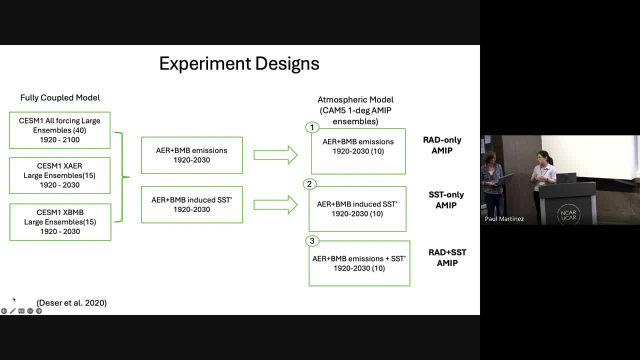 is the, uh, the, the emissions itself. so this is Steve would be, but any of the changes seen in the ssc is still due to the, the emissions. so if you uh uh so the dominant, I did do that. so dominant mode is very identical to what I did here. he's. 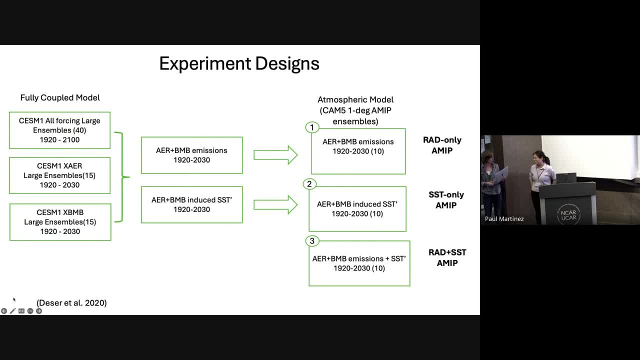 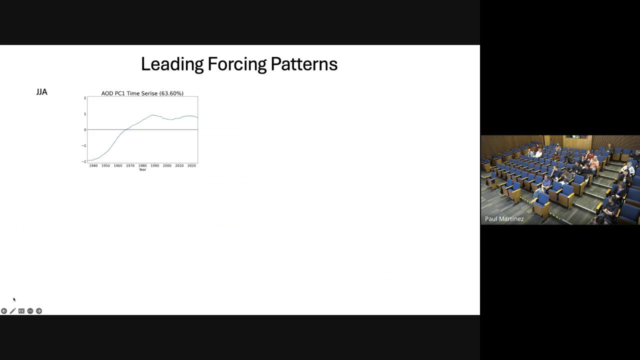 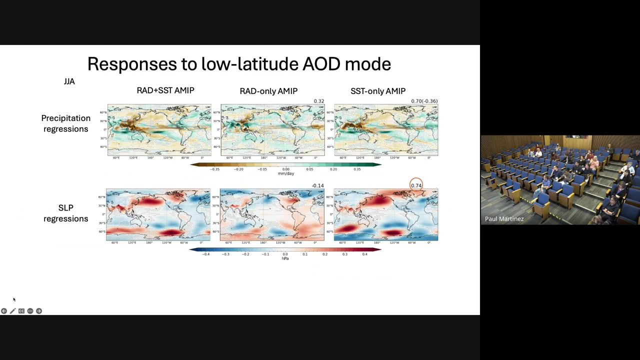 just using based on the aiming, because the data itself is the same. yeah, any other questions? yeah, I'm curious about the causes of the increased pressure in the North Pacific. in, in the, uh, low latitude mode, you have this big, increasing high pressure. do you have any thoughts? yeah, that one. do you have any thoughts on on how is it caused? 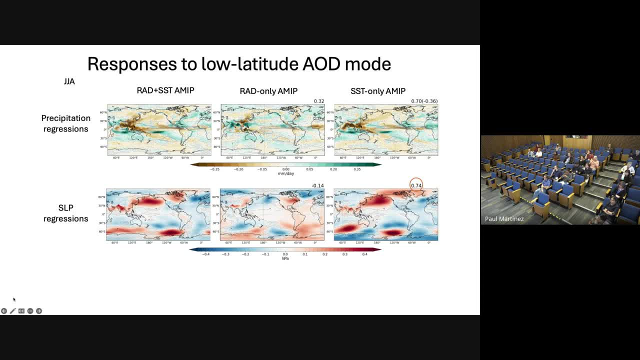 I I am not really clear about what causes it, because the North Pacific here feels more than all the other um motion bases. I wonder if it's because of the cooling they kind of uh more kind of enhanced decent um vertical emotions. so you have kind of a diverging the surface and this is how you're getting kind of a cool high. 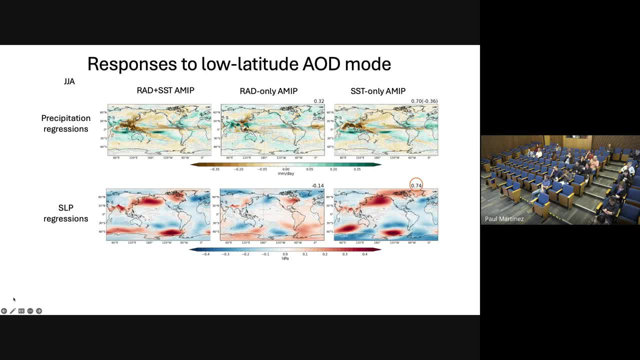 response in the North Pacific. yeah, that makes sense. yeah, yeah, could be a teleconnection. I was just wondering if you had thought about it. yeah, yeah, that leads further kind of thoughts on what causes it. yeah, awesome, thank you. all right, thank you, thank you. so our next speaker is Pedro on the 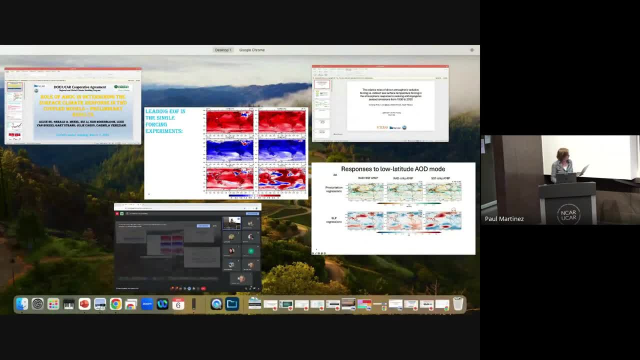 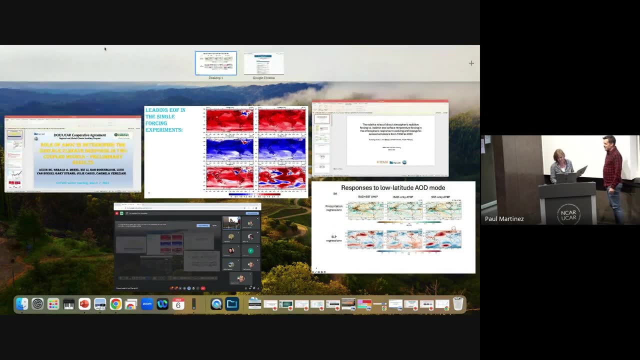 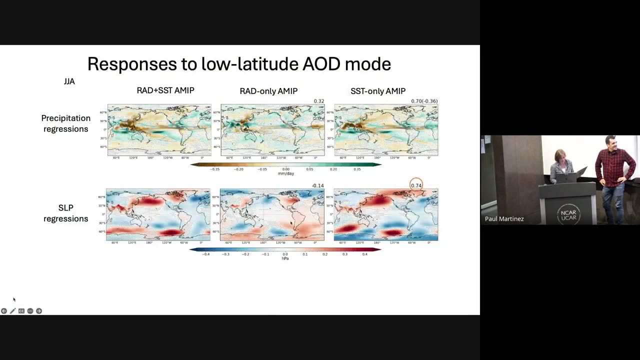 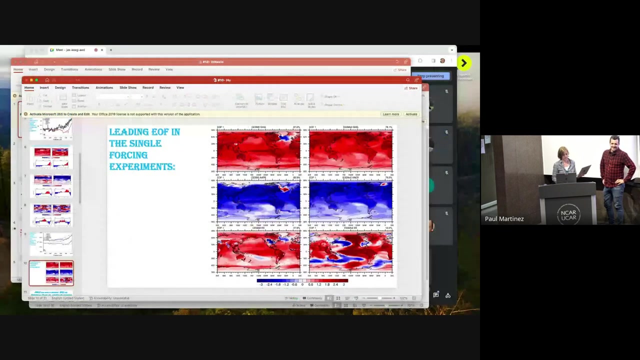 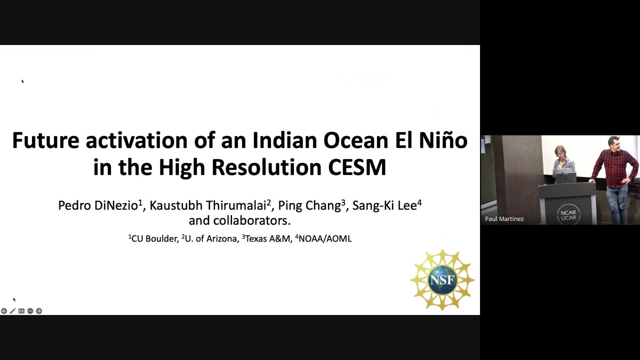 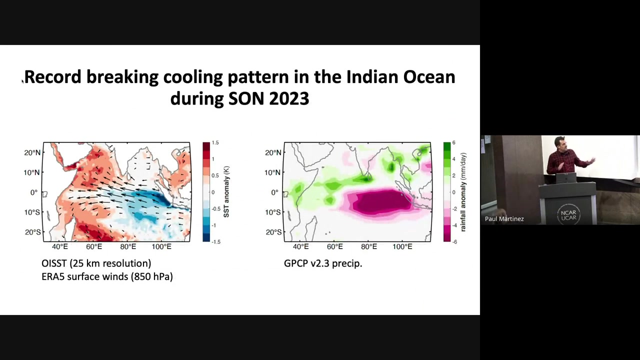 um, because it's a cold, it's a cold pattern. you know we all get confused, but suddenly you know, and so so I'm gonna add to that confusion. maybe you need to abandon media, yeah, anyway. so these are observed SST anomalies and rainfall anomalies for last last year, October. 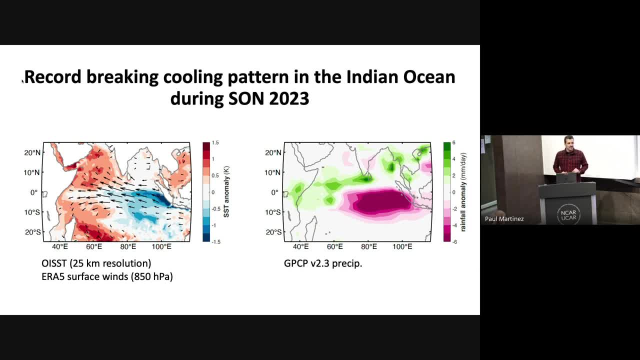 no September, October, November season. and while the rest of the planet was baking, the Indian ocean was in this cold pattern which, um so here I'm using optimal interpolated soldiers with high resolution and and that helps you resolve these really strong cooling on the equator it's hard to see in other SST products. 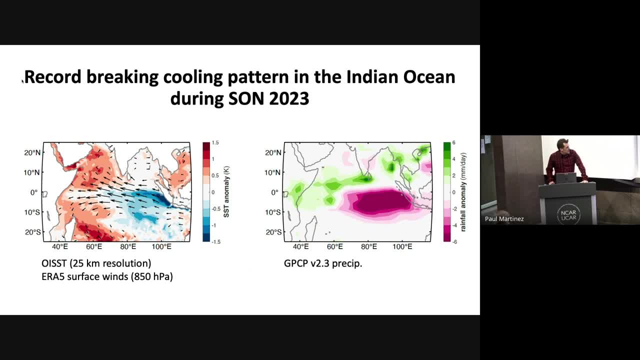 that are more heavily smooth and interpolated, and you can see that along with that intensified equatorial cooling in the Indian Ocean, you had easterlies- anomalous easterlies recall that the of Indian Ocean during this time of the year is weakly westerly, So this was probably close. 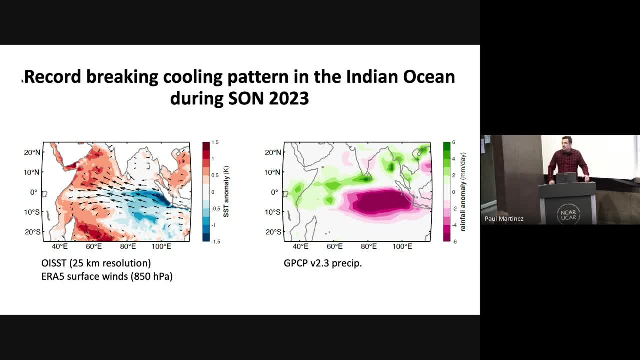 to absolute. easterly. It's driving upwelling, reinforcing this cooling pattern, And with it you have rainfall anomalies that are consistent with the SST anomalies: a lot of drying. Look at the color scale. That's a massive drying over the eastern Indian Ocean during that. 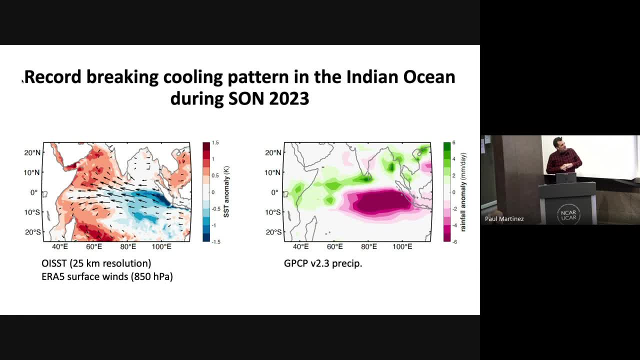 season last year, influencing Sumatra and Java. Recall that Java is the most densely populated island on the planet: There's 200 million people living in Java, that tiny island almost on the edge of my map. And then, in East Africa this season, there were torrential 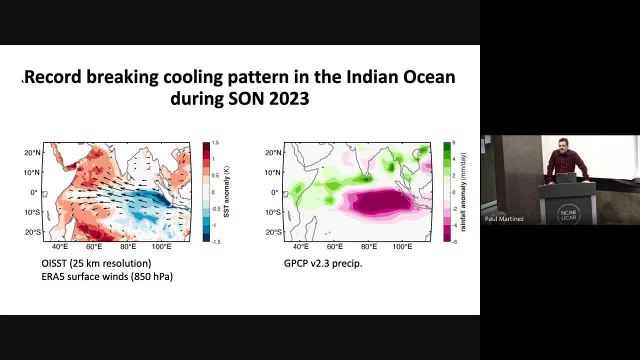 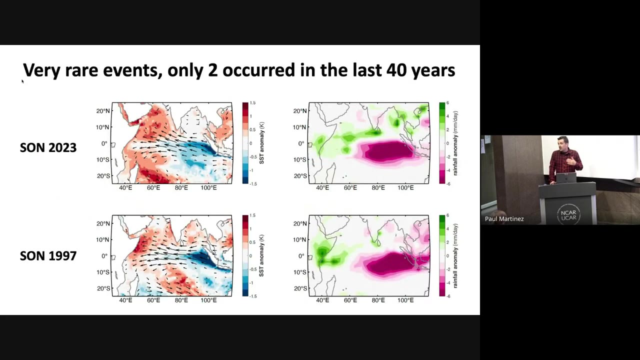 rains. This is a part of the world. Java has been experiencing persistent drought, So this looks like the Indian Ocean dipole, which is one of the leading modes of SST by Indian Ocean. So how rare are these events? Well, actually, the only time that this happened was in 1997.. And this is the same. 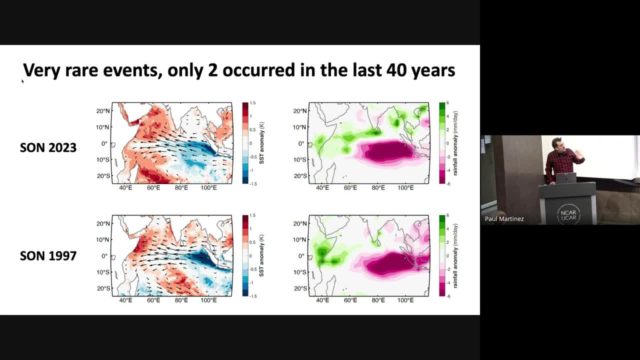 plot for that year. very similar, Perhaps some differences, but I think they're strikingly similar, And actually these are the only two times that these type of events happen in the Indian Ocean since 1980, when we have these high-risk data that can resolve what's. 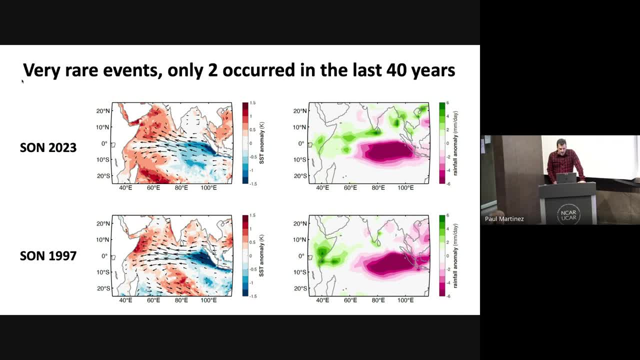 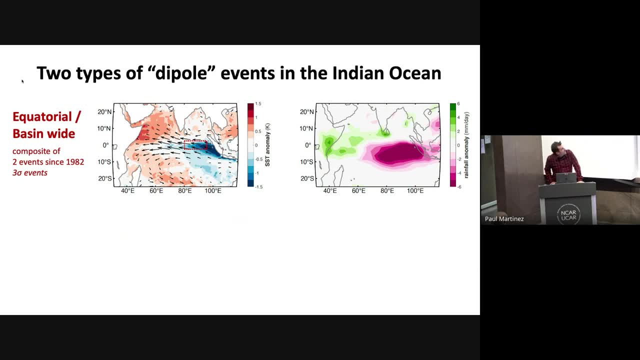 going on in the equator. So it sounds like the Indian Ocean can do this equatorial basing-wide mode. So if you average all those two events and then we have the dipole-mode, which is the rest of the events in the Indian Ocean. 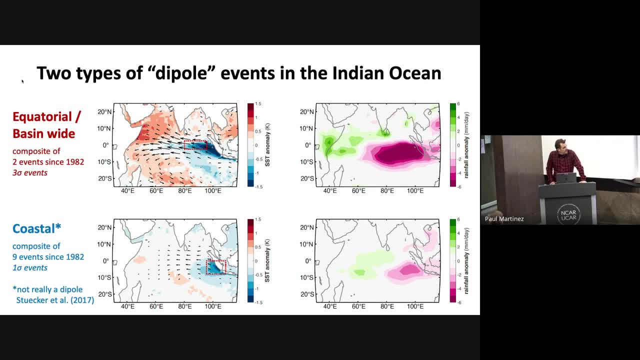 If you compose it based on that box off the coast of Sumatra, you get more of a monopole restricted to the eastern side of the basin, with much weaker rainfall anomalies. So there's a lot of confusion on what's the Indian Ocean dipole And the dipole aspect of these variability's. 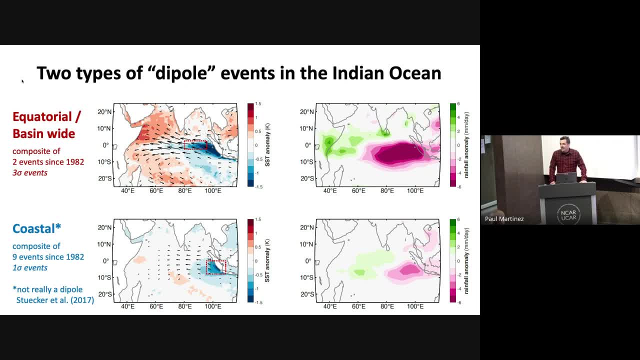 coming from this really strong, very rare equatorial events And most of the events in the observations, at least since 1980, are these more coastally confined cooling events. There's also warming events. The warming events are like this coastal pattern: There's no warming. 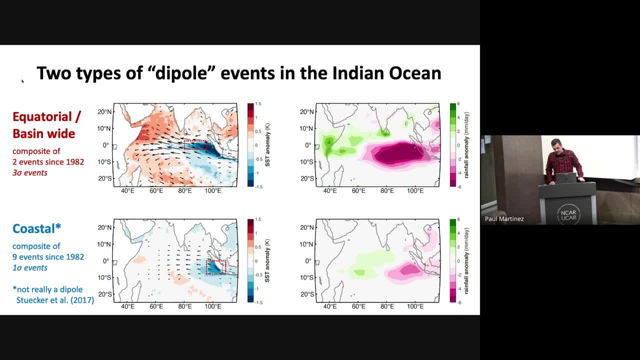 events that are equatorially intensified, like the ones on the top. So every time there's a big anomaly in the Indian Ocean, I get excited, because we wrote a bunch of papers proposing that, as a result of climate change, the Indian Ocean could start experiencing much stronger viability. 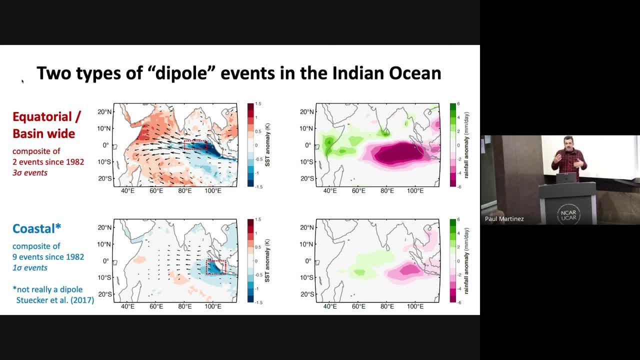 associated with the emergence of an equatorial mode that would involve dynamics more akin to Nino in the Pacific, With wind anomalies more like this. I would call it La Nina in the Indian Ocean. So every time one of these events happens, I get excited. It's like: is this happening? 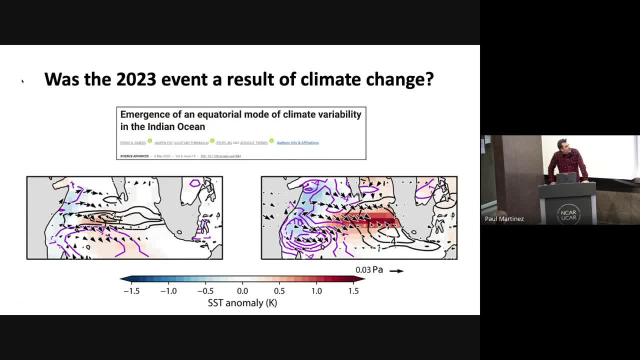 So I'll show you. These are results from one of those papers. These are some idealized simulations of the last glacial maximum, in which we've got rid of ENSO, We've got rid of the dipole mode. We've got rid of the dipole mode by just restoring SSTs And because the mean climate was so altered. 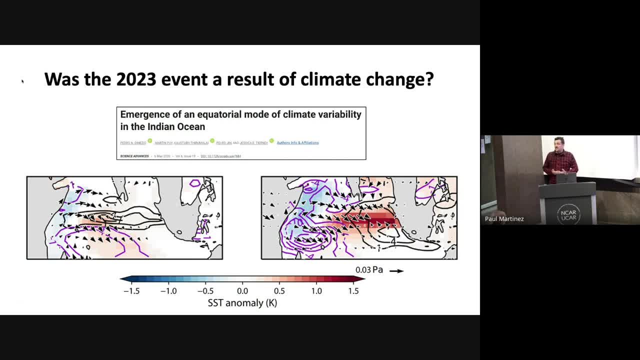 with the climatology that looked more like the Pacific with absolute easterlies. then these climate patterns started emerging in these simulations. When you start having westerly wind anomalies in the east, in the western side of the basin, it would trigger. 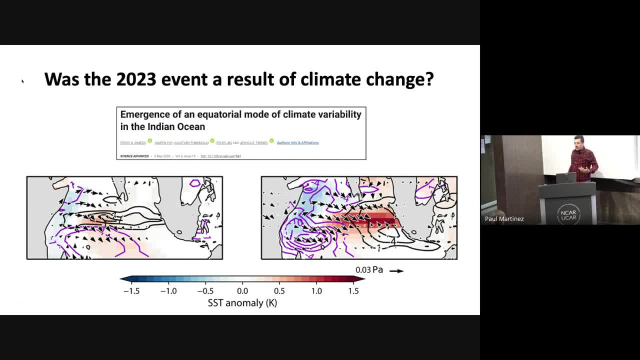 a calorie wave. These contours are anomalies in the thermal climate, the depth of the thermal climate, and a few months later those anomalies would turn into what you see on the other panel. These are composites from these very idealized simulations And we think this happened in the 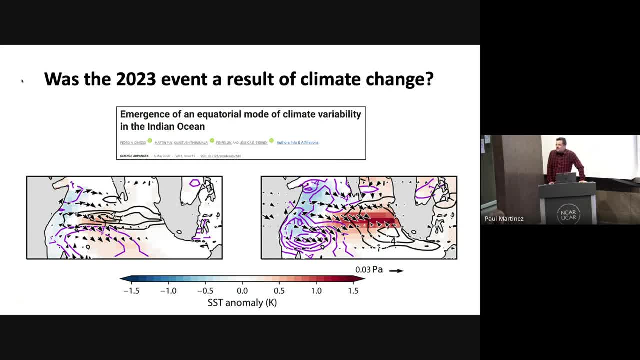 Indian Ocean during the last glacial maximum. We see evidence for this type of mode in CMEAP simulations and they're very high greenhouse gas forcing RCP 8.5.. We see some evidence of this mode but there's there's issues with the CMEAP models And that's. 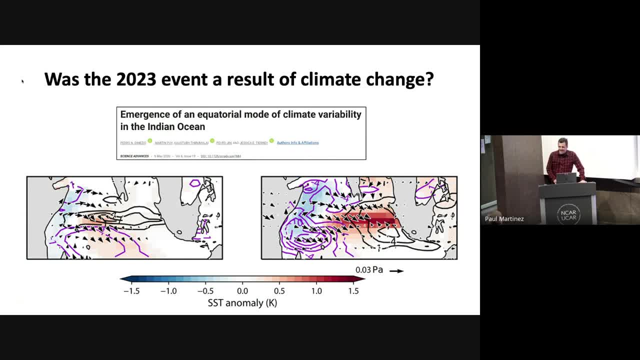 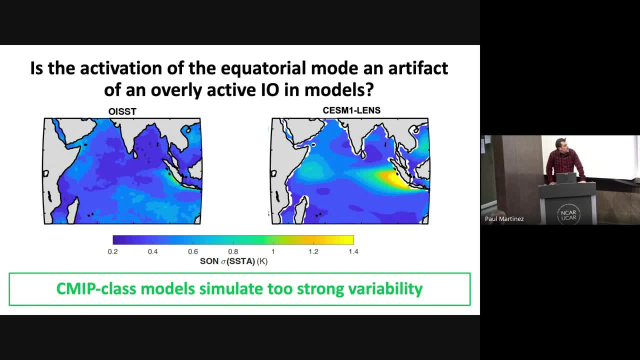 what we've always been interested in, And so we're testing this kind of mode to see if it's going to be a similar one, skeptical about this idea. And the main issue with the civic models is that they're too viable in the Indian Ocean. So that's the standard deviation of SST anomalies. 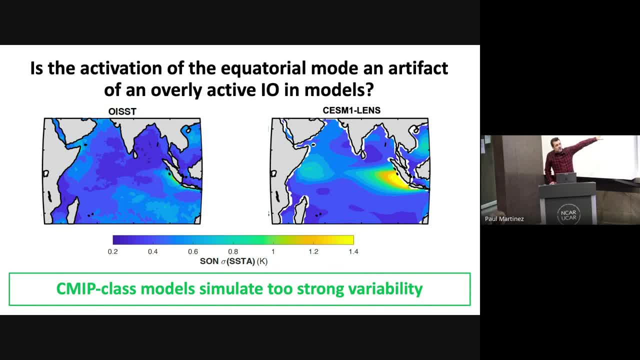 during the September-October season in this high resolution SST product And that's the same exact calculation for the CSM-1 large ensemble During the same period. the map on the right is the average of the standard deviation maps in all 40 members of the lens during the same exact. 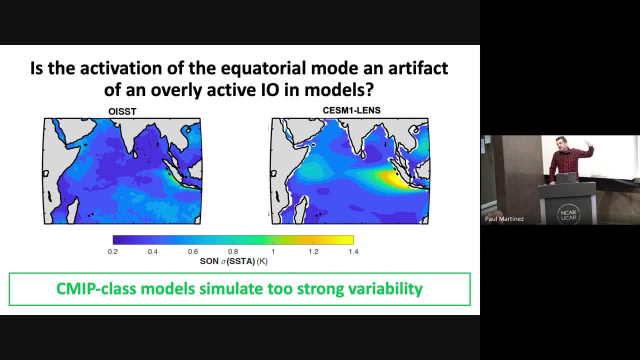 period And there's actually no member in the 40 member ensemble. that looks like this in terms of amplitude. So the lens is too viable and most civic models are too viable in the Indian Ocean. So then this has a lot of issues, because then it probably affects 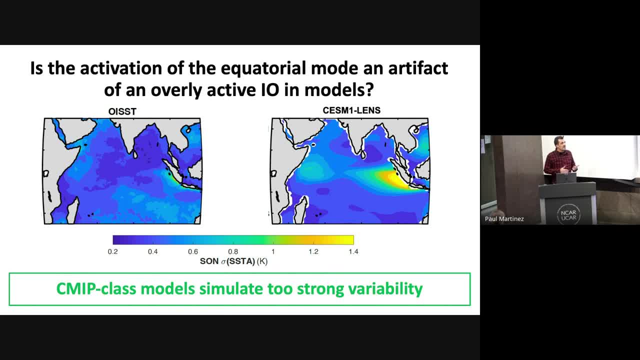 the sensitivity of this viability. The grain has forcing and it's also creating too much climate viability. So we kind of got stuck here and we spent like a bunch of years not doing anything about this problem. And then I had to write an NSF report and I was like I need to make progress on 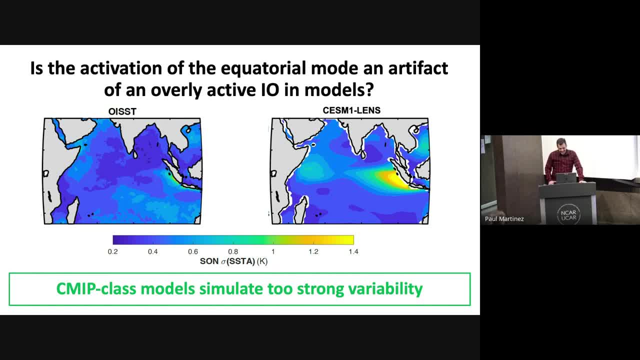 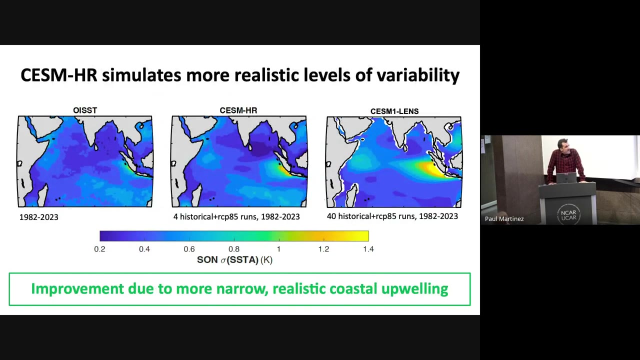 this project. So we're trying to. So that was three weeks ago And we are on the second no-cost extension. So this is. I'm sure you've been there. That's how I roll. So I've been working on the CSM-1 high resolution simulations. So it's like: okay, let me look at the. 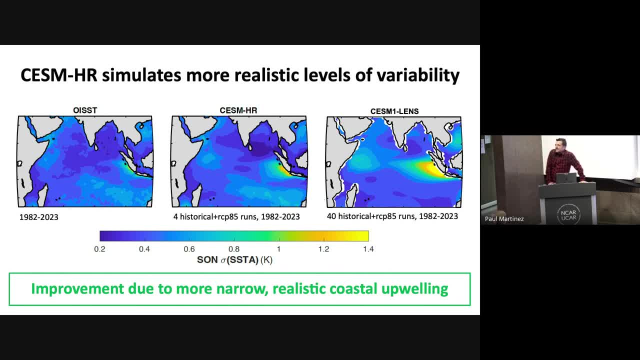 high-res model. How does the model does this viability? So then, if that is similar to realistic by everything, then we can look at what it does under climate change in the future. We don't focus on the SGM in the future And voila, We only have- actually we have three that number. 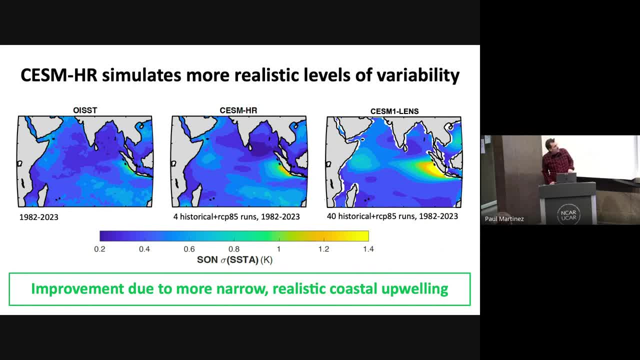 is wrong is we have three historical class RCPA 8.5 runs. there's more coming. So the exact same calculation, the standard deviation during this season And just to give you a little bit of a, you see that it's a lot closer to observed. so this is this is great news, and perhaps you're wondering. 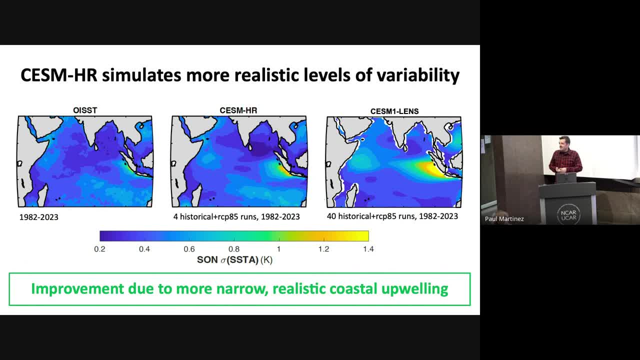 where is the improvement coming from? this is the exact same model, the exact same four things. it's just increased horizontal resolution in both the ocean and the atmosphere. the atmosphere is 25 kilometer resolution, the ocean is roughly 10 kilometer, and this improvement. there's a mixed 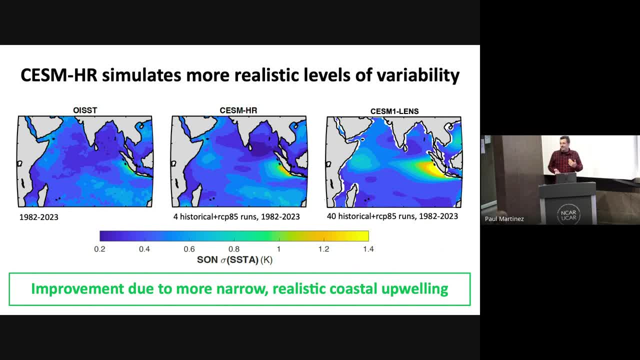 resolution ensemble too, with high resolution in the atmosphere, low resolution and that. i looked into that map and this improvement comes from the ocean. so increasing resolution in the ocean makes the simulation of the value and this is pretty new. i don't think anyone looking at these simulations. 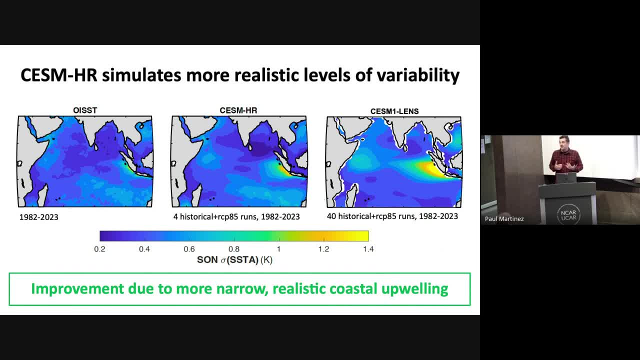 has seen this and it's perhaps due to a much more realistic simulation of coastal upwelling. all these viability is generated off the coast of sumatra by this very narrow coastal upwelling that when you have cooling, then that cooling weakens the winds. that produces more southeast. 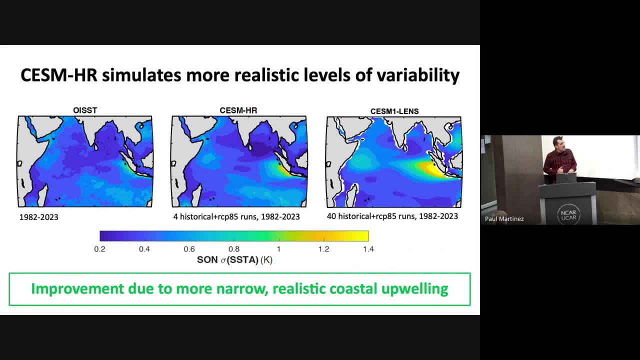 leaves abuse more welling, because those are winning favorable and there's this local feedback. but if the abueling is too broad off the coast, you're going to create a bigger patch of cooling, and perhaps that's the explanation for why the lens is so valuable. um, so you can compare the. 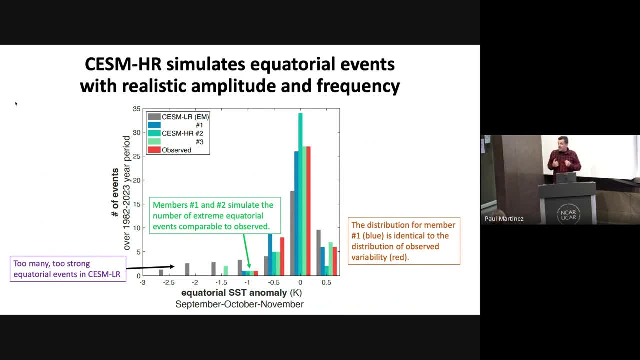 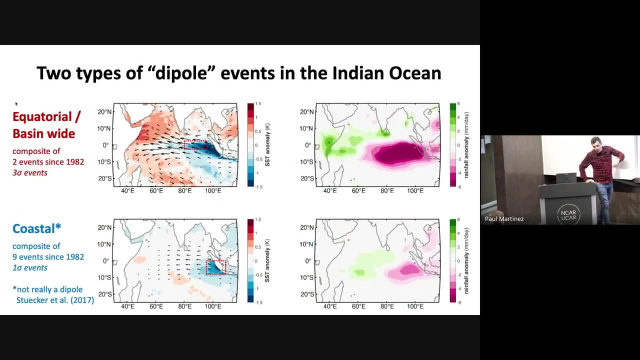 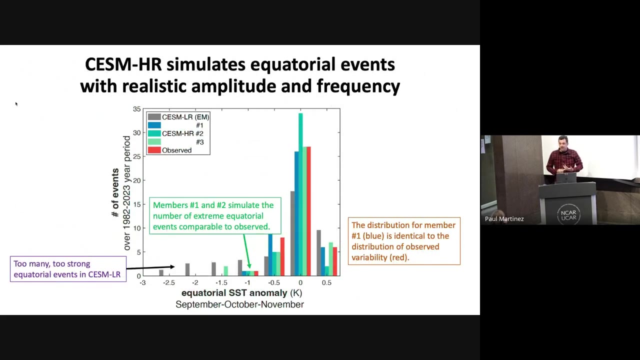 occurrence of this equatorial is really strong, very rare equatorial events and I took the values on that equatorial box that I think I showed you before the box on the top here on the equator in red and did histograms comparing the observations in red: the three high resolution runs and the 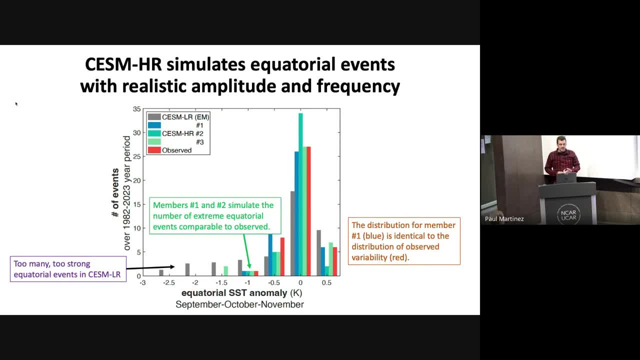 average of the distributions from the lens from the 40 members and you can see clearly what we see: the standard deviation in gray. you can see the lens extremely skewed towards this very strong cold equatorial anomalies all the way up to here: minus 2.5. that's clearly unrealistic. 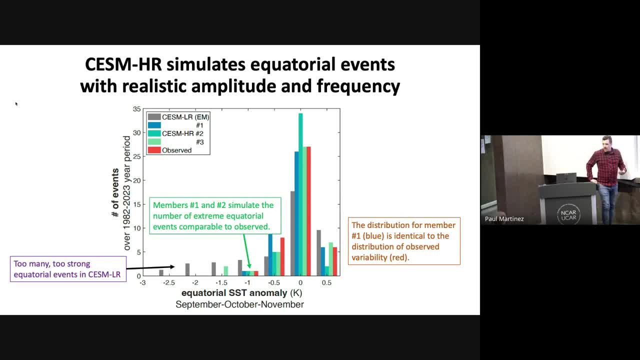 we haven't observed any event that cold and this red, this little bar here. the red bar is the 1997 event and last year's event in this is in this red line and if you look at the greenish, bluish bars they're a lot closer to the observations in the distribution of the sst. 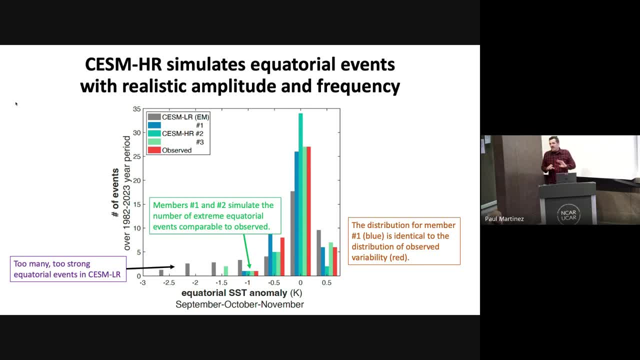 anomalies. in this box there's even one member that looks almost exactly like the observations and there's no member in the large ensemble with a low rest national sample that looks and what we observe. so there's a clear improvement in the model in how it simulates the viability much quicker. so now we can see well the variety is not. 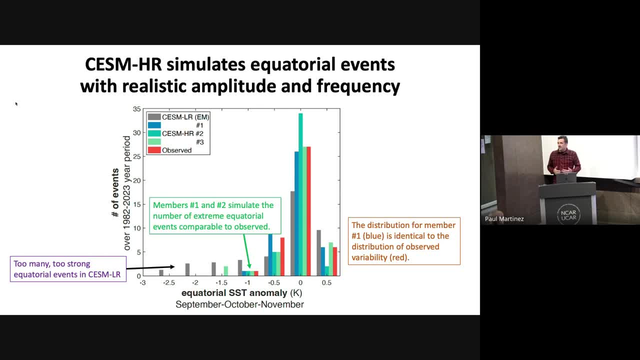 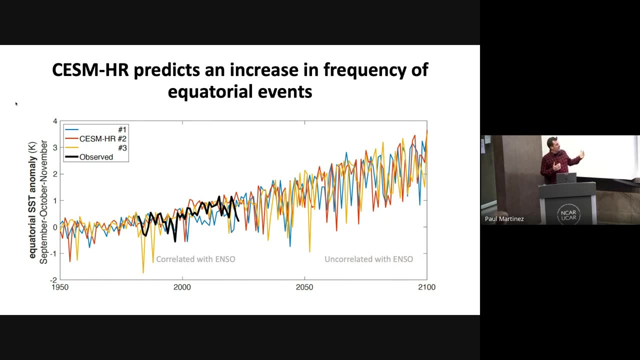 over exaggerated. we can see what it does. as greenhouse gas gases increase and they affect the mean state of the indian ocean, the variability could change. this is my last slide showing that, so now plotting it's actually very simple curve. I'm not. you can see that index on the. 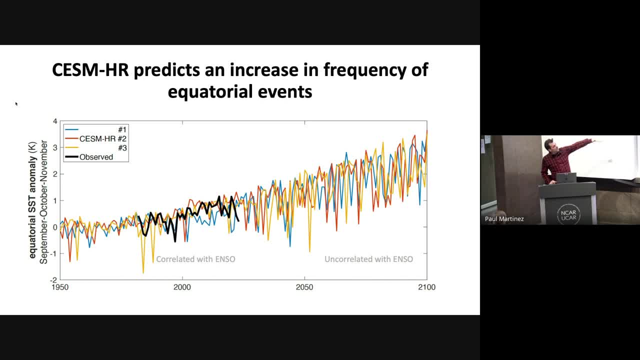 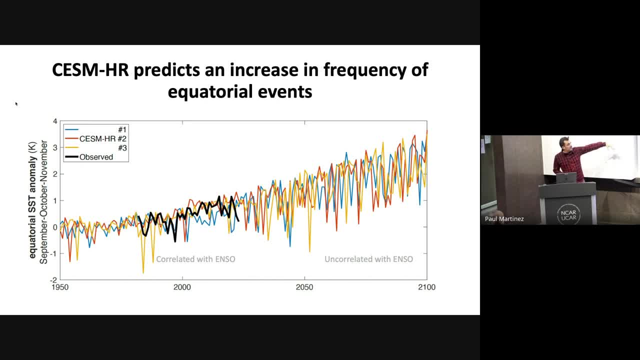 and you can see that these really strong cooling events are pretty rare during the historical period. perhaps they're a little too strong in this yellow run, but some of one of the runs that the the blue one is- really has as many extreme events as observed and then as you go forward in time these events become like a lot more frequent. 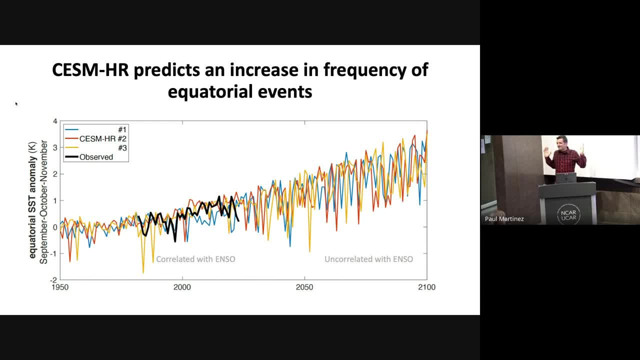 you can. you don't have to do any statistics here, so it's just fraud at the time. I don't think I need to convince you that everything goes up by a lot and they sort of have this event start happening a lot more often in today's climate. they have been correlated with a linear, like last year. 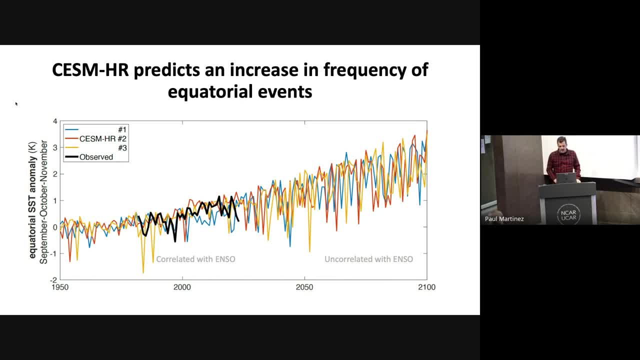 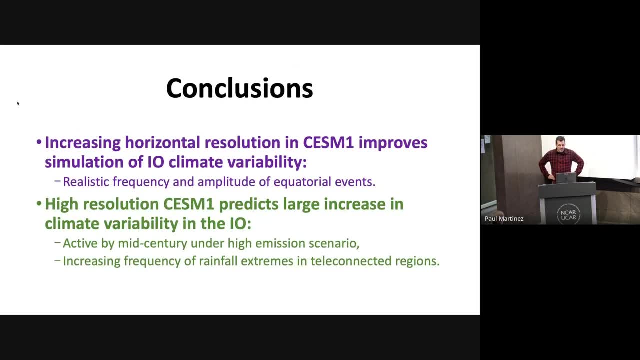 when we go into the future, they start happening on their own, and so you can ask me about the mechanisms after my conclusions perhaps. and so the increase increasing horizontal resolution, mainly in the ocean, improves the simulation of indian ocean climate viability in CSM with a lot more realistic frequency. an amplitude of this very 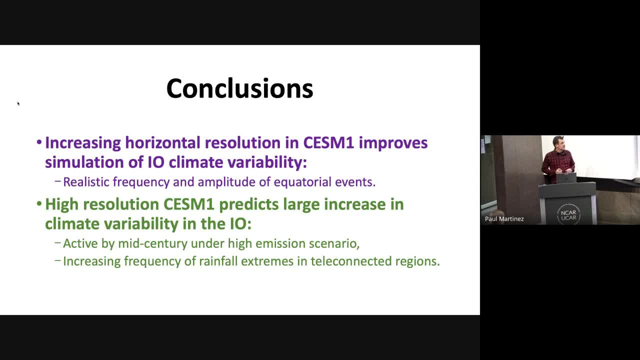 uh, very impactful equatorial events. um, and when we look at the changes into the future, these events become a lot more frequent under high emission scenarios perhaps, I don't know the answer- for medium range emission scenarios, uh, and so you can imagine an increasing frequency of rainfall extremes in teleconnected regions. 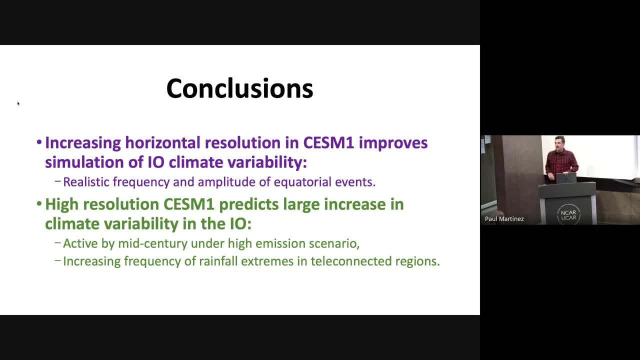 within the indian ocean but also in the southern hemisphere. a lot of the teleconnections, these, these viability in tropical rainfall in the indian ocean correction drives massive teleconnections to the southern hemisphere, australia or even west antarctica and all the way to south america. so with that I'll stop and take any questions. 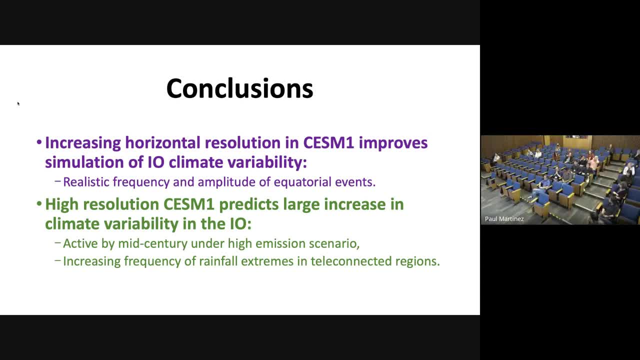 questions. it was really interesting to see that, in contrast to the eastern pacific, that where the warm events become more extreme, in the indian ocean the cold events become more extreme, and I guess that's the mean state change. the indian ocean is just, you know, if it's 32 degrees it can't. 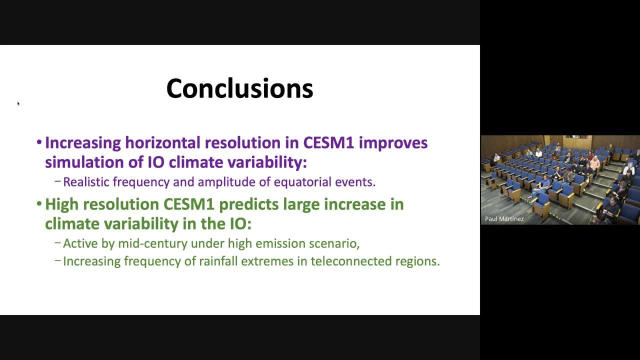 be any more than that. yeah, it can be a lot colder. thanks for that question. uh, yeah, the indian ocean- right recall it's like a bathtub today. it's just unique, almost uniform warm. well, what greenhouse gas do to the climatology? and it's make the eastern side warm less, so it creates room for more. 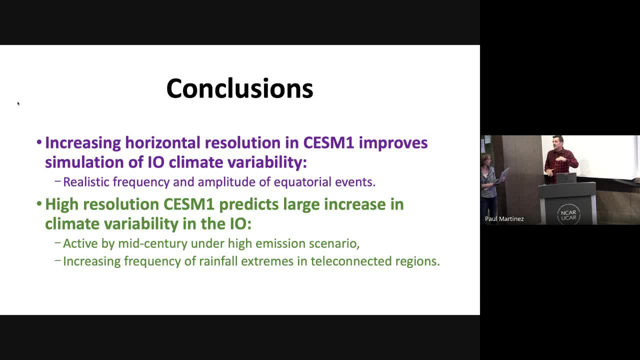 viability, if you think in terms of amplitude. and it also changes the direction of the winds from weakly westerly to weekly easterly, so then the mean climate stops having upwelling and earthy directions can happen more more easily along the equatorial linear ocean, so warm events also start. 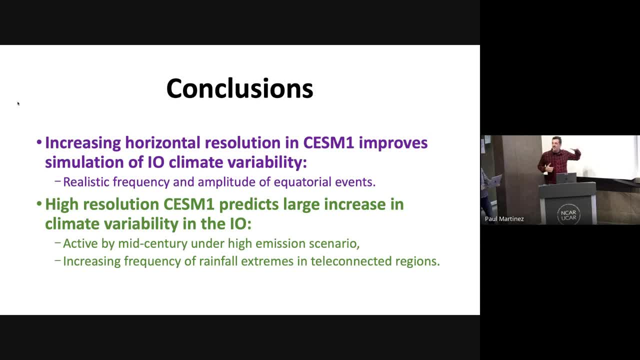 happening actually in the time series. if you, I should have drawn the median to see that also the warm anomalies become more frequent, not as intense, but it's both become. but you always have the cut of the tropical winter that will limit how big these anomalies can be. I was wondering if there's implications for 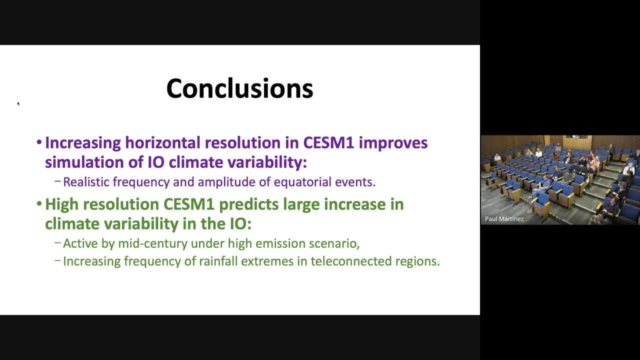 fisheries along Sumatra there, in an analogy with Ecuador and Peru? Perhaps I have no idea. Yeah, but yeah, these are huge changes. Thanks for the question. Yeah, I have a question. So you invoked improved representation of upwelling, but I'm wondering if you think that maybe Indonesian through flow could also be. 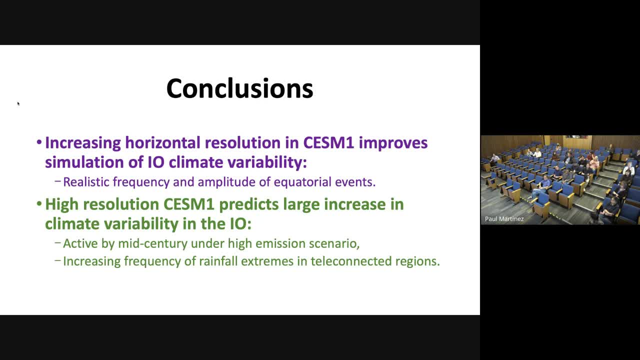 playing a role which is certainly better. Yeah, perhaps, And I've thought about it and again, maybe that's two weeks ago, So yeah, and perhaps even there's the effects on the mean winds during this season, because the models tend to simulate this season, like semi-models, low-res models, simulate. 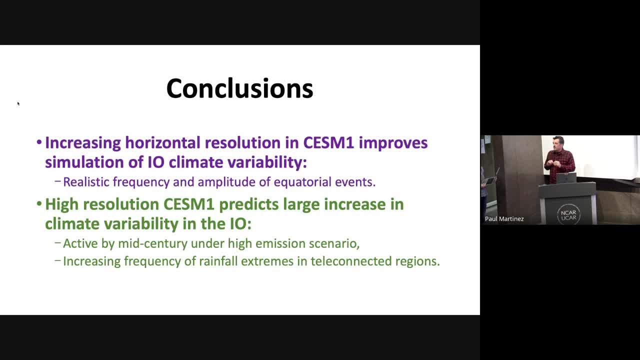 this season. well, The winds are not clearly westerly as they are in nature, So that's why, also biologically, It's a little too strong. It's easier to make the winds more easterly because you're starting from a state that is numb. So it might not be that simple, but I think the first guess- 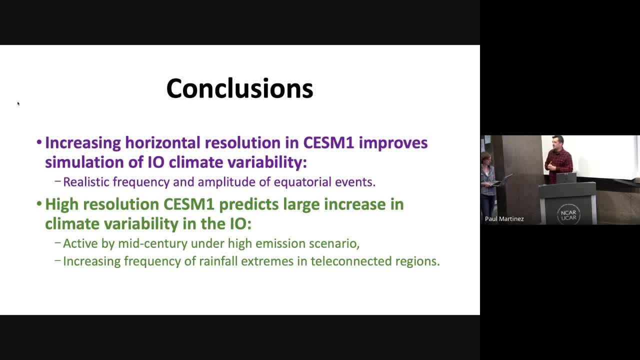 is upwelling And, yeah, nobody's looking at its through flow in these high-res runs And I think there might be really exciting surprises there. Yeah, I'm going to change the slides, but there is a question online as well. 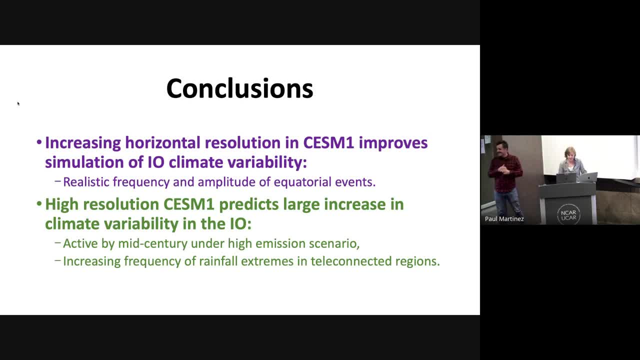 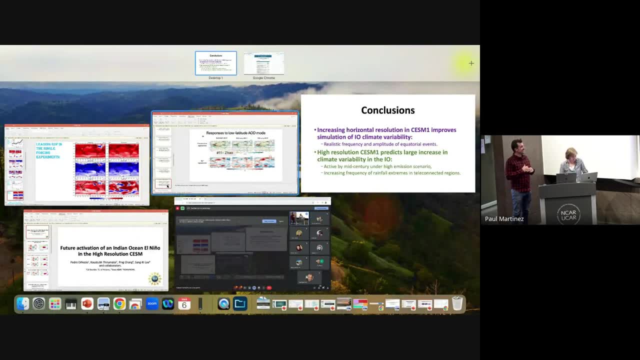 Oh, We have time. Yeah, while we're doing this, he's asking if there's what are the kind of broader impact more generally of this variability of our? Yeah, It's a good question how the I peeked into what it does to rainfall. 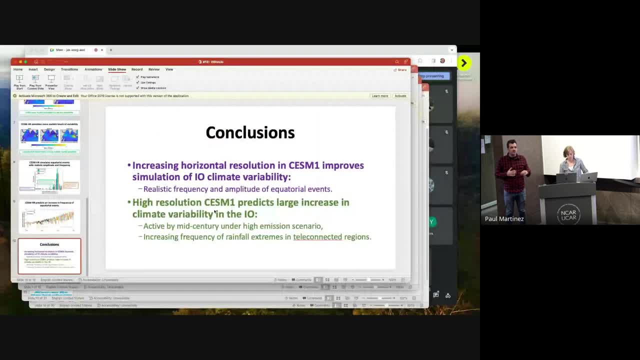 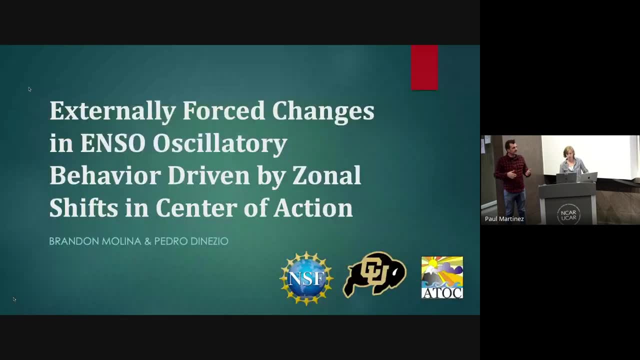 but I think again, the Indian Ocean is a place where models predict large increases in rainfall extremes through thermodynamics changes in the mean state. So this could be another source of extremes through the SST variability. That's someone, that's something someone should look into. 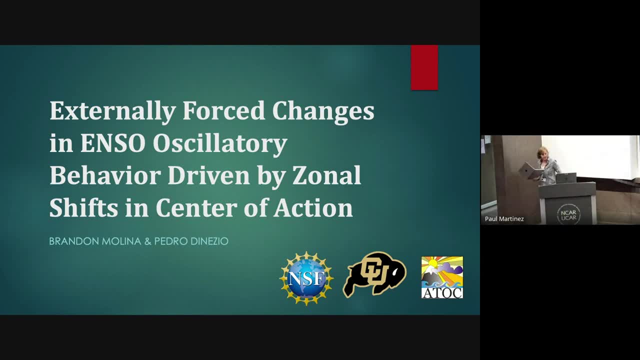 All right, Thank you. Now we have Brad and Melina on externally forced changes in the hemisphere: All right, Okay, All right. All right, Let me try holding at the screen and then moving it over. Perfect, Okay, All right. 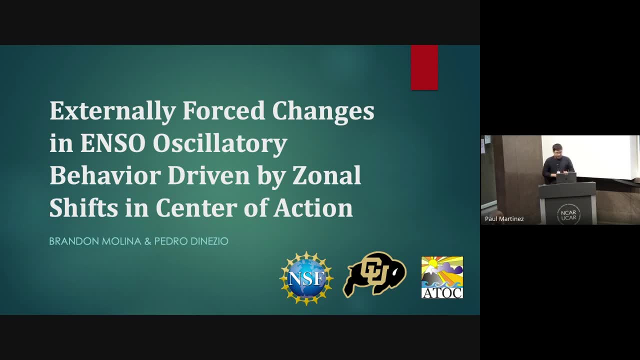 Well, hello everyone. Today I'm going to present some results from my first project that I'm working on in my PhD. I'm a third-year student at CU and I'm working with Pedro Donetsu on this, And this project could not have been done without his immense help. 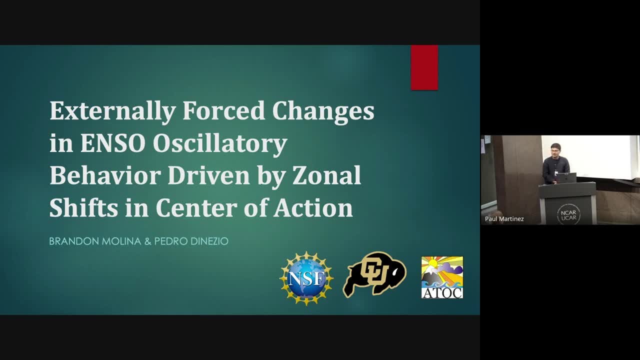 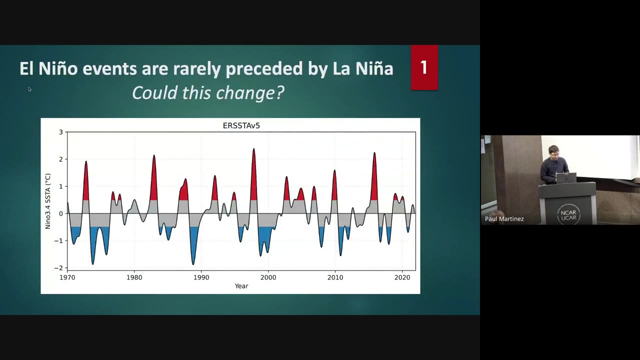 I also have meaningful contribution from Clara Desser in this project, And I'm very excited to share some of these results. So today I'll be presenting on how answers to solitary behavior could be changing under external forcing on the climate, And so we first want to see how the time series of the Nino 3.4 index looks like in our current 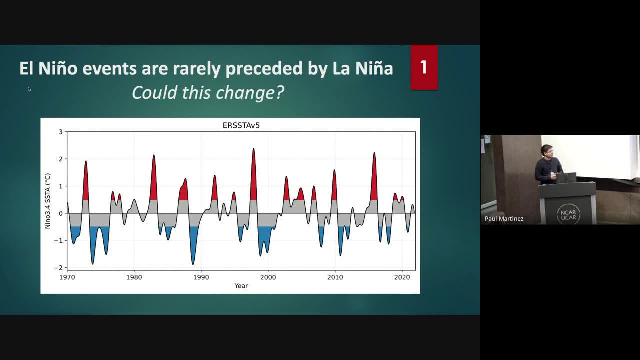 climate. And so we can see that from since 1970, we've had this feature of ENSO, which has an asymmetric temporal evolution between El Niño to La Niña and then La Niña back to El Niño. 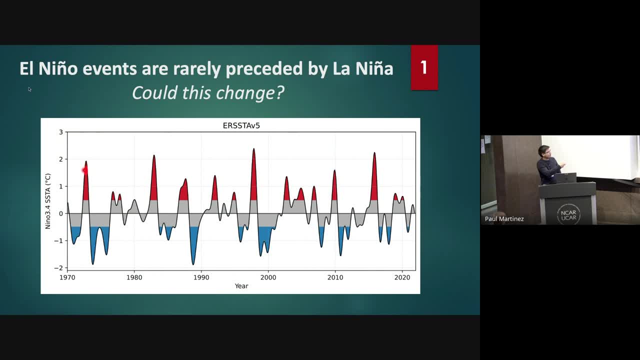 And so we can see is that since 1970, there's a rapid transition between the strong El Niños, and then we have a longer duration between La Niña into returning to El Niño, And so that asymmetric feature of ENSO has made it difficult to really forecast when the onset. 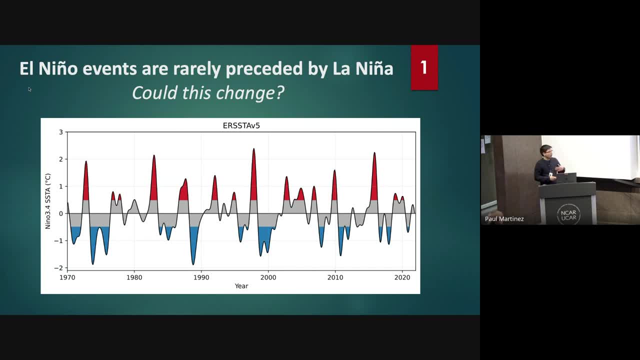 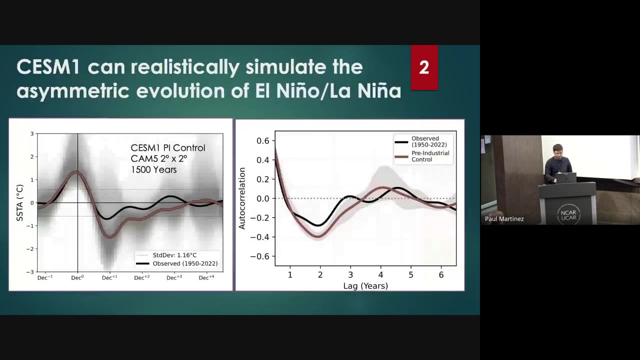 of an El Niño will come, which is different from the predictability of a La Niña event, And so what I'm going to be studying in this project is: how could this feature of ENSO potentially change under external forcing? And so first I want to look at a model that can actually realistically simulate that. 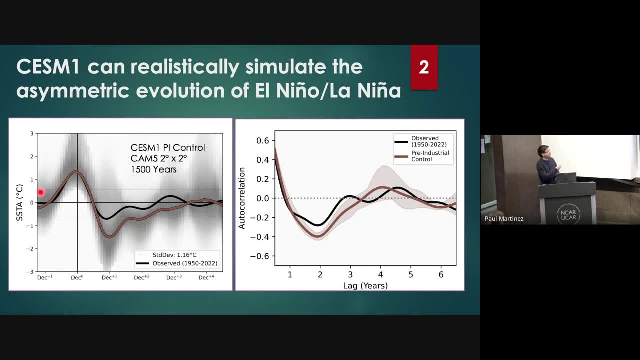 So, in order to simulate that asymmetric behavior, and so here I have created a composite of events for the observations, with 1500 years of pre-industrial control from CSM 1.. And even though the observed observations of an El Niño event are limited to, 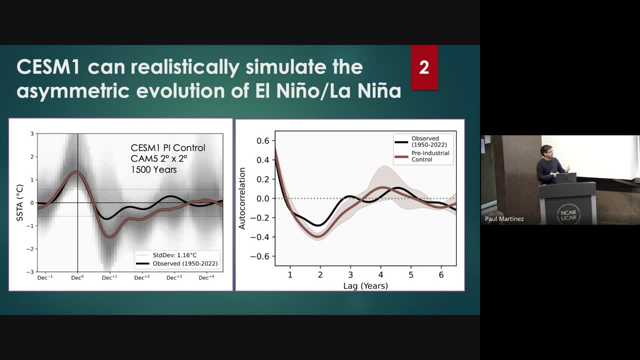 you know only the 1950s. I can still see some features that are being simulated by CSM 1.. And so I'm just going to start by If you had an example please. Hey, I'm a consumer of some factory, Marte. 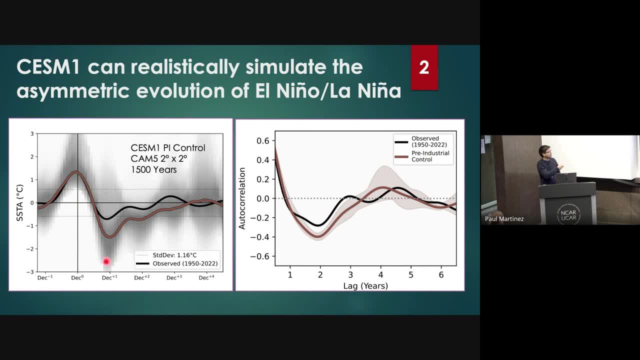 And I'm just going to start by: Well, we have a pancake in the middle right here of an El Niño event, And this is the CA model, which is essentially just the left. And those are, this rapid transition from El Niño to La Niña. 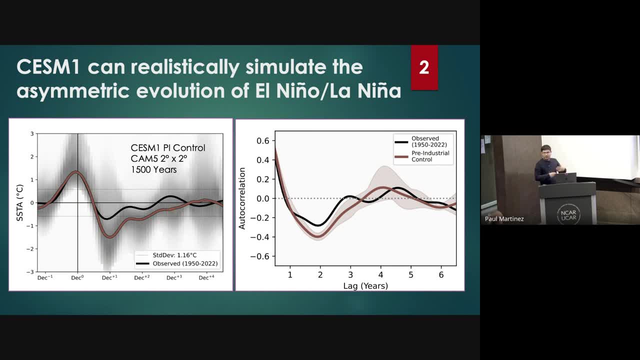 and then that longer duration of La Niña and then just stays in neutral after that. Looking also at the autocorrelation function, we can see this more clearly without any biases on how I choose the threshold of an El Niño event, And I can still see those asymmetric features. 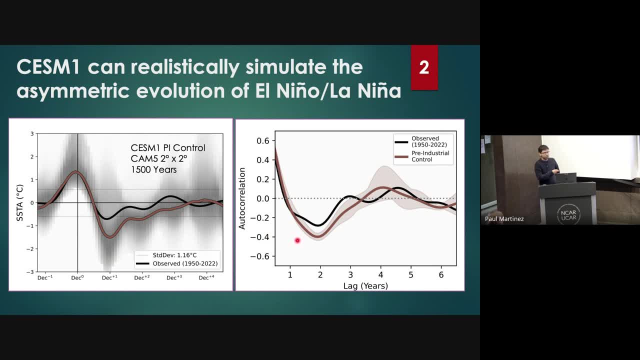 especially in the strong negative correlation at a lag of about two years. So that represents that consistent transition from El Niño to La Niña And then, after any other lag, that correlation becomes severe and weak, which represents that lack of consistent transitions from La Niña back into El Niño. 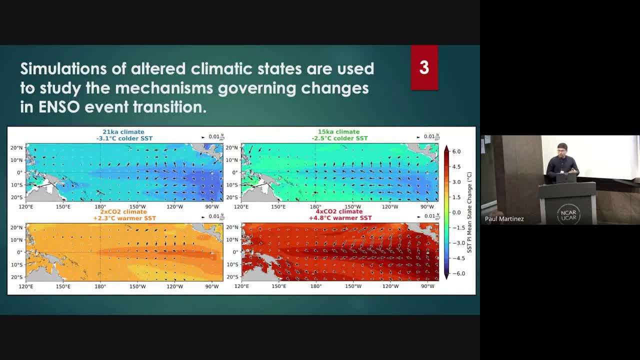 And so now that I know this model is fairly good at representing these asymmetric evolution, I can look at other climates in this CSM1 and see how the oscillatory behavior can change. And so here I have plotted the tropical Pacific mean state changes of SST. 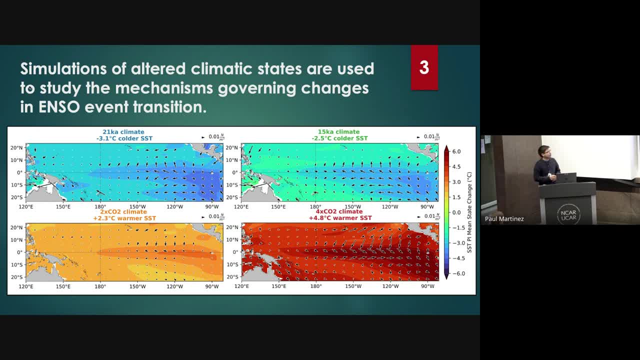 and the winds and the wind stress. And one thing I noticed is that, under these colder climates from when we had glacial glaciers, it produces an equatorial enhancement, an enhancement of cooling, as well as a strengthening of the trade winds, And then, conversely, 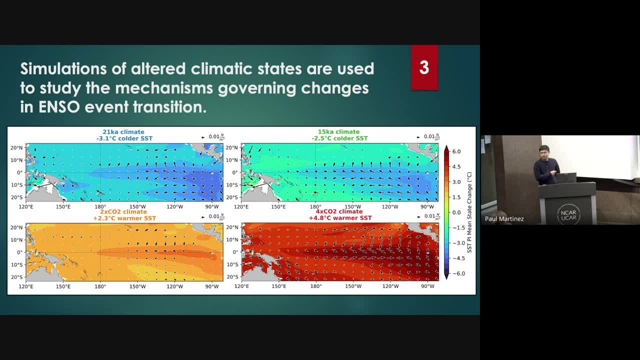 if we look at climates with increased levels of CO2, this global warming scenario shows an enhancement of the equatorial warming as well as weakening of the trade winds, And so just looking at these mean state changes of the tropical Pacific, it gives me a clue at 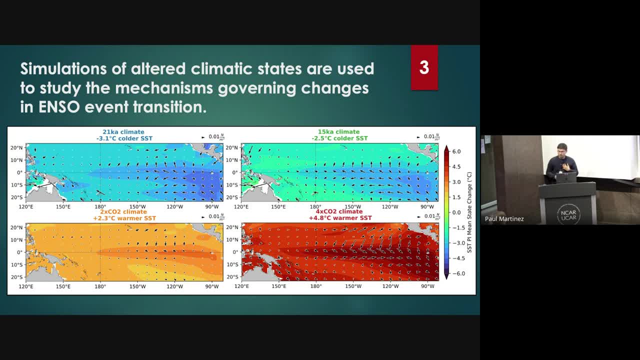 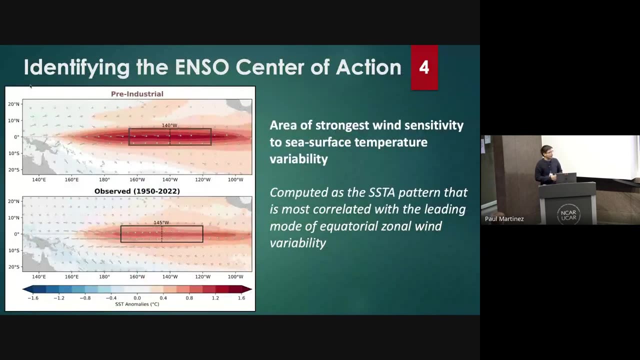 as or an indication to me that there's must be some shifts in where the air-sea coupling might be, which is involved in the dynamics of ENSO, And so a better way to find or identify where that air-sea coupling. 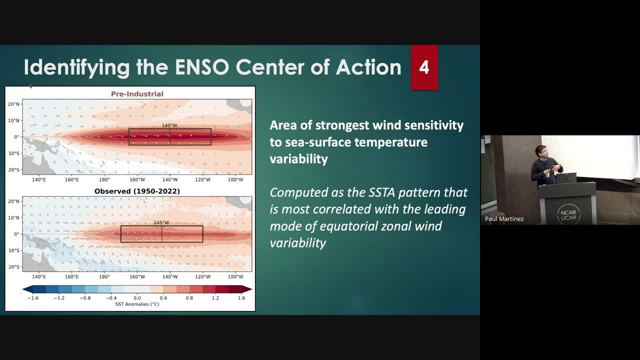 is strongest is to identify a center of action, And so so far, in our current climate, been using the NEO 3.4 region, which is from 170 west to 120 west- and this represents the area where SST anomalies produce the greatest variability in the winds- and using this method. 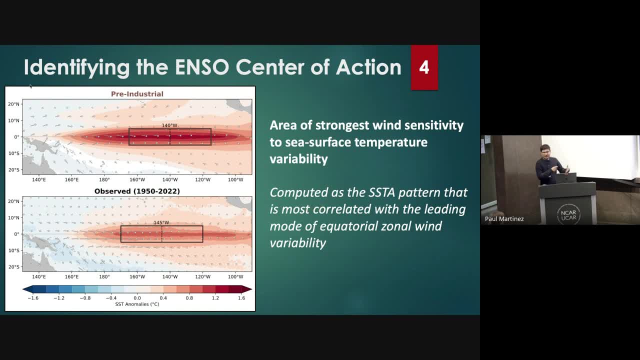 of EOF analysis. by computing the where the SST pattern is correlated with the leading mode of equatorial zonal wind stress, I see that for the observations I get almost perfectly that area. so I find exactly where the peak of Arlongui equator happens. and then I just 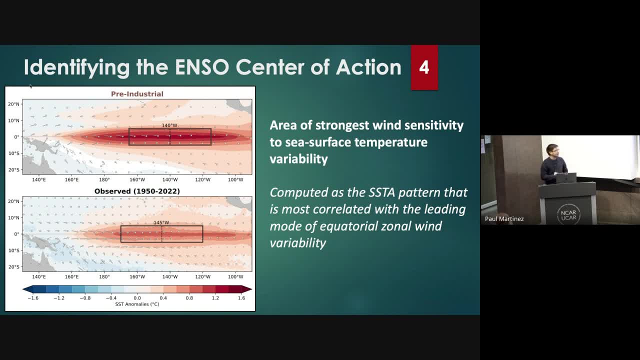 make my box 25 degrees to the east and west of that line and I do the same thing for the pre-industrial control from CSM1 and I can see that box region is fairly similar to observation. so that's pretty good. The only difference is there's a slight bias to the wind stress. 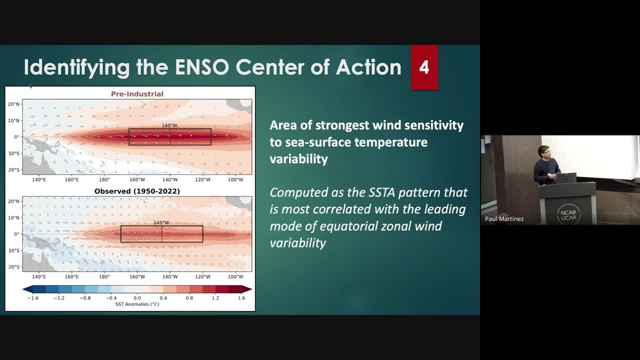 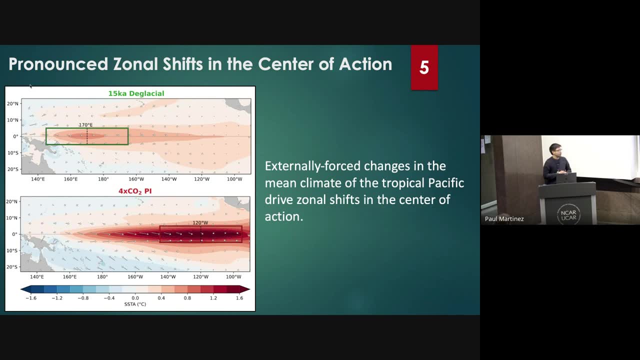 towards a slightly higher magnitude of correlation. But now, if I look at what this looks like for the two different climates- and so here I've just shown the ones- that the climate- the colder climate- that shows the greatest changes in the warmer climate that also shows the greatest changes. 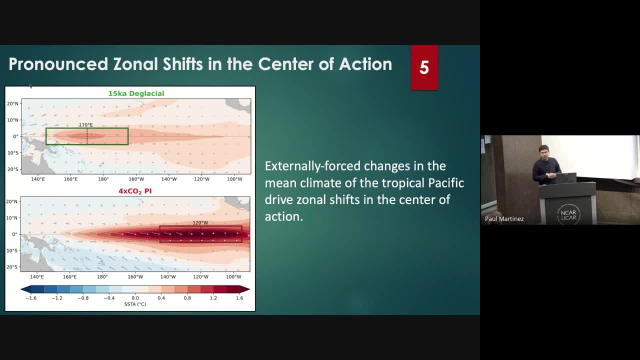 and so this would be the 15,000 years ago. the glacial climate shows a substantial, pronounced zonal shift of that zonal shift. So this is the center of action towards the west and then in the warmer climates we have, we see that that 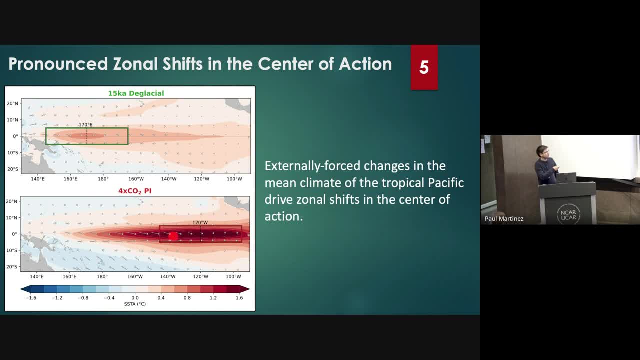 zonal shift is towards the eastern basin of the Pacific. So that tells me that the external forces, changes of the mean climate- is actually driving these, these recent trends. But what I want to know is: how do these zonal shifts of the center of action affect the oscillatory behavior of ENSO? 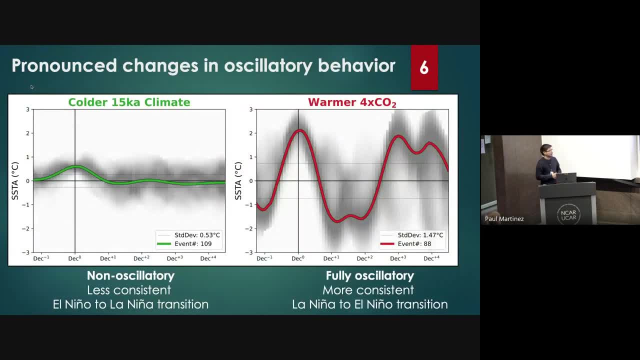 Now, looking back into this composites for these climates, we can see that for these colder climates, ENSO becomes completely non-oscillatory because the transitions from El Niño to La Nina become less consistent. and then, for these warmer climates, we can see that ENSO becomes. 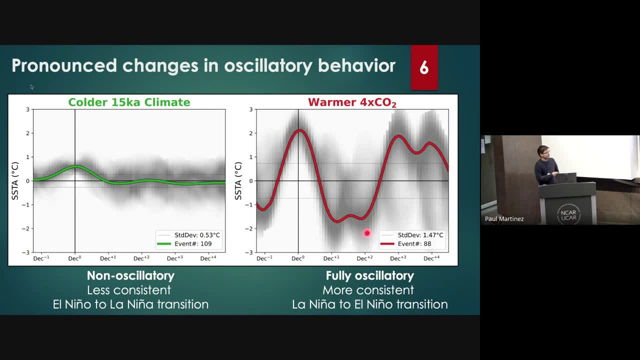 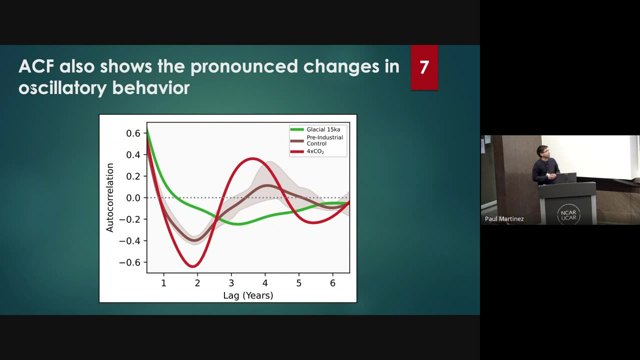 much more oscillatory than it is today, because that transition from El Niño, from La Nina to El Nino starts happening more consistently, and so that's a very pronounced change in the siloed behavior between these two climates. Looking also at the autocorrelation function, we see that those pronounced 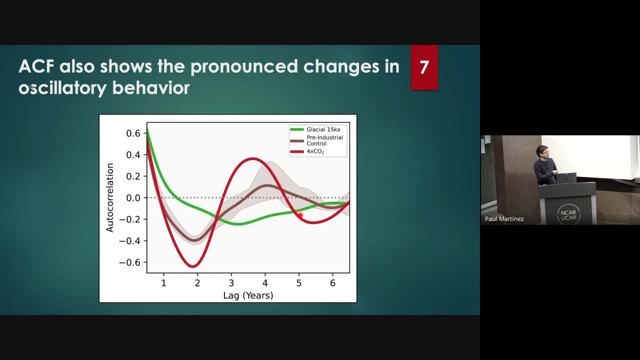 changes are very clear. We see for the warmer climate, at a lag around three and a half years, that there's a very strong positive correlation as opposed to the industrial, and then for the colder climates there's no real strong correlation at the lag around two years where we see that consistent transition. 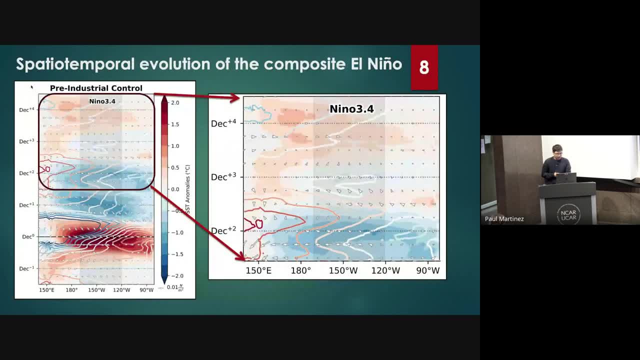 from El Nino to La Nina. But we ultimately want to understand what's really causing these changes in oscillatory behavior, and so we must look at how the thermocline variations, actually how it effective the thermocline variations are and actually kicking off the next. 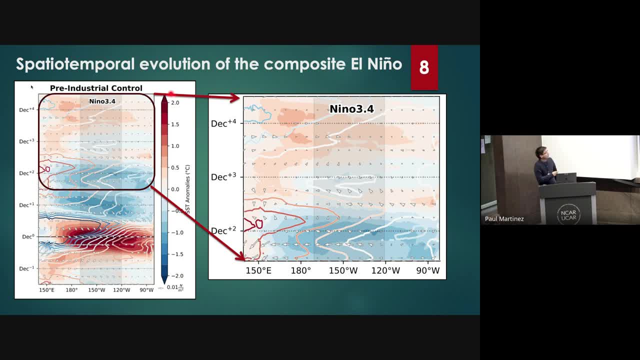 events. And so if we look at these Hopmuller plots with the longitude at the x-axis and then time going up, we see at the peak of El Nino for our pre-industrial control- that this produces a delayed thermocline response that then travels back. 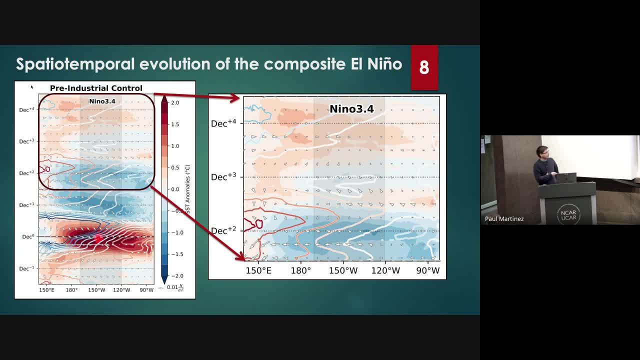 as a shoaling of the thermocline, and so this brings a cooling of the surface layer, and this is what ultimately transitions El Nino into La Nina, because the cooling tendency of the thermocline is able to cool the surface in within the region that the air-sea coupling is strongest, and that would be the El Nino 3.4. 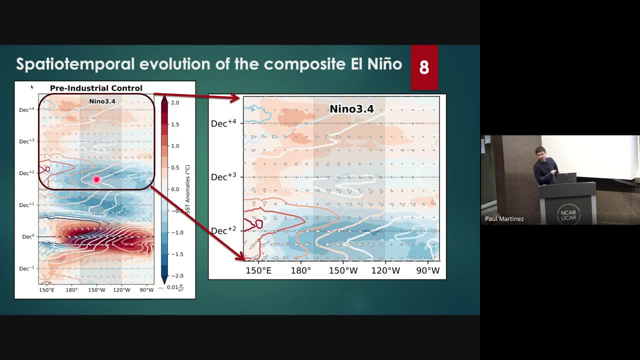 region. However, if we look closer at what happens during the El Nino event, we can see that the associated delayed thermocline response, that is, deeper thermoclines, brings a warming tendency to the upper ocean, but that only happens in the Far East Tern Basin, which is outside of the 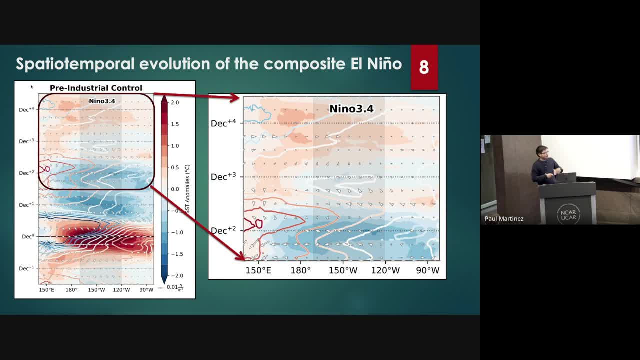 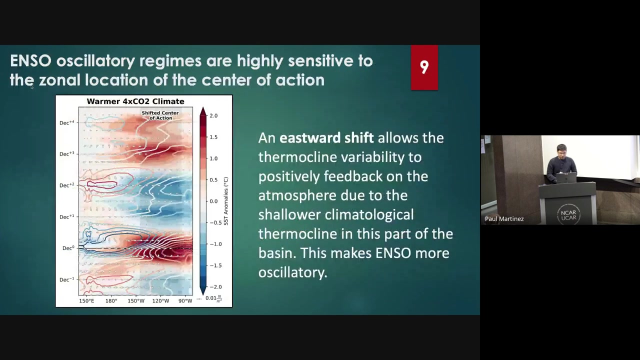 El Nino 3.4 region, and so in that region only the thermocline is coupled with the SSDs, but the SSDs are not coupled with the atmosphere. Therefore those slight warming you see doesn't keep growing because the that region is too cold to actually produce any convection in the atmosphere. But now 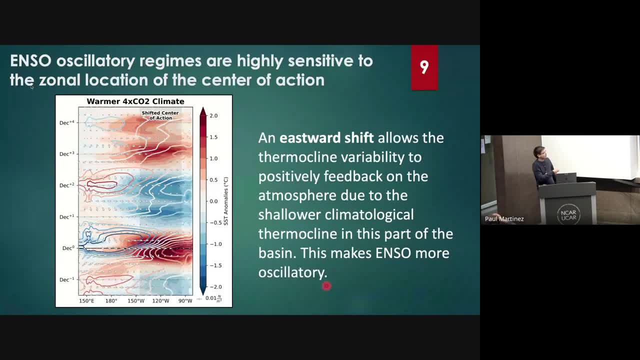 if we look at what happens in a warmer climate, we see a similar pattern after El Nino. but then what's more interesting is what happens after La Nina is that those warming tendency from the thermocline actually produces those warming anomalies within that new shifted region of center of action. 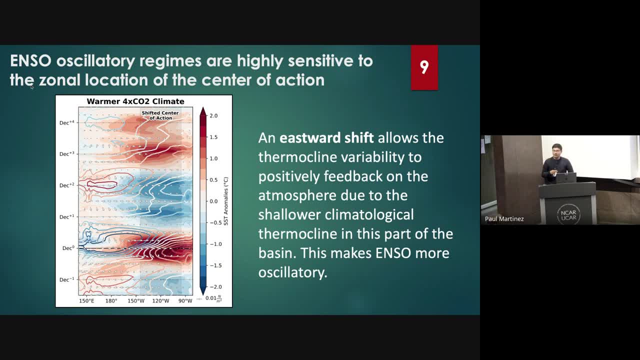 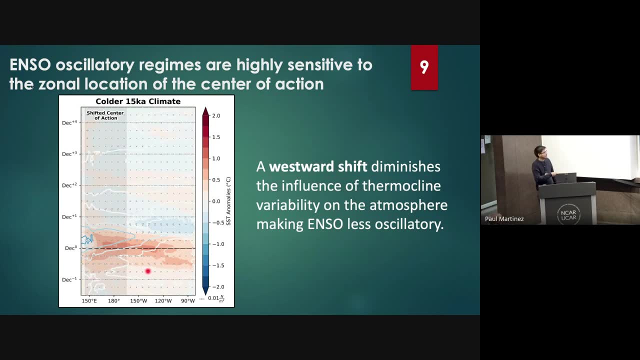 Therefore, those anomalies can actually be coupled with the atmosphere and can keep growing into a fully fledged El Nino. And then, lastly, looking at the colder climates, we see quite the opposite, that our far western center of action has these shoaling of thermoclines that 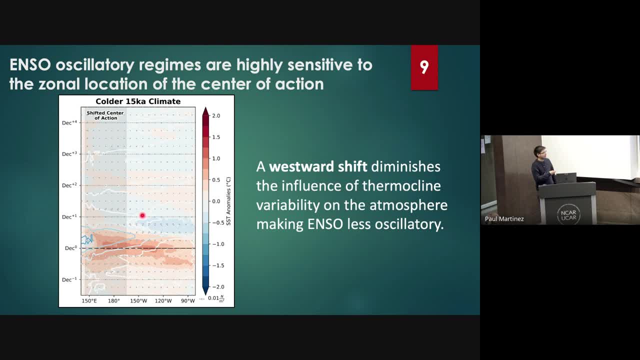 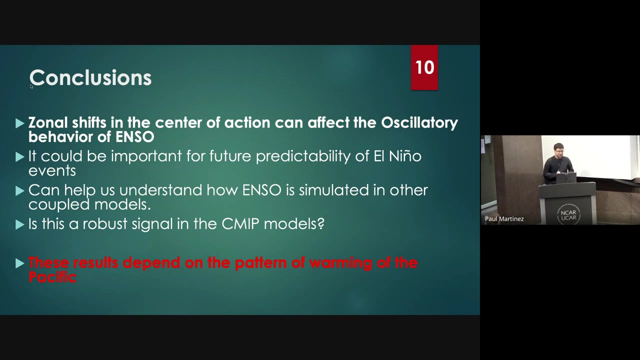 produces shoal cooling only still in the eastern Pacific. but that's way outside of the region where the SSDs are coupled with the air and therefore we don't see any signal of El Nino yet. So, in conclusion, I expect I see that in my 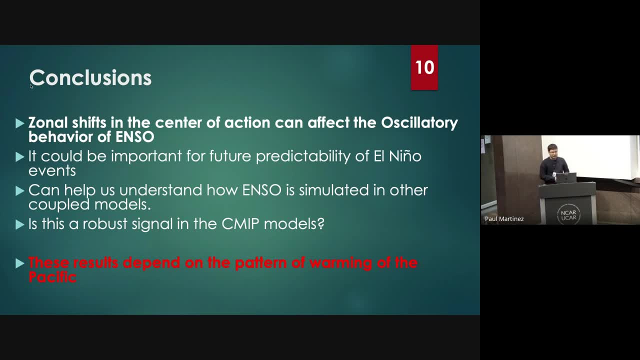 analysis that these zonal shifts in the center of action can affect the oscillatory behavior of ENSO, and this could be very important for future predictability of El Nino events, as if ENSO becomes more oscillatory, then the onset of El Nino will become more predictable, just like La Nina is today. 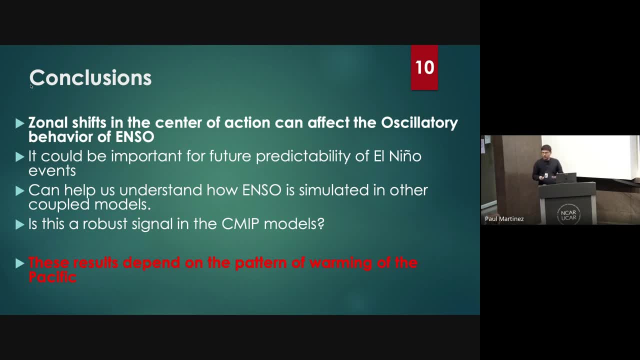 These results can also help us understand how ENSO is simulated in other coupled models, and so I would also like to understand how this signal is, if it's robust, in other synod models, and so so far I've only done it for CSM1, and so 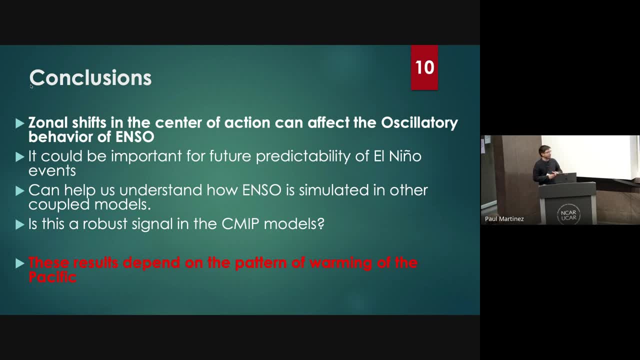 something that I really want to keep working with. this is just trying to find if this is a robust signal, But ultimately these results really depend on the pattern of warming of the Pacific that I showcase in the mean state changes and, as we all know, so far CSM1 has been. 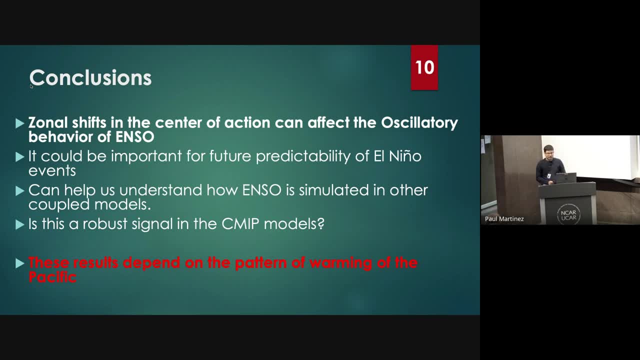 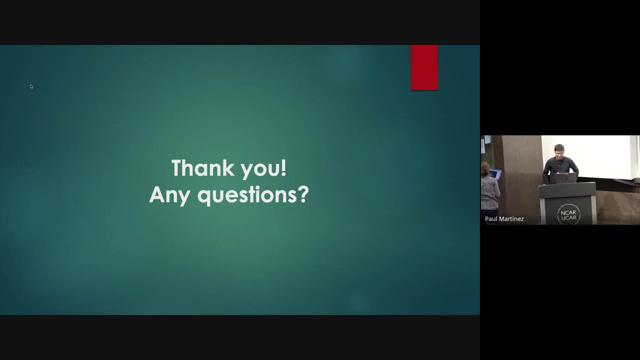 a little on the bias of being warmer than what we see happening in observations, But it's still very insightful results, I think. Yeah, thank you, Any questions? I had a question. You focus on coming back to El Nino, but it seemed like you had a double El Nino. 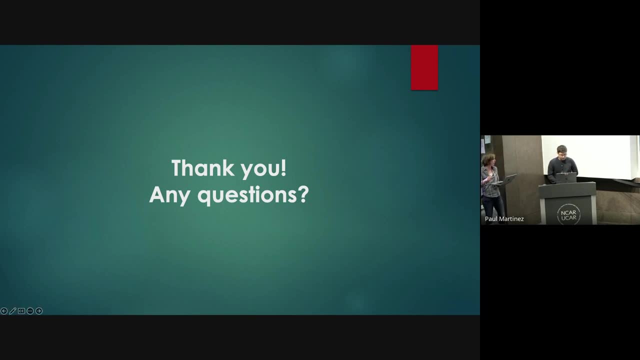 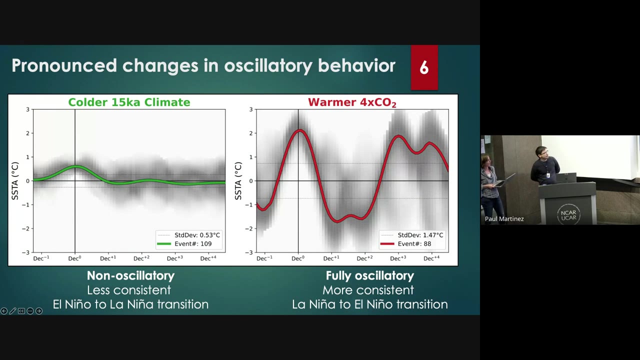 Do you think that's that really happened in individual ever answers It kind of you're averaging different events that end up in the net. Yeah, do you mean like a double capture there? Yeah, My, I made a. so the shading represents all the events that I've made the composite of. 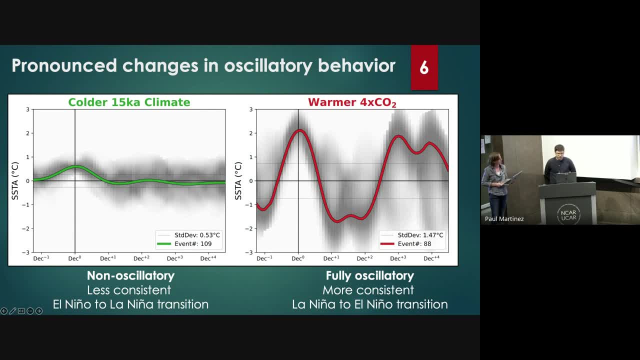 and yeah, it really is just the events that get composited together that produce a two year old. It's very interesting. actually, I have not had a chance to look into it. I'll visit the ones that give you the El Nino in the first year and see whether those also. 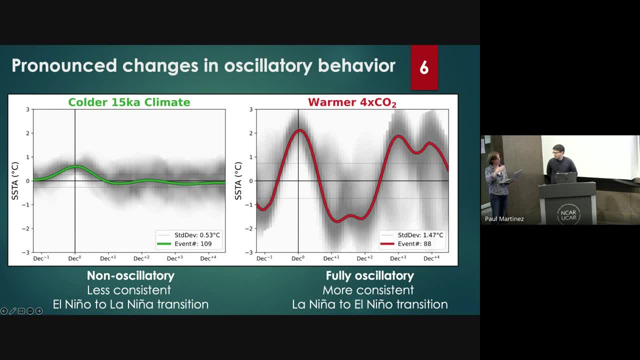 give you the second, as opposed to it being ones that just don't give you the El Nino until the year plus four. Right, right, right, yeah. Any other questions? I'll have a very naive one, because I don't have any clue about ENSO. 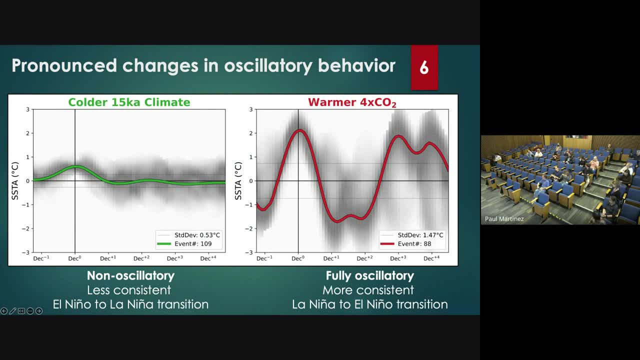 You always talked about the center of action, where the ocean is coupled to the air much more than outside of the center of action and without having any idea what this role, what role of the center of action is. I mean, it seemed like this coupling does not depend on the absolute temperature of SST. 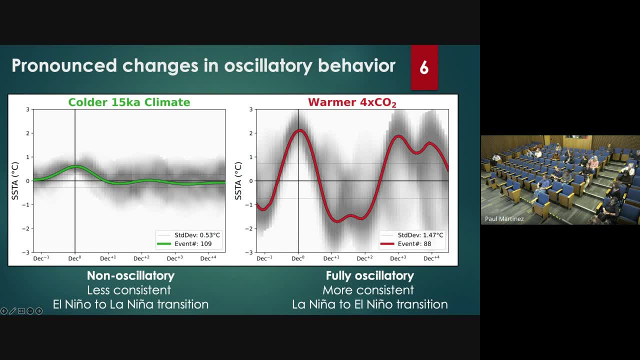 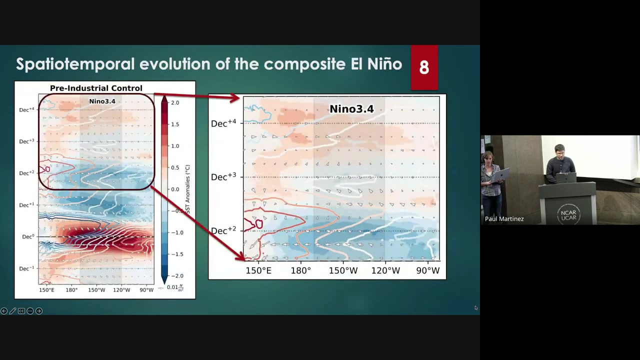 So maybe you could give me a hint how to understand this Better. So what do you mean by the absolute temperature? I saw that outside of the center of action sometimes you can have quite extreme anomalies, but still it's not defined as the center of action. So what like oh? 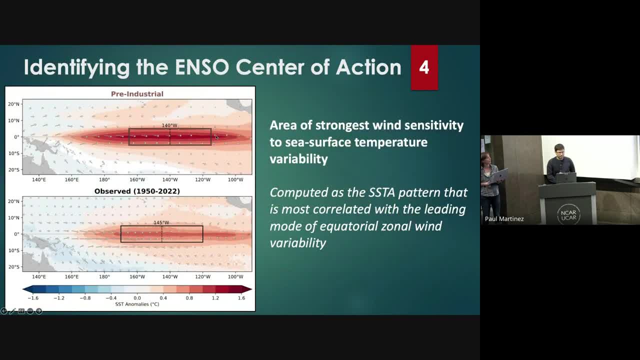 this part right here, right, For example: yeah, So how should I understand that there is? there is for sure, less, but why is there negligible for your theory? That's a very good question. I'm not sure how to respond to that, but that's a very good question. Is it because it matters how warm it is relative to the rest of the tropics and the extent to which that is changing? Yeah, it's. I mean, the eastern pacific is so cold that you can warm it, but the atmosphere will. 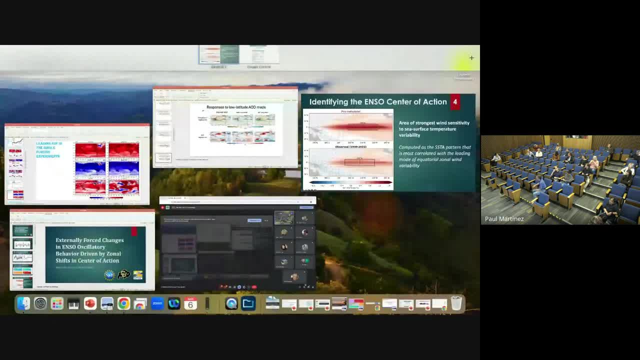 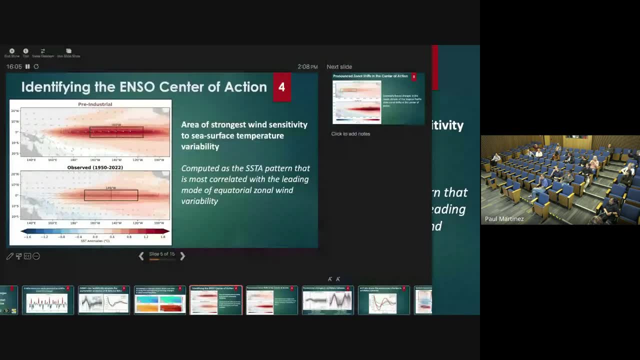 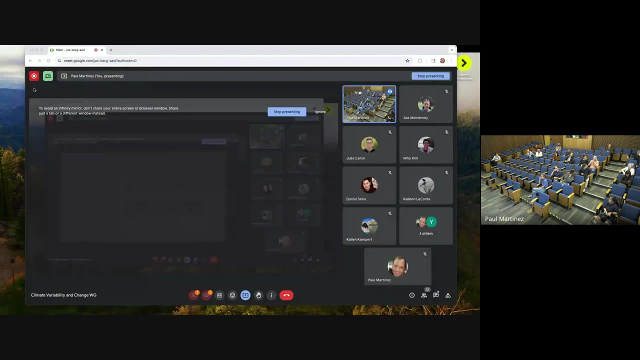 never know. So that's why you have those big the SST anomalies can be there, but but they are not. the atmosphere will not respond to those. It's just to have to be warm enough. Okay, yeah, Does it matter? like how the SST anomalies influence the zonal SST? 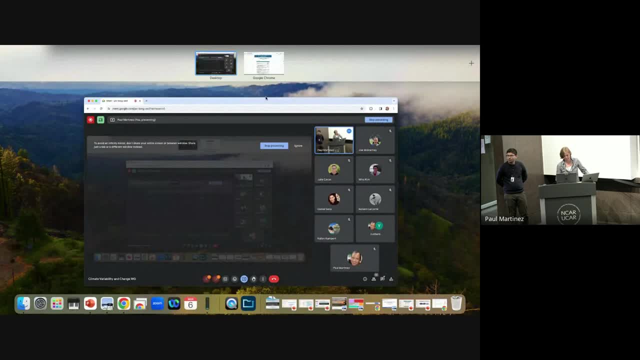 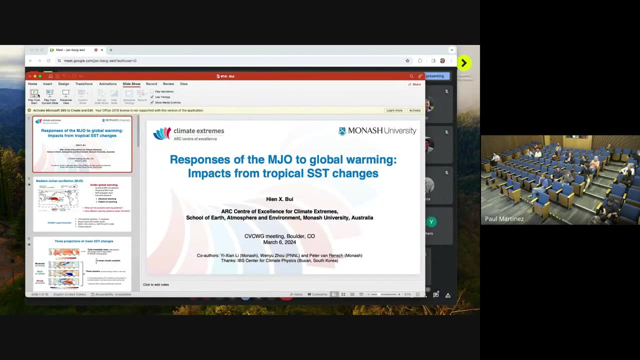 I think you need mean surface wind convergence to get any kind of convection. I think that's what you're talking about. It's both a gradient and they are not, and they manage it right. there's these two mechanisms why how you drive winds? Wind responses to SSTs is more like the gill type. 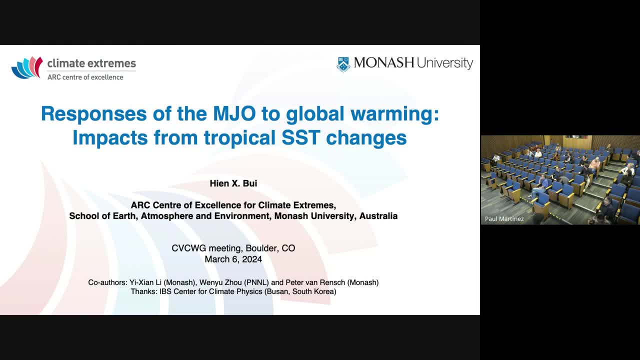 which is just the, the magnitude of the SST anomaly, and heat convert, well convergence, And then, more than linsen and negan mechanism, which is the SST gradient, that would be the pressure gradient that will also affect the treatment and perhaps in climate models and in nature is a mix of both mechanisms. It's the anomaly and the gradient of the anomaly. 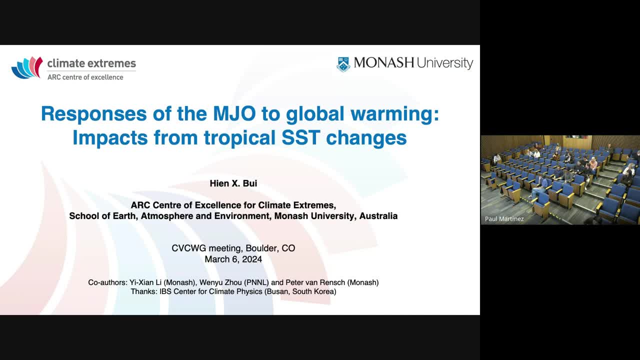 But in the far eastern pacific, like in those plots that Brandon was showing, the gradient cannot drive at eastern westerlies will drive easterlies because the SST anomaly is the absolute anomaly And the absolute anomaly or the SST anomaly cannot excite the atmosphere. 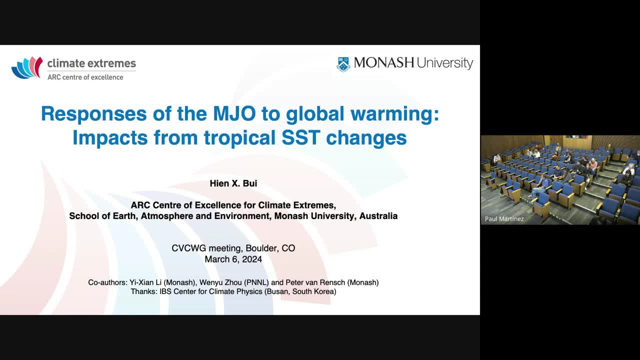 because the mean state is so cold that it cannot produce convection. Thank you, I hope that explained it All, right, thanks. So our next speaker is Hang Bui. Did I say that right? On response of the MGO to Global Warming? 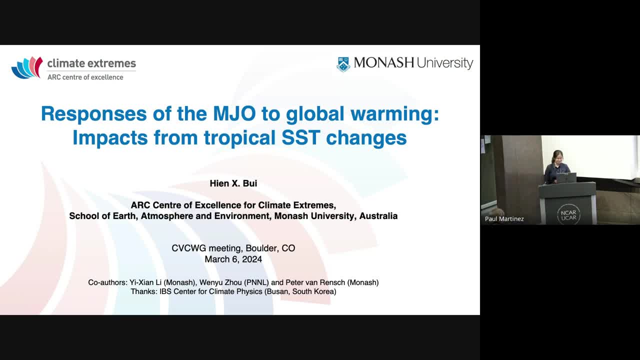 So yeah, thanks. Thanks so much for having me here. I'm currently a research fellow at the Center of Essence for Climate Stream at Monash University in Melbourne, Australia. So yeah, before starting my presentation, I just want to acknowledge the culture of the work, including my colleagues at Monash, Tiji and Amitita. 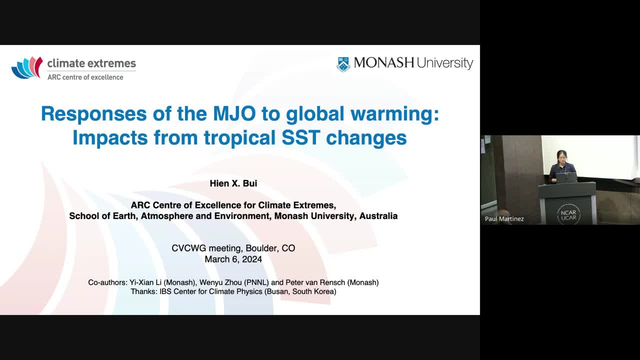 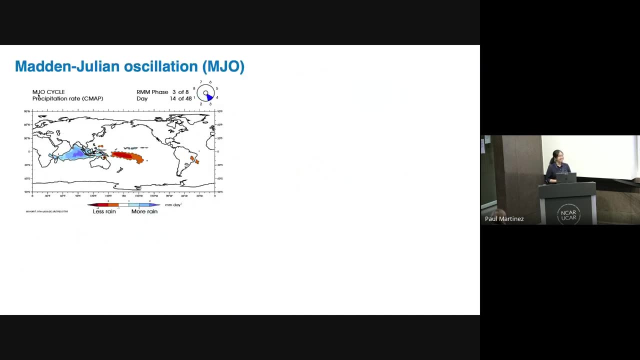 And also Wander from PNNL. I also want to thank the IBS Center for Climate Physics in Busan, South Korea, for providing the data. OK, so, As seen in your own study, you already know about the Mudd and Zulian oscillations, or MJO, or at least you have heard about it. 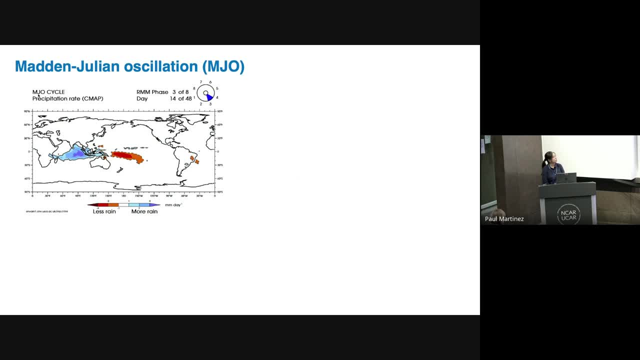 But in case that you are not familiar with the MJO, so it's a phenomenon that causes the tropical precipitation to alternate between the intense and suppressed periods, So you have more rain and less rain, And so the intense of rainfall is associated with the MJO star. in the MJO star, 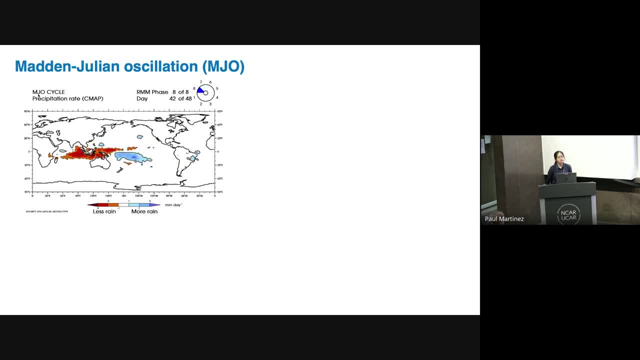 So you have more rain and less rain, And so the intense of rainfall is associated with the MJO star in the MJO star, And this is when the MX is in the ocean and then it moves lower eastward into the west reservists And it's completes the circle there around 30 to 90 degrees. 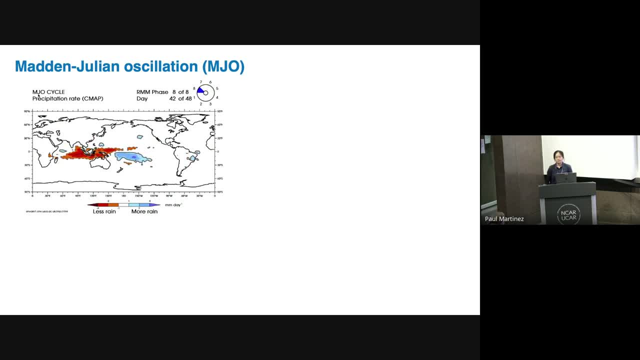 So my background and research interest is more in the global one, So under global warming, So under global warming. So we have a series of papers examining how MJO changes under global warming. So at the time we analyzed the CMIP models like CMIP5, CMIP6, we found that under global 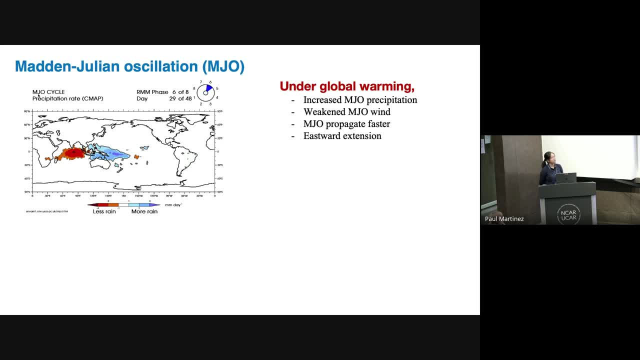 warming. MJO precipitation amplitude tends to increase, but MJO wind amplitude tends to decrease or is increased with a slower rate compared to MJO wind. We also run our planet models from DC-72, and we also found that the MJO propagations 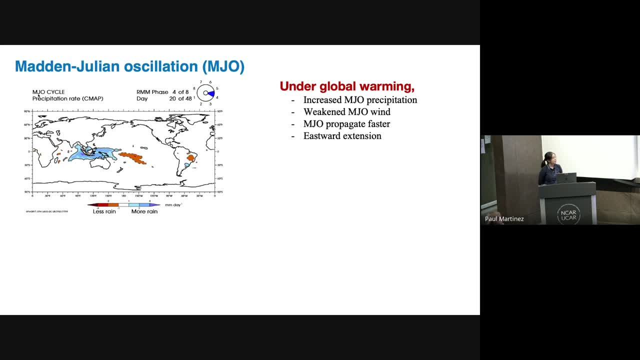 came to be faster for global warming And it's also staying further into the central and eastern Pacific in the warmer climate. However, we also noted that not just the movement has to change, but also the patterns of change can regulate the MJO. 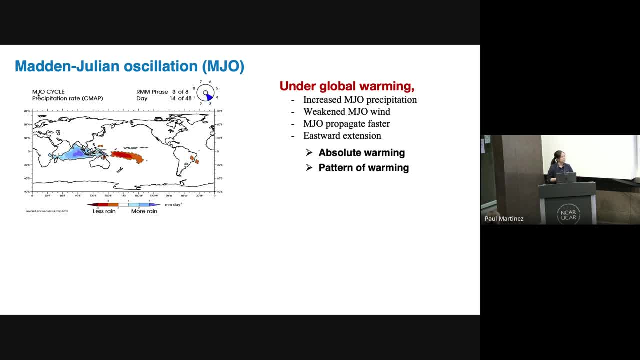 So, for example, I think you probably noted that, like during the El Ninos, the MJO tends to propagate faster, but during the La Nina it propagates slower and tends to detour over the maritime continents. So I think in the next around 10 minutes or so, I will focus on the impact of warming. 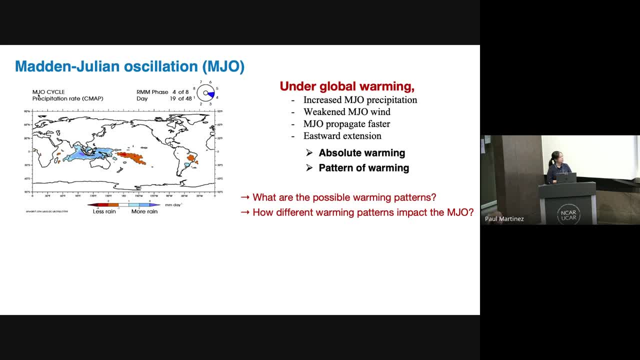 patterns on the MJO And, in particular, we will. I'm trying to answer these two questions. So the first one is what's the possible warming patterns in a warmer climate and how these warming patterns can impact on the MJO. 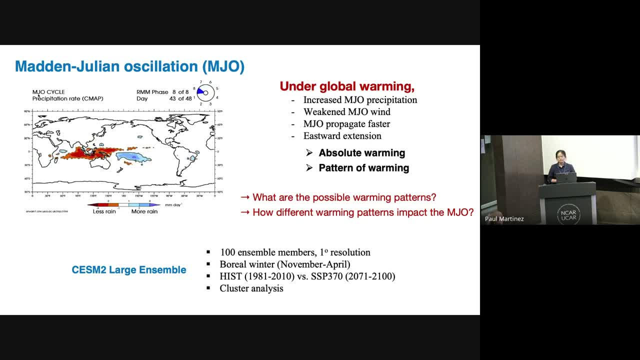 And to answer these two questions, I'm using the CSM-2 loss ensemble, So it's have one current ensemble member around 1 degree resolutions And I will focus on Ivoro winter, where the MJO is strongest. We will comparing the difference. 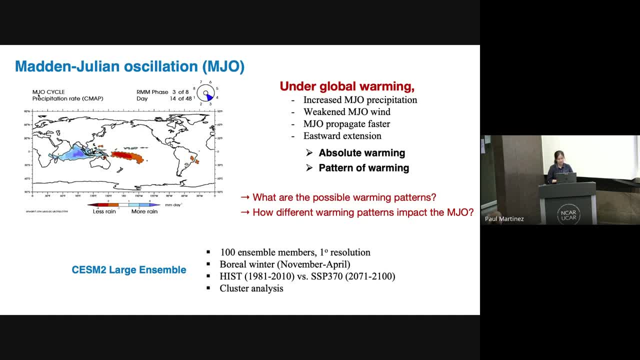 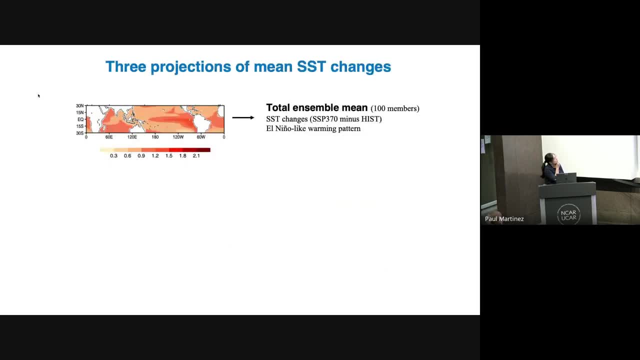 Between the future SSB370 scenarios and the current historical simulations. Okay, so let's move to the results. So here's the map showing you the SSD difference between the future and historical simulations. average of 100 ensemble member. So you can see that the patterns look like the El Nino patterns, with warmer in the central. 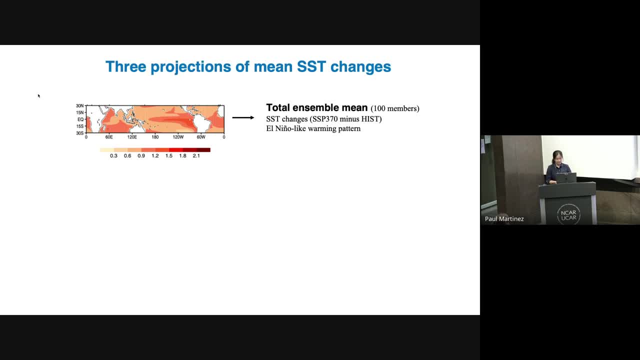 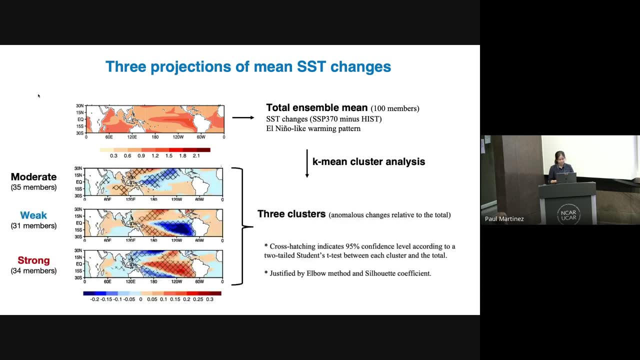 region, And this one is the Pacific. Yeah, And what we did is that we applied the hanging cluster analysis into these 100 ensemble member, And here's what we get. So we have three different group of three, what I call these three potential warming. 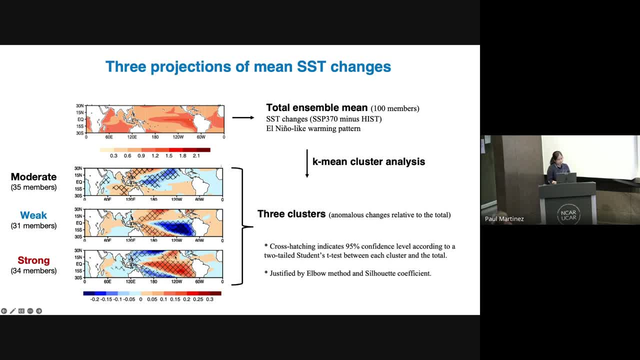 patterns in a filter That we call it moderate El Nino light group, And this is the moderate light group. And this is the moderate light group. And this is the moderate light group And this is the weak El Nino light group. 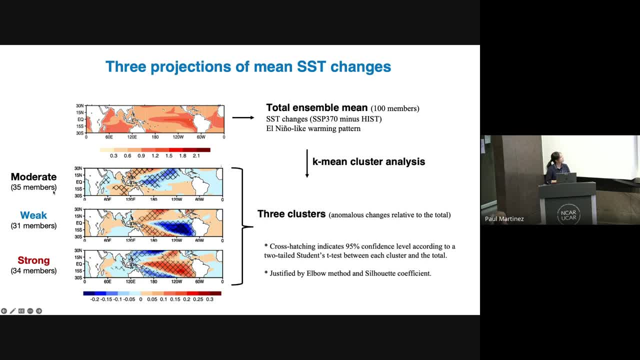 And the strong one with the number of ensemble member in this group. One thing that I want to note is that these are the difference relative to the total And it's not an absolute from this group And we did a few statistical significant tests just to make sure that each group on the pattern. 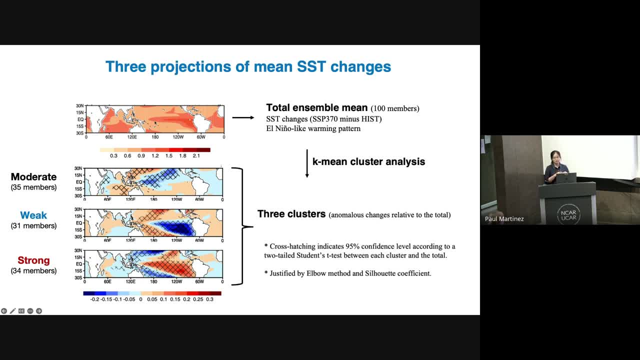 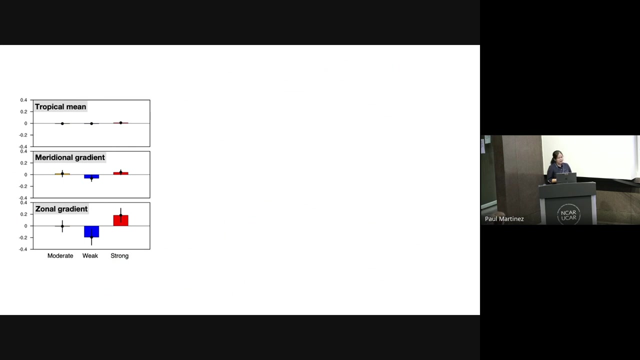 is different from the total And also it is different from the total, different from the other group, And we also justify the number of the group that we use by using the Elbow member. It's going to be the optimal number. So, after classify 100 ensemble members into three groups, 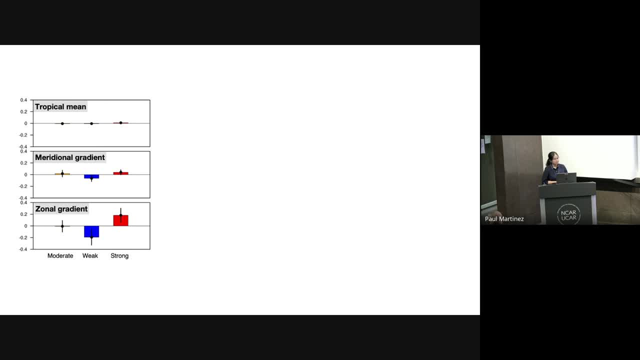 we go further into examining The temperature change in each group. So in the first panel here is just doing the tropical mean of the SSD change And you can see that for the three group the changes is very small, And also the meridian of gradients. 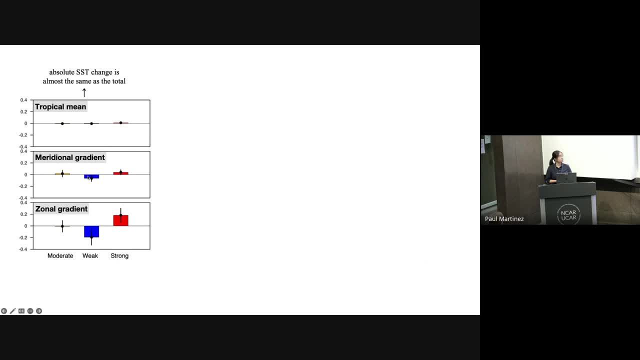 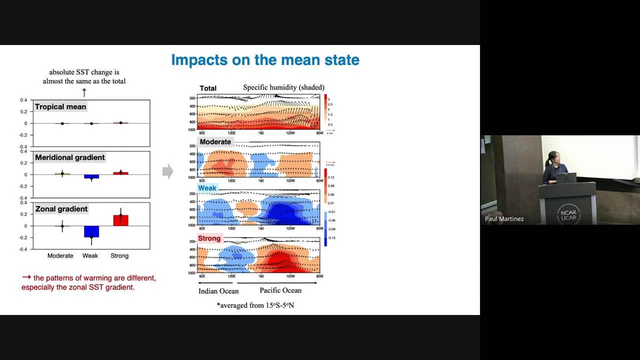 the differences between the northern and the southern here is also quite small. However, the zonal gradients of SSD changes is quite large And significant, which is the differences between the eastern pacific and western pacific. So we then examine how the difference in the SSD change. 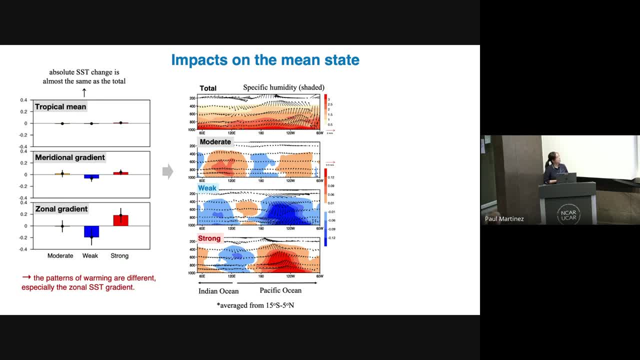 the pattern change can affect on the mean state. So here I'm showing you the vertical structure of the specific communities and also the wind. I'm not going to discuss further on the mean state changes But we have some more discussing in the paper. 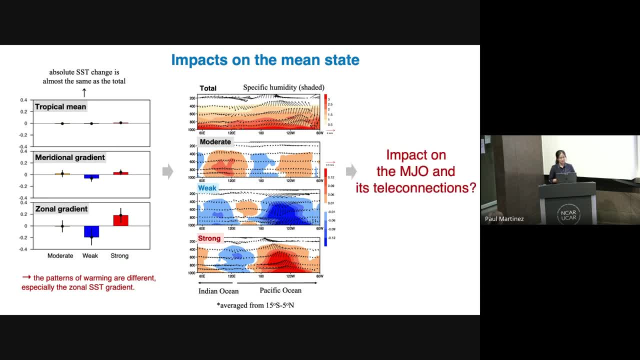 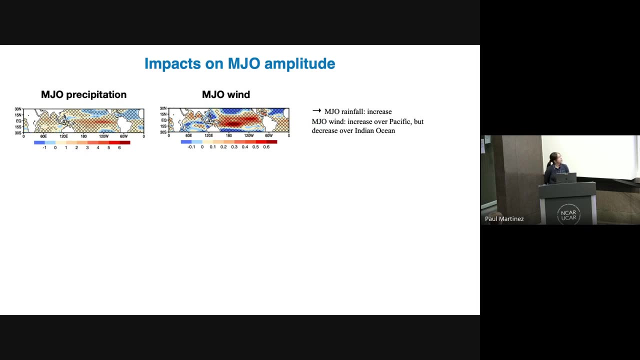 Because here I want to focus on how the patterns of the SSD change can impact on MGL. So here's the MGL amplitude. So again, this is the MGL precipitation amplitude and MGL wind amplitude that I average from 100.. And as a sample number, 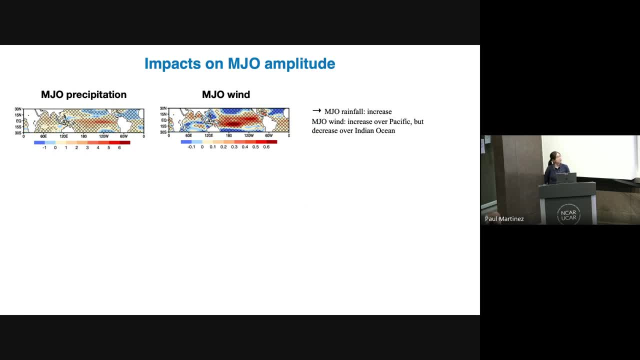 So you can see that in the future. one more climate: we have the enhance of MGL rainfall And for the MGL wind, we have some increase in here. This region is, but over the Indian Ocean is 22,, which is consistent with our previous model. 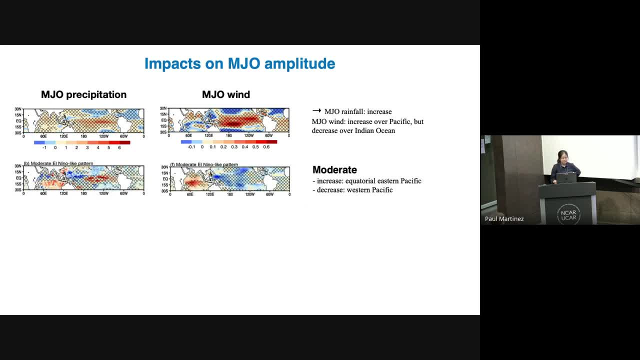 The unified model. then for the first group, the first, the first two warming patterns: waterway warming patterns: we see that the enhance of rain forest tend to be here and also in the Indian Ocean. But for the weak waterway warming patterns it seems quite different that you have a negative anomaly here and enhance all of the regions. 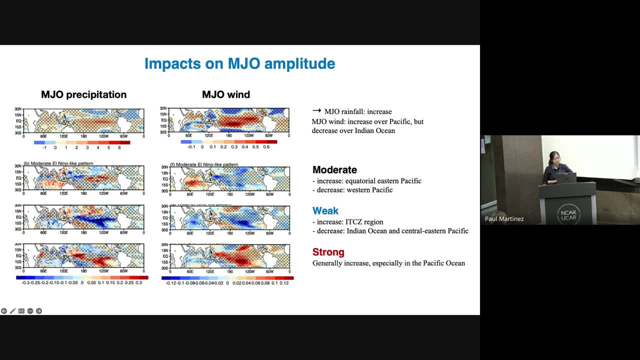 And for the strong. you know, like warming patterns, for MGL precipitation, then MGL wind tends to increase everywhere, especially in the Pacific Ocean. And again, these patterns are the difference relative to the total. So yeah, it's relative to the total, not the absolute one. 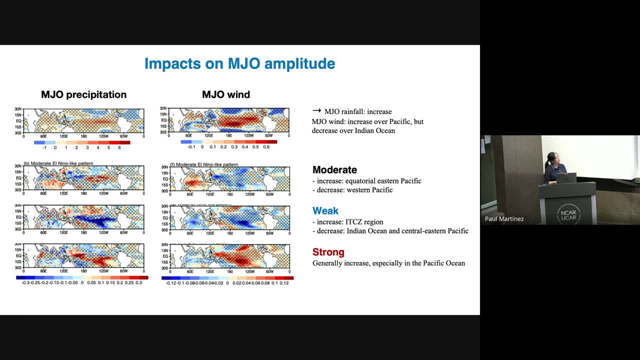 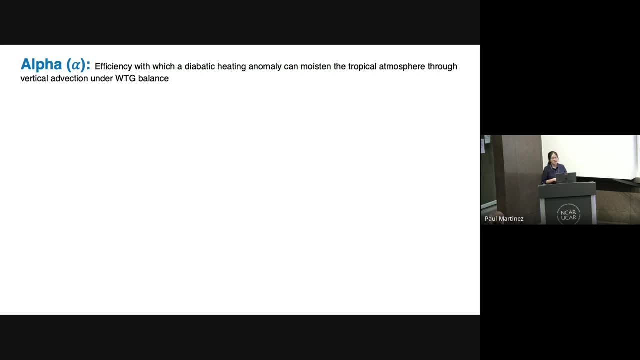 I think yeah, And I think the next question is why they have such a difference in MGL precipitation between clusters. So, to answer the question, we use ANTRA framework. I'm sure that you are familiar with this, But I will talk more about this in a few minutes. 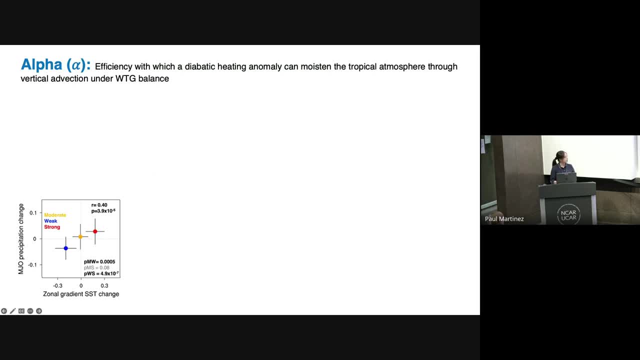 But here I'm just doing the domain average for the MGL precipitation, Just like I showed you in the previous map And on the SSS, here is the Zonal Gradient Excessive Change. Well, you have the MGL precipitation, but you have the MGL precipitation. 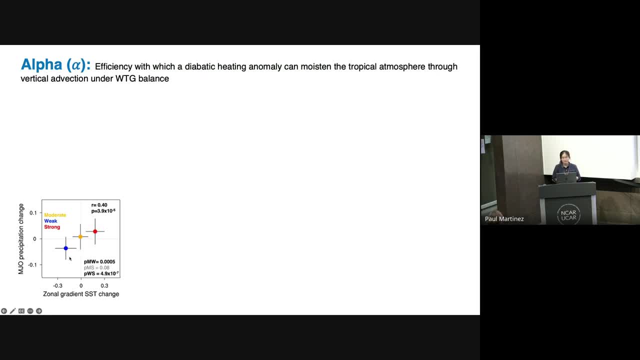 So you have the strong waterway. the strong waterway and the weak SSD warming patterns, And you see how MGL precipitation varies with this. So okay, So the ANTRA is just a property that's proportional to the vertical moisture gradients. 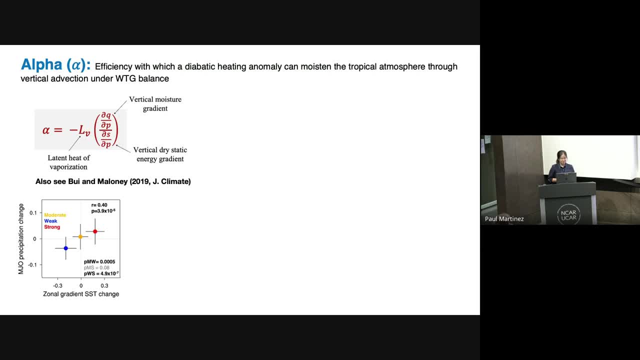 And we were proportional to the vertical dry state gradients. We have a more detailed paper talking about the ANPAR and using it to extend the NPL classification in the other paper, So check it out if you want to look for the details. But here, given the sub-part of the presentation, I'll just quickly show you how the ANPAR differs between blood cells. 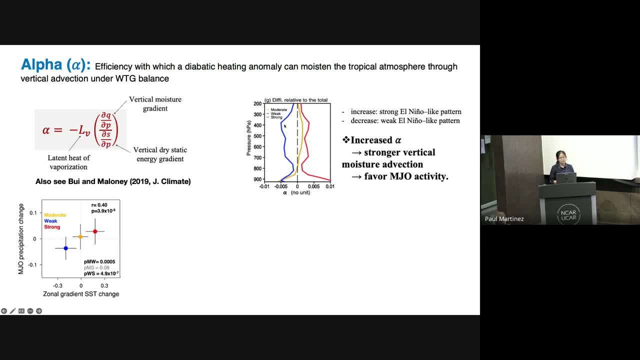 So here's the vertical structure, the anomalous vertical structure, ANPAR. So three different colors for three groups of one pattern. And, like for here, the red color is for the strong aminolite patterns And you see that these have a positive from the lower to the upper stratosphere. 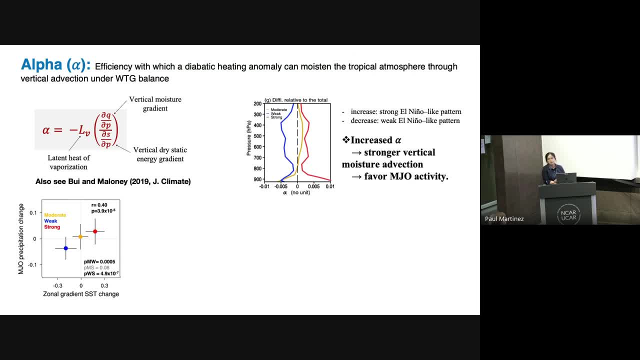 which imply that it will have a stronger vertical moisture affections. And then we expect that we have a stronger axial activity. And then I'm just doing the vertical integrated of the ANPAR And then plot it again with the NPL precipitation change. 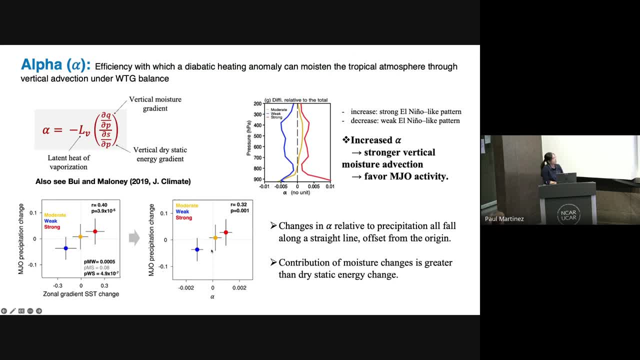 So you can see that the change of ANPAR and NPL precipitation for a lot of the stratolites- Yeah, the stratolites- and offsets from the origins. So which means that we can use ANPAR to explain for a change of NPL precipitation between different warming patterns. 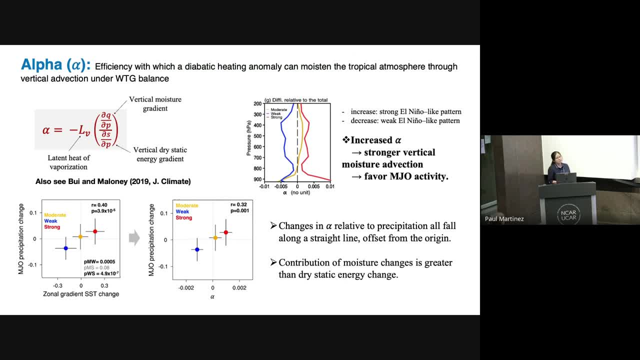 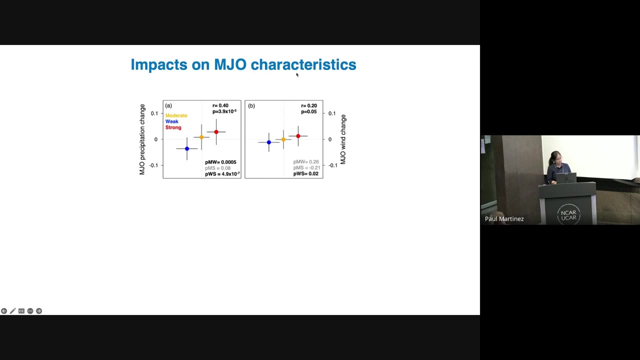 In the paper we also go further and kind of decomposing the ANPAR to the changes of the vertical moisture gradients or the changes of dry static energy gradients And we found that the change of moisture gradients kind of coming in one. OK, so that just showing you again that the change of NPL precipitation for the warming patterns. 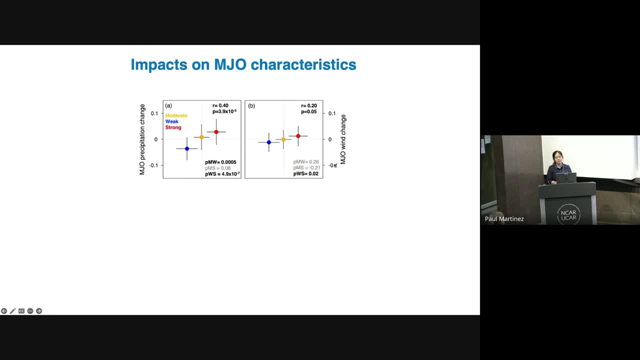 And similarly we also have the NPL wind changes. We also examine other NPL characteristics like the NPL eastward extension and also the NPL propagations. So for the eastward extension we found that the signal is quite significant between the patterns and that the strong aminolite patterns 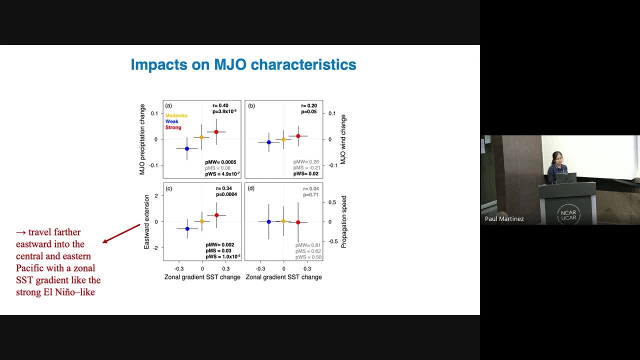 we will have the NPL kind of propagate faster compared to the weak aminolite patterns. But for the propagation speed- as you can see the bar here showing one standard deviations across the ensemble member. So it's significant And we thought that this may be used to a strong inertia over ice. 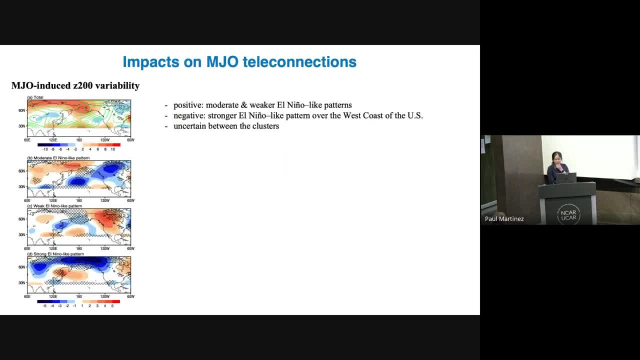 OK, so, OK. so, given the impact of the SST warming patterns on the wind state and also the MGL characteristic, we thought it would be interesting if we examine the impact of warming patterns on the MGL teleconnections. So here's again the map of MGL's induced geopotential at 200 hPa for the total 100 ensemble member and also for the tree. 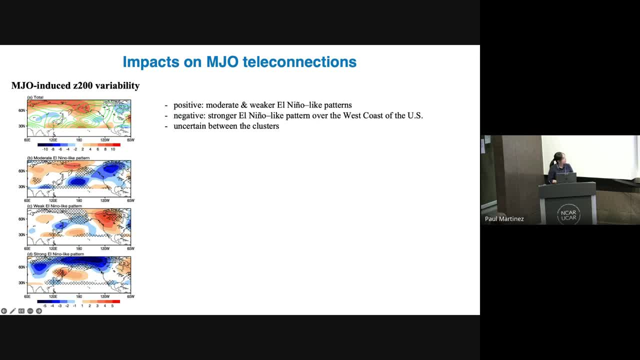 We just want to find out what's the impact of the different warming patterns. Unfortunately, we don't see a significant signal at the regions without a propagation want, especially in the west Pacific regions. But if we focus on the ensemble means for each group, 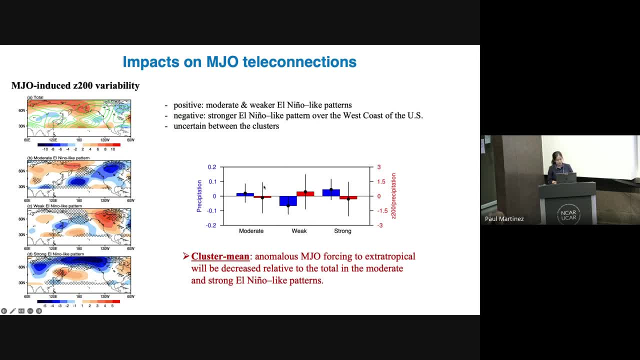 you will see that if you focus on the moderate or the strong group, the blue one is for precipitation and the red one is for Red line is for the potential high. so we show that in the future warmer climate the MGL channel connections become weaker, at least for two tops of the ensemble. 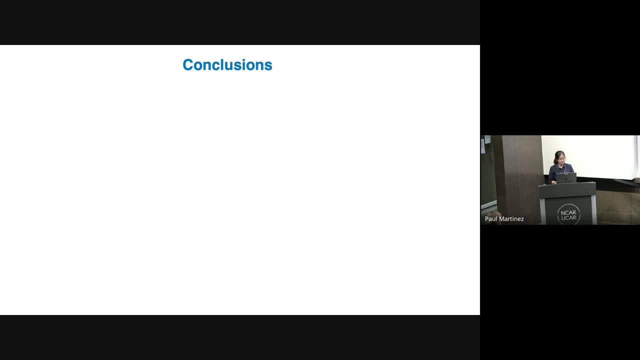 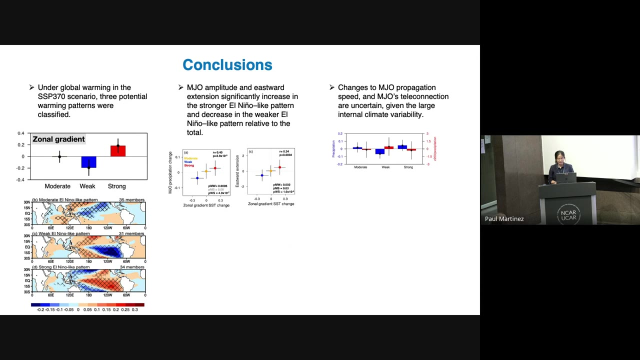 Okay, so summary for what I'm just presenting. So first of all, we have three groups, three potential warming patterns in the future warmer climate, And then we're assuming how these warming patterns can impact on the MGL characteristics and also MGL channel connections. 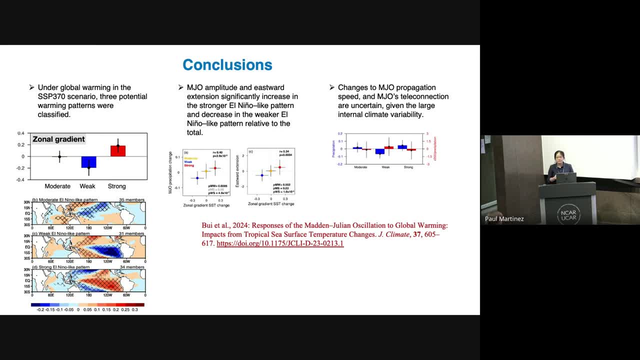 I hope that I didn't go so fast, but I guess I did So. just check out our paper just published earlier this year for the MGL Time for one quick question. I had a very quick one, but I'll get the next slide up at the same time. 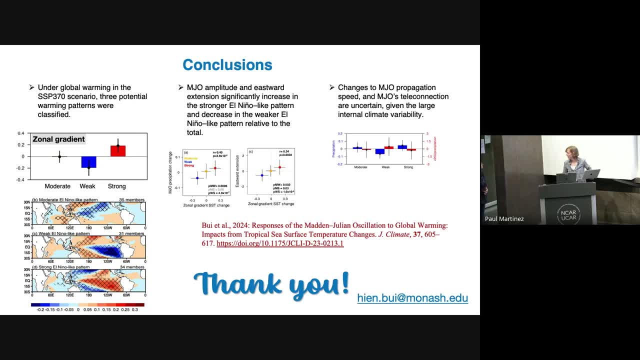 This alpha parameter in the intramural variability. Sorry, could you look at that in intramural variability and connect it with individual observations And, if they might be able to do that, correct that connection directly? Or do you think you really need big changes into the future to be able to? 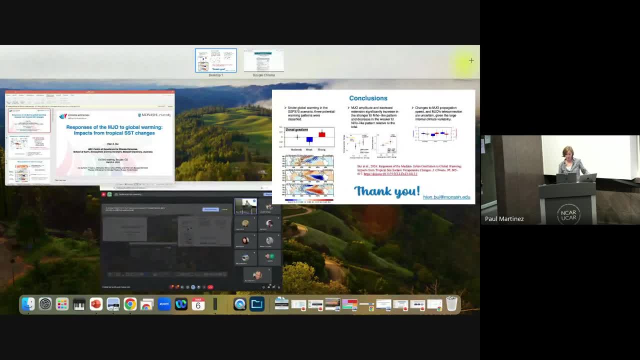 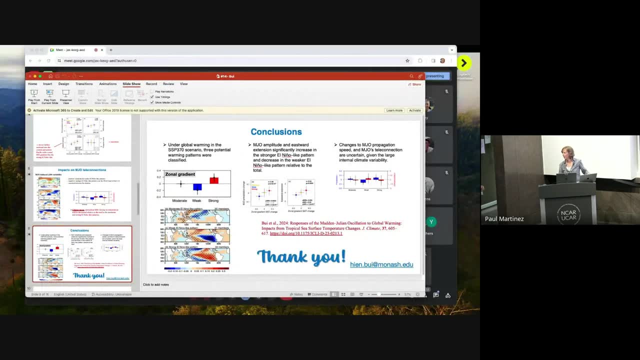 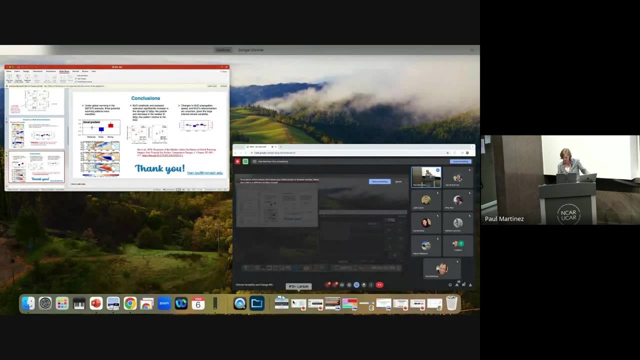 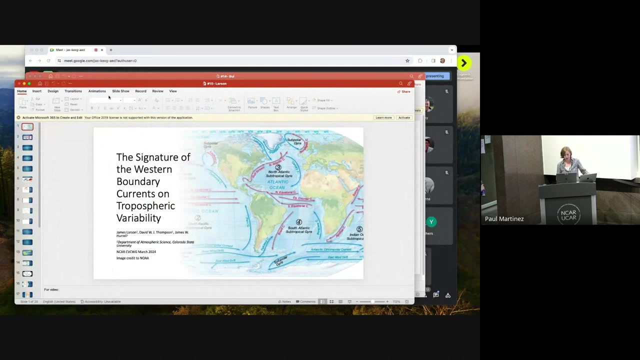 I guess that we It can do with some comparison and more information. Yeah, yeah, Okay, yeah, that would be interesting maybe to see have some confidence as to whether the models are doing things right or not. Thank you, Thank you, Okay. so our last talk before the coffee break is James Larson on impacts of Western bioengineering. 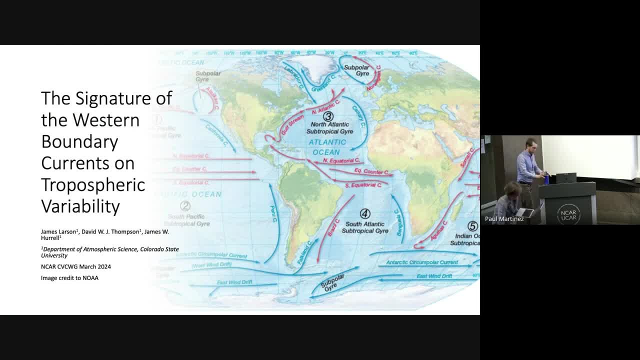 Thank you, Okay, Thanks everyone for being here and for the organizers. So today I'm going to be talking to you about the Western boundary currents, which are narrow, relatively warm ocean surface currents that exist on the Western boundaries of most, if not all, the oceanic basins. 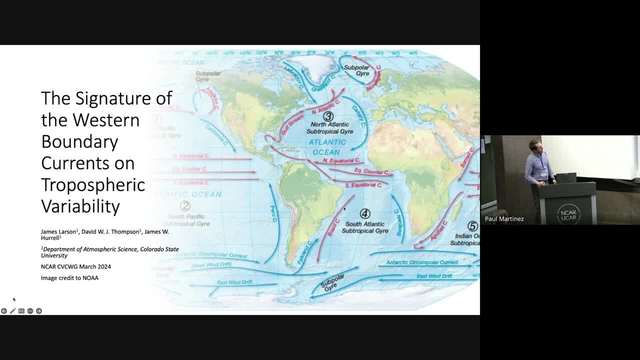 Here's an example. This is the Gulf Stream current coming up And down here in South America, the Brazil current and the Agulhas current coming off the southern tip of South America. I'm going to be talking today about five different Western boundary currents. 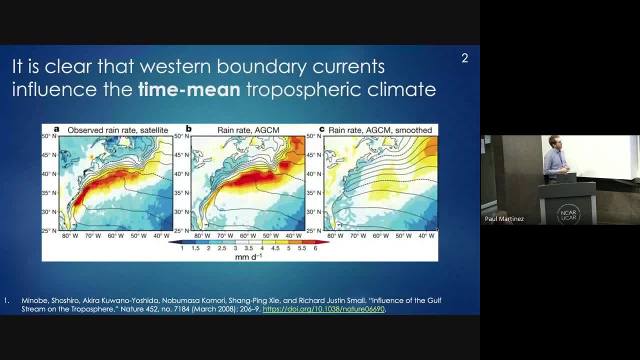 And these are just a few examples. Starting off with some motivation, though, I'm going to briefly highlight Shoshiro Minove and his collaborators work from a 2008 study where they started by looking at precipitation over the Gulf Stream, which is in the colored contours. 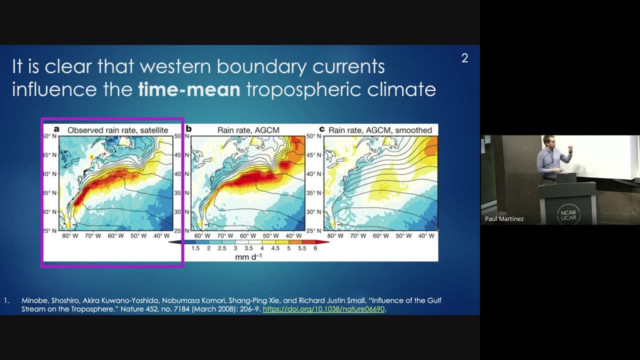 And overlaid are the black SST contours. And this is all, for the time mean over four years for observations And they found that precipitation tightly hugs the sharp SST contours of the Gulf Stream. When they prescribe those sharp SST contours in an atmospheric model they get a very similar precipitation response. 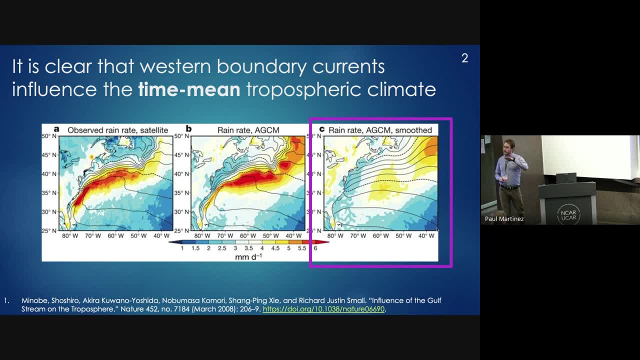 However, when they smooth over those black SST contours into an SST gradient that's much more dense, A gradient that's more similar to what you might see in the internal ocean basin, away from that boundary current, The precipitation response largely disappears, And this kind of paper is kind of. what's really motivating us is how is this underlying ocean boundary current, which is really driven strongly by internal ocean dynamics as compared to maybe the rest of the global oceans? 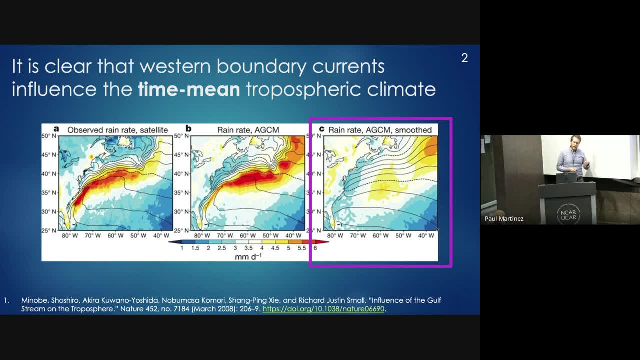 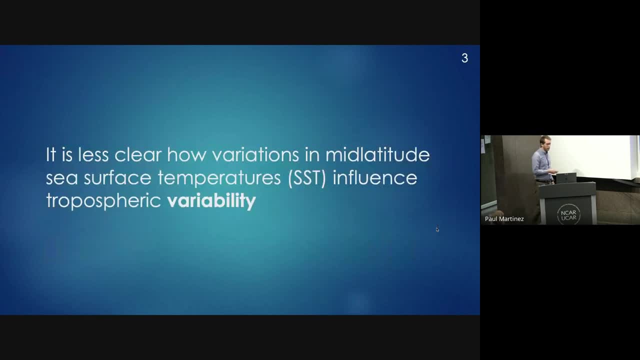 How is this driving the atmosphere above? But moving specific, moving a little more ways. How is it impacting atmospheric variability? Because they focus more on the time mean response And we are focused on the variability because a lot of literature has focused on some of that time mean response. 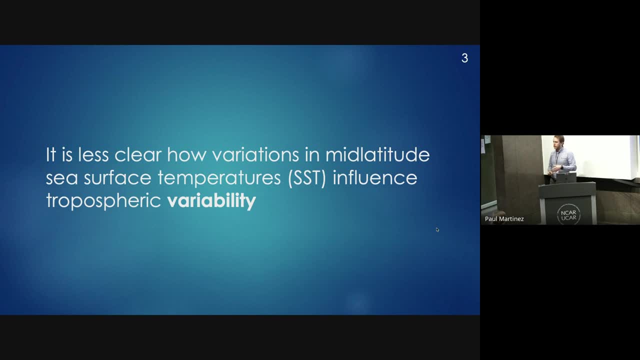 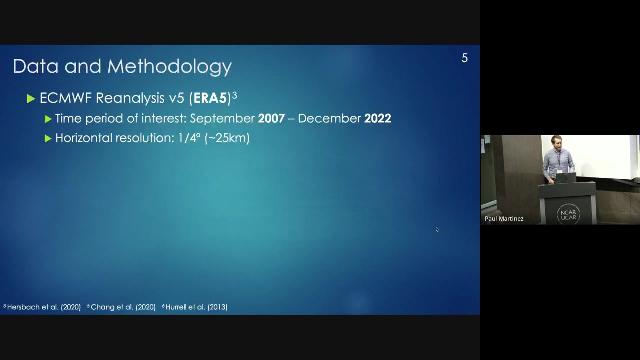 But the variability is less clear, largely due to the fact that the mid-latitudes are just so noisy. There's so much going on, especially in the wintertime, which is what's driving our research question. I pretty much just said that. 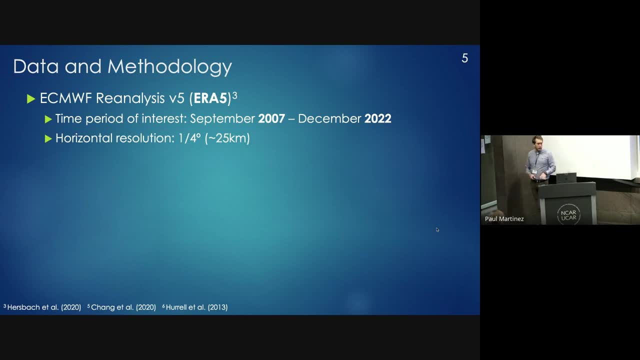 So data methods. I'm going to start off by showing you error five reanalysis. We're going to specifically look at 2007 to 2022.. We found that our results are sensitive to the under the spatial resolution of the underlying SST forcing data set. 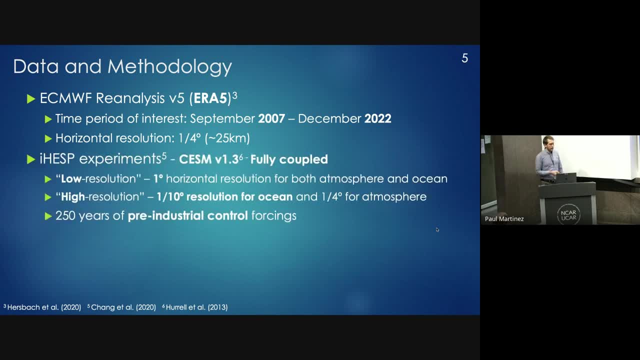 Error five is at quarter degree. And then I'm going to be ending the talk looking at the IHAS experiments, which is CSM version 1.3, fully coupled, comparing the one degree low resolution, Low, More, More Like a standard resolution, right. 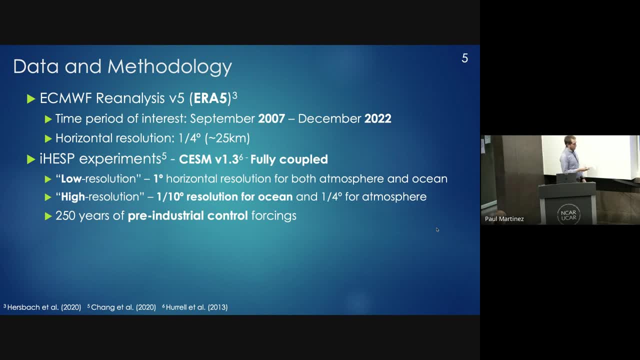 Like your CMIP rhymes To the high, And I really want to emphasize high being. what we found to be interesting is that the ocean resolution is at a tenth of a degree, which is really important for our results, And we're going to be focusing on the 250 years of the pre-induction control, the forcings. 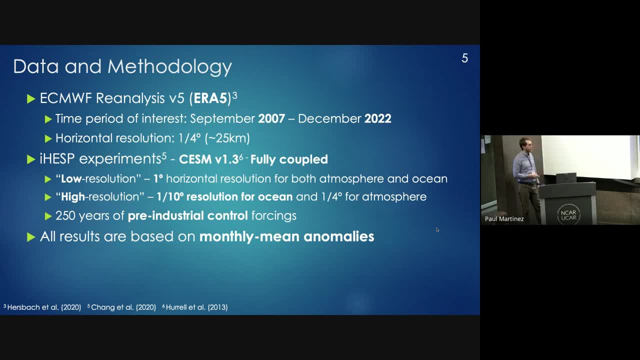 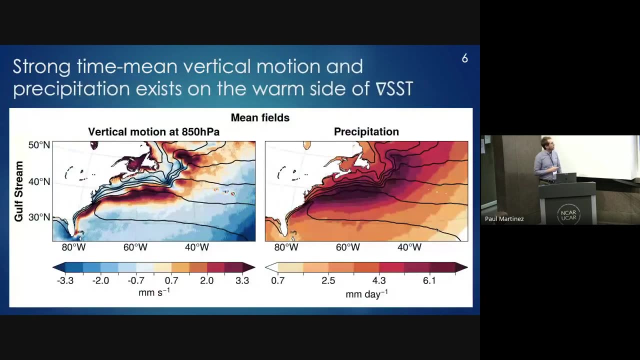 All results have had the seasonal cycle removed. one thing: the anomalies And all results are going to be for the extended wintertime for the respective hemisphere. I'm going to go through this actually pretty quickly. This is essentially just a reproduction of that Minove result for that error five, showing that not only is it just the precipitation but also the vertical motion really tightly hubs SST contours in the timing. 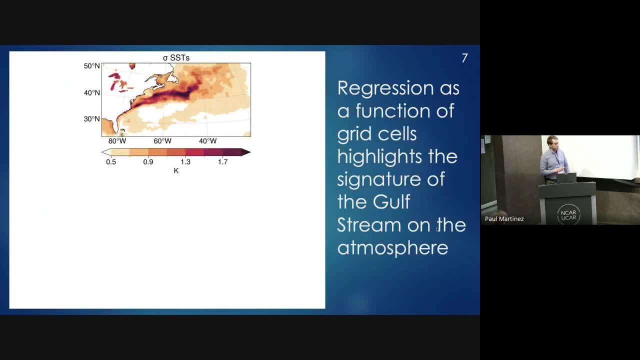 But I really want to focus on other things today. Okay, So here we have the standard deviation of SST anomalies for the Gulf Stream. You can see that where those SST contours were before, We're seeing a heightened SST growth, We're seeing a heightened SST variability. 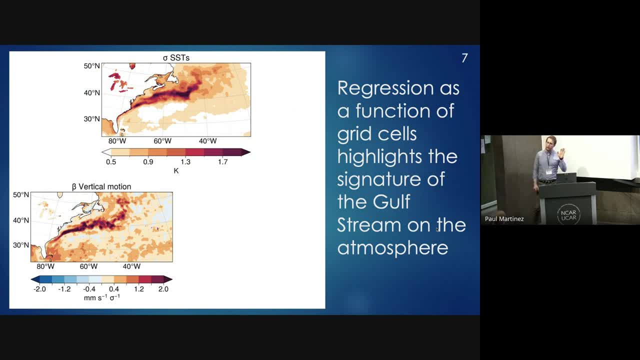 When we then bring in a regression of local to local grid cells- what I mean by that is regressing a grid cell within the ocean to the grid cell just above it in the atmosphere- not any spatial averaging or indices- We find that the atmosphere, the vertical motion, really tightly co-varies with SST anomalies within that western boundary currents. 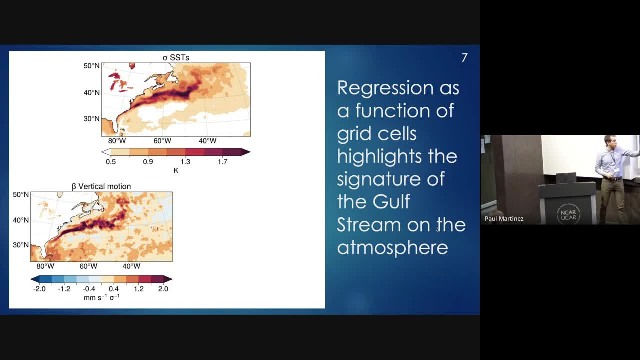 Meanwhile, though, If you look to the rest of the internal ocean basins, you find that a lot of that co-variability largely disappears, Knowing that a lot of these, that the Gulf Stream is driven by a lot of internal dynamics, SST contours or, excuse me, sharp SST gradients, mesoscale eddies. 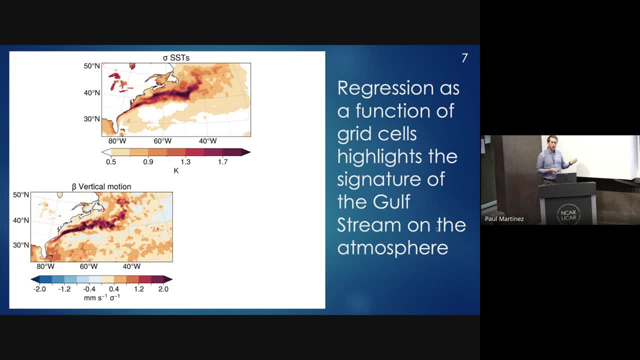 We're seeing that this is sort of suggested that the ocean driving a lot of this variability And the same thing comes through with the precipitation. This is showing error five precipitation. But we've also looked at GPM precipitation, looking at more satellite-derived product. 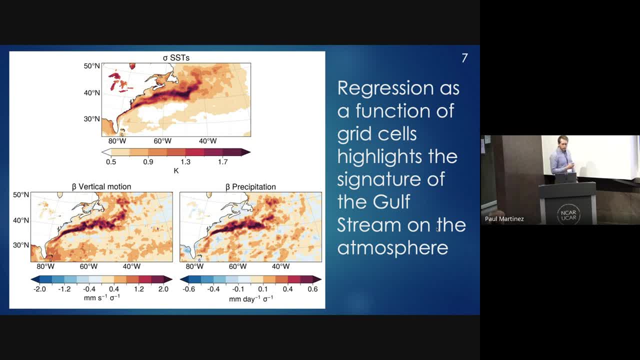 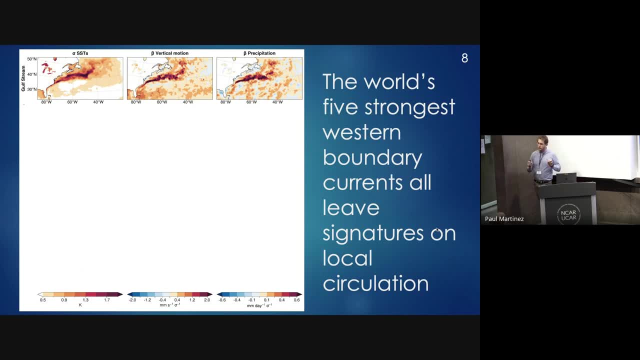 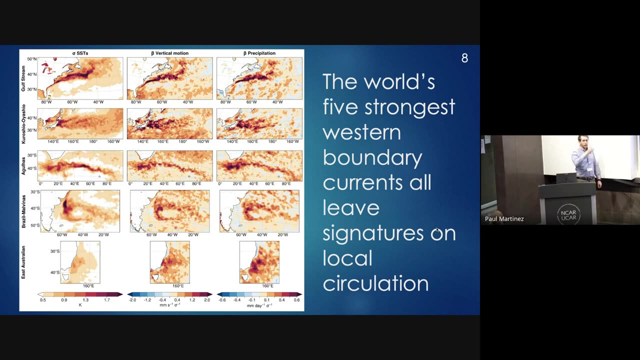 Very similar story. Yes, And it's not just the Gulf Stream. So here are the same three figures I just showed, just like a different layout. And now, when you look at four other boundary currents- five in total- you can see that for the Gulf Stream, the Kuroshio, the Agulhas Current, the Brazil Malvinas and the East Australian, 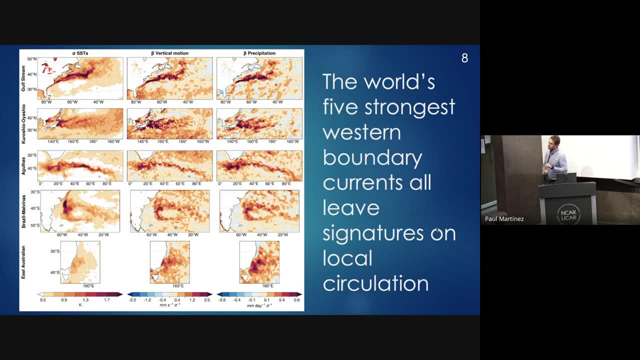 We're seeing this consistency. We're seeing this consistent air-sea signal occurring where away from the boundary current, that tight local-to-local co-variability is not really there, But within the western boundary current you really see it coming through strongly, suggesting that these ocean dynamics are playing a prominent role in driving these localized circulation changes. 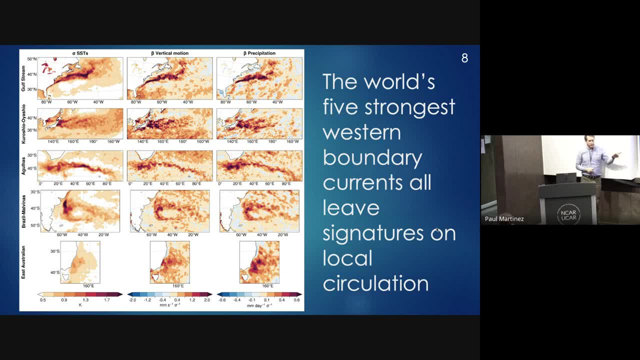 And I'd really like to point out the East Australian. This is a current that is known for having a lot of mesoscale variability, But if you compare it to the other boundary currents, it's not on the same scale as far as SST variability. 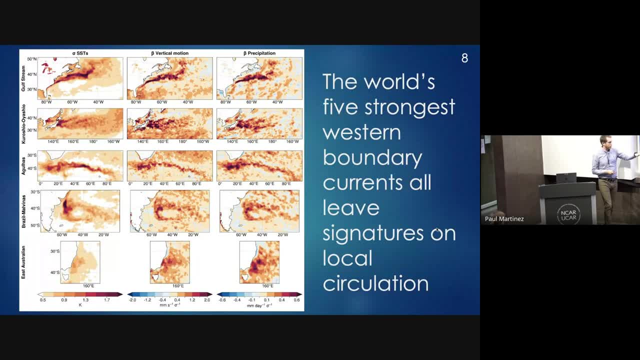 But then even with lower amplitudes of SST variability, we're still seeing this really strong signal of the dynamics at play at the boundary current Moving. But these are sort of parameters that are relatively close to surfaces. Vertical motion at 850 hectopascals. I should have clarified. 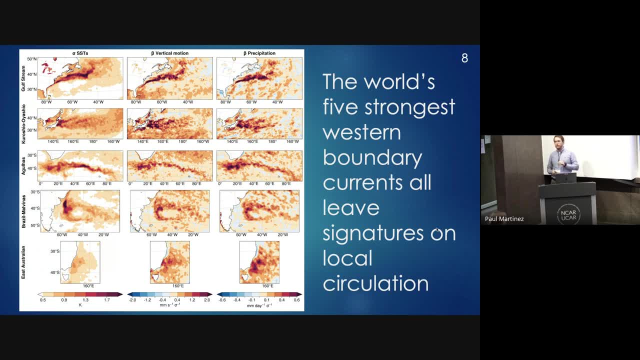 If we take a spatial average of the area just over the western boundary current and then look at vertical motion, not just at 850 hectopascals but higher up into the atmosphere, and perform the same sort of local-to-local regression technique. 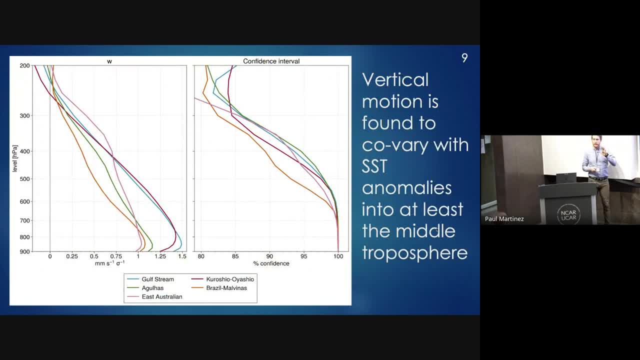 we can see how air-sea co-variability is extending up into the middle and upper troposphere. So here on this left panel I've got the five different boundary currents over different colors And it's just a spatial average of that same regression technique I just showed. 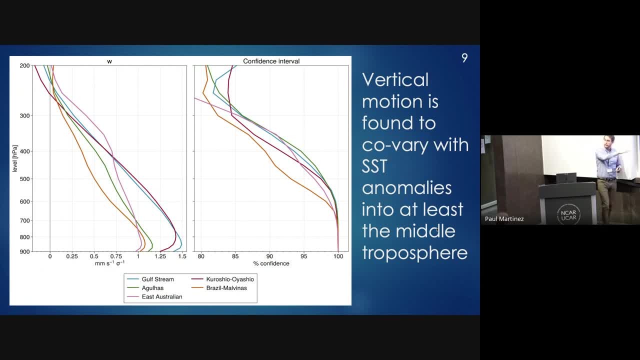 Where, of course, naturally, as you might expect, close to the surface, we're seeing the strongest regression coefficient, the strongest coupling of air-sea co-variability. But that co-variability is not remaining just as close to the surface. 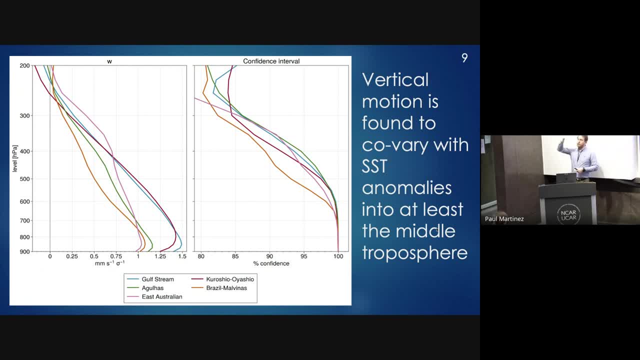 It's extending beyond the planetary boundary layer, extending up into at least the middle troposphere. On the right panel we have a confidence interval derived loosely from the student's t-test. we've played around with a little bit And I can go into those pieces. 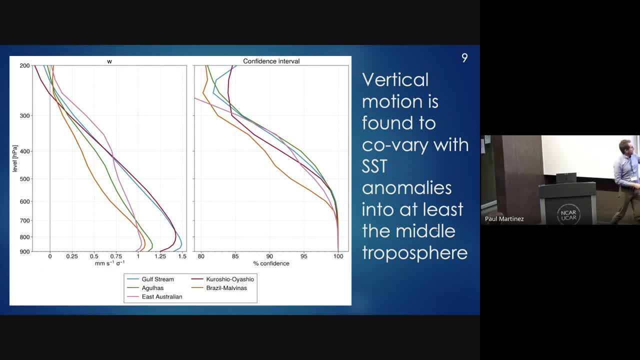 I don't know if you'd like to know more, But you see that, following the 90% confidence, that's extending up to 400 hectopascals, really suggesting that these ocean dynamics are driving these localized circulation changes. But we're here at a CSM workshop, not an ARF-5 workshop. 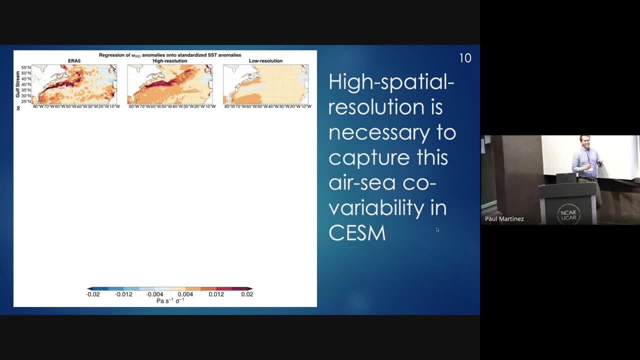 So here are the modeling results that you guys want to see. Okay, So now I'm showing you the regression of vertical motion at 850 hectopascals. Left column is going to be ARF-5.. This is what you have seen. 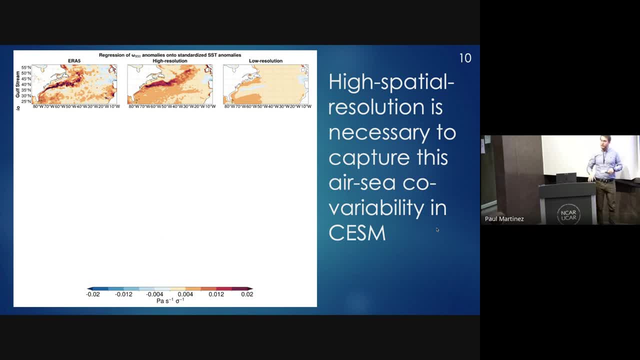 Middle column is that high-resolution CSM And then comparing it to the low resolution. That high resolution is comparing quite nicely, showing that fundamentally the dynamics within CSM are there, are sound, But when you're simulating at that one-degree resolution which is sort of the standard workhorse resolution that we see a lot in the CMIPS, 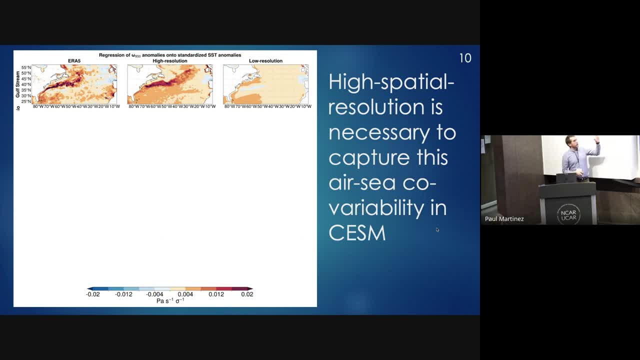 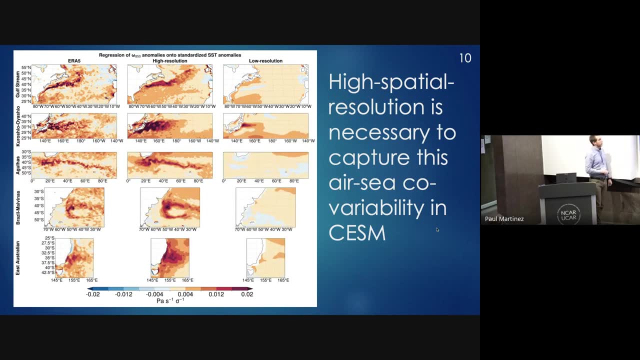 And other style experiments being run at, they're not really getting that ARC co-variability, And that is true amongst all the boundary currents. I really love the shape of this Brazil malvenous current, that you get this cool lobster claw that you would really I mean to think about how the atmosphere might form. that shape is hard to wrap your head around. 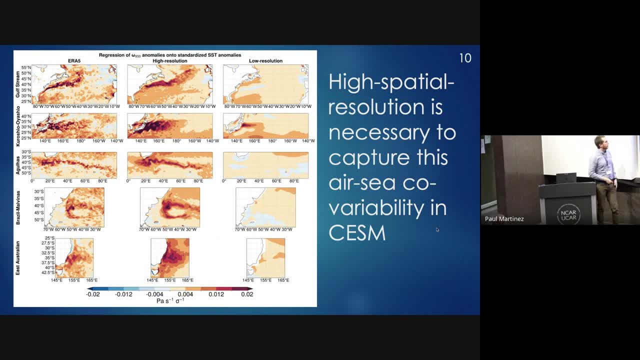 But the way the underlying oceanic currents run, it's just so cool. You can see that in the high resolution and just And so this result is kind of what's going to motivate us moving more into the future. We plan to take these results for digging deeper into the modeling studies, looking to see how these underlying boundary currents might be driving changes in the clouds radiation. 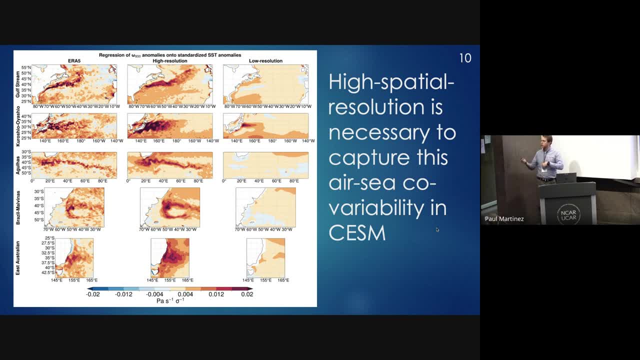 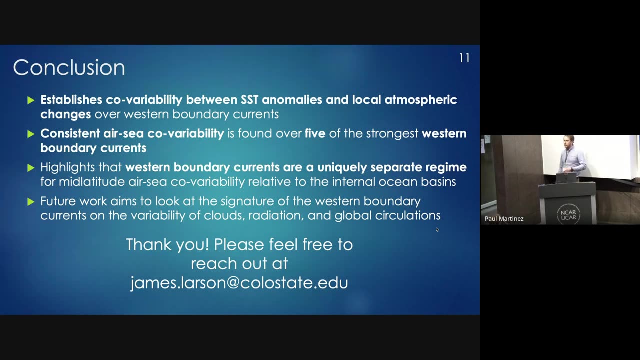 Not just localized circulation changes, but how it might be impacting jet stream variability and the storm tracks as a whole. This works so far within my masters and I'm planning to continue moving forward with it into my PhD Conclusion. really just that we're looking at how these oceanic-driven dynamics are changing: localized circulation changes. 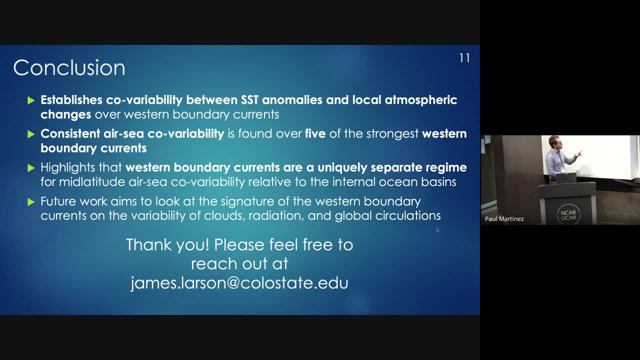 And I also would like to point out that, for those of you that aren't really deep in this ARC interaction literature, it's normal for most papers to maybe just look at one or two matters, But it's not Okay. So if you're looking at all five of these boundary currents, it isn't always normal that people are exploring all five of these boundary currents across the globe, seeing these consistent signals across the different regions. 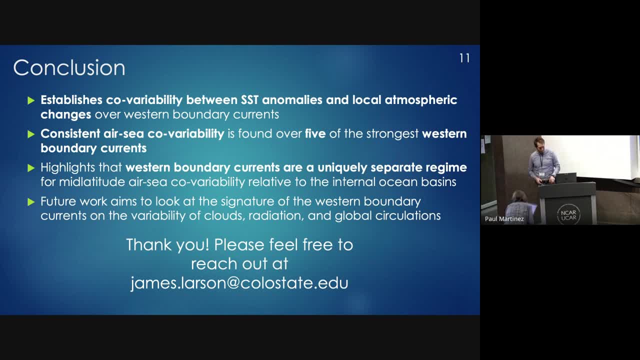 So with that I'll end and take any questions. Thank you, Questions. I love the questions. I was just curious if you've looked into how persistent these precipitation anomalies are. precipitation anomalies are over these western boundary current regions. um, yeah, so we're looking. 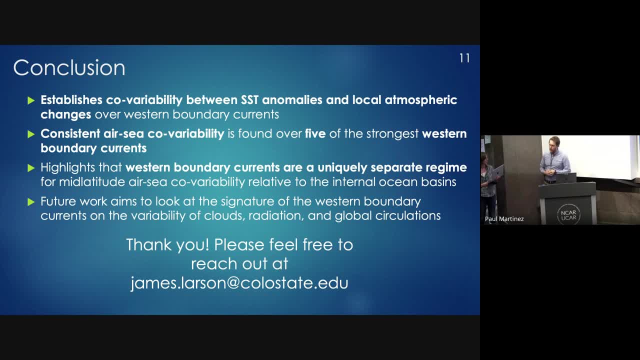 at time scales of month to month, um, not sort of decadal. um, once the maybe like the warm Eddie that's driving these localized changes- kind of dissipates, it does kind of disappear. um, and that was also holds true when you move away from the winter season into the summertime season, when all 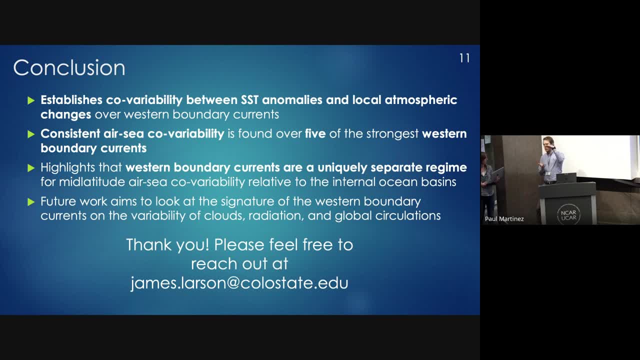 of a sudden that cold continent. there's not as much contrast between the cold continental air and the warm ocean. um given it's not that it completely disappears. we are seeing subtle hints of this in the summertime um months, which is kind of exciting. we're thinking about looking. 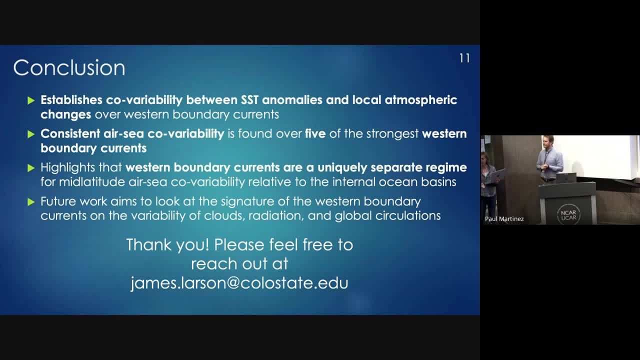 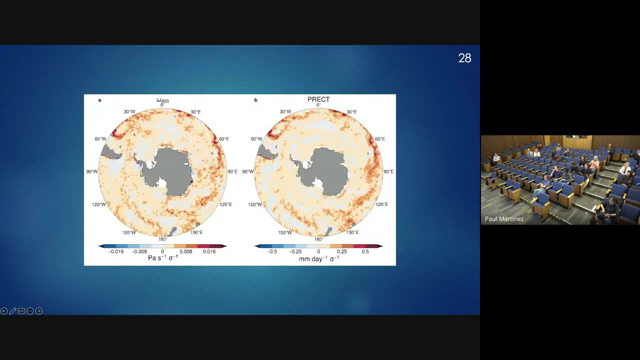 for that more, Steve. yeah, um, in addition to the boundary currents, there's the Southern Ocean, so I'm wondering if you're going to be looking at that as well. yeah, um, okay, uh, this one. these are the standard. here's the regression. it's not clear, and I think they're. I don't know why. my intuition leads me. 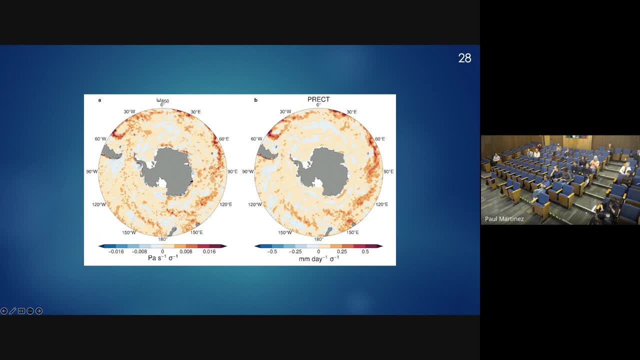 down two different paths. one is that, um, the Southern Ocean isn't as warm as the Western boundary currents are because they're transporting a lot of the heat. I think that might play a role. and two, um, because the Rossi radius of deformation, the Eddie's in the Southern 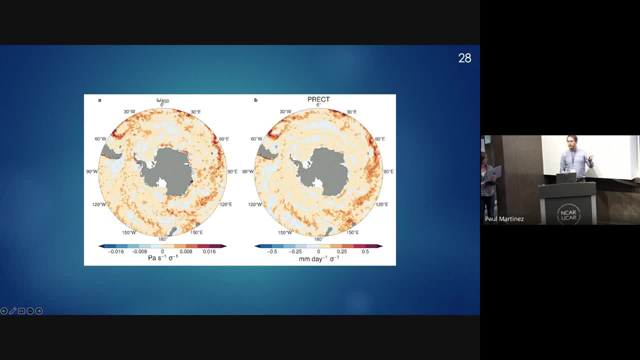 Ocean don't get really small. I'm not sure if the era 5 reanalysis is of resolving that. so it's I. yeah, I'm with you. I think there should be a response of it. I'm not sure um fringer at all 2013 and looked into that. yeah, it just was a nice, very nice talk. I, I was just 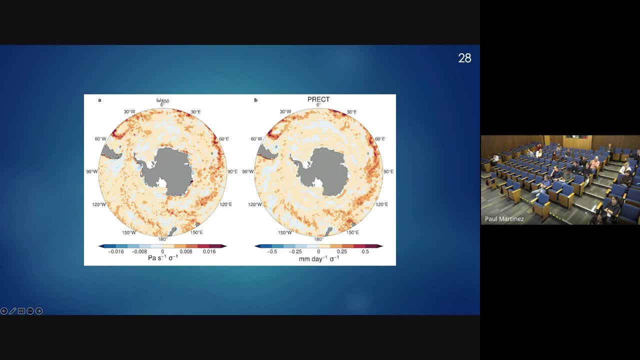 um, making sure I understood, uh, what you were doing. you're taking monthly anomalies, you're doing these local regressions and then you're averaging over the winter season. is that correct? are you first doing the winter anomalies and then doing local? yeah, so I I dropped the summer. um, yes, first I formed the seasonal anomaly and then I dropped. 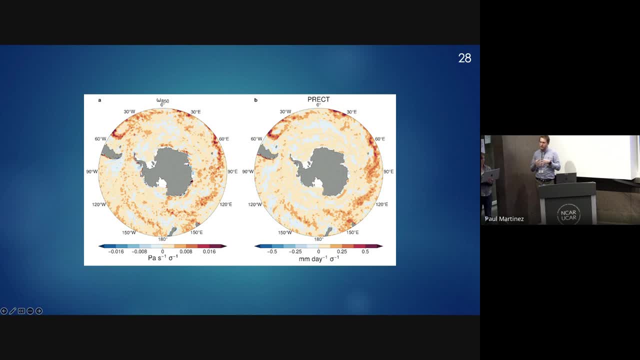 the summer months for my data set. I don't do any time averaging, I'm not, it's not like a seasonal average, so I'm doing monthly regressions. um, one at the month, um, yeah, does that answer anything? yeah, so you're including interest, seasonal, correct and it, and year to year, yes, so I think coming. 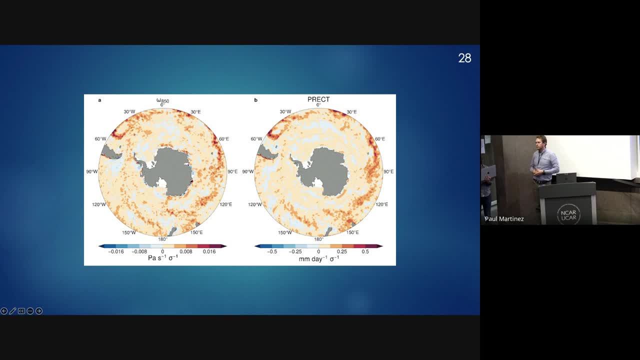 to your point. it was a similar point. I think it'd be interesting to take those apart. oh, yeah, yeah, yeah, that's good, that's great, thank you, yeah. so yeah, thanks everyone. so well, uh, we have a break now until three. gonna be some more cakes, but yeah, the coffee's probably cold at this point. but very well, just for that. 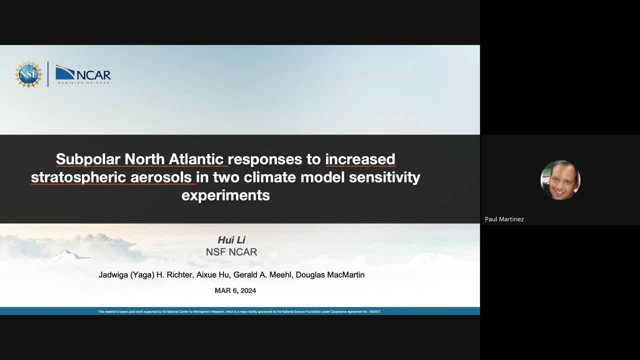 you, you, you hug you. I don't know it's like. from the outside it's pretty obvious that there's this thing. Yeah, I know, Yeah. series of talks: we have three talks on geoengineering related topics and then we'll have the discussion. so the first presentation is really on the South Atlantic. response to stress is very good. 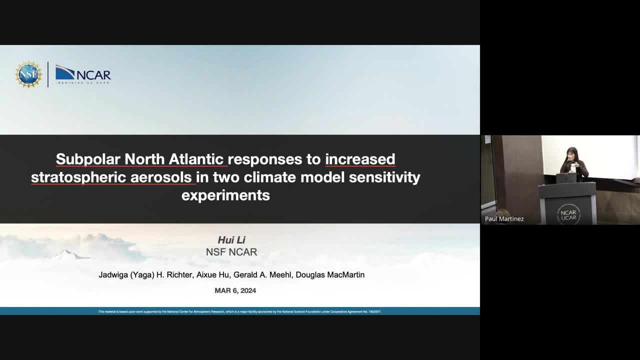 Thanks everyone. I'm away. I'm here at anchor, So today I'm going to talk about subpolar and the Atlantic responses to increase the stratospheric aerosols in two climate model sensitivity experiments, And this is in collaboration with Yaga Aisha and Jerry here at NCAR, and also Daggett Cornell. 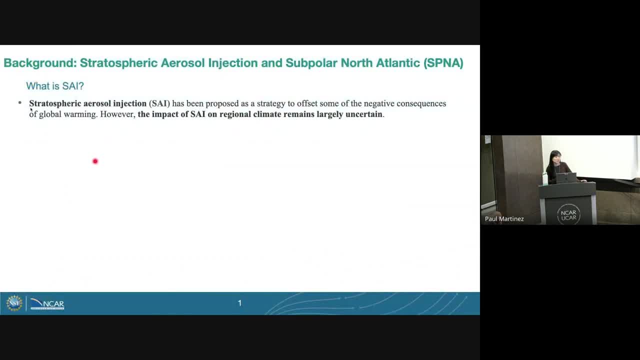 A little bit of motivation, And so talk about stratospheric aerosol injection is kind of a has been proposed as a strategy to kind of offset some of the negative effects, Offset some of the negative consequences of global warming. However, the impact of this expressive aerosols are largely uncertain. 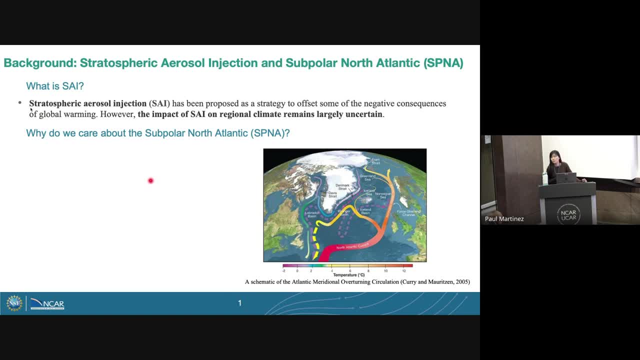 So one of the regions that's critical for the global climate is the subpolar North Atlantic. It is important because it is the region for ocean deep convection and dense water formation, which is part of the Atlantic meridional overturning circulation, or AMOC, which is crucial for regulating global heat and carbon transport. 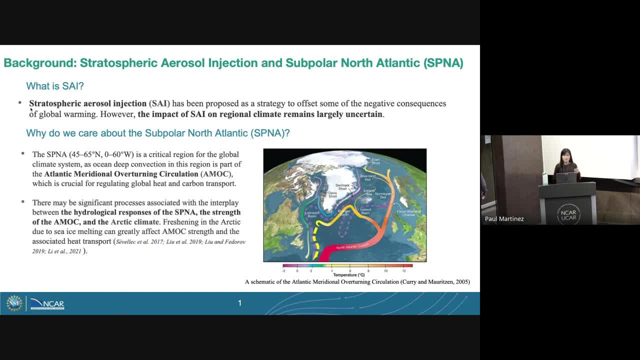 And also there are significant interactions between the hydrological responses of the subpolar North Atlantic- I'll just call it SPNA, It is very long word- and the strength of the AMOC and also the Arctic climate. So it is critical that we understand the impact of this stratospheric aerosols on this region. 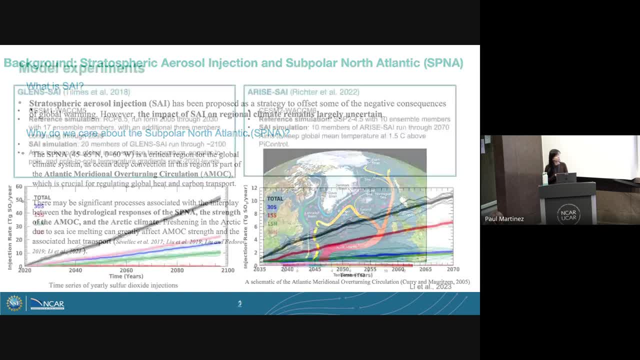 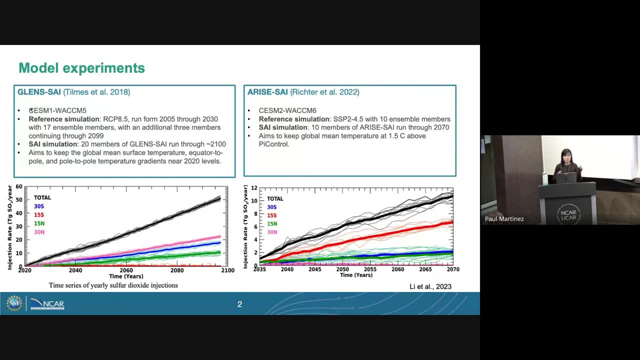 So we're going to use two sets of climate ensemble climate simulation ensembles to investigate this problem. We're going to use these two. They're called Glens SAI and Arise SAI. So basically, in both models, stratospheric aerosols are added in order to counteract the effect of elevated greenhouse gas. 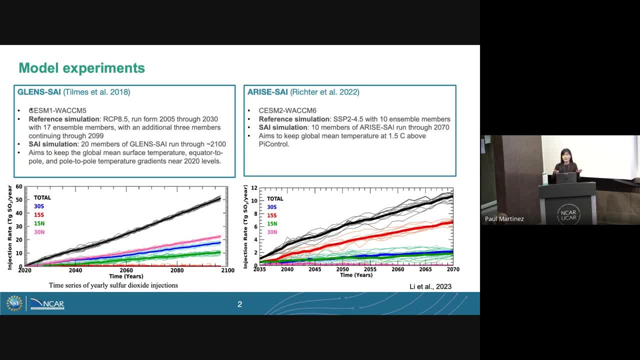 And it's the stress of. aerosols are added in a strategic way. So, for example, this figure: these are injections at different latitudes, with different colors and they also vary with time. So the goal is to kind of add this aerosol. 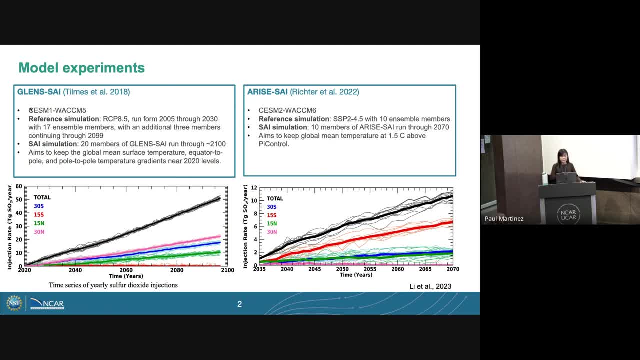 So you kind of add these aerosols in a prognostic manner. So for the Glens simulation, it uses the ECSM-1 wildcard biophysics. The reference simulation without SAI is under the RCP 8.5 forcing. 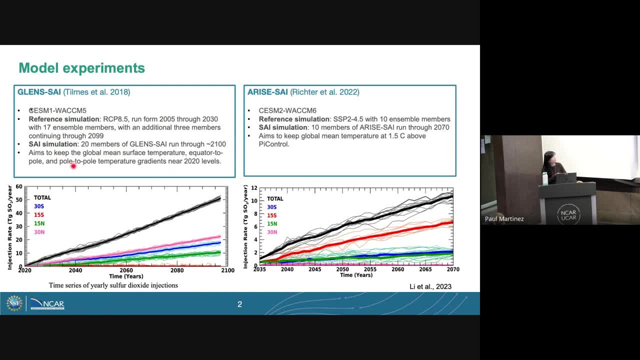 And then the SAI simulation. the aim is to keep the global mean temperature equator to pole and pole to pole temperature gradient near the 2020 levels. And then the Arise simulation is very similar to Glens. It uses an updated version of CSM-2 and WACOM-6. 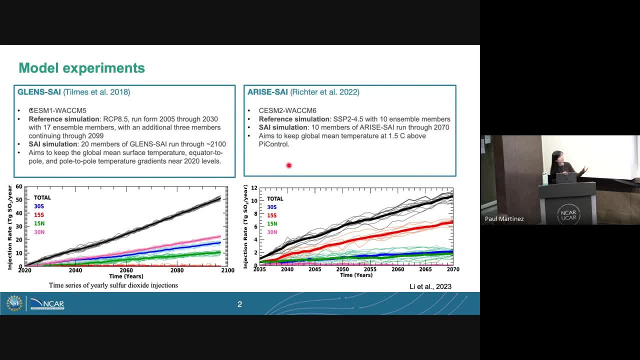 The reference simulation is a more moderate forcing scenario. It's under SSP 245.. And then the aim of this simulation in some ways is to keep the global mean temperature and temperature gradient at about 1.5 degree above the pre-industrial control level. 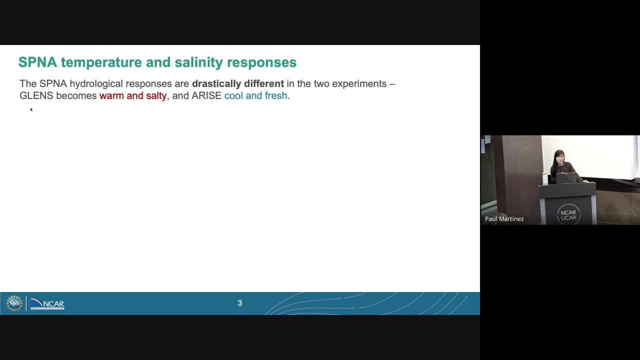 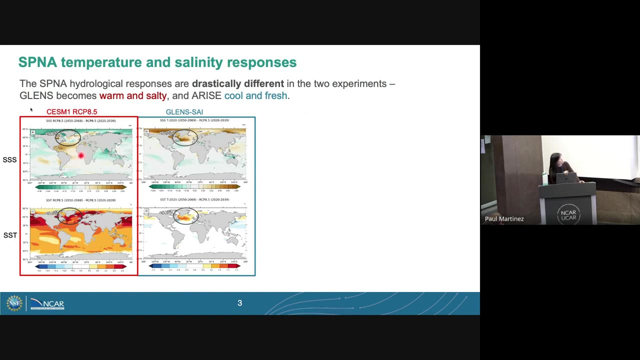 So first of all we're going to take a look at the simulated climatology. It turns out the responses in these two models are quite different. So here are the anomalies of sea surface salinity at the top two panels and the sea surface temperature at the bottom. 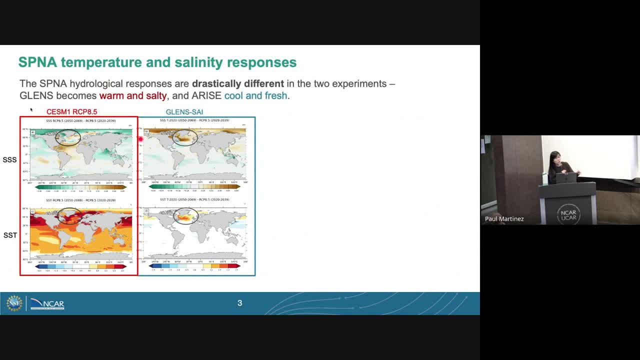 These anomalies are defined as the difference between the end of the century to the beginning of the simulation And on the left, the two panels are the changes in the RCP 8.5 scenario And we can see that with global warming we have a you know. 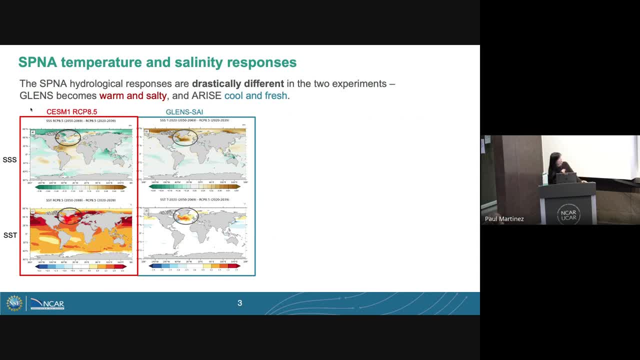 a general increase of global temperature. but in the SPNA region we have a warm and salty response, And when we go we're adding that- stratospheric aerosols First of all. the global mean temperature is indeed kept at a stable level. 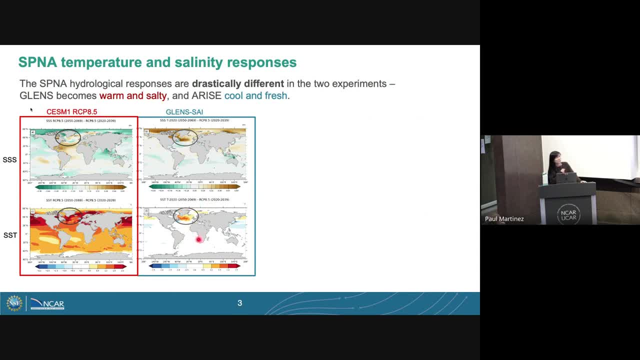 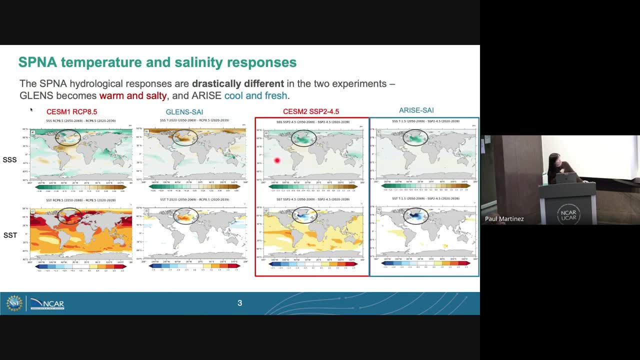 But then if you look at the SPNA, there is still a very significant response and it remains warm and salty And for the Glens simulation. interestingly, in the reference climate the subpolar North Atlantic actually becomes cold and fresh. 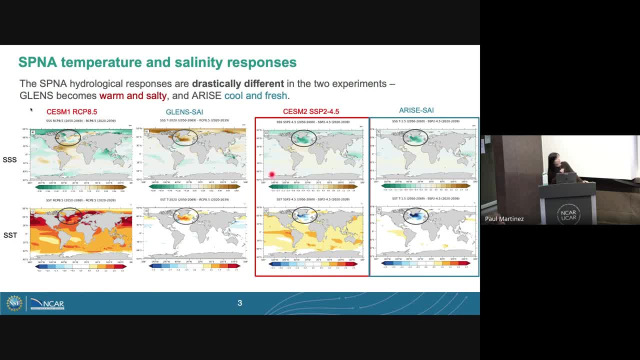 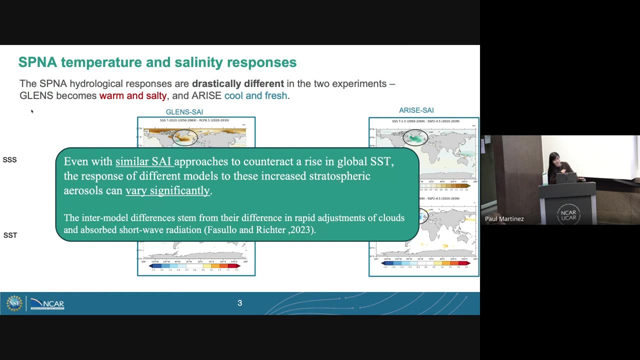 It's quite the opposite from the CESM-1 simulation, And when you're adding the aerosols, the responses also stay relatively consistent. So just by comparing this to the results of these two SAI simulations, we find that, despite the fact that we're using similar SAI approaches to counteract the impact of 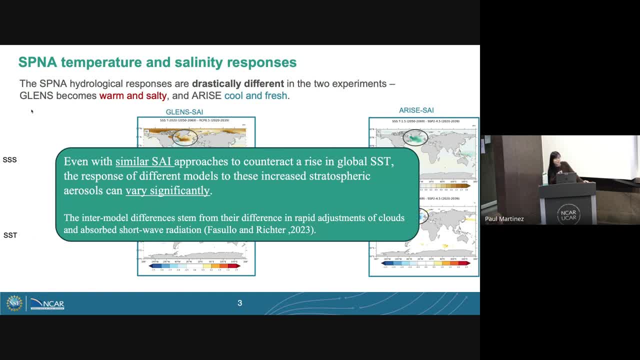 counteract the rising global SST. the response of the different models to this increased stratospheric aerosols can vary significantly, And in this case it's quite the opposite, And this, we find out, is because of it's mainly due to intrinsic model differences. 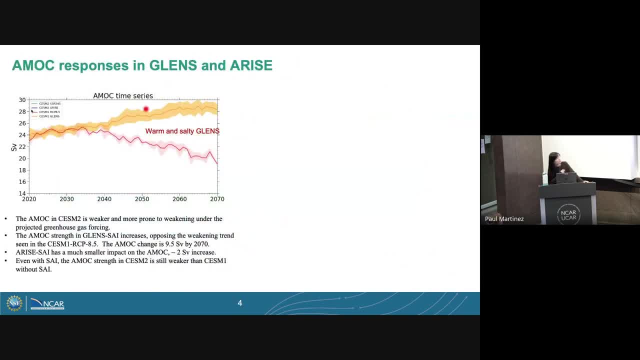 And then the AMOC responses are also very different in these two models. In the CESM-1,. so this is the red is under the reference climate, which is RCP 8.5.. We see that AMOC weakens with the warming temperature. 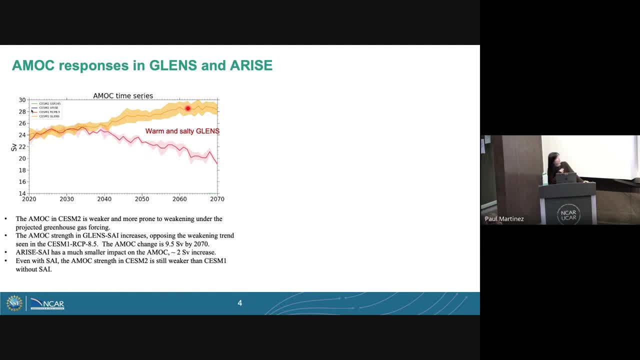 And the orange line is under the Glens SAI. So when you're adding the aerosols, the AMOC strength actually increases, opposing the weakening trend. At the end of the simulation, the difference between the two is actually 10 square drop. 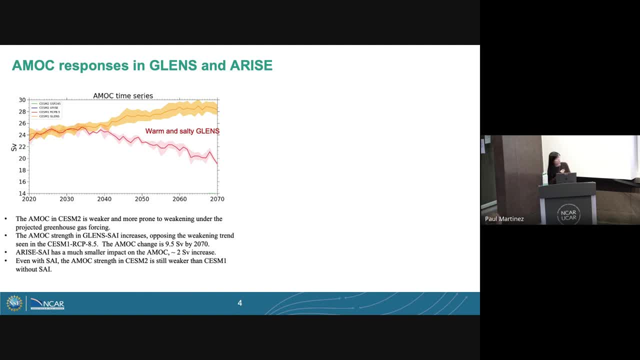 which is around 50% of the controlled AMOC strength. It's a very significant change. And then looking at the CESM-2 sets of simulations, again under the reference climate, you have a decreasing AMOC strength as shown in the green curve. 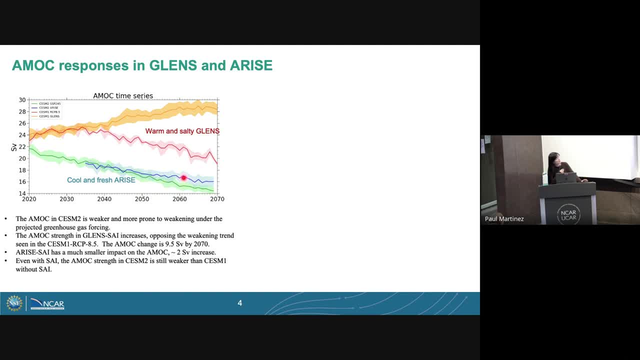 When you're adding the SAI, the weakening trend is somewhat mitigated, but the change is quite small. It's only two square drop of change. And then we also take a look at the subpolar North Atlantic freshwater content. It's kind of similar, consistent with the salinity change we saw in the previous slide. 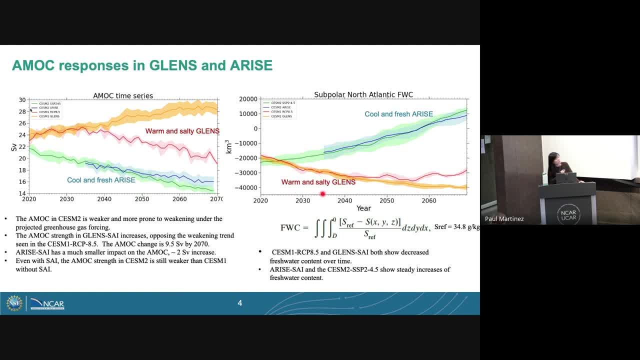 In both CESM-1 simulations we have a decrease of freshwater content corresponding to the salinification in the subpolar North Atlantic region, And then in the CESM-2 sets of simulations we see an increase of freshwater content. But if we take a look, if we compare the SAI simulation with the reference climate, 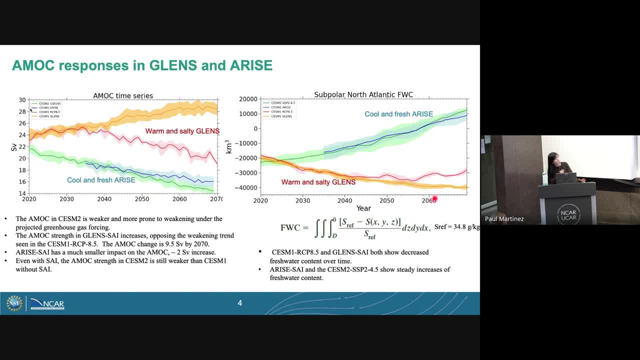 in these two sets of simulations we find that general impact of SAI is to kind of decrease the freshwater content. If you're not familiar with the freshwater content, the definition is here. It's actually the salinity anomaly compared to a reference salinity. 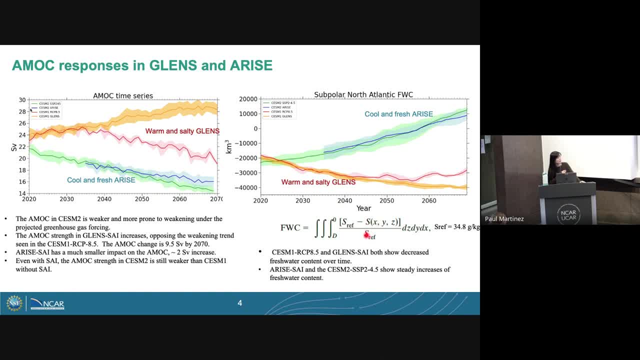 and it's integrated over this region and over the 300-meter depth in the vertical direction. So far we have seen that these two sets of SAI simulations have very different responses. But again, our scientific question is to try to, as a reminder, 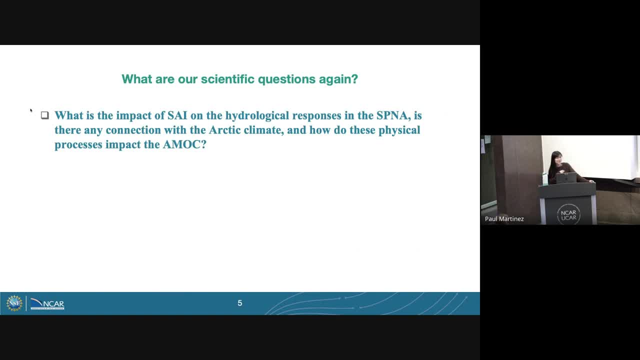 try to understand the impact of SAI on the SPNN-A region and their connections with the Arctic climate and their connections with the AMOG. So in order to do that, we kind of have to isolate the impact of SAI. So from now on, all the analysis you will see is the anomalies induced by SAI. 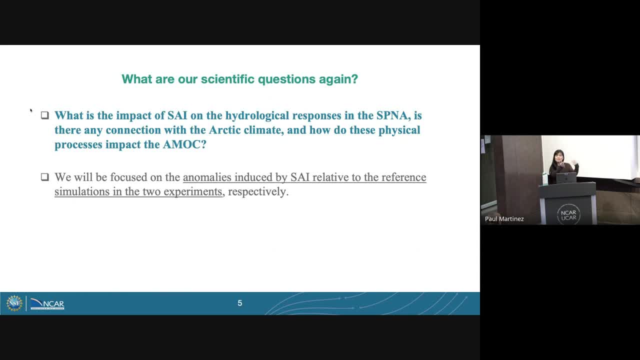 relative to the reference simulations. For example, for the CSM-1 simulation, it will be the difference between Glint's SAI and CSM-1 RCP 8.5, and the array is similar. And also, yeah, and we are going to understand the processes. 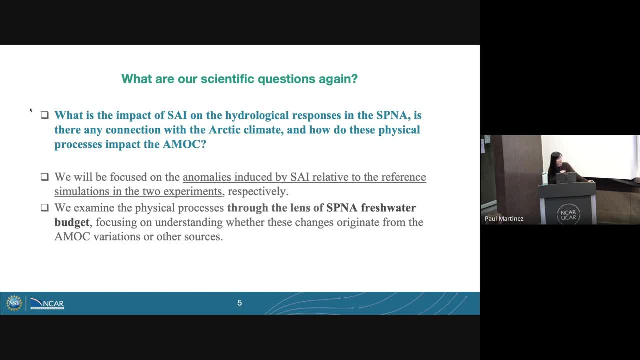 especially associated with the enhanced salinity. through the lens of SPNN-A freshwater budget analysis, We will focus on understanding the sources of the freshwater in order to understand whether these changes originate from the AMOG variations or from other sources. Okay, so the freshwater budget analyses. 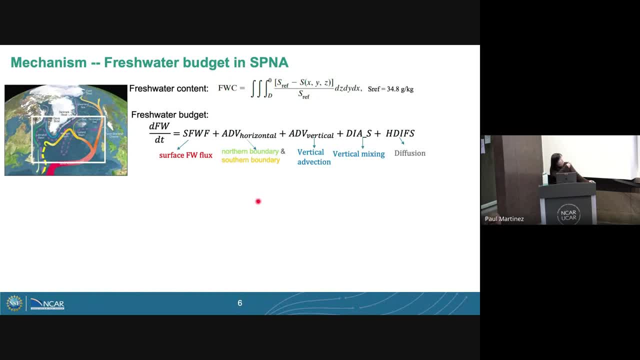 basically the tendency of the freshwater. the total term is comprised of these different terms, including the surface freshwater flux, the advection in the horizontal direction, and then vertical advection, and also vertical mixing, And then the last term is horizontal diffusion. 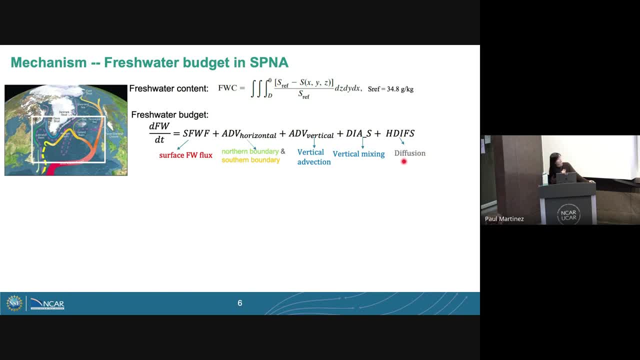 This term is quite small and is neglectable in our analyses, So we're going to take a look at all these terms in our simulation. Oh yeah, I need to mention that the horizontal advection term is also divided into the impact from the transport from the northern boundary. 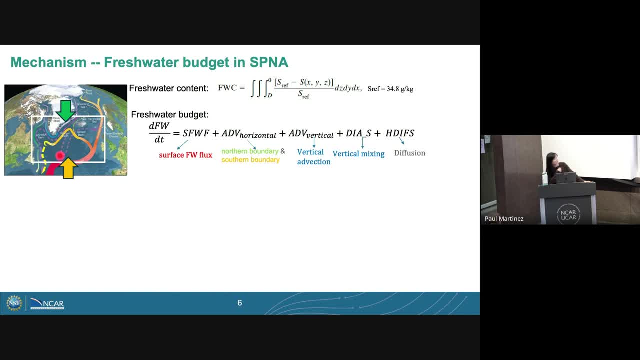 which connects to the Arctic Ocean, and the transport through the southern boundary, which connects to the Atlantic Ocean. So this figure summarizes all of these terms. Again, I want to emphasize: these are showing anomalies, the difference between the SAI simulation and the reference simulation. 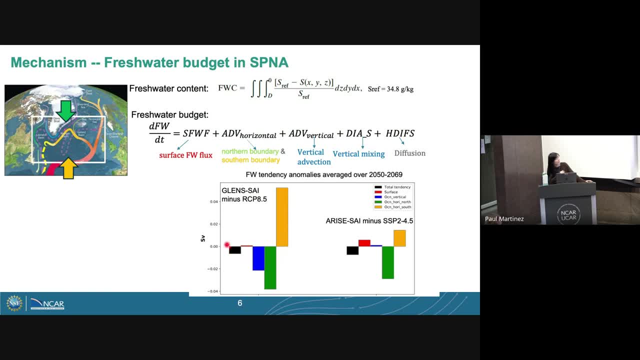 and these are averaged over 2050 to 2069.. So if we just look at the Glenn's sense of simulation for now, the black shows the total freshwater tendency. This is negative, which tells us that the subpolar North Atlantic is now losing freshwater. 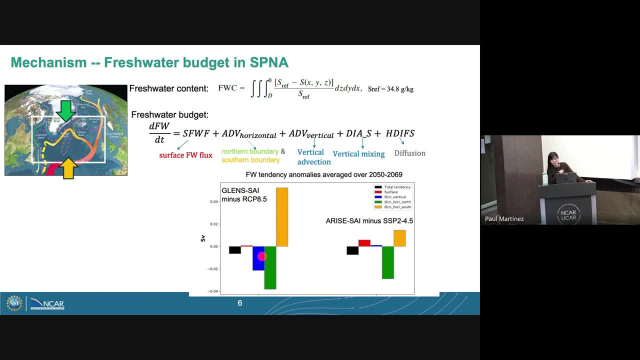 And if you look at the contributions, we see that the negative perm mainly comes from, first of all, the blue, which is the vertical processes, including vertical advection and vertical mixing, And the most significant contribution comes from advection term from the northern boundary. 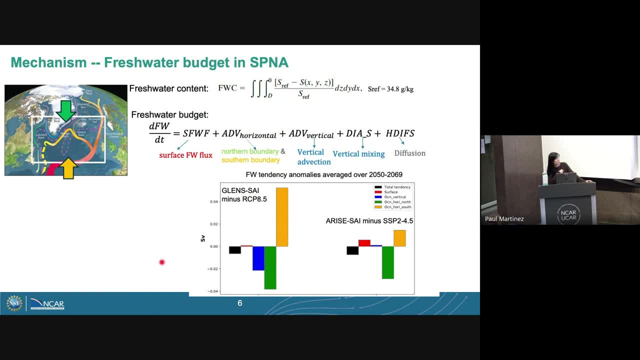 meaning that the main term that contributes to the reduction of freshwater in this region is actually a reduction of freshwater import from the Arctic region, which is quite surprising to me at least, because at first I thought the increase in AMOC may have contributed to the reduction of freshwater in this region. 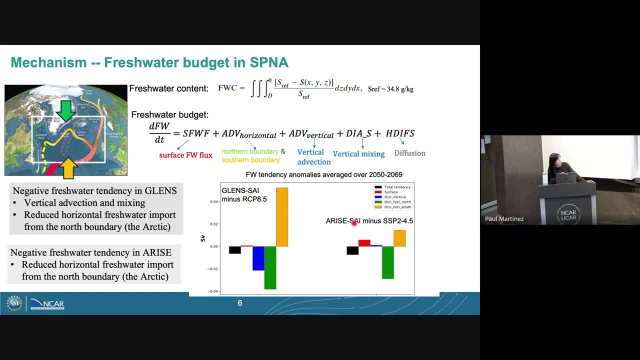 Yeah, this is what I said. And for the Arise simulation we found a similar response, although the contribution from the surface freshwater is different in these two simulations. So now we see that in both cases the freshwater decrease in the subpolar North Atlantic region. 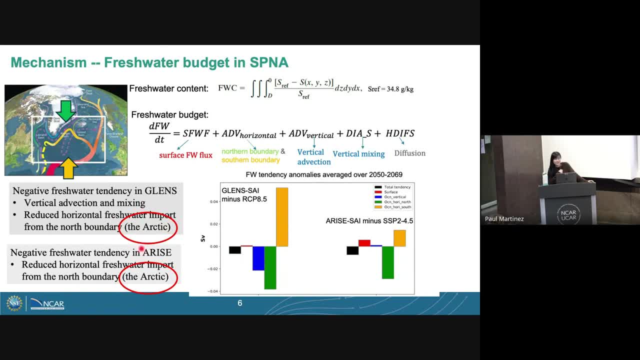 are both closely connected to the Arctic climate. So what happens in the Arctic? Why do we have reduced the freshwater transport from the Arctic to the subpolar North Atlantic region? So next we're going to take a look at the Arctic Ocean. 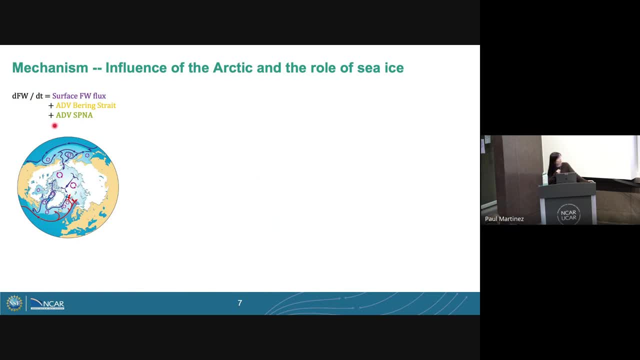 We're still going to use a freshwater budget analysis to look at what happens, But the main terms in the Arctic freshwater budget include, first of all, the surface freshwater flux and also advection through the Bering Street in this part and the advection through the SPNA region. 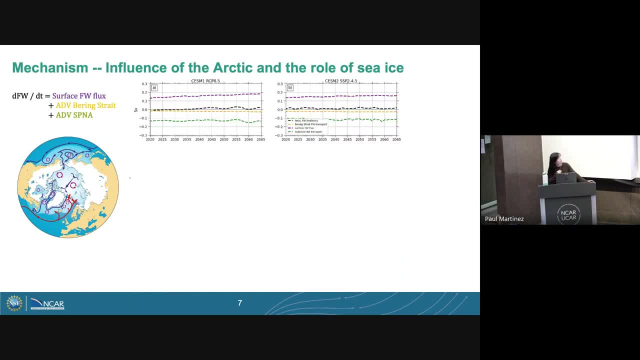 which is the part we care the most. So here these two panels are showing what the budget terms look like in the reference climate. just to give you an idea that in the normal climatology the total freshwater budget in the black is mainly balanced by a positive term. 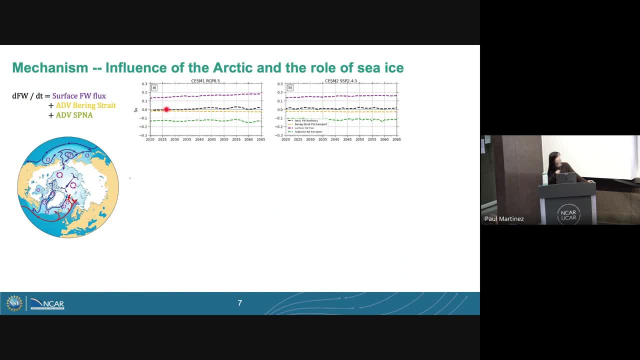 from the freshwater surface flux. You've got freshwater from surface fluxes and then it's largely balanced by the transport outside the Arctic Ocean into the North Atlantic. That's what happens in the reference climate, And now here we're looking at the differences. 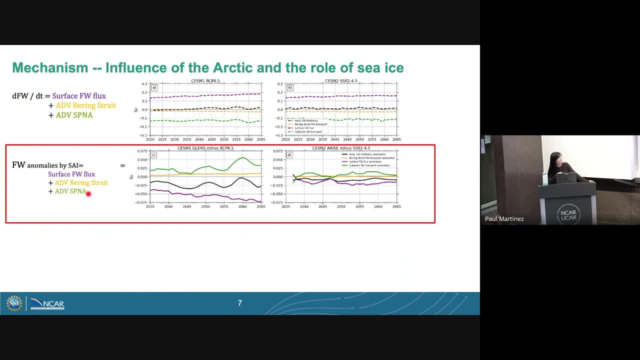 the impact induced by the SAI. So, first and foremost, for the black, the total change we see is negative, meaning that Arctic is also losing freshwater. So the main term that leads to this decrease of freshwater we saw is this: purple. Purple is the surface freshwater flux. 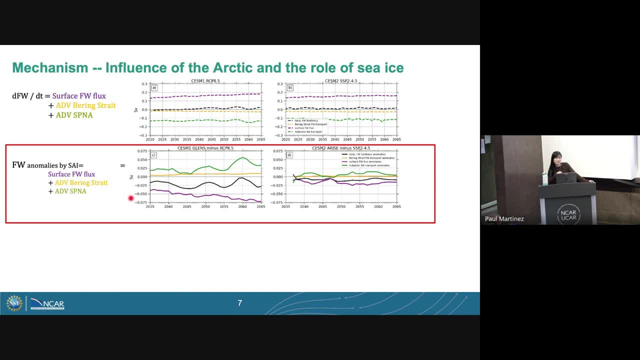 So this tells us that there is a significant decrease of surface freshwater flux into the Arctic Ocean and in order to balance this freshwater loss, we would have this green term becomes positive, which is an eviction through the subpolar North Atlantic. So from here we see that the reduced freshwater export. 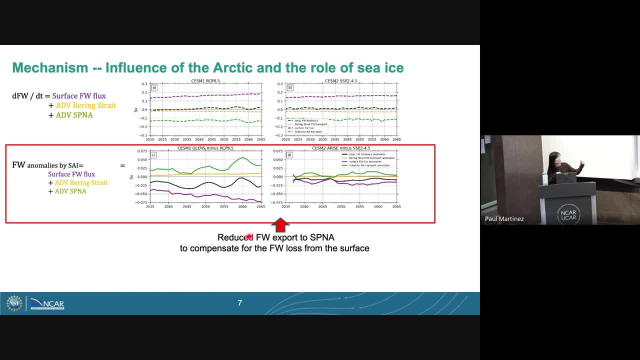 from the Arctic to the SPNA is because it has to be. it has to compensate for the freshwater loss from the surface. So the same process is found in the ARISE simulation, just because this one has a more pronounced response. So we'll just focus on this one. 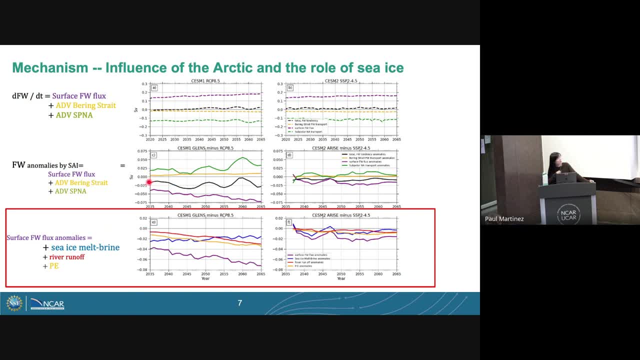 But then we're also curious to what happens to the surface freshwater flux. What causes this significant reduction? So we take a look at this different component, mainly the sea ice processes: sea ice melting minus brine rejection. The second term is river runoff. 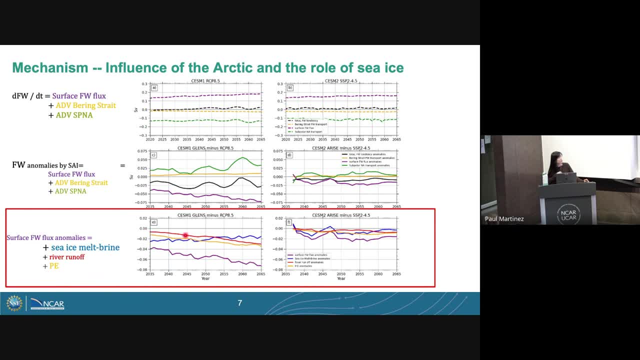 and the third term is precipitation minus evaporation. So again, this purple is the same as this purple is the total freshwater flux decrease. And then we see all of these three terms actually contribute to this decrease, But their contributions kind of vary with time. 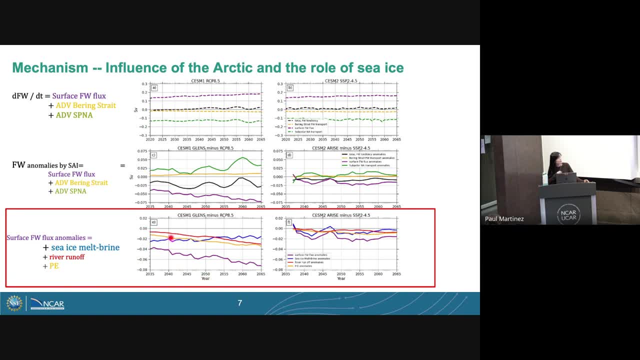 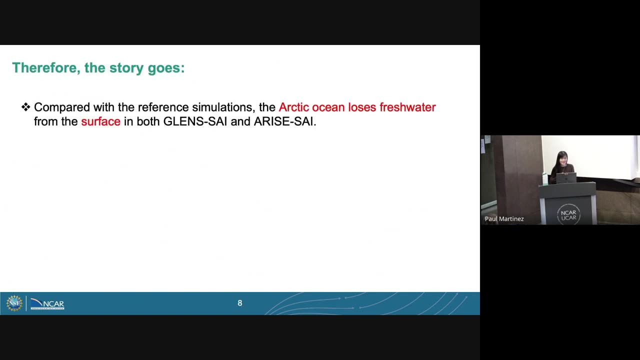 In the first half of the simulation the sea ice processes contribute most to the reduction of freshwater flux, But then later on the river runoff, MPE kind of caught up. Okay, there's quite a lot To summarize what just happened. we found that, compared to the reference simulations, 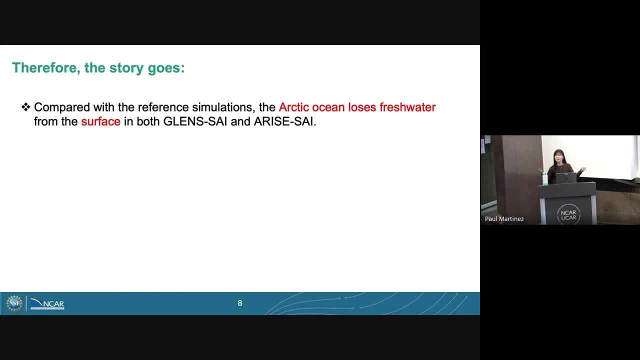 the Arctic Ocean has significant loss of freshwater from the surface, And then we found that the reduced surface freshwater input is due to partly sea ice growth, partly due to the changes in surface precipitation minus evaporation, and also river runoff, And then in the Arctic. 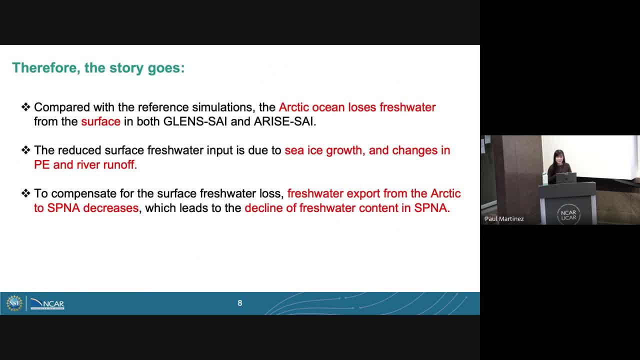 to compensate for the surface freshwater loss, your freshwater export from the Arctic to the subpolar North Atlantic decreases, which ultimately leads to the decline of freshwater content in the subpolar North Atlantic, And that's why we see a solidification in that region. 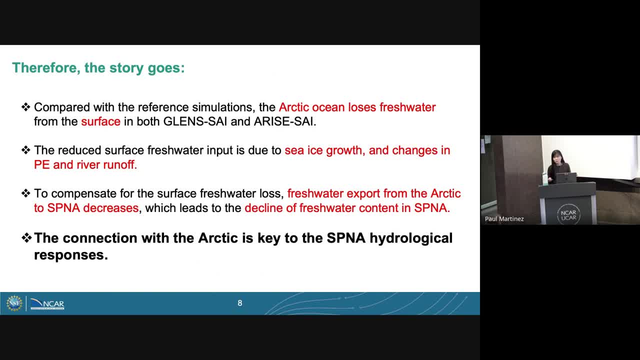 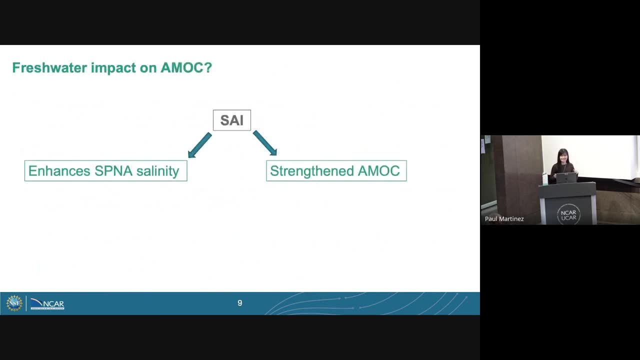 So surprisingly, at least to me, the connection with the Arctic is actually key to the SPNA hydrological responses we saw in the SAI simulations. This needs to be more dramatic. Okay, if we still have time. Okay, maybe not. 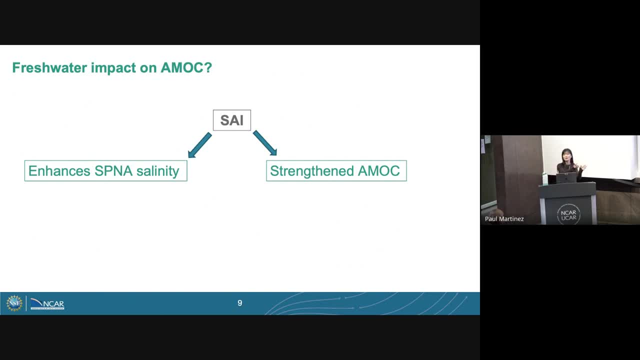 Anyways, we're also interested to find out, you know, the solidification we saw in these SAI simulations. are they contributing to the AMOC stream strengthening, or if the AMOC stream can contribute to the salinity? Well, at least for this part, 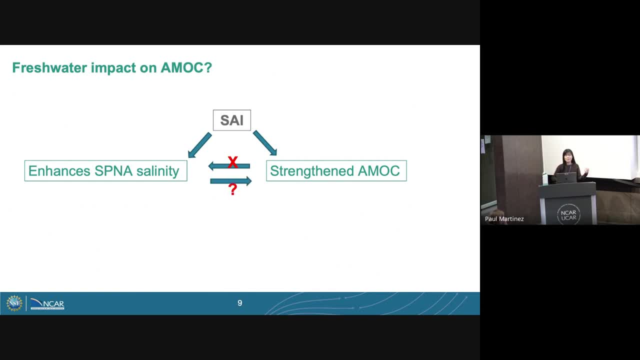 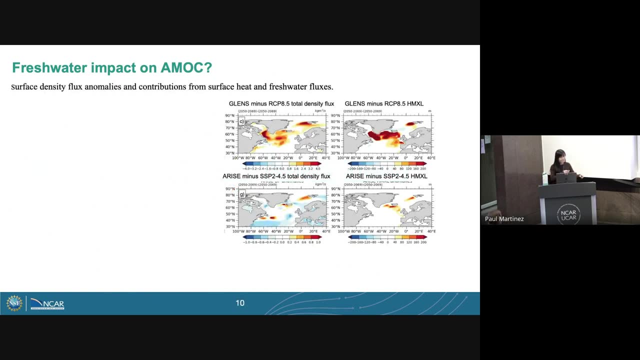 we already know it's not the case, because the Arctic is the main player, But the other way. we kind of want to understand this process by analyzing the surface density flux. So I'm just going to go briefly. The SAI induced increased surface density flux. 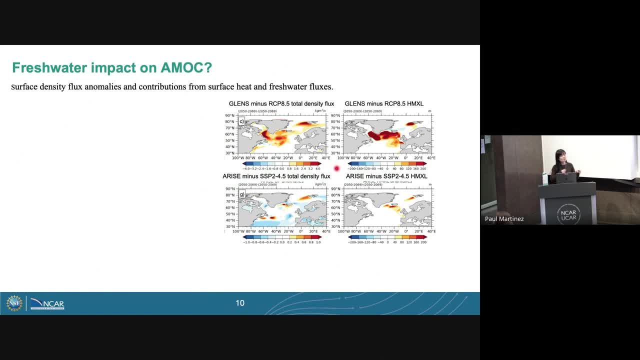 into this region, which will lead to stronger ocean deep convection and probably to stronger AMOC, And we decompose this part into the contribution from the surface heat flux and the contribution from the surface fresh water flux and found that the majority of these changes 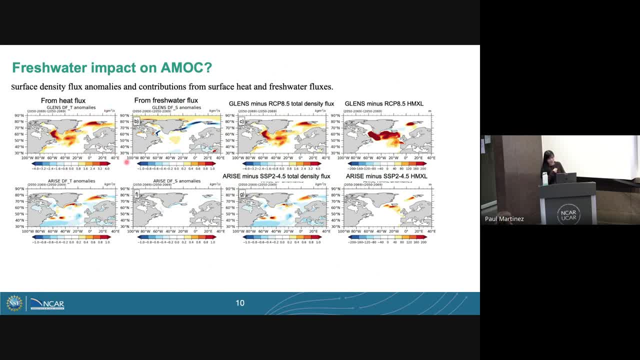 are actually due to surface heat flux. So even though we're seeing the hydrological responses act to reduce the upper ocean fresh water content and increase density, it only plays a small part. The heat flux is what drives the AMOC changes in this case. 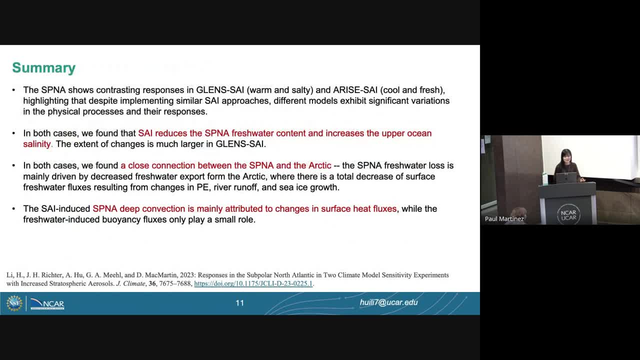 Okay, That's all I have. This is the summary. I'll just leave it here in case it you know. We have one quick question. Yes, Oh yeah, I have a quick question. It seems like in both SAI experiments 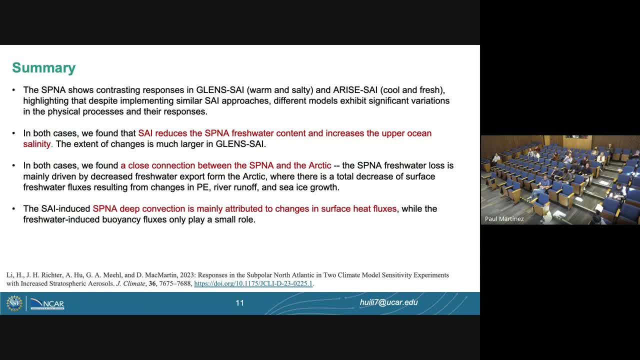 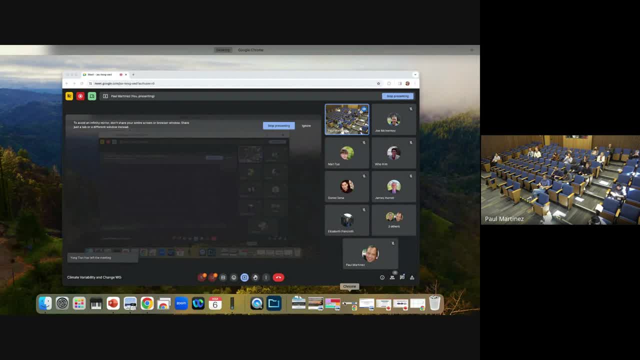 it basically like it seems like the effect has just a lot smaller in that region than like the rest of the globe. So like it seemed like is there a reason why SAI impacts that region so differently than the rest of the globe? 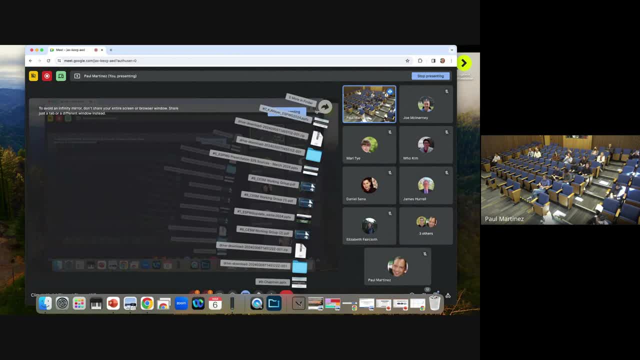 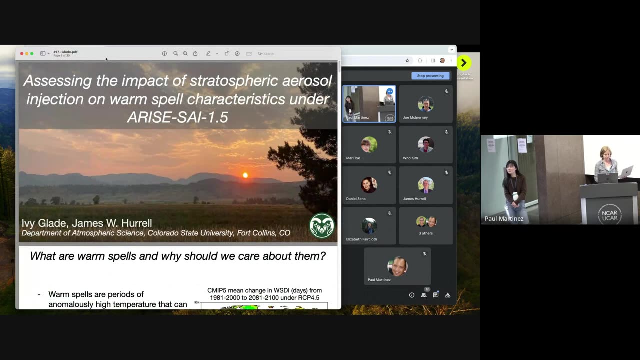 It seemed like a very bull's-eye place where SAI was doing something different. Yeah, So from actually John and Yaga's paper, they actually looked a little deeper into this region. It seems like it's the differences in the rapid response of the clouds to the CO2. 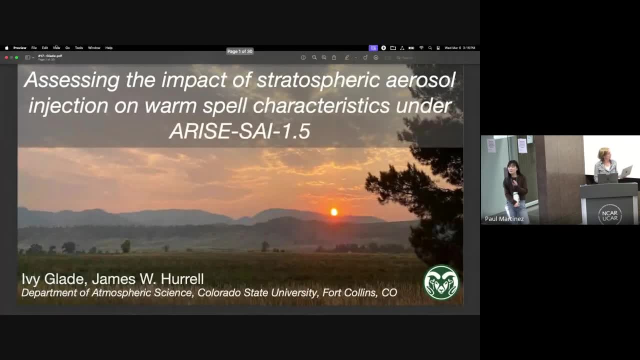 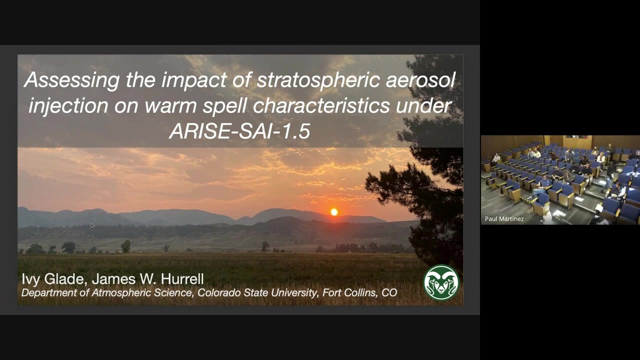 and to the aerosol forcing. So essentially it's because of the model of physics. I would say Yeah, Okay, Yeah, And that also explains why these two models kind of have opposite responses. All right, Yeah, All right. 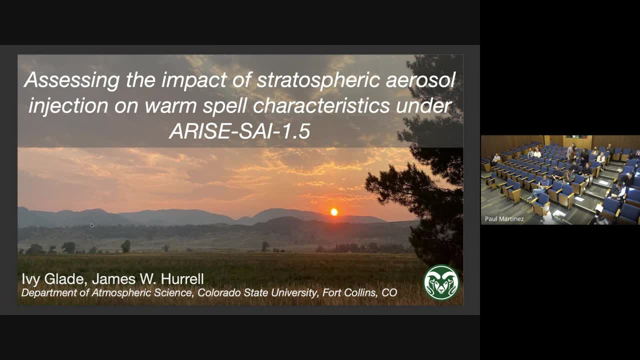 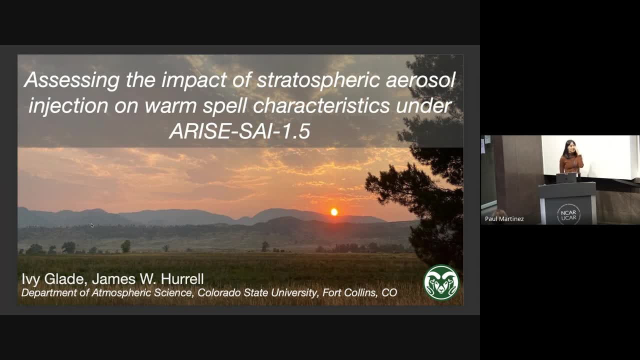 Okay, Hi, I'm Ivy. I'm a graduate student in the Department of Atmospheric Science at Colorado State in Fort Collins, And today I'm going to be talking about the potential impact of stratospheric aerosol injection on the characteristics of warm spells. 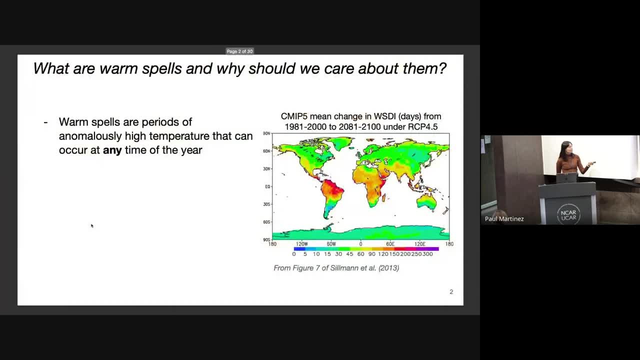 under one scenario of SAI. And so, to start off, what are warm spells and why should we care about them? Warm spells are periods of anomalously high temperature that can occur at any time of the year, And we should try to understand these events. 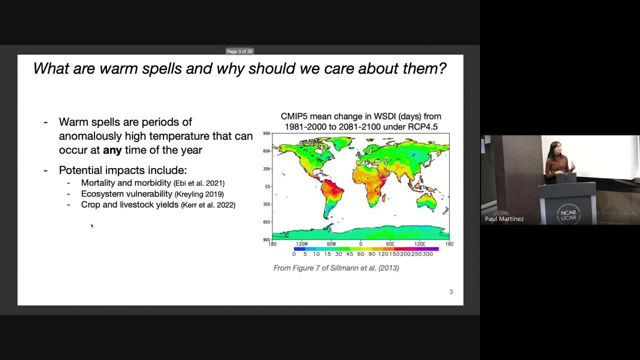 in the context of both like a current and future climate, because they can have impacts on things such as human mortality and morbidity, ecosystem vulnerability and crop and livestock yields. So warm spell events are actually projected to increase in frequency as the climate continues to warm. 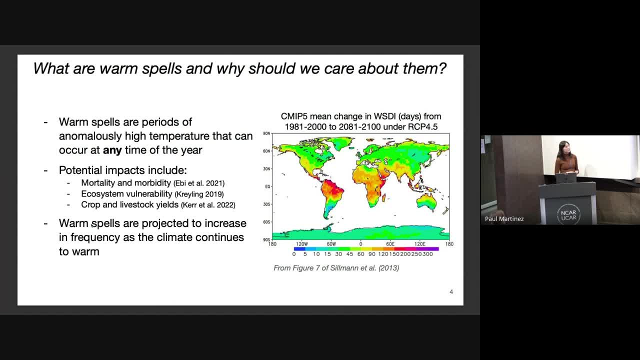 And this is shown in this figure I have on the right which shows the CMIP5 change in warm spell days at the end of the century relative to the beginning of the century, And we can see that warm spells are increasing everywhere across the globe. 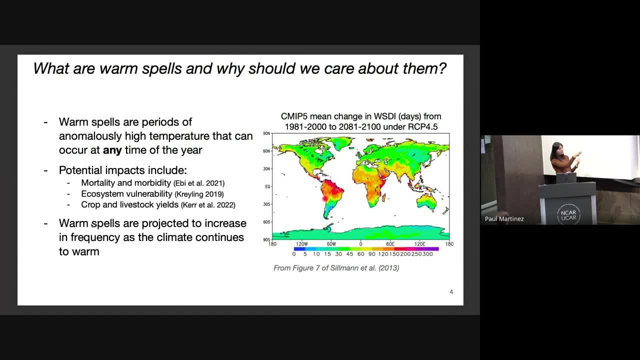 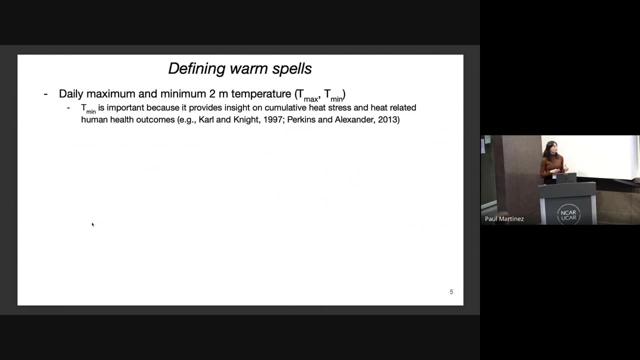 and that the increases are largest in the tropics, where sometimes the increases could even be in excess of 200 days. So these sort of events are increasing a lot as the climate continues to warm, And so to more specifically define warm spells in the context of my work. 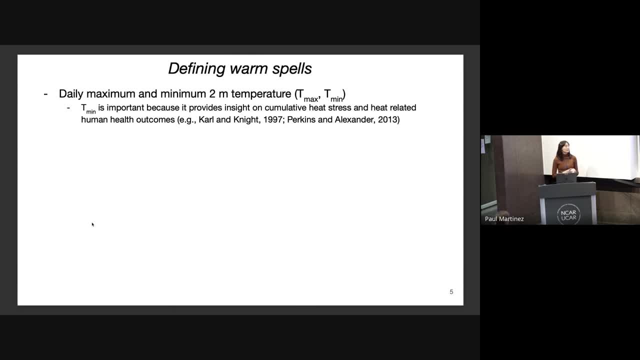 I use daily maximum and minimum two meter temperature to define these events And I use daily minimum temperature in addition to daily maximum temperature because it's an important it can provide, like some insight into potential human health outcomes, And I use these temperature metrics to find when these warm spell events occurred. 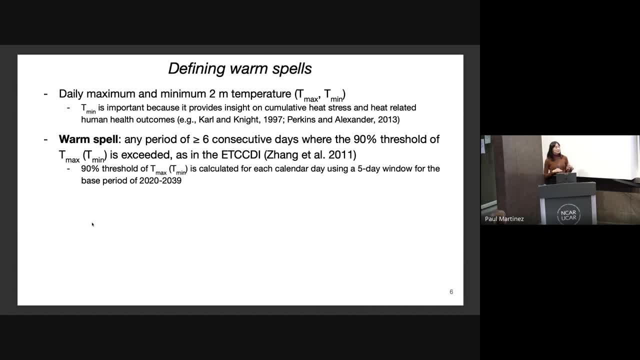 which I consider to be any period that was at least six days in length where the 90th percentile threshold of daily maximum or minimum temperature was exceeded, And I calculated the 90th percentile of daily maximum and minimum temperature using the 2020 to 2039 time period. 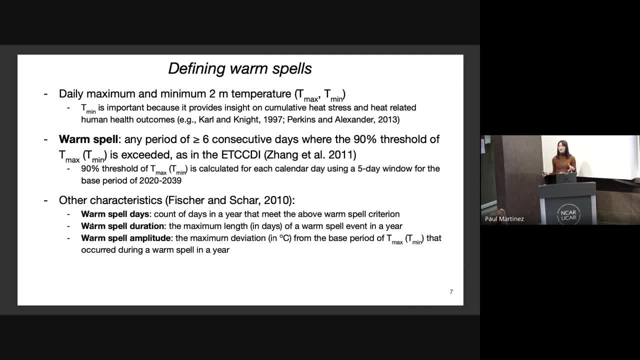 And, in addition to looking at just the occurrence of warm spells, I also looked at several different characteristics, which included warm spell days, warm spell duration and warm fill amplitude. And so because climate risks are increasing as the climate continues to warm, and one of those risks are that warm spells 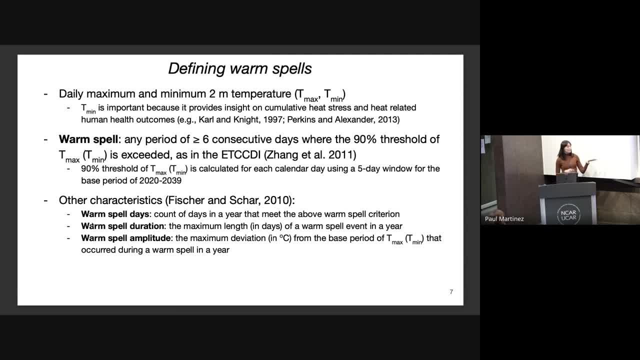 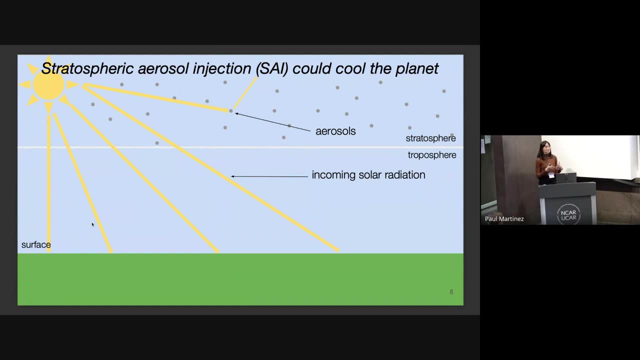 are projected to increase in frequency, it's important that we potentially understand how these might be impacted by potential climate intervention methods, And so, as sort of presented previously, I'm going to be looking at how warm spells might be impacted by the deployment of stratospheric aerosol injection, or SAI. 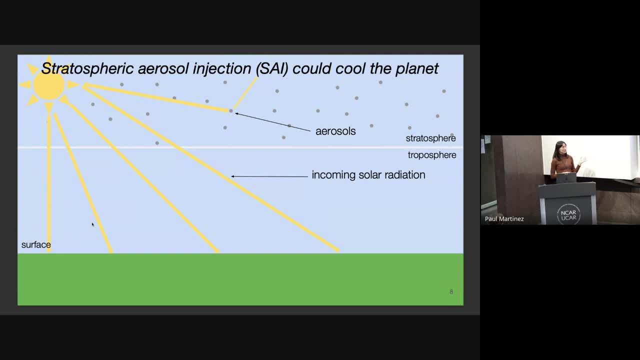 And SAI would cool the planet by injecting particles into the stratosphere that would reflect a small amount of incoming solar radiation away from the Earth. I also just wanted to note that methods of climate intervention such as SAI are just seen as a method to potentially avoid. 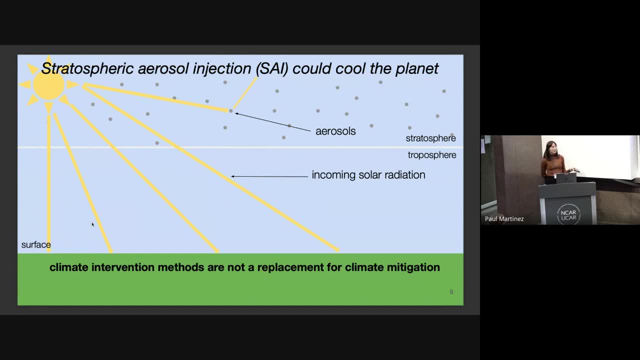 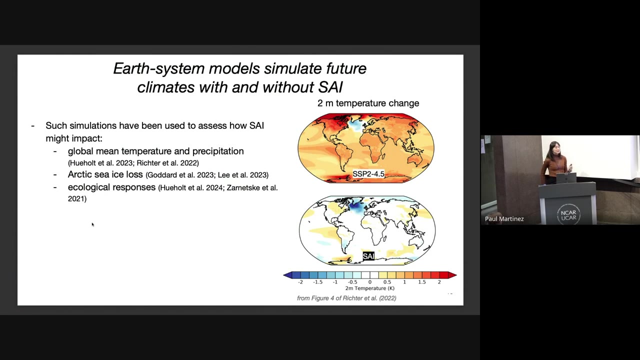 the worst negative consequences of climate change, and also to provide more time for the development and deployment of climate mitigation strategies. And so there have been several sets of Earth system model simulations that have looked at the potential impacts of SAI on things like global mean temperature. 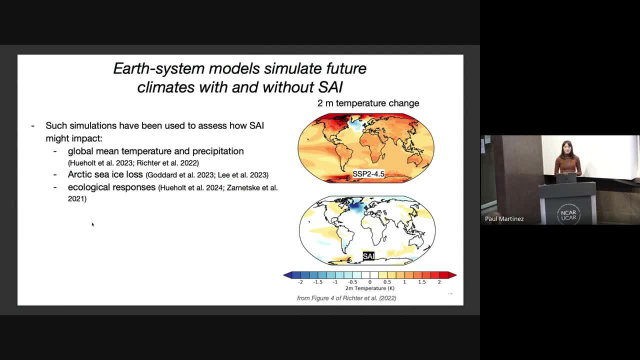 and precipitation, Arctic sea ice loss, as well as ecological responses. Additionally, some research has examined how SAI might impact things such as extreme weather phenomena, But none of this research has specifically looked at how SAI might impact warm spell events and their characteristics at a global scale. 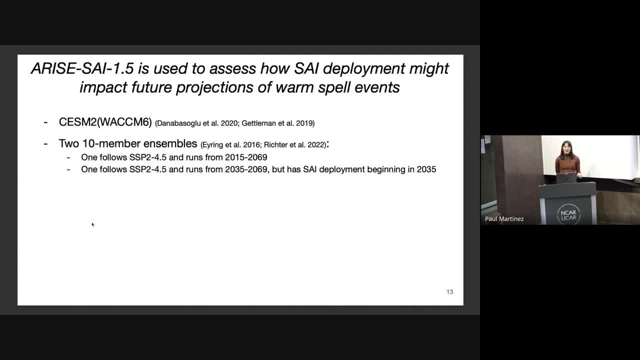 And so I did that using the ARISE SAI 1.5 simulations, and these were run using CSM2 with Wacom 6 as the atmospheric component, And these simulations feature two 10-member ensembles, one which follows the moderate and policy-relevant 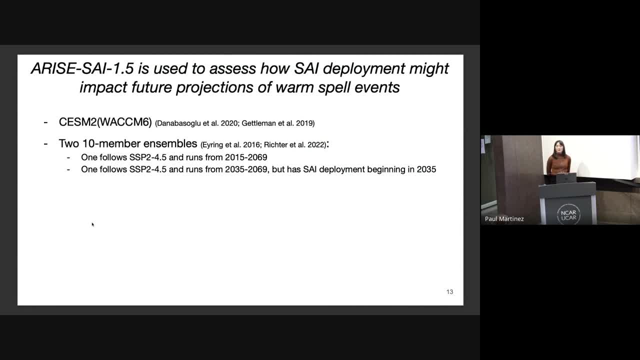 SSP24.5 emissions scenario that runs from 2015 to 2016.. And the other one, which also follows SSP24.5, but that has SAI deployment beginning in 2035.. And so the deployment goals of ARISE SAI. 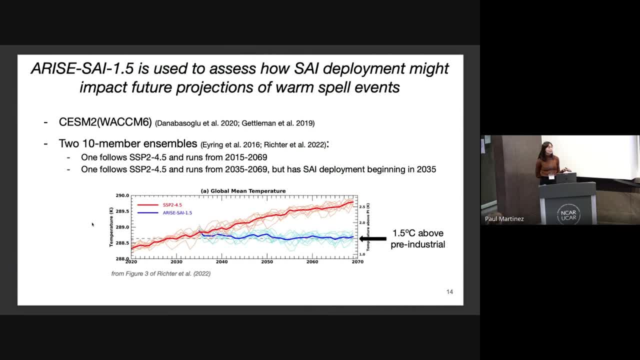 are to maintain global mean temperature at around 1.5 degrees Celsius above pre-industrial, which corresponds to the 2020 to 2039 mean in the model And that's shown in this figure clearly, which is a time series of global mean temperature. 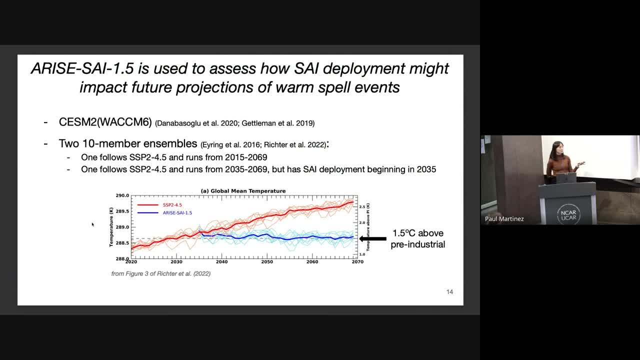 where the red line shows future projections of temperature under SSP24.5.. And then the blue line shows the time series of temperature in the simulations where SAI is deployed. And so, yeah, I just also wanted to note that I used the 2020 to 2039 period as my reference period. 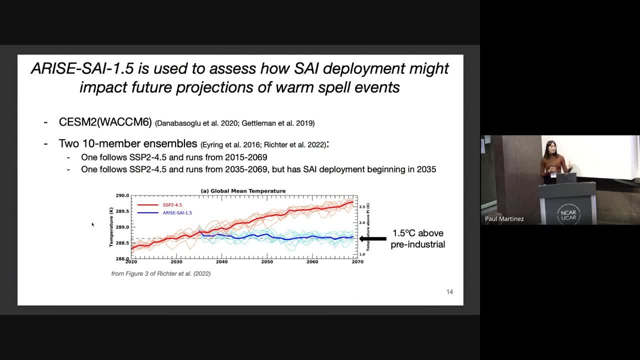 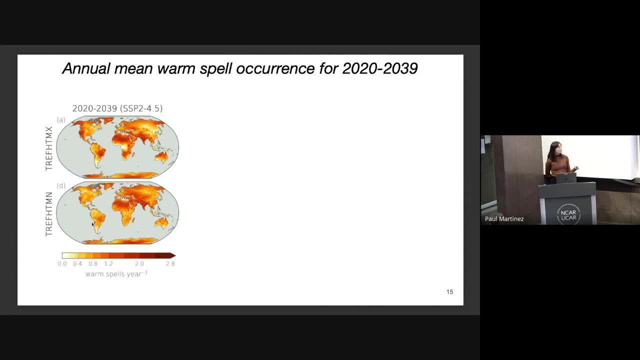 for calculating these events in order to be in line with the deployment goals of these simulations. And so to hop straight into the results, these two figures are showing the annual mean warm spell occurrence for 2020 to 2039.. And the top figure is showing this for warm spells. 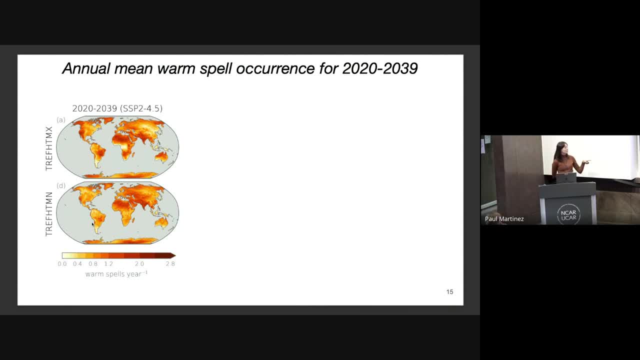 defined by the daily maximum temperature, And the bottom figure is showing this for warm spells defined by the daily minimum temperature. And so I guess what I just wanted to note with these figures is that during this time period, warm spells are relatively rare events. 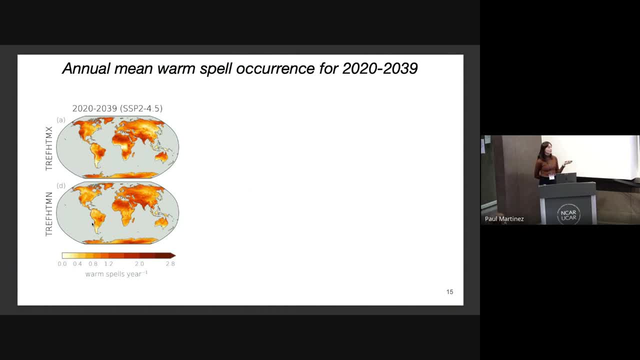 but they do occur most frequently over regions such as Saharan Africa, the Indian subcontinent and Western North America. And then we can see that under SSP24.5, warm spells are projected to increase in frequency, where this center column of figures is showing the change. 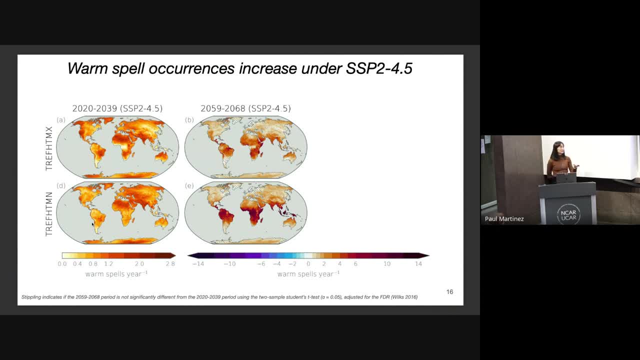 in warm spell event occurrence for 2059 to 2068 relative to the base period. I also just wanted to note here that the frequency of warm spell events increases more for warm spells defined by the daily minimum temperature than for warm spells defined by the daily maximum temperature. 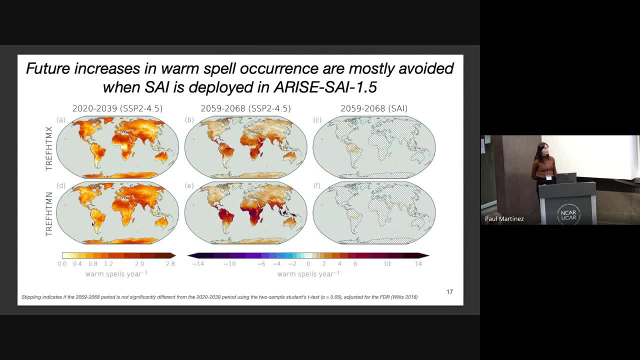 And then in the simulations where SAI is deployed, most future increases in warm spell events are avoided. And I also just wanted to note here that the stippling on my figures indicates regions where the 2059 to 2068 period is not statistically significantly different. 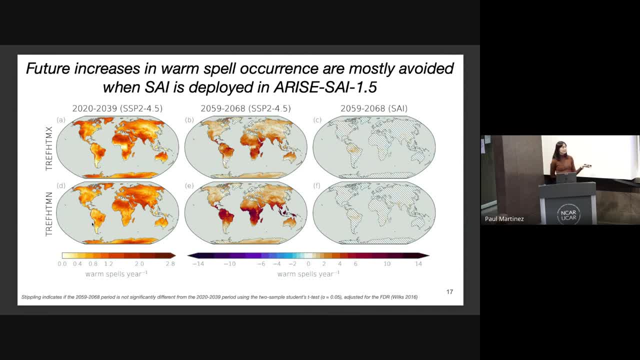 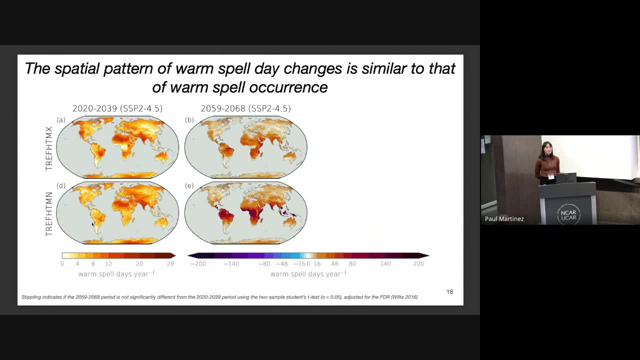 from the base period, and I calculated this significance using the two sample students' details, And so I also looked at how warm spell days are projected to change with climate change, where I defined warm spell days as the count of days in a year that occurred during a warm spell event. 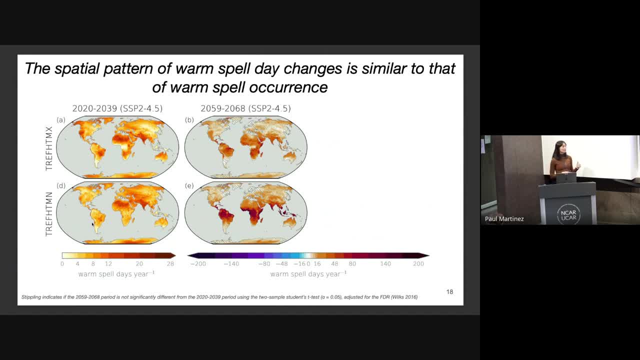 And so we can see that warm spell days increase in frequency in a way similar to that of warm spell event occurrences, where the magnitude of change over the time period is relatively large and the future changes are also widely statistically significant. And then again, when SAI is deployed. 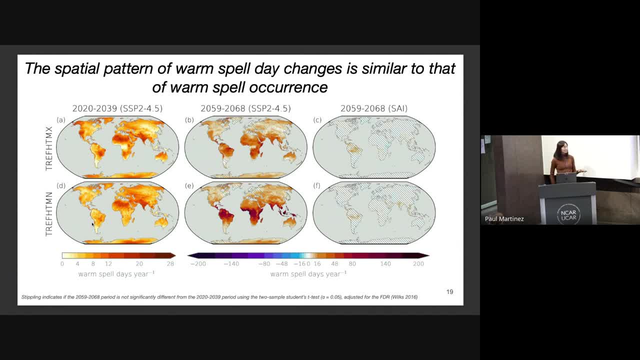 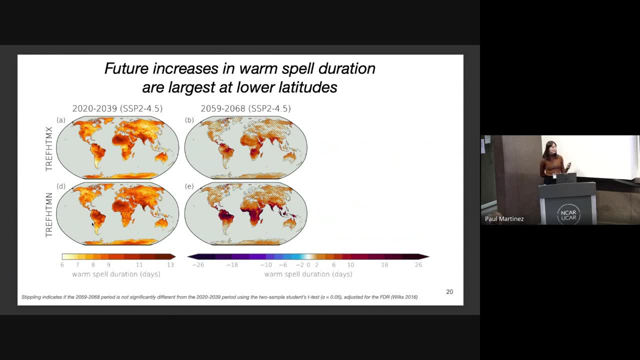 we see that most of these increases are avoided, And so I also looked at warm spell duration, which is the longest warm spell event in days that occurred in a given year, And so, again, we see that, under climate change, the length of these events are increasing. 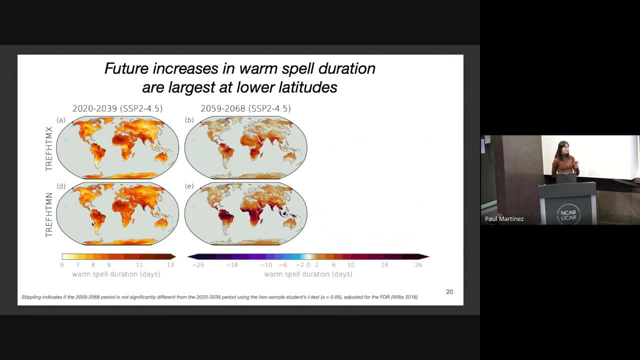 but I wanted to note that the relative change compared to warm spell event occurrence in warm spell days is relatively small, where the increase is only about two times the highest magnitude of the base period for warm spell duration, but for warm spell occurrence in warm spell days it was as high. 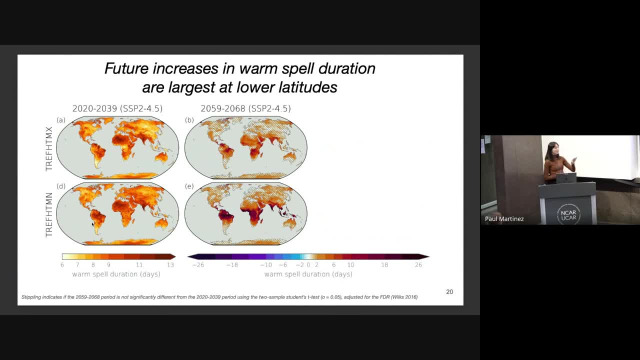 as an order of magnitude, And we can also see that some of the changes are not as widely statistically significant. Again, though, when SAI is deployed, most of the future increases in warm spell duration are avoided, although there are still some subtle regional changes present. 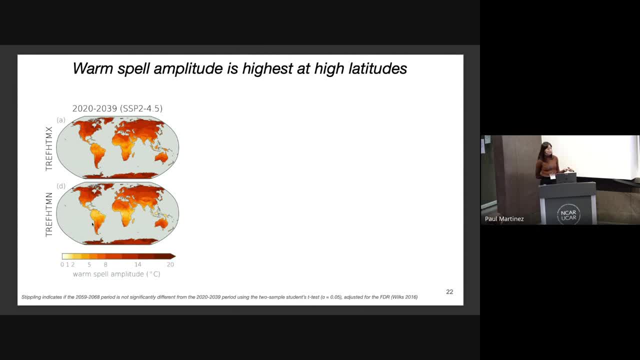 And so the final warm spell characteristic that I looked at was warm spell amplitude, which I defined as the largest deviation of daily maximum or minimum temperature from the 2020 to 2039 mean of each parameter, And something to notice in the baseline is that warm spell amplitude, like climatologically, 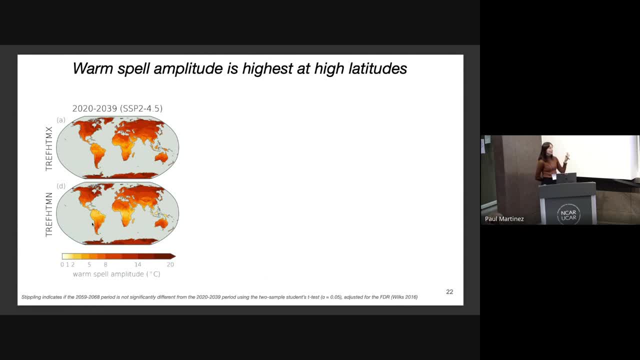 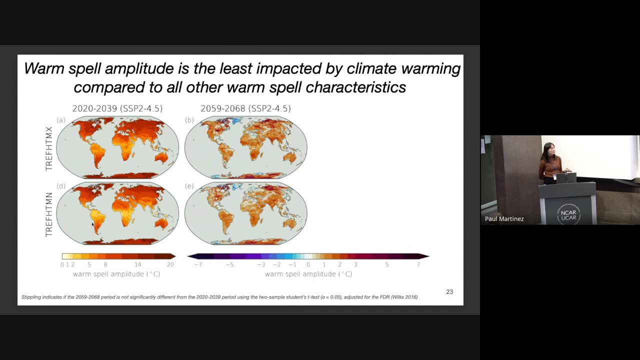 is largest at the higher latitudes, and this is sort of in contrast to with the other warm spell characteristics that I've looked at so far. And then with climate change, again we see that warm spell amplitude is projected to increase in magnitude. 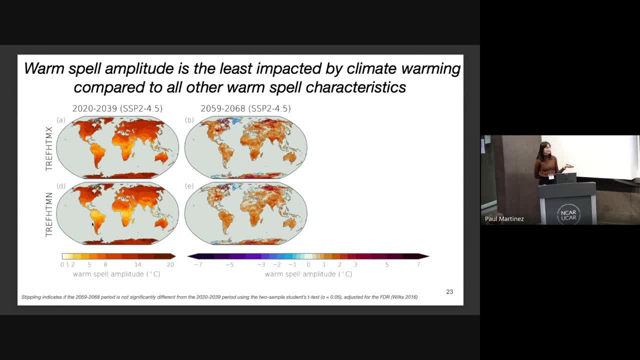 but, similar to with warm spell duration, the relative magnitude of increase is less than with warm spell occurrences or warm spell days. And then when SAI is deployed, similar to with warm spell duration, most of the increases are avoided, although there are still some regional changes. 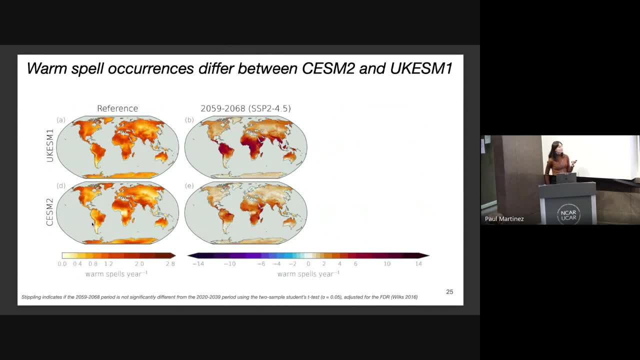 And so I also looked at future projections of warm spell occurrence using a different model but that ran simulations with the same SAI deployment and climate change scenario, and that is the UK Earth System Model. So this figure shows, or these figures show future changes. 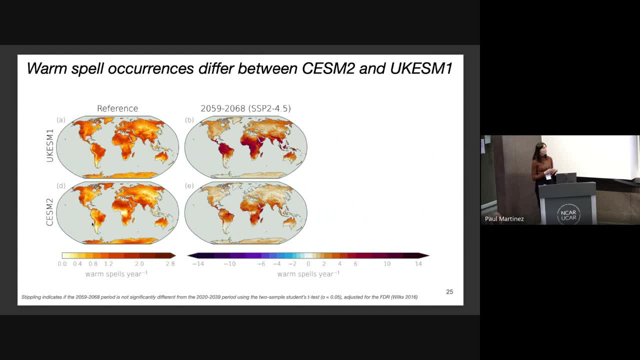 in warm spell occurrence for warm spells defined by the daily maximum temperature in UK ESM. So we can see that the changes in warm spell occurrences in UK ESM-1 and UK ESM-2 are the same as in UK ESM-2. 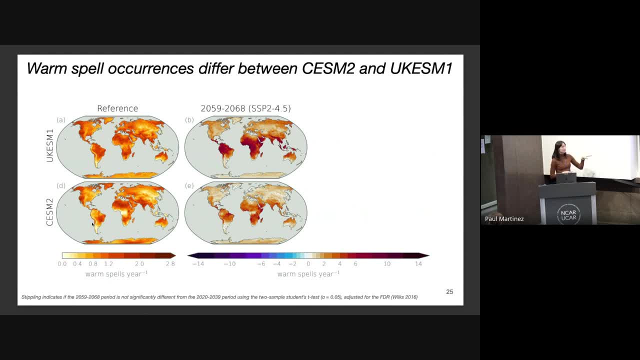 on the top row and then CSM-2 on the bottom row, And if you look at the middle column, which shows the changes at the end of the simulation period relative to the reference, we can see that there are some distinct differences in the future changes. 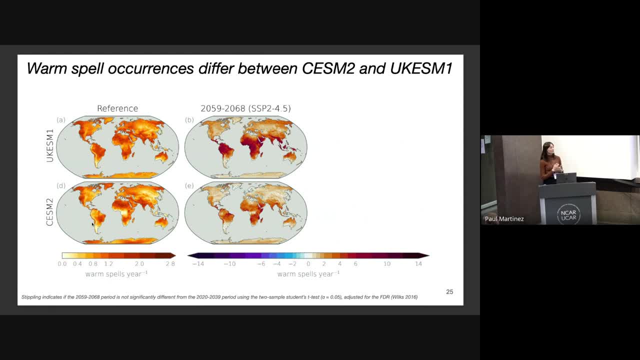 in warm spell event occurrence where, like: firstly, what you can notice is that the changes in the temperature are not the same as in UK ESM-1. And this is just likely due to the fact that UK ESM-1 has a higher climate sensitivity. 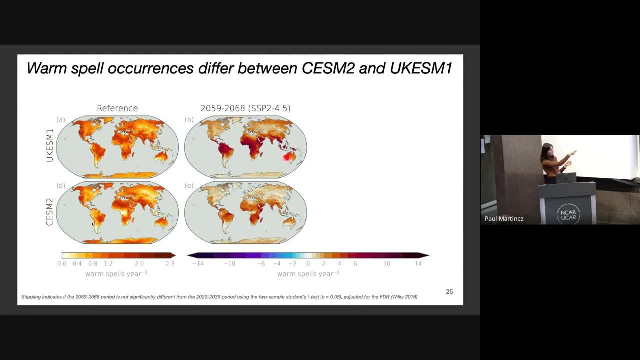 than CSM-2.. And then the other thing I want to point out, which is probably more interesting, is that in some regions, such as like this sort of like Sub-Saharan Africa region, as well as Southeast Asia, 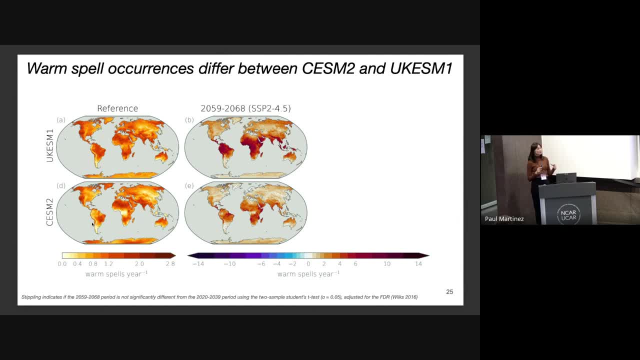 you see that in UK ESM-1, those areas have some of the highest magnitudes of projected increases in event frequency, whereas the magnitude of change is actually relatively small. And there are also some differences in how SAI deployment might impact future projections of warm spells. 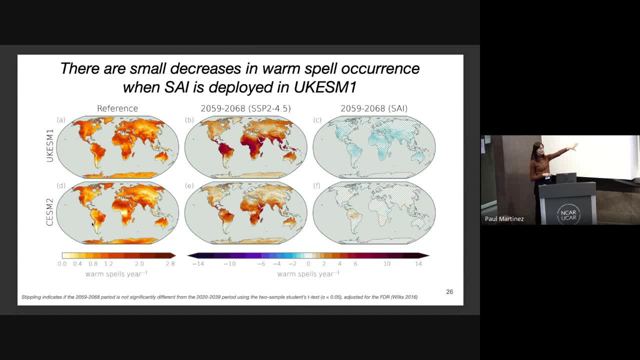 in these two models where you can see distinctly that in the UK ESM model simulations SAI deployment seems to like slightly overcompensate for future increases in warm spell occurrence under SSP 2.4.5.. And so to conclude, 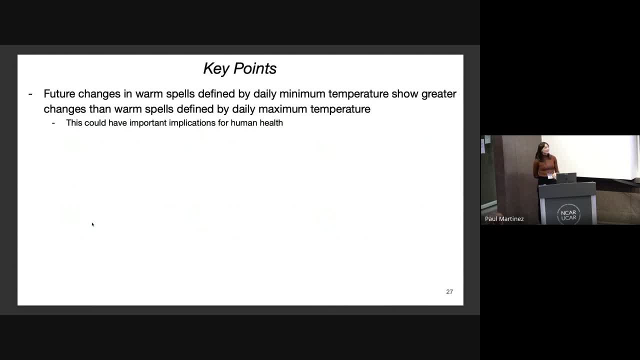 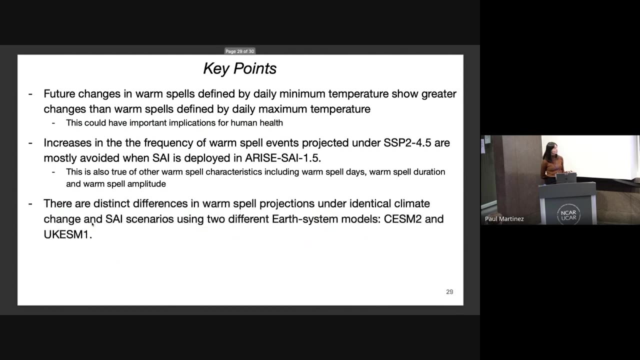 changes in warm spells defined by daily minimum temperature show greater changes than warm spells defined by daily maximum temperature. Increases in the frequency of warm spell events projected under SSP 2.4.5 are mostly avoided when SAI is deployed in these simulations, And there are distinct differences. 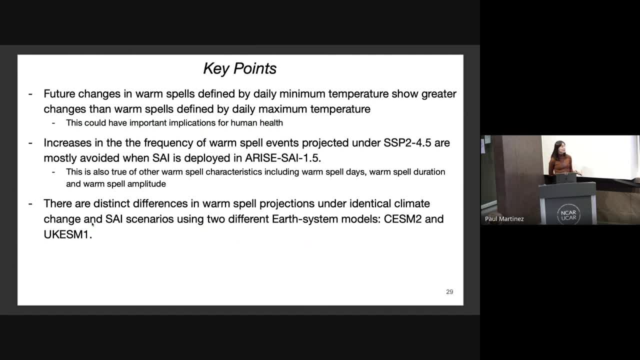 in warm spell projections under two identical climate change and SAI scenarios using CSM-2 and UK ESM-1.. And then future work might investigate the drivers behind the differences in the spatial pattern of warm spell events in these two models. Yeah, great talk. 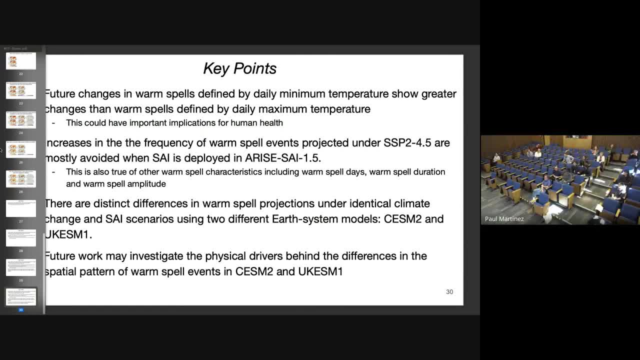 For the CSM versus UK ESM differences. I'm trying to remember: was the controller for the ARISE in the UK ESM? was that responding to changes in that model or was it the same amount of sulfate as in CSM? 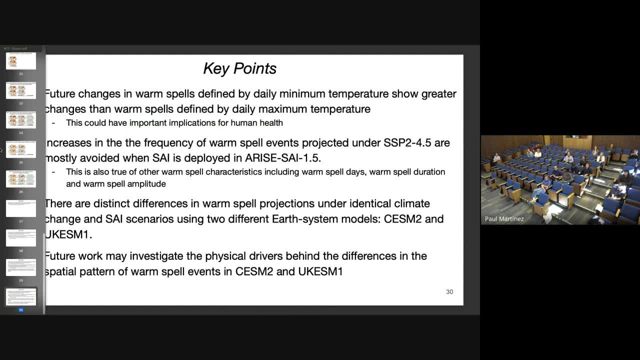 Because that could account for some of the. Yeah, it was responding to in UK ESM specifically, So it was different amounts of sulfate in both models. So, yeah, that could potentially be a part of it. When you were looking at the. 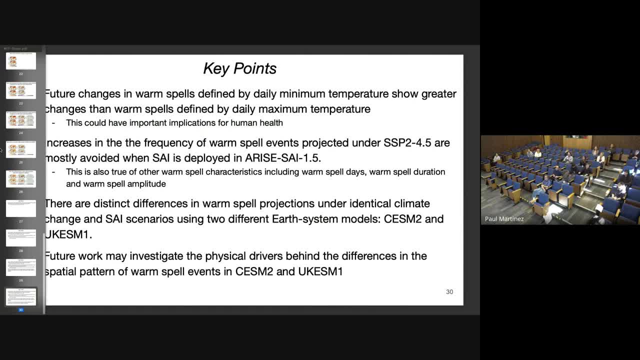 SAI scenario. in the first metrics for CSM-2, it looked like the Amazon was a region where it wasn't statistically significant, but there was still a lot of red under SAI And I'm wondering: is there a reason for that? 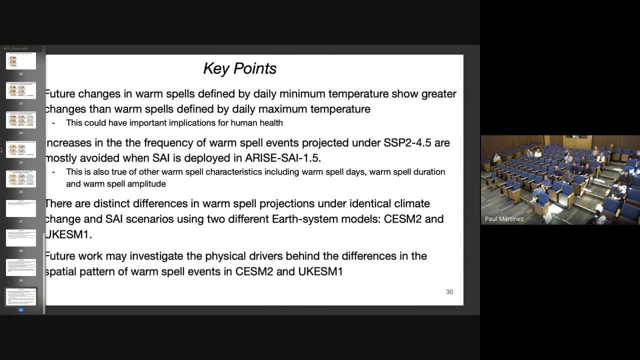 Is there land use changes? Is there some kind of non-reversibility? Yeah, so I think that's a great point and we've noticed that as well. I haven't looked into it yet, but I'm hoping to look into it. 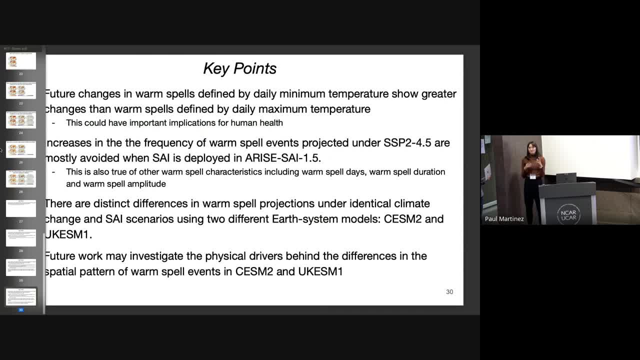 and I think that you're kind of on the right track of it- could be related to potentially land use or land cover changes. I just haven't looked into it to confirm whether or not that's true. Thank you, Could you comment on? I'm putting it out there. 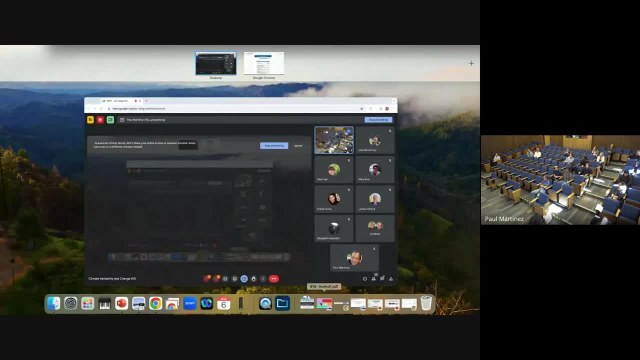 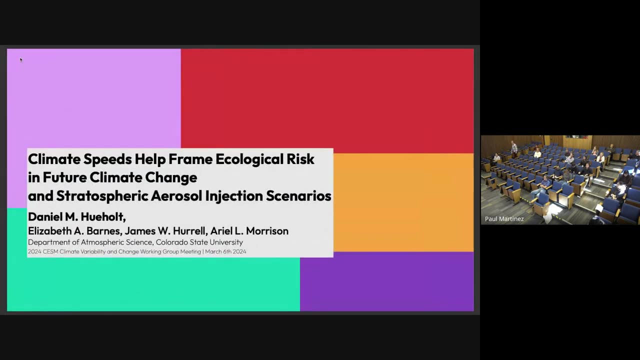 and you can correct me- Is basically your work, a sanity check that preserving global mean preserves the extremes? I think at face value, yes, but I think there are some other insights to be gained from some of these simulations. Also, the UK ESM. 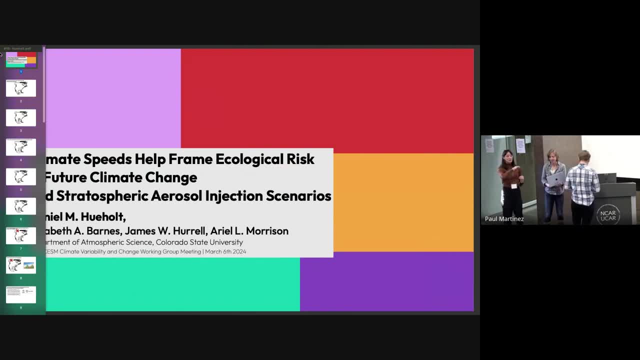 simulations of global mean temperature. So in UK ESM basically the global mean temperature has risen above 1.5 degrees Celsius above pre-industrial before SAI deployment begins, and so there's actually a decrease in temperature when the deployment begins, and so I think that could also. 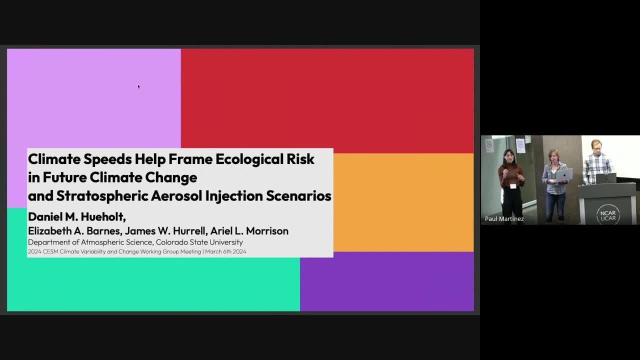 have an impact, And so looking at how just the overall temperature trend over time matters too, if that makes sense, Thank you. So, last but not least, before the discussion, we have Daniel Hügel on ecological risk and climate change. Yeah, thank you. 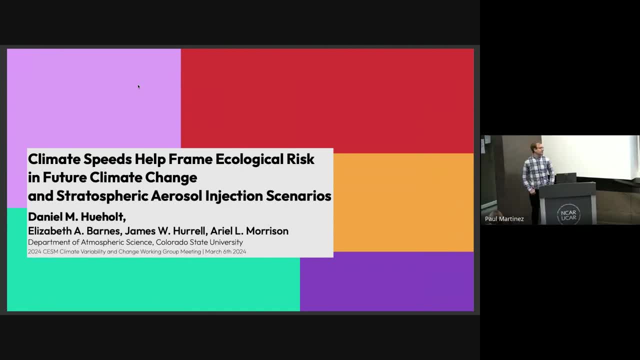 So I'm Daniel Hügel. I'm a PhD candidate at Colorado State University, where I work with Elizabeth Barnes and Jim Hurl, And this is work that I've been doing in collaboration with a postdoc in our group as well, Ariel Morrison. 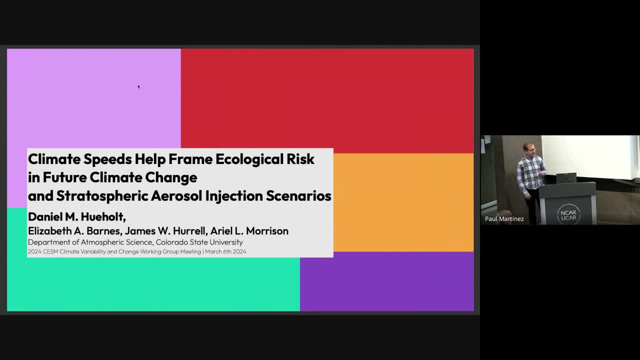 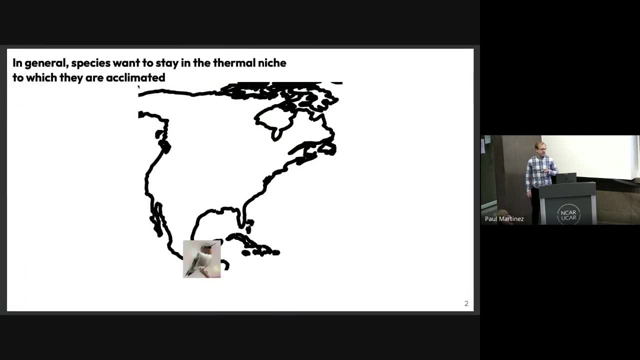 about ecological risk in climate change and climate intervention scenarios. Ecological risk in the future can come from a ton of different sources, And so, to start, I just want to walk through the example that we're going to have today, which is about thermal niches. 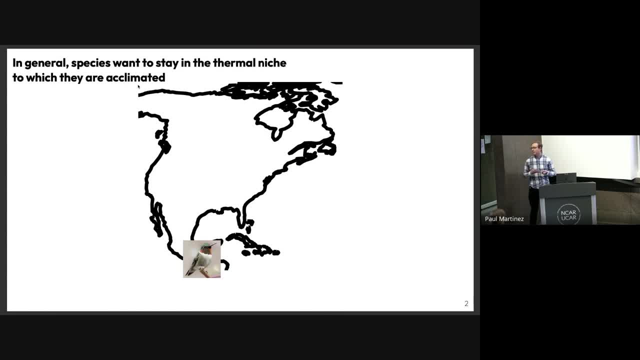 So in general, species want to stay in the thermal niche or the temperatures in which they're acclimated. So you can imagine if you're a hummingbird and you spend the winters in Central America and it starts getting warmer. then you can move. 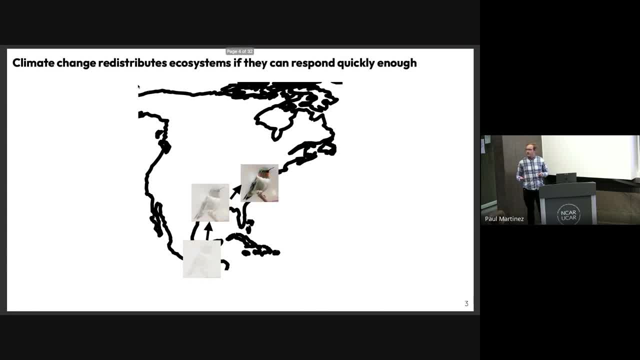 north to the Gulf Coast, And if it keeps getting warmer you can even move further north to the mid-Atlantic. So this is how climate change can redistribute ecosystems, if those ecosystems or species are able to move quickly enough to keep up with those changes in temperature. 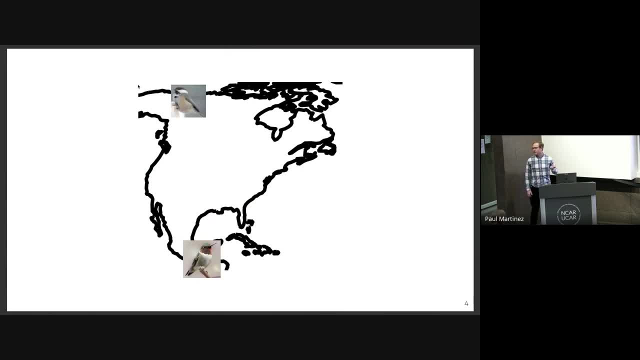 But this time let's imagine that you live in the tundra near the poles or in the boreal forest near the poles and it starts getting warmer And you can't move that much farther north without hitting the edge of the continent and you can't become aquatic. 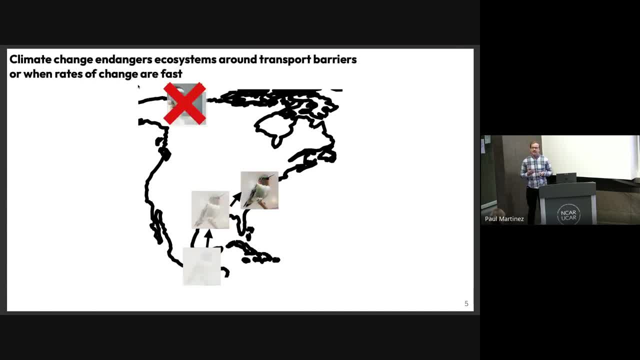 So where you have a transport barrier, this is where climate change actually endangers ecosystems. or also occurs if the rates of change are so fast that the species can't keep up with that change in temperature. And a similar process occurs around topography. You can move up the gradient. 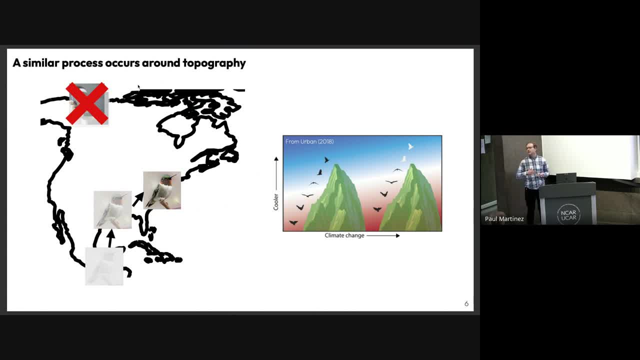 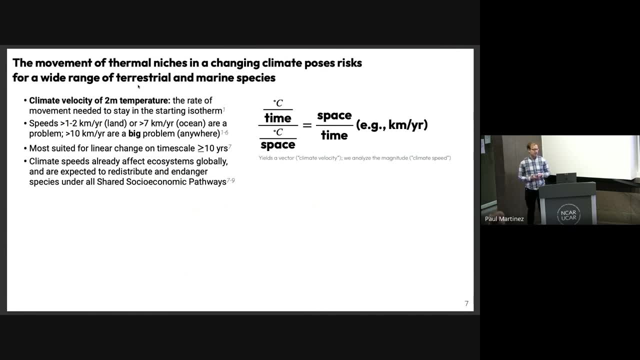 to escape climate change, but only as far as the top of the mountain, and then you can't move off the top of the mountain. So this movement of thermal niches poses risks for a wide range of terrestrial and marine species, and one way to express these rates of 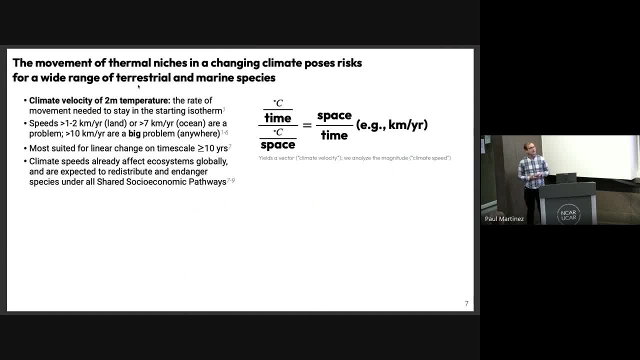 change is called the climate velocity of two meter temperature, which is just the rate of change in time divided by the local spatial gradient. We didn't come up with this, This is from the ecology community and just by unit analysis that gives you space. 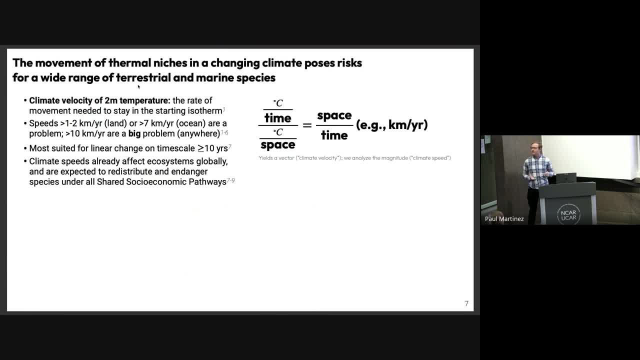 per time, like kilometers per year, so a vector velocity, which we analyze the magnitude and call it the climate speed in this case. So, pulling from the ecology literature, speeds greater than one to two kilometers per year on land or seven kilometers per year in the ocean are a problem. 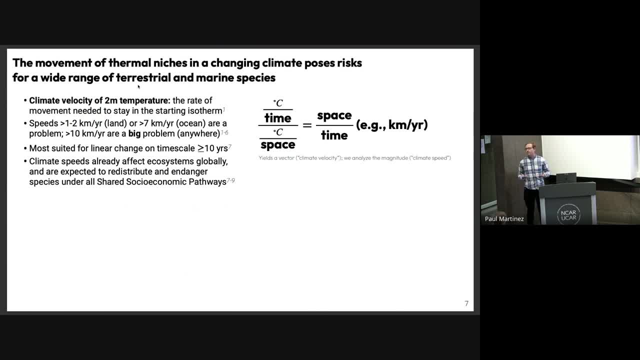 for species Greater than ten kilometers per year are a big problem, no matter whether you're on the land or in the ocean, And this is a metric that's most suited for linear change on a time scale greater than or equal to ten years and climate speeds. 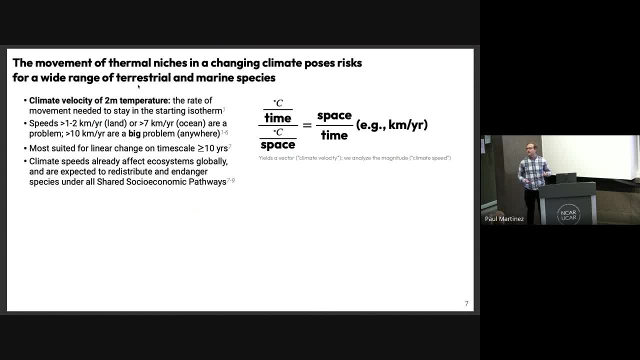 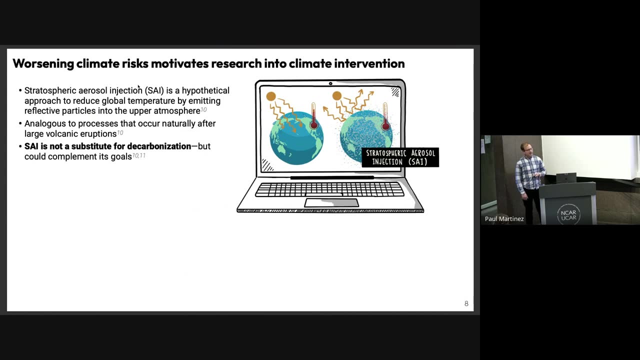 already affect ecosystems globally. Those examples, from the beginning, were based on true stories and they're expected to redistribute and endanger species under all future shared socioeconomic pathways. So risks such as these motivate research into climate intervention, as Hui and Ivy have already talked about, and stratospheric. 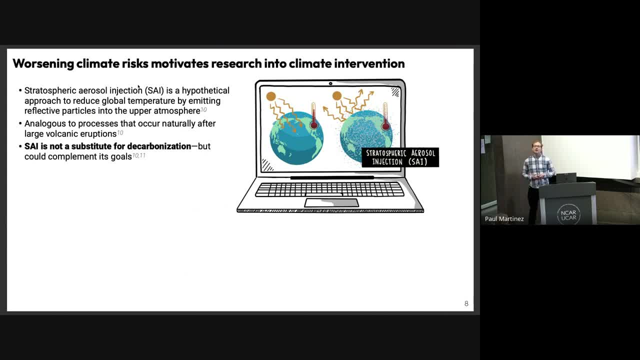 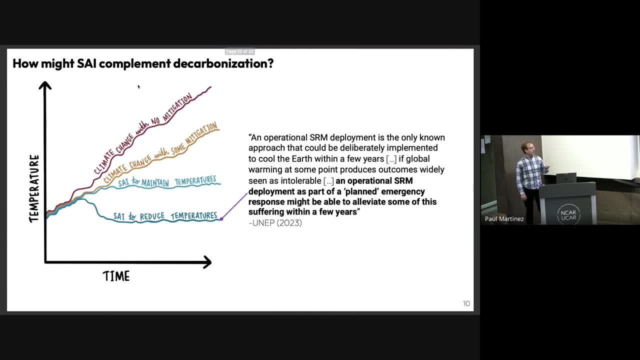 aerosol injection is not a substitute for decarbonization, but in this work I want to talk a little bit more about how it could complement its goals. So the framing, two framings of SAI that are frequently thought about, would be SAI to maintain. 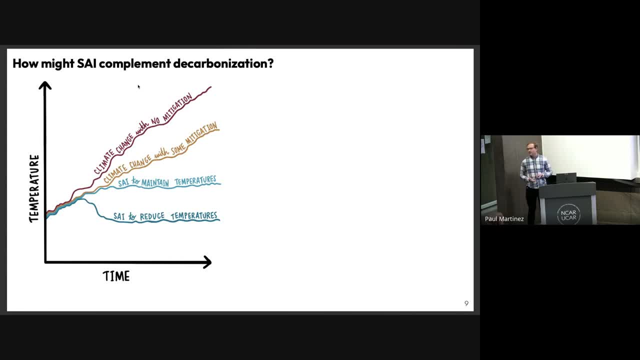 temperature at some value like 1.5 Celsius, for example in the Horizon 1.5 scenario, or potentially SAI to actually reduce temperatures because the response to stratospheric aerosols is quite fast. In a recent UN environmental program report. 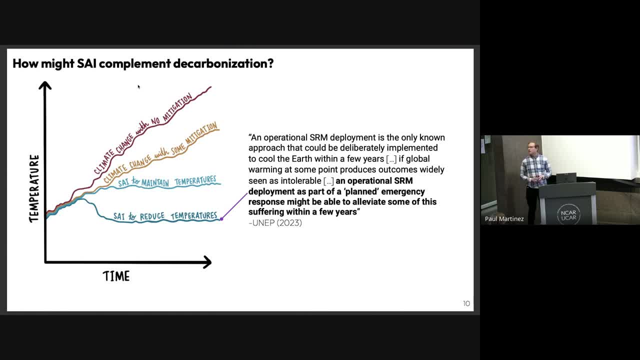 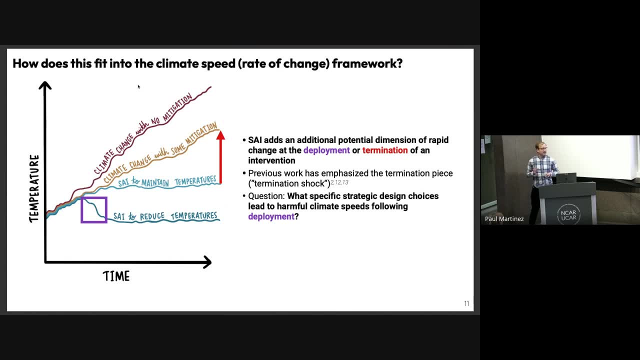 these kinds of scenarios were highlighted as a potential way to alleviate some climate damage within a few years, But from a rate of change framework, SAI is adding an additional potential dimension of rapid temperature change at the deployment or termination of an intervention. Previous work has emphasized 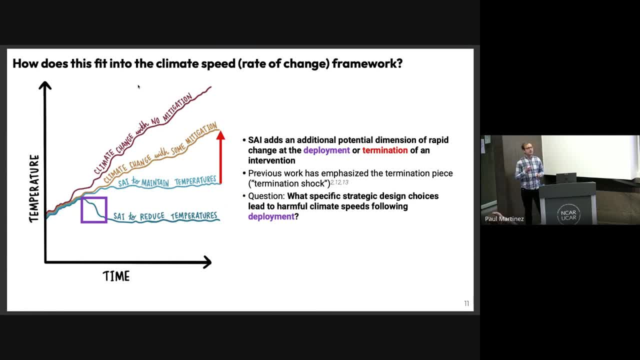 the termination piece. If you shut off climate intervention while you're masking a higher radiative equilibrium, you snap back to that higher radiative equilibrium within a few years and this is called termination shock. Here we're asking the question: what specific strategic design? 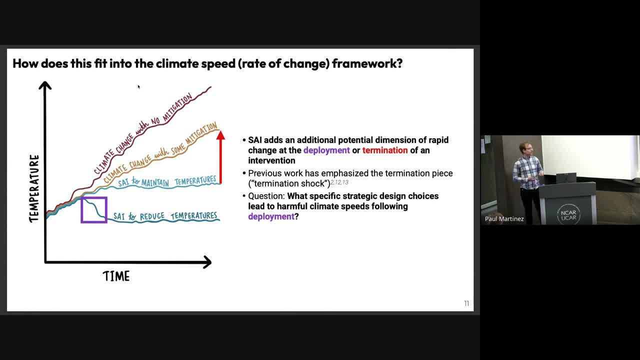 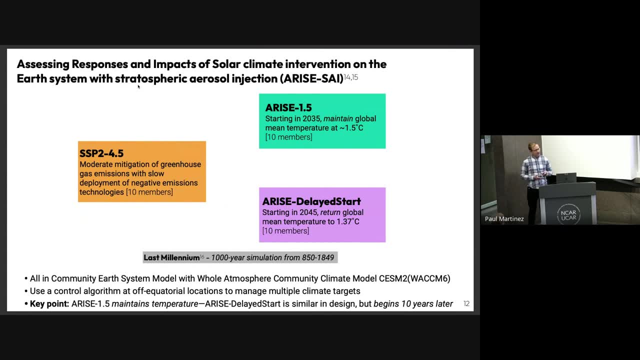 choices lead to harmful climate speeds following deployment from cooling. To investigate these questions, we're using two scenarios from the ARISE SAI project. The first one is ARISE 1.5, which Hui and Ivy have already talked about In this. 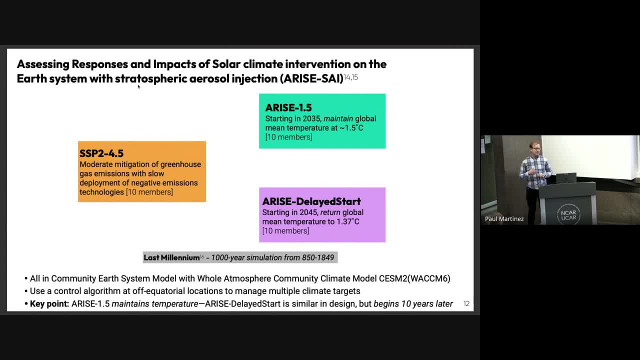 scenario: you deploy SAI in 2035 to maintain global mean temperature at about 1.5 degrees Celsius above pre-industrial. In ARISE, Delayed Start, you have a very similar temperature target, but you begin 10 years later in. 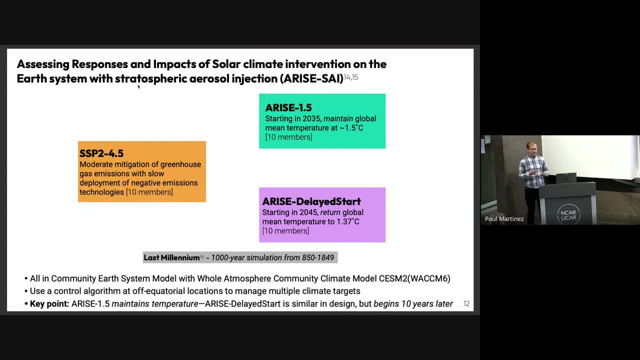 2045.. Because of the warming that's occurred in the meantime and because of a slightly lower temperature target, you have to rapidly reduce temperature to return it to that target of 1.37 above pre-industrial. We also use as a baseline. 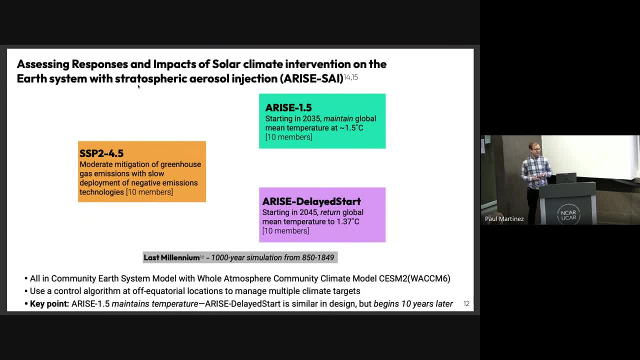 the CESM2 last millennium simulation, which is a 1,000 year simulation from the year 850 to 1849, as a baseline of what kind of climate speeds would be experienced under climate variability and natural forcings. This is used to simulate: 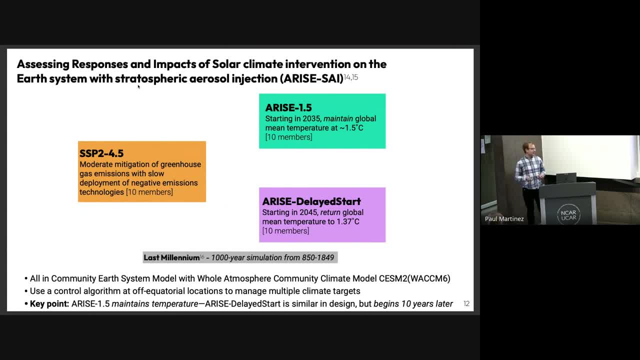 anthropogenic land use changes before greenhouse gas emissions become large. All of these simulations. oh and then, of course, the NO SAI control SSP24.5, as a moderate mitigation policy- relevant future scenario of climate change. All of these simulations are in. 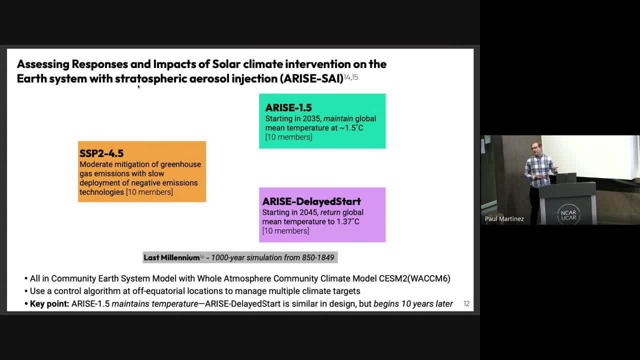 CESM, with WACNM, with the caveat that the last millennium simulation is in a middle atmospheric configuration of the model. But that doesn't matter because we're not looking at chemistry here. But the key point in these scenarios is that ARISE 1.5. 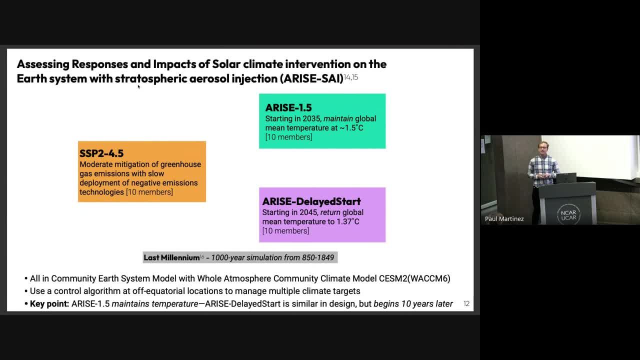 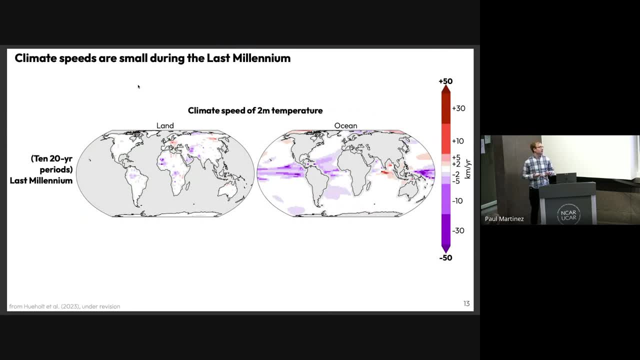 maintains temperature and ARISE. Delayed Start is very similar in design, but it begins 10 years later. So to begin, these are the climate speeds over 10 20-year periods of the last millennium simulation and this kind of matches your expectations: Natural forcings. 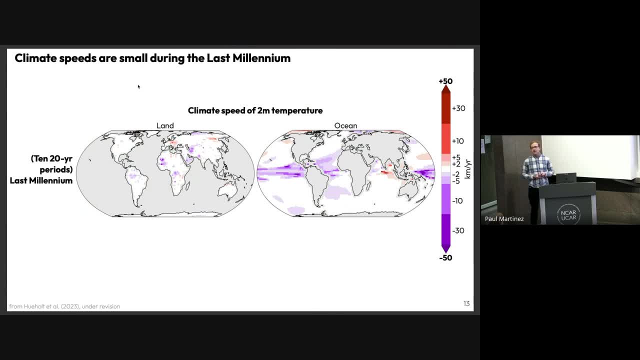 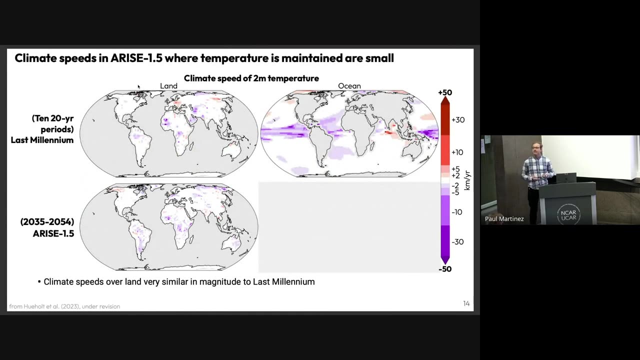 evolve quite slowly, so you do have climate speeds. Climate variability exerts very significant influence on ecosystems, naturally, but they're very small overall. And in ARISE 1.5, where you're maintaining temperature, your climate speeds over land are quite similar in magnitude. 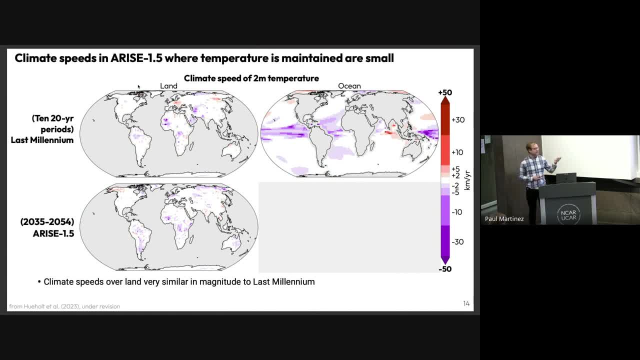 to what you saw during the last millennium simulations And this is the 20-year period immediately following deployment of the SAI intervention Over the ocean. your climate speeds are negative overall because that 2035 deployment year is slightly above the 1.5. 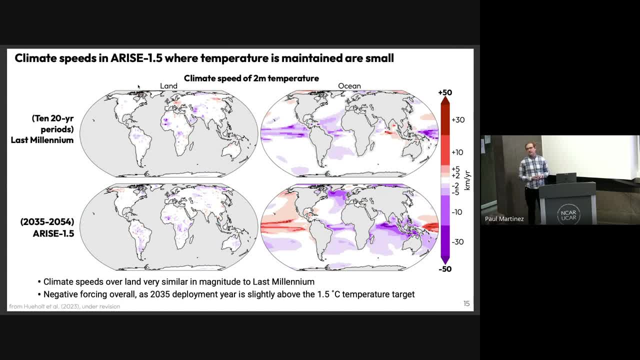 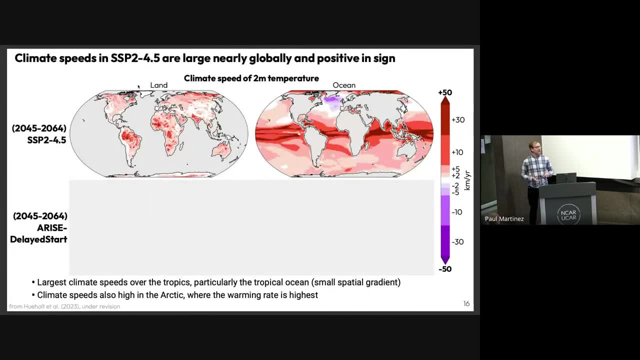 Celsius temperature target, so you do have a small negative temperature trend during that 20-year period. following deployment In SSP 2.4.5,, climate speeds are large and positive everywhere except over the North Atlantic warming hole, And this pattern matches our expectation of ecosystem. risk from the ecology literature. You have your largest climate speeds over the tropics, particularly the tropical ocean, where your spatial gradient in temperature is quite small. So even a small perturbation to temperature means you have to move a very large distance to keep up with it. 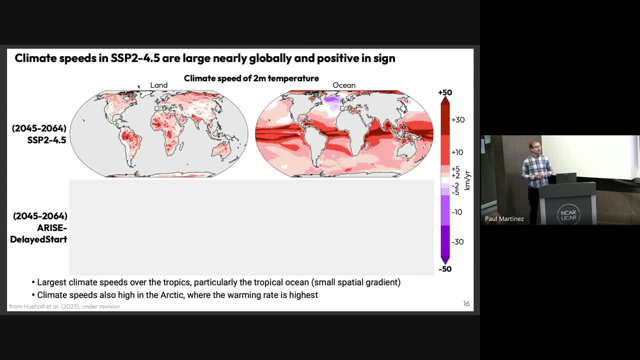 And the climate speeds are also high in the Arctic because here your warming rate is highest. So those are the two parts of that climate speed calculation and how that gives you a large climate speed everywhere. Then in a rise-delayed-start, your magnitudes are. 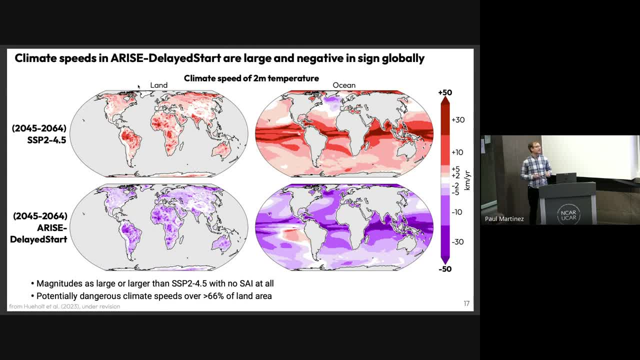 as large or larger than SSP 2.4.5, with no SAI, And the potentially dangerous climate speeds occur over greater than two-thirds of the land area because of this rapid temperature reduction that's forced during the 20-year period immediately following deployment of the intervention. 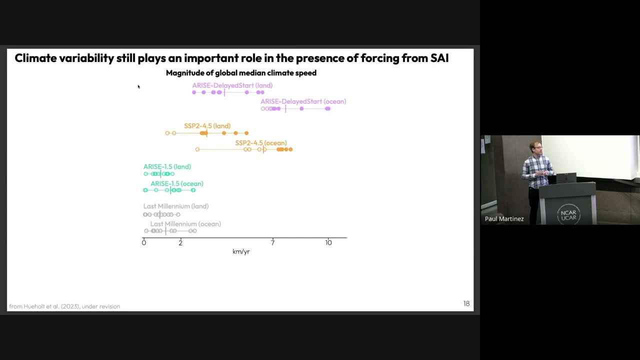 Climate variability still plays an important role in the presence of the forced response. So here, each one of the dots represents an ensemble member or a 20-year period. under these simulations, The dots that are filled are past those thresholds that are of concern from the 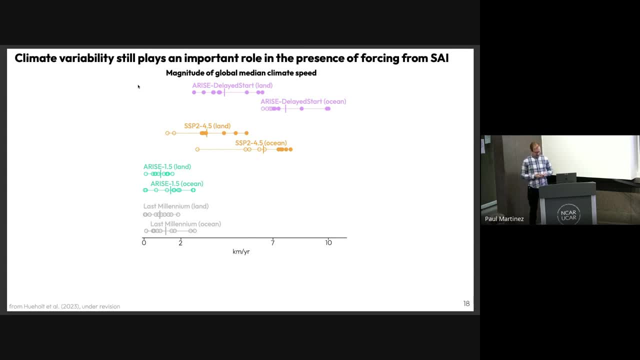 ecology literature and the bars denote the ensemble mean And the take-home point is that a rise 1.5 is actually statistically indistinguishable from the last millennium on this planetary scale. but there's no overlap between a rise-delayed-start and 1.5. 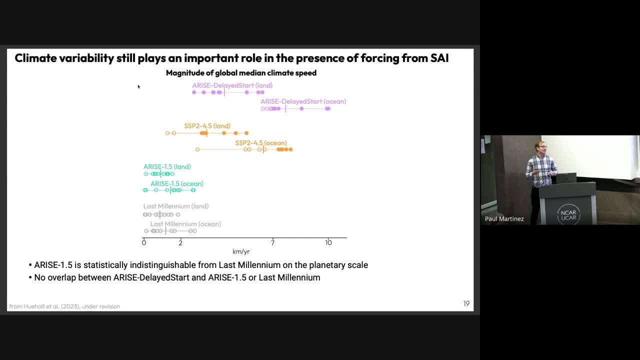 or the last millennium. That's how large the difference is. here The minimum number of delayed-start over land is greater than the maximum number of rise: 1.5 over land and similarly over the ocean. And again, the biggest difference between these two scenarios is the. 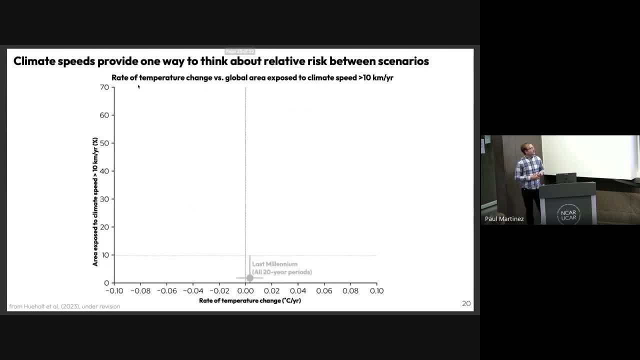 10-year delay in deployment. So the climate speeds provide one way to think about relative ecological risk between a range of future scenarios. So here we have a phase space where on the x-axis you have the rate of temperature change per year On the y-axis, 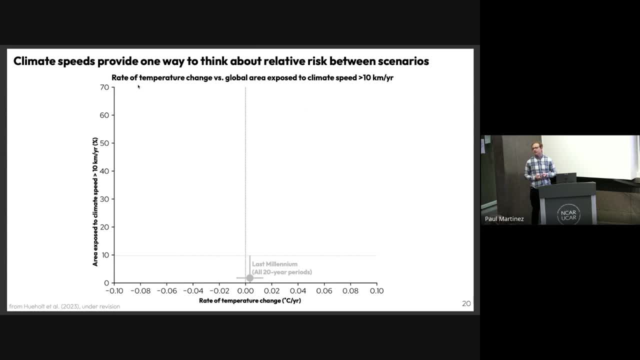 you have the area exposed to climate speed greater than 10 kilometers per year. So, again, this is the kind of threshold of extreme ecological risk from these climate speeds, and the area exposed in the last millennium is your warming rate is quite small and there's 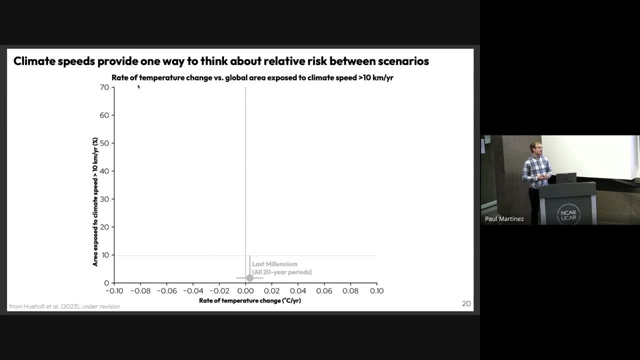 never a very large area exposed to these climate speeds under the last millennium. That horizontal bar is the maximum variability of 20-year periods, excluding large volcanic eruptions, Climate change and recent historical observations or reanalysis. cluster on the right side of this figure above that last. 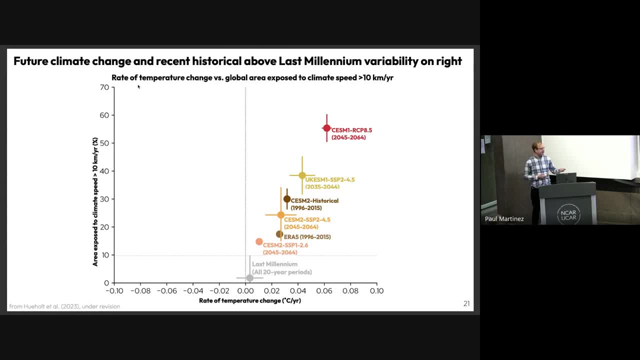 millennium variability. This scales more or less as you would expect, but more mitigation you do the less areas exposed to these climate speeds. So a lot of mitigation. you're bringing that down. Moderate mitigation- you're a little higher up, and then no mitigation at all your way up here. 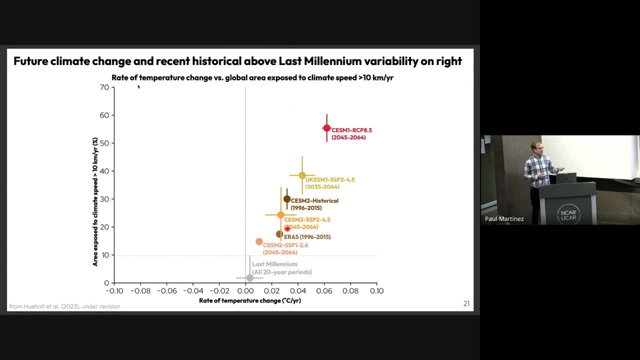 on the top right, And then this is where we've been in the last in the recent 20-year period in ERA5.. Rapid temperature reduction, SAI scenarios, cluster above that last millennium variability on the left side, And what's useful here is: 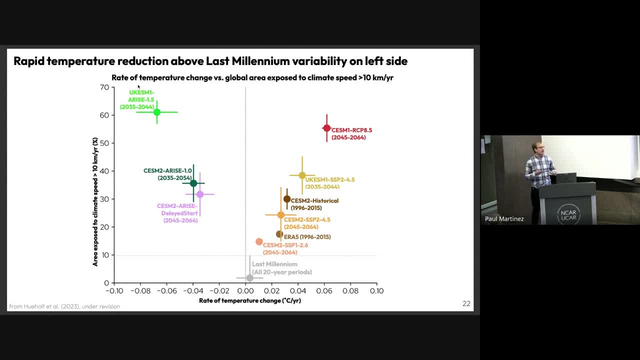 that, because of how these ERA5 scenarios are designed, we can connect these rapid temperature reductions to specific design choices. So for the CESM simulations, here's your no SAI control SSP2 4.5.. This is that ERA5 delayed start scenario, so that's a 10-year. 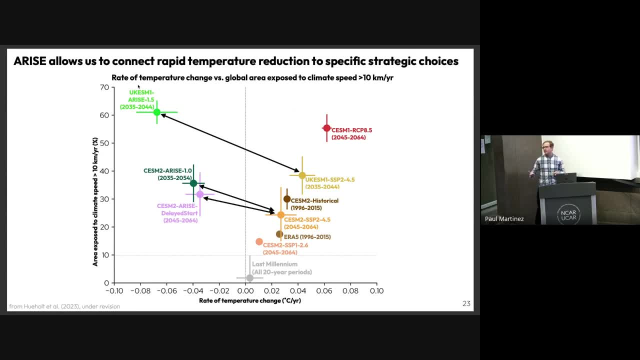 delay. and then you have to reduce temperature and that rapid temperature reduction gets you to the purple dot In ERA5 1.0, you're starting in 2035, but you have a lower temperature target, so you have to rapidly. 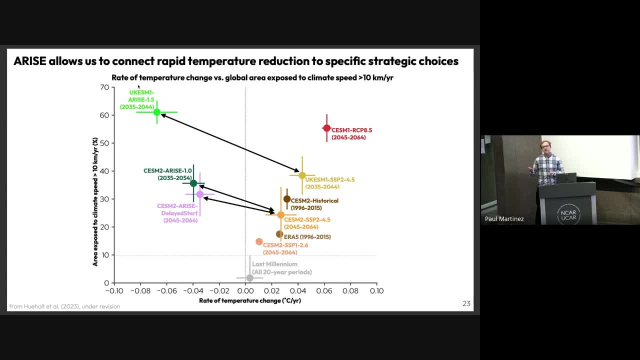 reduce temperature to reach that temperature target. This kind of follows up on one of Ivy's points In the UKSM simulations. because climate sensitivity is so high in UKSM you actually overshot 1.5 Celsius significantly by that 2035 deployment time. so you 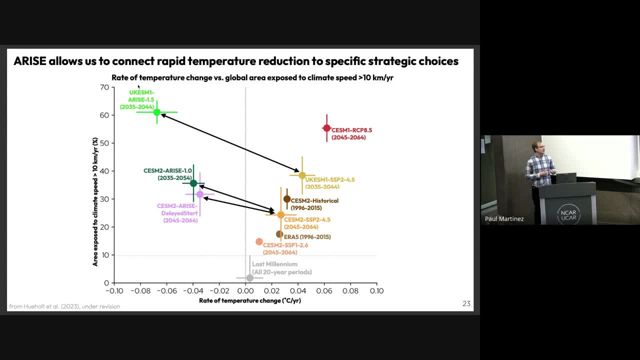 have to bring down temperatures again to reach that temperature target. And in each one of these simulations the area exposed to these extreme climate speeds is greater in the SAI scenario than in the no SAI control scenario. And then the final class of simulations. here are those scenarios: 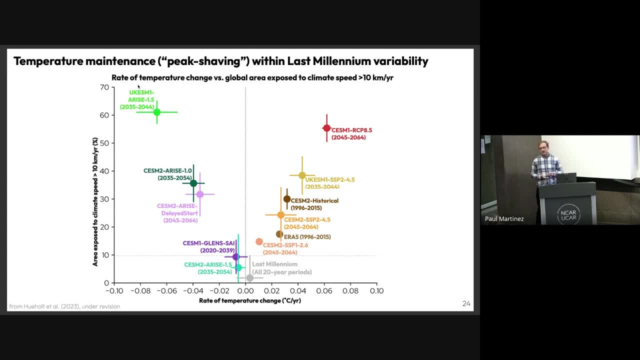 with SAI, where you maintain temperatures, sometimes called peak shaving, And here we have the ARISE 1.5 and the GLEN scenarios. Both of these are temperature maintenance scenarios. These are the only products we have here where you're within that last millennium variability. 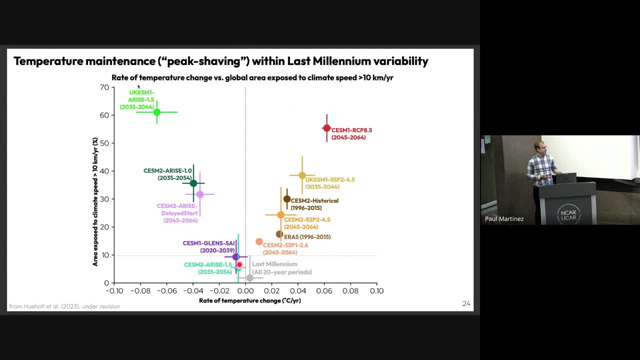 But again, the primary difference between that ARISE 1.5 and the ARISE delayed start is that 10-year delay in deployment. So a relatively small change to your scenario design has created a very large change in your ecological risk, And that's. 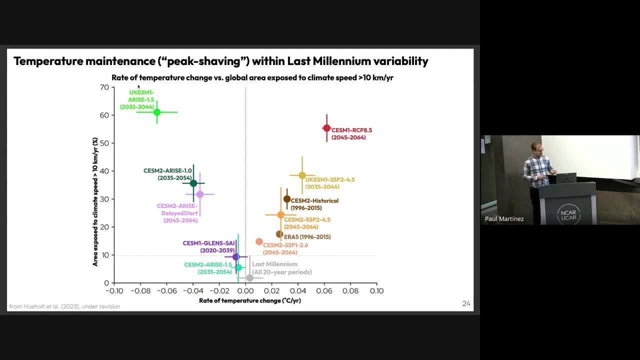 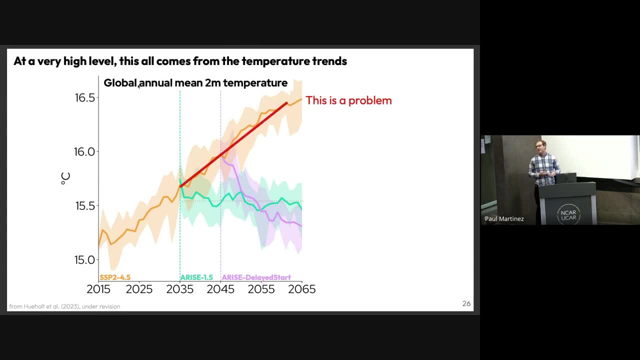 not necessarily intuitive when we think about designing these scenarios At a very high level. this is all just coming from the temperature trends. So if this is a problem because that's no SAI climate change, then on this one specific metric, ARISE 1.5 might not look. 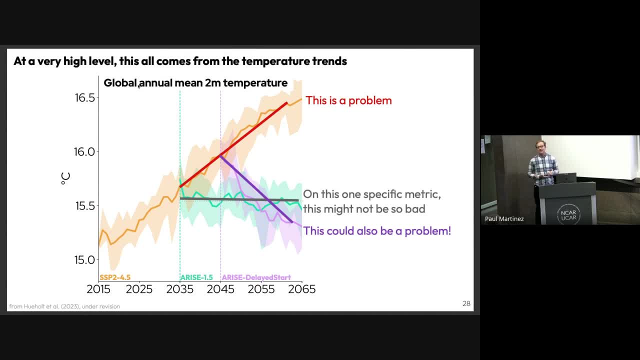 so bad. But this could also be a problem because it's very rapid temperature change just in the other direction And you could imagine scenarios to avoid this so-called deployment shock. You could do a delayed start, but with a higher temperature target to maintain temperature. 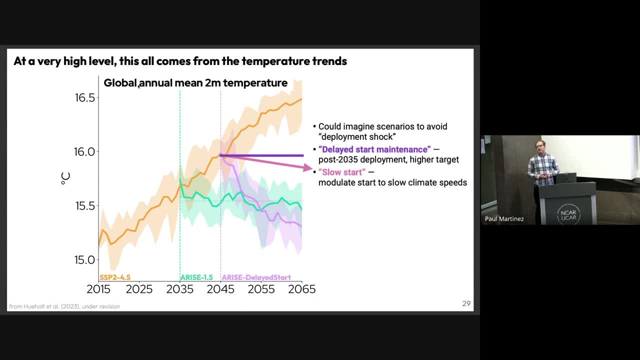 Or you could do a delayed start with a lower target, but have a slow deployment of SAI in order to make sure that your climate speeds are never too quick. So, in summary, these ARISE simulations allow for outcomes in different scenarios to be 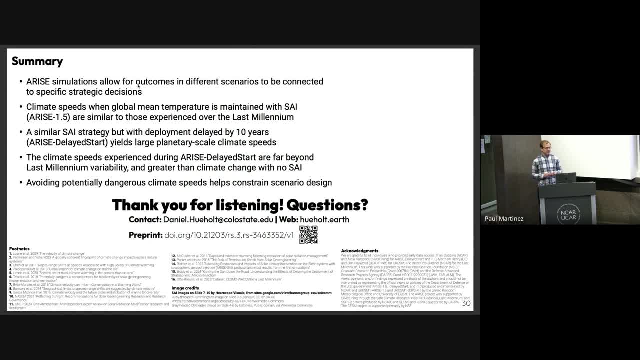 connected to specific strategic design decisions, which is really, really useful. Climate speeds, when global temperature is maintained with SAI in ARISE 1.5, are similar to those experienced over the last millennium. A similar SAI strategy, but with deployment delayed by 10 years. 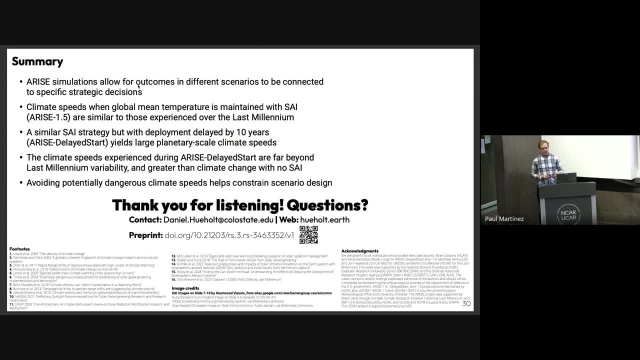 yields large planetary-scale climate speeds which are far beyond last millennium variability and greater than climate change without SAI at all, And avoiding these potentially dangerous climate speeds may help us constrain future scenario design. So thank you for listening. I'm happy to take any questions and 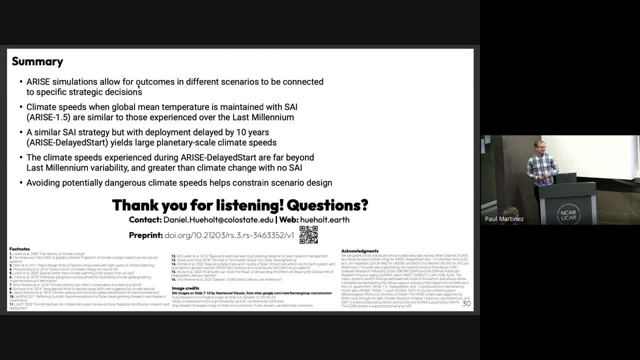 feel free to take a look at our preprint, which will hopefully be published soon, Thank you. Thank you, Any questions? That was really interesting, Thanks, I'm trying to wrap my head around this idea of like some birds example. 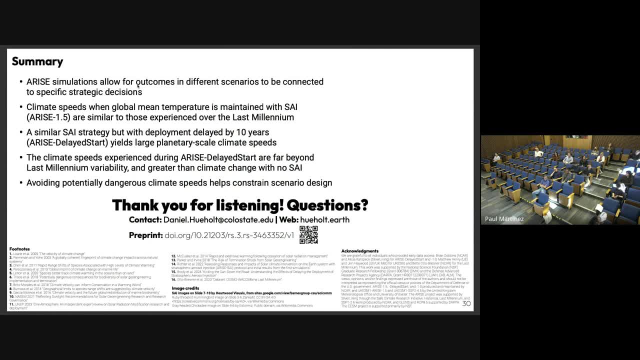 not being able to adapt fast enough in these kind of decadal rates of change when you have seasonal migrations that cross continents. So I'm curious, like: are the implications for these climate velocities specifically for species that don't migrate, or does it also apply to? these migratory birds? Yeah, so it does apply in general. Seasonal migration is just a very, very different process than adjusting the range that you breed in or the range that you're used to wintering in. Those are just really different. biologically, and so being able to migrate large distances seasonally doesn't necessarily mean that you're able to move your breeding or wintering range far distances to keep up with a climate change, And there's a lot of precedent for this in the historical climate. 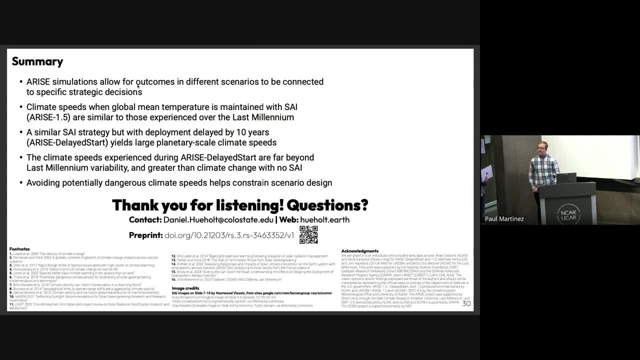 variability literature and the climate change literature. Lots of examples of this. Could you maybe comment on different- how would you call it- tolerated speeds differing between vegetation and animals? Yeah, so this is a really complex point. how kind of different species and different families. 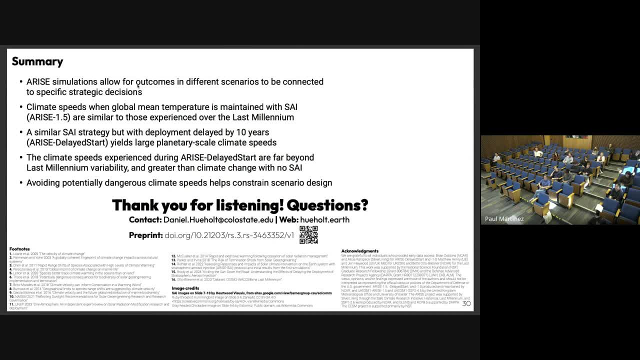 and different classes of species have really differing abilities to keep up with climate change. Obviously something that's sessile, like a tree you can't move at all. The range can move over time, based on seed dispersion and that kind of thing, but an individual tree, literally. 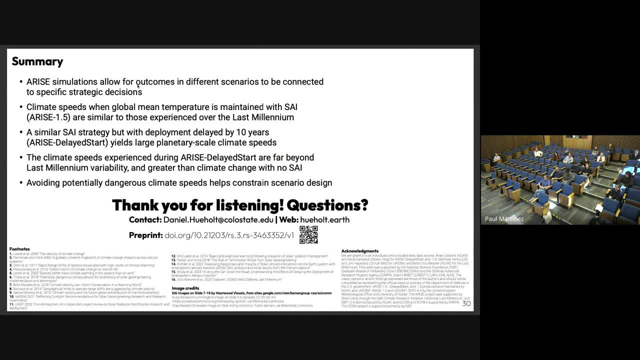 it's not going to just walk up a mountain. So yeah, that varies a lot by species. It's kind of getting granular with analysis. like that is really difficult to do from a climate perspective, because as soon as you start thinking about individual species there's questions. 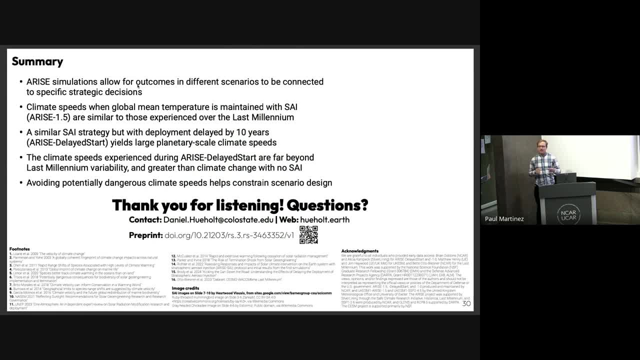 about. you know? can it adapt through evolution? Can it? is it, you know, just tough and doesn't really care about climate? Is it out of phase with the climate? but it's not going to notice that until it gets burnt down Like it gets really complicated. 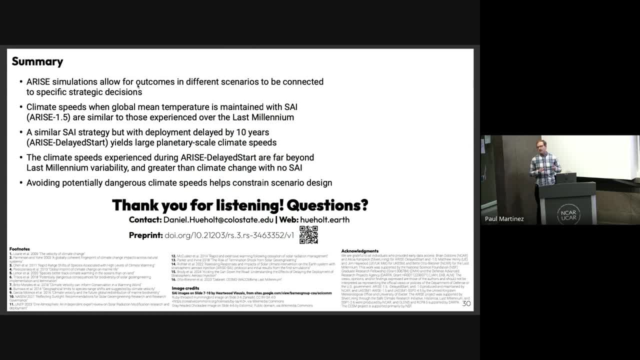 So that's why we kind of don't get into the species level questions. Climate speeds excel as a high level metric to talk about basically how big of a hammer are you hitting the ecosystem with? But for kind of a granular species level analysis you're going to need to do a lot. more work to talk about that. Thank you, Yeah, have you thought about so like like if you were doing something like we didn't start deploying SAI until like the 2060s, and so like temperature has warmed so much more? 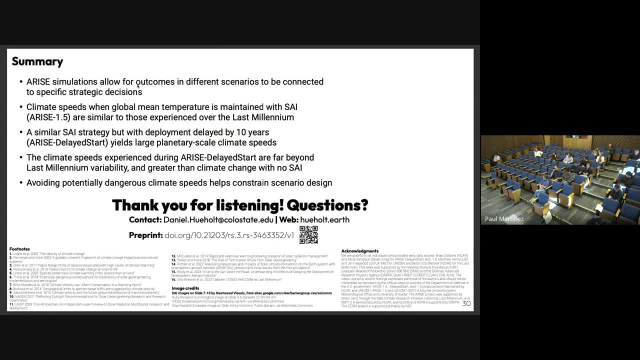 like what would happen if, like, the ecosystem that animals are accustomed to living in, like has already been destroyed by climate warming. Have you thought about that at all? Or like if there's a way to quantify, if there's like a max, like, if there's like for: 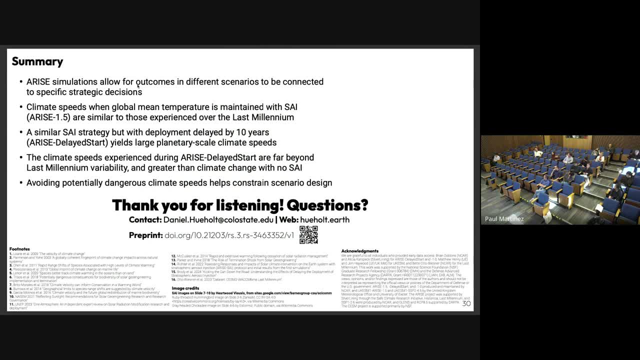 different regions, if there's like a maximum amount of warming that we can have before like the damage is kind of done. So we think those ecosystems are really where this sort of deployment shock would be most harmful. So, for example, the Mediterranean ocean ecosystems have swathed. from being a kind of mid-latitude environment to a much more tropical environment over the last 30 years. And then if you suddenly snap temperatures back colder, what happens to those species? I mean, yeah, they're not going to love that. 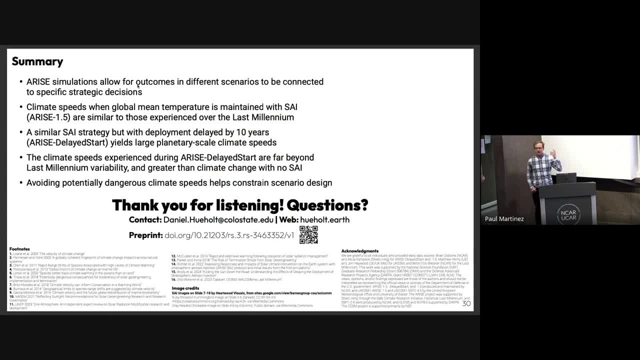 Or another example would be like ecosystems in the Rockies that have transitioned from being forest dominated to grassland dominated. If you snap temperatures back, what does the grassland do? So I think those ecosystems are the ones that would be most at risk in this kind of scenario: Those that have survived climate warming by being tough or living in a microclimate would probably love it if temperatures suddenly snapped back. So that would also that kind of analysis would also get really complicated really quickly. But there's clearly large forces pointing. 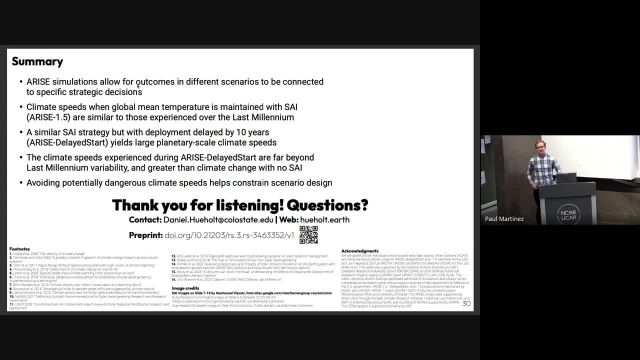 in both directions. so I kind of suspect it comes out on net to be similarly risky to large climate speeds from conventional climate change. And just one final point on that is that in the paleoclimate literature the closest analog you have to something like this: 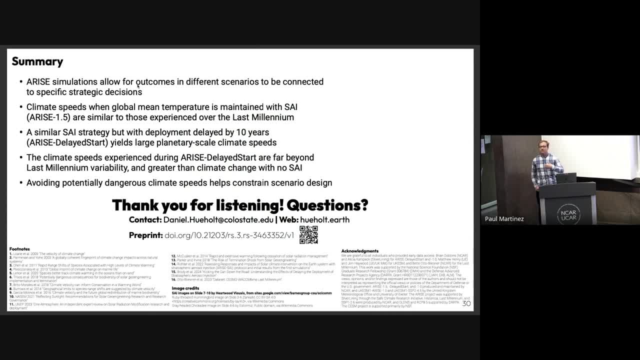 would be the onset of the Younger Dryas, we think, where you've had very rapid decadal scale cooling and where you have paleoclimate data. it looks like the regional climate anomalies during the decades following the Younger Dryas are relatively similar to what you see. 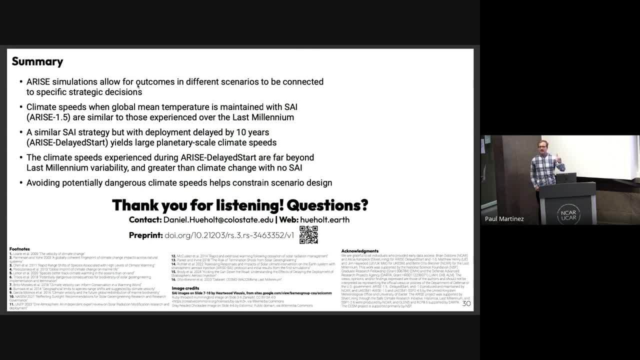 in a delayed start and that is accompanied by a planetary scale redistribution of ecosystems. So we think that this would be noticed if it happened. One last question: I was wondering if you could do something similar but with a different variable, for example, precip or. 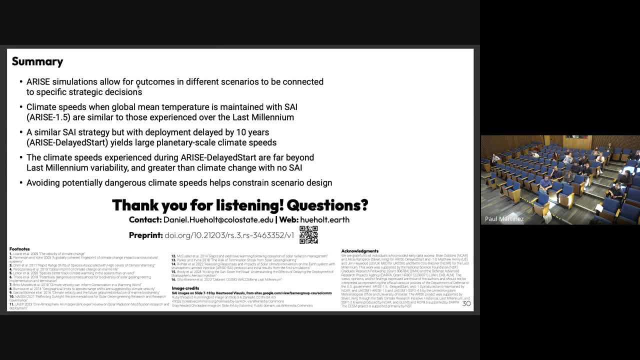 I don't know other things that species care about, and if you've thought about doing that, Yeah, so thanks for that question. I actually. that now completes it. Every time I've given this presentation, I've gotten that question, so thank you for that. 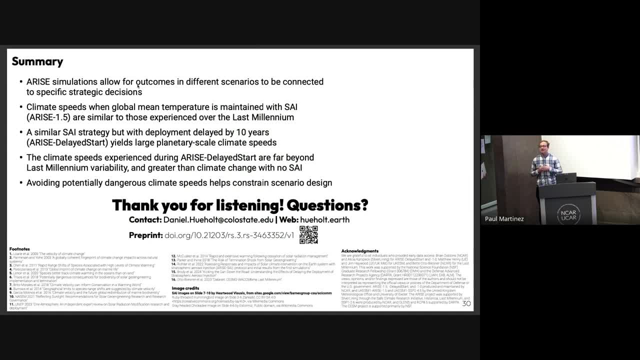 But yes, you can define a climate velocity of literally any variable that you want, One that you see commonly is called the- I think it's called the bioclimatic velocity- which is the climate velocity of the species potential distribution you get out of an ecological 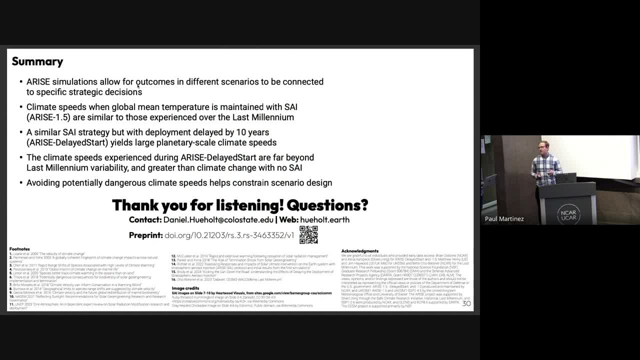 niche model, But one that people ask about frequently is the climate velocity of precipitation, and the answer that comes out to a lot is that, yeah, you can define that. It's just that climate velocity works best when you're confident in the sign of your 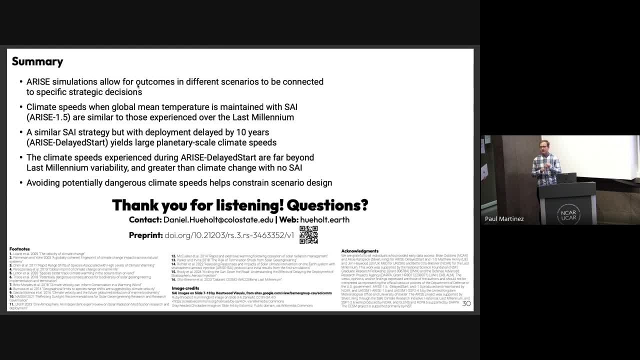 response and you're confident that the spatial gradient of the variable is represented well in the data that you're using. Other authors have published and looked into climate velocity of precipitation and that's great. We didn't have that confidence in the precipitation data that we have here, so 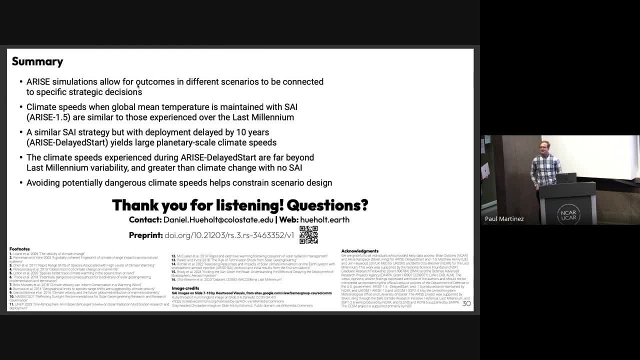 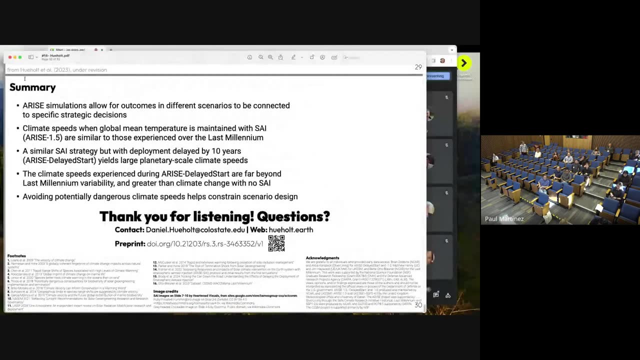 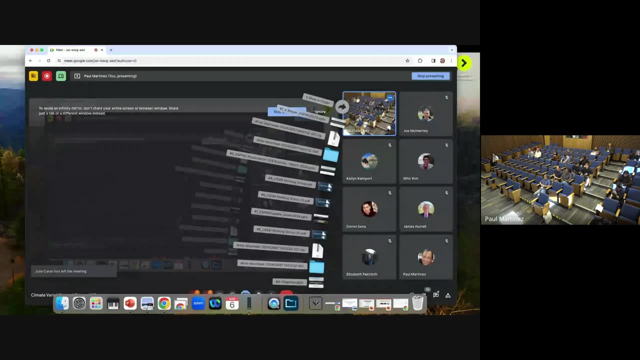 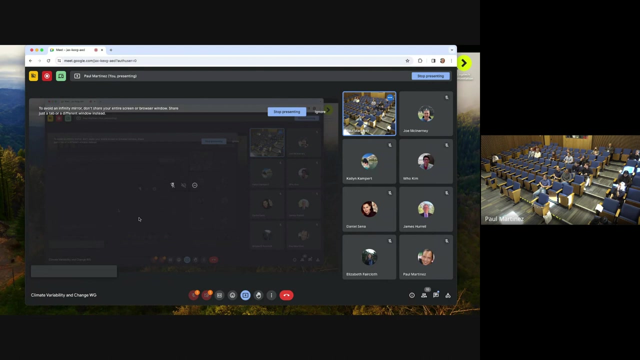 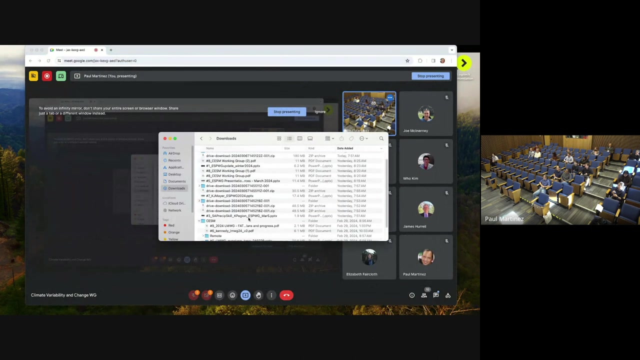 we stuck to temperature. But you can totally define that if you want to. Yeah, All right, Great, Thank you. So now we have our discussion. I'm going to try and bring up this one from this morning, So we have about half an hour, We don't have to. 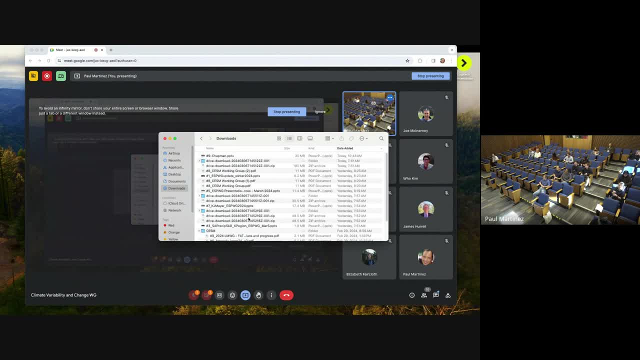 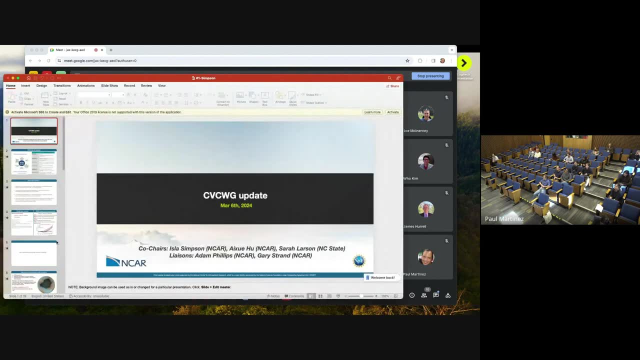 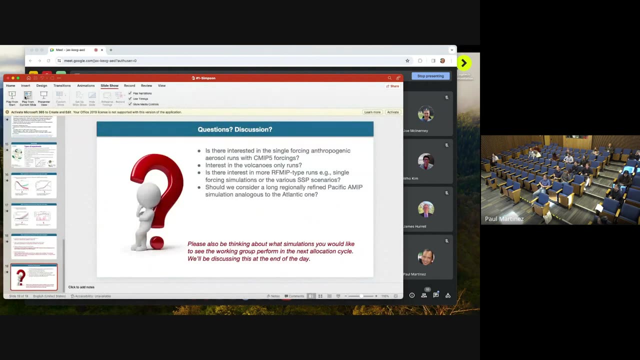 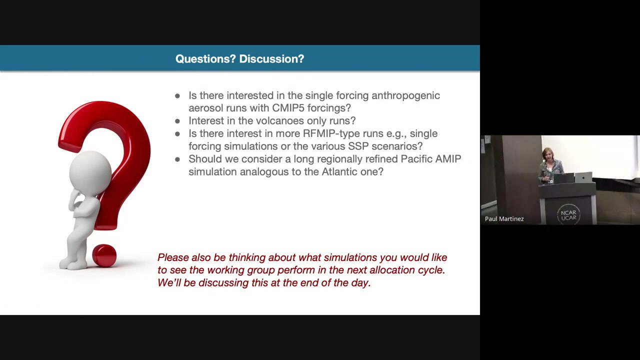 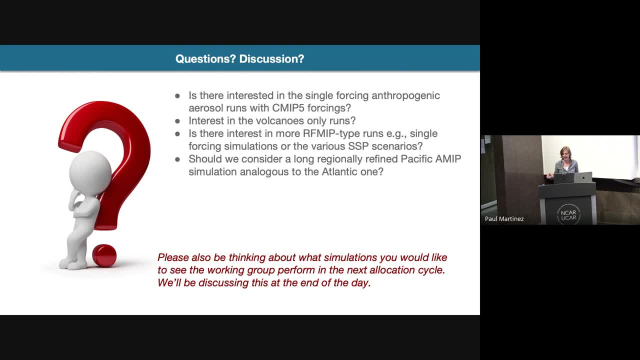 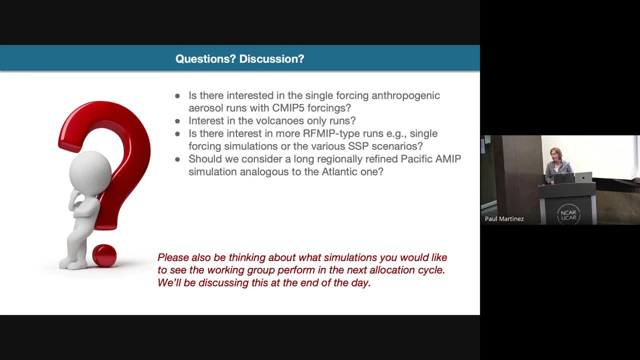 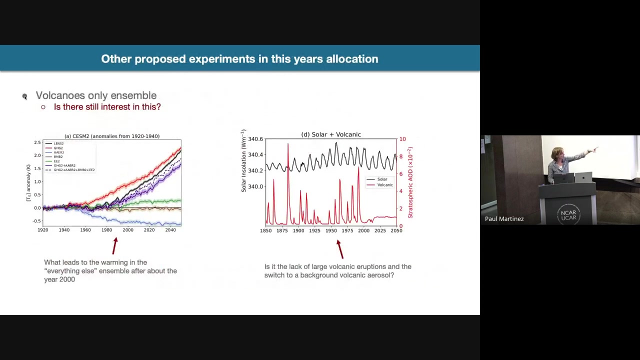 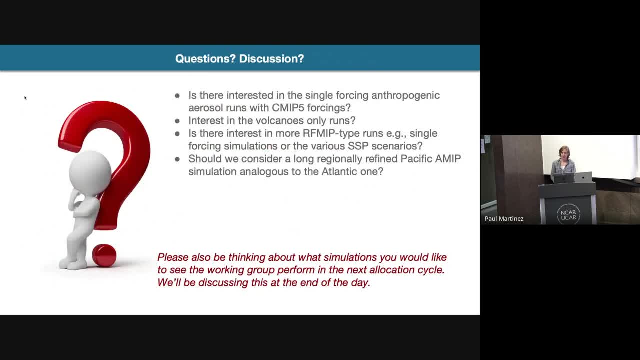 or the next year, or the next year or the next year or next three the figure, exactly what CSM3 would do. but I think, yeah, give it. I think I mean right now all we have is CMIP6 forcings, and then at some point we'll change to CMIP7, and that's kind of what happened. 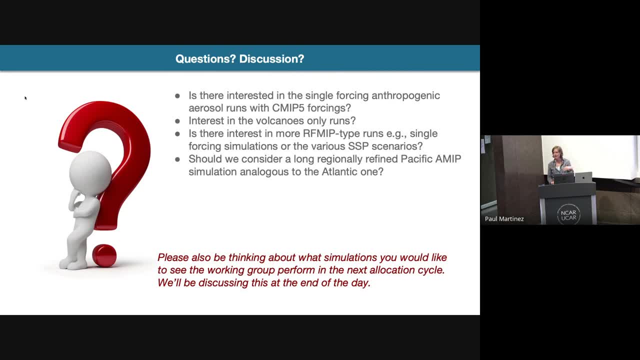 last time is the model was running fine and CMIP5 forcings. then we got CMIP6 and it didn't warm anymore over the the 20th century. so those weren't, like you know, really clean runs. they were the development runs. but you can kind of already see the impact there. I know that D8MIP is going. 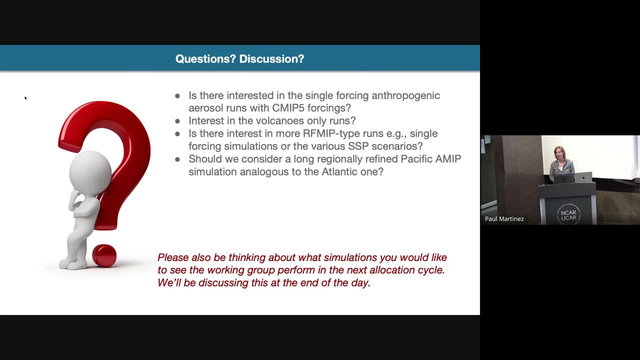 to propose a CMIP6 simulation, so running the historical with CMIP6 forcings as part of CMIP7. so hopefully multiple models would end up doing that experiment and hopefully we would be one of them. yeah, so, yeah, it makes it. I think, yeah, I don't think I had not appreciated how important the historical forcing uncertainty. 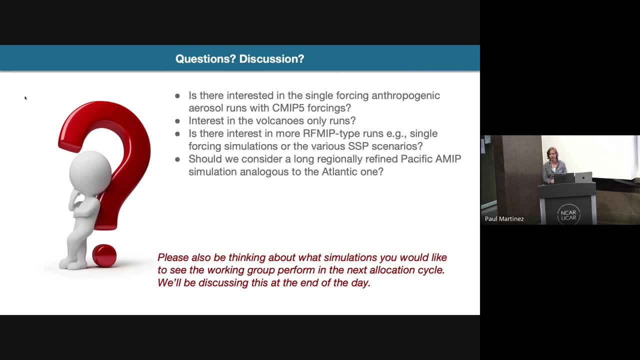 could be until last time around, so I think we should. we need to do that. yeah, I wonder what the possibility is of running more ensembles with the globally high resolution. I know Pedro had some results like three ensemble members. is it possible to add more members to that? yeah, I think they are running more right now. on the text. 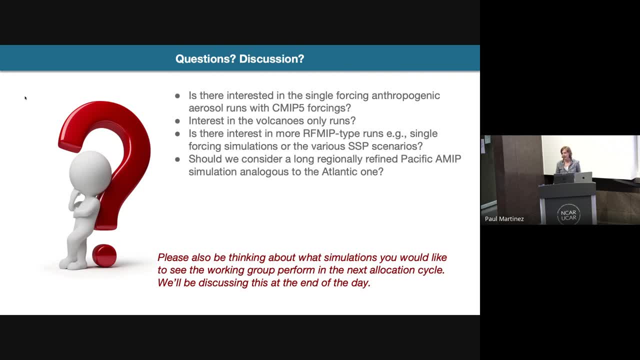 there's going to be 10.. yeah, I don't know when we're going to be public this year. the 10 members, probably soon. yeah, I don't want to take too much air from this discussion with my obsessions, but I was thinking how to frame this question is. 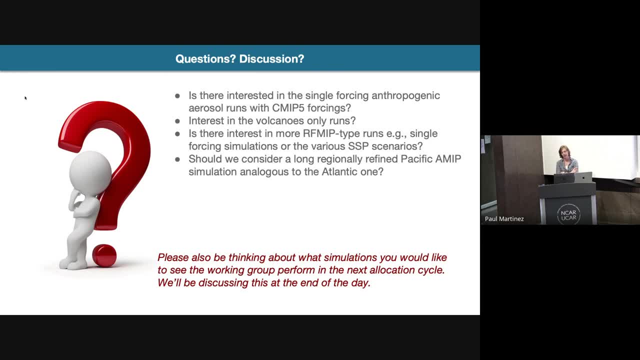 I don't think the the working group allocations are large enough to to run useful ensemble, usefully large ensembles with a high resolution model. but perhaps we can have a conversation of what could be useful and apply for computer time on on on Frontera or find a way to do it here on the Ridge on some bigger allocation, if we think there's something that is. 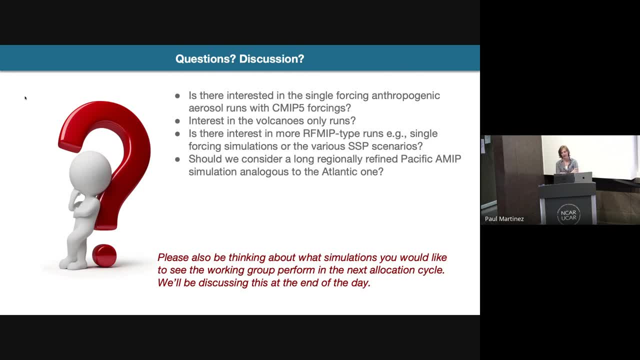 necessary to what is being done. yeah, so I was wondering. no pacemaker runs, single forcing runs. the advantage of the larger of the high-res model is that the ensembles all need to be so large because the four signals regionally tend to be larger, so you don't need 40 members, perhaps 10. 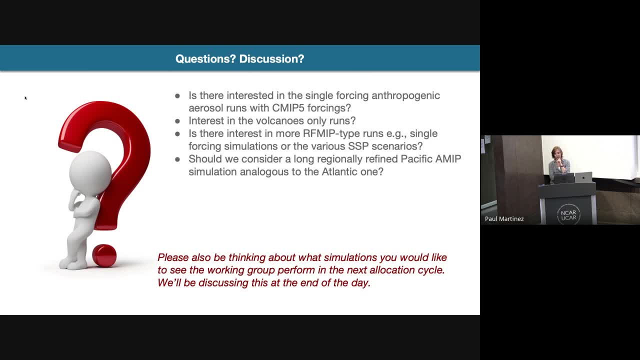 members is for some of the stuff we're looking at. the members can isolate regional force, regional changes of how much 10 members is and millions of core. it can be done on those frontier. look on those allocations on from there. these are community allocations so they have to be submitted by 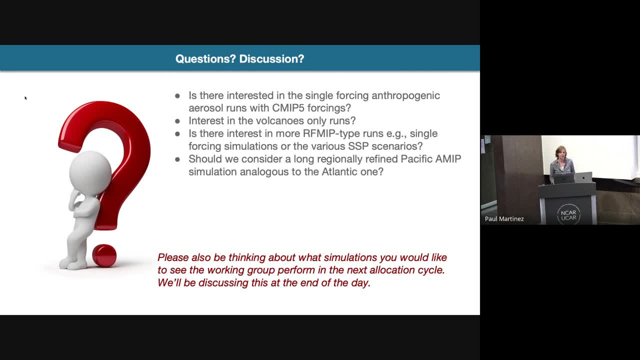 by a group of people from multiple institutions and i got- so there's two sizes, i got one of the smaller ones to do value with a group of value people and it was not that difficult to do it. i mean require some coordination. but so my question perhaps is: what's the of all these? 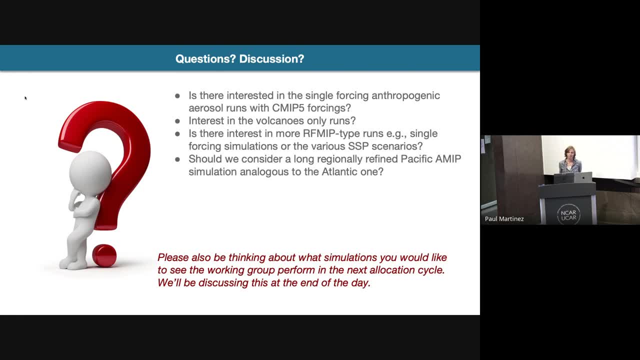 experiments that we do with csm, with the standard rest model, which one is the most important, other than the full forcing runs, right, those are going to be available. i mean, i feel like what would be nice is to pull apart the role of the atmosphere versus the ocean in the scene in the car. that's exciting. yeah, and there's a bit of it. there's a three. 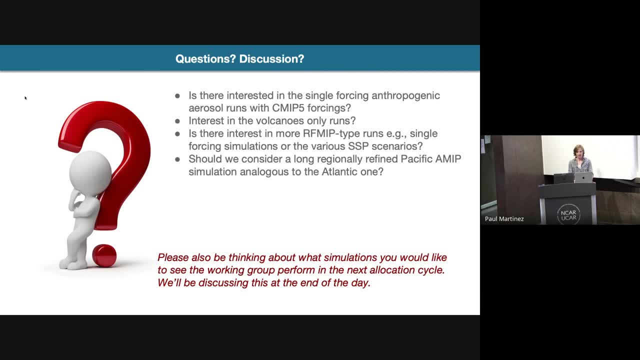 minute video. that's a three minute video. that's a three minute video. that's a three minute video. member ensemble for that from what's the name of that other project, catalyst. yeah, perhaps enlarging catalyst is a good, a good idea. yeah, but also doing, maybe doing the opposite, to test for a linearity. 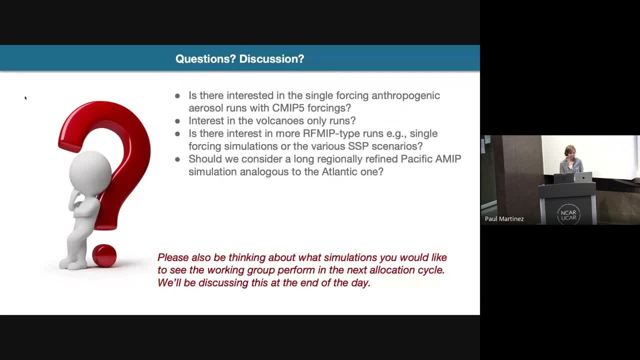 whether are there non-linearities. high-resolution, low-res, atmosphere, yeah. and then i feel like a big question is: what would csm2? but maybe we should be going on to csm3. what would that look like at high resolution? because, steve, you have results showing that there are improvements in predictability in the tropical pacific. 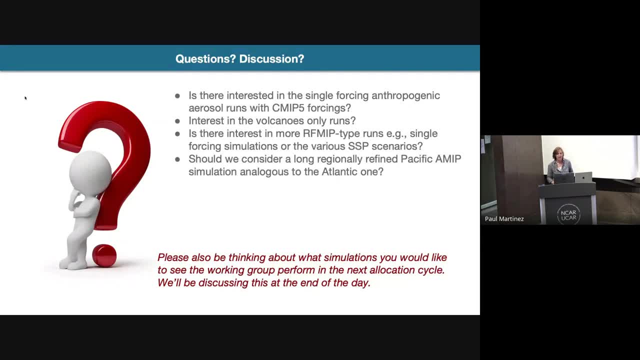 a low res with csm2. and then there are other, um sarah kang's paper showing that the cloud feedbacks give you a better connection into the tropical pacific and csm2. and so, like the combined influence of resolution and physics, does everything get better in csm2 at high resolution. 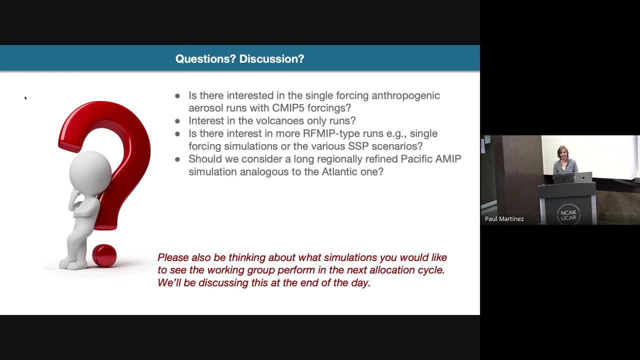 i don't know if we can afford to ask that question in the future. if we can afford it in the future to do that, I'm. it's gonna be so expensive, Steve, what do you think? but there is a plan, I think, to make a CSM 3 quarter degree and degree models and yeah, 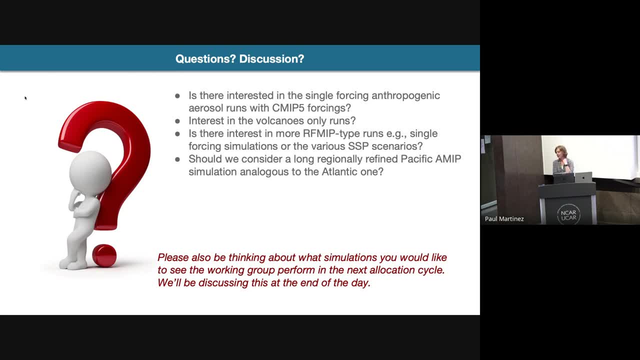 I think, if you're thinking ahead to the next proposal, it makes sense to think about yes and three high-res experiments. yeah, and you know, maybe, like Pedro is suggesting, we can't do it on derecho. you know, maybe working groups need to collectively submit a proposal to tack. I mean, that's the only place that we can. 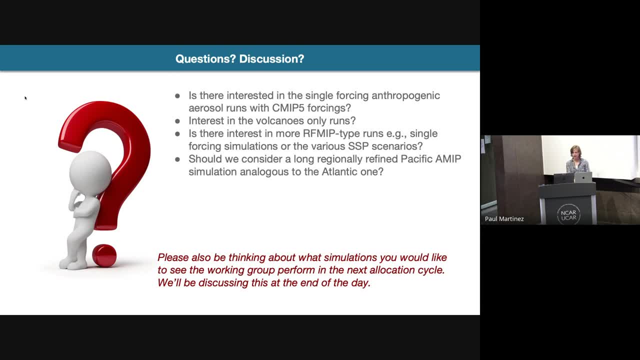 run. yeah, that's something we're allowed to do. yeah, I mean, anchor people, university people, we can do it right. yeah, I think you can go. you guys are beings proposal right in the computer than proposal if you have access to the users on tack. yeah, yeah, I'm happy to do, I'm can. 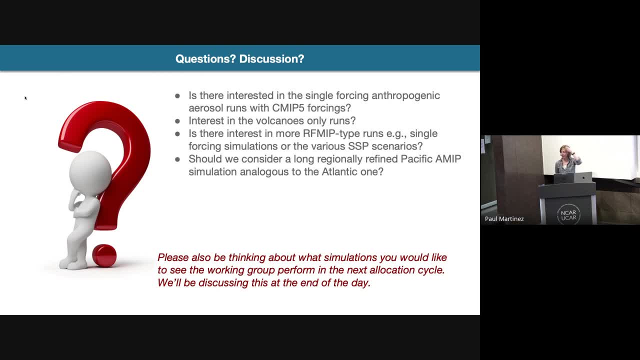 obsess with it. compelling evidence, I think there's plenty. the process representation is greatly improved. yeah, yeah, I don't know. I mean Julio was talking about running, starts and runs the other days, because there are things to look at in terms of like gravity wave drag, that it could help with solving biases that we currently have in the 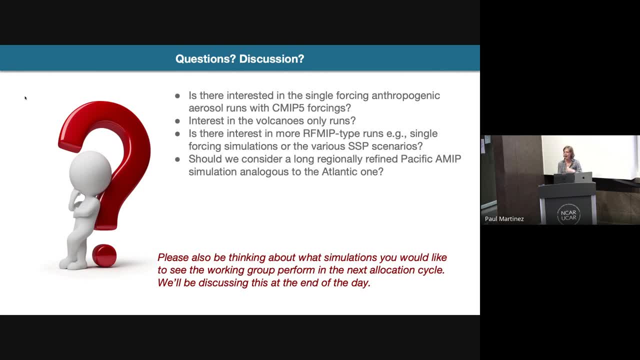 low-rise CSM 3 development version. so I guess it depends- how difficult would it? yeah, how many challenges come up? I think there's a catch on all this conversation that no one has to look at ENSO in the high-res model and I think it's pretty crappy. it's not that great. 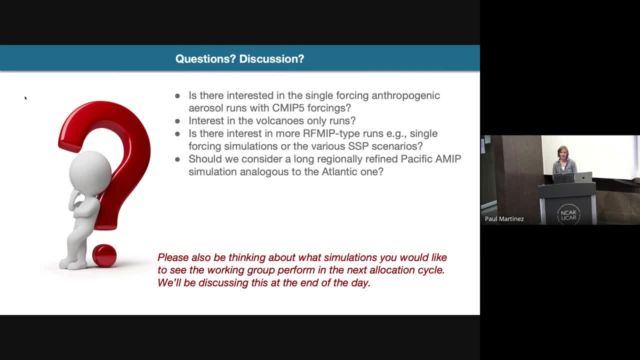 by my super superficial exploration. again, sounds like something I know. yeah, they only have 24 hours to tell us what it looks like. no, I mean, perhaps is something very close to observation in the high-res. the amplitude, the patterns are wacky. yeah, I think. I mean, again, I don't want to get a hit. perhaps, perhaps we need to do that. 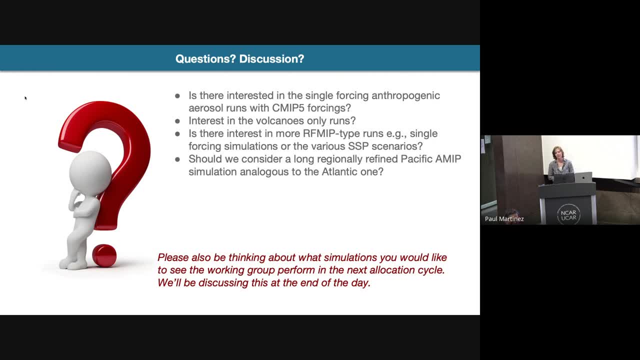 homework- don't look at me so hard- but yeah, perhaps the mix of resolution I I think perhaps a single think about single forcing, at least aerosols. Yeah, But I guess our question in that case it would be build on IASP. 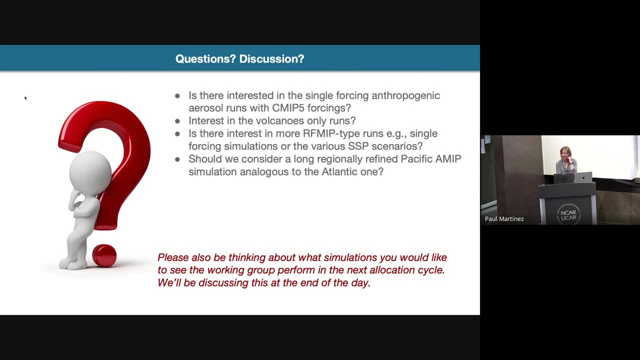 I would do it on. yeah, We don't even know the cost of CSM-3 on. this is gonna take years to know. Yeah, it's three times the number of levels, so Exactly, But it has a QBO. so 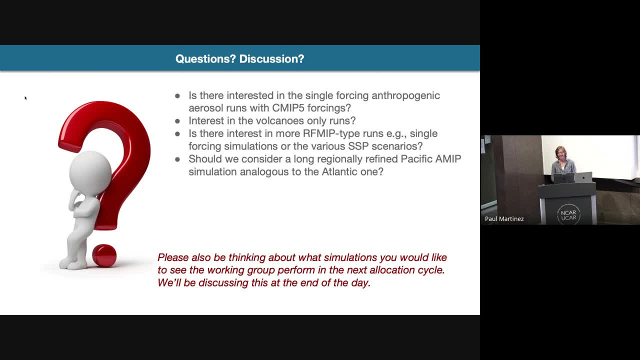 Maybe we get QBO-MBO connection at high-risk, Yeah, but there's so much to learn from this. I mean, there's already a 10-member ensemble, right? So I think to leverage that ensemble with anything else we could do. 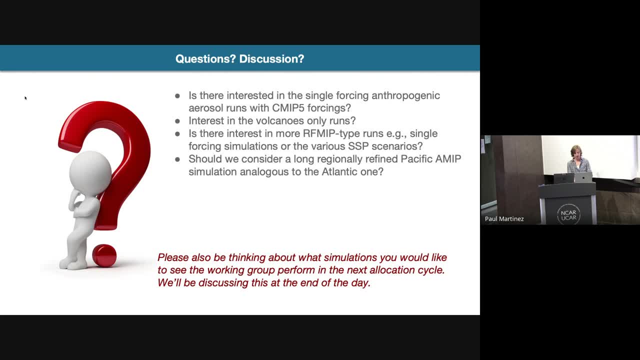 could produce so much science. Yeah, Maybe you can propose a single-force, in-cable nation, you see. Or perhaps it'll have to be 10 members, perhaps it could be five members with five and five. Yeah, It's still a ton of. it's depressing. 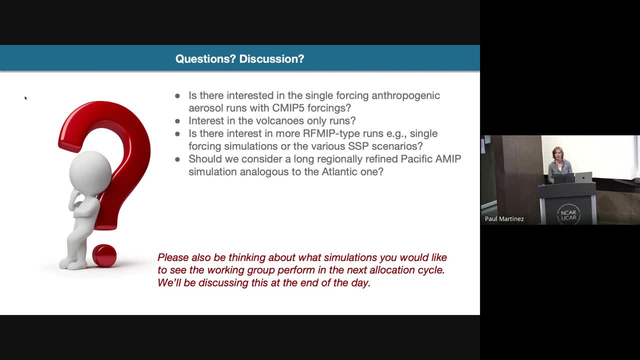 When you see the numbers it's totally depressing. Yeah, I haven't really grasped like how, what even order of magnitude are we talking about? So I'm running a mixed-resolution run with a forced catalyst member and it's 10 million core hours. 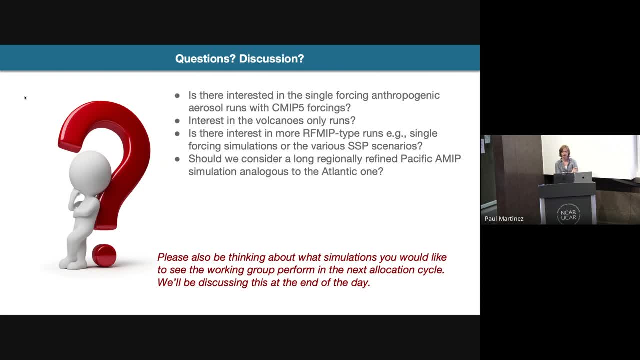 the ratio. just one run, because we have these other a lot, though. at the nsc you think they have to be over 10 minutes, but i don't know. maybe you could get three members or something of those. i'm not sure we know how big those are. that is the nsc, or something has to be over 10. 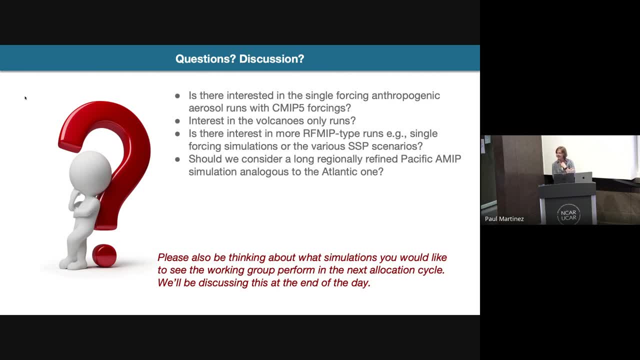 million. yeah, okay, what's the? i don't know. okay, perhaps, yeah, one on one computer. again, it's a lot of computer time. this is the group that should do that. who's who else is going to do it? yeah, you have space for the data that comes out of here. 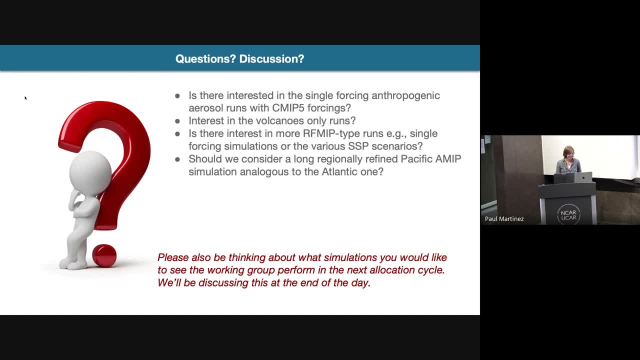 yeah, that's the thing about it. it is a pain because these things are hurricanes. so then we need hourly data. on the six hourly data, no, but i think the common theme is that we're seeing that both increased atmospheric resolution and also oceanic resolution matter, depending where you are. 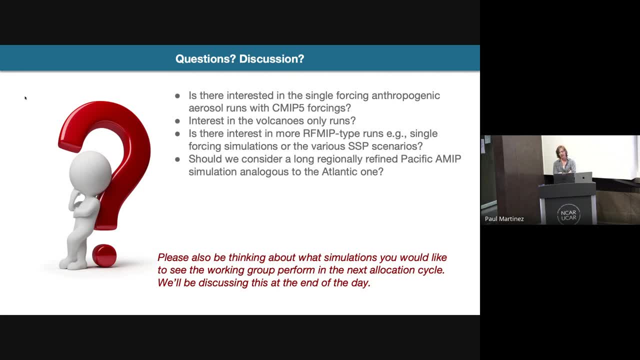 one is going and we still don't know exactly which one is more important where. but but a lot of physical processes are better represented, and another thing we could do if we don't have enough computing time is to try and leverage the regional refinement more if we knew which area we thought was the most interesting. 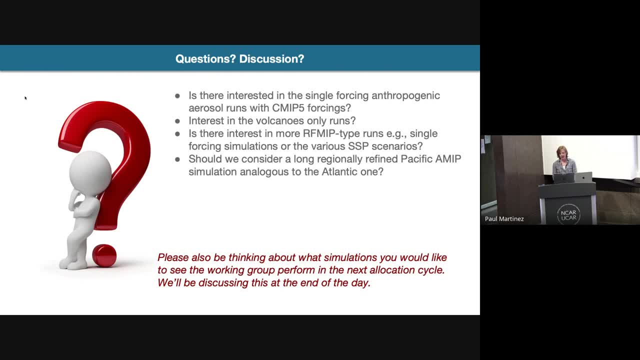 is that difficult to set up? uh it, yeah, i think setting up the grid takes some time but it's not impossible and there are some that already exist. but i guess there's less being done with coupled regionally refined but you don't have a high-res ocean in those and it sounds like the ocean is important. 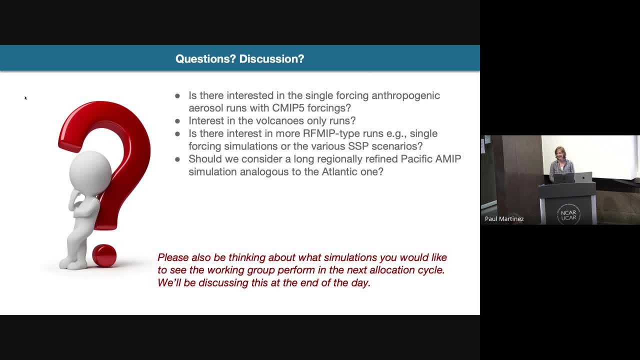 yeah. well, we could do like i don't know, ssts from them, from yeah, yeah. i mean, that's essentially where we got stopped. is we're thinking that perhaps the way to do those experiments that we were on the past allocation is to take the sscs from ihasp, yeah, and then see if, increasing the atmosphere even further? 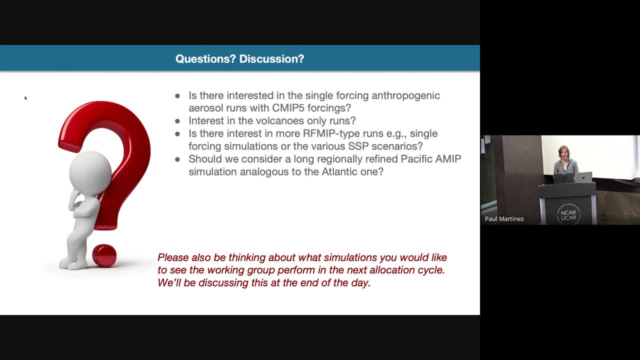 gives you a bigger atmospheric response. yeah, that's where we're stuck. thought it doesn't have to be about high resolution. well, for i'd have. high levels will be very valuable, but even for low res or standard resolution, like existing simic, uh, cs1 or system levels, no, it would be. 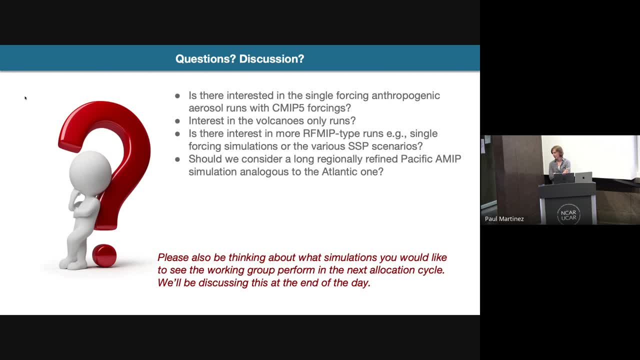 very valuable to have the- uh, of course, running argument type of realms, not only for studying, like common sensitivity or the feedback rate of forcing, but also like motivated by students work, like having those prescribers difference. allow you to study broad sql response to direct as a radio forcing versus sd force. yeah, so which, if you had to choose your top four things to have? 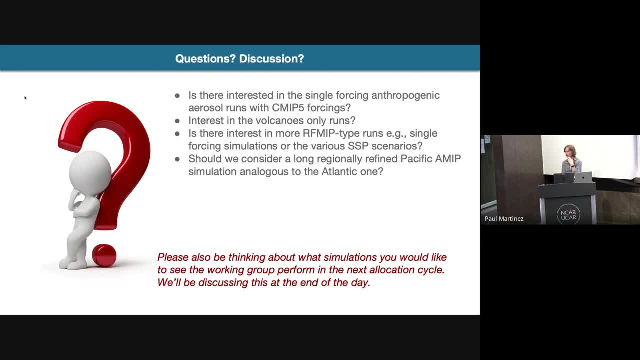 those fun runs for with what would you choose? yeah, like we're. well, we have cs in two single portion rounds. we'll be, uh great to have those associated for corresponding our form, our board, and they've been around for just three or four years. okay, but if we, if we only had allocation. 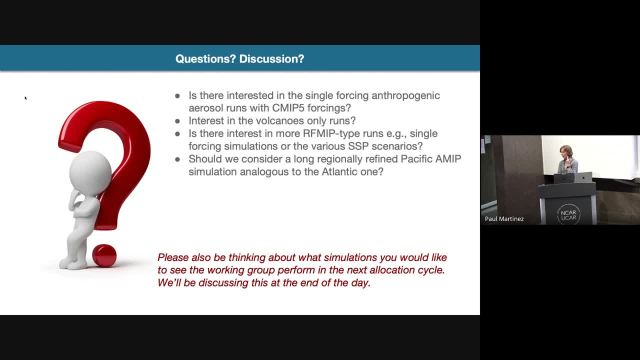 per se, two or things. would you choose greenhouse gases and aerosols or did you prioritize? you know we have both forces right now, right, yeah, aerosol force one. yeah, yeah, because i think we could manage to do some of those in this allocation, even though we haven't really proposed it. but 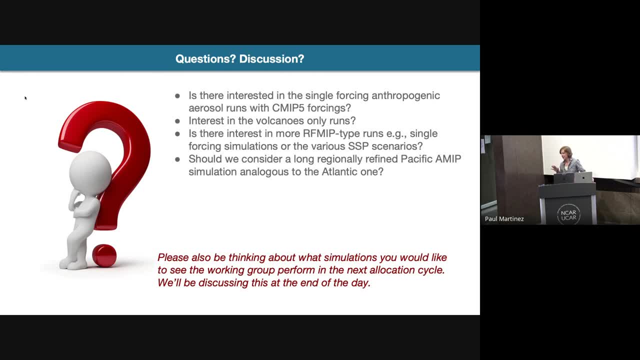 um, it's related, you know, to what we've done already, so it's kind of okay to just change for that way. but whether we could do all of them, I mean, we'll just start with the high priority ones, I guess so it would be. aerosols is probably the highest priority, yeah, followed by 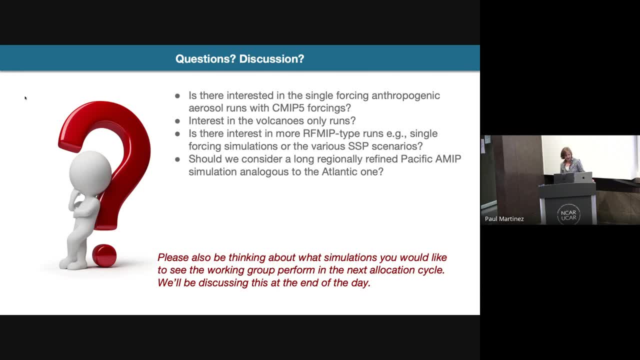 greenhouse gases, followed by the others. well, I guess biomass burning aerosols would be the above greenhouse gases, or yes, yeah, I think more about like yeah, yeah, you can talk offline about it, but I feel like it would make sense to kind of pair them with the four things we've done. so I would 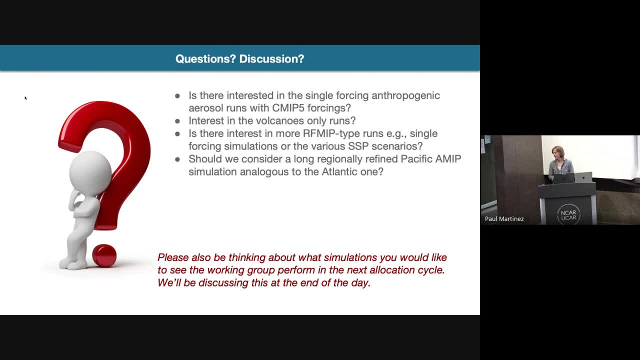 separate out those two, just just get there, and that's the way it's being done. yeah, eventually it would be great to have the paired rounds with a full couple um you talk about like global Goga a-mips forced with ihesp sst, like you're doing. 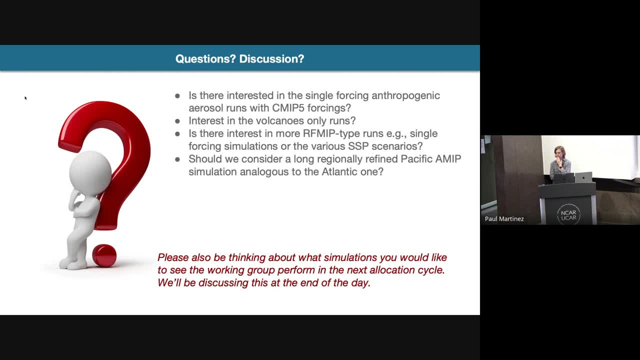 more time. but what if you did global high-res atmosphere elements? so this would be global quarter degree atmosphere forest, where that has ssts. even the Goga runs with the with observe ssts. it's not, it's only five members. so even making that larger could be useful. 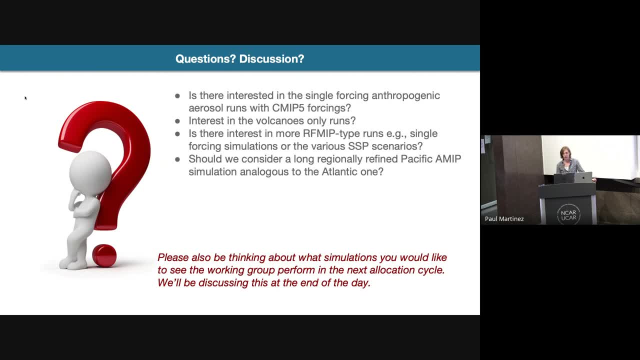 right, there's only a five member cam, five high-res. yeah, I guess they would have not that high res ssts in them, I know. yeah, perhaps after seeing today's results it sounds like perhaps one run with hybrid observed the the optimally interpolated ssts. yeah, so what would be the the primary thing that that would tell us that, beyond what we just 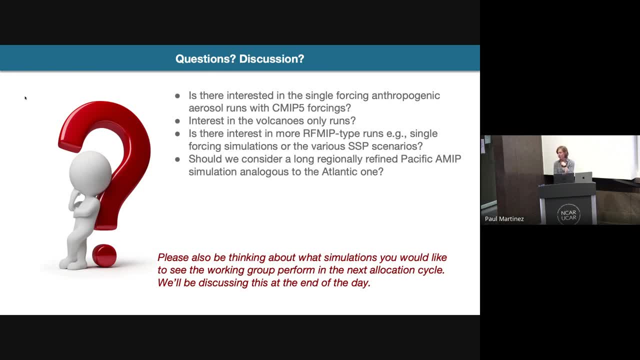 know from the couple of runs would just be boosting the ensemble size or what would be historical, right, yeah so so we're talking about taking couple model ssts. I'm talking about taking high-risk Fossey ssts. oh, okay, yeah, yeah, okay. so it would be like you know historical aim at, but it would have you know some. 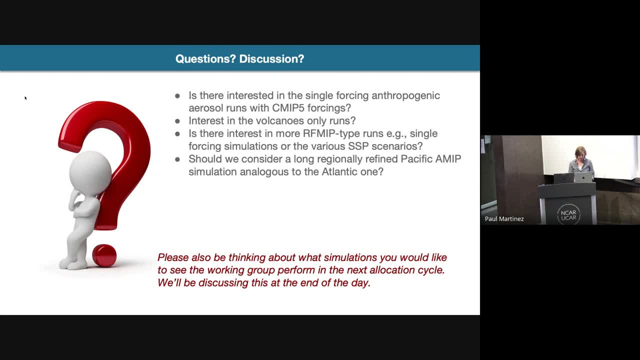 of the high-risk coupling, at least one-way coupling. yeah, that's a good idea. so that would be. that would complement the existing game of simulations because it would have higher resolution. that says the high-risk Fossey. what can the entire resolution be used for the entire 14.. for the high-risk Fossey, right? yeah, the entire 14 resolution is a quarter degree. 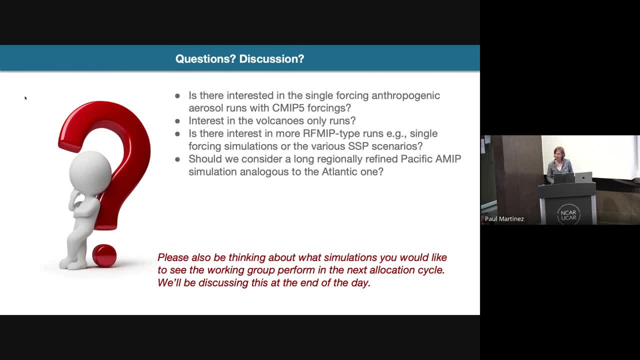 50 kilometers, January 55. but it's a- you know, it's a pretty good global reconstruction of observed sst coming out of that. yeah, a lot of fine skill feature, yeah, and then you could do smoothing experiments off of those. yeah, they don't have to be too long then either if you wanted to spin them up from. 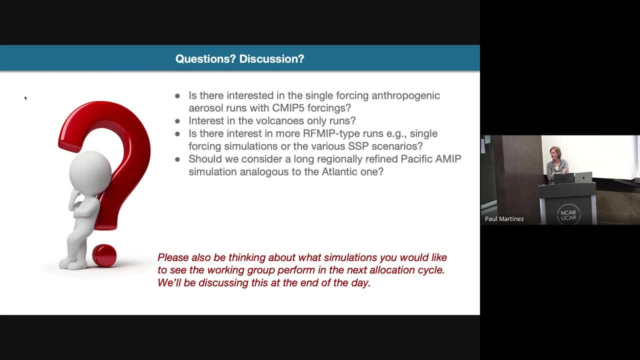 1850. you could just run 1980 to 2020.. yeah, that would be good. so we have a tropical band, regionally refined. I wonder what people think of having the rest more like latitude band refinements, like mid-latitudes and and so forth. yeah, that's, that's not a good idea. 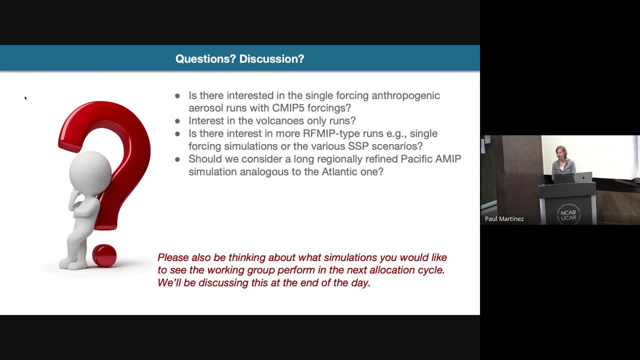 and then a polar cap or something like that. that might be more, uh, that might be a broad interest to wider people than having a specific lat lon area. yeah, so there is work going on with this polar grid which is regionally refined at both poles. adam harrington is running simulations. 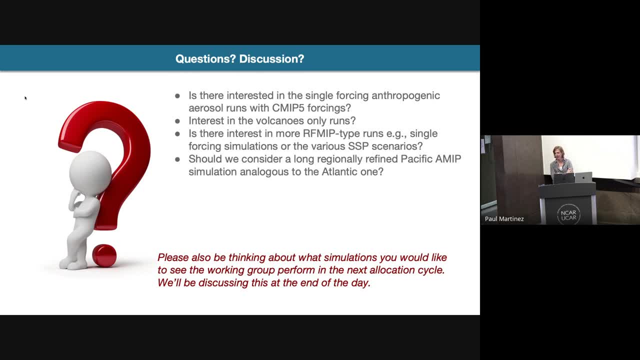 right now- and there were. there are already interesting results that have helped with the development of cam 7, showing all those missing gravity waves in the southern hemisphere, high latitudes at low res. compared to that regional refinement, i think it's going down to a quarter degree at uh at both poles, so i guess the one that would be missing would be a mid-latitude. 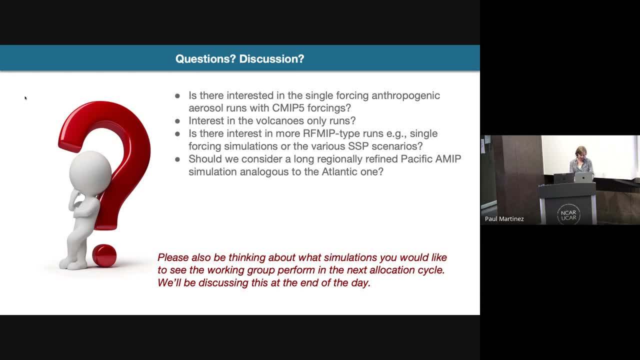 band which would like complete the set. um, oh yeah, i have no idea if this is the right and car working group to to bring this up in, but the the last millennium simulation. um, so with csf1 there was a last millennium ensemble, uh, which was done with cam. 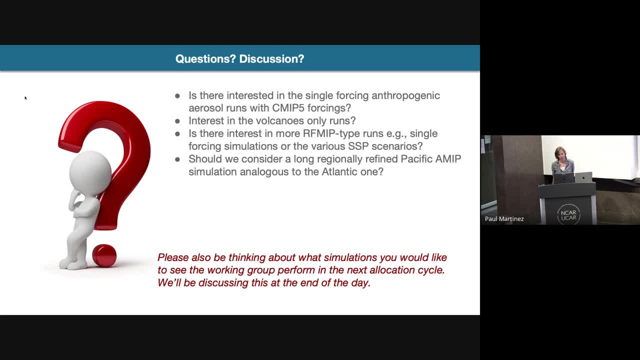 and then, with this simulation that we used, it was a um, it's the whack of middle atmosphere, but it's just the one ensemble member over the last millennium. well, just the one ensemble member over the last millennium, and a perpetual 850 as well, and i guess 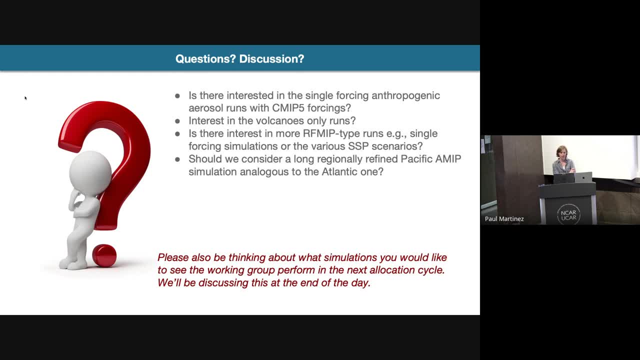 um, just the, the last millennium ensemble at ces, and one was pretty a pretty cool data set. we're sort of obsessed with the, the cesm2 last millennium simulation. we have like 50 ids on what to do with that um, so i guess i was just wondering about, kind of on, whether there were plans. i know that. 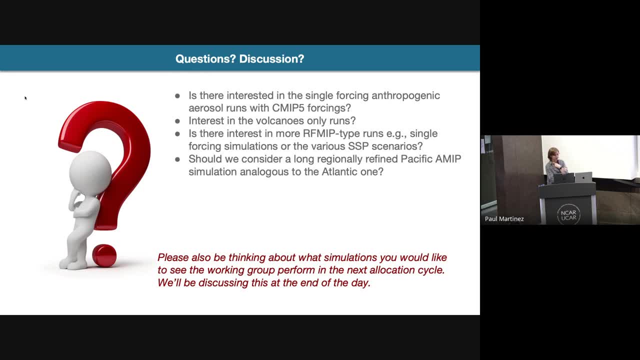 simulation was really recent, whether there were plans to do an ensemble with the new last millennium. yeah, i don't know that. yeah, that would be the paleo climate, okay, but i can take a note of that and, uh, ask them or tell them: that's the life simulation. yeah, we've been emailing with. i guess it's betty. 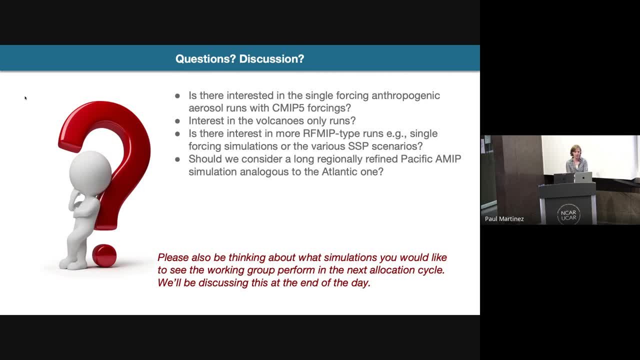 otto bleissner over there. yeah, yeah, yeah, she would. she would be the person that probably would either know whether they're planning to do that or that you would try and persuade, so there's more chance to have him. so, really, august is going to be the time.